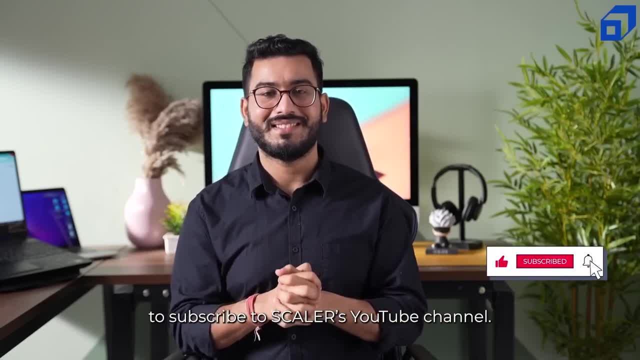 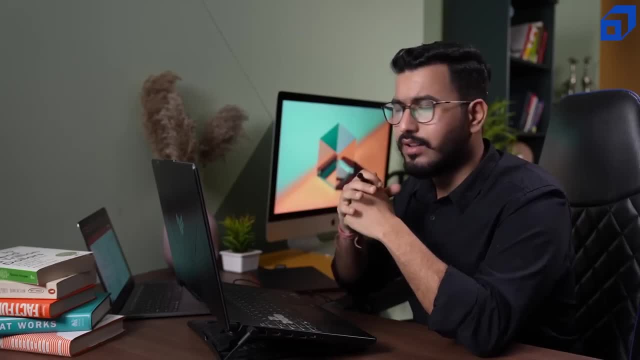 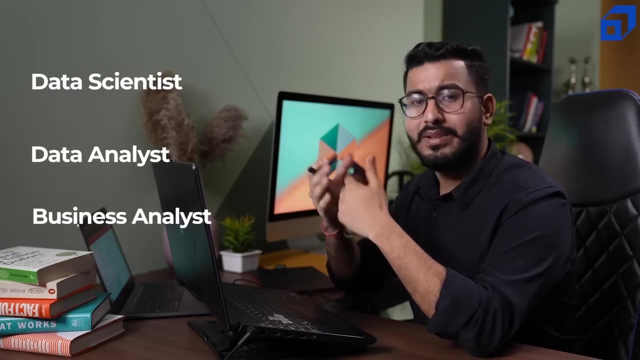 video. don't forget to subscribe to our Scalar's YouTube channel. Let's get started. Let's now understand how much math you need to become a data professional. Now, please remember I am not using the term data scientist or data analyst or business analyst or machine. 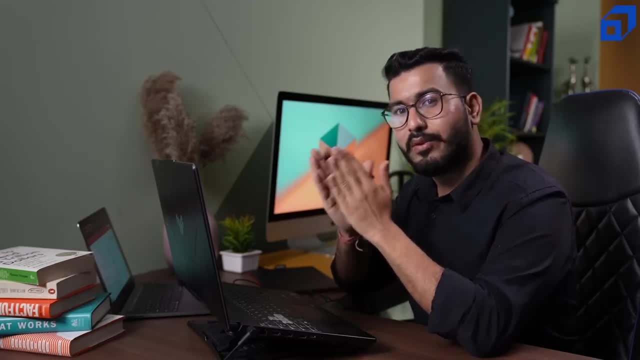 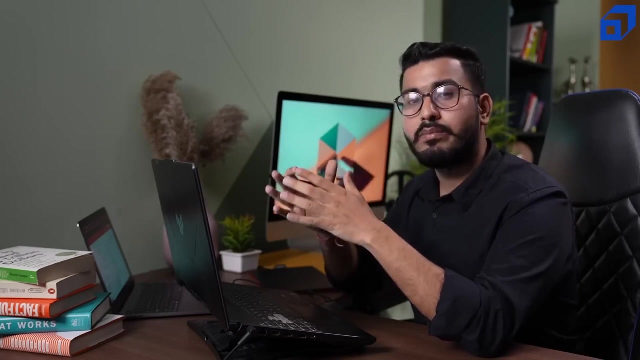 learning engineer because, being a data professional, you need to have certain knowledge of math, And in this particular video, I'll try to explain you how much math, and from which topic, which all subtopics, you need to prepare so that you can be a very good data professional. 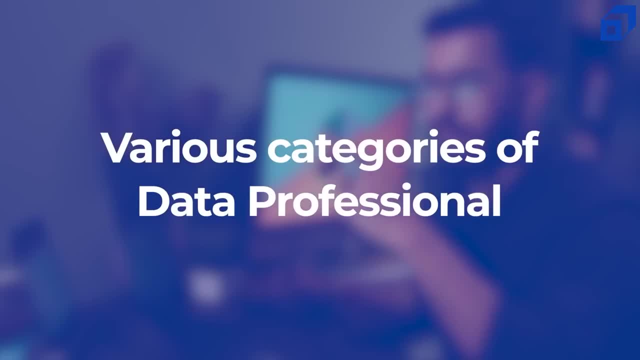 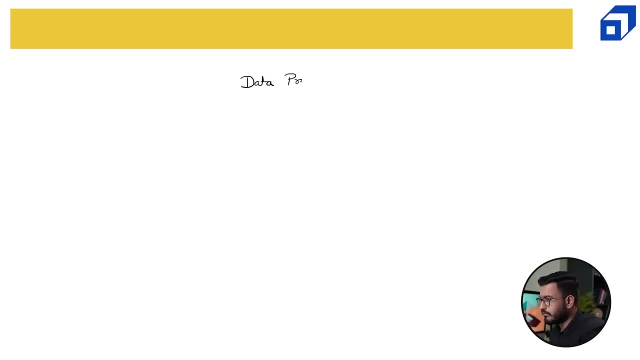 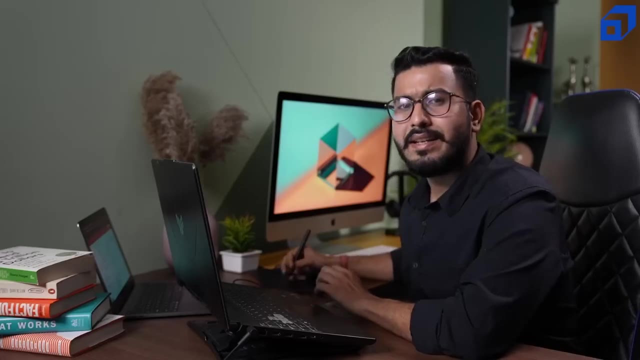 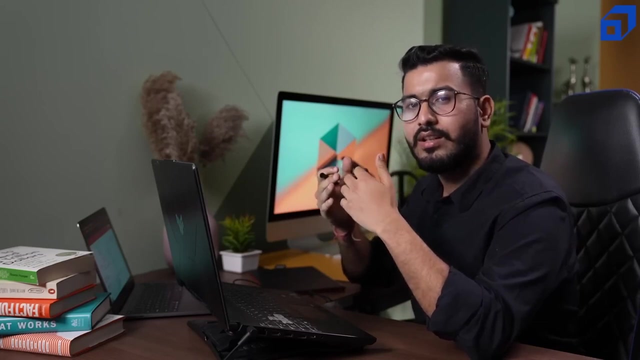 So let's first of all understand the various categories of data professional. If I try to understand how many data professions we have, the very basic and the very starting point. So let's say, if I wanted to be a data professional, the very first thing that I should start with is to be a data analyst. 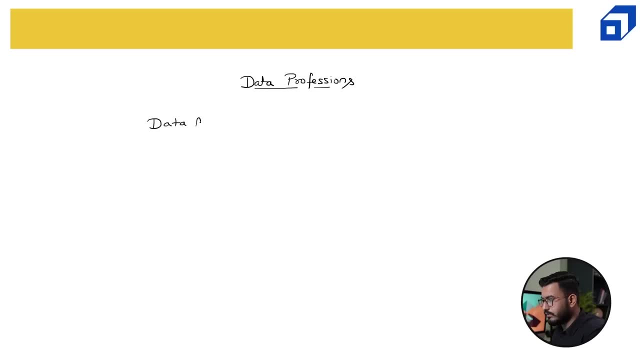 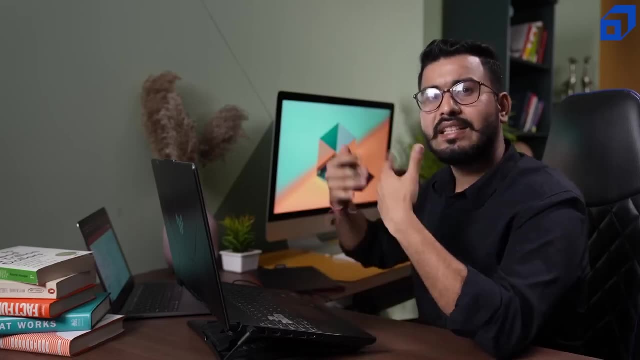 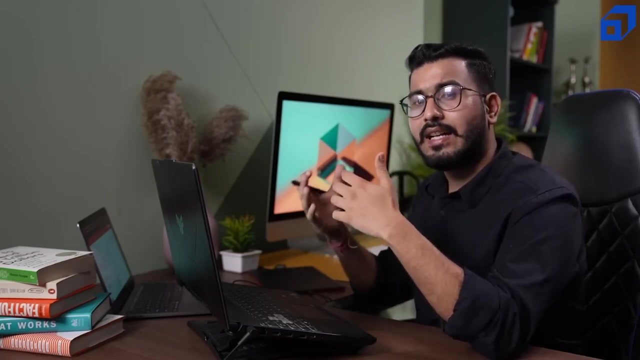 So the very first step is data analyst. A particular person can become a business analyst. So let's say I'm working as a data analyst at Amazon. Now, once I get the knowledge of business, I can start interacting with the business heads, business managers, stack holders, to. 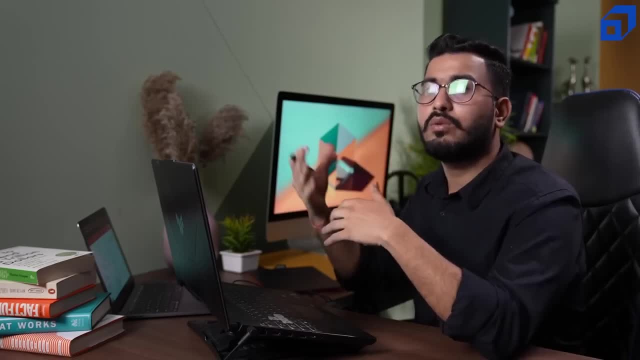 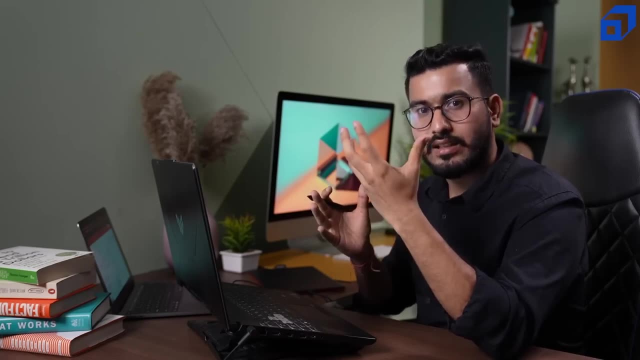 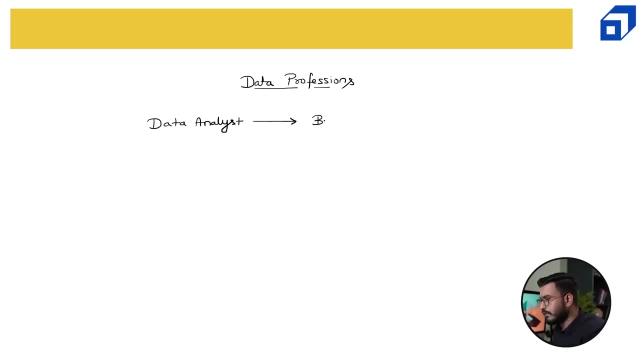 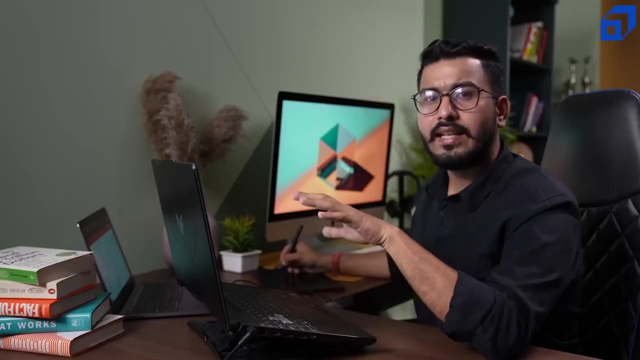 apply the logic and the learning from the data to the business, And that is what business analysts do: Get or extract the insights from the data and try to resolve the business problem. So that is business analyst, While on the other hand, the people who are data analysts- they are more like not working. 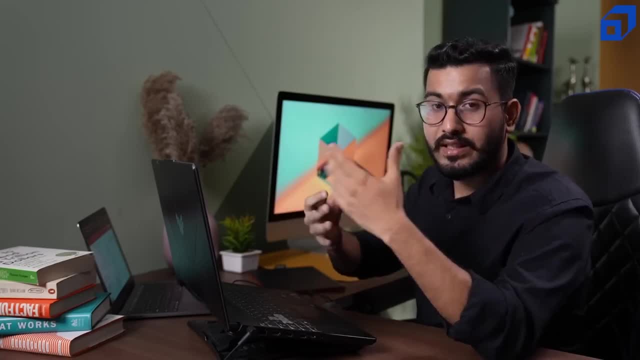 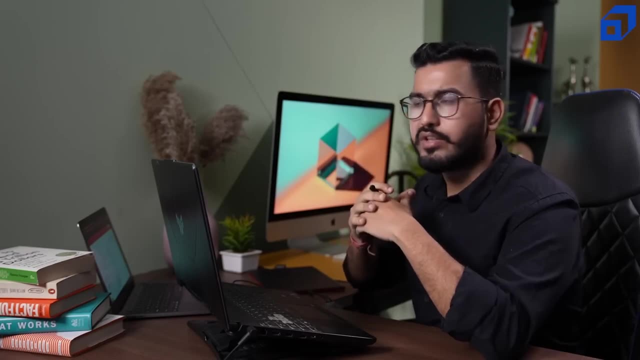 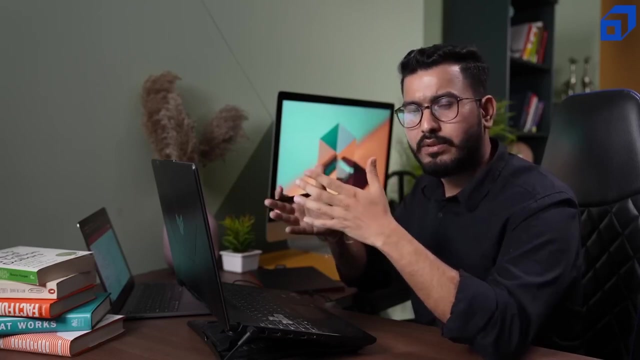 on the analysis side, but they are trying to interact with the data. So they are the first point contact of all the data requirements. Let's say I wanted to fetch my top 10 customers. Now the person data analyst working in your company would be the best person to return you the top 10 customers. But if I have to, 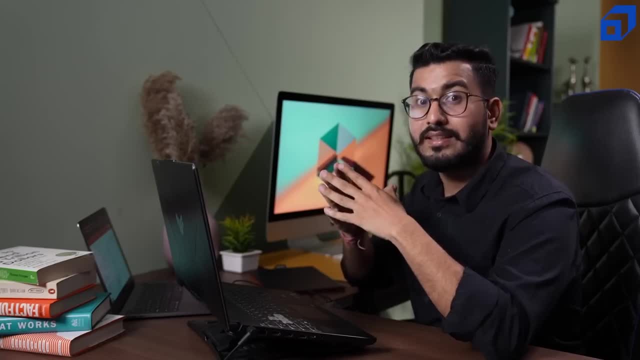 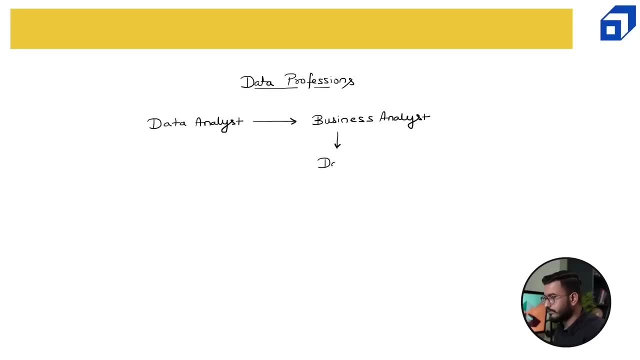 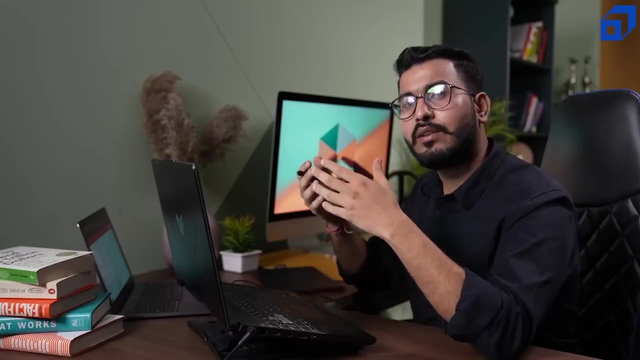 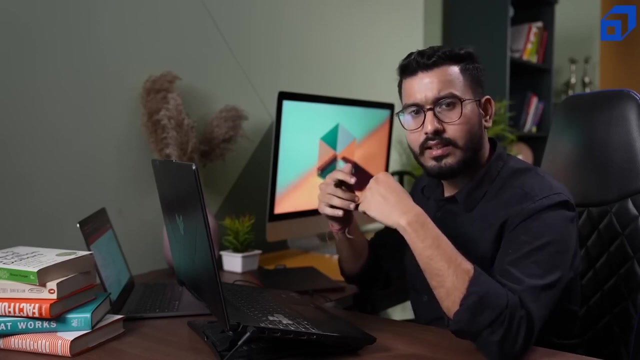 take a business decision. on top of it, you have to reach out to the business analyst. The next step in this ladder is being a data scientist. Now, data scientist is that person who tried to utilize the data and come up with some complex algorithms, complex models. 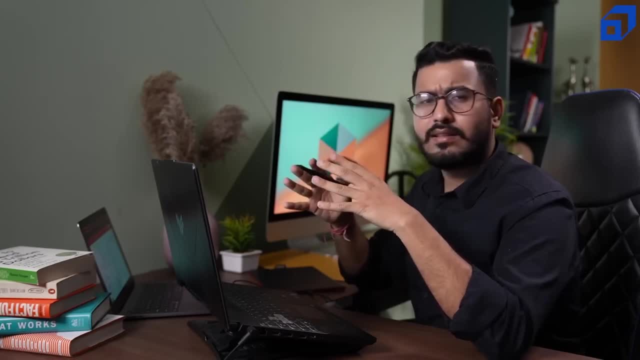 that can start predicting. So, business analyst, or being a business analyst, you are trying to resolve problem by taking decisions based on the insights that you have derived from the data. But data scientists try to forecast, try to predict what can happen, how we can enhance. 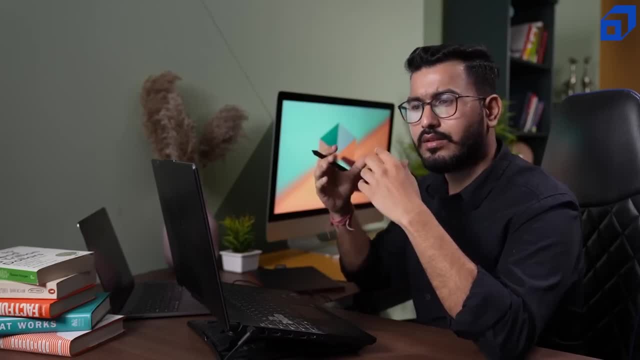 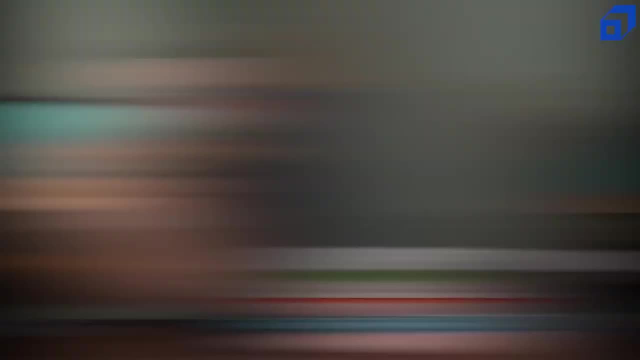 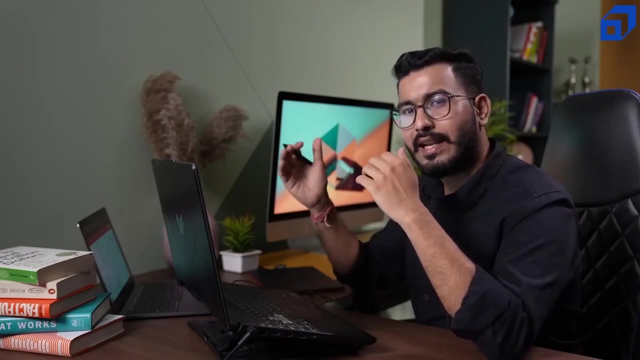 the performance of a particular business and various others. So adding more complexity to your current work is going to make you a data scientist. Please remember: with each step that you climb up in this ladder, you are adding more and more business knowledge to your current knowledge of business. So the more knowledge of business, 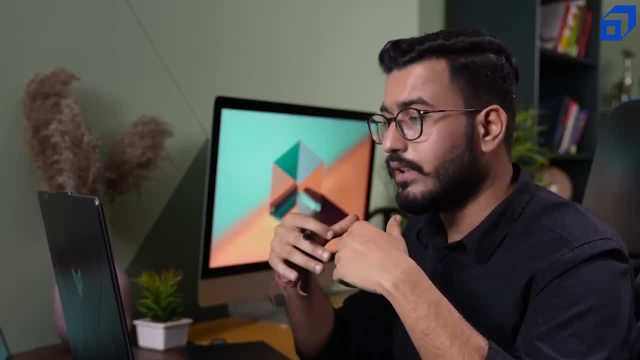 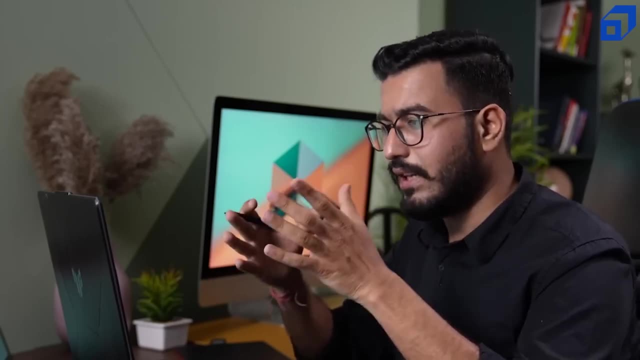 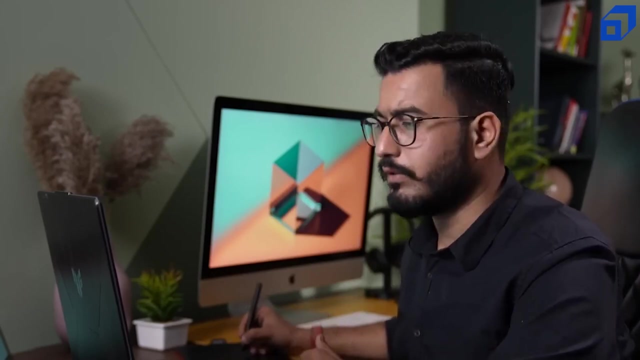 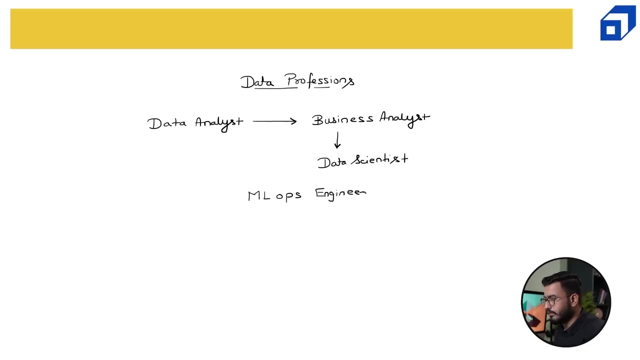 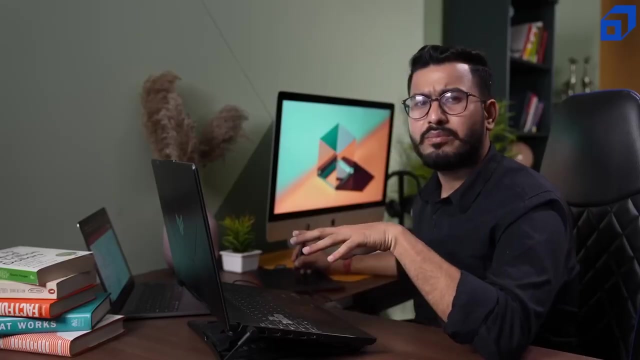 and the more familiar you get with the problem solving, it will help you to become a more profound and a more successful business. Thank you, Thank you so much. find out the position of AI manager, and we have multiple other positions that that you can find. 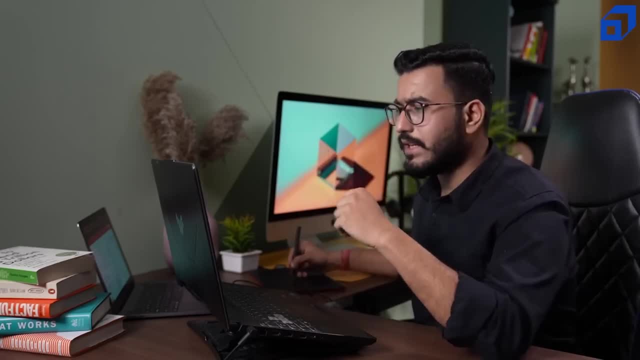 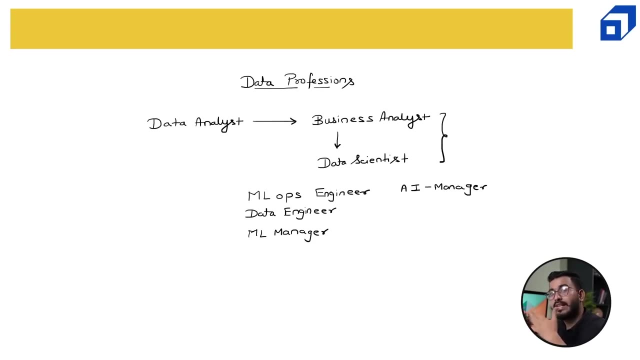 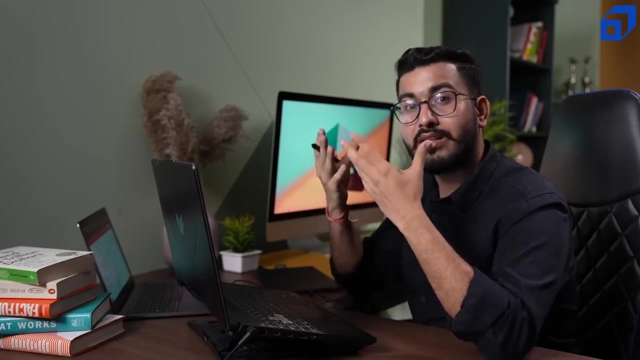 out right now in the market, but according to me, these are the three basic positions with which you can start or with which you can enter into this data world. coming to the actual question, and for which you are watching this video, is how much math you need to become a data professional. 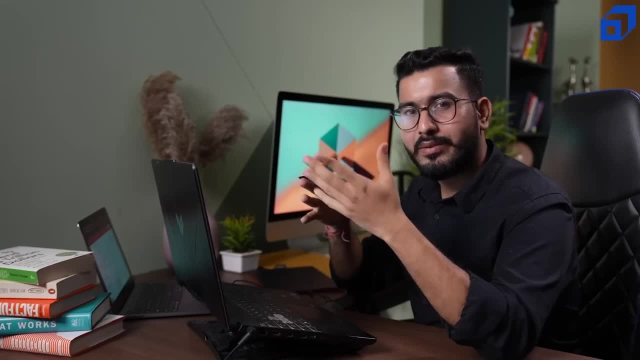 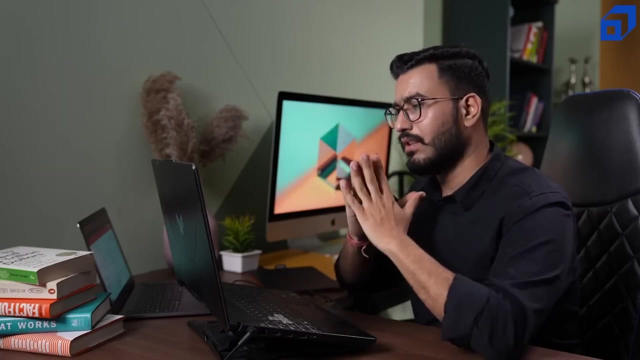 math is very important and those of you who think that, okay, I don't need to learn math, I can become a data scientist or a data analyst just by learning python, sql, just by learning some machine learning algorithms: my friend, that is not going to happen, even if you want to. 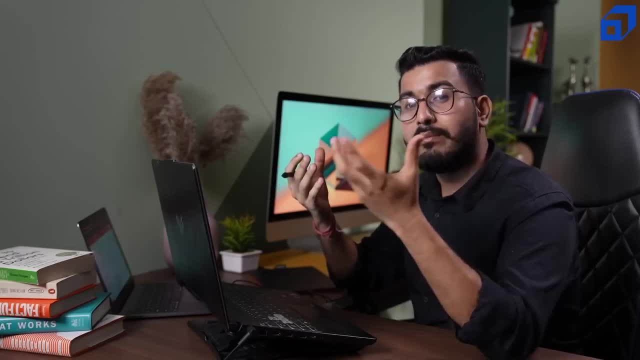 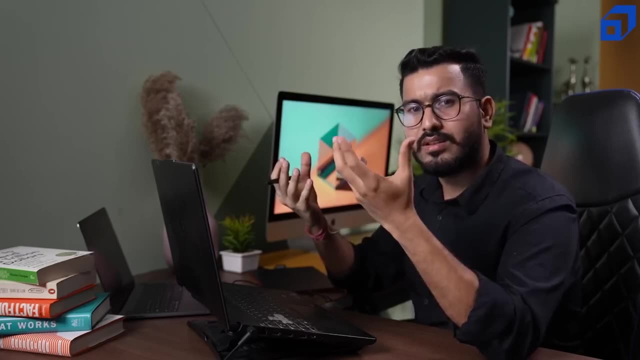 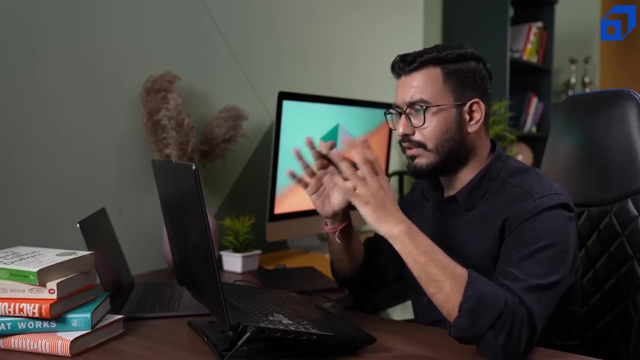 learn any machine learning algorithm. you need maths because every machine learning algorithm is a mathematical model. it is running on some numbers, because data is all numbers and wherever there is numbers, there is math, so you need math. so let's try to understand how much math and which all. 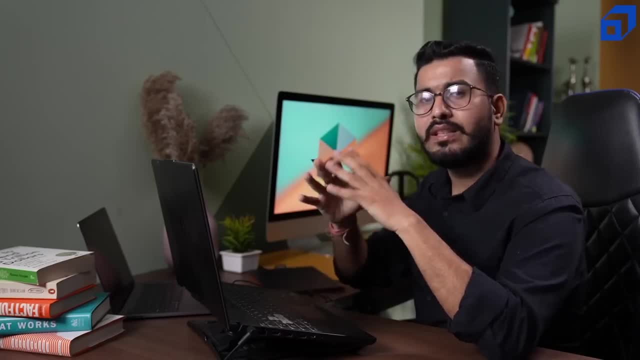 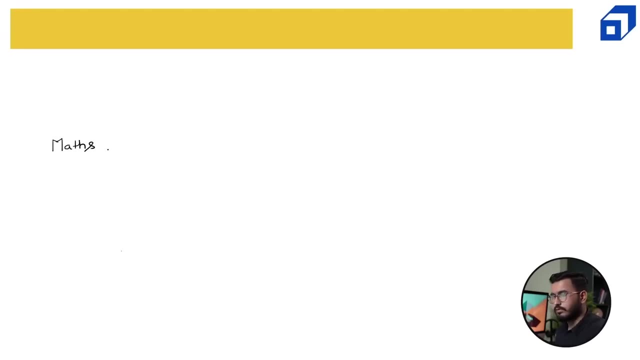 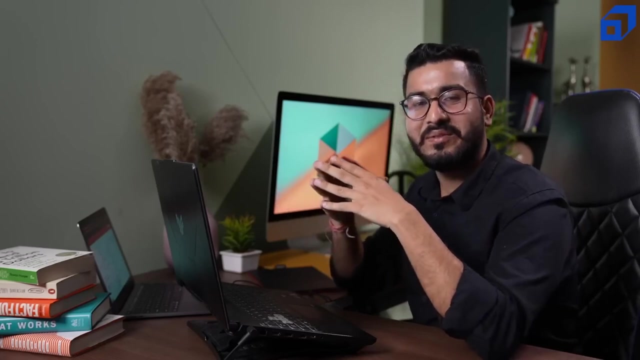 topics i need to learn. i'll help you with a flow chart. so, when we talk about maths, there are four important topics. number one: statistics. number second: linear algebra. number third: calculus. number fourth: discrete mathematics. now, if you, if you are listening to these terms for the very first time, don't worry, because 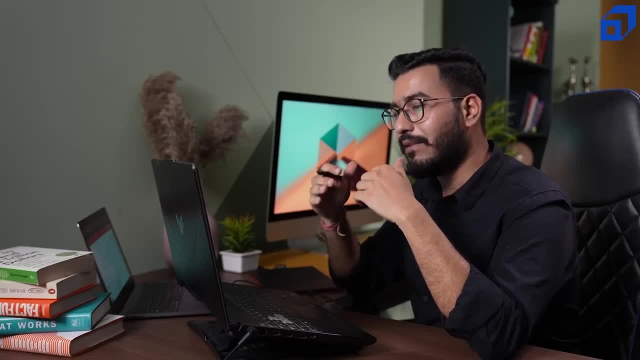 we are going to first of all look into the pipeline and then i will also be taking one, one example, so that it can help you to understand that. okay, this is not rocket science. this is something which you already know, but you have to just brush up your 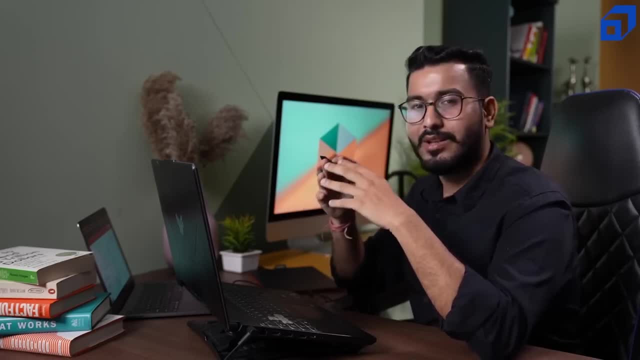 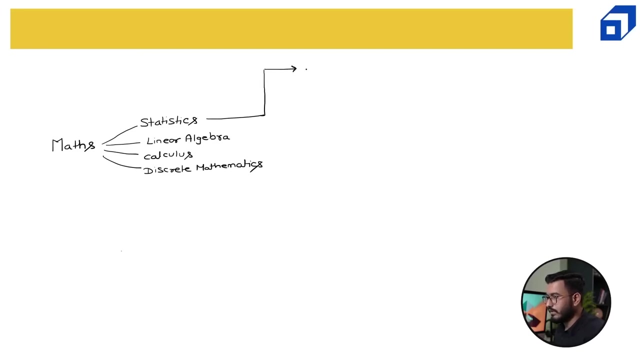 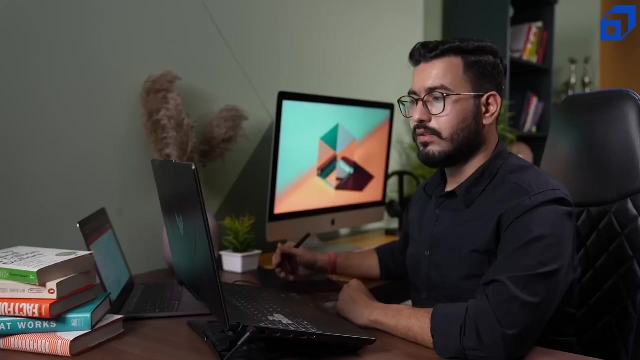 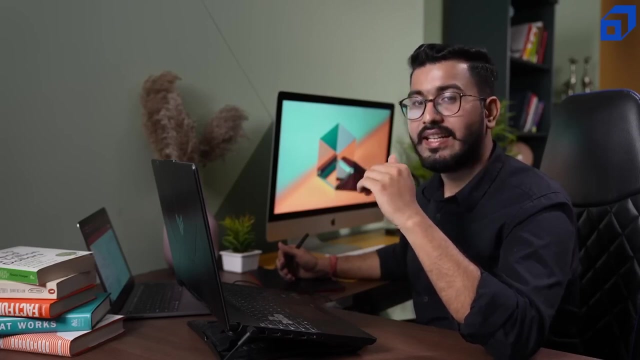 basic maths to understand these high terms, or maybe high words. so statistics is further divided into various subcategories. let's understand: we have descriptive, then we have inferential, then we have hypothesis, which is hypothesis testing, followed by regression and finally time series. so these are the sub topics that a particular data professional has to be clear with when 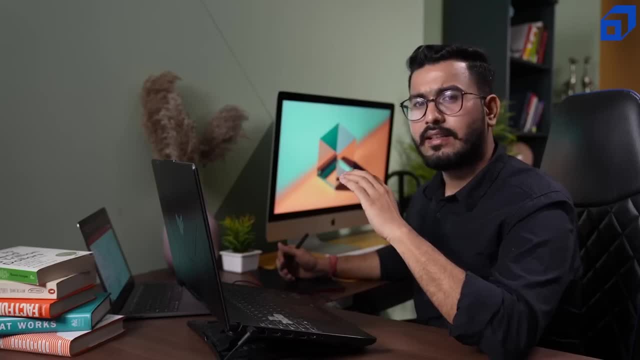 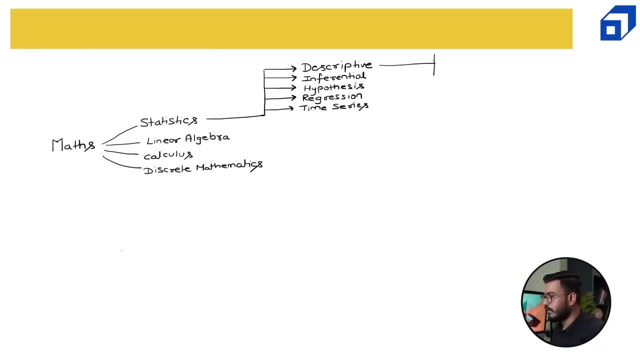 it comes to statistics now, descriptive statistics, which is the very basic statistics, or maybe all of you already know about it. it is the very first thing. so the first thing- if you are familiar with statistics today, you already know what statistics means- gives you a basic idea of what a statistic. 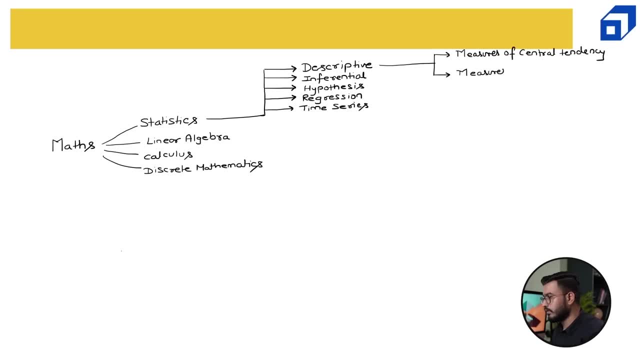 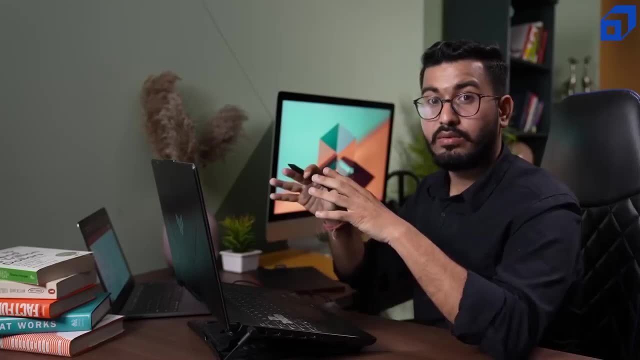 names can mean so for a statistic like E, g, x, g or y, z and hol moon or whatever fishing equation. now, for example, we will have two categories. key question numbers are main and secondary. try to take examples from both: measures of central tendency and measures of dispersion. 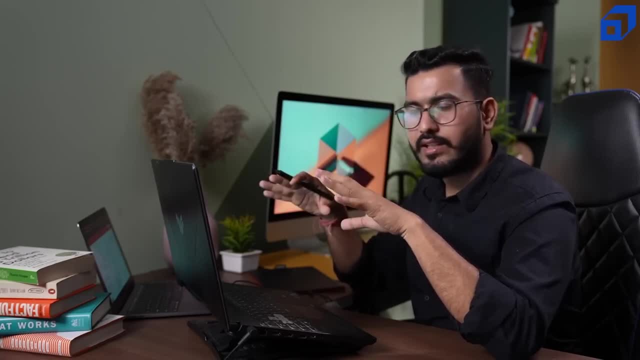 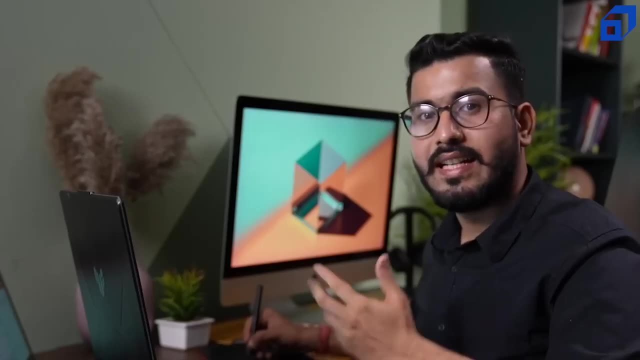 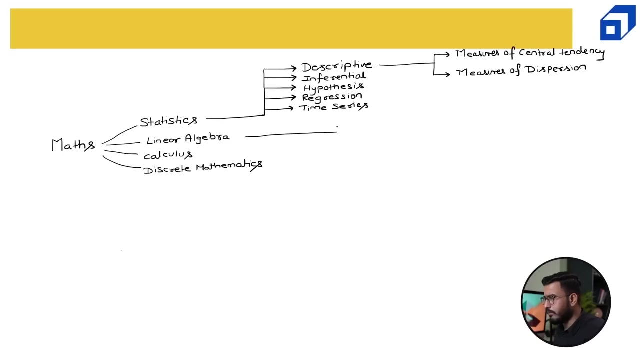 But first of all, let's try to complete this particular tree so that you can have a clear idea regarding how much math you need from all the subtopics. Now let's focus on linear algebra. Linear algebra starts with the concept of matrices and vectors, So number one, matrices. 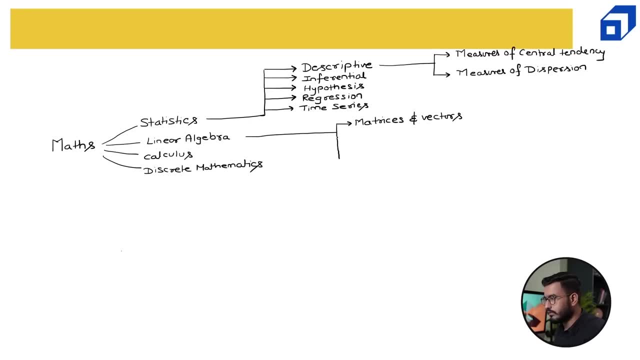 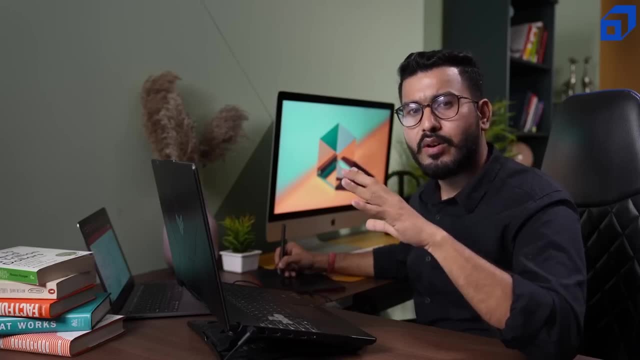 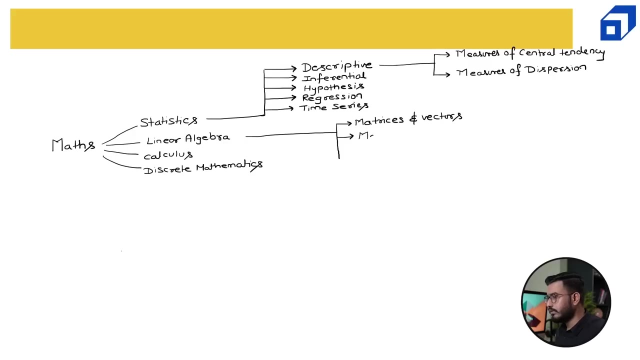 and vectors, followed by matrix operations. When we talk about matrices and vectors, it is really important that you are clear with how to operate on matrix. So matrix operations, This is followed by linear equation and finally, optimization. Now when we come to calculus Under calculus, 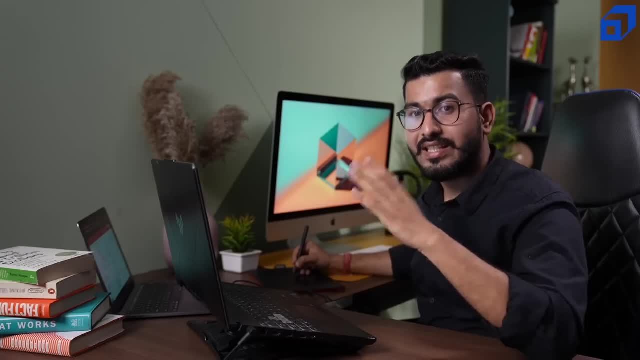 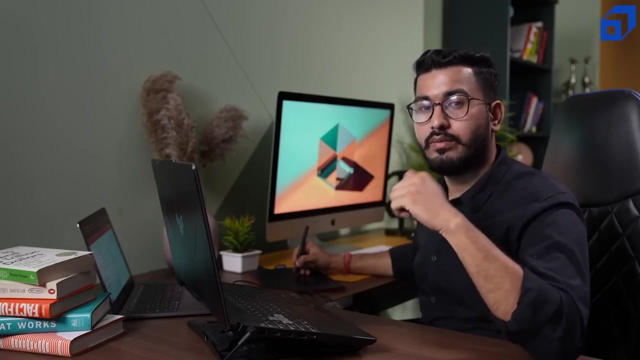 we have topics like differentiation and multiplication. You guys must have learnt about calculus in your 11th class or 12th class, But calculus is also a very important topic when it comes to machine learning. We use calculus. we use a very high amount of calculus when it comes 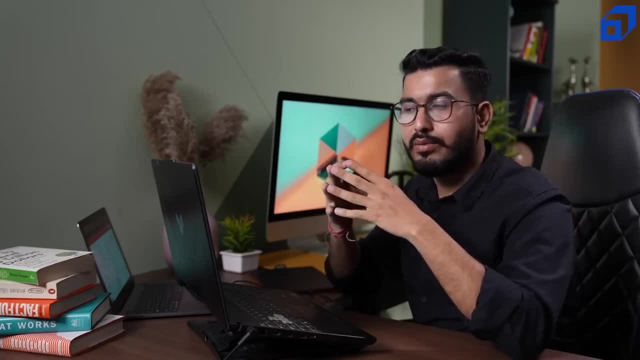 to neural network. Now, those of you who wanted to use, let's say, those of you who are looking to use a machine learning tool, you can use a machine learning tool. You can use a machine learning tool to use neural networks to detect what is the content of the image, Or maybe, 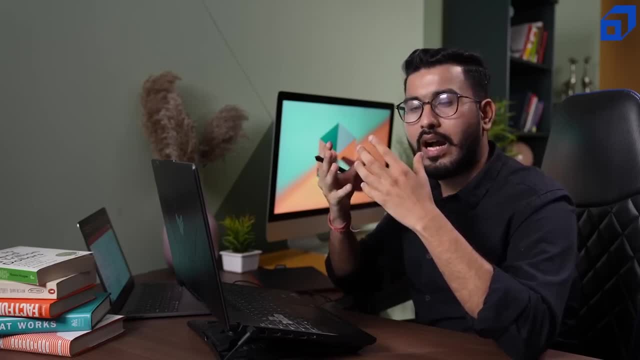 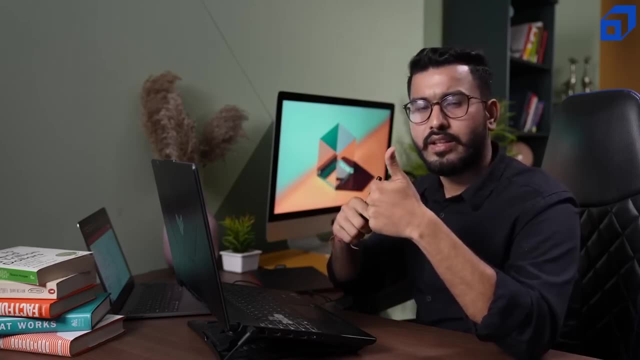 you wanted to use neural networks to find out how each lecture. So let's say, if I am doing something like this, Now, what is the meaning of this? So we use image processing, We use computer vision for this, And while we are working on these applications, we use 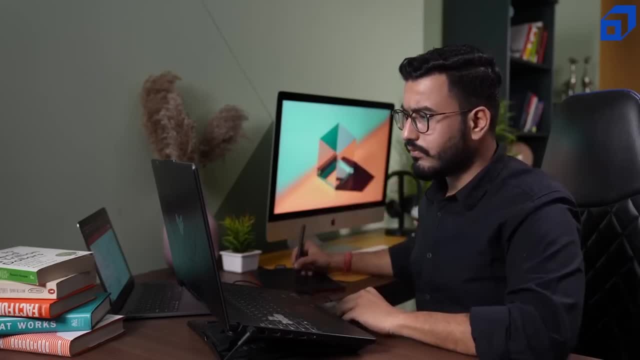 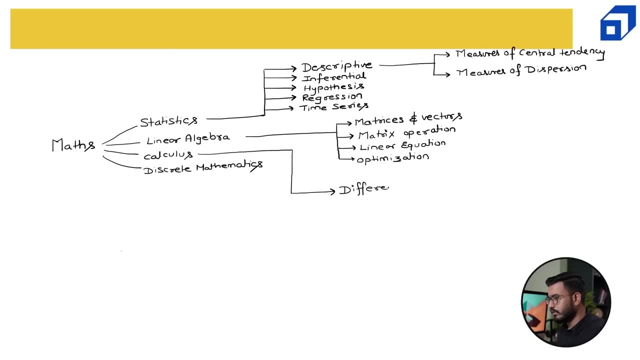 high amount of calculus. So, within calculus, we need to be clear with differential, which is basically differentiation, as well as partial differentiation. We also need to be clear with the optimization of the visualization technique that comes under calculus. Now, finally, is discrete mathematics. In discrete mathematics, we have the very utilized or. 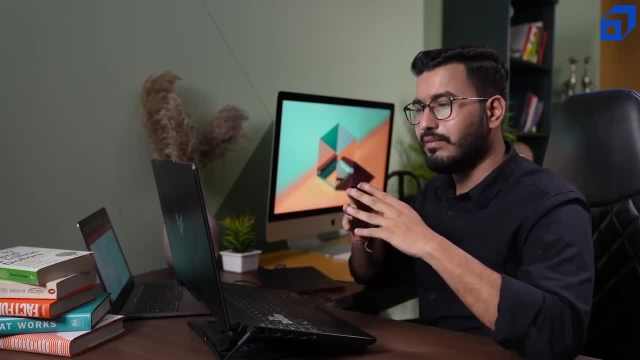 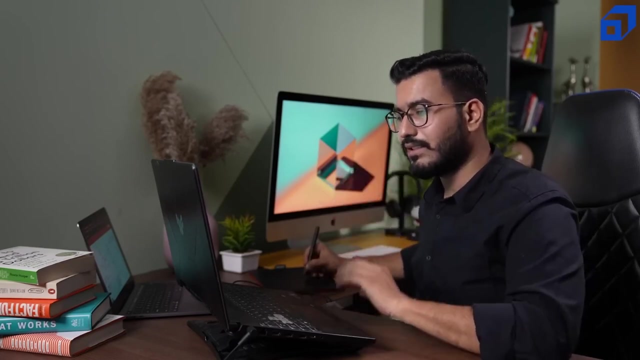 maybe the most important topic when it comes to playing with numbers. If you wanted to play with numbers, discrete mathematics is something that you need to be clear with And you need to be confident with. The reason is, discrete mathematics consists of topics like 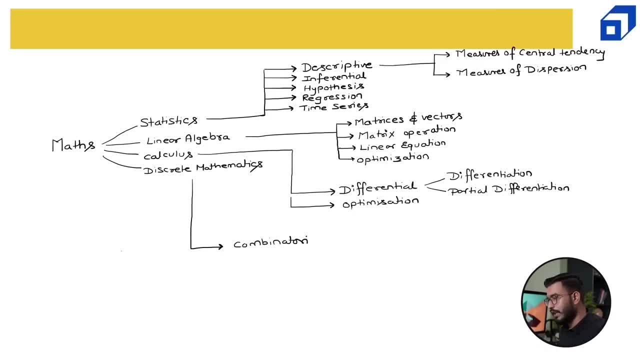 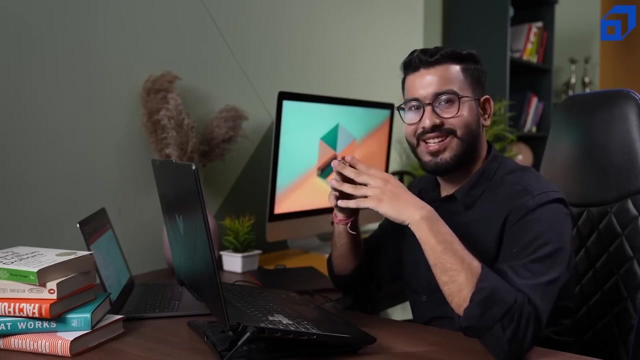 Combinatronics, which is permutation and combination. The next thing is graph theory, Followed by probability theory And finally, set theory. This is everything, Like those of you who are thinking that, okay, I can become a data scientist just by mugging up. 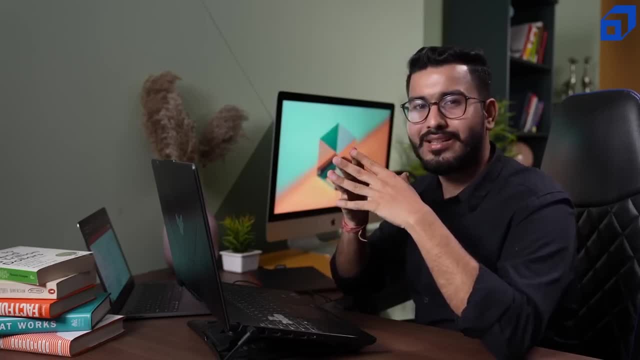 or maybe just by having a very good coding knowledge, Having some very good knowledge about various algorithms and how to apply those algorithms in Python. Uh, this is the reality, This much math you need to be aware about so that you can become a very strong data professional. Now let's try to understand each component. 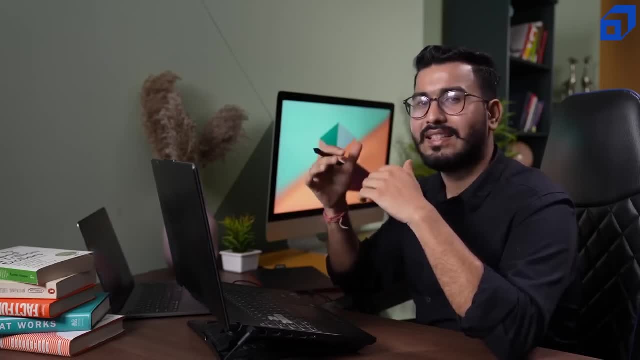 Like, when I talk about descriptive statistics, what exactly is it? When I talk about matrix, what is that? When I talk about differentiation, what is that? So I I'll take an example from each of this category so that you can get a little sense about what. 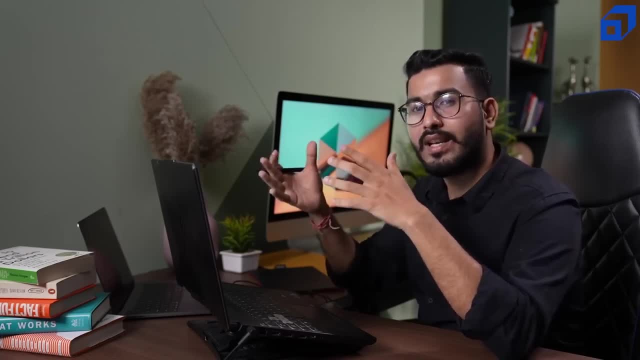 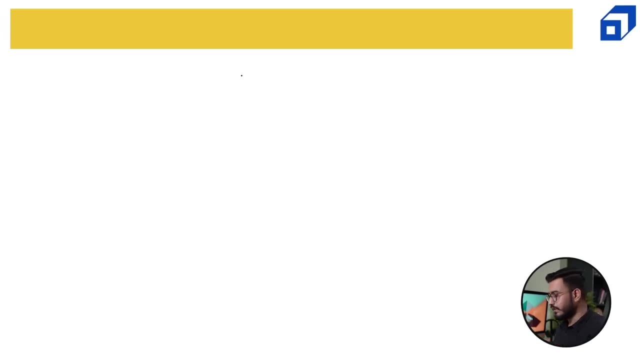 exactly you will be learning if you take one particular topic. So let's understand. Now let's start with measures of central tendency, which is basically the part of descriptive statistics. You guys already know about it, but let me just help you with the basic understanding. 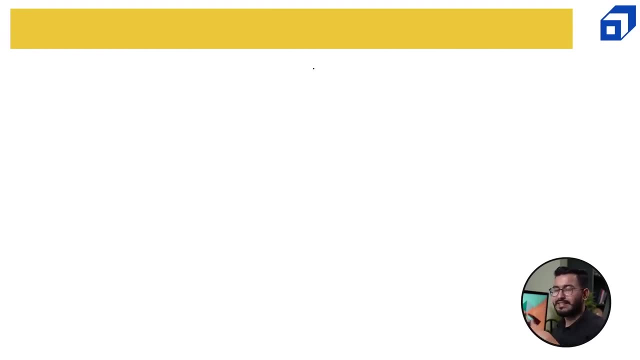 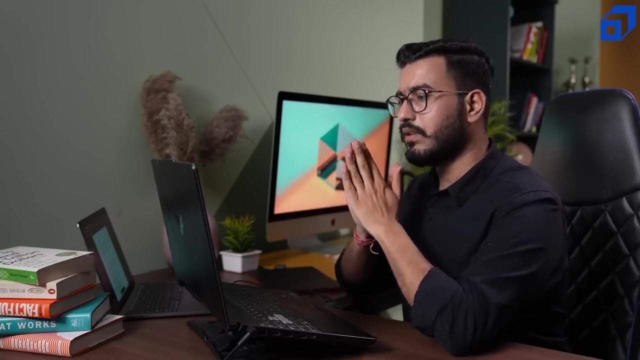 of it so that you can start your journey in descriptive statistics and you can enjoy it. So, descriptive stats, and the very first topic is measures of central tendency. Now, measures of central tendency is something that can help you to find out the center point of a data. 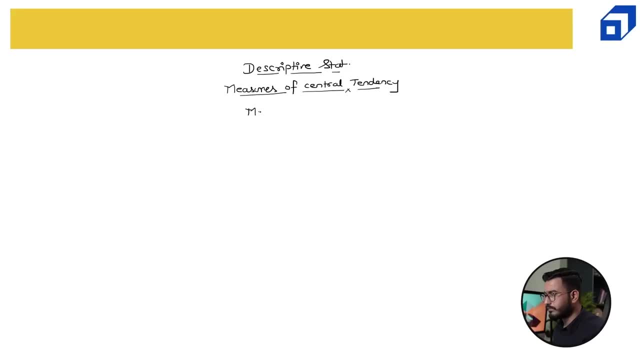 Measures of central tendency are basically your mean, median and mode. Mean is also known as average. Let's try to understand it. Okay, Let's say I'm having the data regarding, uh, let's say, the marketing budget, or let's. 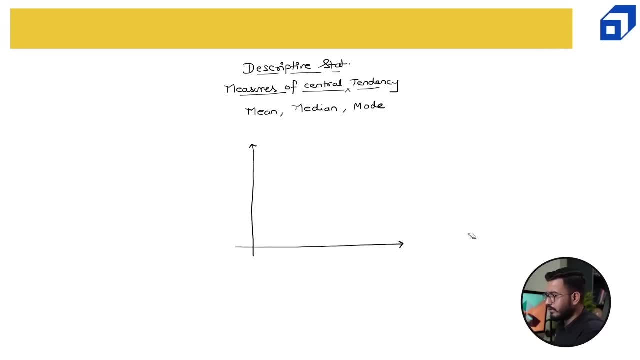 change the example. Let's make it more realistic and something which you guys can easily understand. Let's say: this is my years of experience. Okay, And in y-axis I'm having salary. Now let's create some data points. First of all, let's define the axis. 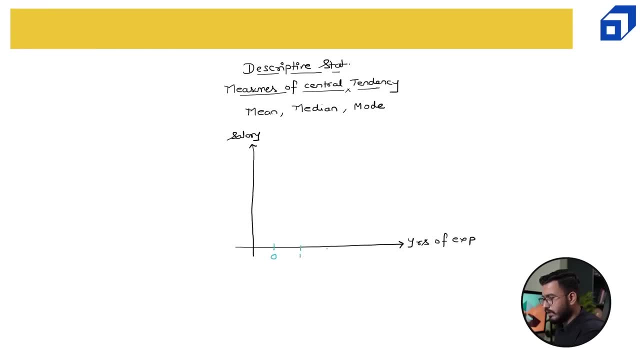 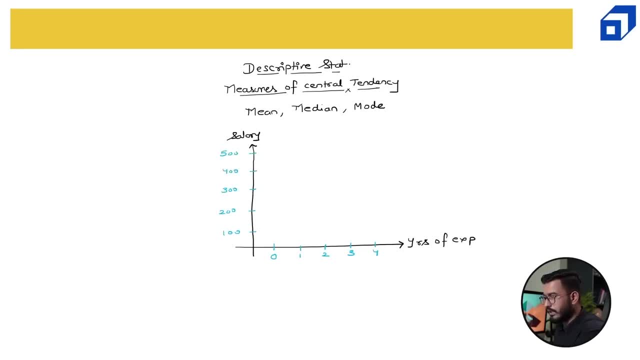 400, 500.. Now let's point or let's create some data points. So for um zero, zero years of experience, I'm having a data point over here for one. I'm having, let's say, a data point over here for two. I'm having over here three. then 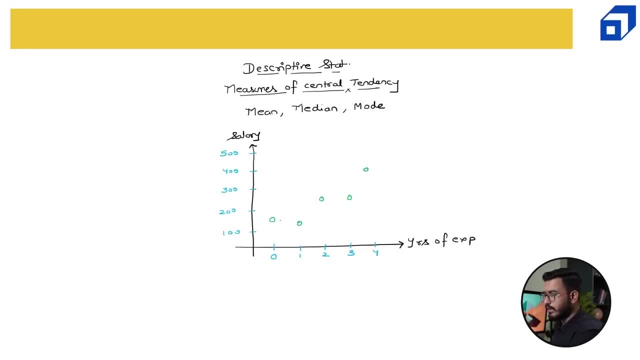 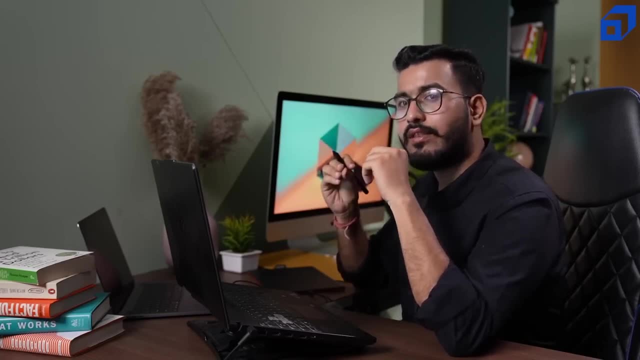 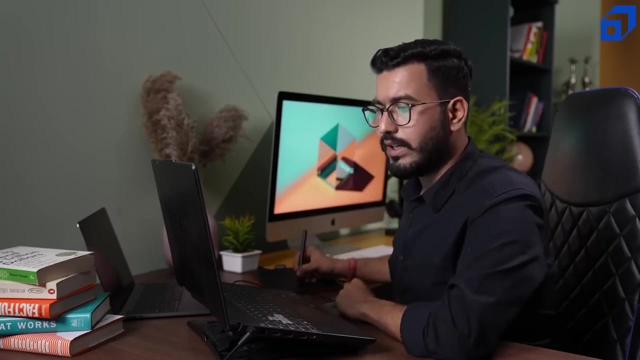 four. Now this is the data that I'm having. If I try to find out a middle point, Okay, That can help me to get one value that represents this complete data- Then that value is known as mean- how to calculate mean or average. 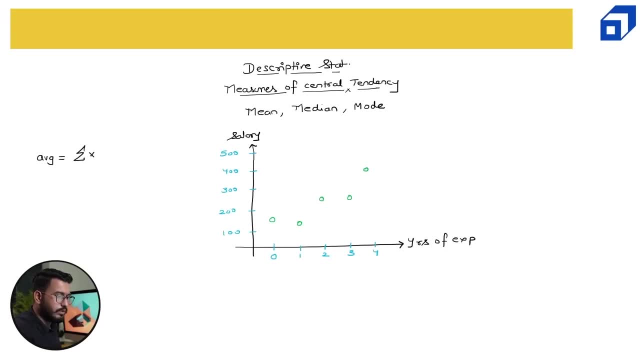 It is given as some of all the observations divided by total number of number of observations. So here I'm having observations like I'm having. let's say this is 150.. Okay, I'm having another one which is below this, So let's say this is 110 comma. 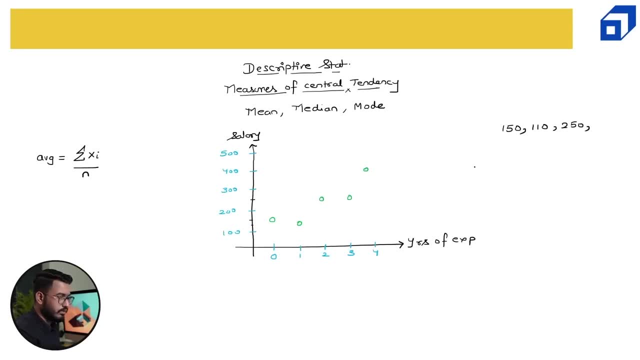 This is, let's say, two 50 comma. Let's say this one is again two 50, and then we have a point 400.. So these are my data points. Let's add them. So is equal to one 50 plus one 10.. 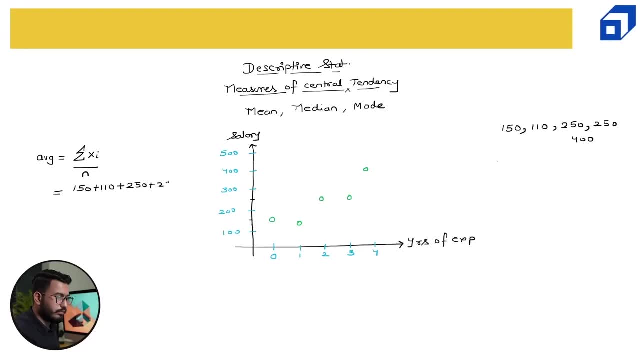 Plus two, 50 plus two, 50 plus 400, divided by one, two, three, four, five, So we'll get 500, 900, 1000, 1000, 200.. So this will come out to be one, one, six, zero. 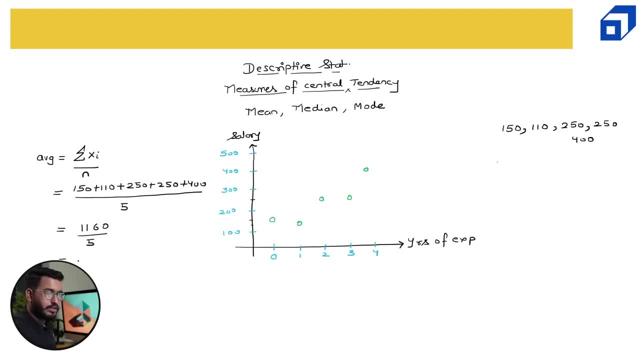 We have to divide it by five And if you do the calculation, it will be two 32.. Now, if I try to point this particular data in my graph, so two 32 would be, uh, less than 50.. So somewhere around, somewhere around here, and I create a line for this. 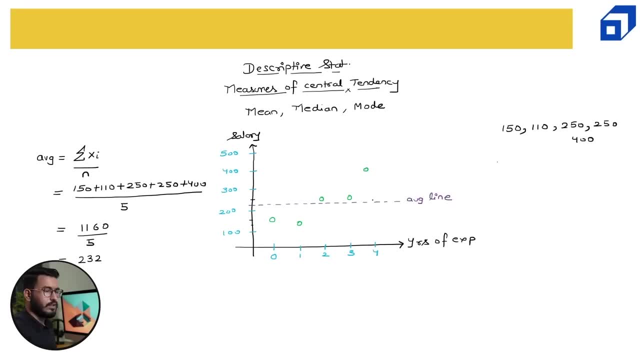 Now, this is my average line. So here you can see that it is basically the center point of the data where you can see that There are approximately half data points above it, half data points below this. So average defines the center of the data. 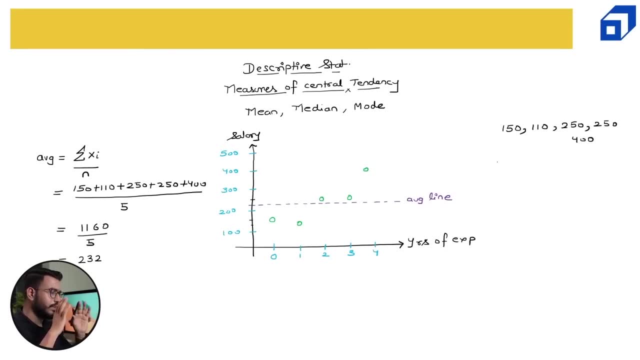 And that is the reason it is a part of measures of central tendency. But there is one problem with average. Average is influenced by outliers. Now, what is outlier? Let's say I'm having one particular employee whose salary is around uh, so the person? 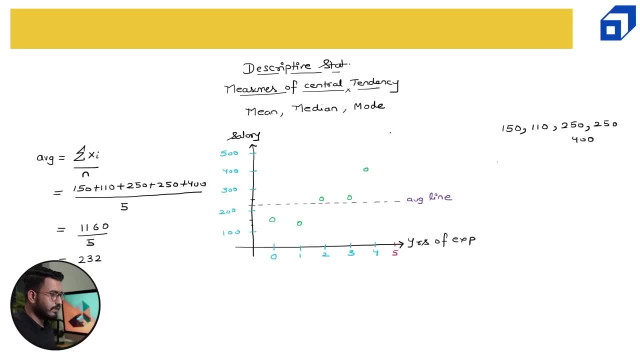 is having experience of five years, but the salary is somewhere around here And this salary is, let's say, uh, 2000, with very less years. the person is still having a salary of 2000, while other people are having a salary in a range of hundred to 500 maximum. 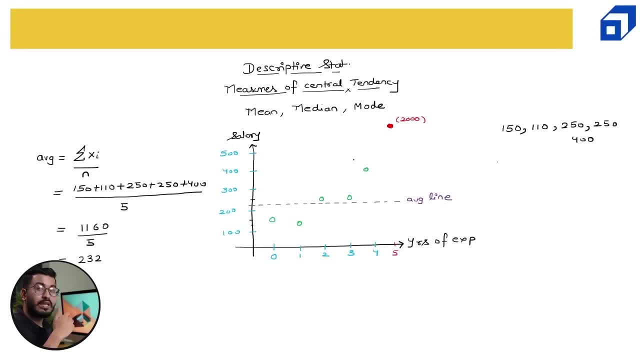 is 400.. Now what will happen if I can try to calculate the average? So now the data points would be One, 50 plus one, 10 plus two, 50 plus two, 50 plus 400 plus 2000 divided by six. 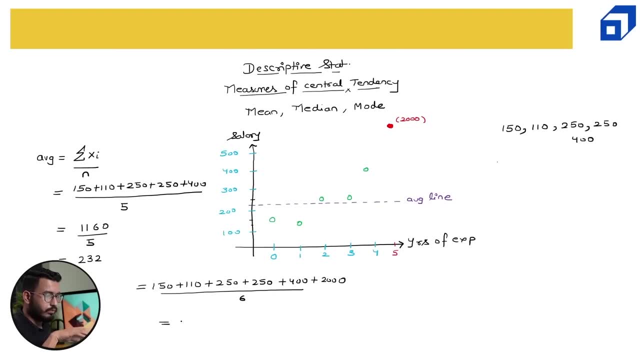 So previously the summation was 100 and, sorry, one, one, six, zero. I will add 2000 to this to divide it by six. So this will be 3,160 divided by six. So you will get five, 26 point something. 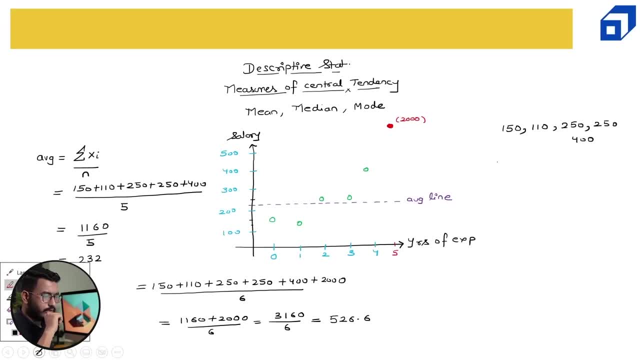 Now here you can see that just because of this particular number, which we call it as outlier, your average salary has been shifted to somewhere over here, And this is not the center point. This is your average line Without Outlier And this is not the center of the data. 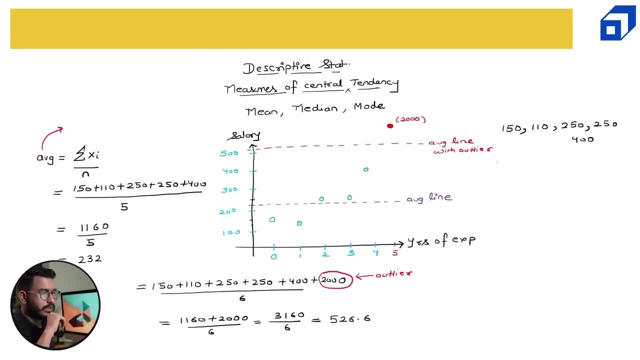 So that is the problem with average. your average, as a measure of central tendency, is influenced by outlier, influenced by outliers. Now, how to get rid of them? That is the reason we have median. If I try to calculate the median with the same data, 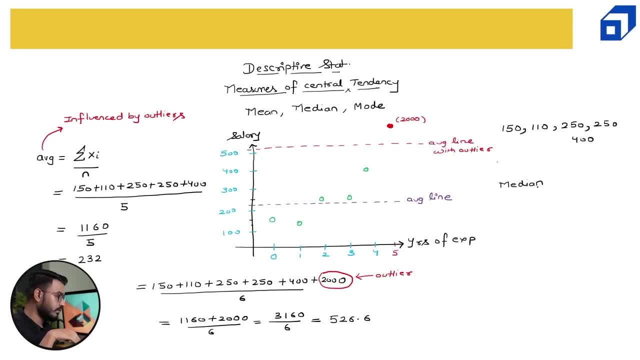 So median, median is basically the center point or central point in the data, No matter if you have outliers, if you do not have outlet, it will be always center. So when I say center, let's say this is zero, this is hundred. 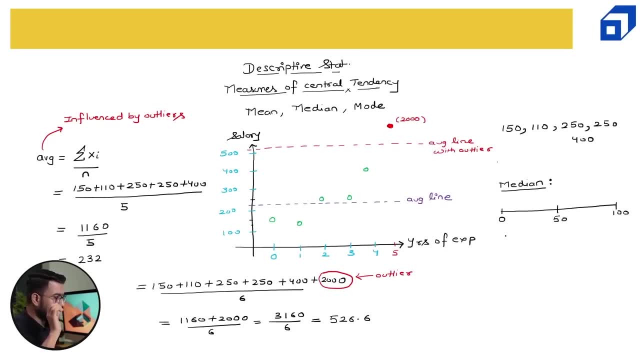 So your center will be 50. So you're 50% of the data. Okay, So your median will be below this point- 50% data- while your rest 50% will be above this point- 50% data. 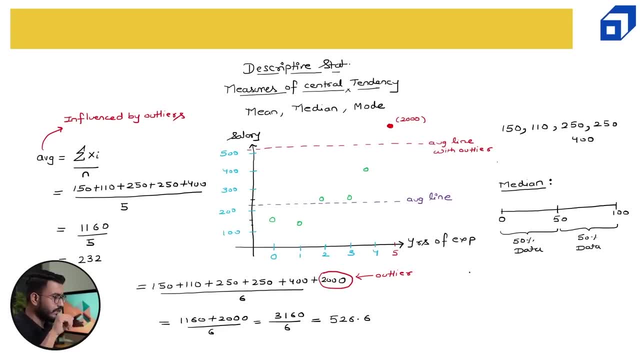 That is what your median is. If I have to find the median for any given data, a step number one is sort the data or order the data in ascending order. So order the data in ascending order. Okay, Okay, Okay, Okay. 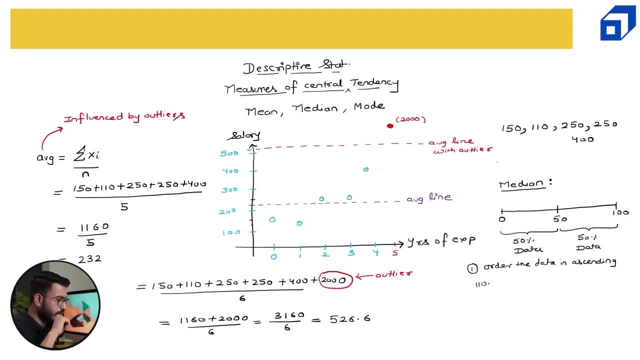 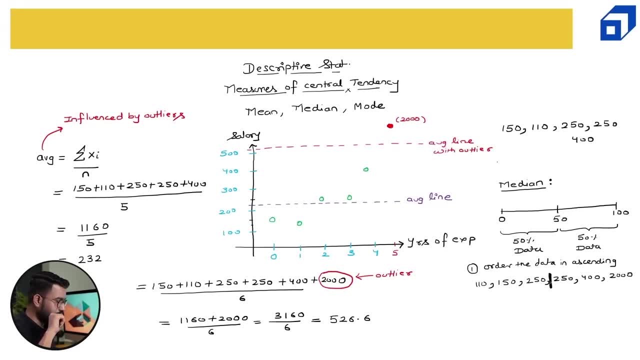 The middle value is is basically this: Because below this point, I'm having So three data points, which is 50% of my data about this point. I'm having three data points, which is 50%, But how to find out this middle value? 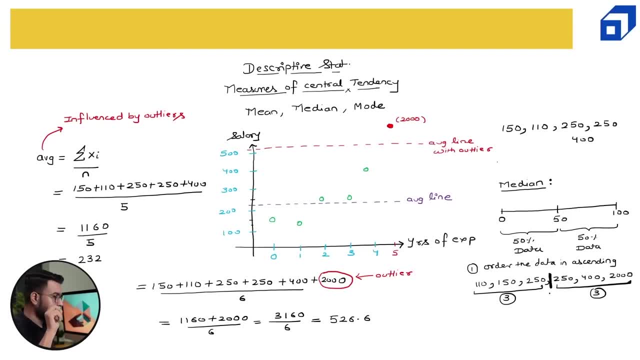 If my data is having odd number of data points, I'll directly get the middle value. But if you have, if you are having even number, that is simply the average of these two values. Average So two 50 plus two 50 divided by two, you will again get two- 50.. 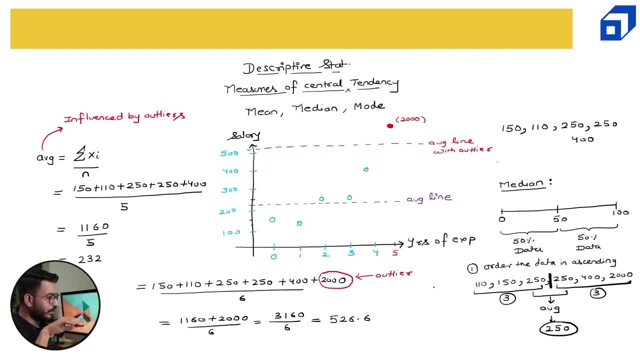 And this is my average. So you can see that even this particular data is having outlier, which is 2000,. which is this value is still. my average is two, 50,, which is near to center. So my average is over here. 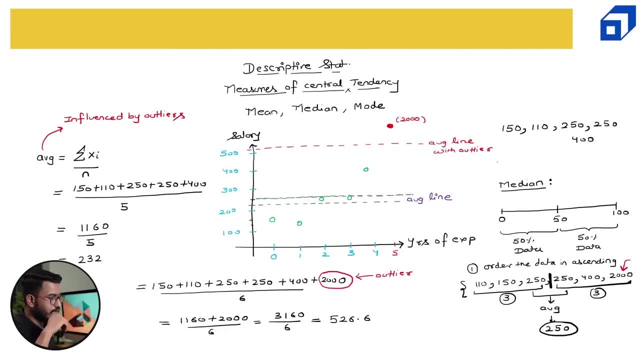 This is my average line or the median line. This is my median line, Median. Now, what is mode? So we have understood mean, we have understood median. What is more, mode is that observation which is having highest frequency in your data. 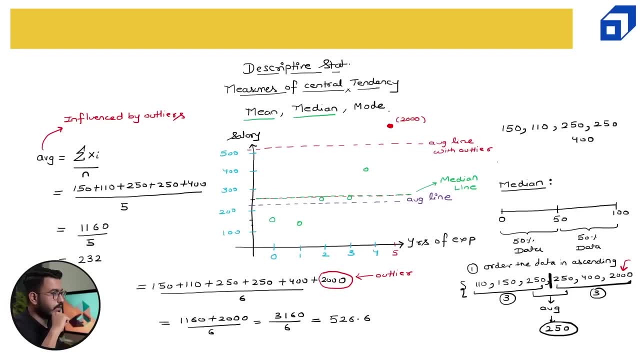 So the particular observation mode is the observation with Okay Highest frequency in the data. Highest frequency means most number of occurrence. So if I look into my data- and I should add 2000 also in this- the particular value which is two, 50, has occurred for two times, while other values like one 51,, 10 and 4, 402,000,. 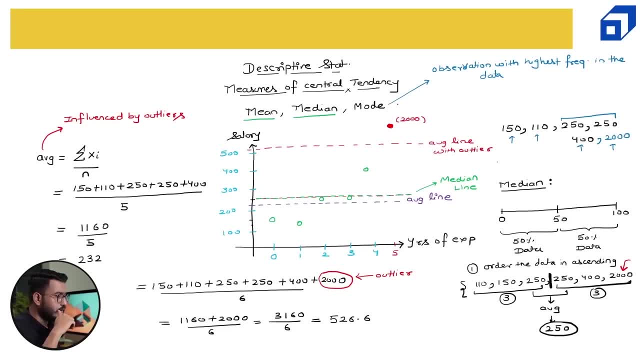 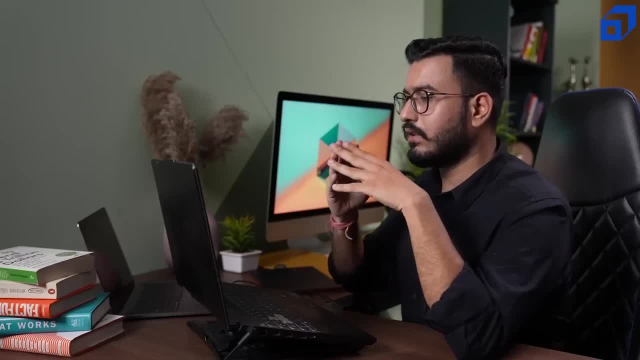 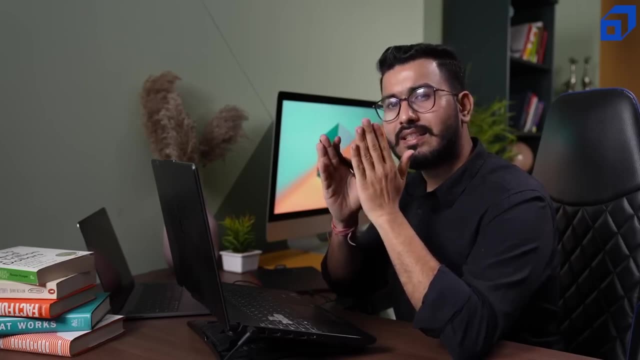 they have just awkward for one more time. Okay, So my mode would be two, 50 in this case. this is my mode, So you can understand that all these measures, which are the measures of central tendency, are basically helping you to find out the central point of the data, while mean is a. metric that get influenced by the outlier. Median is still a metric which is not getting influenced by the outlier. Another advantage of median is that it will give you a point Okay In the data from where, below that point, you will have 50% of the data above that point. 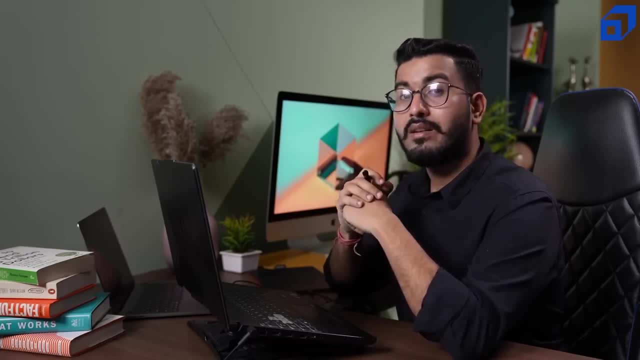 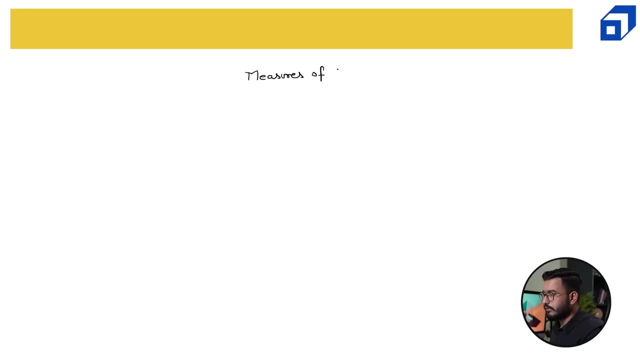 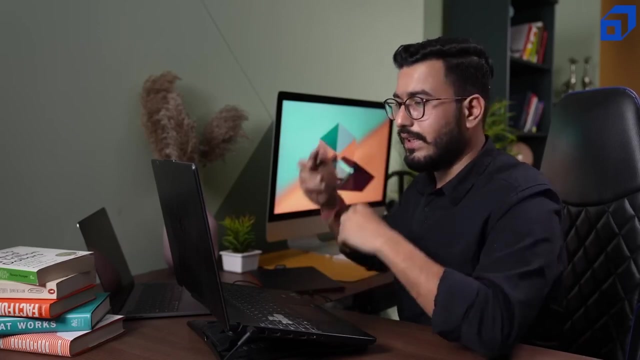 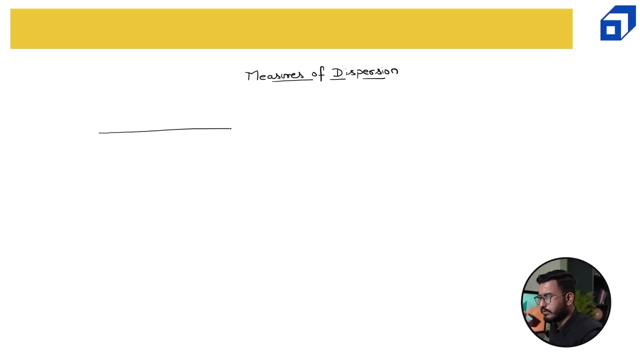 You will have 50% of the data. Now let's try to understand measures of dispersion. measures of dispersion: Now my objective is to find out how far the data points are from the central point. Okay, So let's say, if I'm having a particular number line and this is the center of the data and 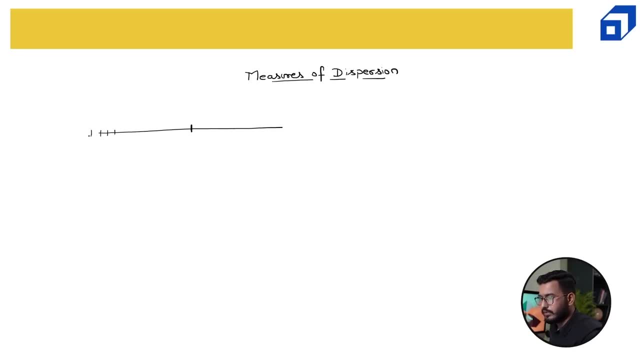 I'm having data points which are very far away over here. So, remember, this is my center of the data, while these are my data points. Okay, So here you can see that your data points are very far away from the center of the data. 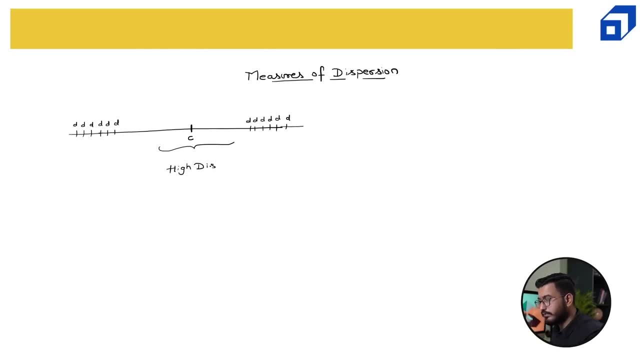 So it will have high dispersion, while if I'm having this case where this is my center and data points are concentrated around the center. So these are my data points, Okay, Okay, Okay, Okay, Okay Now. this kind of data is known as the low dispersion. 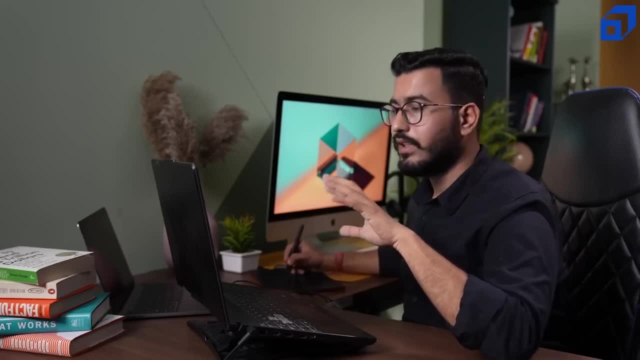 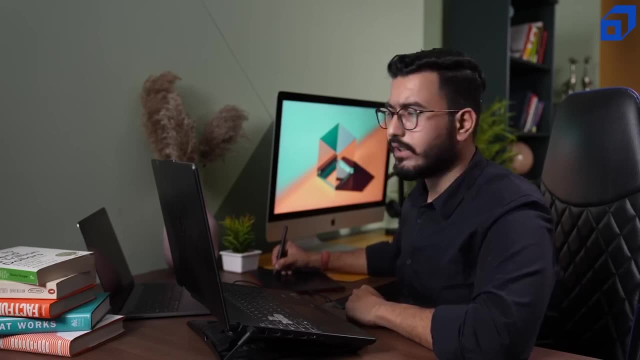 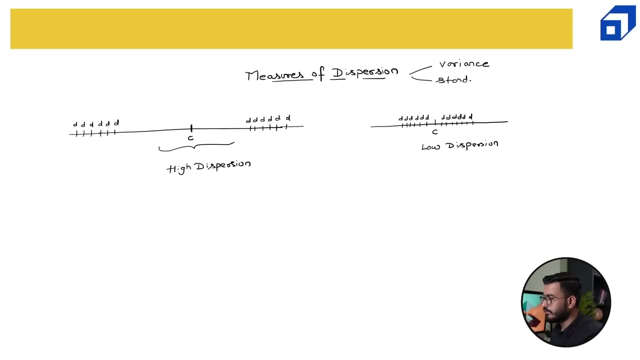 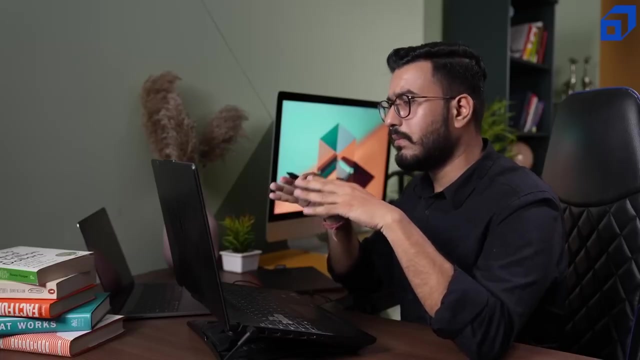 Now the metric that can help us to calculate this is known as the measures of dispersion. We have various metric around this, but two basic metrics are variance and standard deviation. Okay, Okay, Okay, Okay, Let's try to understand it by performing a calculation on Excel. 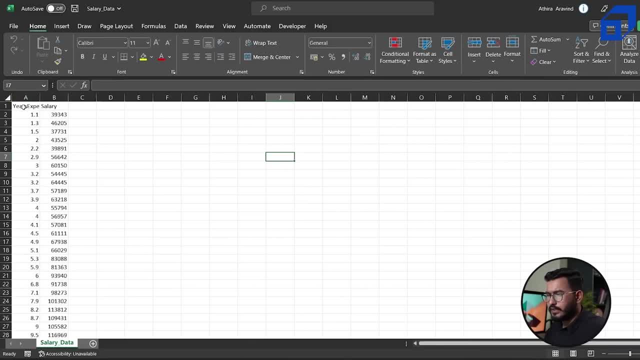 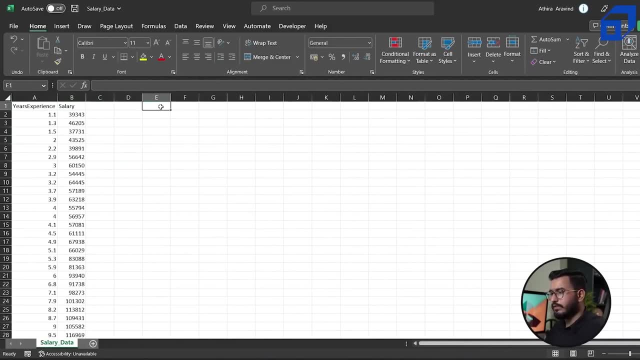 So here I'm having my Excel data with years of experience and salary. Now let's first of all find out the average, which is nothing but mean. So mean, we will apply the formula is equal to average. I'll find out the average salary. 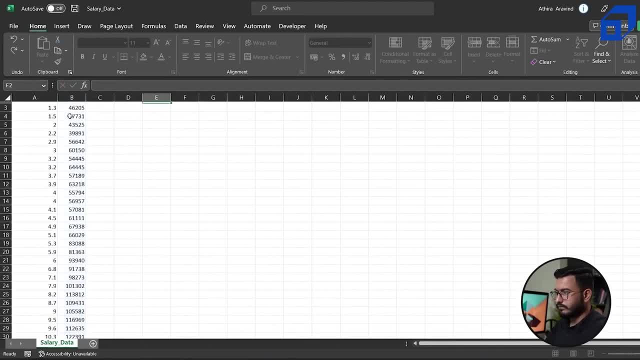 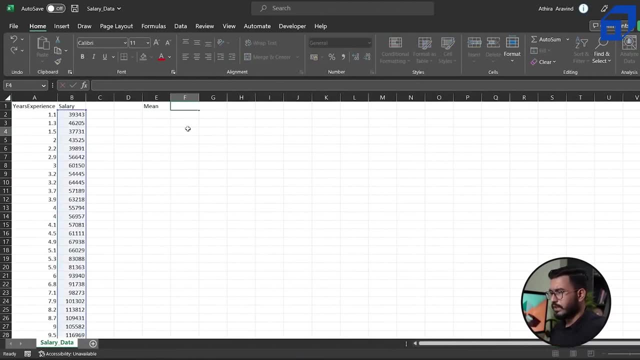 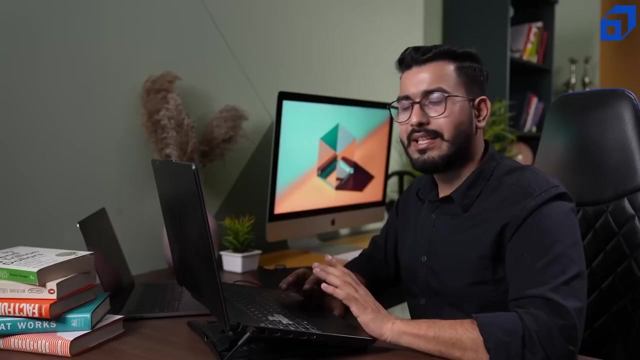 All right. Or let's use years of experience, because that is more simple to understand. So average years of experience, So is equal to average and I'll select my data range. So this is my average, which is 5.31. basically mean the central point of the data is five. 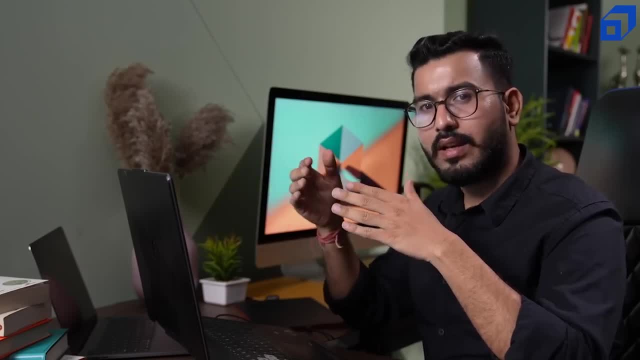 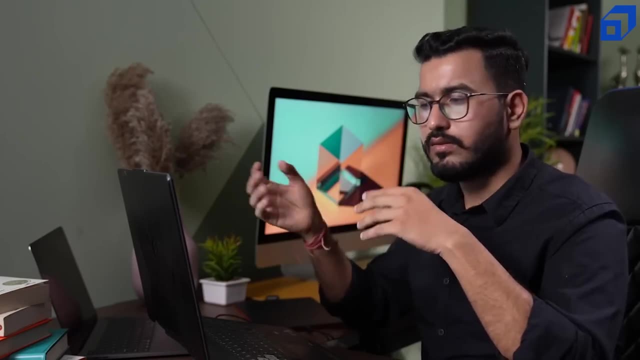 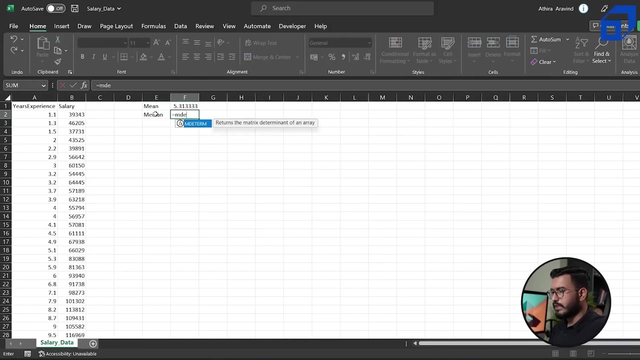 You have some employees below this. you have some employees above this. So maybe we have some employees with one years of experience. We have some with 15 also, but this is the center. Similarly, let's find: median is equal to median and we will use the same data range. 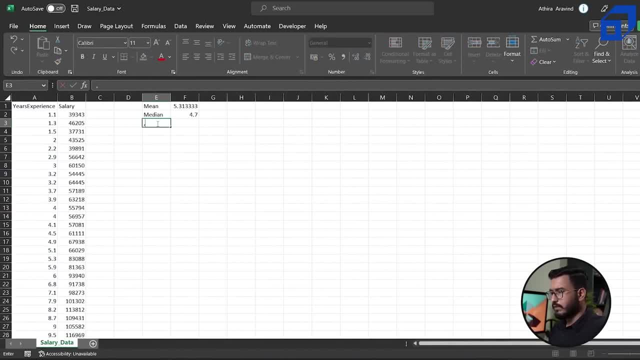 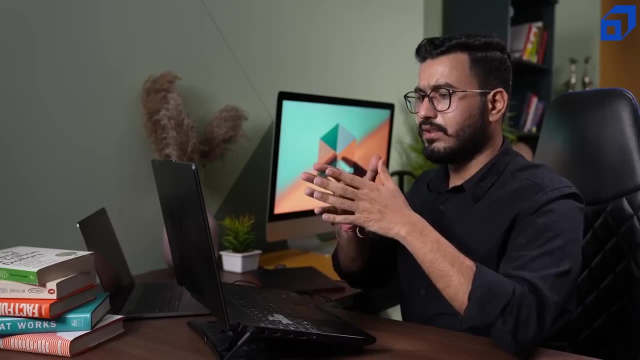 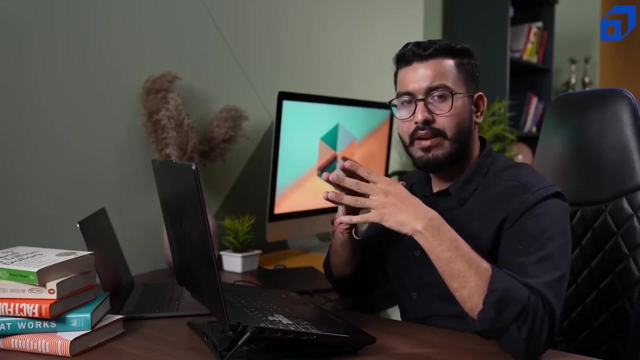 And that's 4.7.. And let's find mode. Now Is equal to mode And my mode is 3.2.. Now you can see that these three values are not equal to each other. They are different. One thing we can understand is the data must be having some outlier, due to which this particular 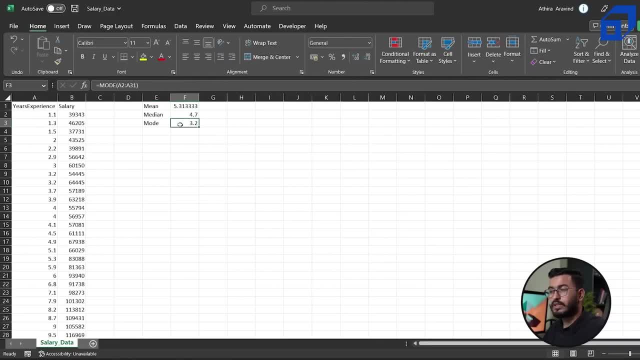 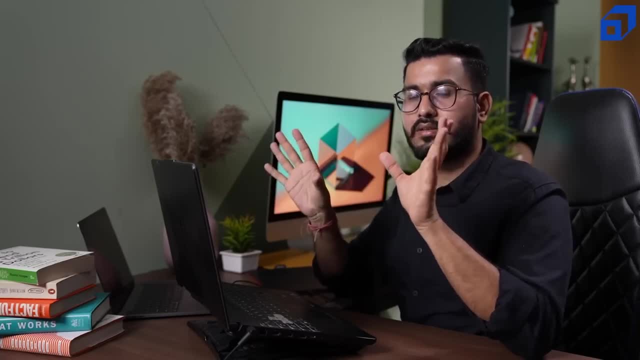 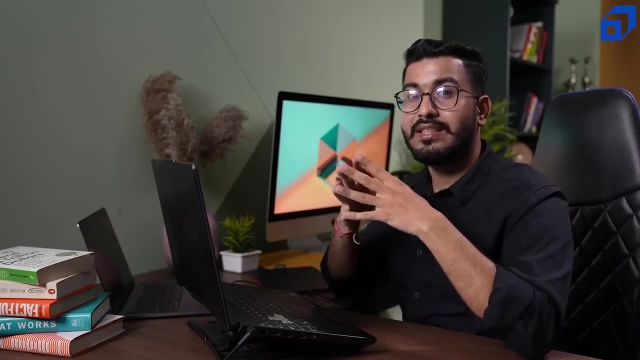 thing or mean and median is not matching. Also, mode is not matching. If a particular data Is having mean is equal to median, is equal to mode, Then the data is balanced, which basically means it is exactly having the center point: 50% below, 50% above. this kind of data is known as the normal distribution data, which is 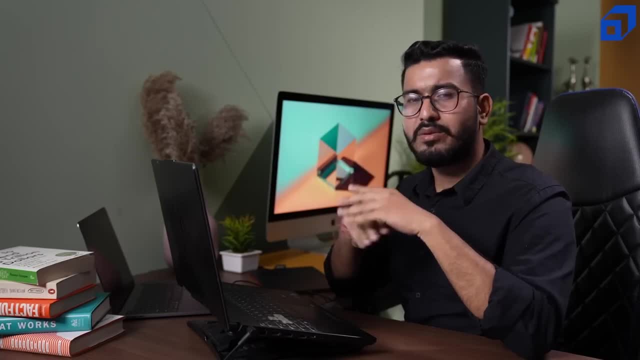 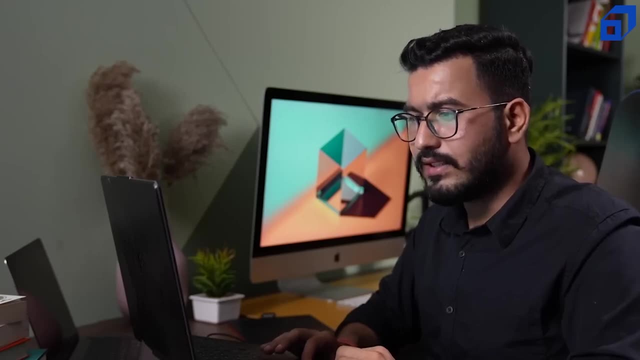 difficult to find out in reality, but our objective is to understand variance over here. So let's come to the point Now, what we will do. we will find out the distance of this point from the average, So from the center, How much? 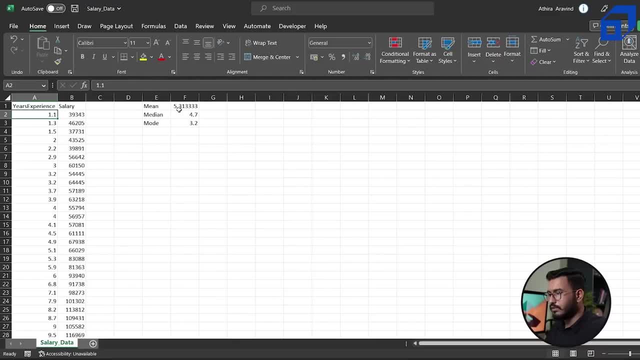 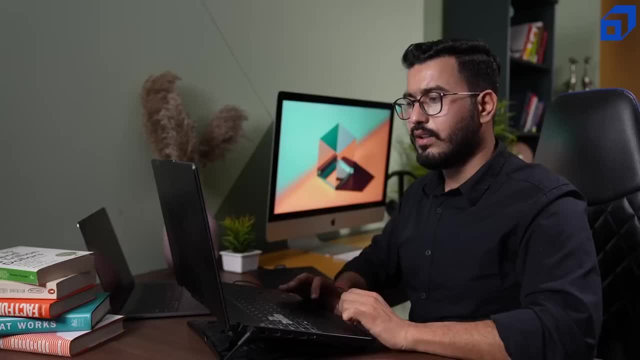 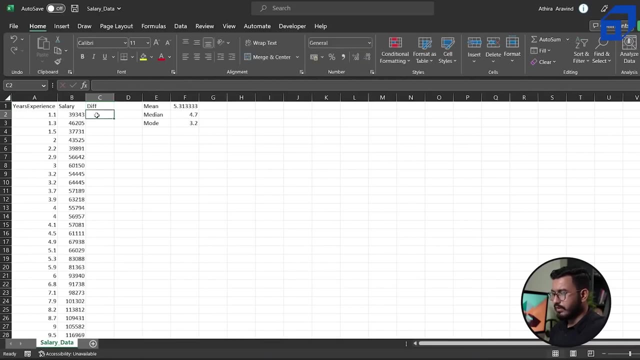 What are years, or this particular employee is. So the average or the middle point is 5.3.. This particular employee is having a year of 1.1 and the difference is 4.2. So let's calculate that difference. So I like D, I, F, F, which is difference, is equal to average minus the value. 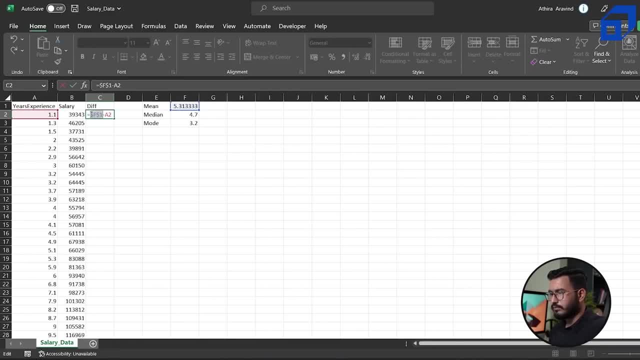 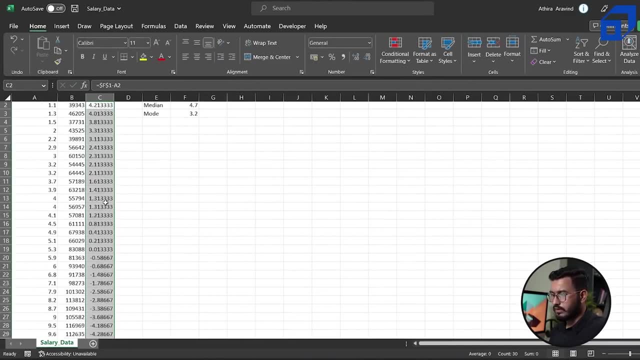 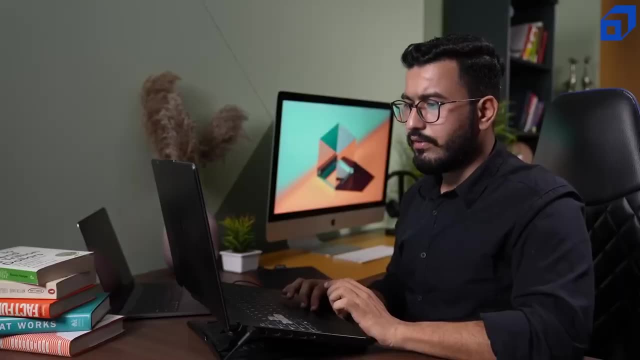 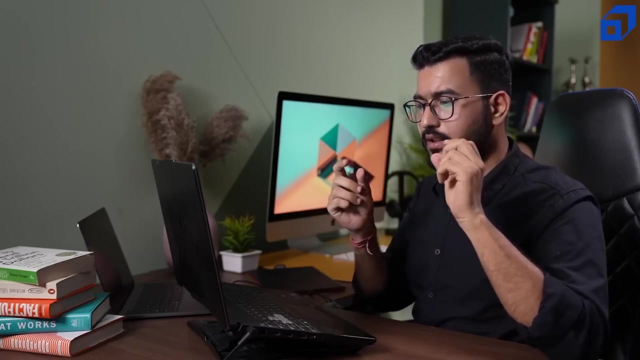 And I'll fixate the average value And press enter. Now this is 4.2.. Let's apply the formula to all the rows. Now, here you can see that I'm having some positive value, some negative values. If I wanted to find out on an average how much the value is above or below the mean, 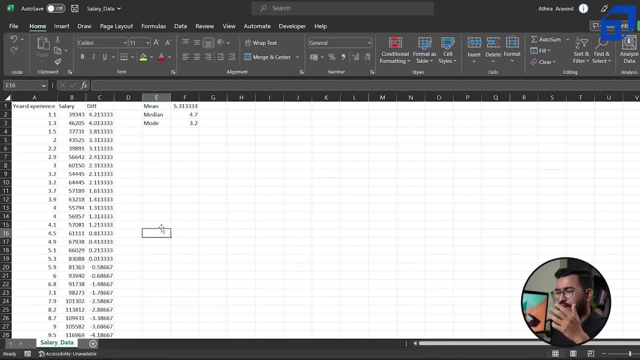 I need to take the average of this column, right. But if I take the average, my positive values will cancel out negative value. That is a problem, right? The easiest, Because we take the square of these values. So D, I, F, F. hyphen square. 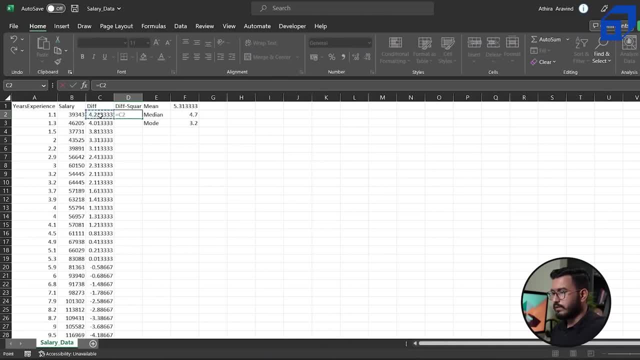 And let's take the square of each value. So this value to the power of two, And I'll expand the formula to all the rows, And now we'll take the average of all these values. So is equal to average Of all these values. 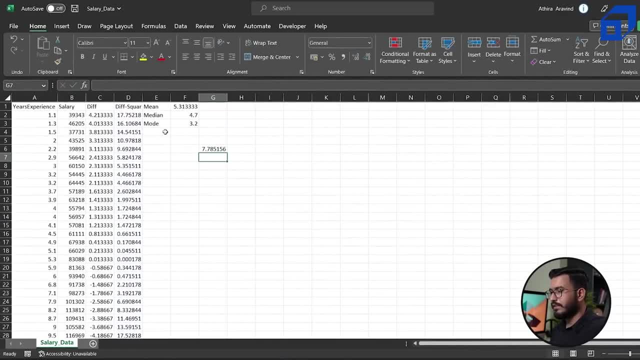 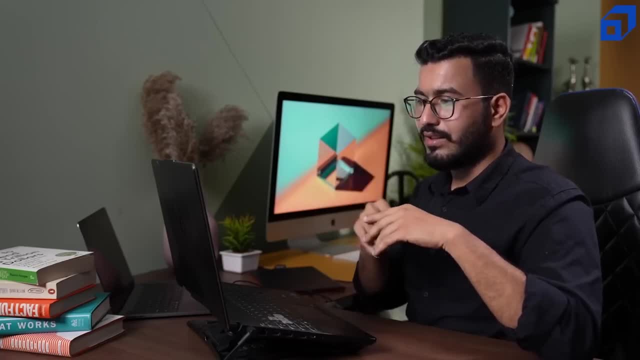 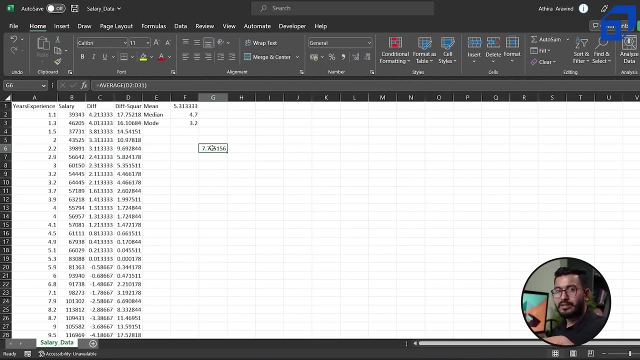 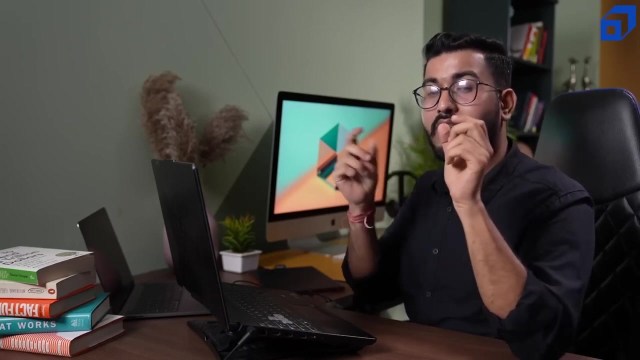 And here the average is 7.7.. Which basically means: Now, this is something which is wrong, Because, remember, we have taken the average of Squared values, So this is also a square value- How we can get a actual answer to understand how much a particular data point on an average. 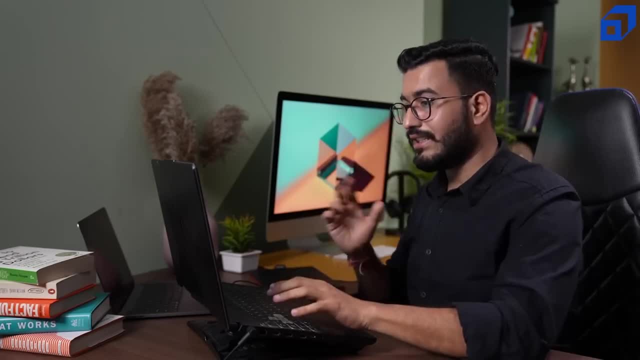 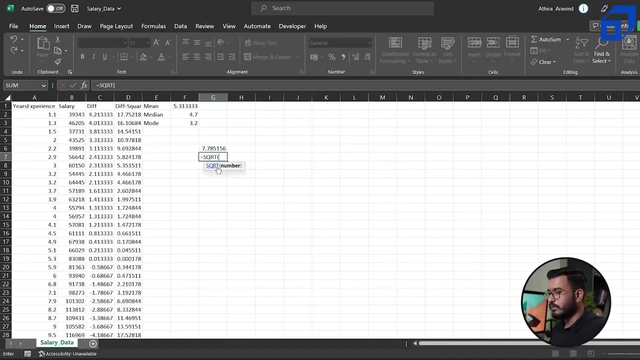 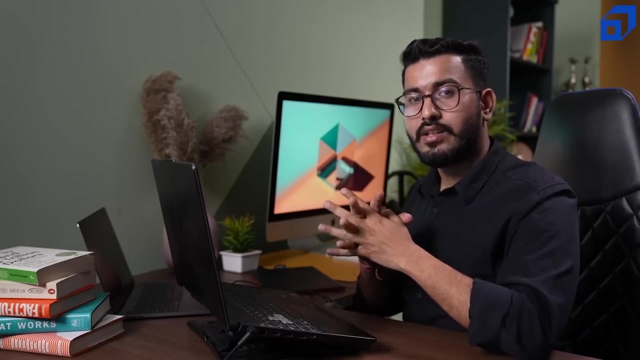 is above or below the central point. I'll take the Square root of this value. So is equal to a square root of This value, And that is 2.7, which basically means, on an average, A particular data point is 2.7 units above or below the mean. 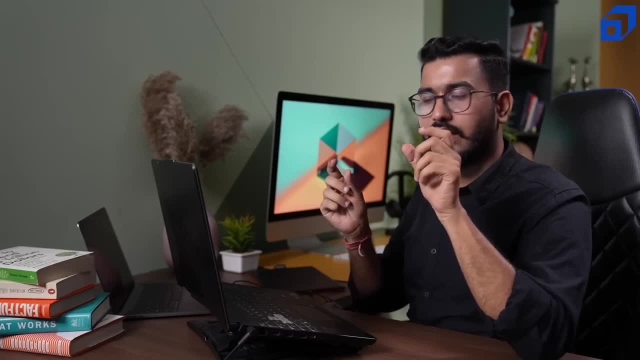 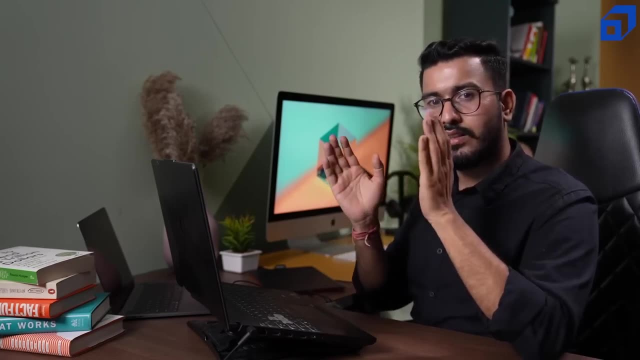 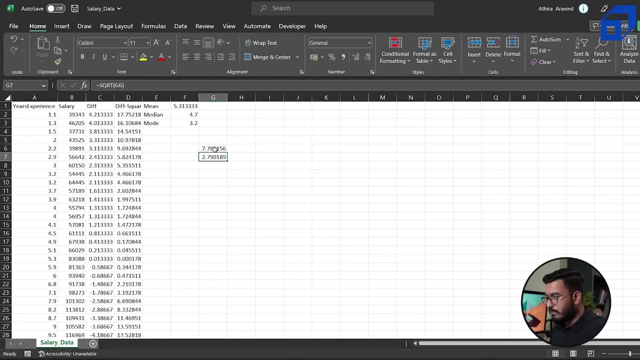 And that is the standard deviation of the data. Now, higher this number, The data is having higher variance. Lower this number: The data is, or maybe most of the data points are, concentrated towards or around the mean. Remember this particular Number that we have derived. 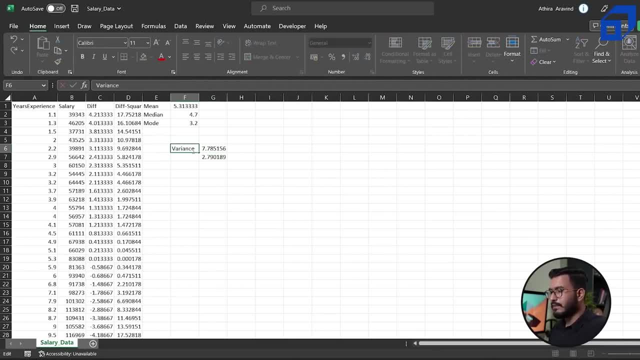 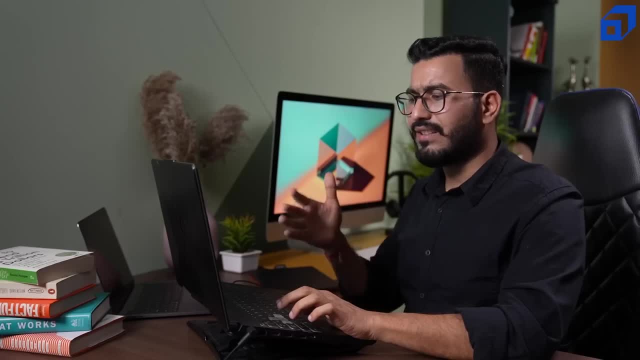 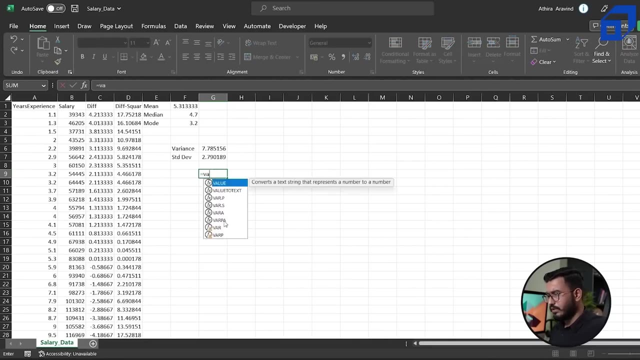 This is known as variance, And various in some is something that is hard to interpret. That is the reason we use a standard deviation. We have direct formula to calculate these numbers in Excel. Also For variance, We have VAR Over here. 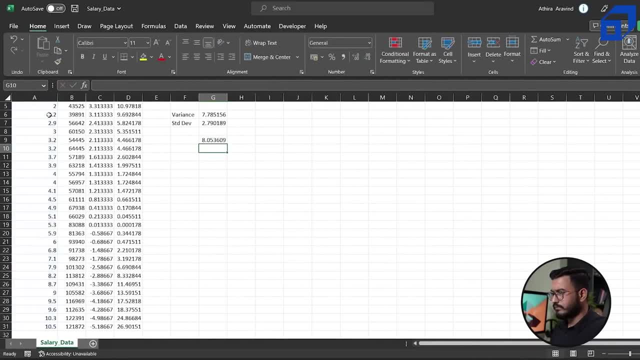 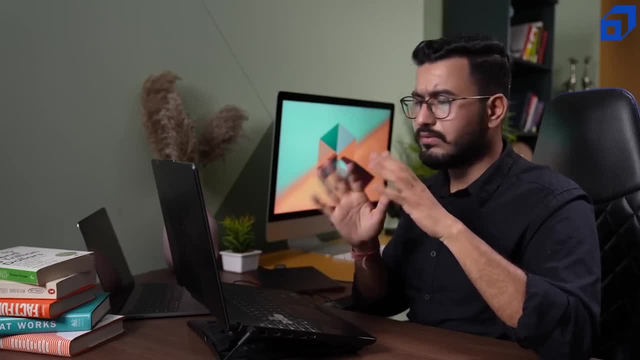 And it will give you the exact same answer. Or which is 8.5.. Now there is a difference. The difference is because of a degree of freedom. Please do not worry about this particular concept As of now, it's again a mathematical topic. 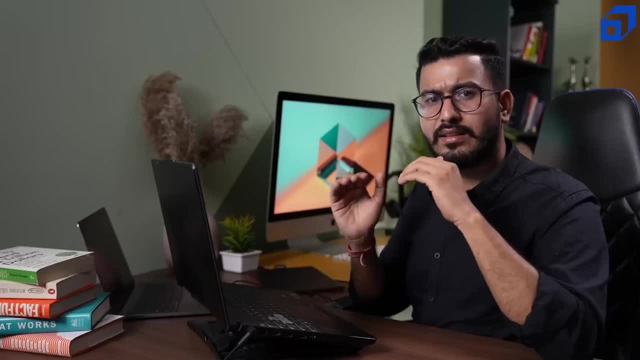 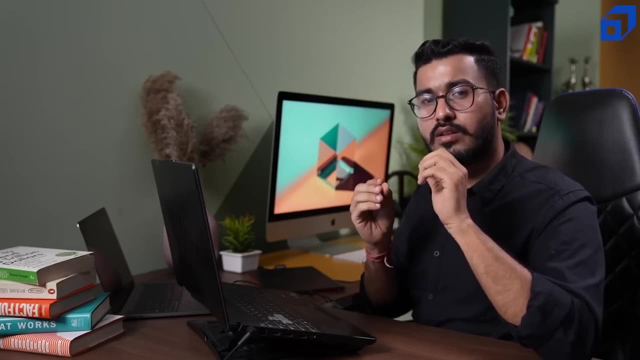 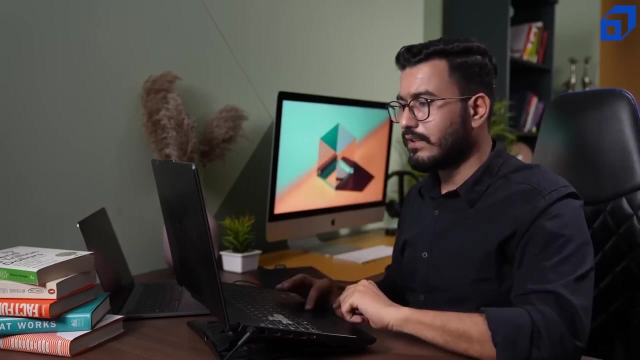 But as of now I'll delete this. Let's summarize What is a standard deviation and what is variance. So this standard deviation will help you to understand how much. What is a standard deviation, particular value or how much on an average, the values are below or above the mean, and that is. 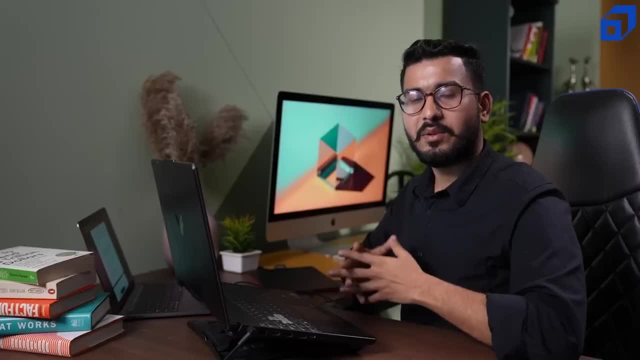 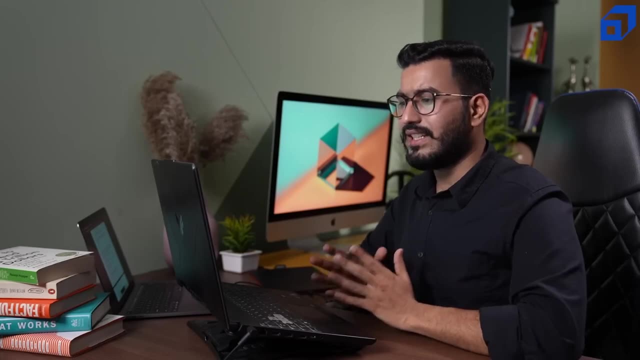 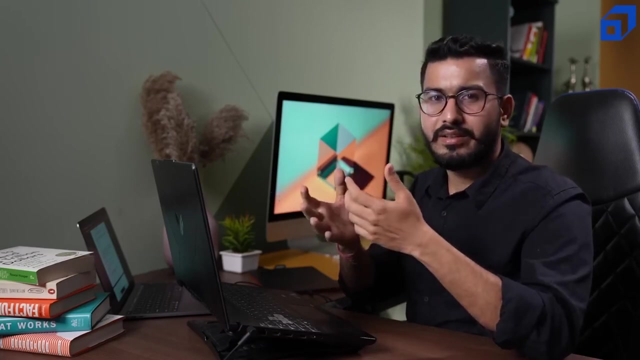 2.79 in this particular case. now let's try to understand the second category, which is linear algebra, and the most important topic under linear algebra is matrix. now i hope everyone knows that the data with which we work it is a two-dimensional data. we have rows. 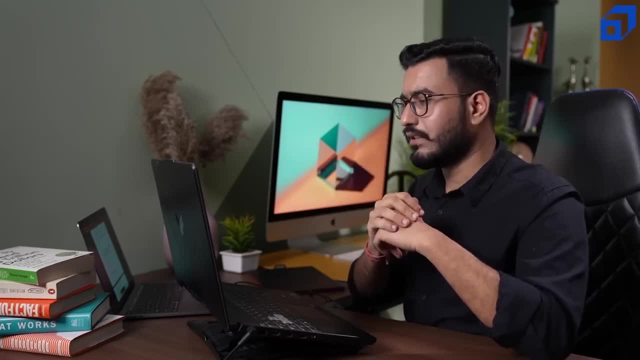 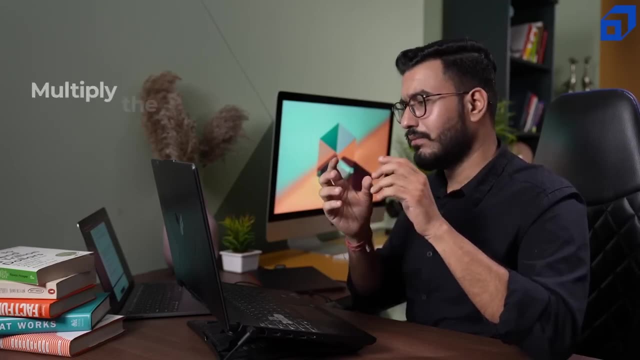 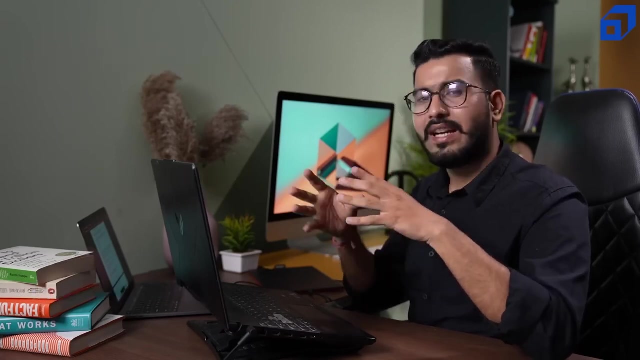 columns, and the best way to represent that data is using matrix. now, when you have a matrix, you have to perform a variety of operations like multiply the matrix, transpose the matrix, find the inverse of the matrix, and so on. let's try to understand some basic operations in matrix. 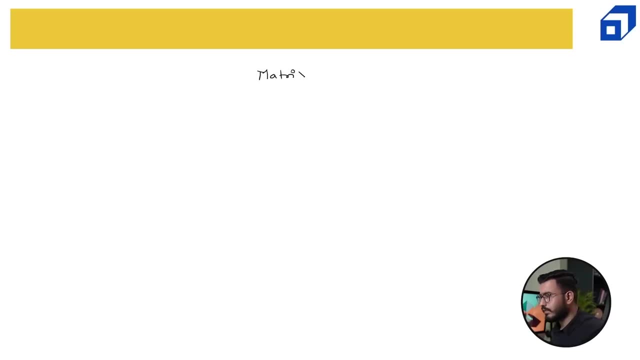 so a particular matrix is a 2d structure defined by rows and columns. so here we have rows, so these are my rows: row 1, row 2, row 3, and these are my columns: column 1, column 2, column 3, and these are my elements. 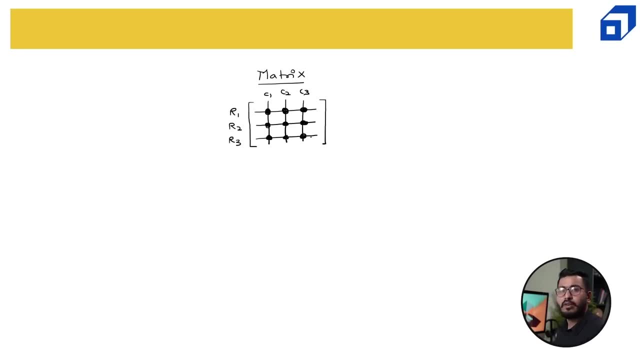 a particular matrix have variety of shape. the shape of a matrix is defined by the number of rows, followed by number of columns. so this matrix is having a shape of 3 cross 3 because it is having 3 rows and 3 columns. now, when you have two matrix, 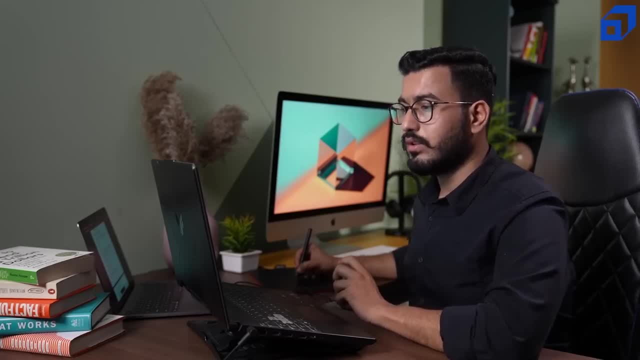 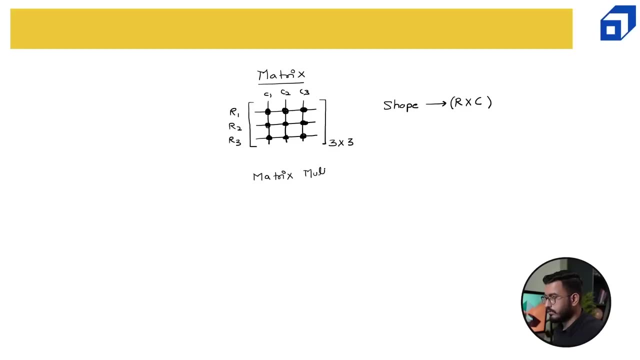 there are certain rules that you have to keep in mind before performing matrix multiplication. matrix multiplication: the very first rule is the number of columns of the first matrix should be equal to the number of rows of the second matrix. when you multiply two matrix, the output that you will get will have the number of rows. 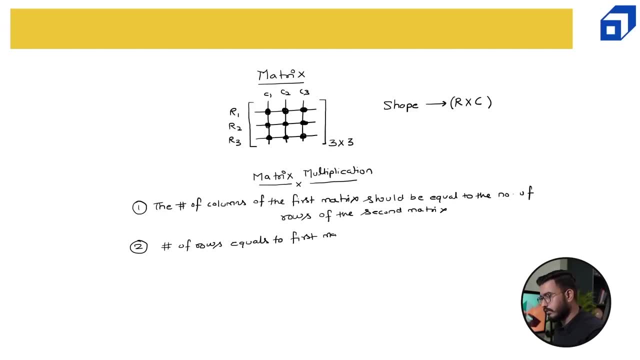 equals to first matrix and the number of rows of the second matrix will be equal to the number of columns of the first matrix. and then let's take one general example. let's say i am having a matrix with 1, 2, 3, 4, 5, 6, and here i am having a matrix with 2, 2. 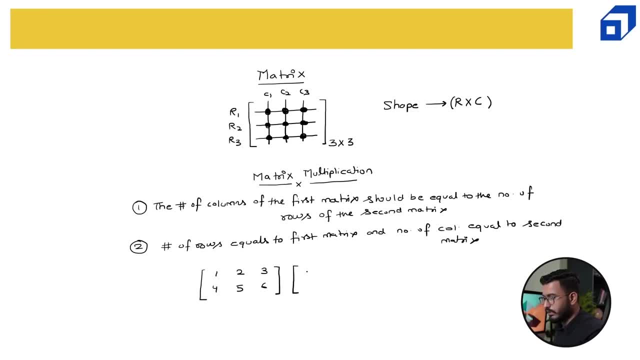 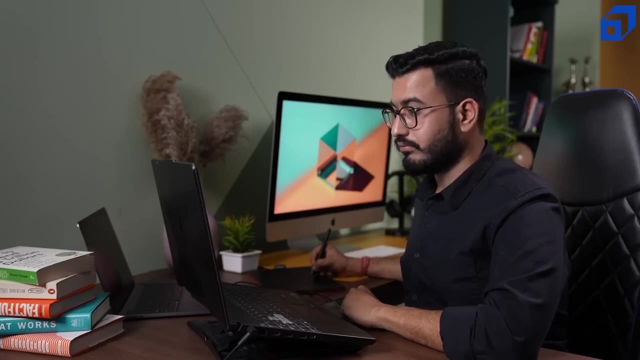 and here i am having a matrix with 2- 2- now this is my matrix a- with a matrix a. and here we have a matrix a with a matrix a with a matrix a. this is my matrix B. can we perform matrix multiplication? the answer is no, these two. 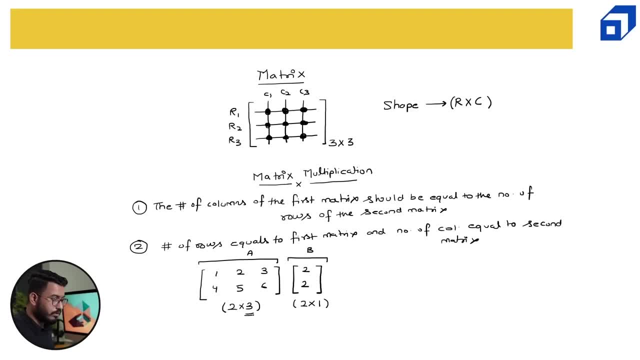 matrix cannot be multiplied, because the number of columns of first matrix should be same as number of rows of the second matrix. so what we have to, let's add one more value. so let me make me, let me make this as 2, 2 & 2, so this is now 3 rows, 1 column. now this is matching. 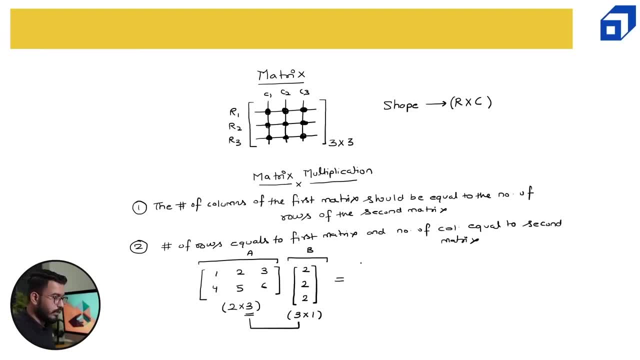 this so we can perform matrix multiplication. how the matrix multiplication will happen, remember: R will be multiplied by C rows multiplied by column. so this is my one row. I'll multiply this with my entire column. let's do that. so my first value will be 1 into 2 plus 2 into 2 plus 3 into 2. my second value will be 4 into 2. 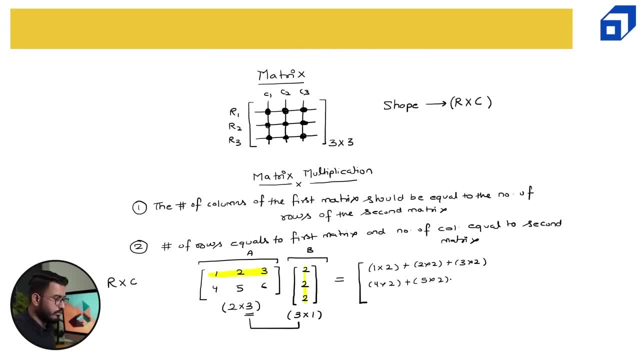 plus 5 into 2, plus 6 into 2, and that's the answer would be 2 plus 4 plus 6 Multiplied by C. killed by C times like this is my first value, so i put 1 in section is not what. will be given number or argument. yeah, second value will be 2 & 2. now we can see this is my value between 2 & 2 & 3, and i'll put 1 on every row. it is 2 and parts of my adults, this is my. value between: here will be a column, and on top i will bring number 1. so at this point b represents base force for 2. this is my second value. so this is my second value. so this will be. i will put my first value. this will be. i will put my new problem in the next page and that's my second value. 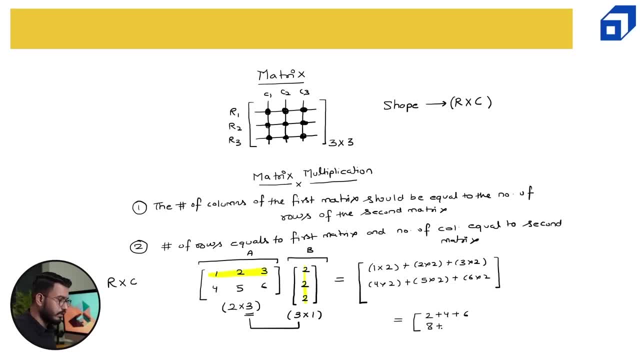 that this is the first value system, that this was loved to define the loop. second, i will be plus 4 plus 6, and this will be 8 plus 10 plus, I think, 12. so here the total is 12 and here the total is 30. this is your answer. now the number of rows. this is for the resultant matrix. 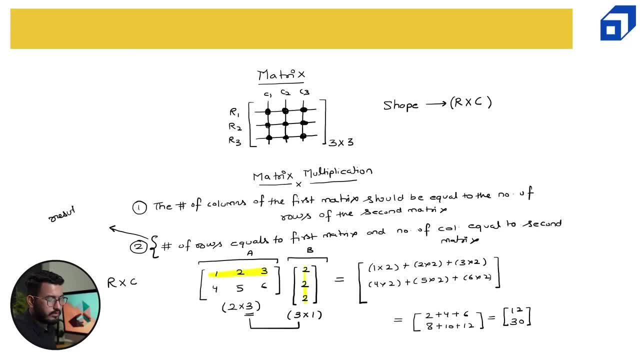 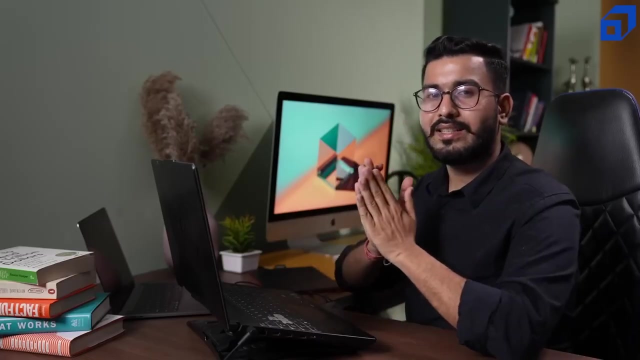 after multiplication. resultant matrix after multiplication. so the number of rows equal to first matrix. we have two rows, which is equal to first matrix. number of columns equal to second. number of column is 1. so 2 comma 1 and this is my answer. so I hope now you guys are clear with how matrix multiplication happen and what is exactly. 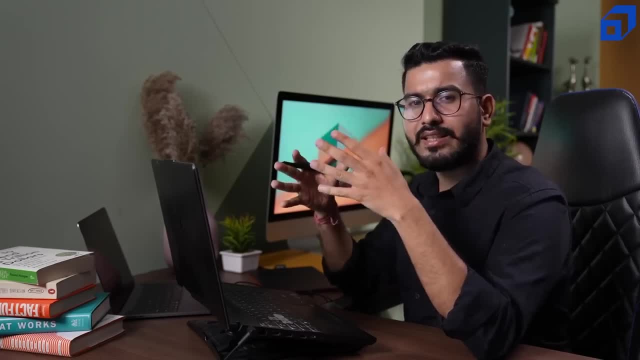 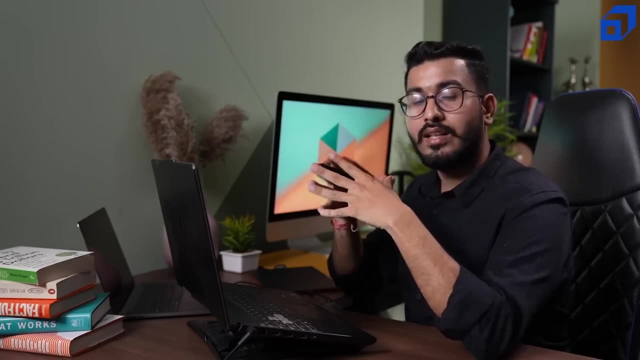 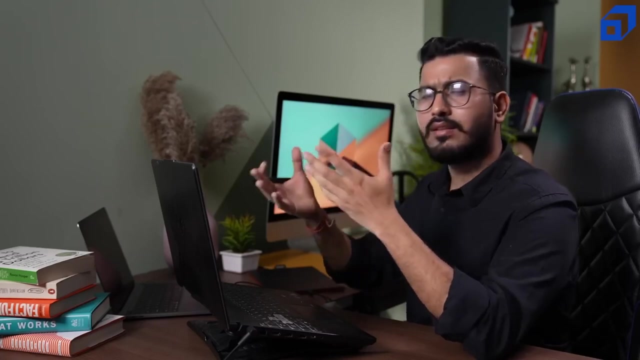 a matrix. again, we are not covering up everything in this video, but I am trying to help you guys with the essence of each topic that you have to learn in detail when it comes to mathematics required for data professional. so let's move to the next topic now. now let's try to understand. 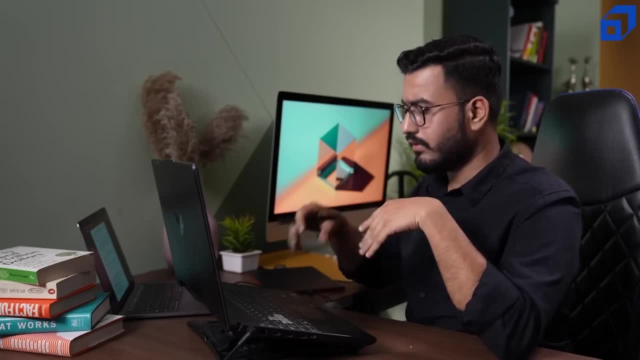 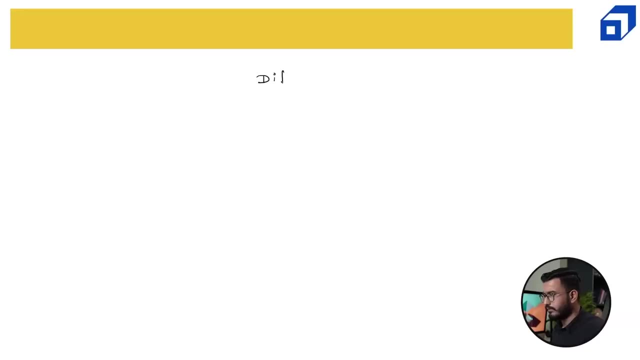 the differential, such as differentiation and partial differentiation. I will give you the idea regarding how to perform differentiation. so let's say I am having a function: f of x is equal to x square. now why I call this as a function? because assume that it is a machine which takes input. 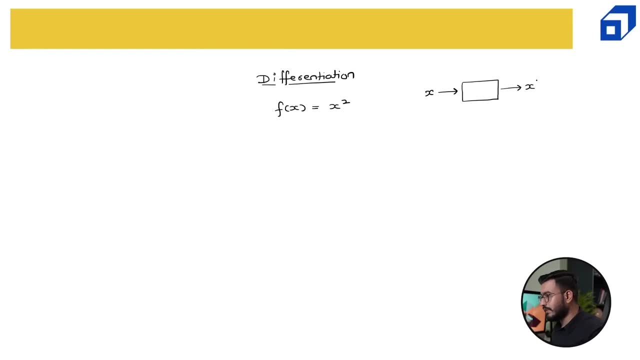 as x and returns an output as x square. so this is a function of x. this is my input to the function, this is my output to the function and this is function of x. so that's how we call it: function of x. now, if I have to differentiate this function, then we use the term dy by dx. 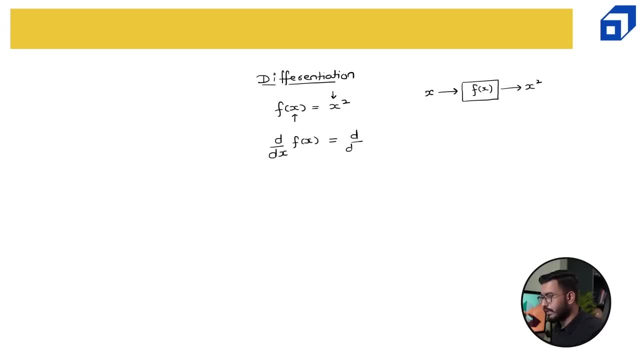 of f of x. here also we will apply dy by dx of x square. there is a general formula of differentiation which is f of x plus x square. dy by dx of x to the power n is nx, n minus 1.. That's the general formula. So this will. 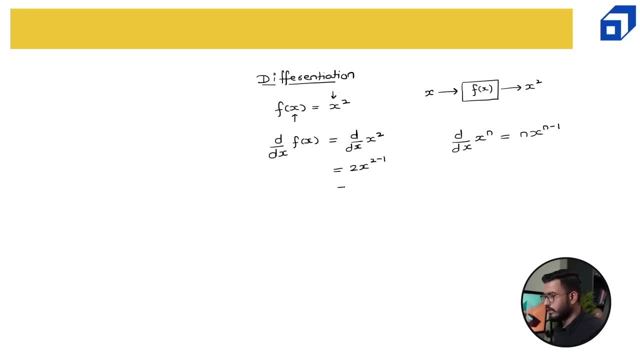 return me 2x, 2 minus 1, which is 2x. So the differentiation, or the differentiation or the differentiated value of the function x square is 2x. In machine learning we call this as the slope. So when you differentiate it you get a slope. And now we are not going. 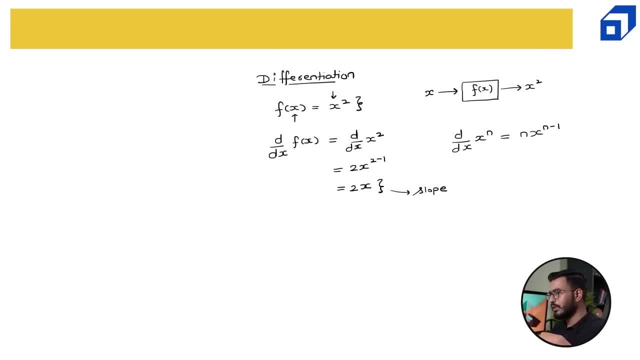 to talk more about what is slope and what is machine learning or maybe which algorithm I'm talking about right now. But this is what differentiation is and you have to learn this topic in detail: How to perform differentiation. The chain rule- I'm just putting the topic name over here: the chain rule, which basically 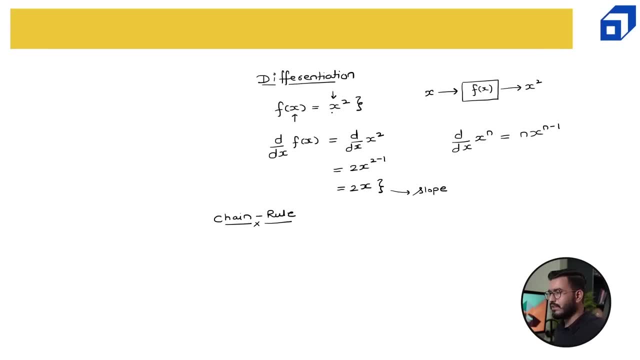 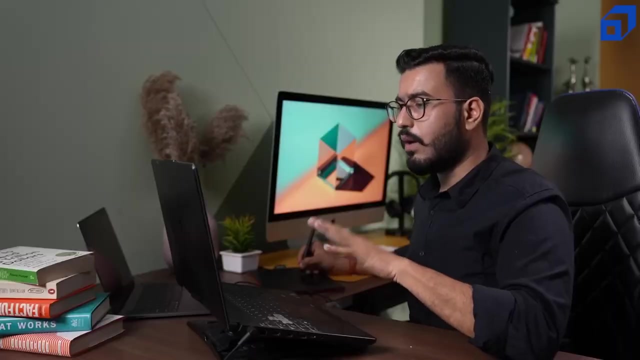 means if I do not have the function, which is this as one particular element? let's say I'm having a function: f of x is equal to x plus y plus 2x square. let's say then how we can differentiate this. There is a chain rule that will help you to differentiate the. 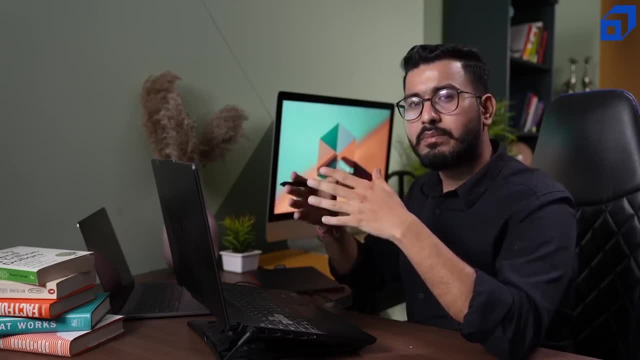 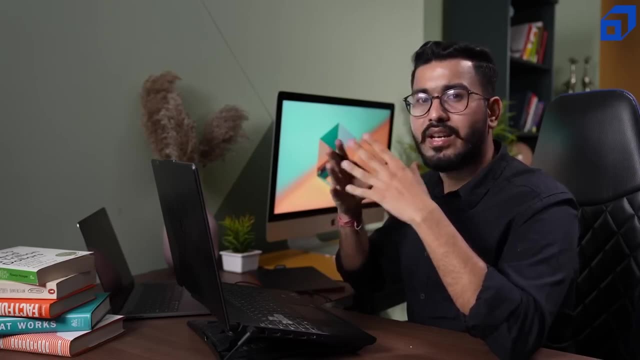 function. So this is how we can differentiate this, And this is really important for any person who is trying to enter into machine learning. So this is the topic that should you should be clear with when it comes to differentials. Let's try to now proceed with. 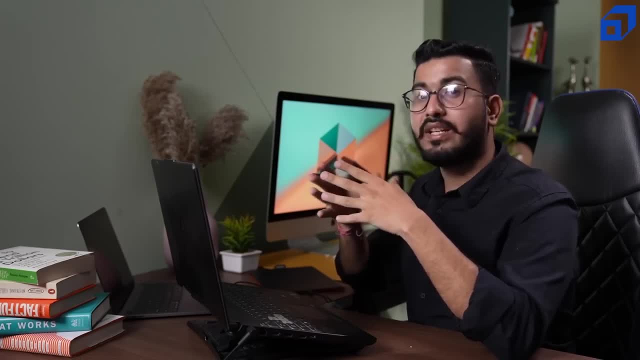 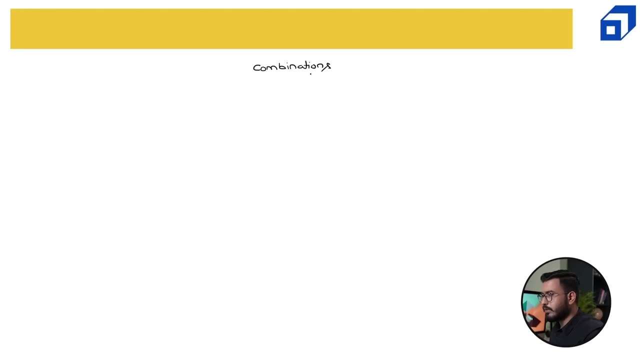 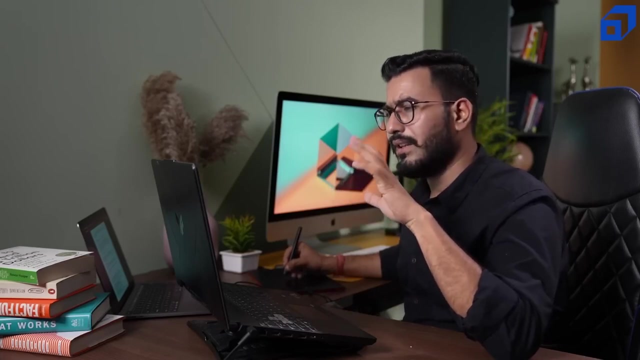 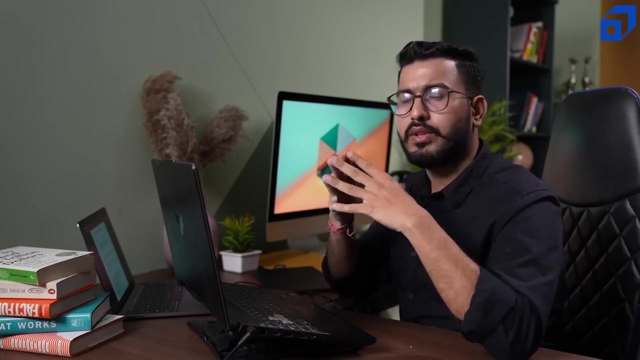 the last topic, which is combinations and permutations, Combinations. This is a very important topic. when it comes to sampling, Combinations and permutations are something which we generally apply in real life also, But when it comes to machine learning- or even not machine learning when it comes to data- 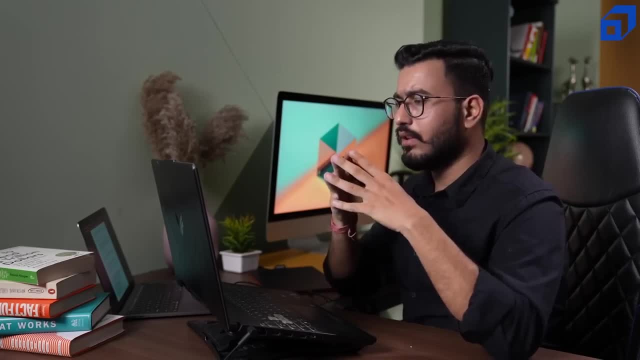 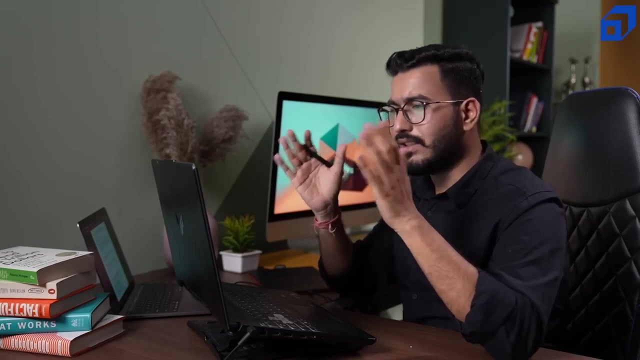 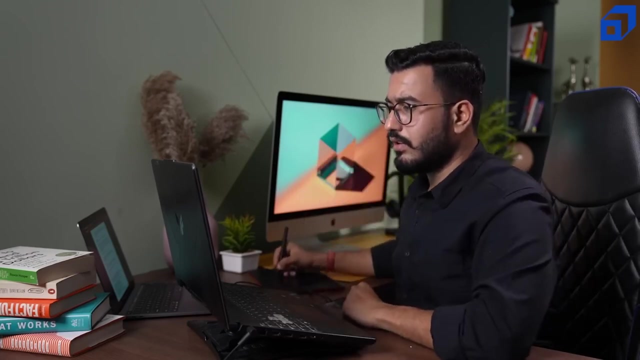 science. when it comes to general data analysis, combinations and permutations are really useful to find out how many iterations or how many times I have to perform a certain task or how many possible variations are possible in this given data. Let's take one example to understand the difference between combinations and permutations. 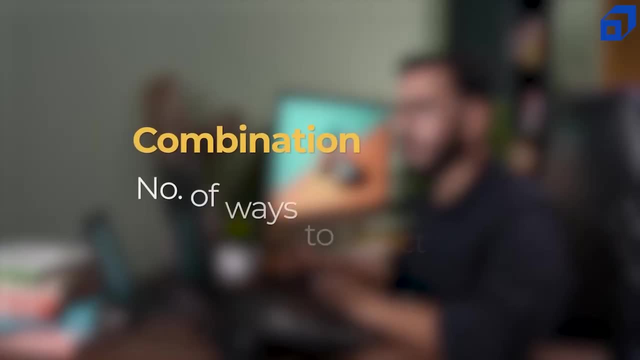 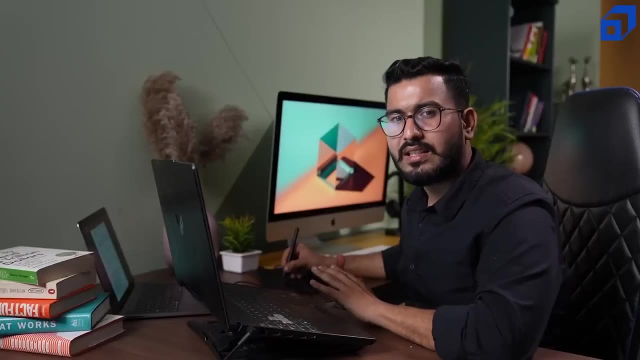 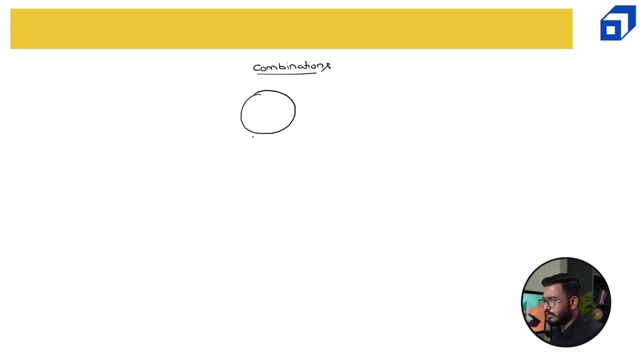 So let's start with combination first of all. So combinations talks about the number of ways to select a particular data point from a given data. Let's try to understand this with one simple example. Let's say I'm having a population, So this is my population, with 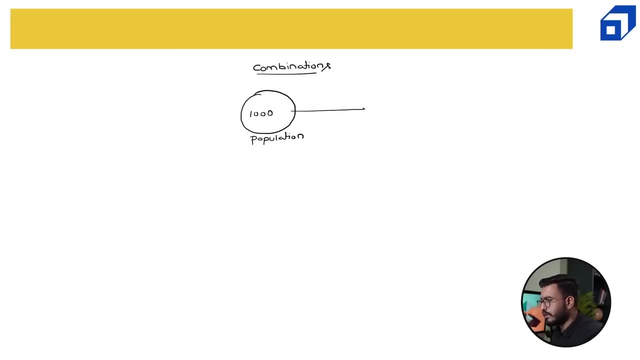 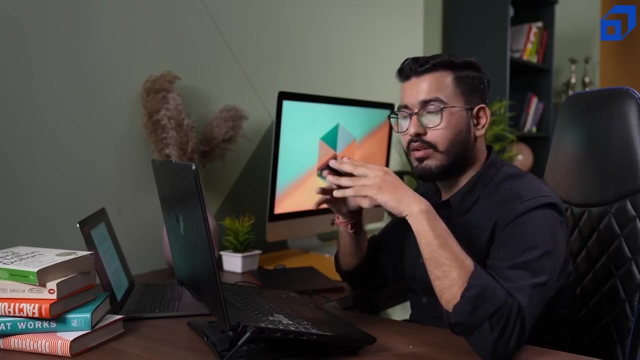 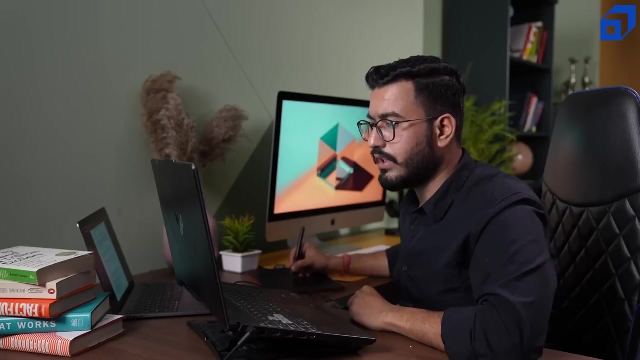 1000 people And I wanted to sample out 100 people. Now, how many combinations are possible? Like which? all 100 people should I select? So how many possible ways are there? Let's try to calculate it. The formula for combination is given as NCR is equal to N factorial divided by R factorial. 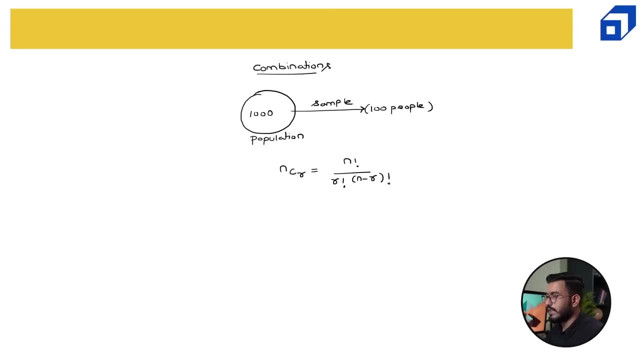 N minus R factorial. Now, what is N? N is the total number of observation, R is the selection that you are trying to make, which is 100.. Let's apply the formula: 1000 factorial divided by 100 factorial. 1000 minus 100 is 900 factorial. If you wanted to expand a factorial, 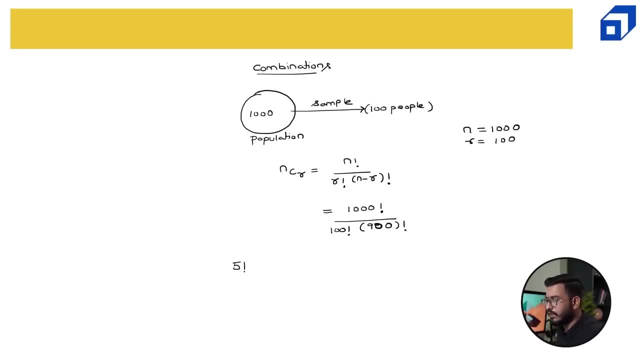 it will be 100 factorial divided by 100 factorial. If you wanted to expand a factorial, it will be 100 factorial divided by 100 factorial. If you wanted to expand a factorial, it will be 100 factorial. So if I expand 5 factorial, it will be 5 into 4, into 3, into 2, into 1, which 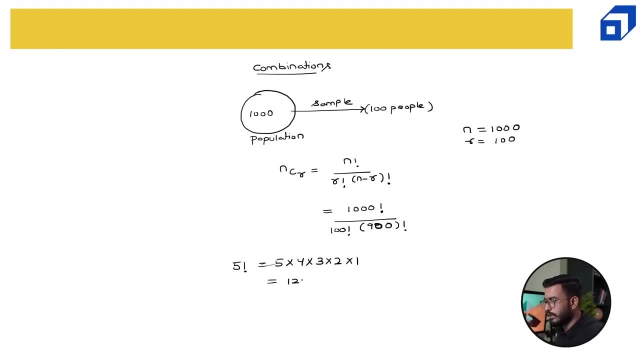 is 5 times 4, is 20, 60 and 120.. Similarly, if I try to solve this, 1000 factorial divided by 100 into 900 factorial, you will get 7.53 into 10 to the power 16.. Now these many combinations. 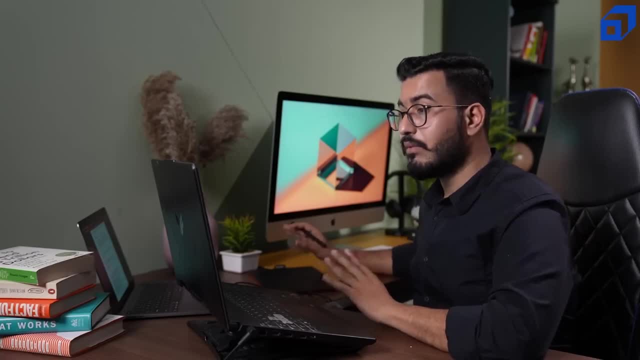 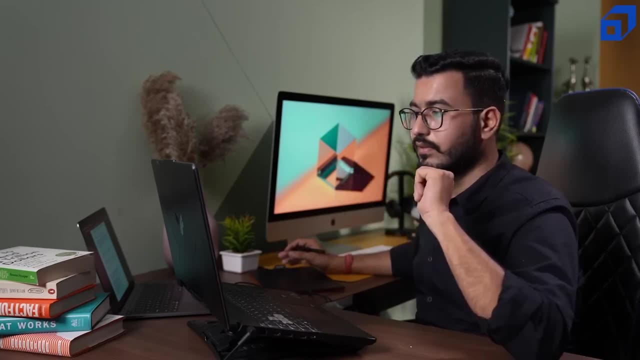 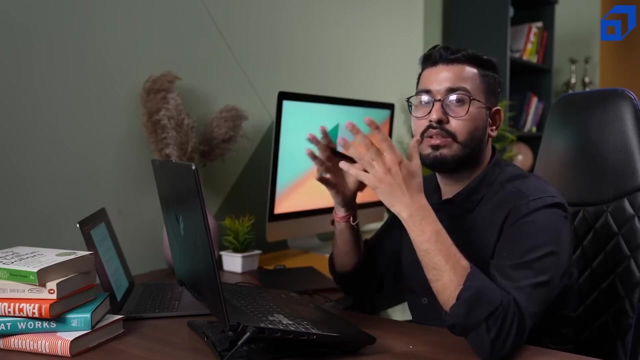 combinations are possible. these many combinations, these many ways you can select 100 people from the group of thousand people and it is a good way to understand, uh like, at what scale we are going to work on, or maybe how much efforts we have to put while performing a certain task. so, combinations, 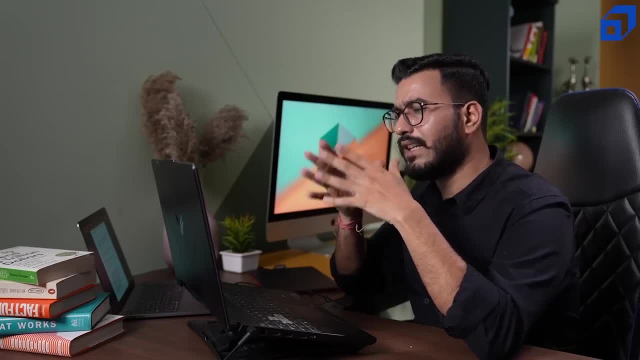 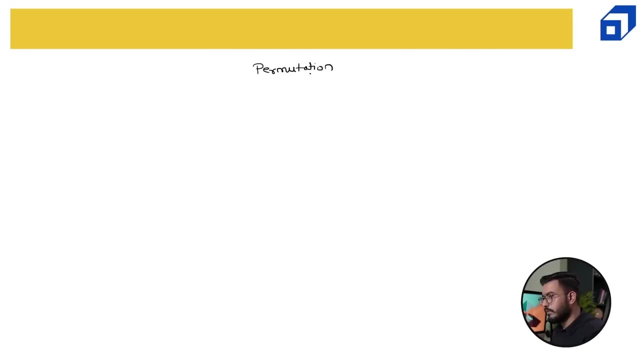 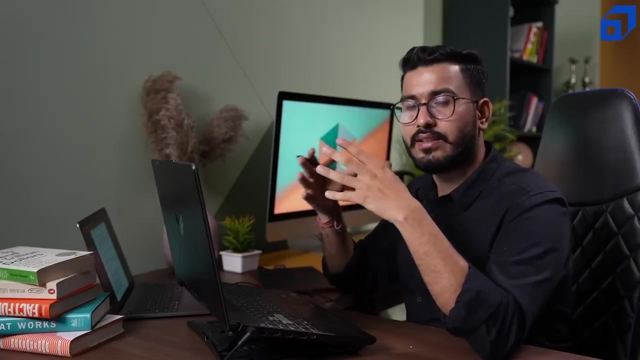 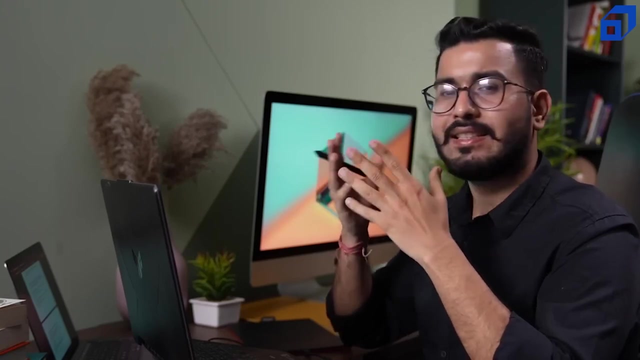 are of great use when it comes to data science. let's try to understand permutation also- permutations now in combinations. we are trying to understand the various ways in permutation. we are trying to understand the arrangement. let's take one general example. so let's say i'm having five books. 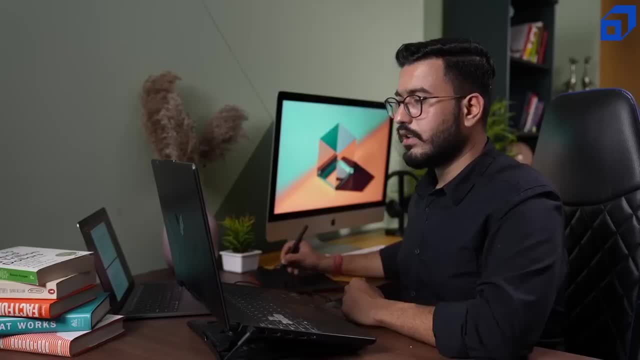 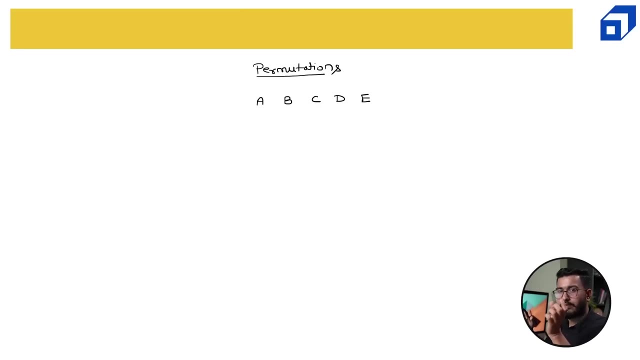 a, b, c, d e. now, how many ways are there in which i can arrange these books in the shelf? so should i keep a first, followed by b, c, d e. so this is one combination. sorry, this is one permutation. similarly, if i place b first, followed by a, c, d, e, this is permutation number two. similarly, 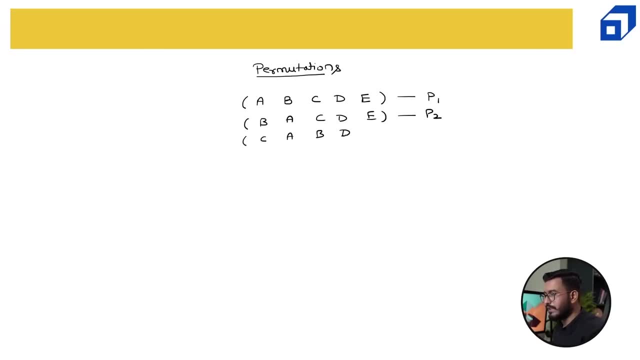 if i keep c first, followed by a, b, d, e, this is permutation number three. so how many such permutations are possible? so for this we have a formula, npr, which is n factorial upon n minus r factorial. so here, n is the number of objects, which is 5, and r is the number of places, which is again 5, in this case. 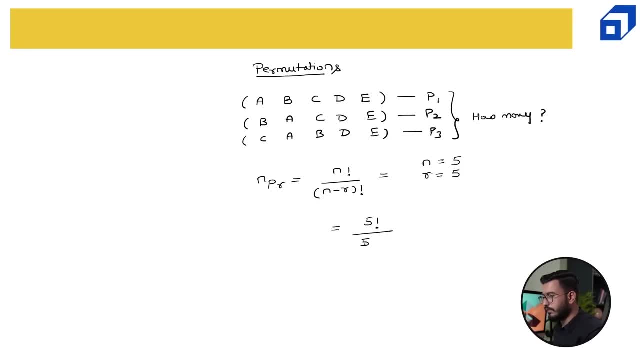 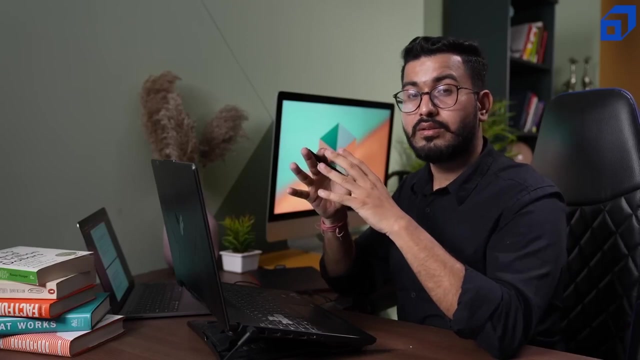 so 5 factorial divided by 5 minus 5 factorial, this will give me 5 factorial, which is 5, into 4, into 3, into 2, into 1, which is 120. so there are 120 possible ways in which you can arrange these books in your bookshelf, now that 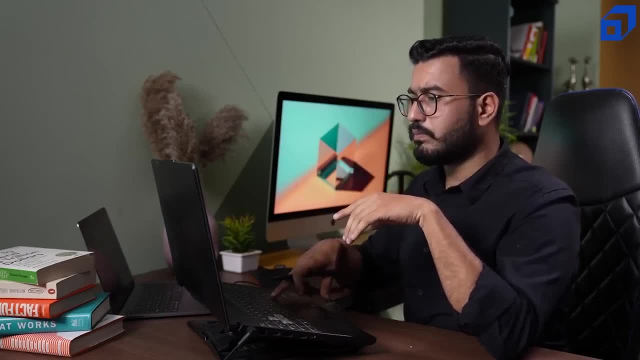 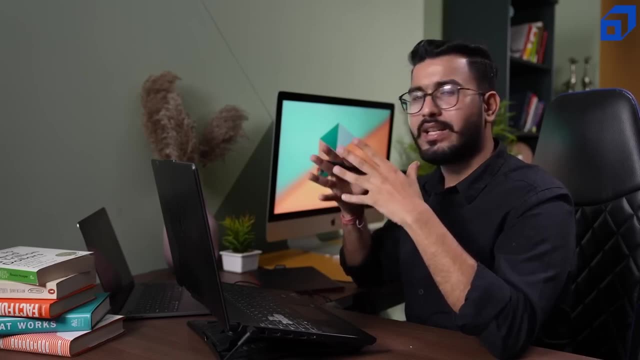 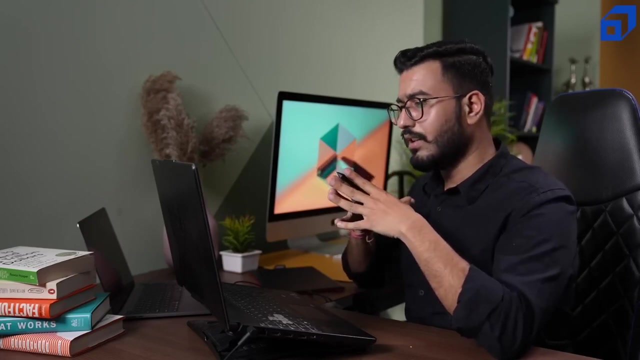 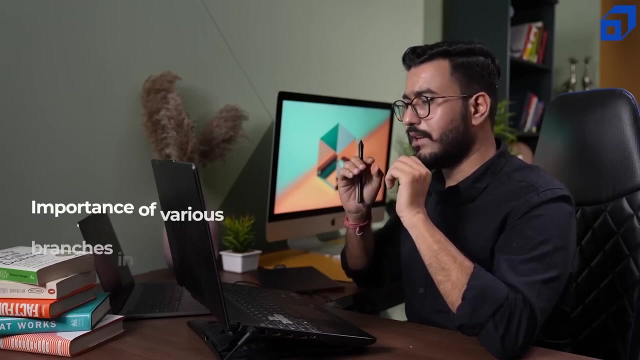 is what permutation is. so I hope now you guys are clear with how much math you need to be prepared with if you are looking to enter into the field of data science or maybe trying to become a data professional again. in this particular video I have tried to make you understand like the importance. 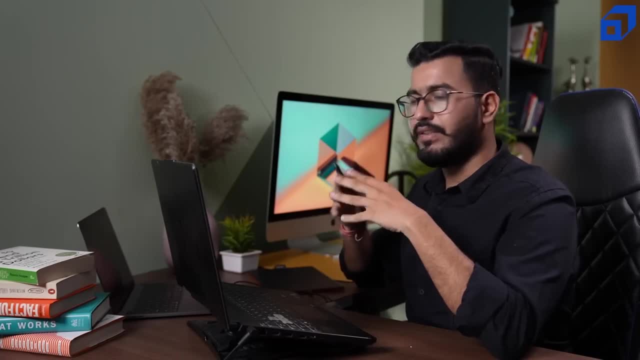 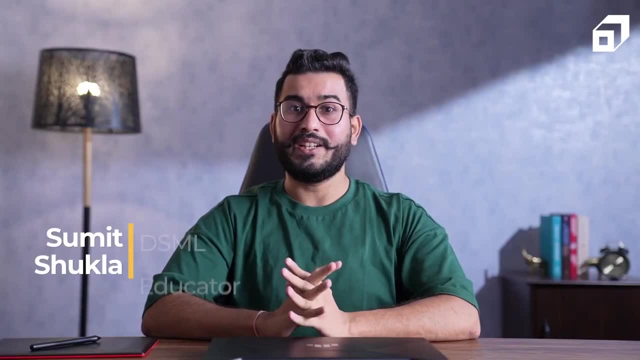 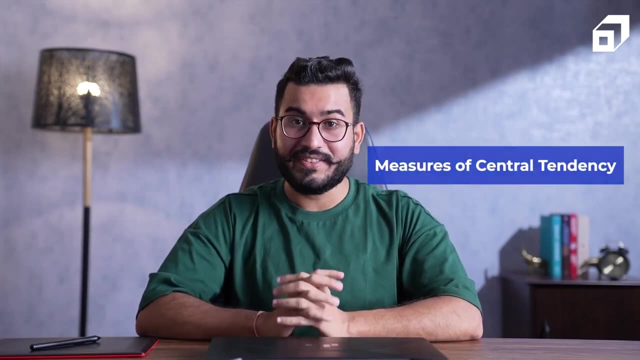 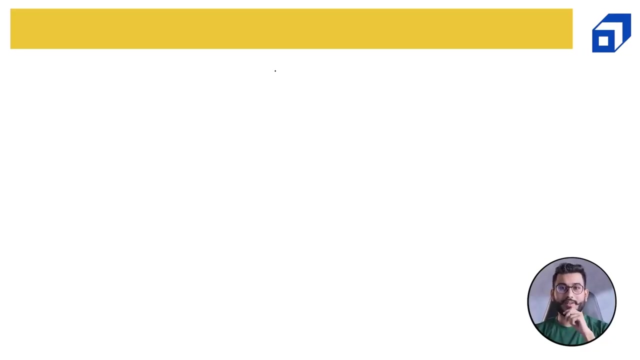 first module of statistics and probability full course. in this particular video, we'll be talking about introduction to statistics and descriptive statistics. we'll be also talking about measures of central tendency and measures of variation. so let's get started. so let's start with first of all talking about statistics. now, if we talk about statistics, 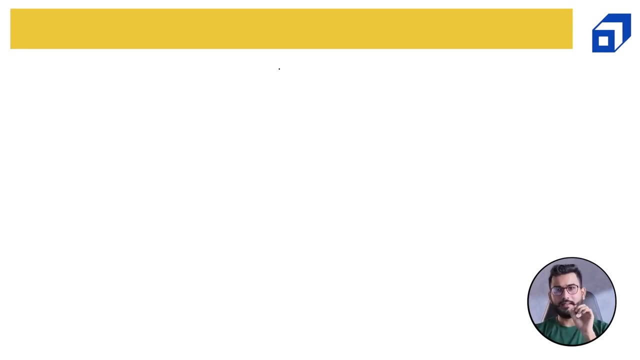 statistics is broadly classified into three major categories, so let's discuss about them, and I'll be writing all these notes. so if you feel like increasing the speed of this particular video, you can do that, but I'll be going in my very normal, normal pace, so you can just adjust your. 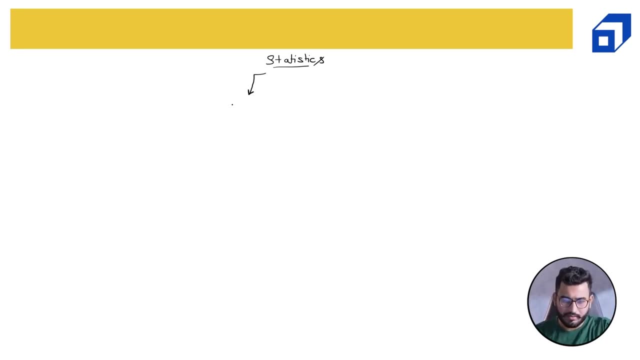 speed about this video, as you like. so statistics: the very first category is descriptive statistic. then we have inferential and finally hypothesis. we'll be looking at all these three segments in a very detailed way, but let's start by understanding a little bit about each of these categories. so we will briefly talk about 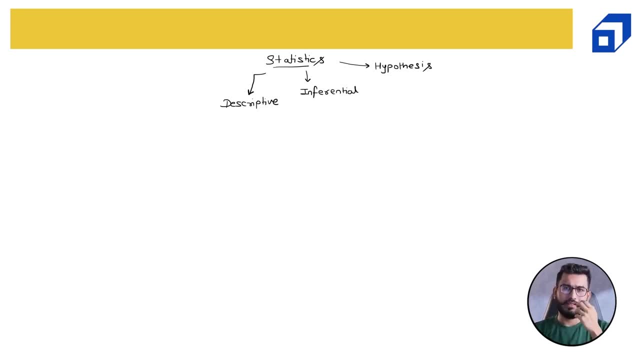 what is descriptive statistics, what is inferential and what is hypothesis? let's first take some random data. let's say we have this kind of data, so we have the data of that's a few students with their student ID, the name of the student, their marks and, let's say, their age and from which city they belong to. so 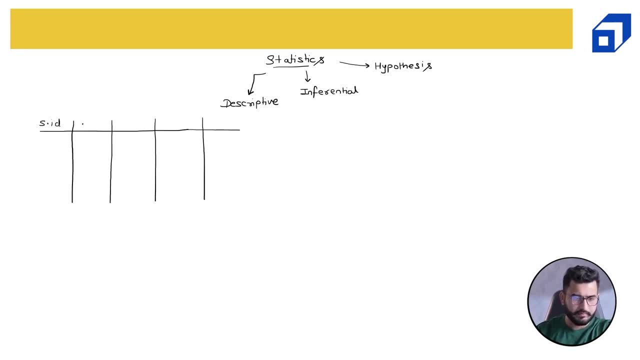 for the student ID. I'll just write SID, then name marks, age and city, and let's say we have few data points, let's fill this tables with some random data. so 0, 1, 0, 2, 0, 3 and so on till 0. 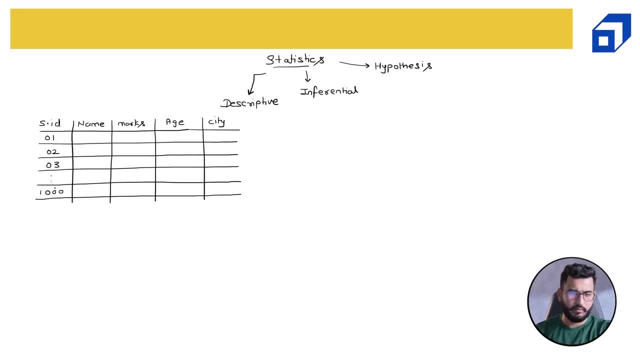 let's say we have some thousand students, so 1000 name is, let's say, Sumit, maybe Ravi, Sanju and Ankita. then we have marks. let's say one, one hundred ninety five, eighty two, maybe this is 60. then age: let's say 29, 28, 25. 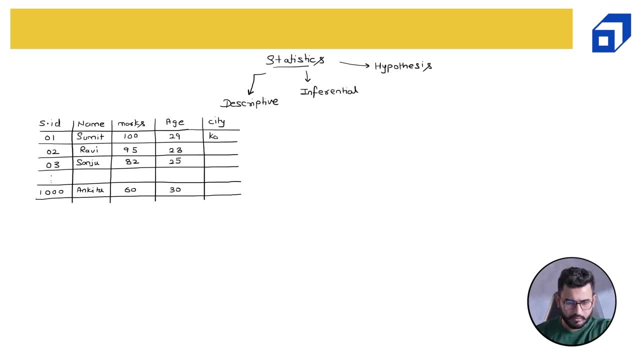 and 30 city, so I am from Kanpur, then Ravi may be from Bangalore, then maybe this is Chennai and finally Ankita from, let's say, Jamshedpur, so we can just write Jamshedpur. okay. now, given this particular data, we have to understand. 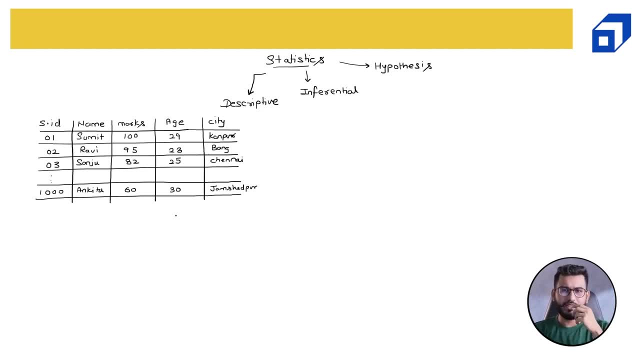 this data. so if your manager or maybe, let's say, the principal of a particular school is asking you to summarize this data now, you will not be able to provide the information regarding each student, right? so you will not be going to your principal, or maybe the head of the school, to explain. 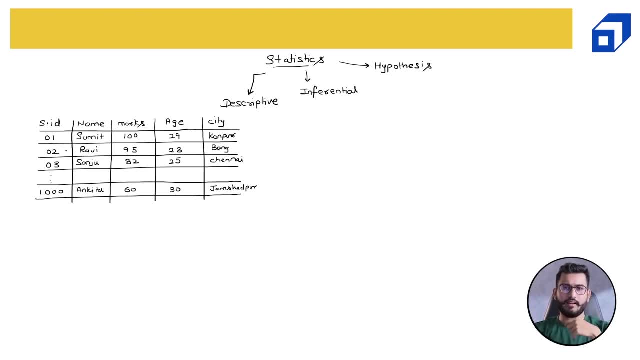 the person that, okay, we have Sumit, we have Ravi, we have Sanju, we have Ankita. the marks of Sumit is 100, the marks of Ravi is 95, the marks of Sanju is 82. it will take a lot of time and it is also not feasible, and the head of the school will not be having this much. 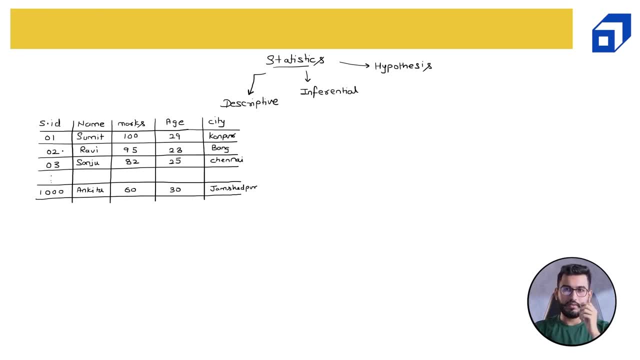 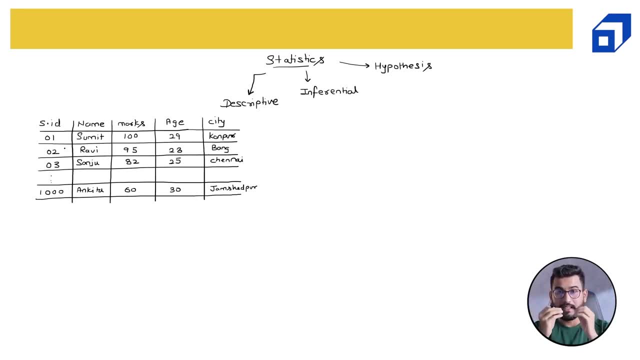 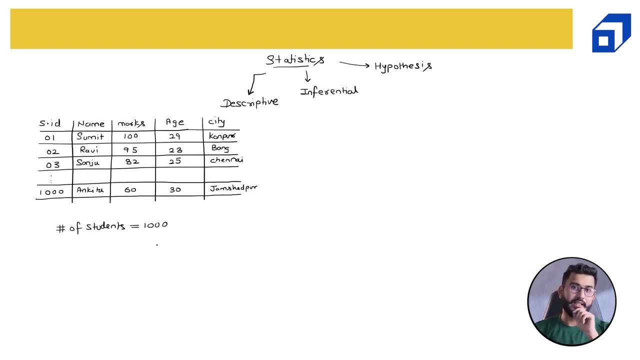 now, this is a statistic which is describing the class and hence descriptive statistic. let's say, the average marks of this class is 85. again, this number, just this one number, is describing the complete class and we will be talking more about what average is, but this number is talking about. 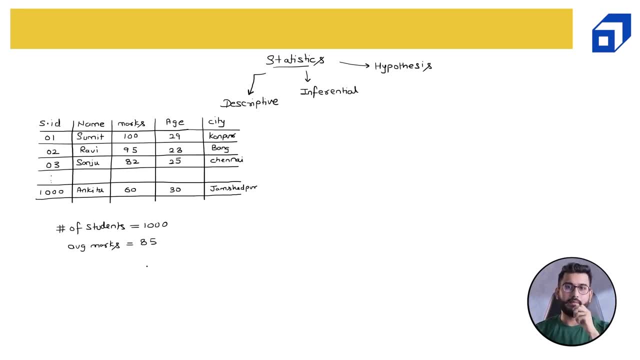 the complete class and hence this is a descriptive statistic. for example, let's say the average age is, let's say, 25, similarly maximum marks. then we have minimum marks. so all these numbers which describe the data in such a way that we just need this number to explain the complete. 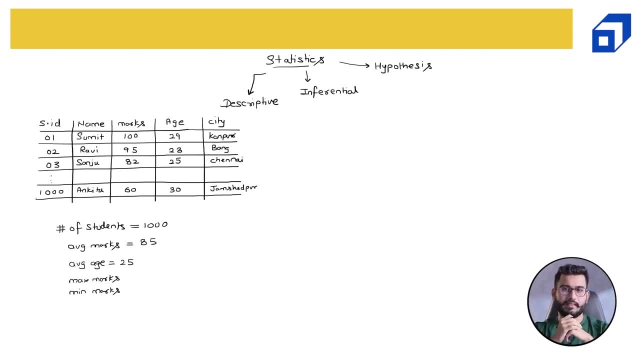 data points Is basically known as your descriptive statistics. it's very simple to understand right now we have. descriptive statistics can broadly be classified into two kinds of measure, So I'll just change my color and we'll write over here. So one is known as measures of central tendency. 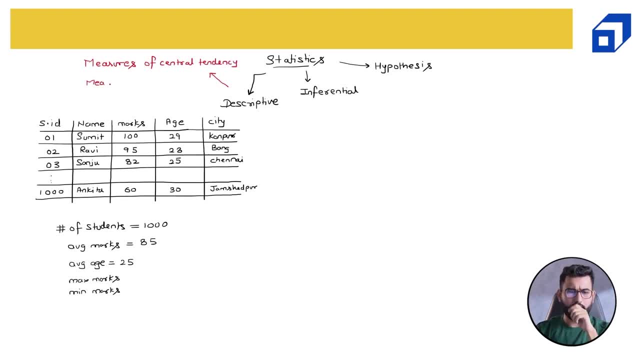 And then we have measures of variance, Or you can say it is measures of variation, So I'll just simply write it as measures of variation. So we will be talking in detail about what are the various measures of central tendency is and what are the measures of variation is. 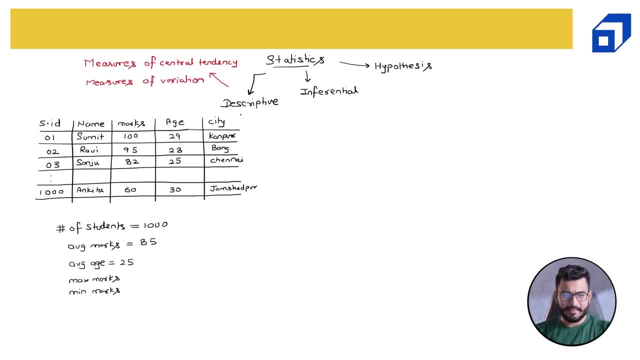 So what we have learned regarding the descriptive statistics, It's basically Those Metric, So those metrics that can define the complete data, or that can help us define the complete data. we do not need to look into each and every row. we do not need to look into each. 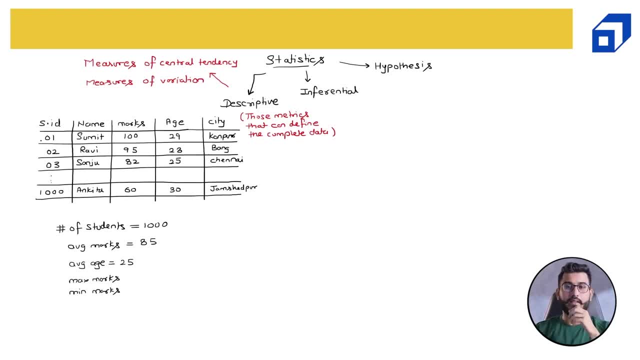 and every information. remember, in a particular data, which is cross sectional, having rows and columns, Each row is known as the information, The information. So, using the power of descriptive statistics, we do not have to go through each and every information. we can just use these metric to describe the complete data, right? 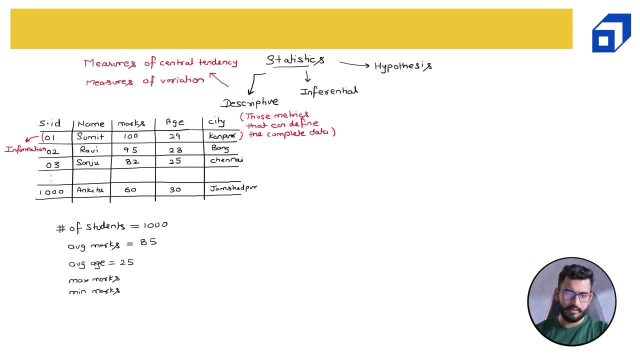 Then we have inferential. Now how we can understand inferential? So I'll just quickly change the color And We'll take one example. Let's say that is company. Let's take any name of the company. Let's say there is a company known as Scaler. 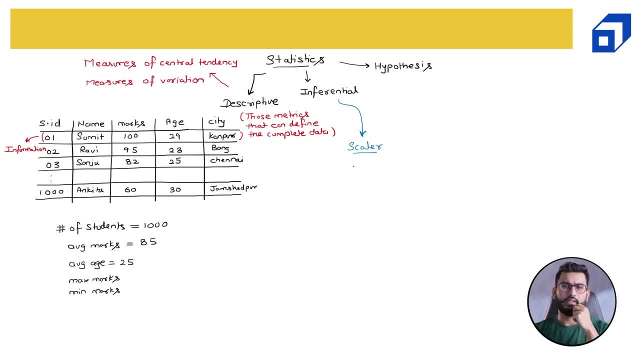 Now Scaler wants to know, on an average, how many hours a student is studying in 12th class. So what's the question? How many Hours A student Studies When the student is in 12th class. so I'll just write in bracket 12th class. 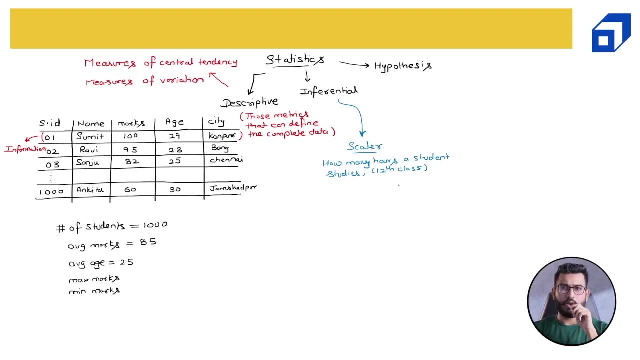 Now, if I look into this problem overall, there will be millions of students in India, right, And if I just limit my scope of study to India itself, So there will be a lot of students in India, Right, And there will be a lot of students that will be present in India right now. 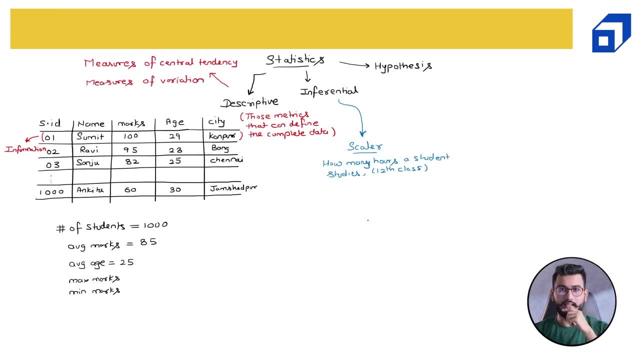 Those who will be in 12th class right now. Right, And it is impossible for any company to perform survey in such a large scale. So let's say, if, if Scaler has to get this number, Scaler has to basically get a average number. 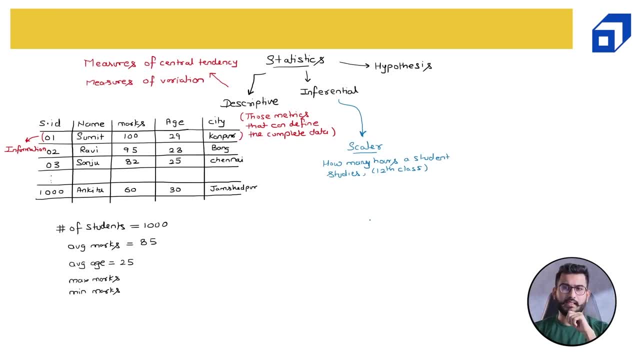 So I'll just write average, how many Average hours So how many, Or maybe just simply write that's what's the average, So how many Hours Hours So how many Hours, Hours, Hours, Hours, Hours, Hours. 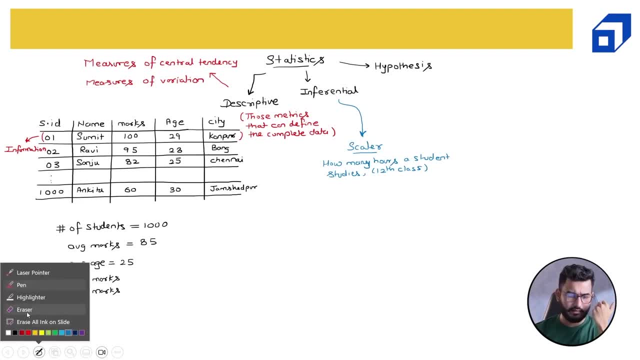 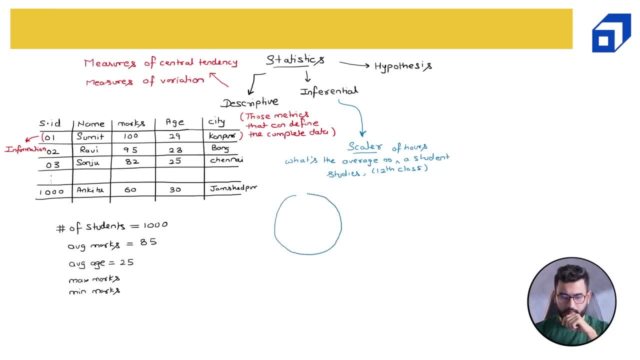 So let's say this is my complete population, Right? all the students who are in 12th class this year. so 12th class students. now there will be so many students, right? or? if I just have to take a number, let's take there. 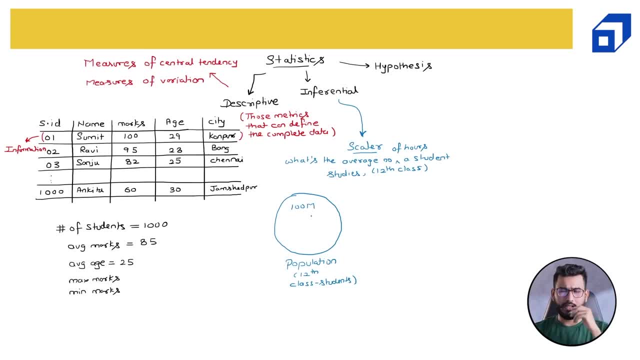 are 100 million students. I'm just throwing a number. so 100 million students. in order to get this statistic, which is what's the average number of hours, I have to reach out to each and every student. so let's say the entity scaler is performing the survey, they will. 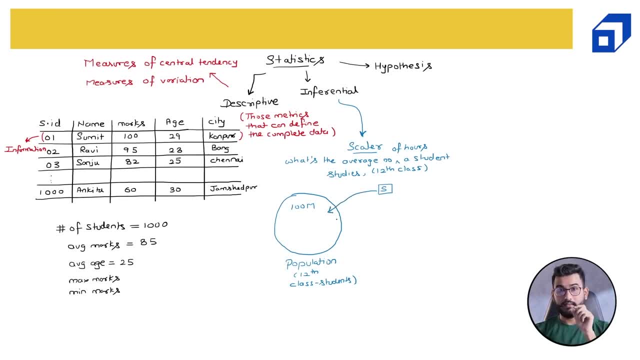 reach out to each and every student. they will ask the student whether the particular student is suffused for 1 hour or 2 hour, 3 or 4 hour or maybe n hours. then we will collect the data. the scalar team will collect the data. so let's say we have the data of a student number. 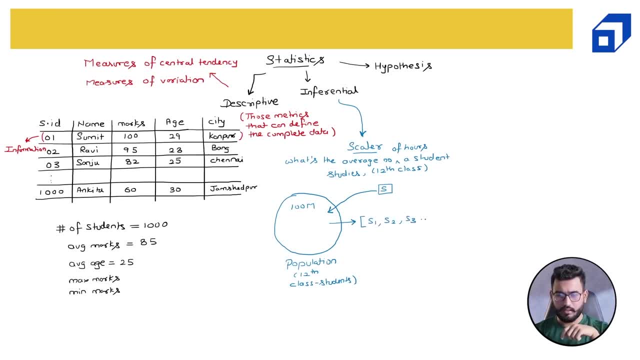 one, student number two, student number three and so on, till student number 100 million. now, once we have this data, we will take the average and that is basically my output that i'm looking for. now, if we practically look into this procedure or into this problem seems like this is practically impossible, because it is practically impossible for any company. 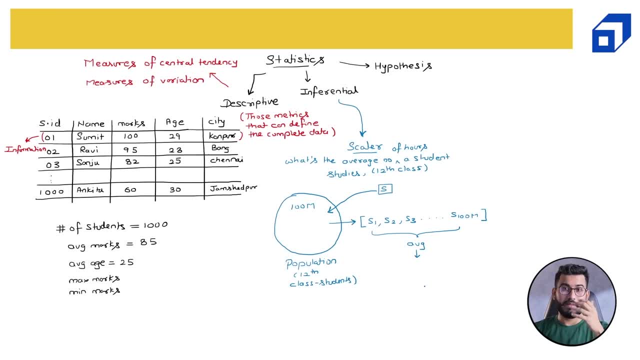 or individual to reach out to these many people, or to reach out to these many observations or entities or individuals, you can call it any, anything right, if even it is possible. it requires a lot of time and lot of money, lot of investment. so what are the practical problems? 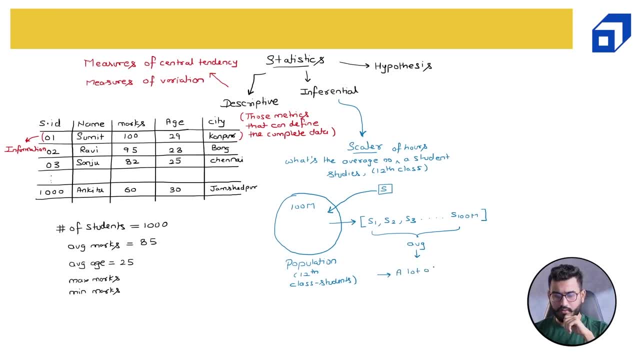 number one: a lot of investment, a lot of time investment. similarly, a lot of cost investment, a lot of lot of cost investment. so we have to invest a lot of time and none of the companies having this much time. so what is the practical solution for this? well, the practical solution is very simple. 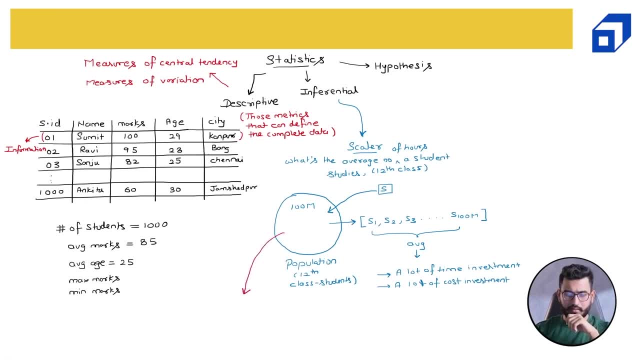 what we are going to do. we are going to take some few students, which we call as the sample, and we will also talk about how the sampling is performed. when we will be discussing about inferential statistics, we'll be talking about how sampling is performed. so let's say we are having a simple random sample and the 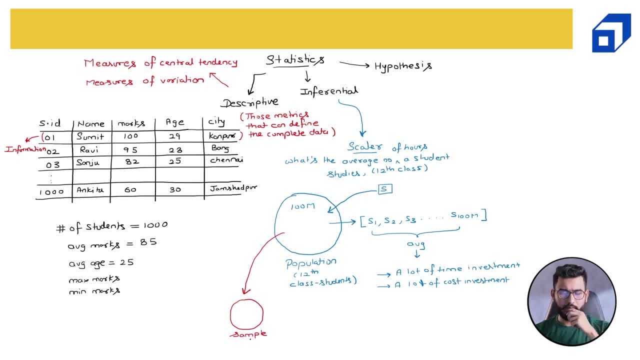 term simple, random sample will be. i'll be explaining you in a better way, so don't worry. so let's say we are having a sample. i have taken some random students. let's say we have taken 100 students from uthara pradesh. we have taken 100. 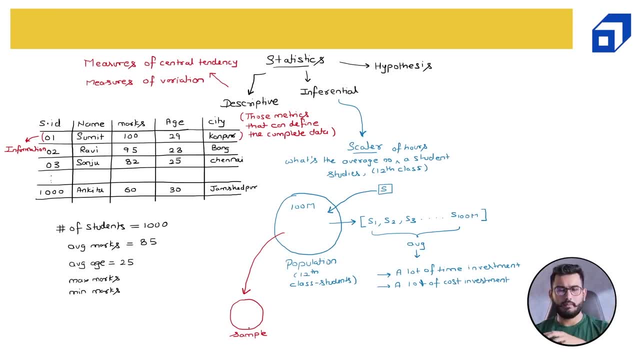 from, let's say, andhra pradesh, 100 from tamil nadu, 100, 100 from delhi ncr region. so, like this, we have created a sample and let's say, this sample is having around one lakh student, one lakh now, in order to perform survey on one lakh people seems quite quite practical right. 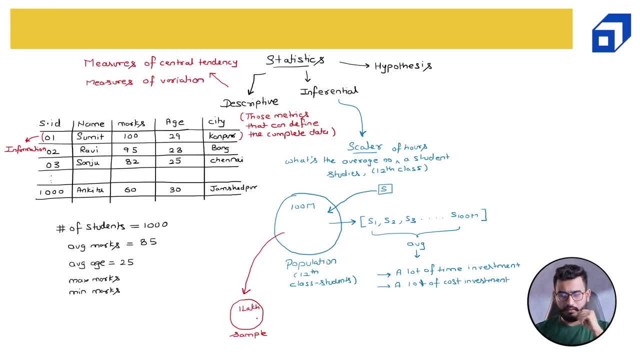 we can perform the survey on one lakh people. so let's say, after performing the survey on one lakh people, we have the data with us- s1, s2 and so on, this till s1- lakh, and now we can take the average. once we have the average, this is known as the sample average. so we 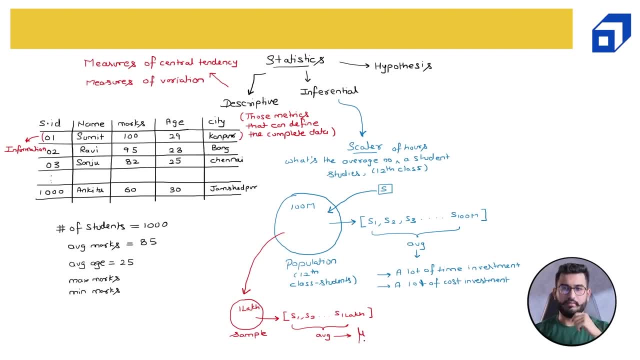 will just write mu. mu is a greek letter which is commonly used to represent average, so average, then i'll write s sample average. i'll just write it in brackets. also: sample average. now. inferential statistics is a branch of statistics which deals with approximating the 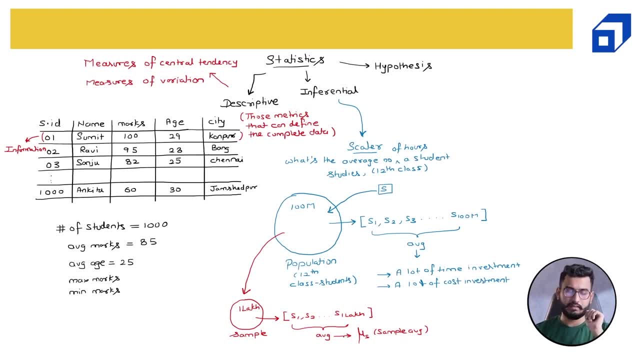 population average or population parameter. uh, remember one thing: if i am talking about the average of population, it is population parameter. if i am talking about the average of sample, it is sample statistic. so there is a difference. so please remember when i'm when i'm saying a statistic, i'm basically talking about sample. 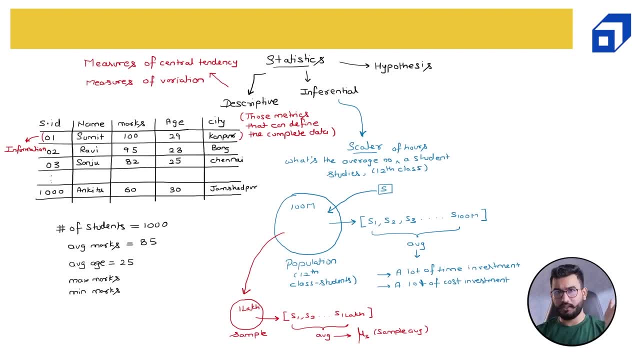 because practically it is impossible to do anything on population. there are two problems: either we are not able to reach out to all the data, or we are not able to reach out to all the data, the observations in the population. so if I ask you, find out the average of average. 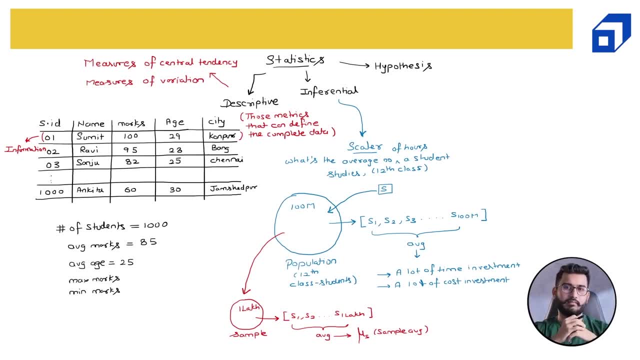 height of Indian men. now, it is impossible for any individual to reach out to each and every Indian male, right? so that's basically my population and if I can get that number, if I can get the average age of all the Indians in this, all Indian males from India, then that is known as the population parameter. okay, 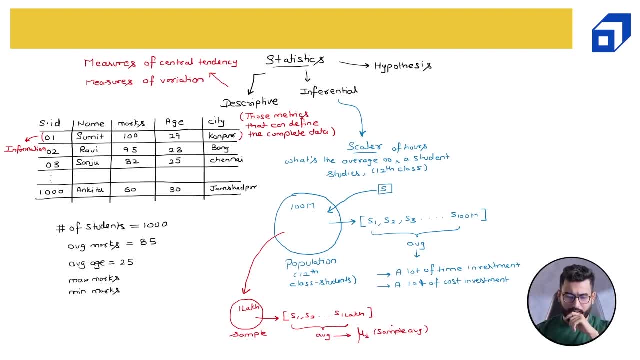 so inferential statistics. coming to our point, inferential statistics is a branch of a statistic which help us to perform approximations. so, using this sample statistic, I will try to approximate the population parameter. so let me just quickly write it over here: using sample statistic, we will try to. 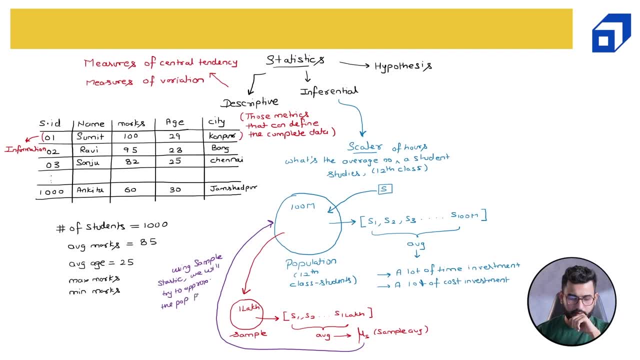 approximate the population parameter, and that is basically known as these inferential statistic. now, there are some procedures, we have some parameters, we have some parameters. we have some parameters. we have some few formulas. we will be talking about that, but this is basically the belief idea behind why we need inferential statistic. okay, the last portion, or maybe 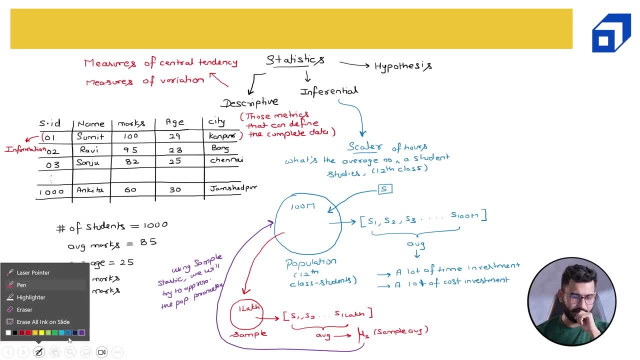 the last segment, which is known as the hypothesis testing. when we talk about hypothesis testing, as the name suggests, we are trying to test something. now, what we are trying to test? we are trying to test something that is which has been proven, or maybe a claim, or maybe an statement there can be. 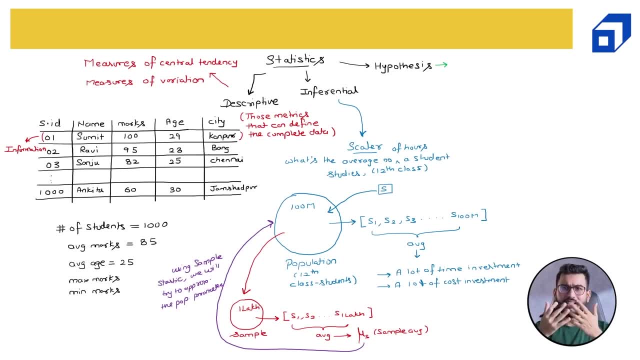 anything that we are trying to test. let's take one very general example. so you guys would have watched this Dettol advertisement which says that Dettol kills, or Dettol soap kills ninety, nine, point nine percent of the germs. right now let's say you are suspicious about it. you are suspicious. 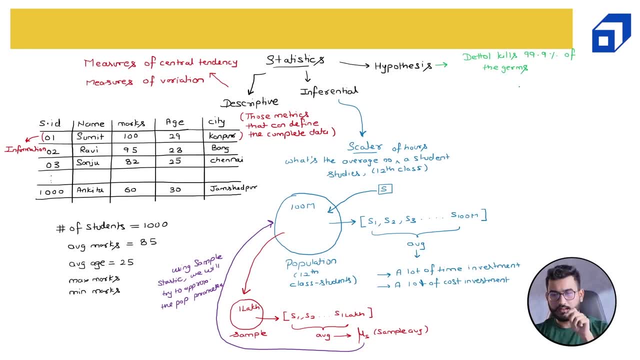 you wanted to test whether this claim or statement made by the Dettol company, is it having some statistical significance or not? is it statistically correct or not? and that is where the power of hypothesis testing comes into picture. so we will try to test here. we perform test to check if a 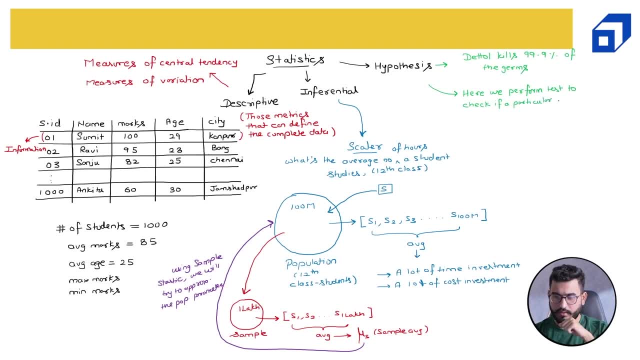 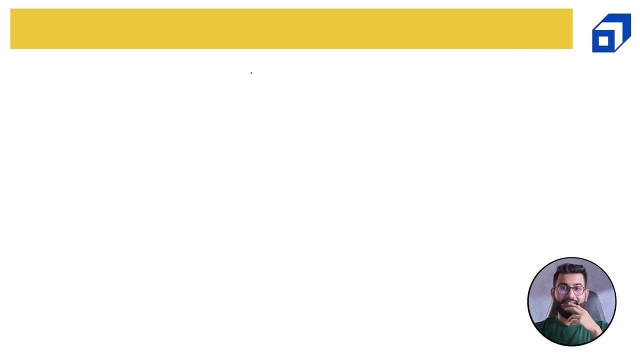 particular, if a particular claim or a statement can be statistically proven and can be statistically so. these are the three major segments which we are going to discuss now. before we jump into any of these segments, we have to understand what kind of data we are working with. so we will be briefly talking about how we can explain our data, and when I say explain, 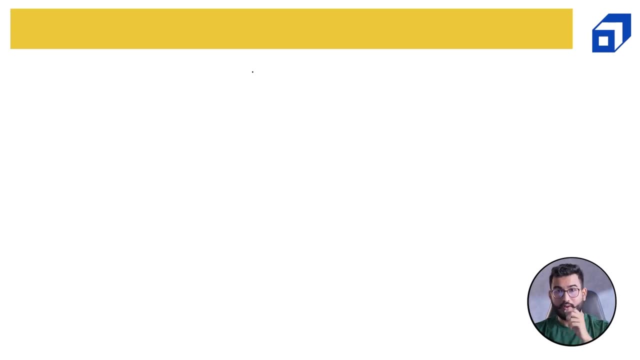 our data. what are the various types of column or variables we get in a data? so let's talk about it. we will be taking one very random example, so let's just quickly create a data. again. we can extend the same example that we have taken in the last slide. 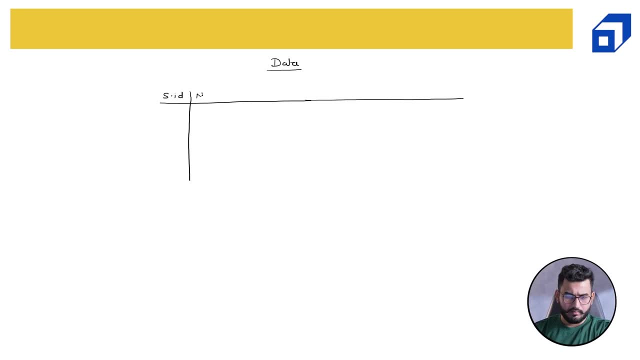 we were. we were having student id, the name of the student, salary, age, or instead of salary let's put marks: age, then city, then we can go about writing grades and maybe subject. and then we can go about writing grades and maybe subject, And finally we can talk about the gender. 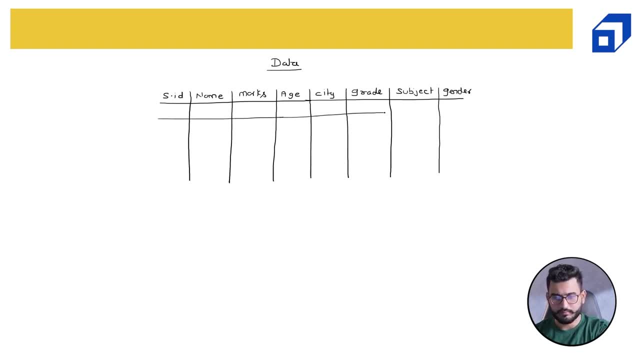 Let's fill this table with some few data points. So let's say we have 01, 02, 03, 04, name is Sumit Amit Ajay. Ankita Mark says, let's say, 89,, 98,, 95 and 62 ages. 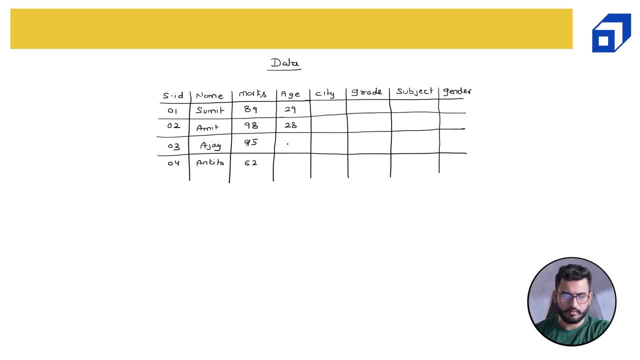 29,, 28,, 25 and 30, so TA is let's say K and P, B and G, R and C, and let's say TA, TA Then grades A, B, C and B subjects. So let's use A. 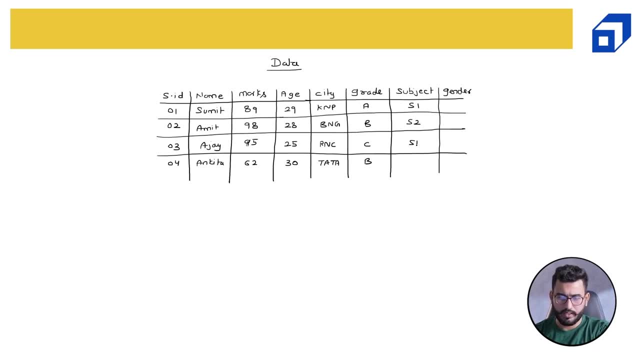 S1 as subject number one. S2, S1, S3, gender- male male, male female. Now, this is my dummy data. Now, if I ask you, are you guys able to observe any kind of distinction among all the kind? 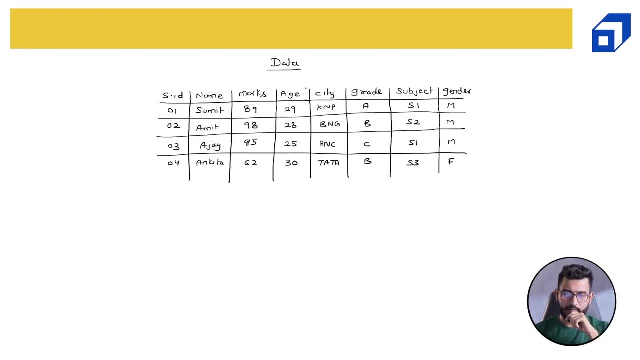 of variables that we are having in this data. So remember These are. these columns are also known as, so these columns are also known as the variables, So I may I may be using the term variables or columns, And, as I have told you that each row is basically my group of informations, 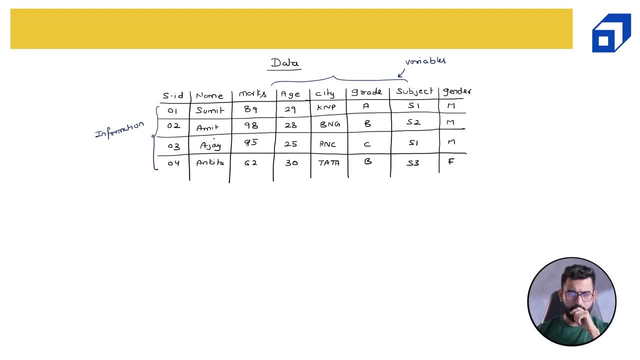 So each row is my information. Now, if I carefully observe, Marks age. these two columns are my numerical columns. And why I'm calling it as numerical? Because the data, which is which these columns are holding, are the numbers. These numbers are something that lies between a minimum and a maximum right. 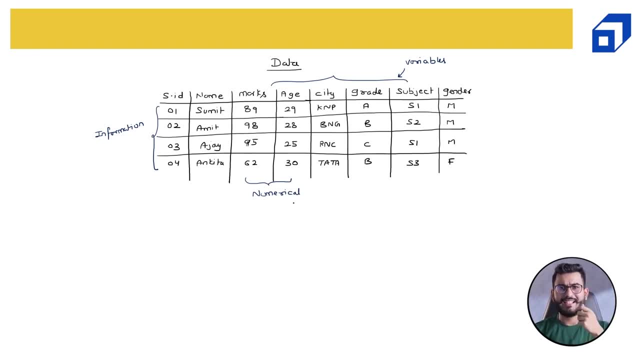 So marks can be between 0 to 100.. Age can be between- let's say so, since it is a school, let's take 25 to 35. Then, if I talk about city grades, subject and gender, all these are my categorical columns. 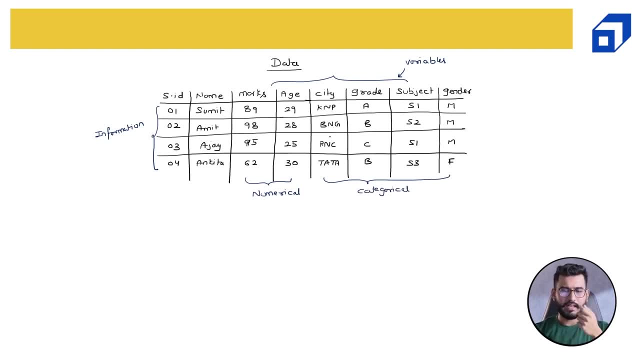 categories because city is having Kanpur, Bangalore, Ranchi, Tata. These are all categories right Grades: A, B, C, D Categories. Subject: S1, S2, S3, etc. Gender: Male, female category. 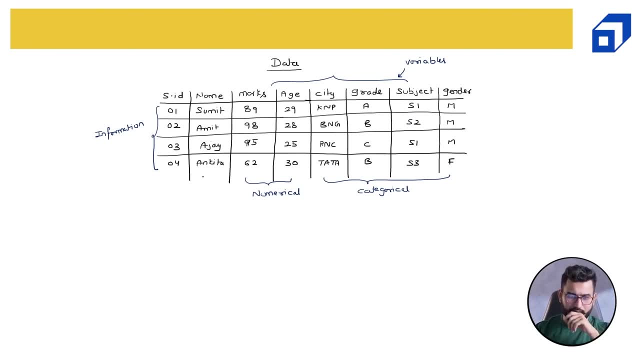 Similarly, this name is a categorical column because each name can be termed as a category. Student ID is a identity column. It is neither categorical nor numerical, So I can just complete call it as an identity column. Now there are like, in order to better explain these columns, 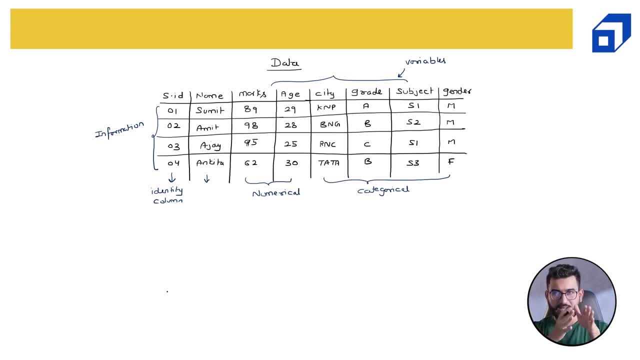 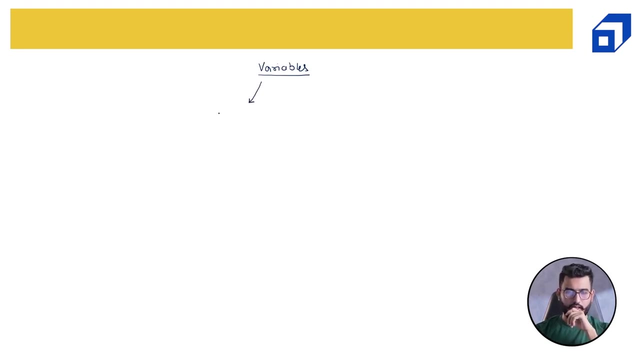 We have a formula, We have a functional name given to all the numerical columns and all the categorical columns. Let's talk about it. So, when we talk about variables, it is formally divided into qualitative and quantitative. Now, Qualitative Data is basically those columns which consist of non-numerical data. 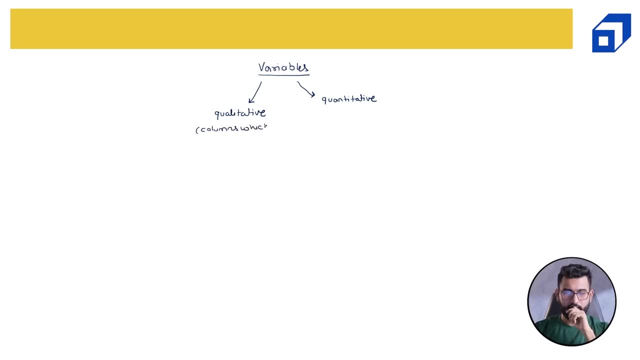 So columns which consist of non-numerical data, That's basically my qualitative data. Quantitative Data Is Those columns Which consist of numerical data. So simply, I'll write numerical data, Numerical data. Now, within qualitative, there is a further distinction, which is your nominal and ordinal. 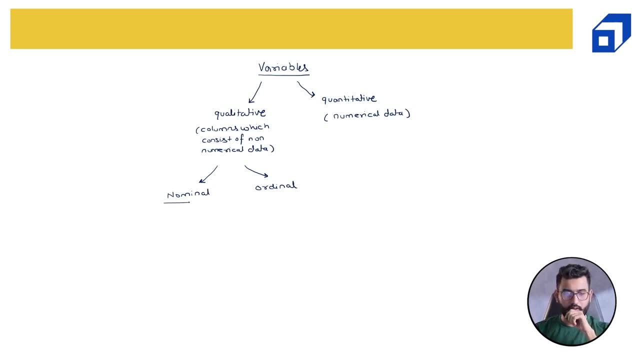 Now, what is nominal? So when we talk about nominal, These are which consists of categories. that does not comes with any kind of order among the categories, for example. I'll first take example, for example, city. let's say there is a column city and the column is having categories as Kanpur, Delhi and 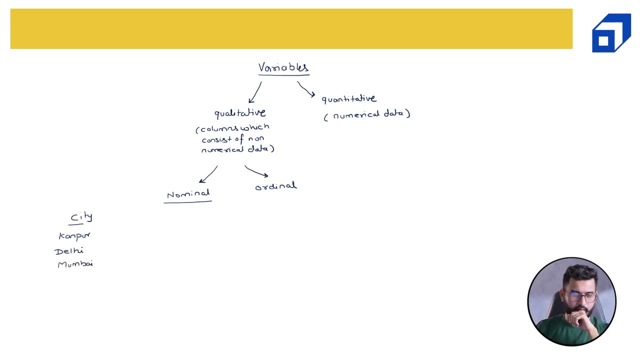 then Mumbai and Kolkata. now I cannot say that Kanpur is better than Delhi, Mumbai is better than Kolkata, because these are four distinct categories. they they do not have any kind of orderness among them. so this is simply the nominal categorical variable or nominal qualitative variable. so I'll just write: 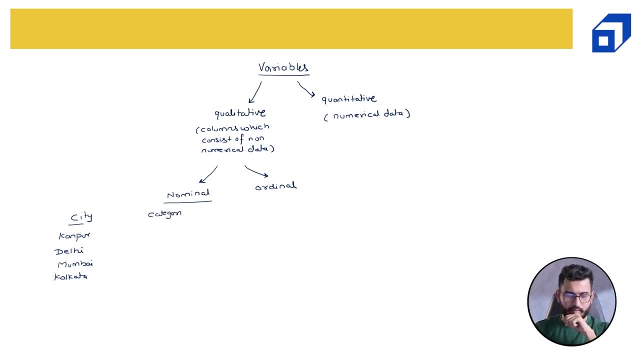 down number of categories and then I will point it out and then I will rank the definition. categories that does not follow order among them are basically known as nominal data, ordinal data. you guys would have already guessed it. it is basically those categories that follow orderness, orderness among them, for example, grades or 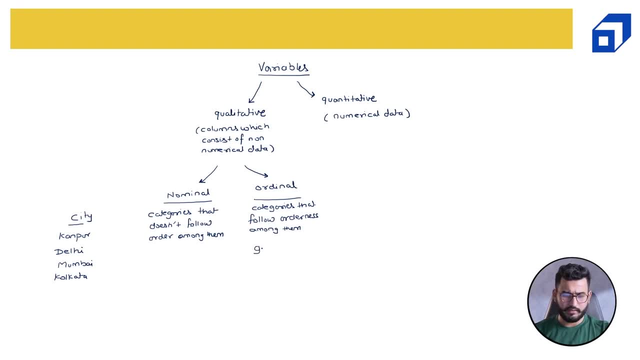 for example, I will if I say: yeah, grades is the best example, so grades, so a grades can be a, a, a plus, or maybe I should write a plus first. so let's take a, b, c, d, a, b, c, d. now we know that a is better. 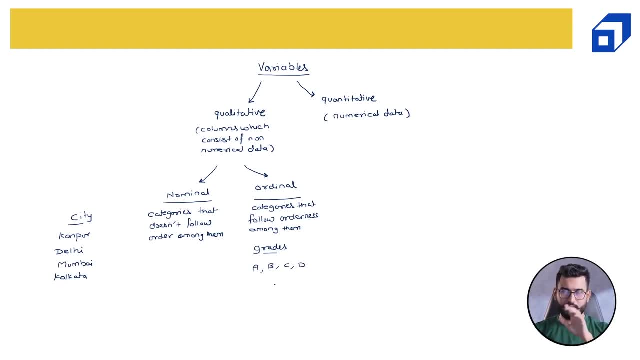 than b, b is better than c, c is better than d. so there is some orderness among these categories and that's the reason. ordinal data. we can also talk about class, like first class, second class, third class, fourth class, so there is orderness if I talk about, let's say, your educational. 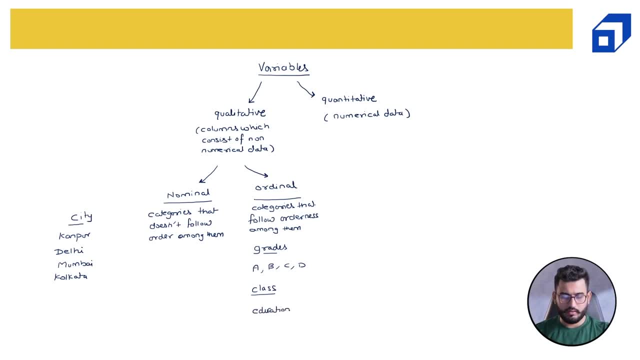 qualification, educational qualification. so let's say a person is graduate, a person is a post graduate, a person is intermediate. so I know that high school, then we can have intermediate, then we can have graduate, then we can have, then we can have graduation and then post graduation. so these are the four categories which will definitely 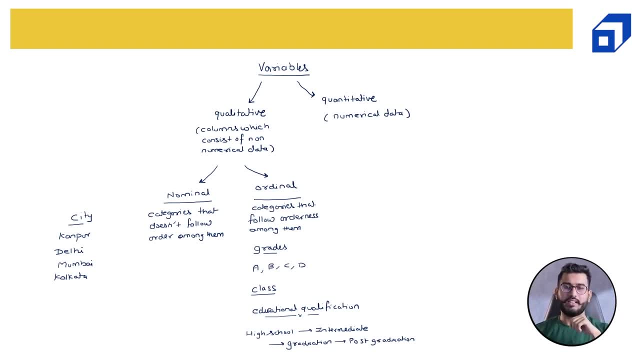 have a order among them. so these are known as the ordinal qualitative variables, now quantitative as the name suggests. these are those variables which can be quantified. quantitative means quantified. we can extract some quantity out of it. for example, minimum, maximum, we can perform addition, subtraction, so we can apply all those mathematical operations on these columns. and after applying, 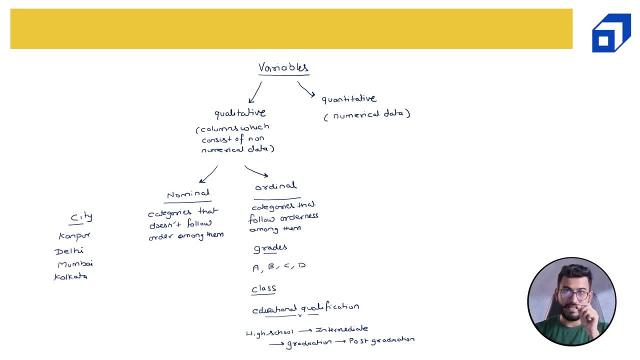 the mathematical operations, the value will still make sense because they are qualitative, sorry, quantitative. now quantitative are further classified as number one: quantitative. and then let us move on very briefly. so some element that we like to speak about, Suppose inside the number of students who, after heading, we will connect it into second column, which 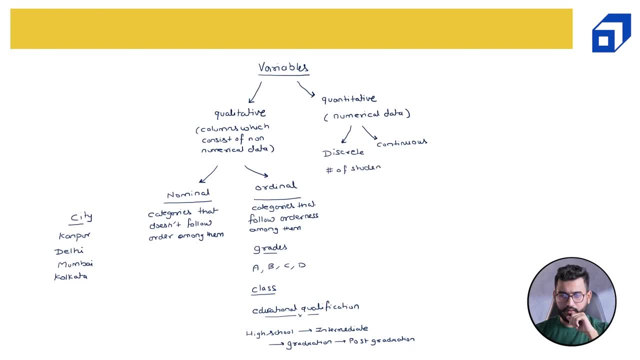 is singled out. we will represent the number of students with dare. then we can also know if this students might be either low income, a nghir or a huge income, or female. максимize a class. now we know that a class can have two students, three students, four students. 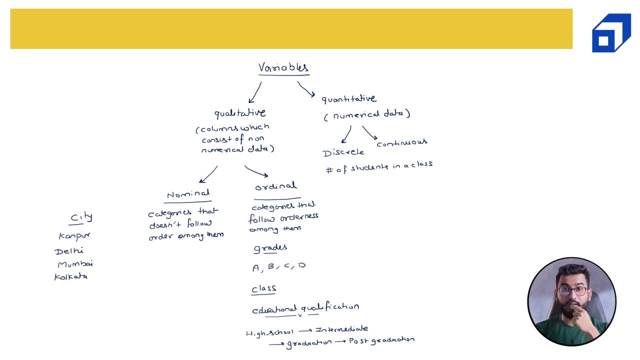 hundred students, 200 students, but a class cannot have 22.57 because this practically does not make any sense, right? so this is discrete quantitative variable. similarly, number of citizens in a country. again, it will always be a natural number which is countable and finite. so I'll just quickly write it in a bracket: countable and finite when we talk. 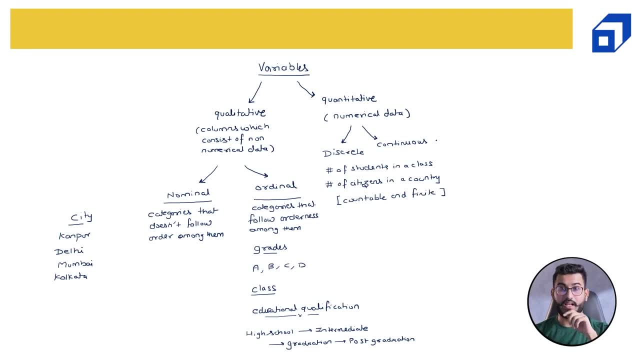 about continuous. these are those variables which are non countable or uncountable, and infinite and infinite. Let's take an example and it will make better sense. For example, let's take income Now. income of a person can lie between a minimum and a maximum value. 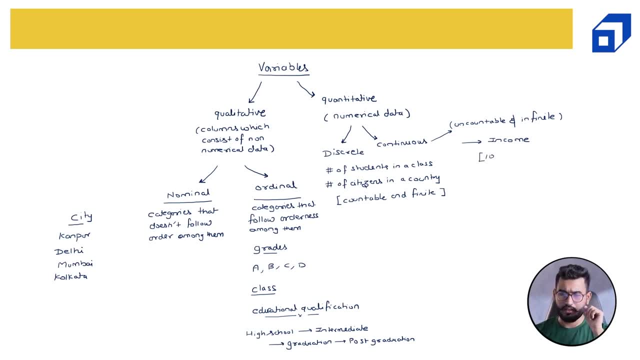 For example, purpose. let's take the minimum income is 100.. The maximum income is, let's say, 1 million. Now, between these two numbers, I have infinite number of observations that are valid. Can a person earn? let's say 100.15. let's say these are in dollars. 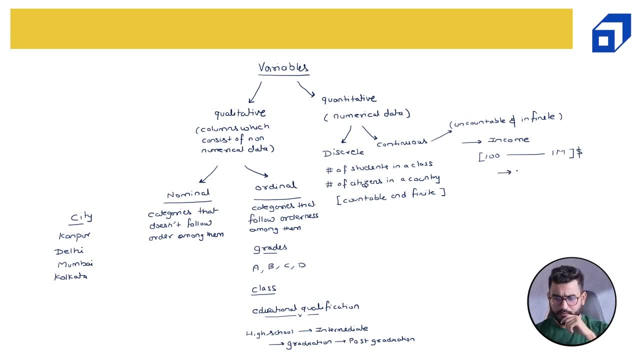 So it will make more sense. So is a person earning 100.15 a valid income? Yes, Is a person earning, Let's say, 100.15.. So 1 million, or let's take a smaller value so that you guys can understand it. 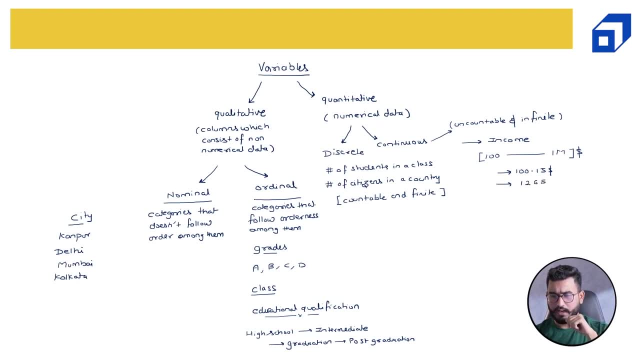 So let's say 1265.778.. I'm going very like I'm taking more decimal values just to make make you guys understand that this is also a possible value which can, which can exist and which is practically possible. So a person can earn this number also. 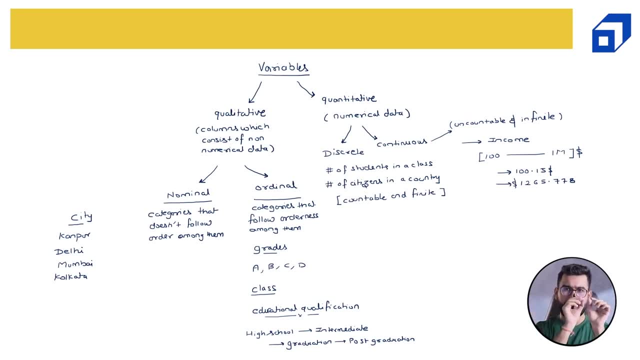 Right. So between 101 million, I have endless possibilities and each possibility or each observation is possible to exist. Similarly, we have age. Now let's say our minimum age is 27, maximum age is 35. Can I have a person with the age 27 years 5 months? 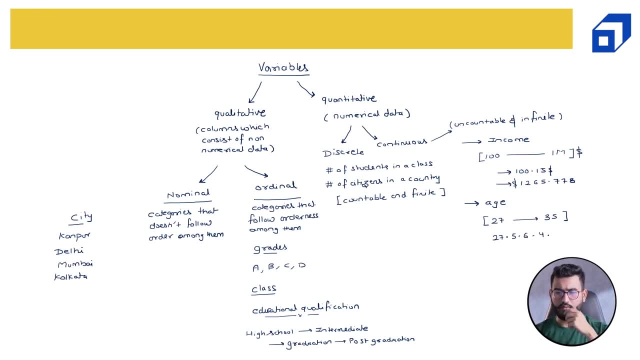 6 days? No, Can I have a person with the age 27 days? 4 hours, 5 seconds, 6 milliseconds, 7 nanoseconds? Yes, Practically possible. So at every nanosecond I can have a particular observation that can lie in this scale. 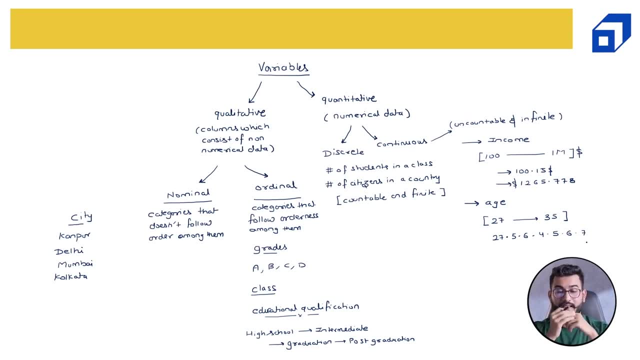 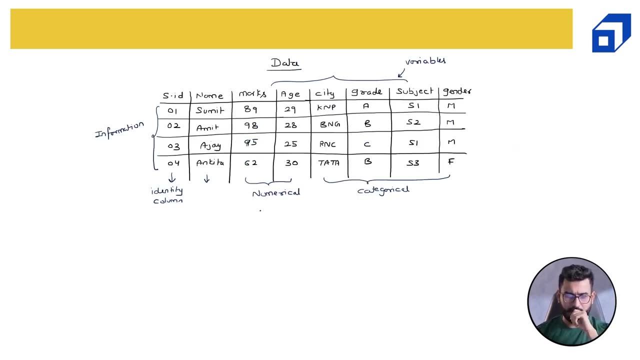 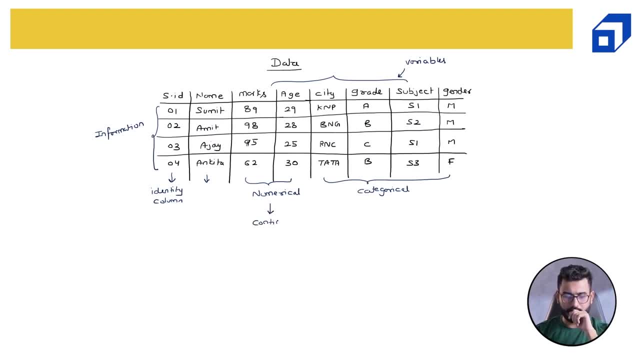 They are your continuous quantitative. Similarly, if I look into grades, they are qualitative, but it is ordinal. Then subjects, They are qualitative, But it is nominal. Similarly, grades, gender: qualitative nominal, because I cannot say male is better than female. 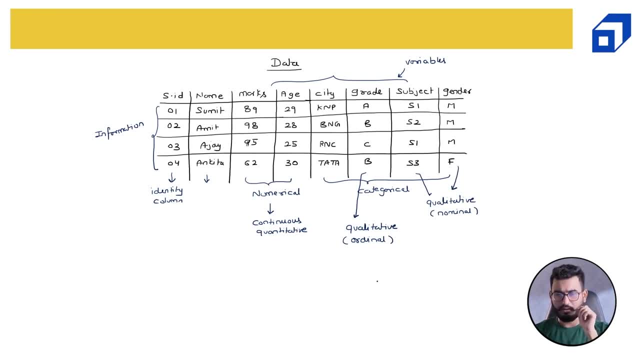 or female is better than male. So these are two categories. and it is nominal City, again qualitative nominal. So I'll just write Q, hyphen N, so name: again qualitative nominal, and I have already told you. that. So student ID is basically an identity column. 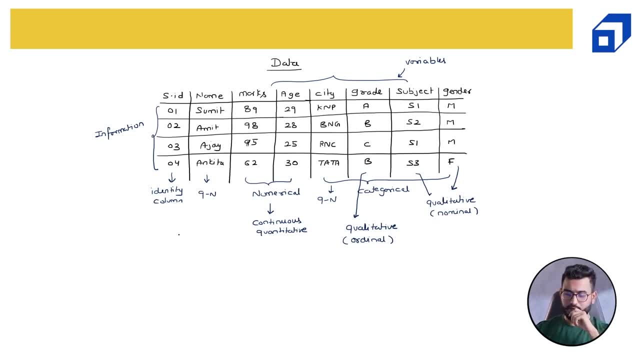 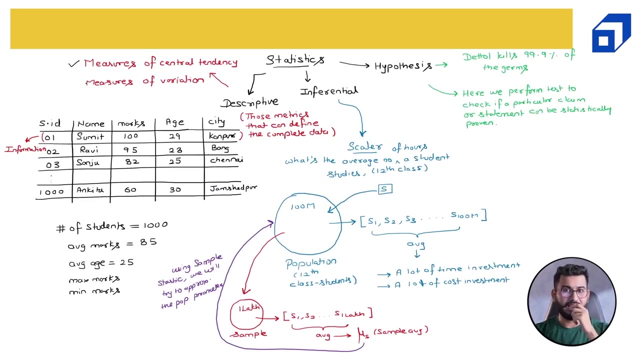 It is neither qualitative nor quantitative. So this is how we describe our data into various types of variables. Now we are going to talk in very much detail about what are the various measures of central tendency is and what are the measures of variation is. So, with this particular topic, we will initiate the first. 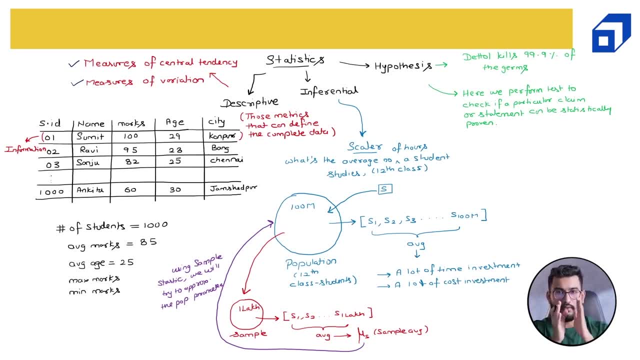 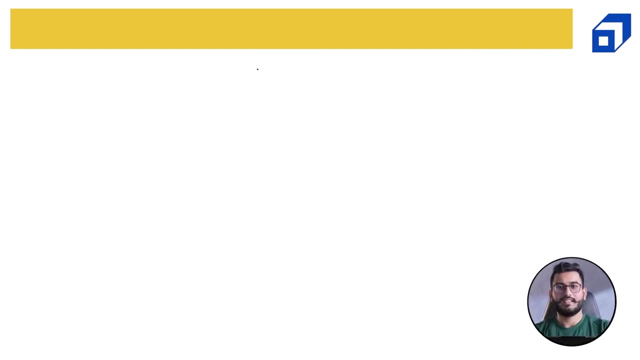 Category, or maybe first group of discussion or the first branch of our discussion, which is talking about descriptive statistics. Now let's try to understand what is descriptive statistics. As we have discussed previously that descriptive statistics is all about describing the data in one number or in few statistics. 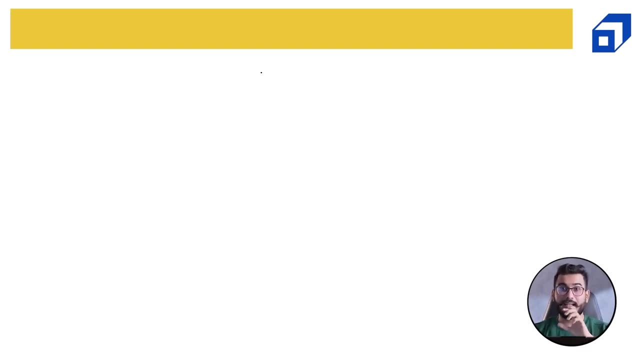 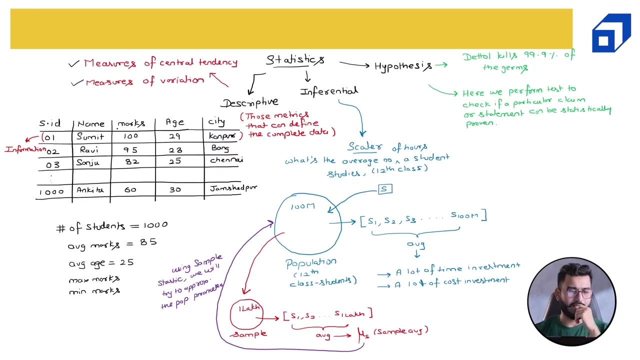 Parameters In such a way that it can describe the complete information. And if I go back to my first slide here, you can see that I was having the data of some students: their name marks, age and city. And if the principal of of this following school ask the teacher that, okay, tell me. 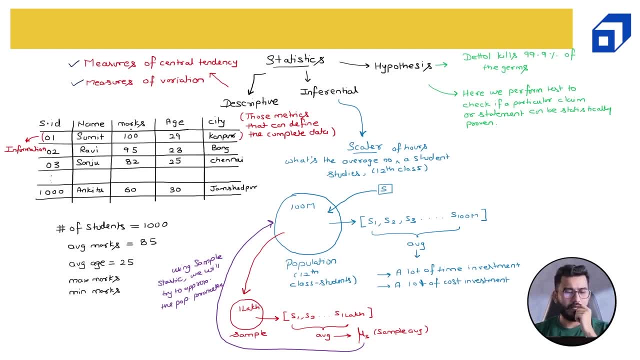 how your class looks like Now. the teacher will not be taking the principal To each and every row or each and every information or each and every detail of the student, So let's assume that if I am one of the teacher, I would not say my principal. that okay, I? 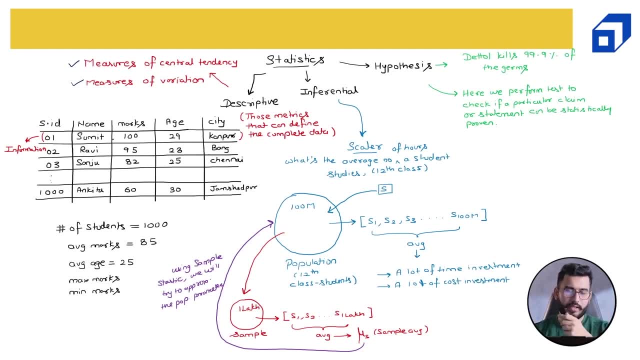 have a class who is having summit, who's a who's ages 29,, whose marks are hundred. And then we have another student whose name is Ravi, who he's from Bangalore. he's he's a 28 years old. 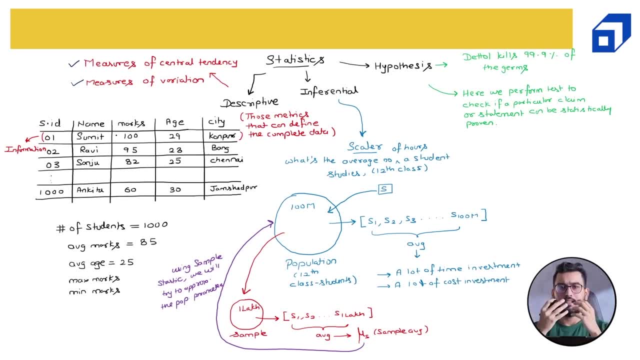 As you can see that, It will take a lot of time and I would not be getting a complete picture of how my class looks like. Right, And that is the reason we have these descriptive measures And, as we have discussed before, the descriptive statistics measure are broadly classified. 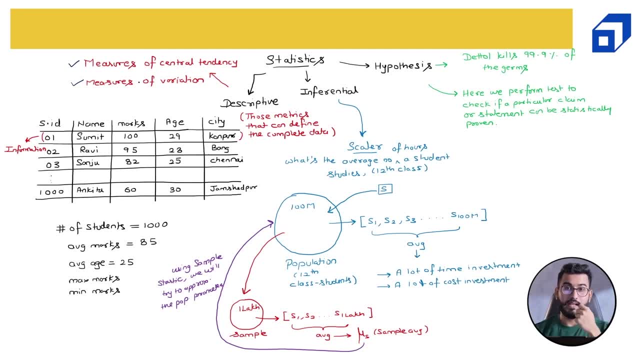 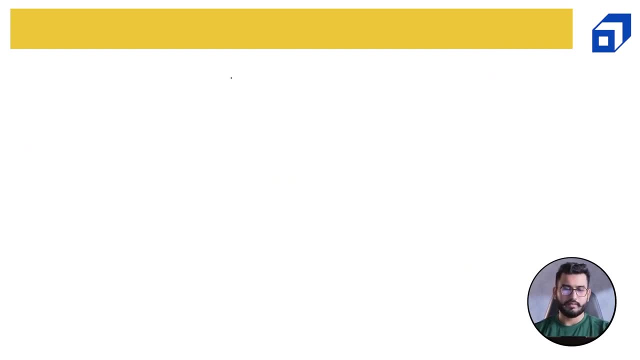 into two buckets. Number one is measures of central tendency and measures of variation. So let's try to Now deep dive into these two particular topics. So descriptive statistics: As we already know that we have two majors: Measures of central tendency, and then we have measures of variation. 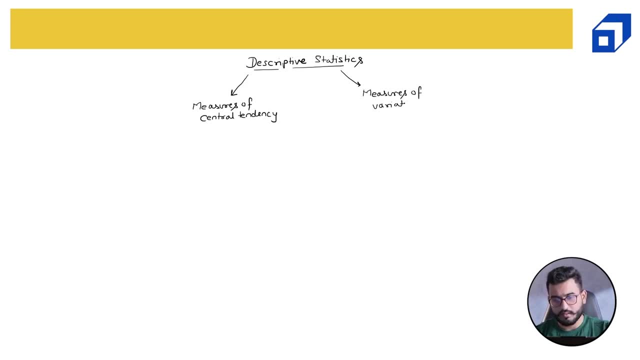 You can also say it's a general tendency, It's not a general tendency, It's a general tendency. It's a general tendency. So that's the general tendency. measures of variance or variation to be, to be in general English. we can call it. 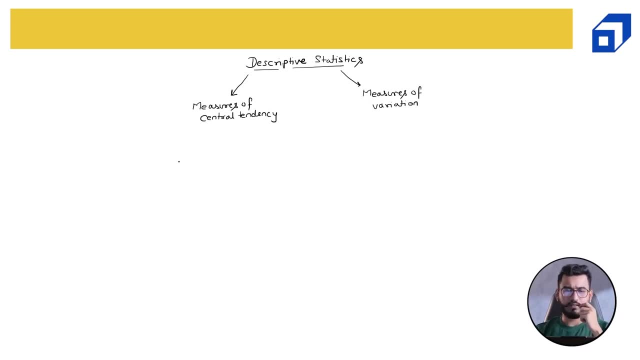 as measures of variation. now, what is measures of central tendency? as you know that, if you, if you carefully read the name, it says measures of central tendency, we are talking something regarding the center. now, is it the center of the data or is it center of my all the observation? let's try to. 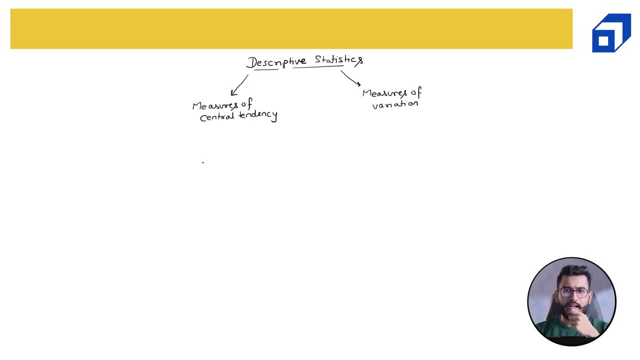 understand. before we can quantify, before we can find out any of these measures, measures of central tendency, we need some data, right? so let's create some hypothetical data of a class. and we have age. so let's say we have age of some 10 to 15 people and let let me just throw some numbers on my screen: so 24. 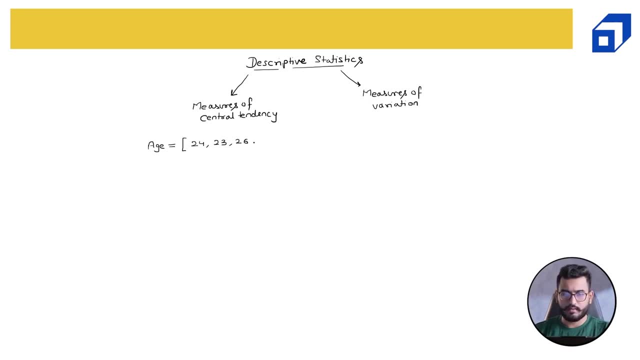 24, 23, 26, then 21, 26, 27, 28, then one more 28, one more 28. okay, let's make it as 26, then 32, 26, 29 and finally 28. this is the data I'm having, that is the data i have here, and all right, so i have this 축 a here. so 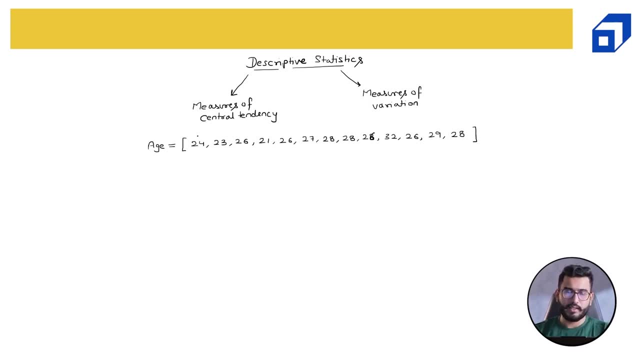 please remember that, guys, and we do have students here, so please make interviews. in this case of the public health crisis, we need what is information about a particular student, not the students. yes, they know about this whole橋. does parents imagine this child remember this story? because we all know? 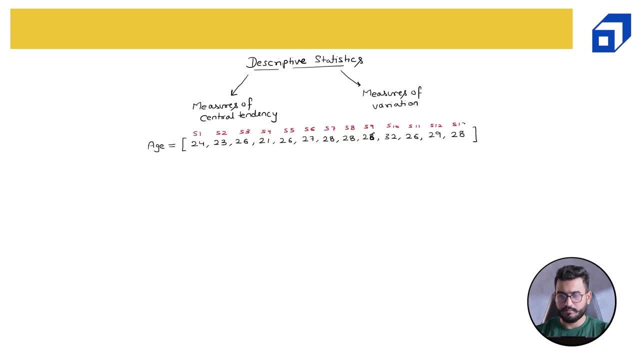 about. we've talked about this example- that, like right now, a student is identical to us. simply joking and beingavoir like that, that is also a characteristic of an other student. yes, that's true, and teadyvhere are going to basis how I can explain the complete data in one number. Well, we would try to extract. 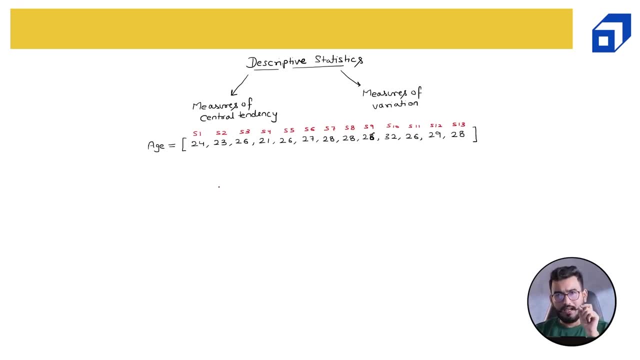 that particular number which lies in the center of the data, so that we know that below this number- So assume that this pen is the center of the data. So I know that below this point I'm having few observations or few students And above this point I'm having few students. 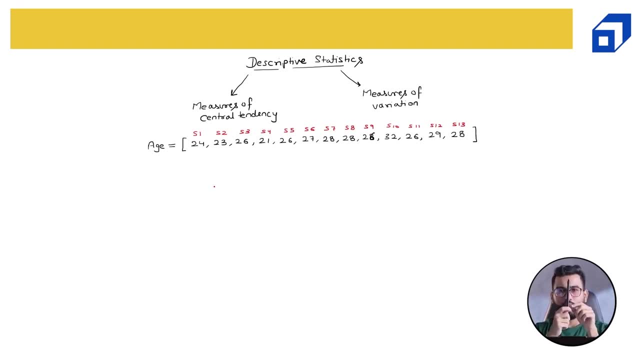 and it will give me a better idea about how my data looks like. right, And that is what the measure of central tendency is. In this particular data, the very first measure of central tendency is the mean, or the average, And many of you would have used it already, So mean. 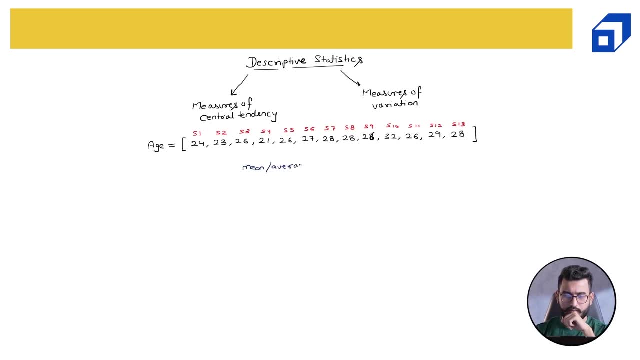 or also known as the average. now, um, i hope you guys already know the formula. if you don't know, it is basically the sum of all the observations divided by the number of observations. mathematically, we can write it as summation of so this. this is a greek letter again: summation. 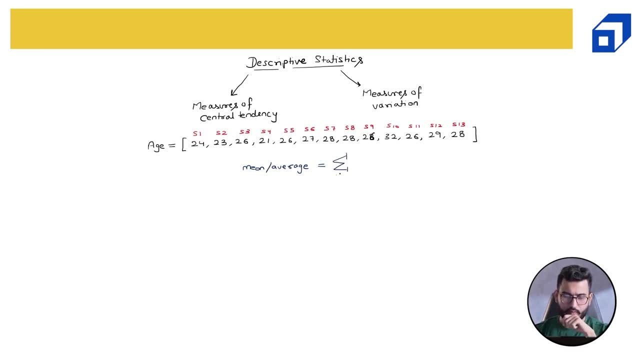 i'm taking a summation over i, or, sorry, over s, and s is nothing but my student number, so si, or just write it as s, si divided by n. so if i expand this it would look like this: s1 plus s2 plus s3, and so on till s 13. this is my sum of all the observations divided by n. now here are. 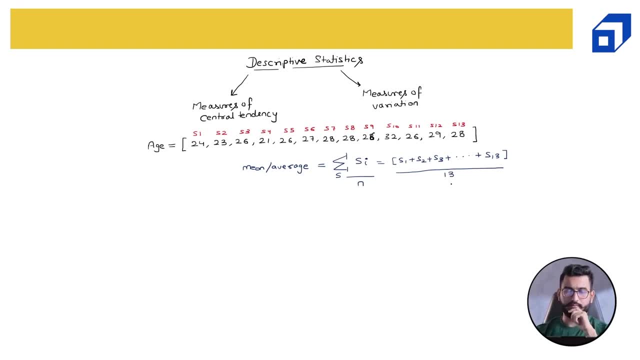 you already know that we have 13 students, so divide by 30. if i solve this, so i have already done the calculations, just to save some time. but if you want, you can pause this video, do the calculations and i would suggest all of you to. 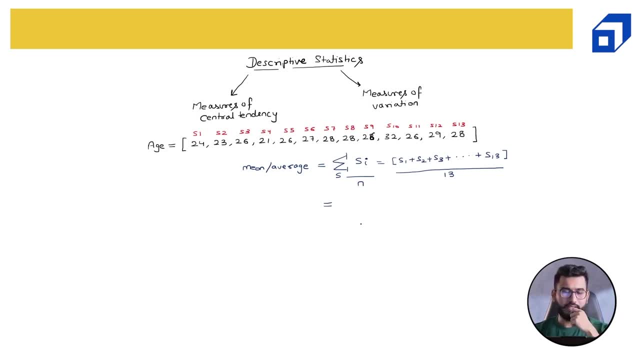 please have a pen and paper with you while you're watching this video so that you can also fully understand the complete concept. so please watch, uh, please stop the video. please pause the video and calculate it by yourself. if you have already calculated it, it is basically 26 point. 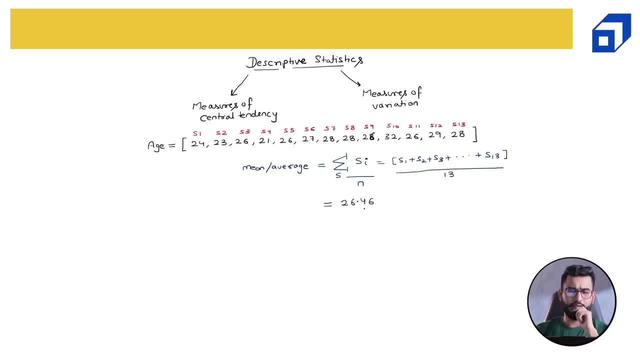 four, six. now this is the average age. what is the meaning of average? assume that i have a number line. now in this number line, this point 26.46 is lying at the center of the data, or maybe at the center of the number line. now it might be at exactly center, it might not be exactly at center, but 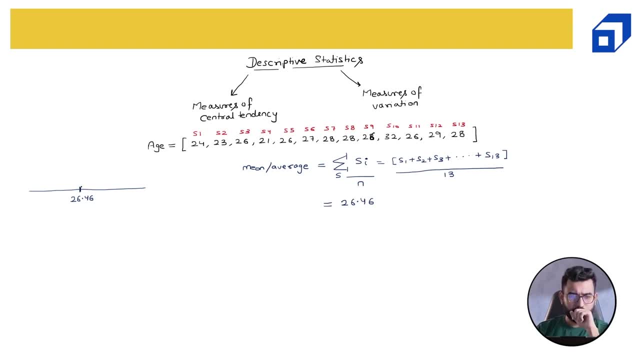 moreover, it will be around the center, so assume that this is- and this particular data point, which is nothing but average. and average can also be written as x and this bar. so if you put x and over it or above it you put a bar, it's. it's also known as x average, or we can call this as. 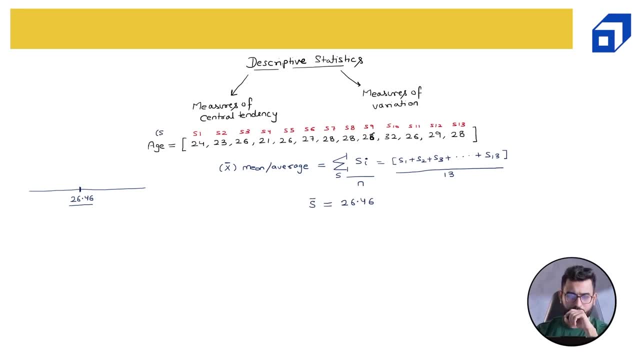 s average, because here we have assumed that this list is s, so this particular number is my s average. now, what we can understand from this number? we can understand that below this point, i'm having few observations. above this point, i'm having few observations. now you already know that. 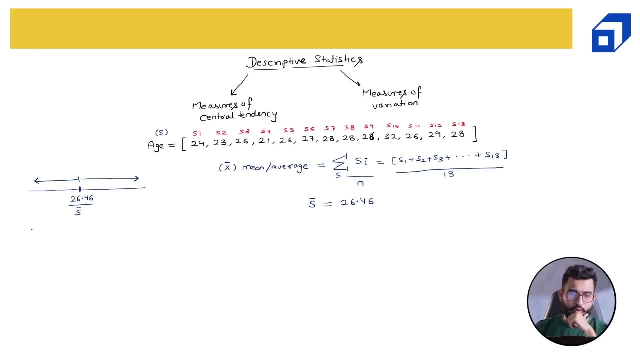 in the class i'm having 13 people. so what we can conclude? we can conclude that in the class of 13 students we have few students above the age of 26- and i'm just taking 26- and few students below the age of 26.. 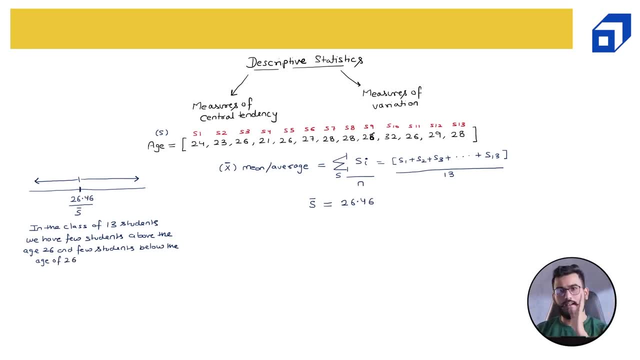 so we are having few students above 26 and few students below 26, and this 26 is basically describing the center of my data. now, it might be exactly the center. it might not be exactly the center, why? let's try to understand this. let's say, given this data, i intentionally add: 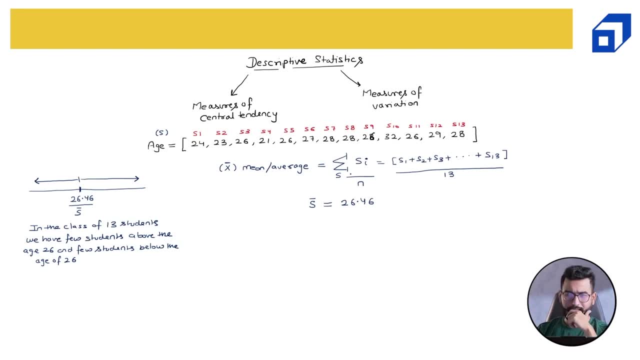 a particular observation. so let me add one particular observation: 40.. or let's add 50. so i'll write it over here and maybe let me change the color 50. so i've intentionally added a student whose id is 14 and the age of this student is 40. and even if you look into this particular data, 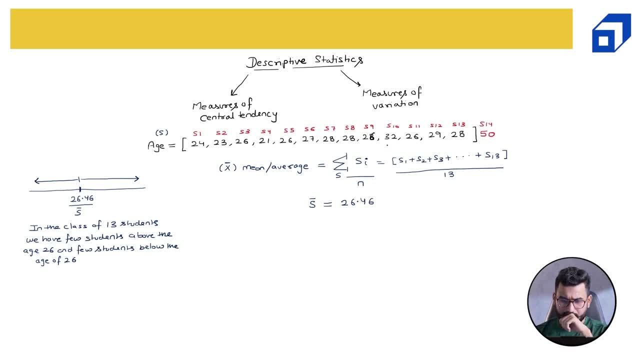 which is having 13 students. you can see that almost all the students are having age of 20s, which is 21, 22, 23, 24 till 29. we have a lot of observations, but there is one student whose age is 32, right. 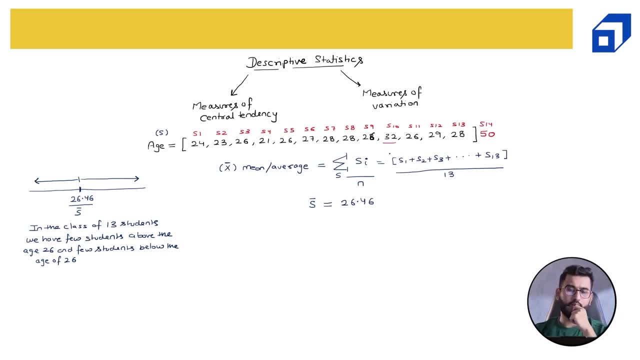 now these observations are basically known as outliers. let me just remove this for a particular data point and let me write them in ascending order, and that would actually help us to derive the another measures of central tendency. so i'll i'll write: age is equal to now the minimum number. 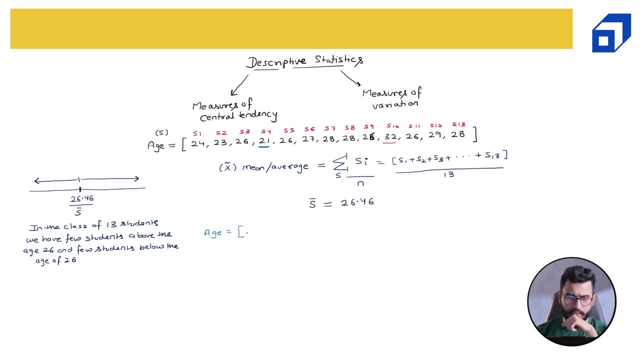 over here is 21, so i'll just draw a line over here. 21, then we have. so we don't have 22, so we have 23, so i'll write 23 over here. then we have 124, so 124, then we have. i don't think. 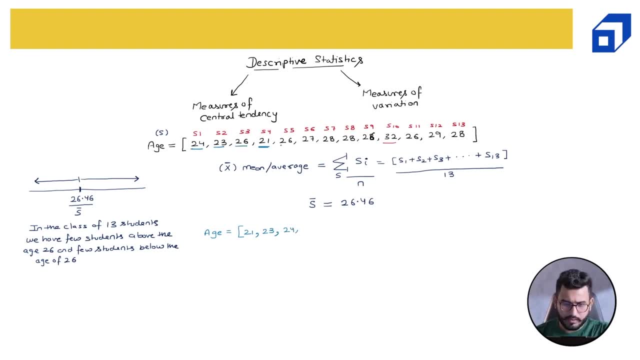 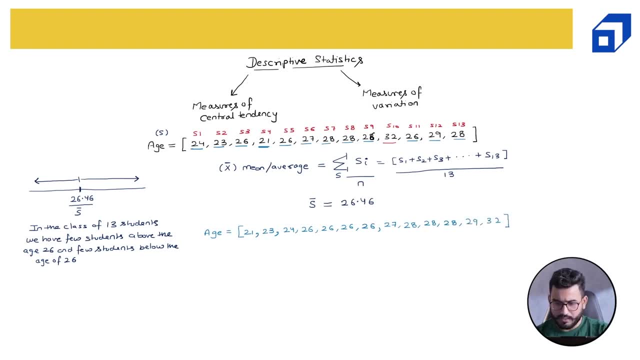 32, 29 and 32. so all i have done is just rewritten all the age of all the 13 students in ascending order, where this is the minimum age and this one is the maximum age. now, if you carefully observe, you can see that 32 appears to be. 32 appears to be very different from majority of the data. 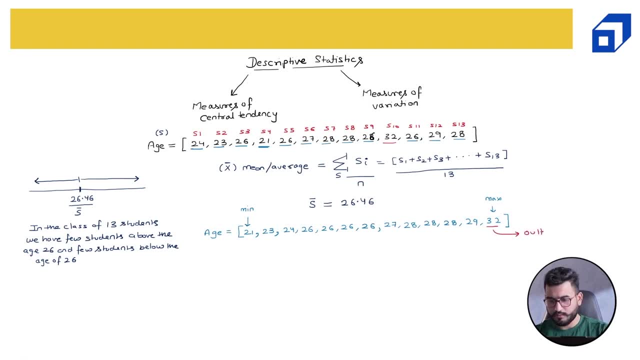 now this observation is known as the outlier, so i'll just draw a line over here and let me just write it down. so this is the outlier, so this is known as outlier. the formal definition of outlier is: outlier is that particular observation in my data which is very different from majority of the data points. so let me just write it down: outlier. 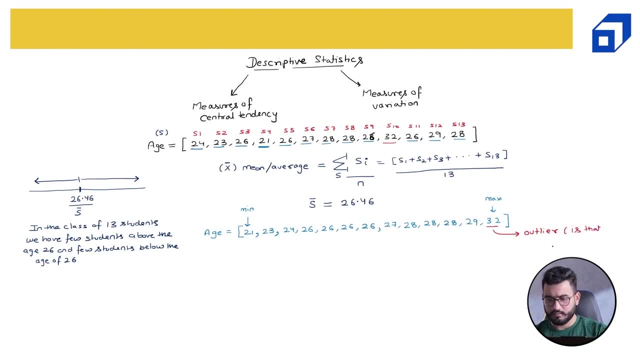 is that particular observation, observation in the data, that is, that is very different from majority of the data points. so if you carefully observe here, majority of data points belongs to 20s, 21, 22, 23 and 24, 20, 28 till 29, but suddenly there is a number 32 and that is basically the outlier. now what is the 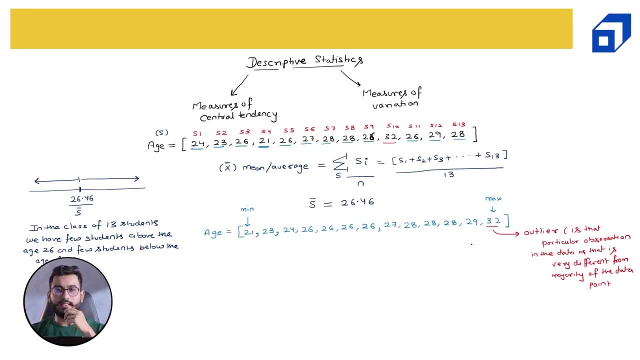 problem behind this outlier, why outliers are problematic when we talk about the descriptive statistics. if i try to look at the median now, what is median? median is another measure of central tendency. so what is median? median is another measure of central tendency. so we have already talked about mean over here. then we have median. median is exactly the center of the data. 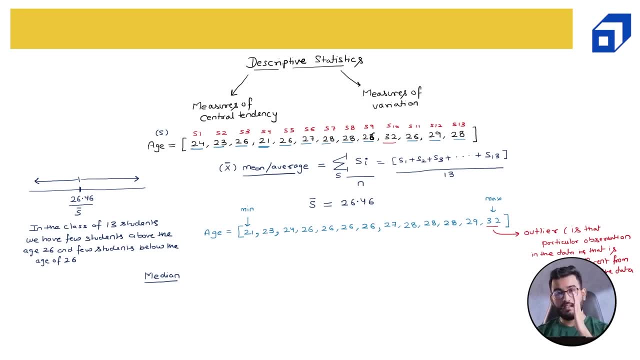 exactly center. when i say exact center, that basically means: above this, i will have 50 percent people, below this, i will have 50 percent people. so it is exactly the center. how we can find out median? so there is a simple formula: n plus 1 divided by 2 if the number of observations are. 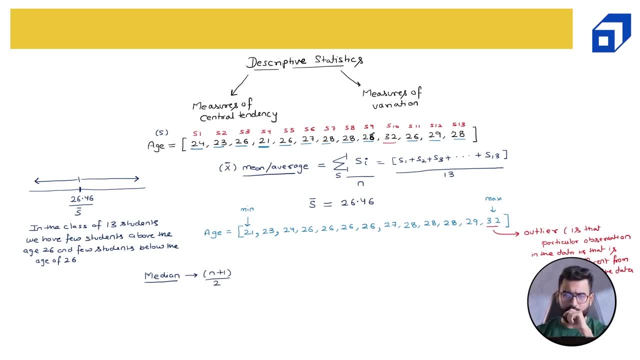 odd. here we have odd number of observations: 13. so 13 plus 1, divided by 2, is 14 divided by 2, which is 7. so my 7th observation is the center of the data or is the middle point of the data, and let me just quickly mark it. so it is. 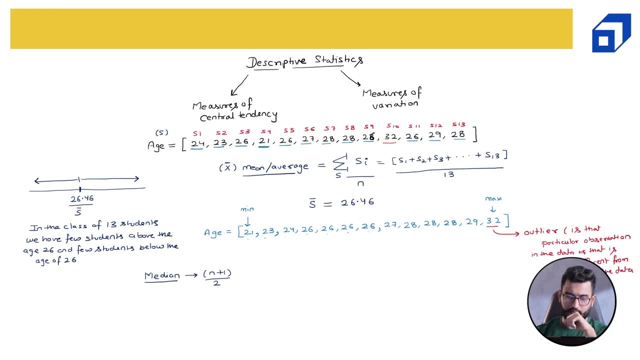 1, 2, 3, 4, 5, 6, 7 over here, and it is my center. now, if you just number, if you just calculate, if you count below this 20, you will get the number of observations: 13. so 13 plus 1 divided by 2 is 14. 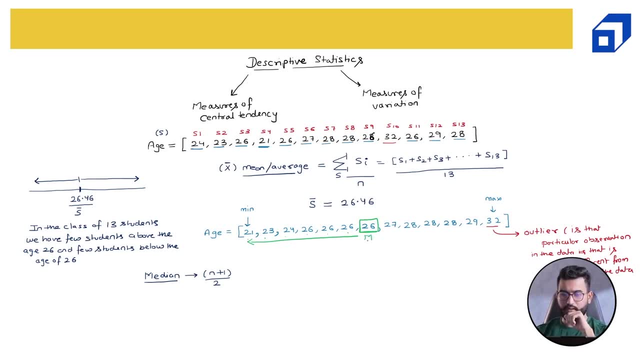 26 without this middle point. i'll just write m to depict that this is a middle point. i am having 1, 2, 3, 4, 5, 6. i'm having 6 observations above this: 1, 2, 3, 4, 5, 6. i'm having 6 observations. 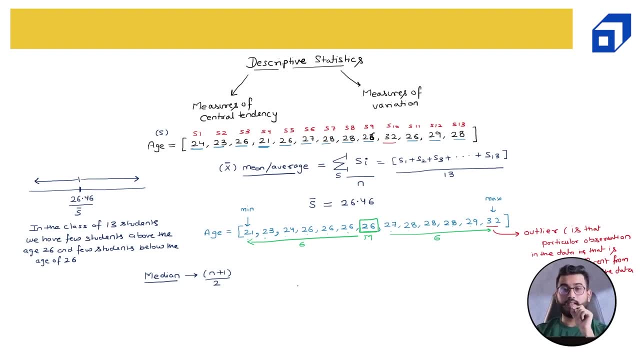 so median describes the exact center point of the data. so what is median? this value exactly in the center of the data in such a way, in such a way that we have 50% observations, 50% observations above this point, above this point, and here we have taken 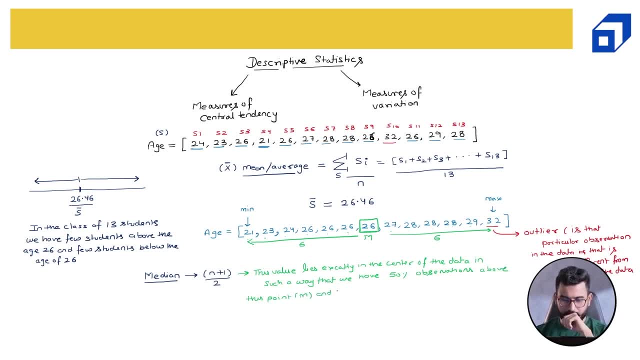 M, so above this point M and 50% observations below this point. and again, this is M, so below this point M. So median describes the center of the data in such a way that it is lying exactly at the center, where 50% of the data is below this point, 50% of the data is above this point. 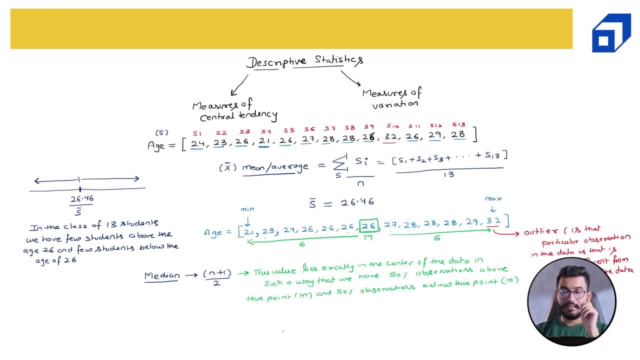 While I cannot say the same thing for average, and you can see why Average is basically taken out by considering all the data. When I have to calculate average, I am summing over all the data. Here you can see the formula. The formula is sum over all the data points. 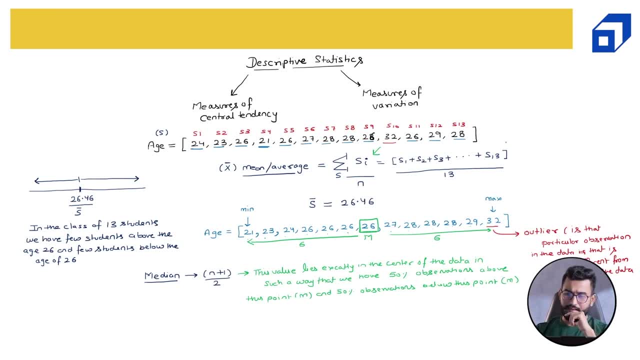 divided by the number of data points And due to these influential observations, which are known as outliers, my average can shift towards the outlier. Here you can see mean, as I have told you, mean is also the center of the data, while median is also the center of the data. These both metric describes central point of my data. 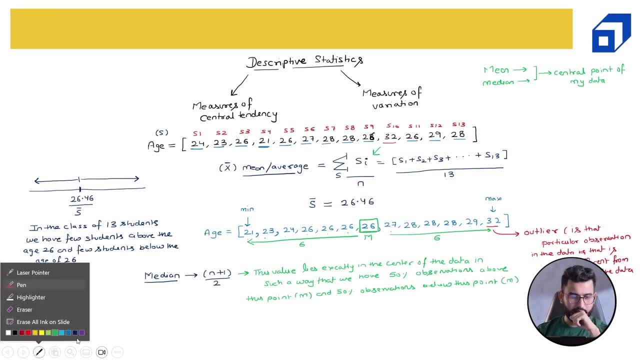 But why there is a difference, Why my average is 26.46 and why my median is 26.. So my median is 26.. Now, this is because of this outlier. So where I am having outlier, I am having outlier on the higher end. This 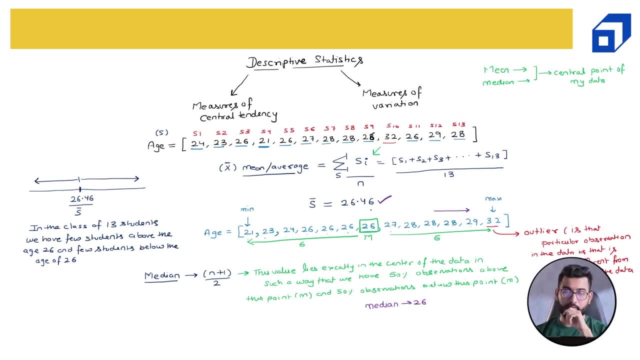 is my higher end. So what has happened to the mean? My mean has also shifted towards the outlier. Now, please remember this. I will just write down as a note over here that your average gets impacted with the presence of the outliers and will shift. 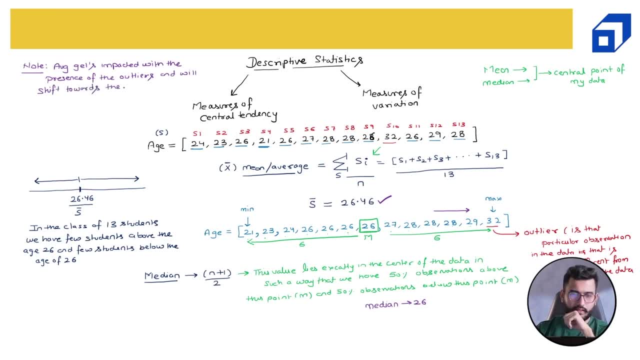 towards the mount. So if my outlier- so assume that this is my number line- and if my outlier is on the lower side, then my average will shift towards the outlier, so my average will shift towards the outlier. If my outlier is on the higher side, then my average will. 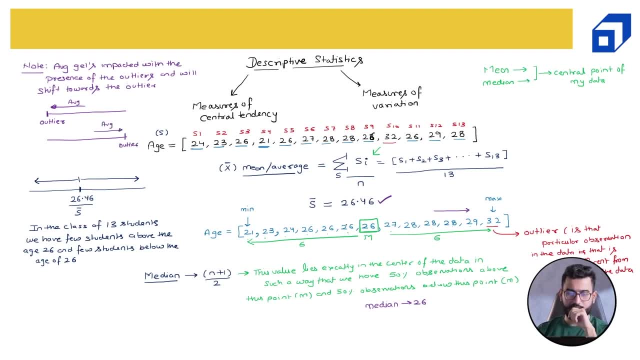 shift on the upper side, higher side, and we have already seen this example. my median was 26, but my average came out to be 26.46 because my average has shifted towards the outlier right. then we have one more major measure of central tendency, which is mode, and mode is very simple to understand. 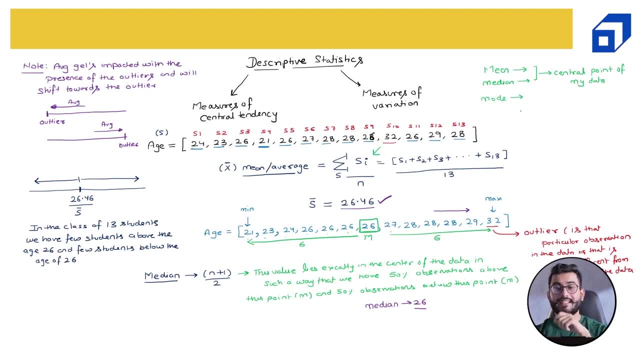 mode is the observation with the highest occurrence in the data. so let me write the definition over here. i'll just simply write it as observation with maximum frequency. observation with maximum frequency. so if you carefully observe, in this particular data i'm having the observation number 20. 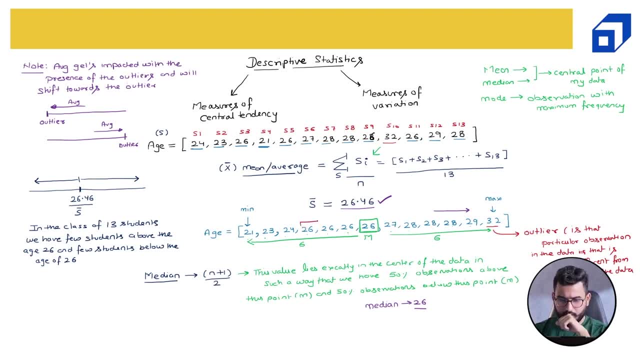 not number 26, observation 26 to have to two. this observation has appeared for four times, right, so the frequency is highest for the observation 26 and hence my mode of this data is 26.. mode of the data is 26.. now there might be cases where you do not have any mode for. 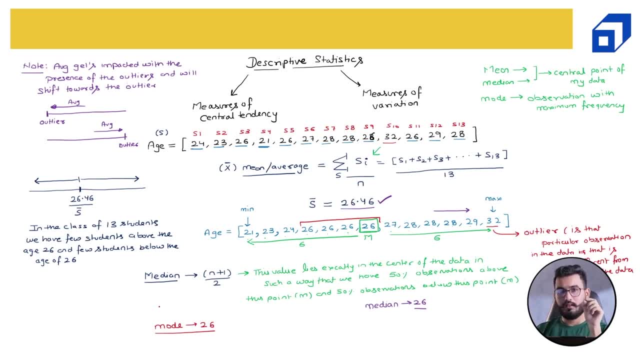 example, let's say I'm having four observations, sorry, four observations. four observations 26, or there are four students with the age 26, we also have four students with the age 28. now, in that case, when there is a tie or there is no mode, so you will simply write no mode, in that case you have to use 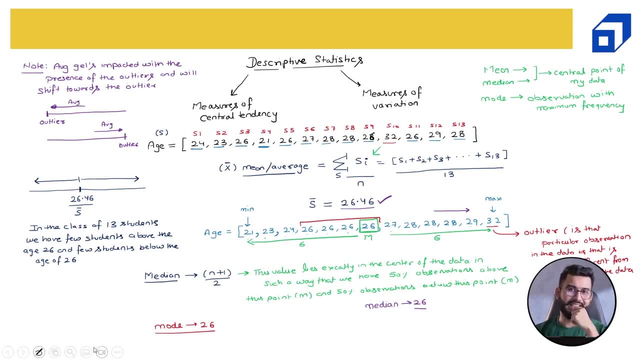 mean and median to describe the center of the data. so I hope you guys are able to understand the measures of central tendency, as the name says, this or all these three measures which are mean, median mode, they basically describe the center of the data. and if your data does not, 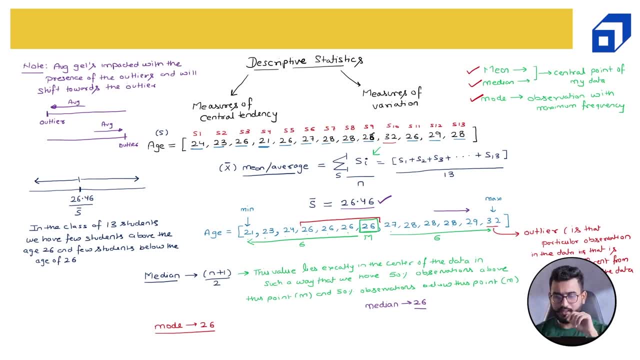 comes with outlier, and here you have seen that 32 was the outlier, and here you have seen that outlier. but if your data does not comes with outliers- maybe either on the higher side or on the lower side we do not have any outlier- then these three measures will fall very close to. 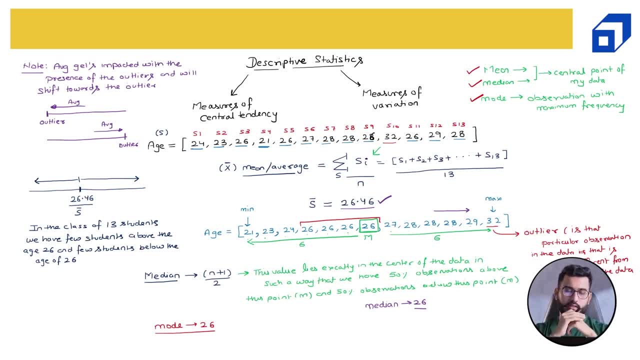 each other, or approximately, they will be equal to each other. so your mean will be equal to mode, equal to median. and here you can see I was having average to be 26.46. if I was not having this outlier, which is 32, I would have gone, got this value close to 26 only. sorry, 26.46 is my average. 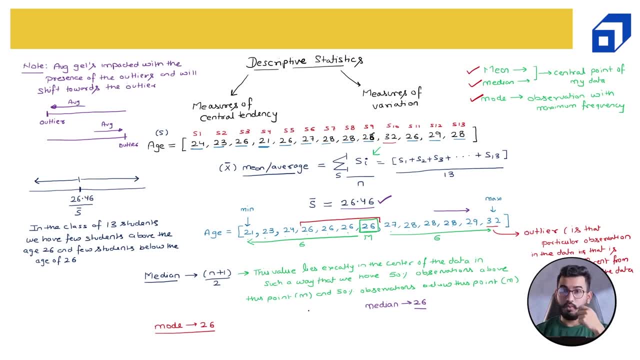 my median is 26. my mode is 26. in this case, I can say that my data is having a center of 26. now if I go to my principal and if I tell to my principal that the average age of my class is 26, with 13 students, then it gives the 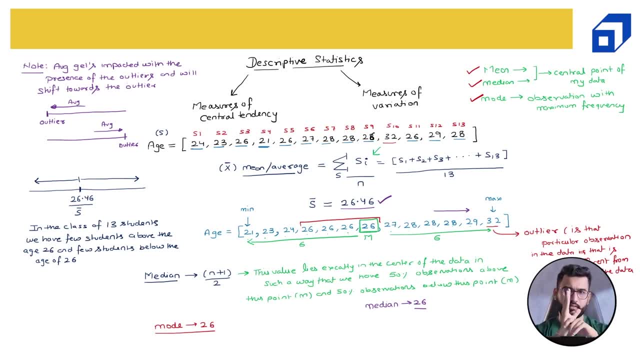 rough idea to the principal that, okay, we have a center, point 26, and we have few students above this point, few below this point. if I tell to my principal that the median is 26, with total number of students to be 13, then in that case the principal will be able to do a little bit of math. 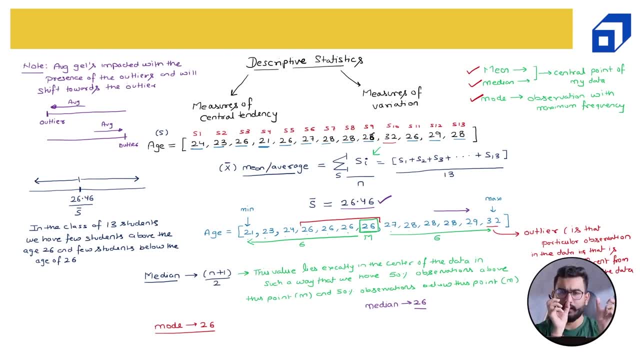 and he will be able to understand that. okay, we have six students below 26, six students above 26. so I hope you guys are clear with measures of central tendency. but there is a problem. the problem is I'm still not clear how the values are varied. so I know that center of 26, but 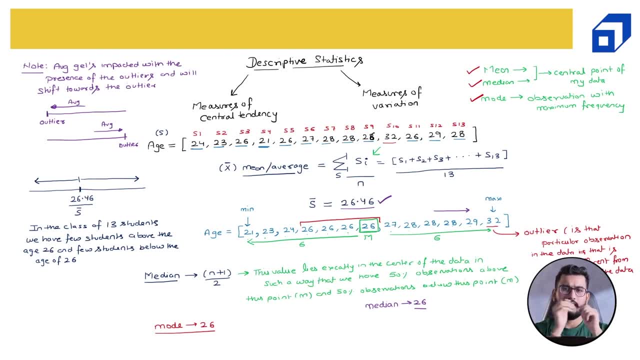 how would? the variation is there in the data. so am I having on the age of the students to be very much varied? when I say varied, that means that means always one Keema girl, many岐. the values are very, very far away from the center. so let me just give you a very simple example over 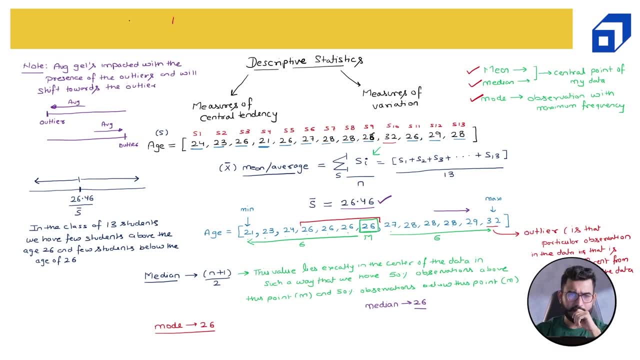 here let's say this is 26, this is 26 and here also we have 26. so in these two number lines the center is 26, excel. but in this number line on, that is on my left of the side, left of my screen, the minimum is 15, maximum is 30. here you can see that the minimum is 20 and maximum is 30. 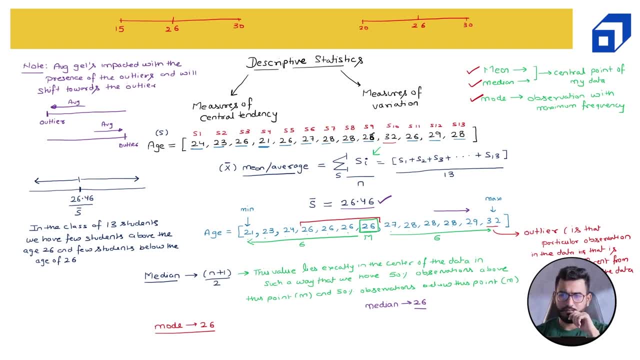 or let's let's take it as 29 now. here, if you see that the values are very far away from the center, there is a high variation, while here the values are very far away from the center. so here you can see that the values are very far away from the. 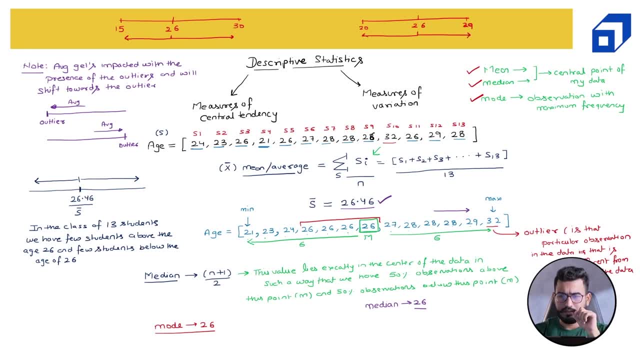 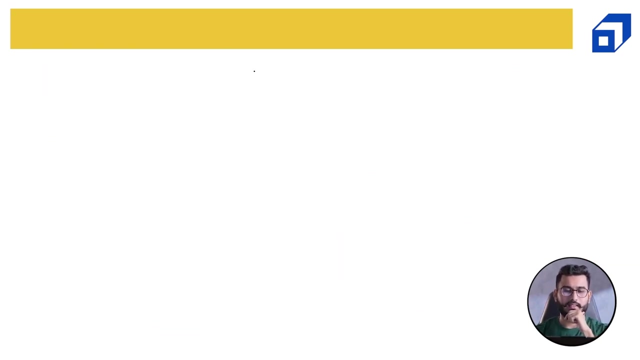 center, the variation is low. so measures of variation tries to quantify this variation given a particular data. how much values are scattered around the center? this is what we are going to learn in measures of variation, which is our next topic. so now let's talk about measures of variation. 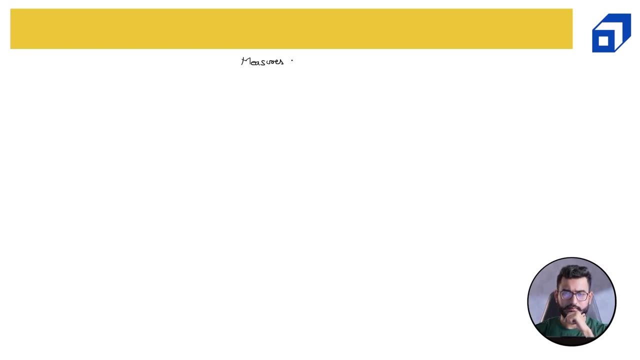 measures of variation, and i have already given you a very, very short example i would see in my last slide. but now let's try to have a more insightful example which will clarify your doubt regarding what exactly is measures of variation. so let's try to take two examples or two subjects, and i'm just plotting these two subjects to get you a visual. 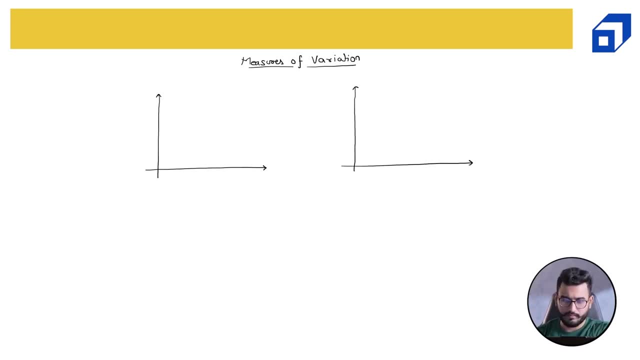 picture about what exactly i'm trying to explain. assume that here the x-axis represent the student id for both the plots and y-axis represents the marks. these are the marks. so let's say, the average marks are represented by this red color line, red color dotted line. these are the average marks, or this is the average marks. 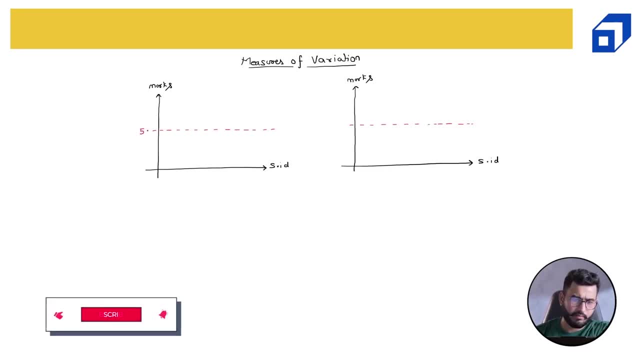 for example, you can assume that the average marks is 50 for both the subjects, but for subject a and this is subject b. i'm not just naming any subject, i'm just saying a and b. for subject a the student marks are scattered like this, so this represents the marks of student number one. 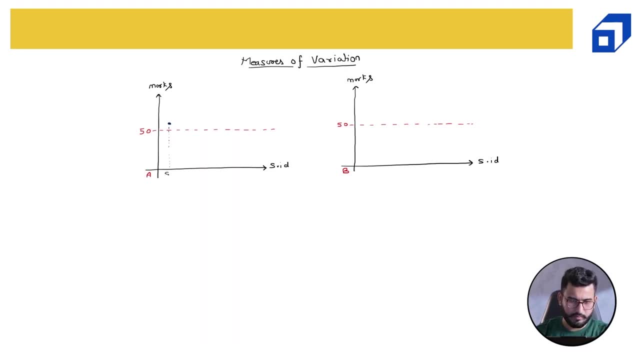 so this is student number one, then this marks of student number two, then we have student number three, and so on. so i'll just draw it now, because i hope this gives a clear picture about what i'm trying to explain. so this is basically the scatter plot for subject a, for subject b. 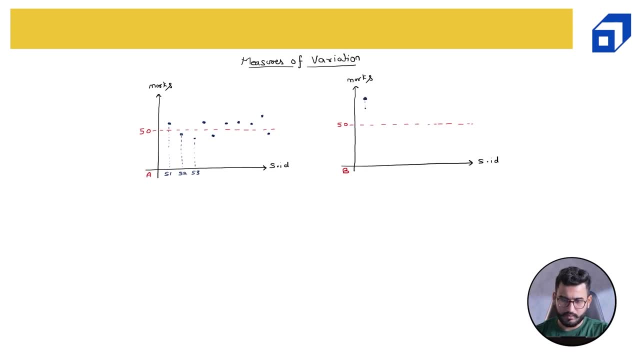 this point represents the marks of student number one. this for student number two, then three, four, five, six, seven, eight and nine, and let's say ten. here also i think we have ten: one, two, three, four, five, six, seven, eight, nine, ten. So you can see that in both A and B we are having 10 students, but for subject A you. 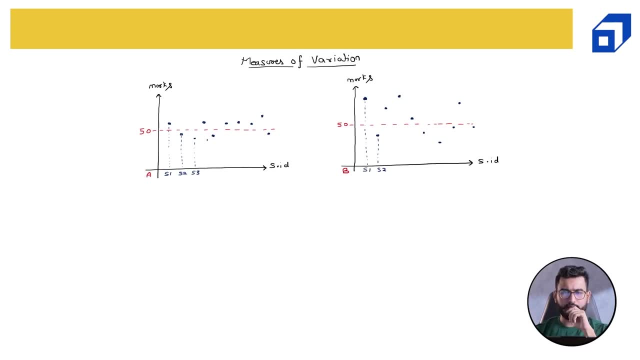 can see that all the marks or all the students have scored. they have scored marks which are very close to the average. Most of the people have scored. let's say, if I just create a band, let's create this band, a dotted band. 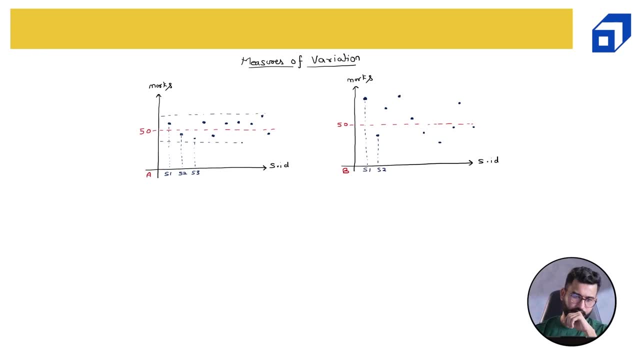 So most of the students fall in under this band or within this band, While here, for subject number B, you can see that there is a lot of scatteredness. You can see that there are data points which are very far away from the average line. 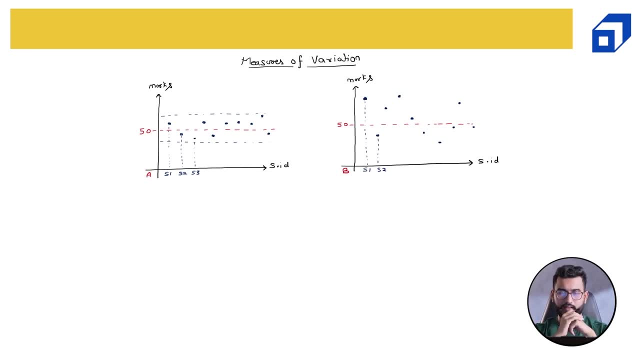 There are data points which are also close to the average line. But in student, In subject A, all the data points are very closely scattered around the average line. right Now can I say that for subject A, the variation around the mean. so this is my mean, the red. 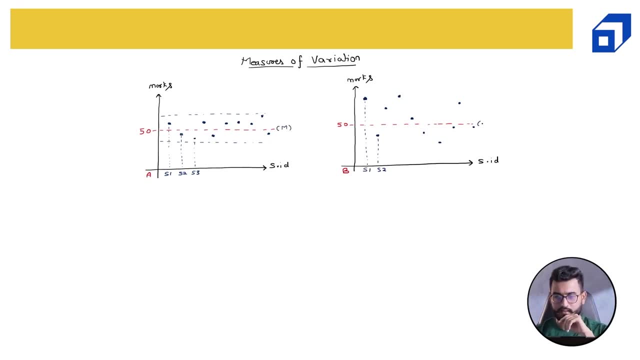 color dotted line is my mean or the average line. So M represents the mean or the average line. So for subject A, the variation Of the marks around the mean is low. For subject B, the variation of marks around the average line is high. 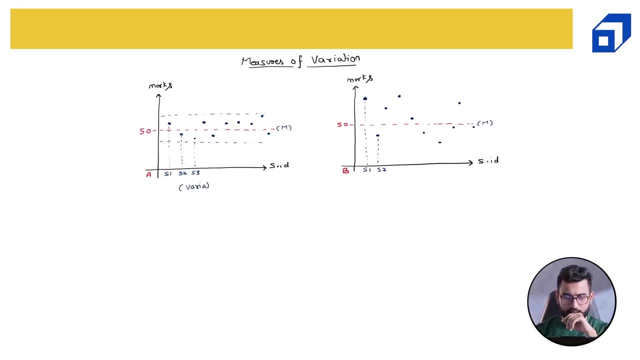 So here, variation around the average line for subject A. So here variation around the average line for subject A is low, is low, while for this variation around the average line for subject B is high. Now the measures of variation tries to quantify this, How I can say this is low and how I 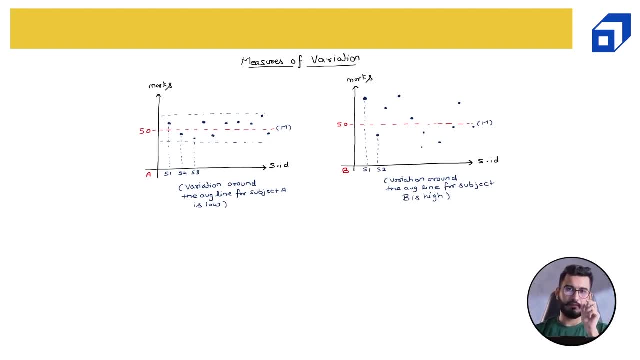 can say this is high. We need a number right, We need some quantity. We need a number that can describe this measure, or describe this is scatterness, or describe this variation. So measures of variations are those metric. that describes the variation of the data as 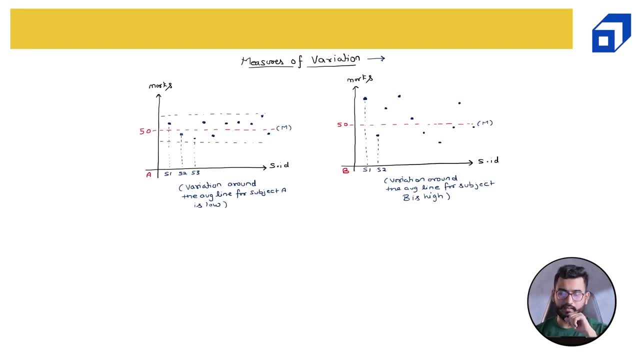 around the center or around the average line. So measures or metric that describes the variation of the data around the center of the data. Now, what all measures we have? So number 1. So I'll write it over here: We have. so we. 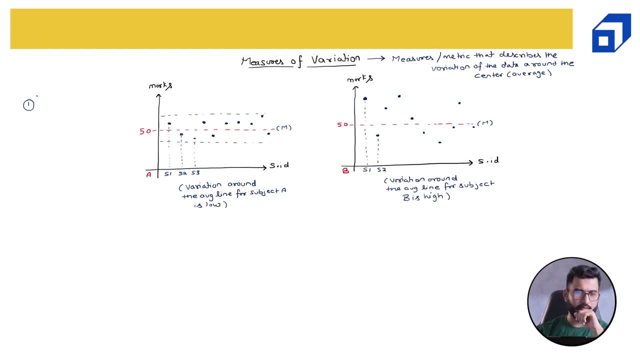 exactly have 4 measures. let me write it down. So we have range, We have variance, We have standard and standard deviation, standard deviation and finally, we have the coefficient of variation. coefficient of variation. so let's talk about each of them now. in order to talk about any of them, we 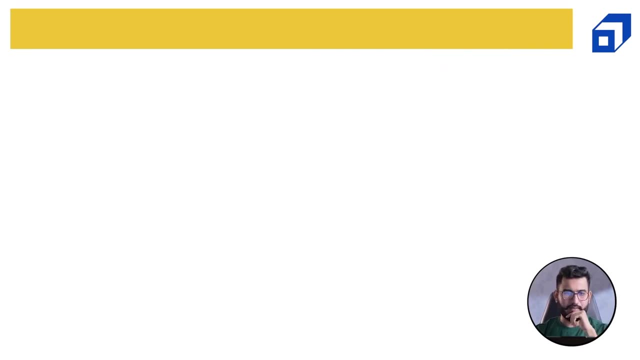 need the data. so let's create some random data. so let's say, here we have the data of the marks of a student in one particular subject, and I'm intentionally drawing this table a bit large because we will be calculating a few few parameters in order to arrive to the 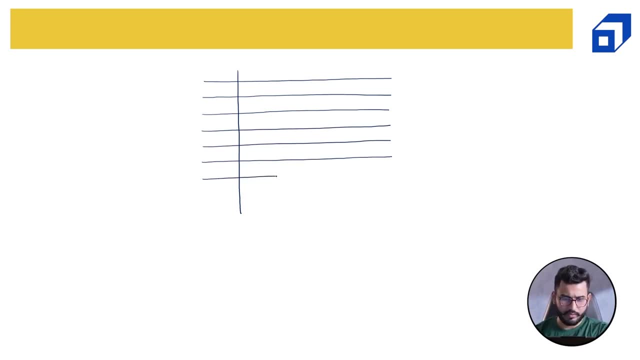 exact quantity that we are looking for. so let me just quickly draw the table. so here we have the student id, which again runs from 1 to, let's say, 10. 1, 2, 3, 4, 5, 6, 7. then these are the marks. 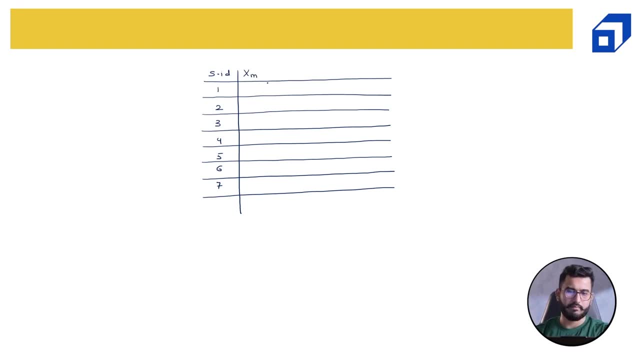 so I will write x, m, x. m means marks of students. So let's say the marks are 27,, 52,, 48,, 33,, 39,, 65 and 82.. Now, this is my marks of the students. Now, if I have to calculate the range, range is nothing but. 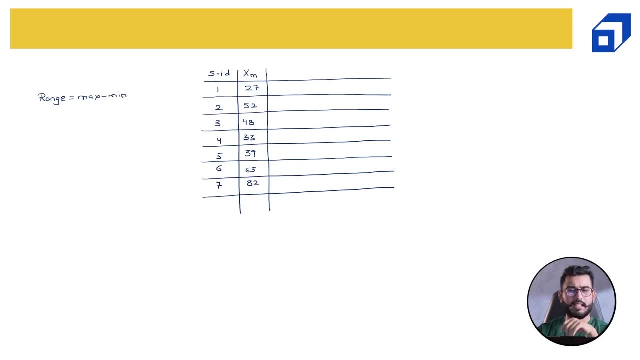 the maximum minus minimum. It gives you a very raw idea regarding what is the range of my, what is the range at which we are trying to work, or if we are trying to work, we are talking about the marks. then what is the minimum marks scored? What is the maximum? 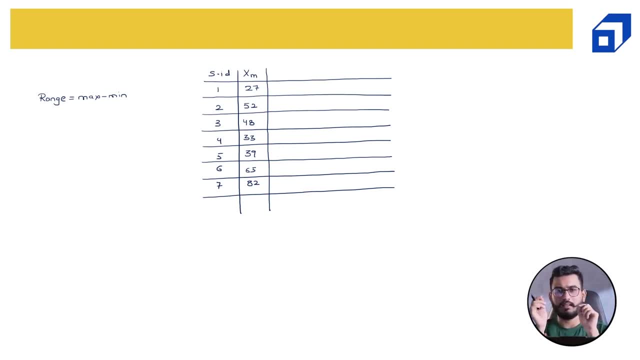 marks scored And the range is nothing but the difference between max minus min. So my max marks is 82 minus minimum, which is 33.. And if you subtract this you will get the range. The second measure is variance, which is a. 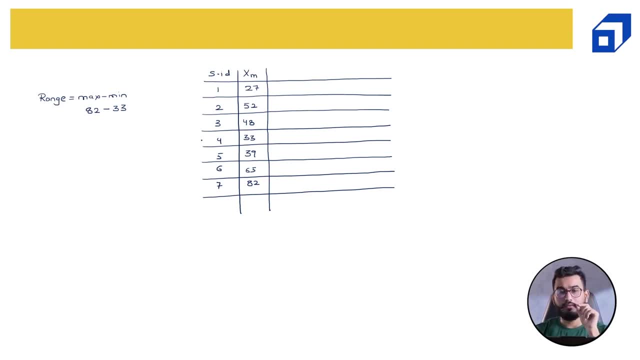 better measure To define the variation in the data. What is the problem with range? Range is again influenced by the outlier. So let's say if there is one student in the class who has scored 100, while most of the student has scored, let's say, close to 33,, 33,, 35,, 39,, 40, then 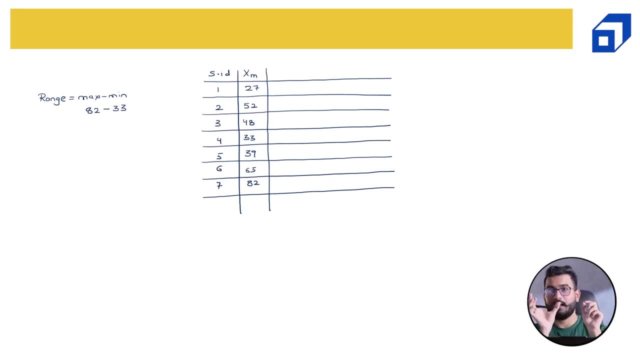 in that case also, the range would be very high. So it would. it would mislead you. It would give you- give you a misleading idea that students have scored in a high range. but that is wrong. Range gets influenced by the presence of outlier And that is the reason. 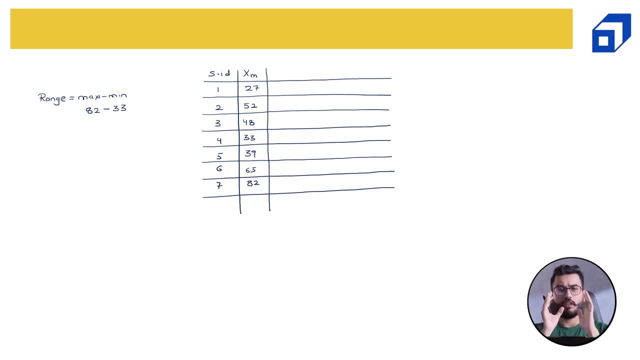 we don't use range as a measure to to make or to understand about how the data is, how the data is scattered around the center of the data or center line. So let me write it down over here: Range is A metric that gets influenced with the presence of outlier. Now how to arrive to the variance? 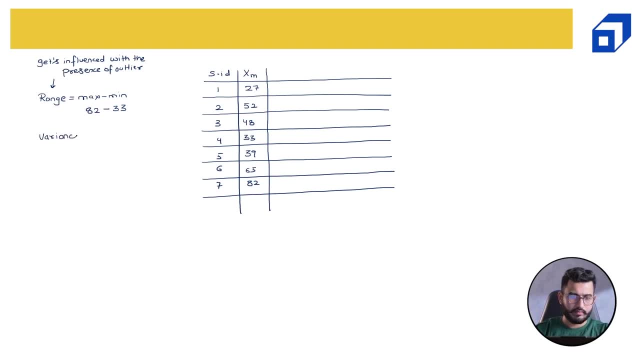 So we are talking about variance. now, In order to calculate variance, We will first of all find out the center, because, as I have told you, variance is all about calculating the scatteredness, or calculating the variation of the data from the center point, which is the mean or the average. So we have to find out the average first of. 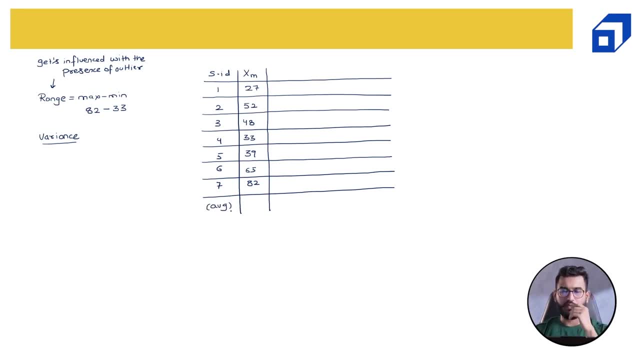 all the average And if you guys want, you can pause this video and quickly calculate the average, because we have already learned about it. So just take the sum of all the observation Okay, By seven, because seven is the total number of students in the class, And that would give 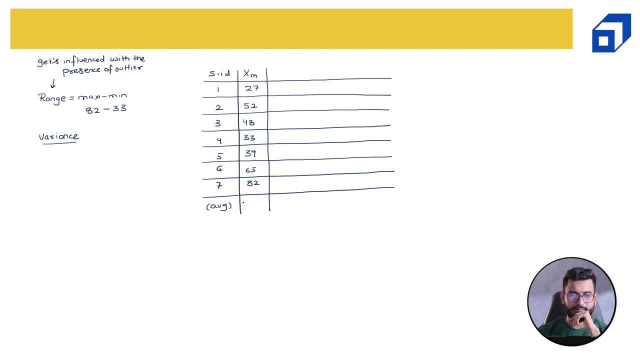 you the average. So the average of this particular uh marks for the students would came out to be 49.49.. Now for uh simplicity purpose and for the for making all the calculations very simple, very clean, let's take this number as 49. So assume that the center is 49.. 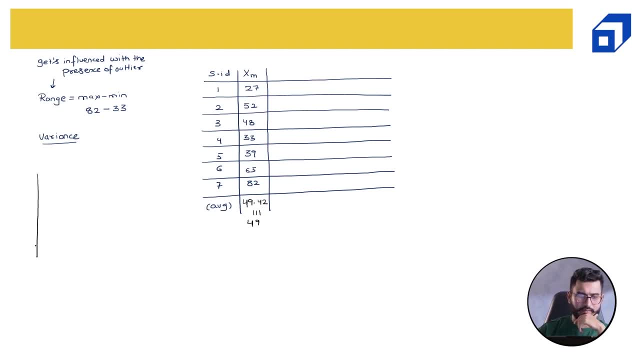 Now we have the center. So let me just quickly draw the graph, the same graph that we have seen in the last slide. Uh, this is a student ID. These are my marks and we have the center Now at 49, so somewhere in the middle, but one point below. So assume this is 49.. So 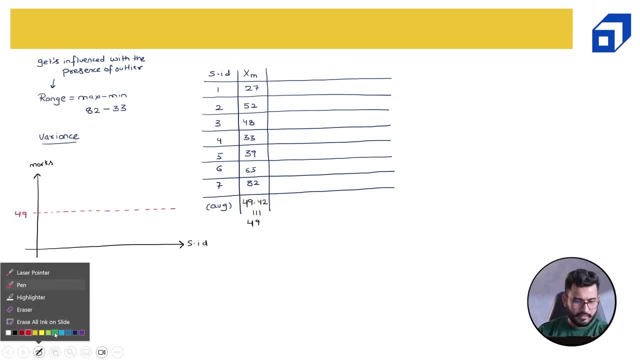 this is my 49. Now let's mark all these numbers. So 27 would lie somewhere around here. So this is a student number one. Then we have 52.. So this is my student number two, and then we have 49. So 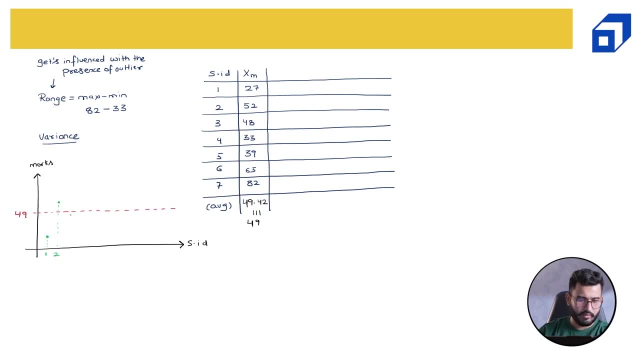 48,, which is very close to the average. So this is 48 and 33 somewhere over here, 33,, then 39, maybe over here, then 65 over and above the average line And finally 82,, which is again over and above the average line over here. 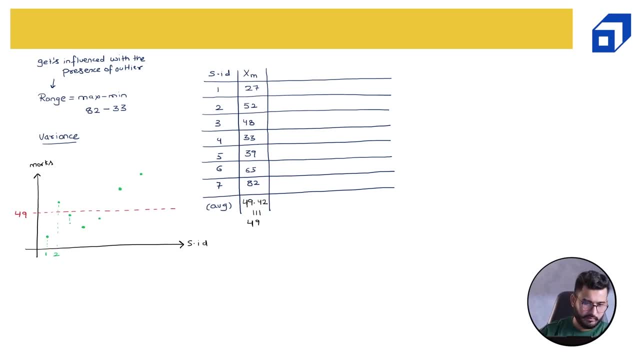 So these are my data points. This is my student number three. This is four, five, six, finally seven. We have seven data points. Now we will calculate the distance of each of this data point from the center. from the center, which is average. 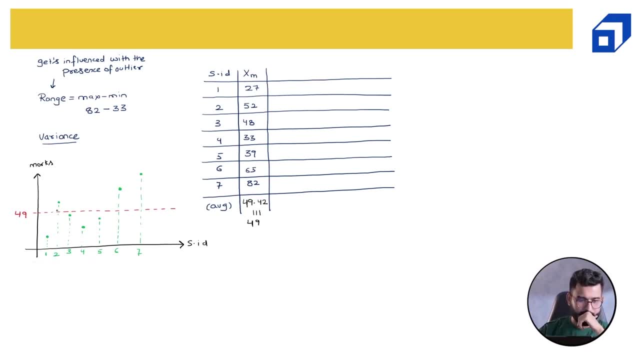 So when I say distance, I'm basically interested in this distance. This is D1.. Then this is D2.. Similarly, this one will be D7.. This one will be D6. So distance is nothing, but I'll take the data point. 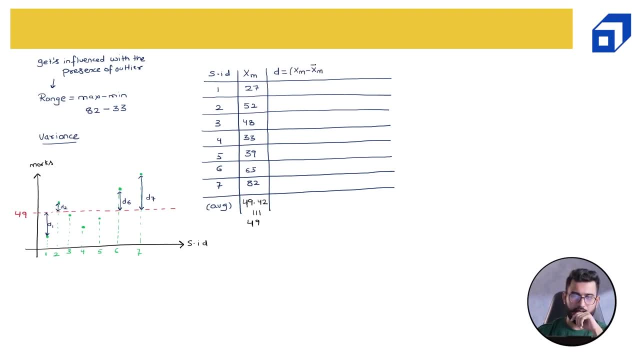 So XM minus XM bar. I hope you guys remember. If I put a bar on a variable it becomes the average. So this is my average marks, which is 49.. Average marks So: 27 minus 49.. That will be my D1.. 52 minus 49,, 48 minus 49,, 33 minus 49,, 39 minus 49. 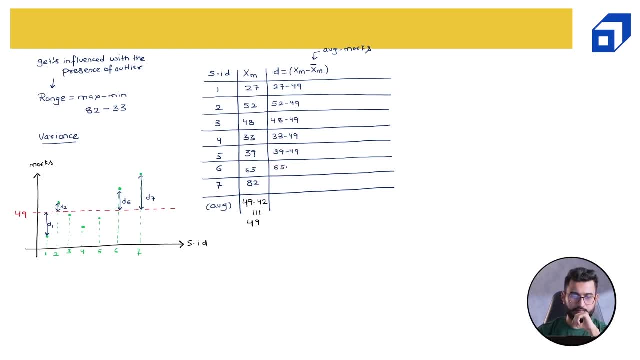 39 minus 49,, 65 minus 49, and finally, 82 minus 49.. Now, if I ask you what is the average distance from the center, It basically means how much, on an average, a data point is deviated from the center. 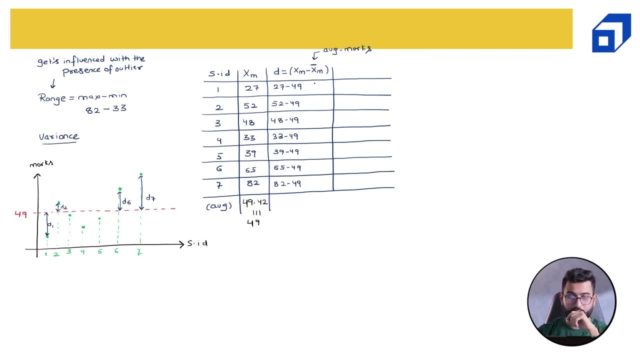 Now, if I have to find out average, I have to take the sum of all these values, right? The problem is that few of the values are above the average, which would result in a positive value. Few of the values are below the average, which would result in a negative value. 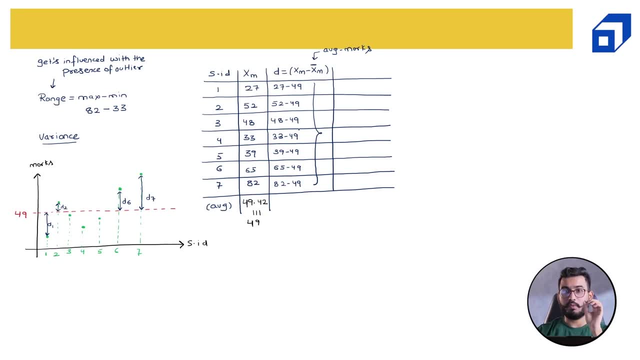 And if I simply take the sum of all these data points, the positive will cancel out negative, So we would get a very wrong value. And if I know that the center is 0, and we have some positive value, some negative value, 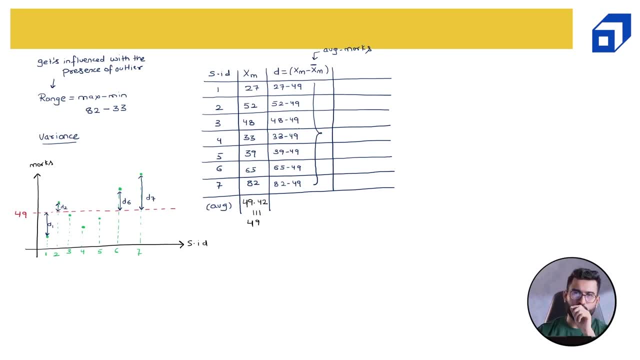 then you will get a value close to 0, which basically means there is no variation, which is wrong, right? In order to overcome this problem, I will take distance squared. I will convert the positive error or the negative error into the square. 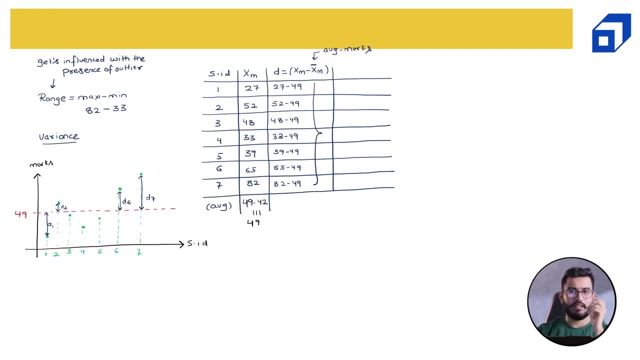 so that the positive and negative can be nullified. We can get rid of these positive signs and the negative sign. So let me just quickly write down what we are left with So this will result in. I'll just quickly write down all the numbers, because I have already calculated it. 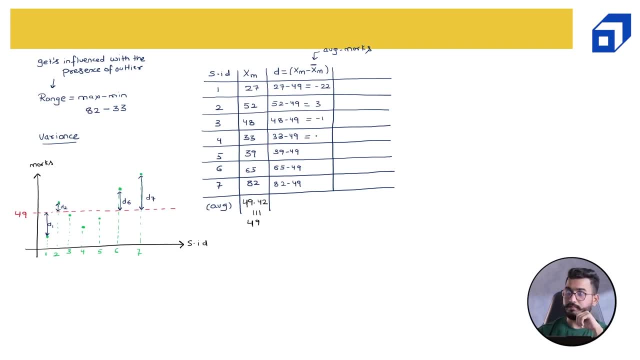 So this will result in: I'll just quickly write down all the numbers, because I have already calculated it. Now. here you can see that I'm having minus 16 and plus 16.. And if I simply take the sum over all the d, this minus 16 will cancel out plus 16.. 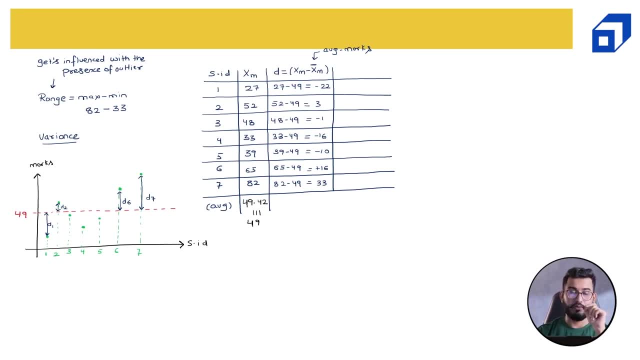 So I will not get the contribution of these two numbers. Similarly, you can see that I have minus 16 and plus 16.. Similarly, you can see that I'm having minus 22 plus 33, minus 1 plus 3.. 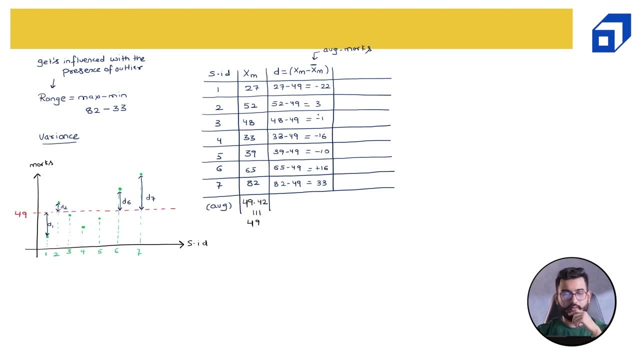 So we are having some values which are positive, some values which are negative, and we cannot simply take the sum, So we will take distance squared. So 22 to the whole square is- I have already done it- So- 484, 9,, 1,, 256,, 100.. 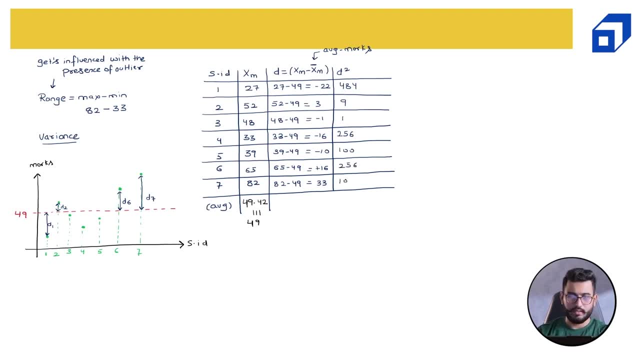 Again 256 and 1.. Now we will take the average of the distance squared. So what we have to take: Average of distance squared. Now you guys can ask me that Sumit why you have taken a square. 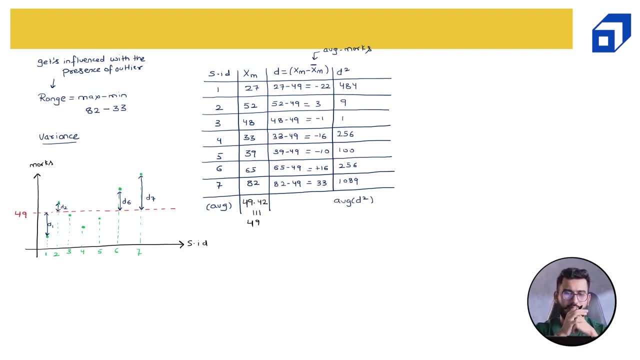 Why you haven't taken the absolute value. So I would have simply taken minus 22 as just 22 and minus 16 as just 16.. So I would have taken the absolute value. I would have taken the absolute value. So I would have taken the absolute value. 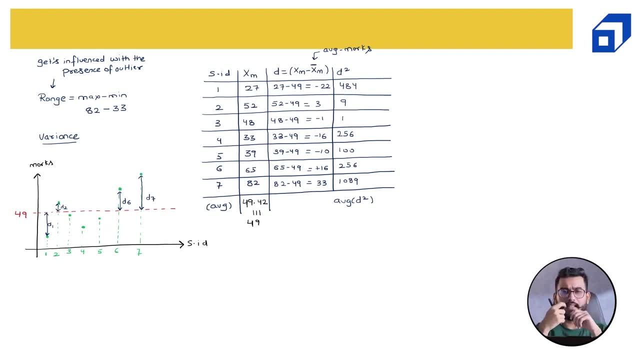 So that's what we have to do Now. please remember that when we are working with statistics, we are using a lot of calculus also, And as of now I cannot show you where I would be working with calculus, But as we proceed forward, you would see that statistics is heavily dependent on calculus. 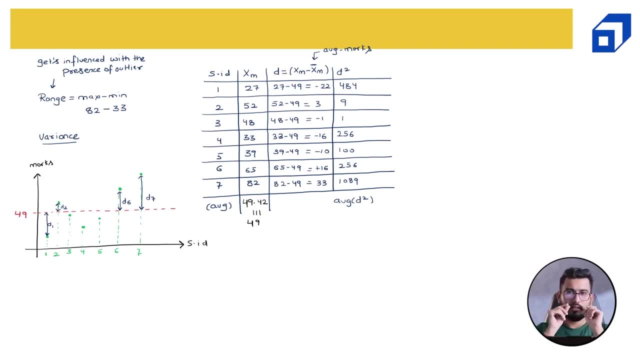 And when we talk about functions, The function or the derivative of a constant is always 0 and derivative of a square term which is b square, or maybe a derivative of a function which comes with a polynomial value can be differentiated. So your calculus does not works with constant, does not works with functions which are constant, and that is the reason we will not be using those. we will not be using the absolute term and we will be using the square term. 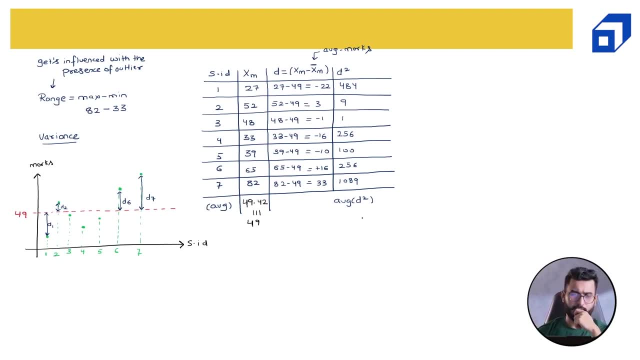 So we have to take the average of d square and you already know the formula, which is summation over d square And divided by n. so if I take the sum of all the observation which are present in the column d square divided by 7, I would get the average distance, or not these, just the average distance, I would get the average of d square. 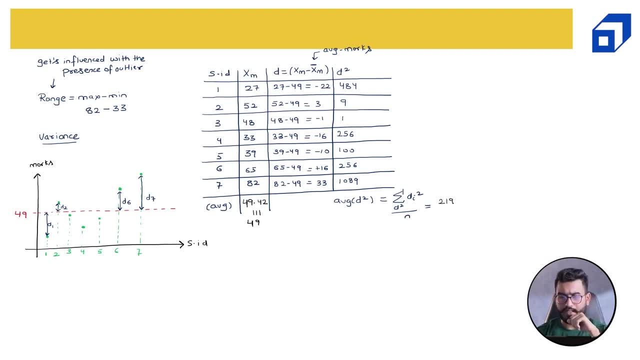 So this would be 2195 divided by 7, which is 313.57.. Now this Value is known as Variance Variance, Which is 313.57.. The problem with variance is that you can practically not make sense out of it. 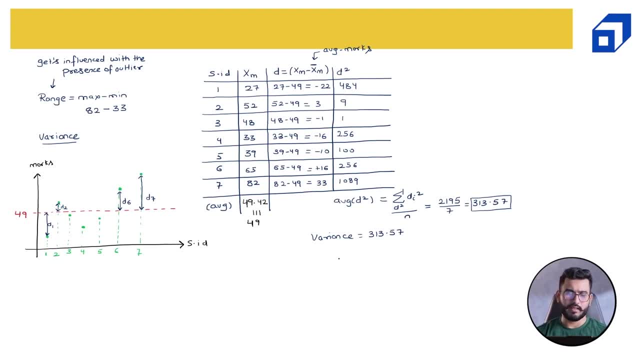 I'm not able to understand what this value mean, And if you remember, it was d square. d square is equal to 313.57.. Variance is also known as sigma square. it is known as sigma square. this, this is a Greek letter: sigma, sigma square. so so my sigma will be square root of 313.57, and this would get us 17.65. this is my sigma. 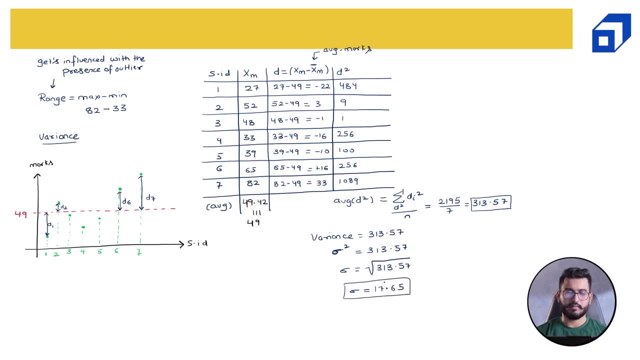 Now, what is the meaning of this? Now, sigma square is my variance. Variance is basically my sigma square, While sigma is my standard deviation. Standard deviation, standard deviation, is my sigma. So standard deviation talks about the average distance That the data points are deviated from the center. 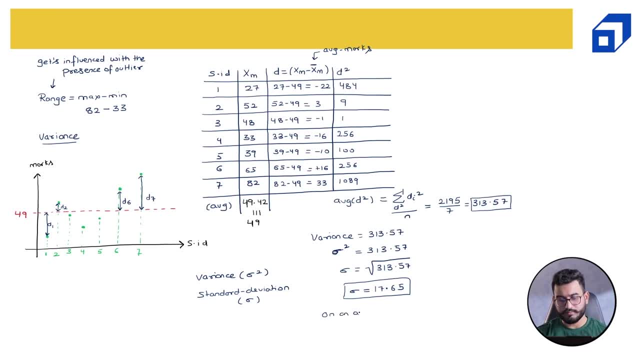 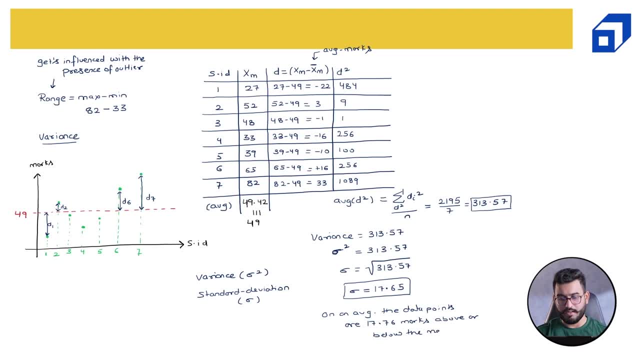 Below the mean. Below the mean, And that is what this is standard deviation mean, And that is what this is standard deviation mean: How much, on an average, The data points are points are deviated from the center, and that is 17.65. now, if this value is very low, which? 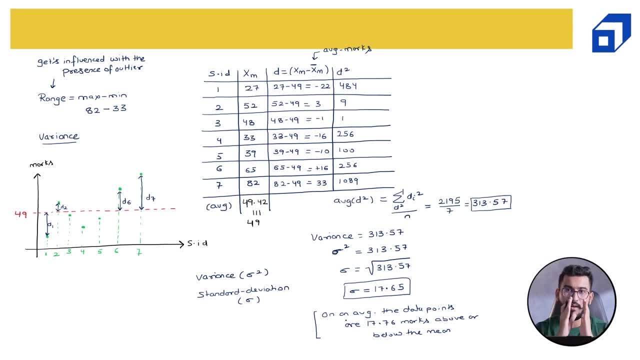 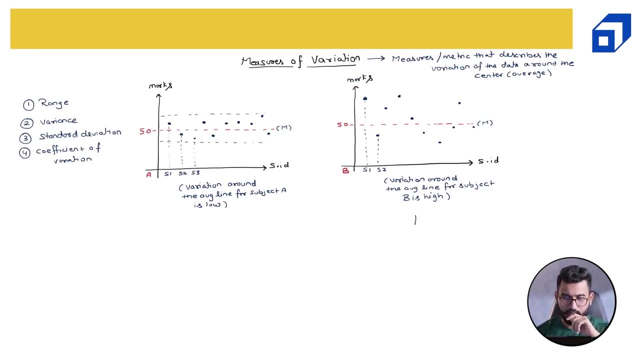 basically means the values are closely concentrated around the center point. for example, if I go back for this subject B, this one- you will get the value of Sigma, which is my standard deviation, to be high, while for B- sorry for A, which is this case- I would get the value. 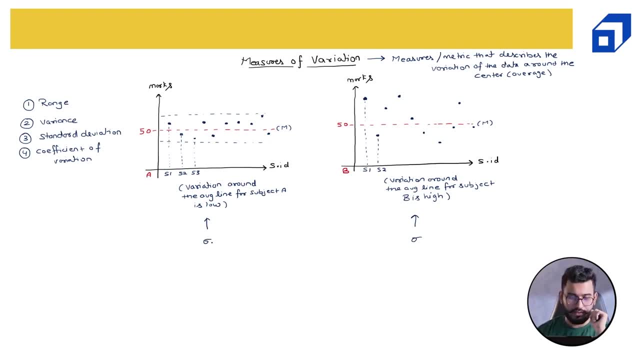 of Sigma, which is standard deviation, to be low. so if I call this as Sigma A and Sigma B, then my Sigma A would be less than Sigma B. the standard deviation in subject A would be less than standard deviation in subject B. when I say the standard deviation is less, 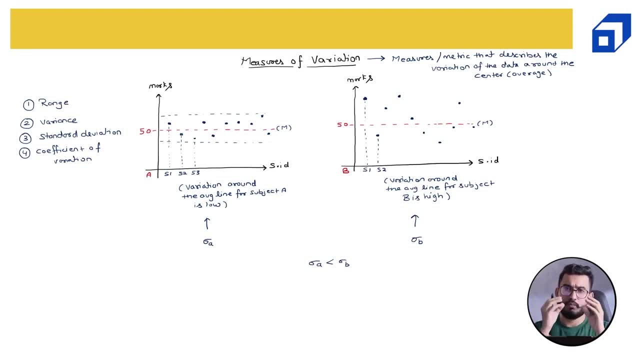 that basically means All the observation, or most of the observations, are scattered very close to the mean while when I say standard deviation is high, that basically mean most of the observations are scattered far away from the mean. now this gives you a better idea regarding how your 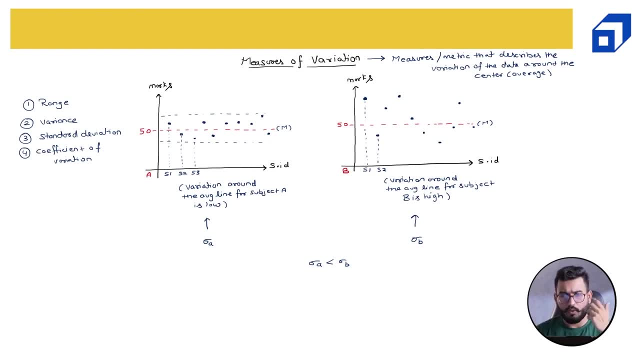 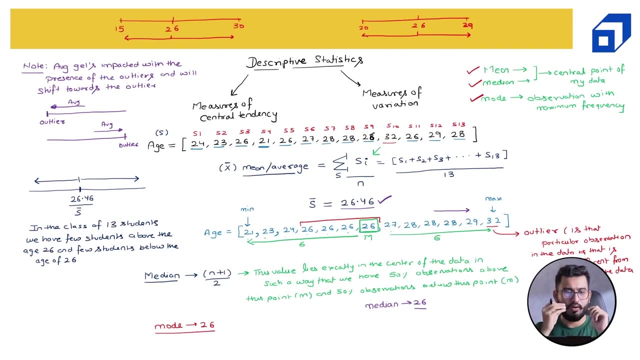 data looks like. if you guys want to practice, you can see that we have already calculated the mean, median and mode of the age variable. we were having 13 students and their respective age. we have already calculated mean, median and mode. now for practice, what you guys can do. you can quickly calculate the standard deviation of this particular. 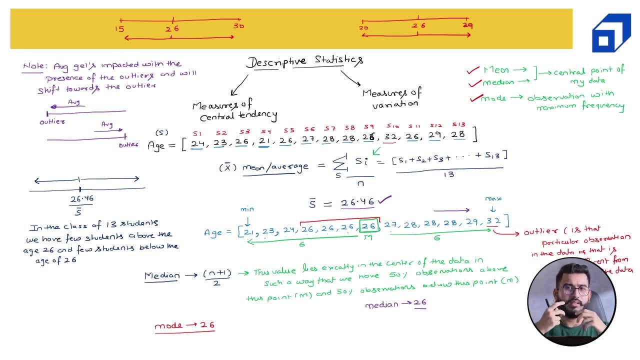 data and then you can try to understand it. so if you have to explain to the principal or to any person About how this class looks like. so we have already seen one segment that this class is having the median to be 26, which basically mean 50% people or 50% students fall below. 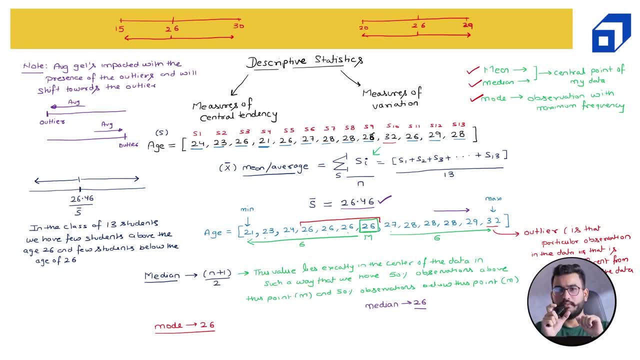 the age 26 and 50% fall above the age 26. now, if you get the standard deviation of, let's say, 5 years- I'm just throwing a value, don't? I have not calculated it, so I'm just giving you this task to calculate this- but let's say, if the standard deviation of this data is 5 years, 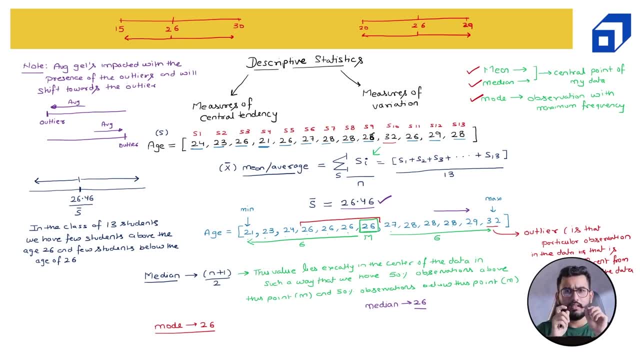 then that basically means on an average. on an average, these students are having 5 years above the above the central point, which is 26, so let me just quickly draw it. So Let's say This: This is my student ID. This is my age. 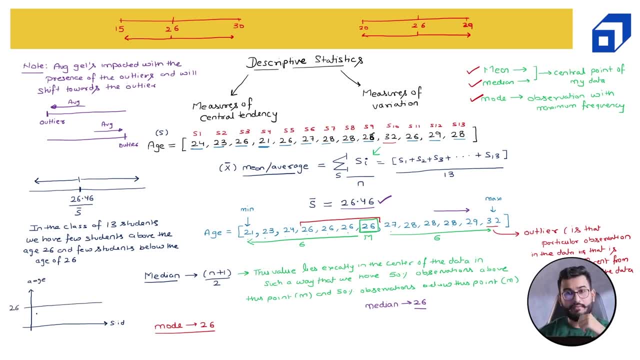 This is my center, which is 26, and if I'm having a standard deviation of 5 years, that basically mean I'm having few students who are above the age, above the middle age by 5 years. So 26 plus 5 will give you 31, right. 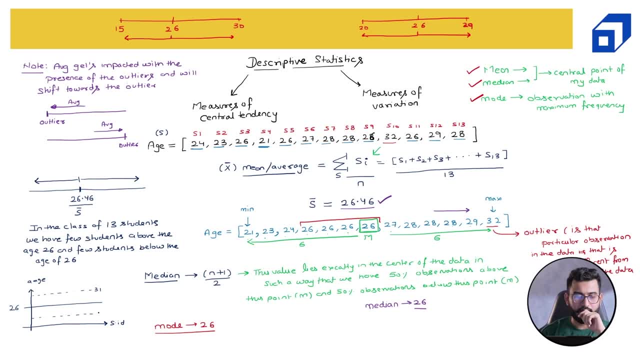 And Minus 5 will give you 21.. So you can see that. you can see that most of the students in your data are between 21 to 31.. Right, So using the measures of descriptor, measure of central tendency, we get the central point. 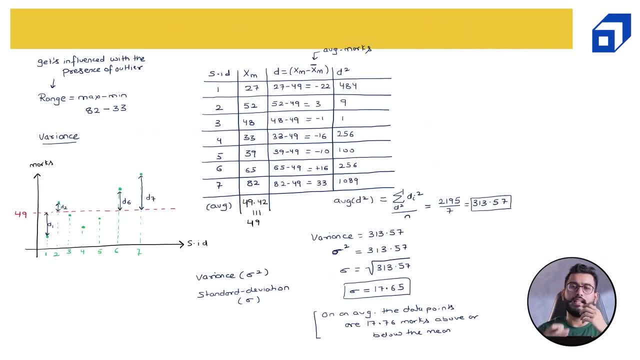 using the measures of variation, we get how the data is scattered around the central point. But There is a problem. The problem is, let's say, if I'm having two subjects, let's say I'm having a subject- maths- having a standard deviation of, let's say, 15 marks, and then I'm having age having. 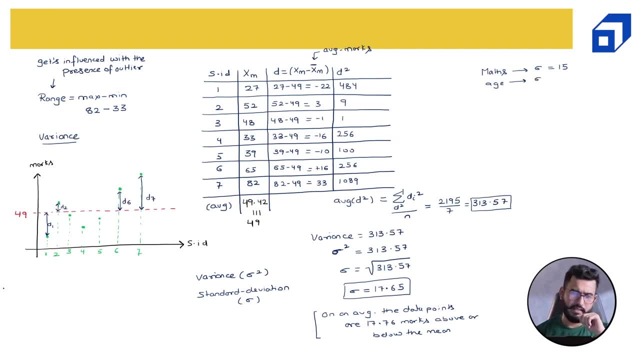 a standard deviation of maybe. let's say I'm having another subject, Another Six signs, Having a standard deviation of, let's say, 20.. Now can I compare these two standard deviation? can I say this is high and this is low? Well, we cannot do that using a standard deviation. we cannot compare the variations among the 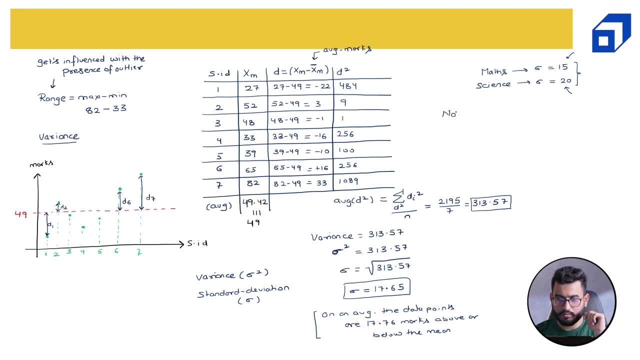 series. Now please remember- this is a very important note- That Standard deviation, Standard Deviation Talks about The variation In the individual series, Individual cities, And We cannot Use it To compare The variation Among the cities. 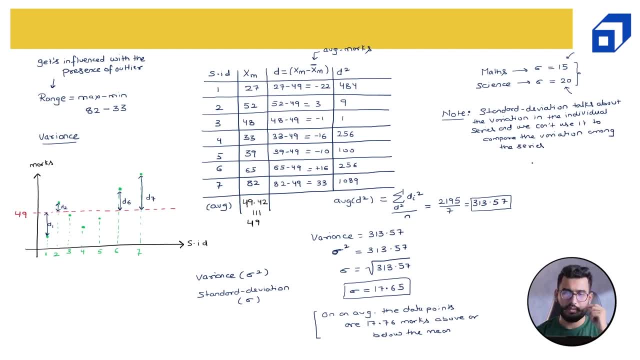 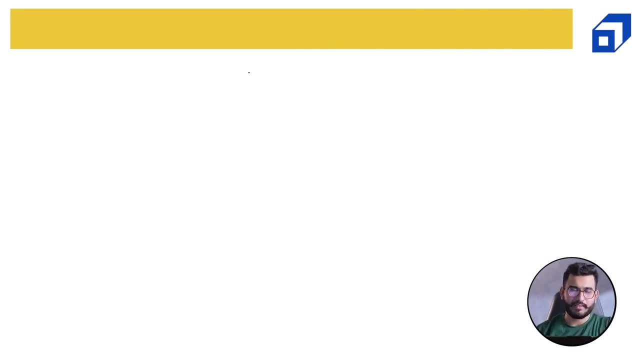 So how we can compare the variation among the cities. For this we have the next major, which is coefficient of variation. So now let's try to understand coefficient of variation. Coefficient of Variation: As I've told you, The standard deviation is limited. 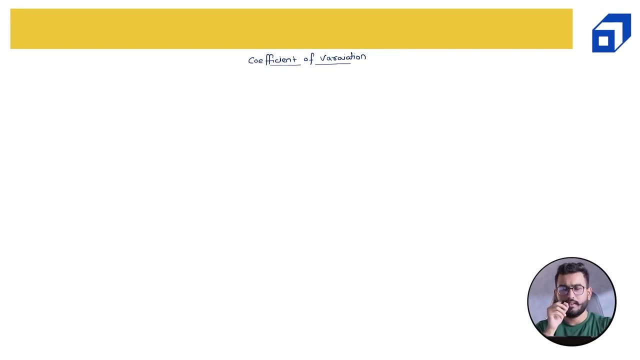 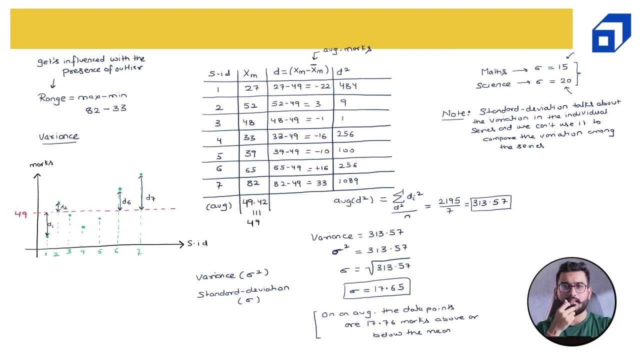 To describe the variation Within that series. So if I'm if I'm saying that the standard deviation Of the maths Marks is 15 and the standard deviation of science marks is 20.. I cannot use these two individual standard deviations to compare. 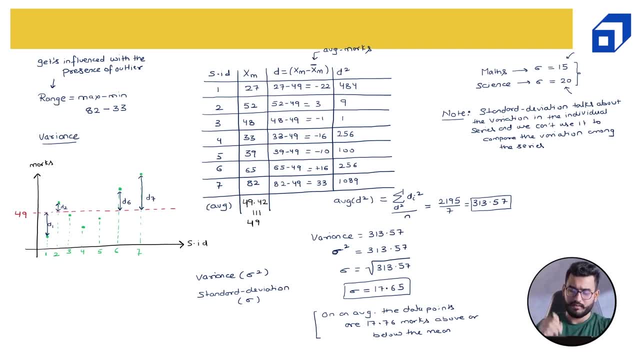 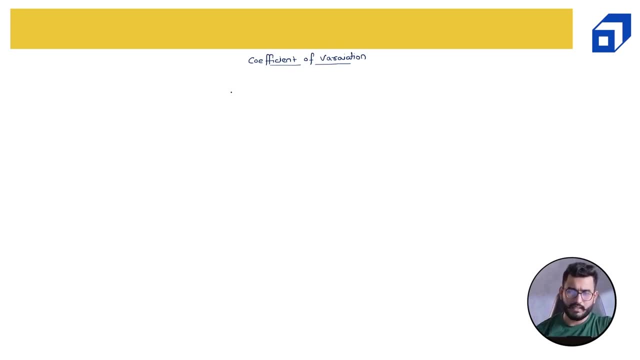 The variation Among the cities. For that We have a Different metric Known as coefficient of variation. Let's take one example. Let's take two series: Series X, Which is having One, two and three, Three data points. 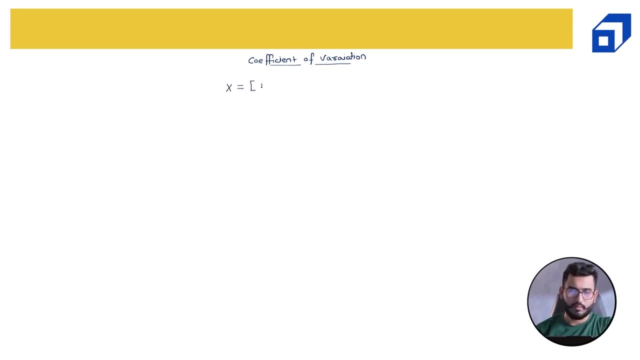 Series Y, Which is having Again three data points: One not one, One not two, One not three, One not three, One not four, One not five, One not six, One not seven, One not eight, One not nine. 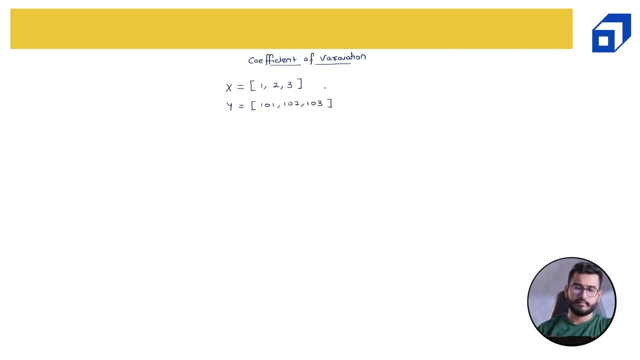 One, not ten. One not eleven. One not twelve. Now, if I take the average Of X, Which it will came out to be Two, Average of Y Will came out to be one, not two. Similarly, standard deviation of X. 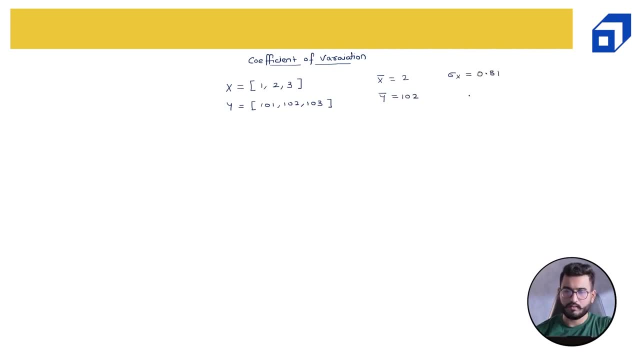 Will be Point eight to one. Standard deviation of Y Will be point eight to one. Now Both X and Y Are having the same standard deviation. Can I say that They have the same standard deviation, Or can I say that? 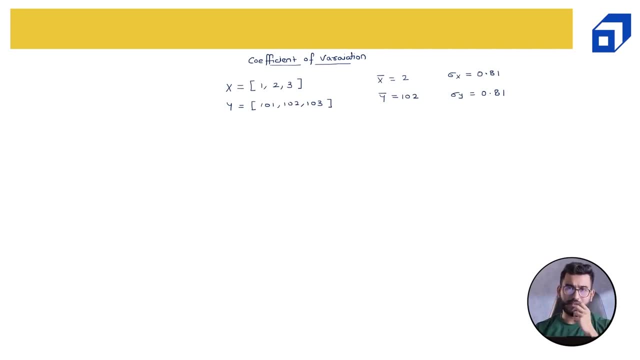 They are having the same variation. If you closely observe, You will find out that This is not true, While in the series X You can see that The third Element, Which is three, Is Three times Of the first. 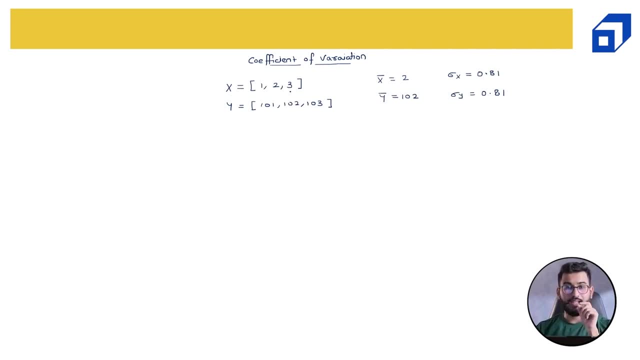 While in Series Y I cannot say The third element Is three times Of the first. But In Series Y I cannot say The third element Is three times Of the first. So They Both. 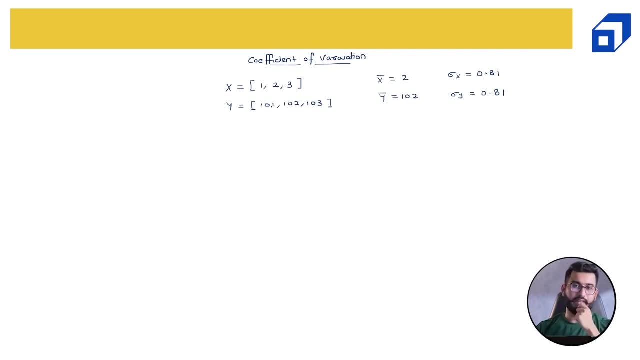 Are Not Having Same Variation. X And Y Are Not Having Same Variation. How We Can Compare The Variation, How I Can Say That X Is. 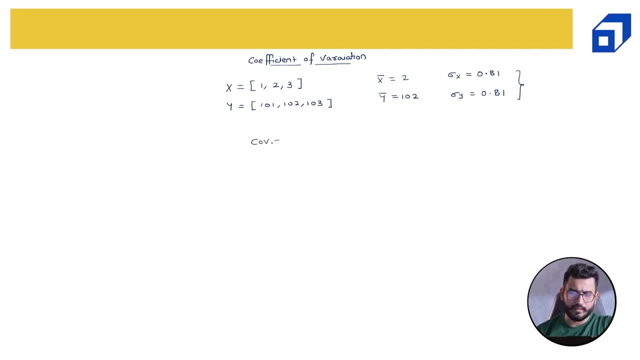 Having The First, We Have Coefficient Of Variation, Which Is Nothing But The Ratio Between The Standard Deviation To The Mean X Bar For Coefficient. 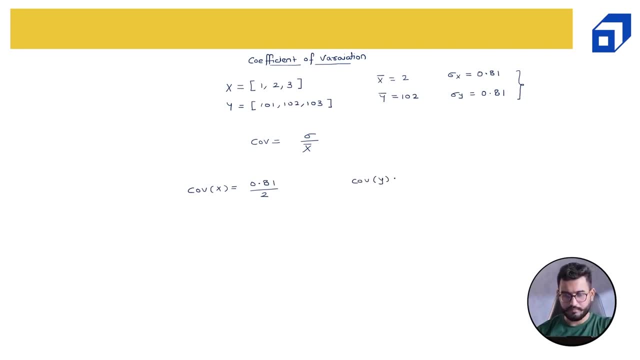 Of Variation For Series X Is No One, Not Two. So This Would Be Point Four Zero Five, And This Would Be Point Zero, Zero Seven. 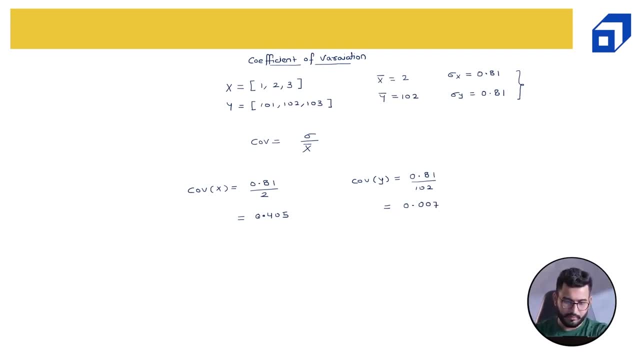 Now, If We Closely Look Into These Two Value series, which is, series X is having the coefficient of variation of 0.405, while series Y is having the coefficient of variation of 0.007, and I have already told you that the series X 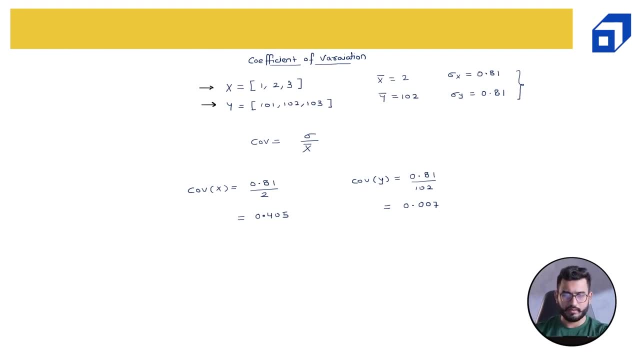 is having more variation than series Y, because in this series the third element is three times the first, while I cannot say the same thing for series Y, right? so when we have to compare two series, or we have to compare the variation among two or more series, we look 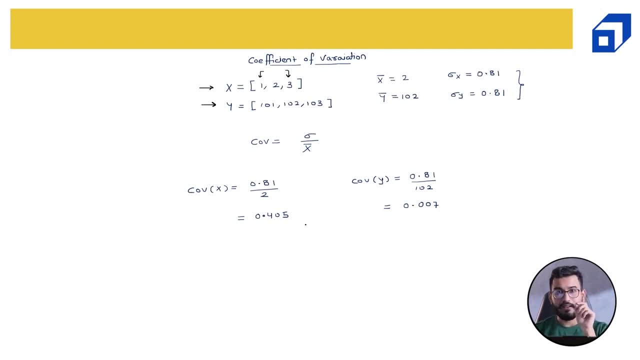 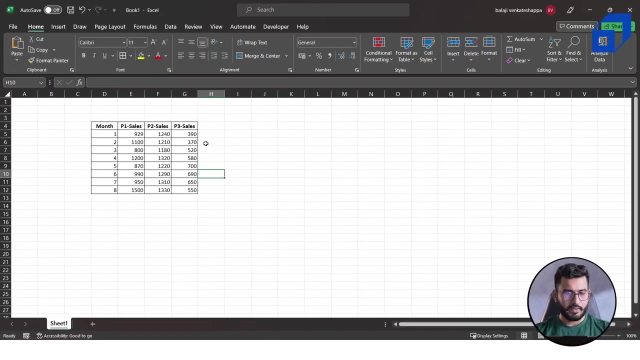 at the coefficient of variation. a higher value represents higher variation, so this series is having higher variation when compared when compared with series Y. so using coefficient of variation, we can simply compare the variation among the series and we should not be using standard deviation. I hope this makes sense now. here you can see. I have taken one simple example and here we'll. 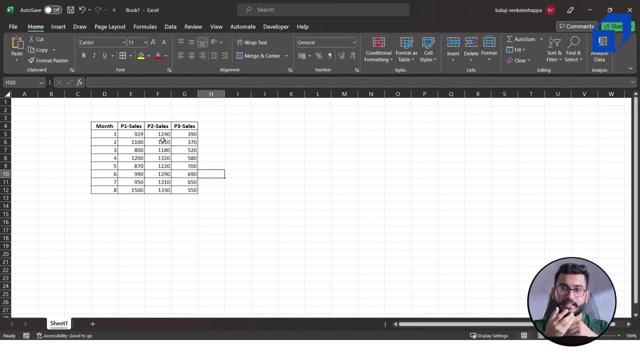 be using all the measures, which is, you can see, I have taken one simple example and here we'll be using all the measures, which is measures of central tendency and measures of variation, to understand how these three products are performing in terms of sale. and please remember, this is the number of units. so for 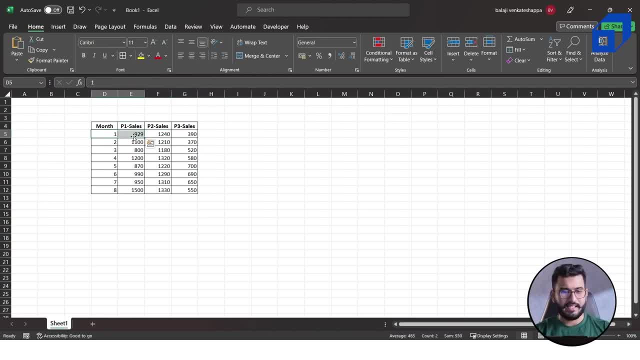 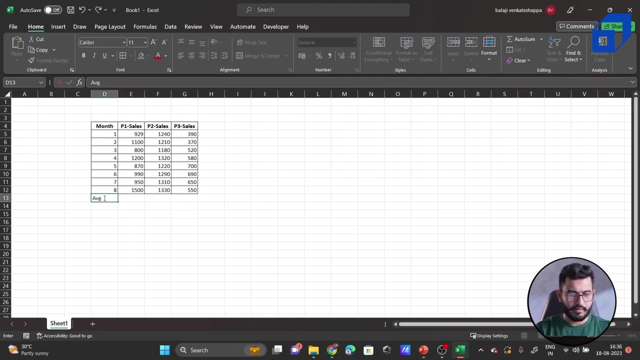 product number one in month one, 929 units were sold. similarly, for product two in month one, 1240 units were sold, and so on. so we can quickly find out the average median and mode for each of them. so is equal to average average of this particular column and I can simply extend this formula to all other sales. 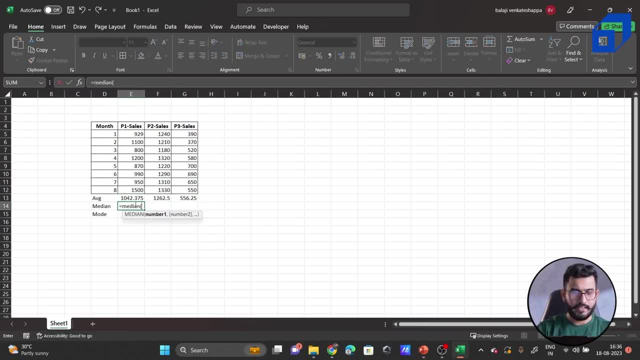 similarly, median will be is equal to median. I want median of all these sales and I can simply extend this to all other sales, and then we have mode. so is equal to mode. now, here, if you carefully observe, I do not have any mode, so my mode is not. 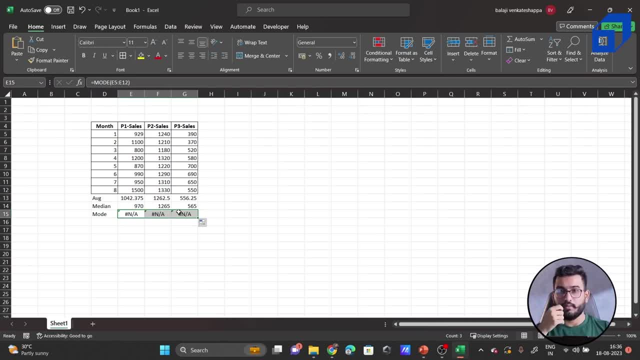 available and I have told you previously. so if I do not have any observation, which is, which is duplicator, which is repeated for more than one time, which is having the highest frequency in our data, we will not be having a mode, so we only have average and median. 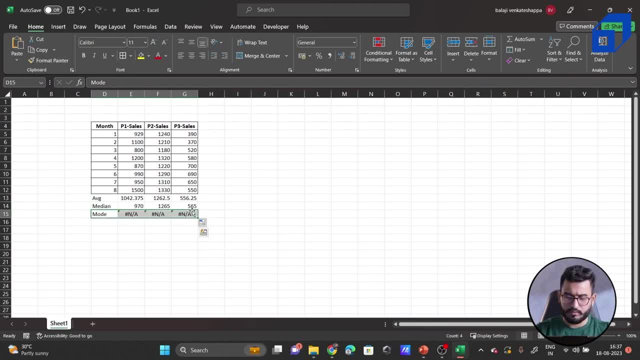 so I will simply delete this because we don't have a mode, so let me delete this now. if you compare the average and the median, you can see that for the sales of product number two, the average in the median is quite close to each other, While the same thing can be viewed for product number. 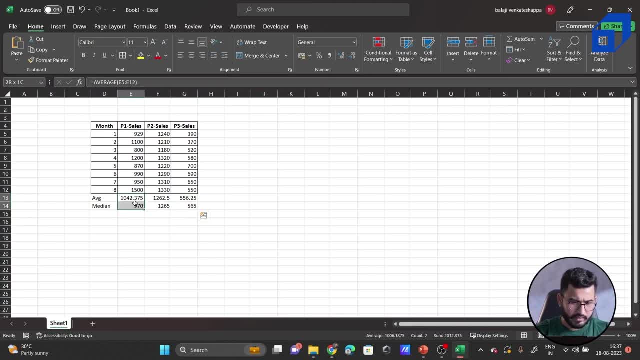 3, but there is a difference. There is a vast difference. I would not say vast, but there is a quite a good difference in the average and the median for product number 1.. Let's try to look at the measures of variation also. So we will calculate the standard deviation. 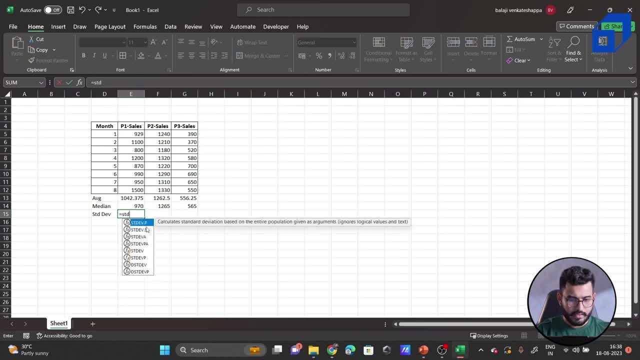 So is equal to SDDEV, and we will use this SDDEV, this one, a standard deviation, And I can just simply extend this. Okay, And now we will calculate the coefficient of variation, COV. So this is given as uh. 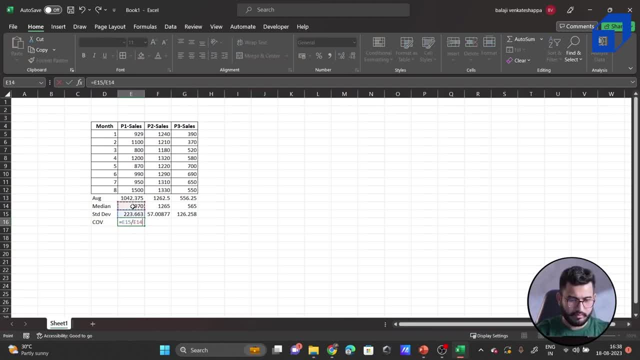 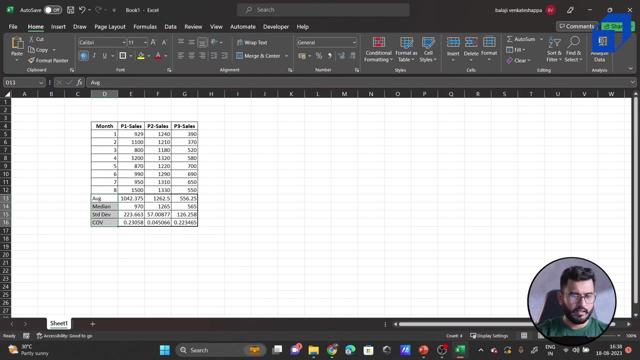 the standard deviation divided by its average. Now, these are the numbers which we have to carefully read and make sense out of them, What we can conclude about these three products. Let's try to understand them. Okay, Now, if you carefully observe- and uh, I would start with product number two, first In product, 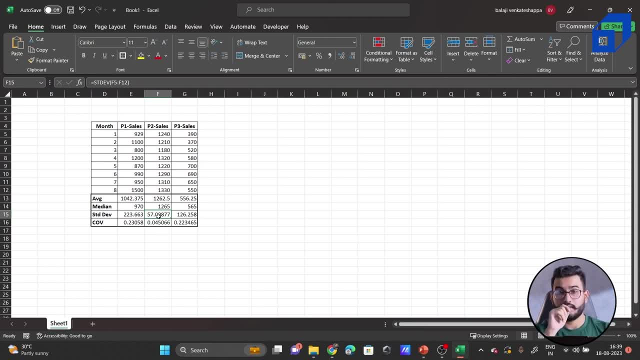 number two, you can see that the standard deviation is very small, Um, while the coefficient of variation is also very small. Uh, here also, you can see that coefficient of variation is 0.23.. Here it is 0.22, but here it is 0.04.. 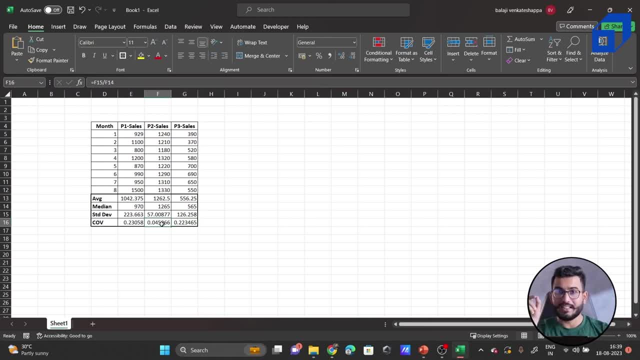 Which basically mean among all these three series, the lowest variation is with the sales of product number two. Also, if you look carefully, the median and the average is very close to each other. Also, the average is highest among all the three products. So what I can conclude? 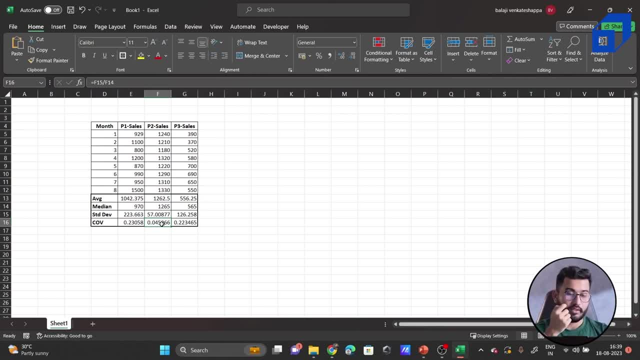 about product number two. number one: the product number two is very stable And number two is very stable in the market because it is not. it is not having variations in month Number one: same sale. in month Number two: approximately same sale month, or three same sales, and so on. 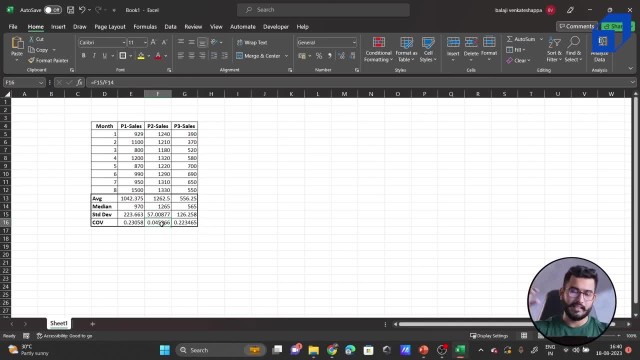 Also, it is always consistently high, And that is the reason that average is, uh, the highest, at 1262.5 units. for product number three, a similar behavior can be seen, but on the lower side. uh, the average is 5, 56,. which basically means, when compared with product number one product. 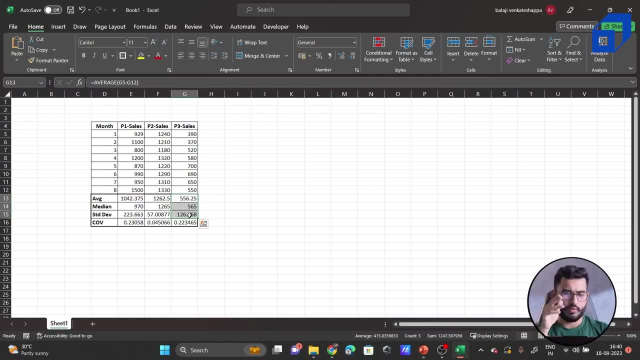 number two and product number three. when, when compared with product number one and two, the sales of product number three is on the lower side, all the lowest, decide by in the coefficient of variation. This, which is product three and product one, is approximately the same, which basically. 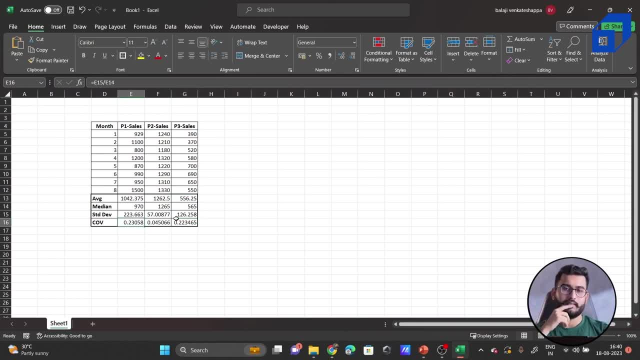 means they both are varying at the same rate. the variation is approximately the same. So you can you can assume that one, which is product number three, is on the lower side and it is varying around that. product number one is on, is on, maybe second lowest and varying around that and product number. 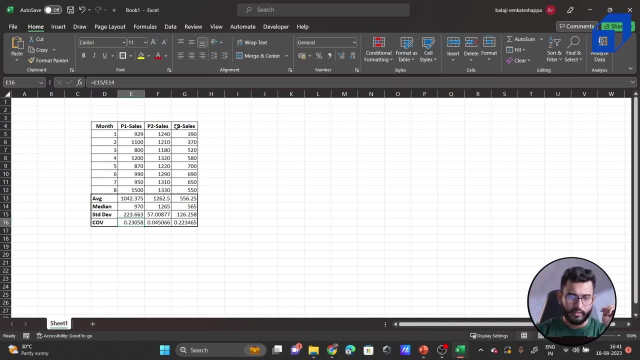 two is on the highest. so if I just color code them, I would say product number three would be coded as red product, one I can put it as yellow and two I can put it as green. and the reason I'm putting it as green? because it is the most stable product in the market, while 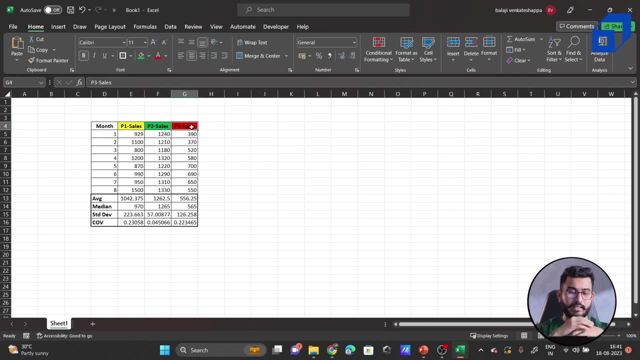 sales of product number three is on the lower side. that's the reason we have assigned a red color. and product number one is having the sales between the highest and the lowest sale, which is product two and product three, So we have assigned it Yellow color. 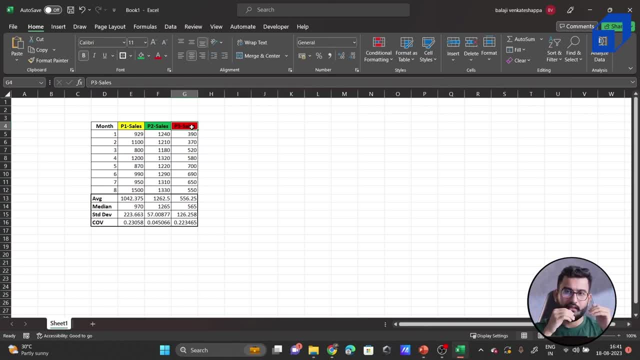 Now you can see that, using these measures, we can better make conclusions about the data, we can better explain the data, and that is the power of descriptive statistics. So you have seen that in this particular descriptive statistics segment, we have talked about how we can explain the data, we have talked about the various types of variables, we have talked 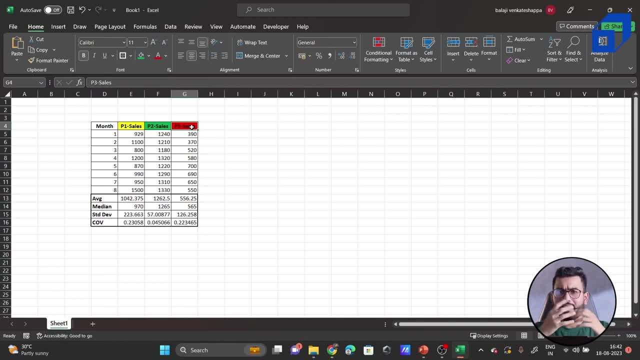 about qualitative, quantitative, Quantitative, quantitative, Quantitative, quantitative, Quantitative, quantitative. Right then we started our discussion around what are the various measures of central tendency. we talked about mean median mode, then we compared all of them. then we talked about measures of variation, where we looked into range, variance, standard deviation, coefficient of variation. 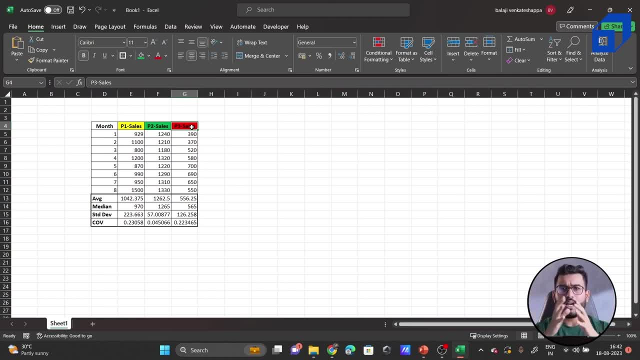 and, finally, we have concluded all our learning into this table, where we have compared the sales of these three products to conclude About which product is better and which product is not good. Now, this is what the application of descriptive statistics is. there is one small topic which 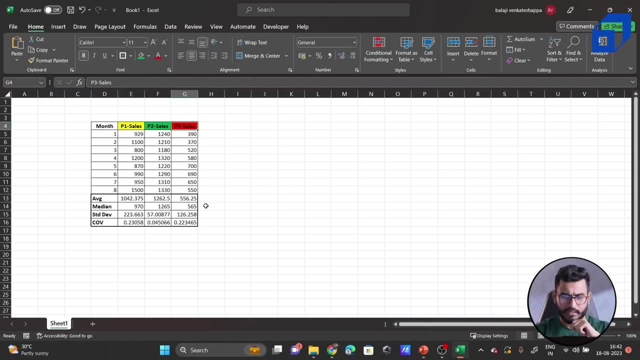 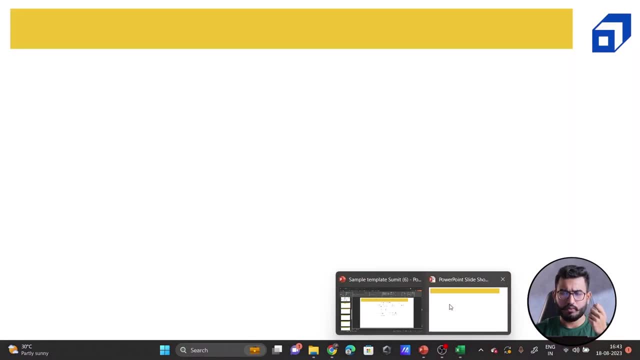 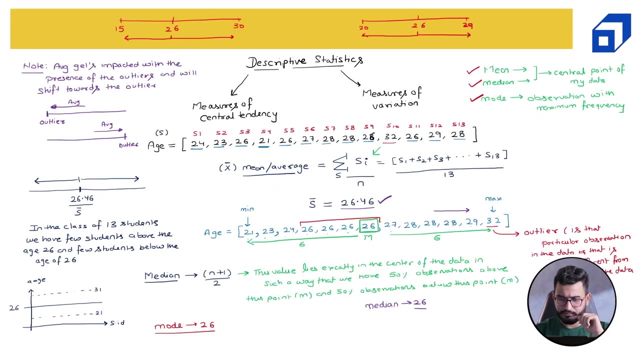 is very little related to outliers. I'll just quickly explain you that, though that is not so much common in the in the descriptive world, but quite important to understand. I have told you about outliers right over here, So I have told you that in this particular series where we have, the age, 32 is considered. 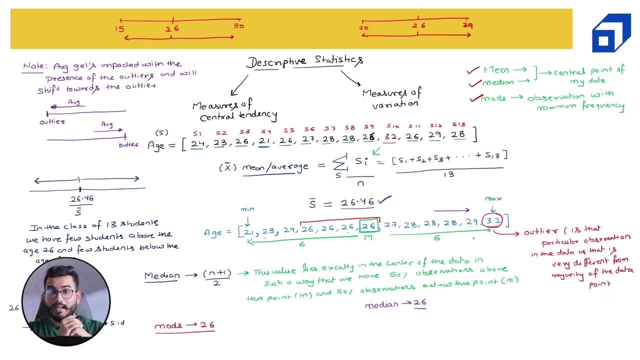 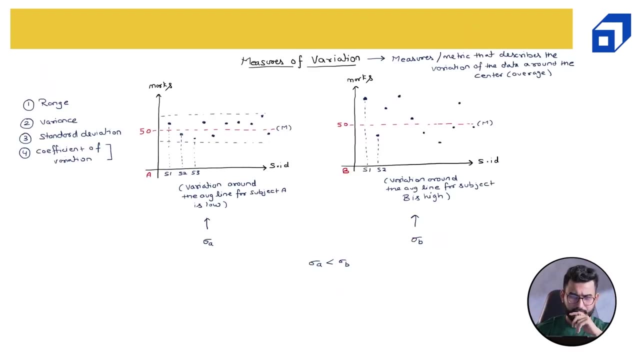 as outlier, and what is outlier? outlier is that observation which is very different from majority of the data. Now, there is one particular topic which is known as the leveraging point or leveraging data point. What is that? Let's take one very small example. So let's say: 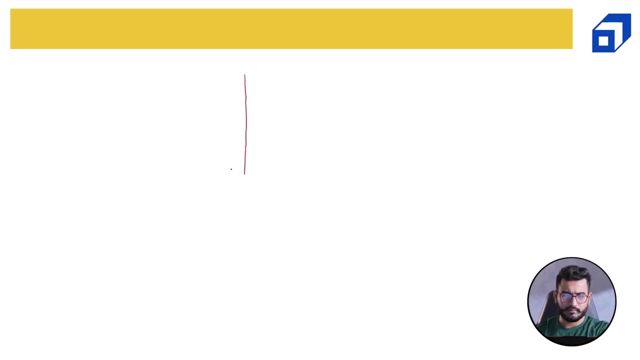 I have this data And this is the stock price. So here we have the day of the month And here we have the stock price, Stock price of a political stock. Let's say, on day one the stock price was somewhere around here. 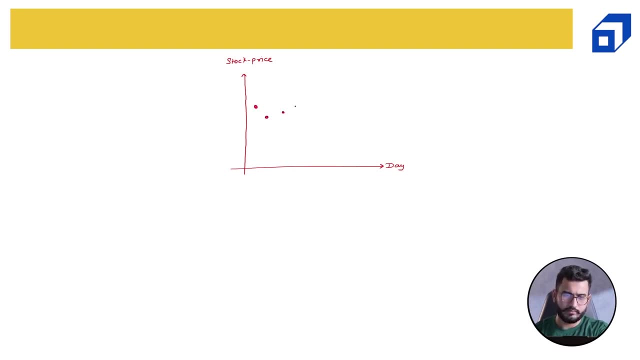 Then over here, Then here, then here here, And one day it jumped over here. One day it jumped over here, then came back to its normal position, like this: Now, at the very first like: if I provide you with this data, all of you will say that this: 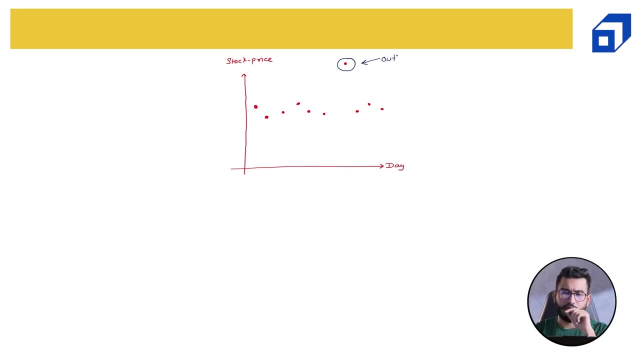 is outlier. This is particularly the outlier data point, Which, is true, This is outlier, But as soon as I provide you one additional information, your answer will change. Now, if I told you, if I tell you that on this particular day- let's say this is day- 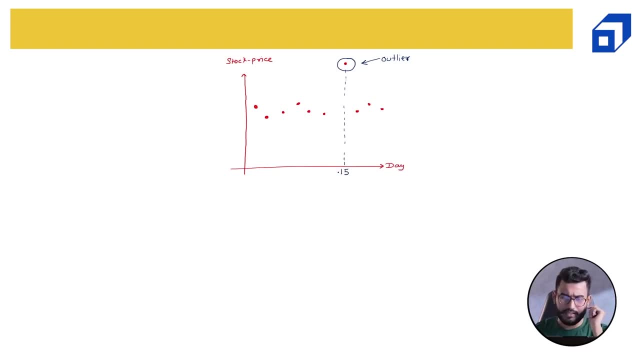 Day number 15th, or maybe let's say day number 25.. So in the 25th day, 25th day, 25th Day Of Of Month, Month, Let's say March 2023.. 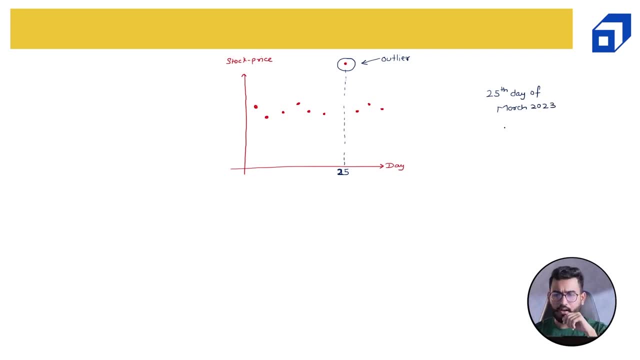 Let's say the stock market or the stock exchange, Stock exchange, or let's not talk about stock exchange. Let's say this company. Let's say this is the stock price of the company Reliance, Reliance. So On 25th, 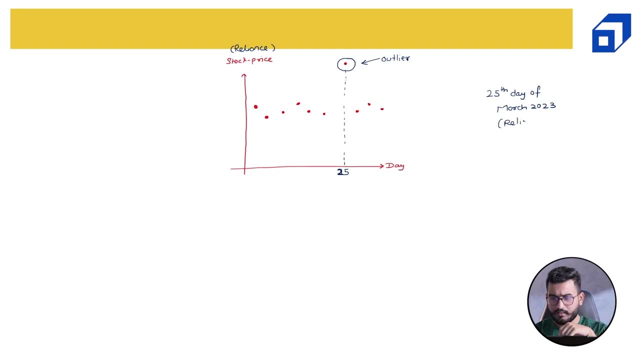 Day Of March 2023.. Reliance Announced A Major Product. Announced A Major Product. Announced A Major Product Or They Made. They Basically Conducted. 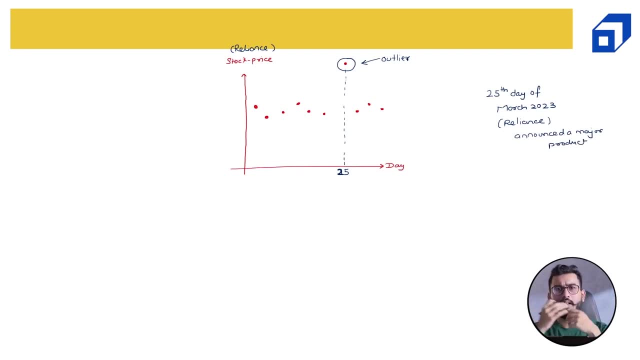 A Conference. They Conducted A Conference Change In Their Policy Of Major Change In Their Product, Due To Which The Stock Price Suddenly Raised To 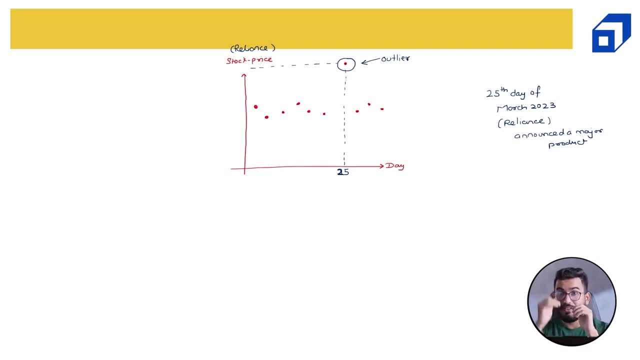 This Particular Point. Now, This Is Not An Outlier, This Is The Leverage Data Point. So There Is A Difference Between Outlier And Leverage. 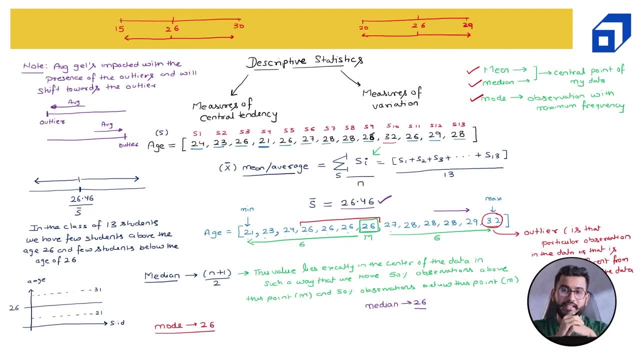 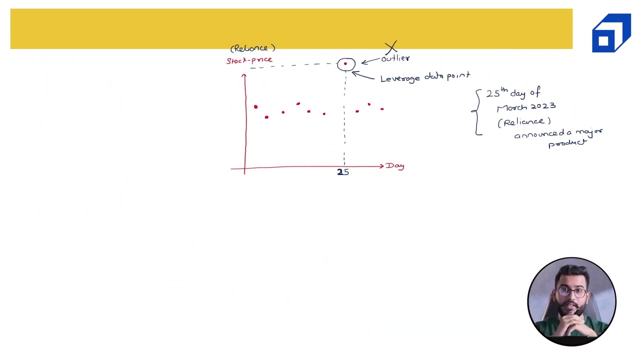 Data Point. If I Go To This Particular Example Of Age, I Can Not Say This Is An Outlier For, But In This Case, Where 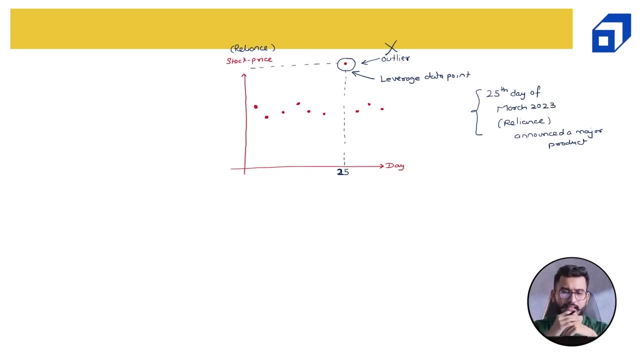 We Are Considering The Sales Of A Particular Stock Price Or Stock Price Of A Particular Stock, Let's Say Lines. This Data Now We 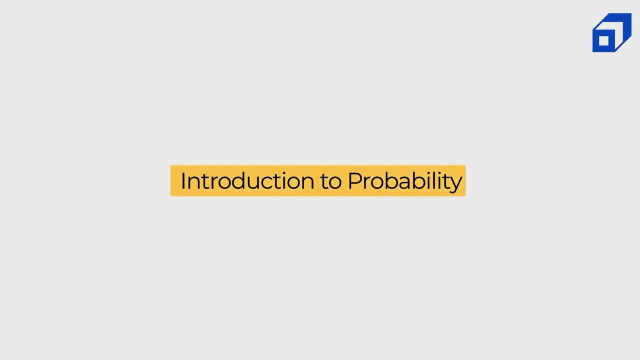 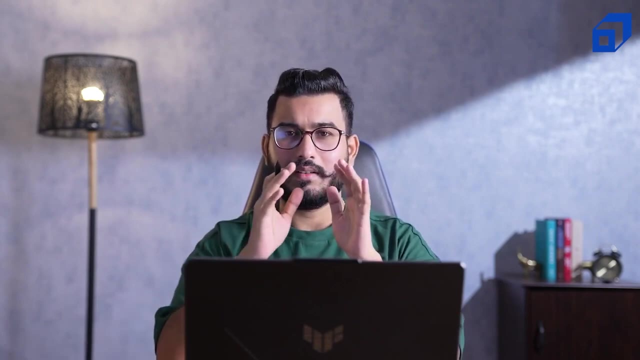 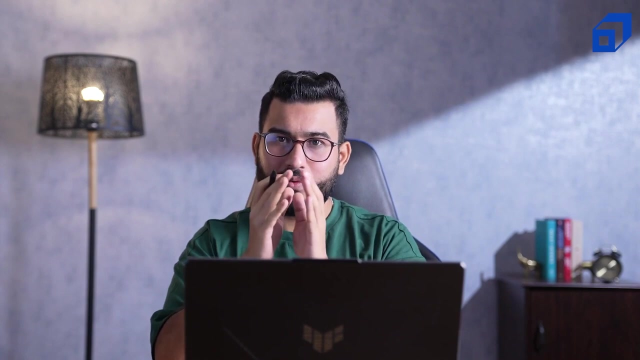 Will Move Forward To The Next Particular Discussion, Which Is Probability. So Now Let's Start With The Topic Probability. Now We Started With Descriptive. 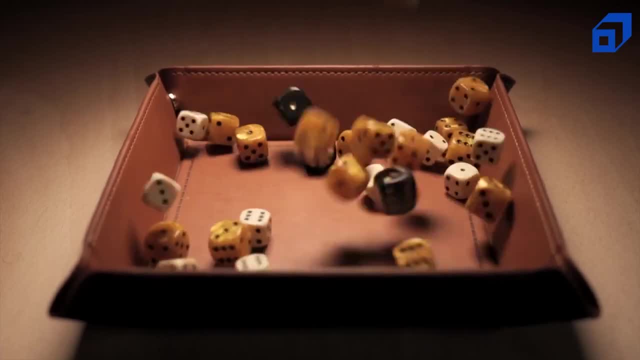 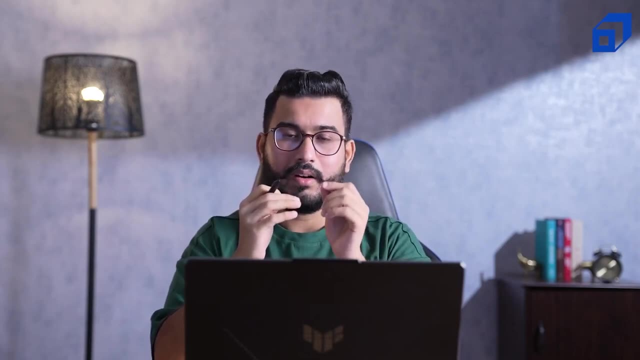 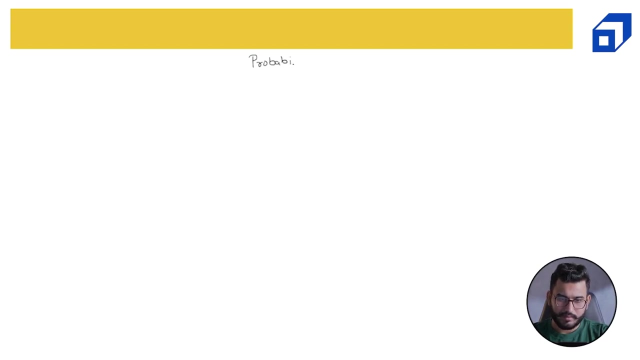 Statistics. We Have About It In Your Tenth Standards Or Maybe In Your College Days, But Today We Will Try To Understand The Most Important. 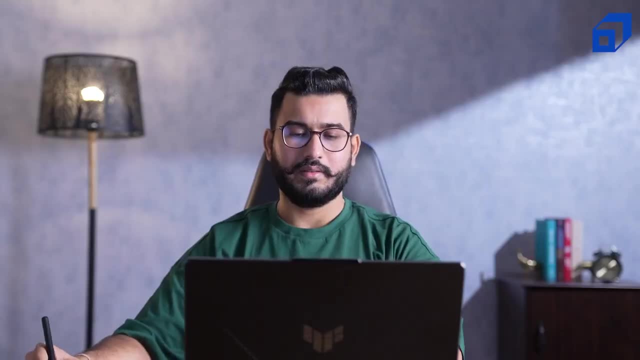 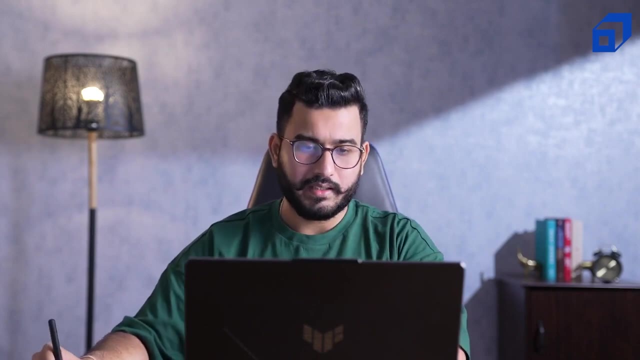 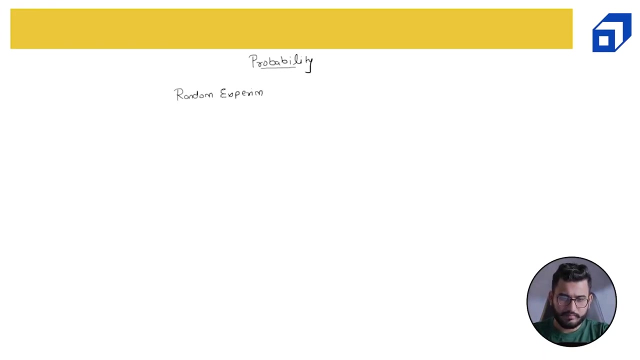 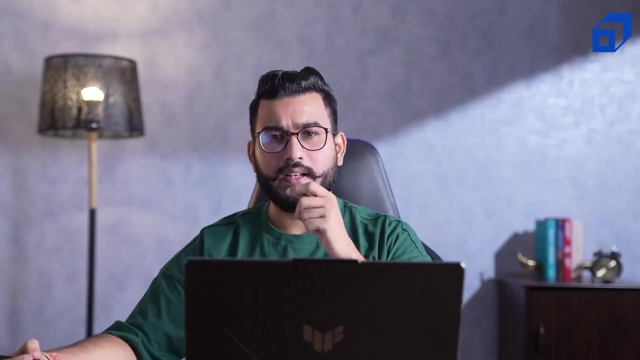 Topics Within Probability Which Will Help You In Probability. We Have To Understand What Is A Random Experiment. Random Experiment Is A Particular Experiment In 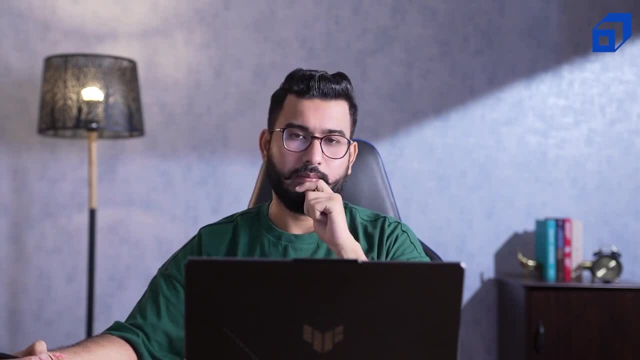 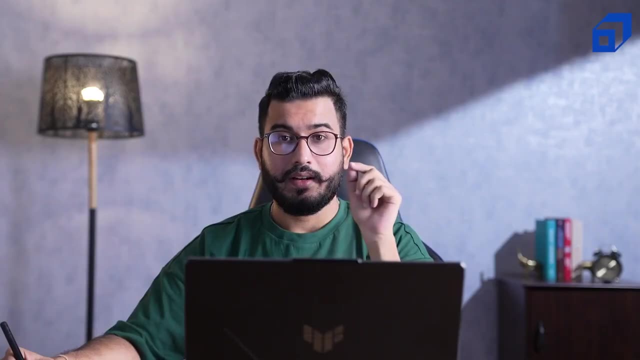 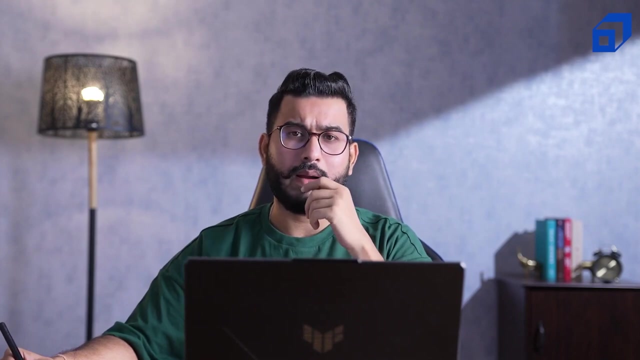 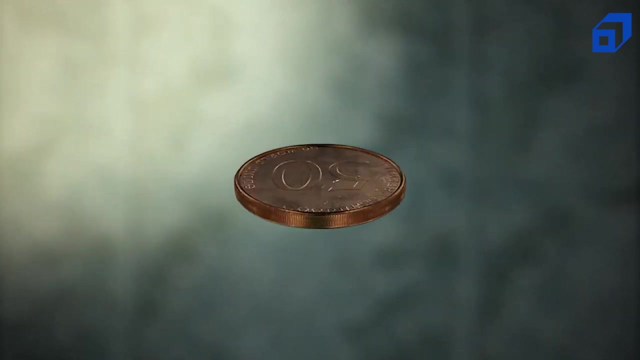 Which You Are Not Certain About The Outcome. For Example, If I Have A Head Or A Tail Right, If You Are Certain About It, Then 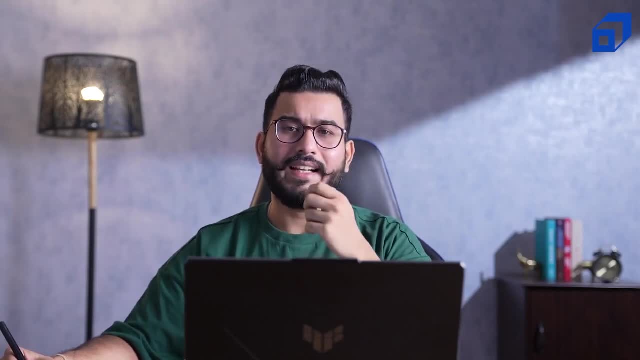 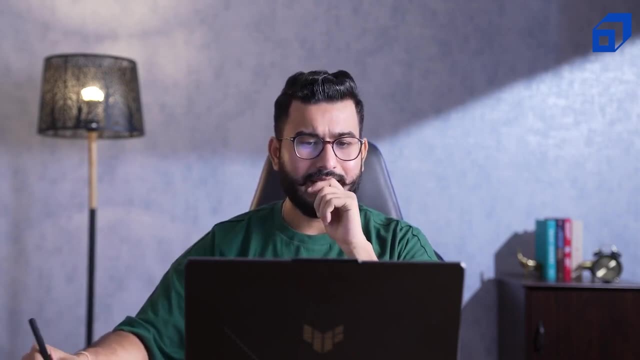 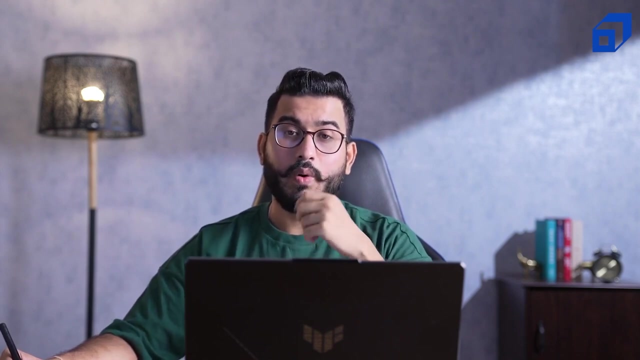 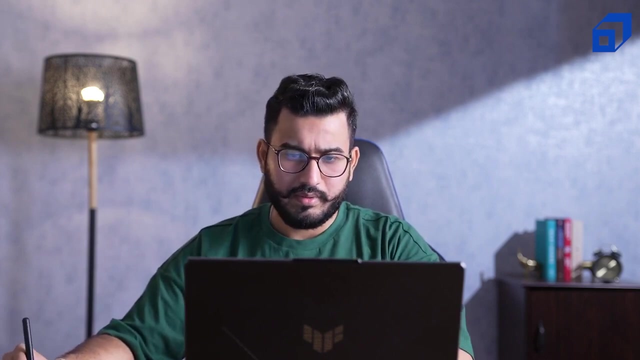 We Don't Need Probability, Right? So Let's Say, If I Already Know That The Coin Is An Experiment Or An Event For Which I Am, 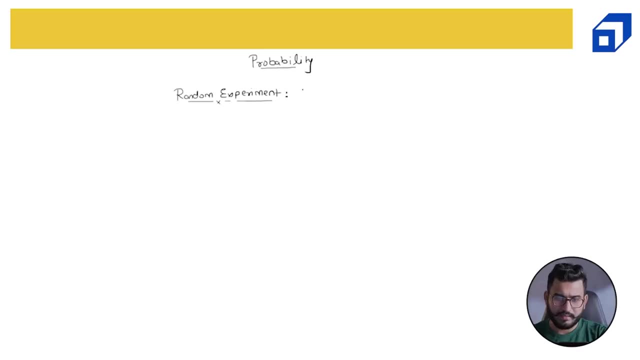 Not Sure About The Outcome. I Am Not Certain About The Outcome, So Let Me Just Quickly Note It. Outcome For Example: Roll Roll Of A. 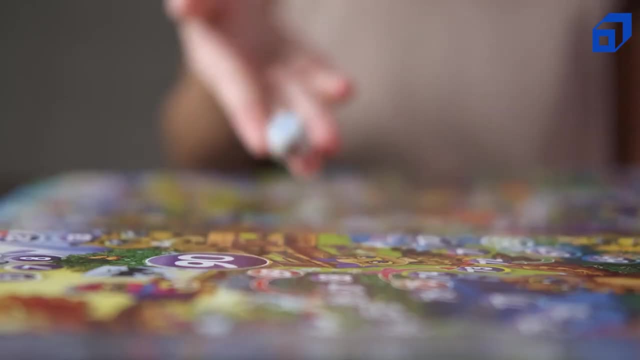 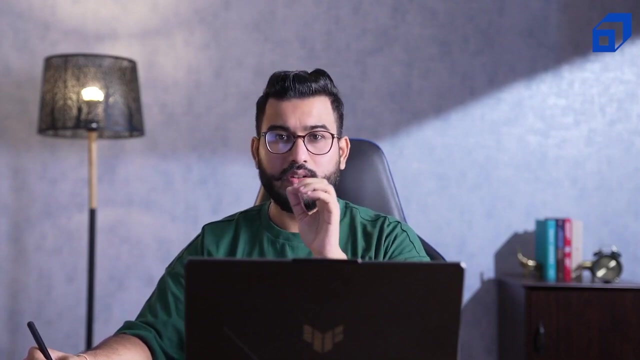 Dice, Roll Of A Dice. Now, If I Roll A Dice, I Know That I May Get One. So Either One, Two, Three, Four, Five, Six. 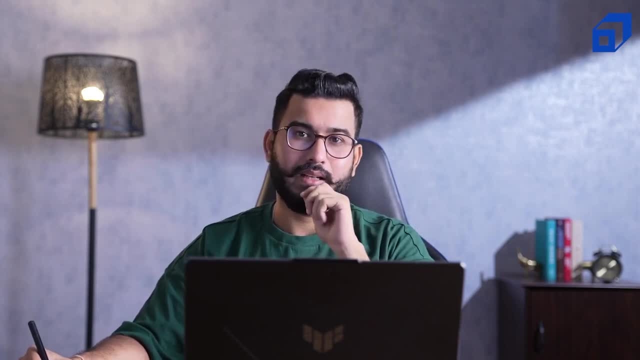 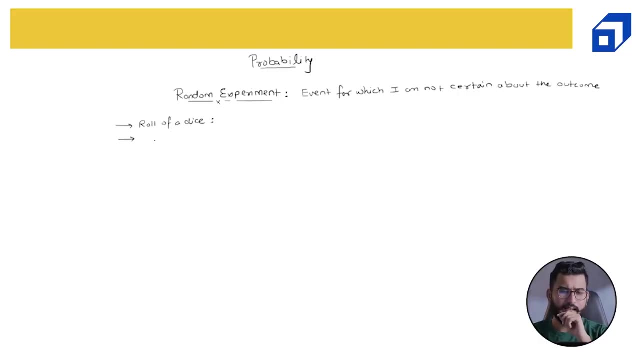 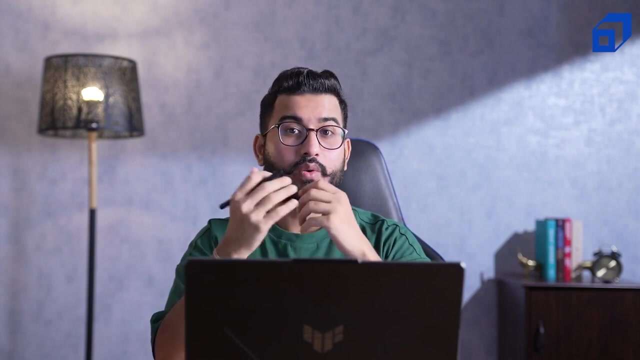 So Rolling A Dice Is Particularly A Random Experiment, Because I Am Not Certain About What Is Going To Be My Outcome. Similarly, Let Say Again: 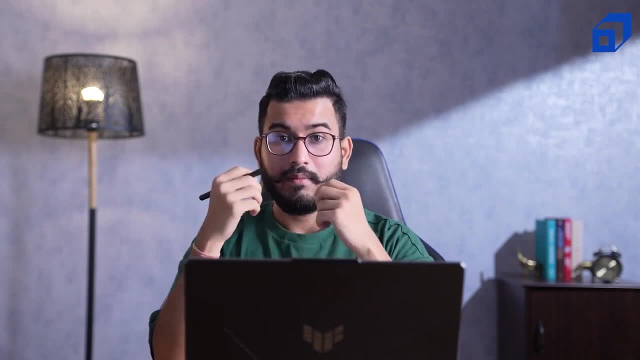 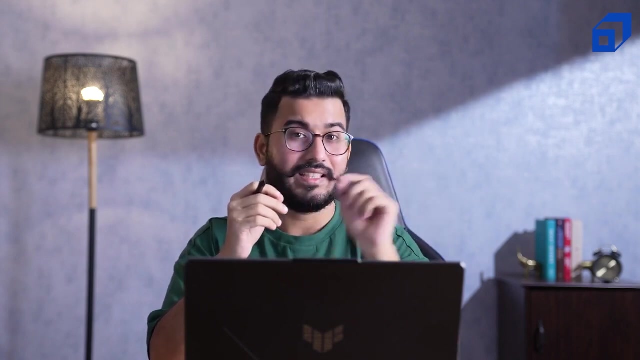 About What Is My Birth Date? So For My Mother, My Birth Date Is Not A Random Experiment. But For All Of You Listening My Birth, 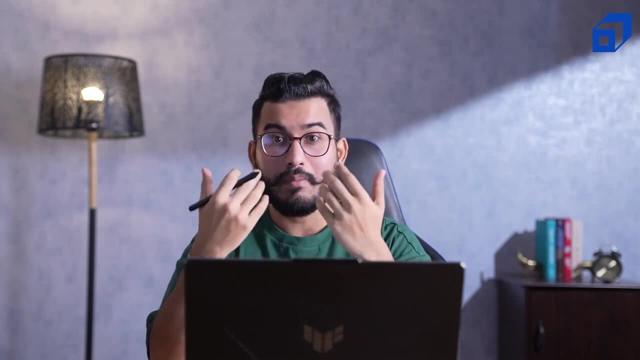 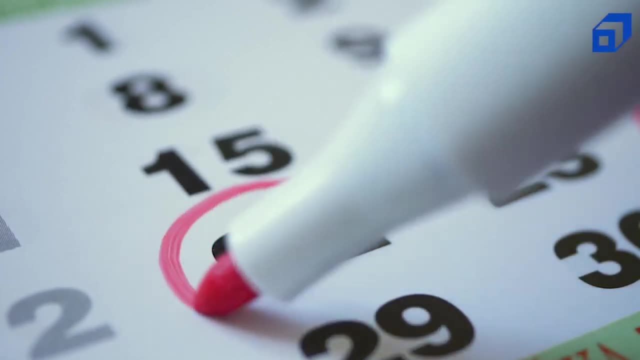 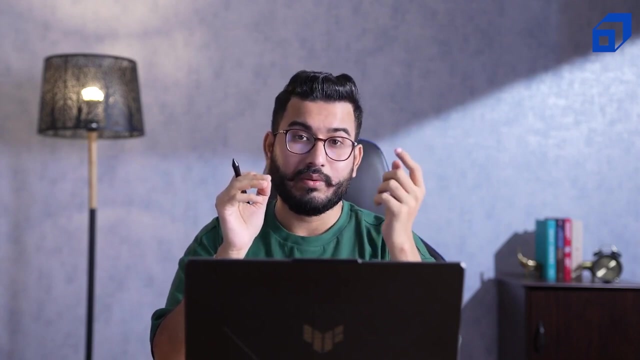 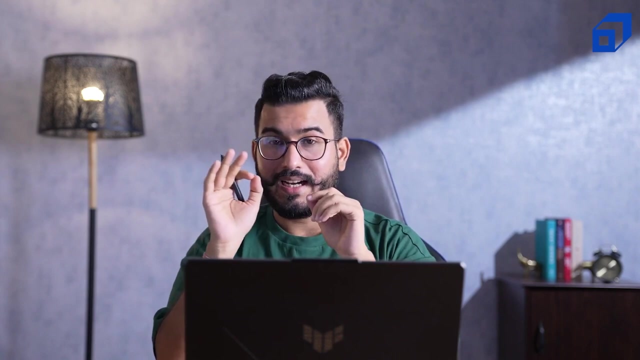 Date Is My Birth Date. If You Know About Me, If You Are My Friend, Then You Might Be Very Much Certain That My Birth Date 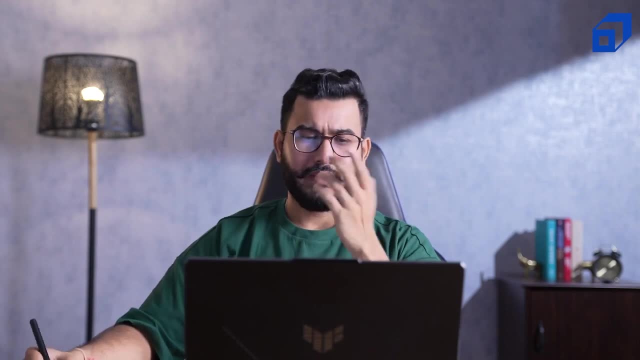 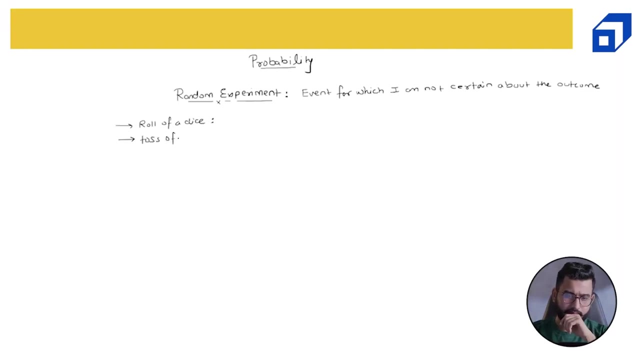 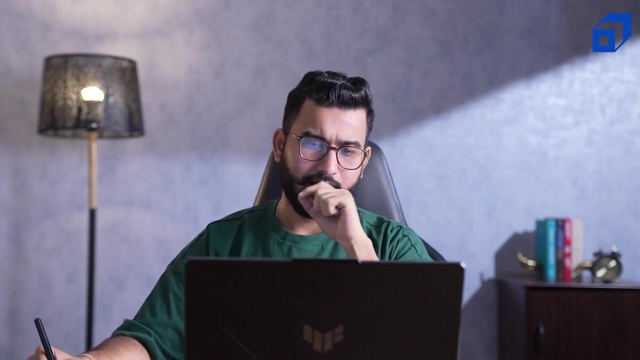 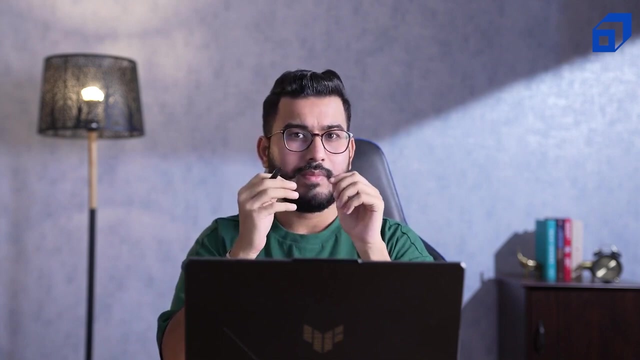 Is In This Year. This Is My Birth Date. Is Not A Birth Date. Is My Birth Date. Is My Birth In You Birth Date This. 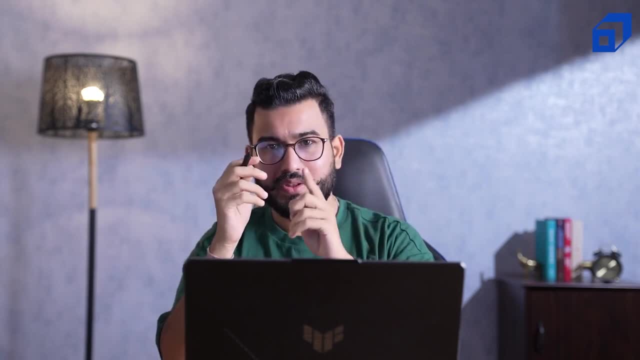 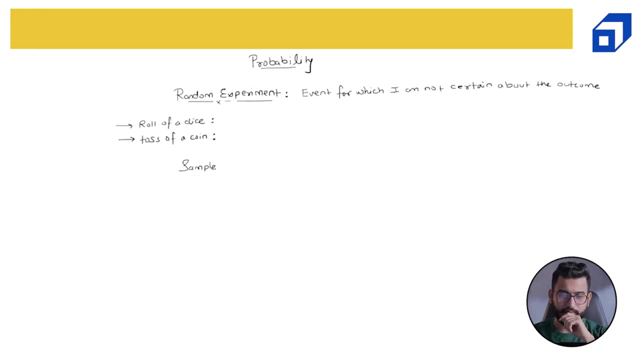 Is My Birth Date Is When My Birth outcomes out of an experiment is known as the sample space. So what is the sample space? The set with all the possible outcomes out of an experiment. So if I take the example of roll of a dice, I may get one, two, three, four, five, six. 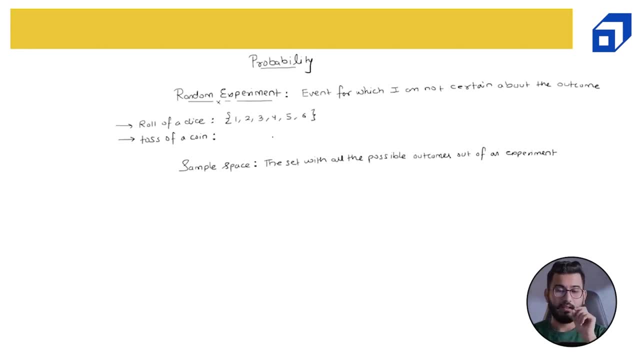 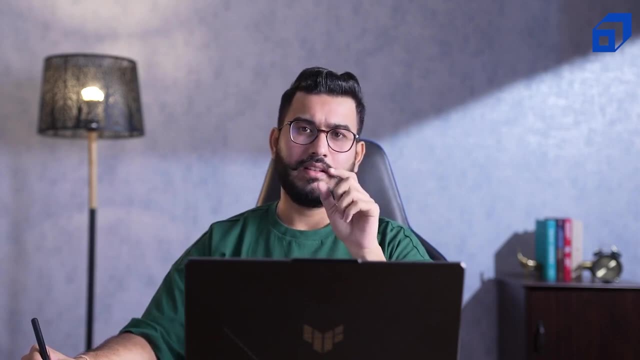 five or six. So this is my sample space for rolling a dice for toss of a coin. Now, if the coin is a fair coin, which basically means one side will be head and one side will be tail, So I may get either a head or a tail. Now this is basically my sample space for the 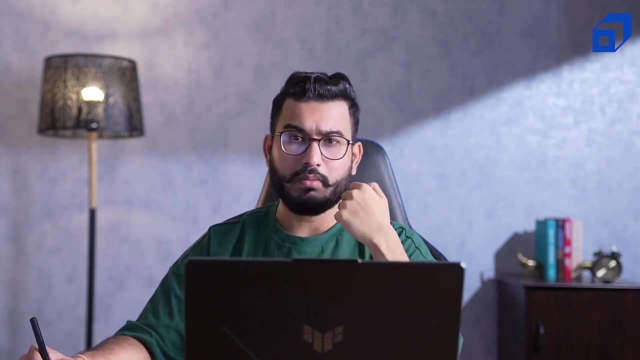 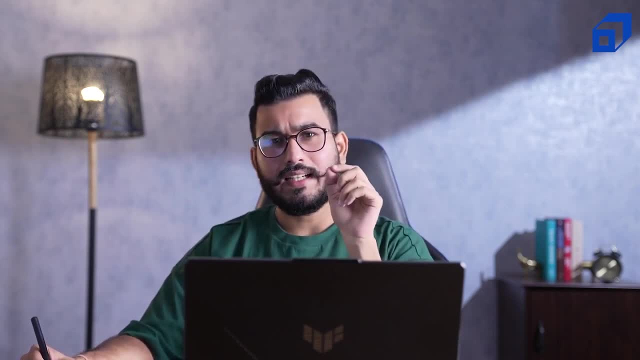 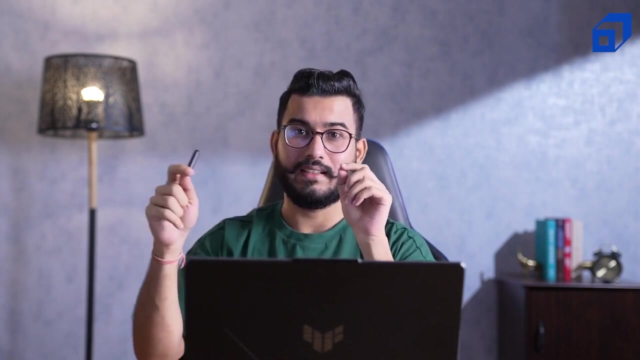 let's say, let me not, Let me just limit the sample space to 19- 96.. So if you know that the birth year is 19: 96, that in that case the sample space will be all the months and within each month all the dates or all the days, So your sample space will have quite 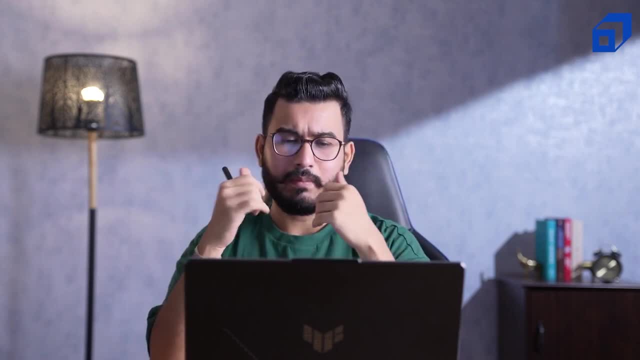 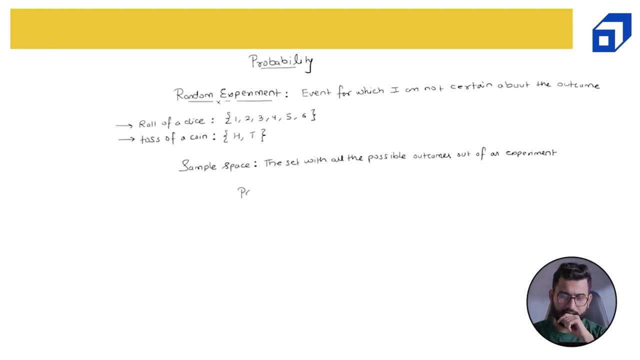 a good number of outcomes, right? So this is what my sample is Spaces. Now, what is probability? So probability of a potential event? X is basically how many times that event has occurred in your sample space, So number of times the event occurred in the sample space, and we divide this by 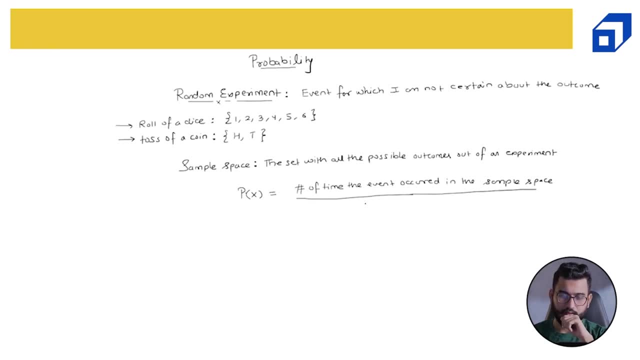 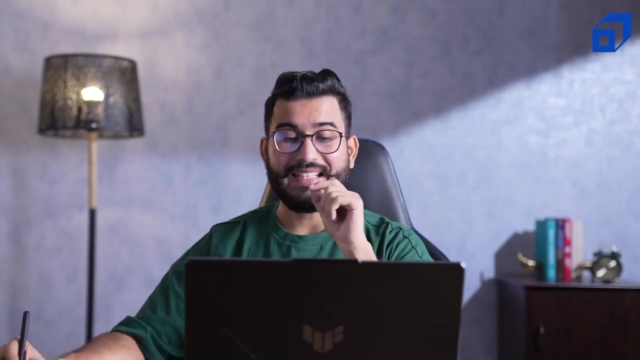 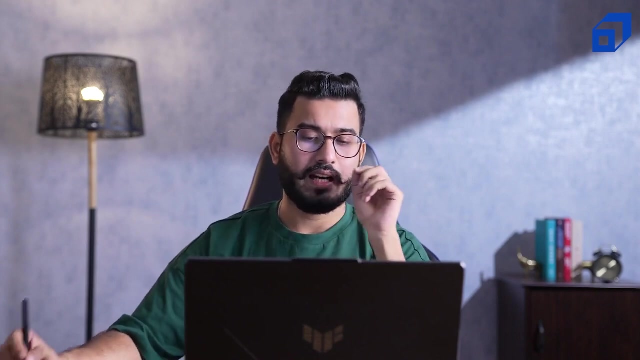 the total size of the sample space in total number of outcomes. so total number of outcomes in my sample space. Now please remember one thing: if I go with the definition- this is the very accurate definition- that the number of times a particular event has occurred divided by the total number of outcomes. 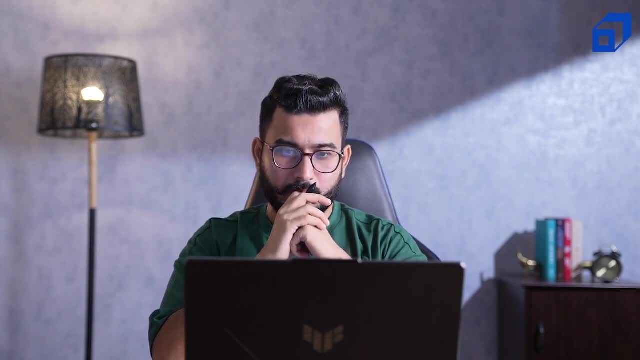 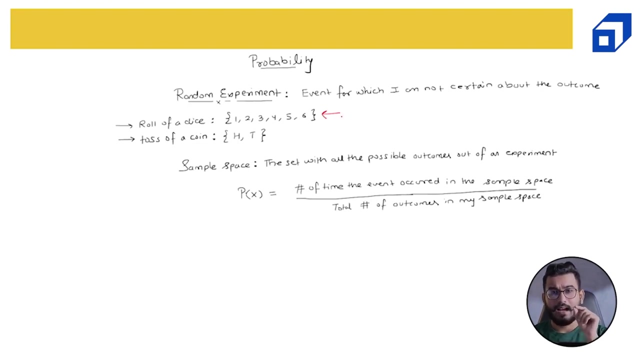 or total size of the sample space, but there might or there may be various ways of writing a sample space. let's try to quickly understand the difference, because this is the major mistake most of the students commit while calculating probability. so this particular sample space is having all the outcomes which 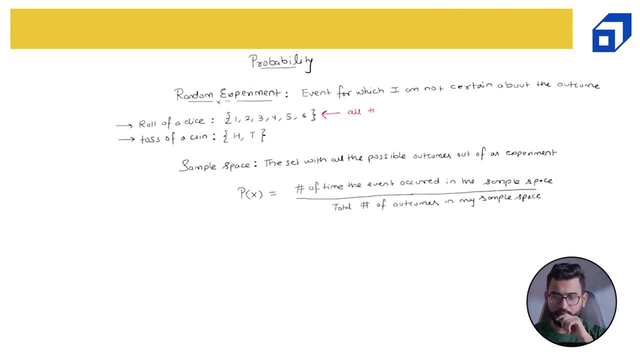 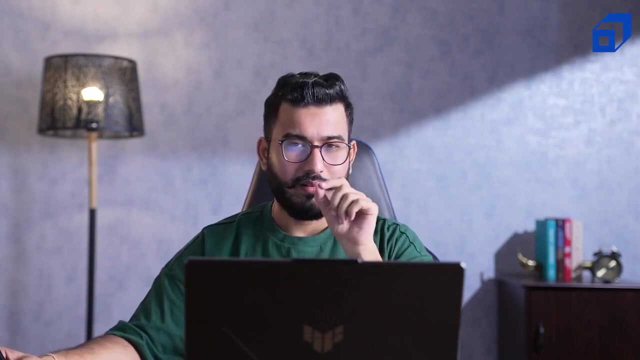 are equally likely. so all the outcomes, all the outcomes in this sample space, are equally likely. what is the meaning of equally likely? so if you already know about it, you can just pause the video and comment on this particular video. but equally likely basically mean that if I choose, 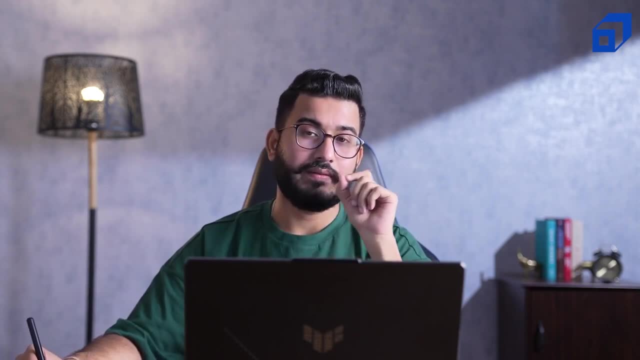 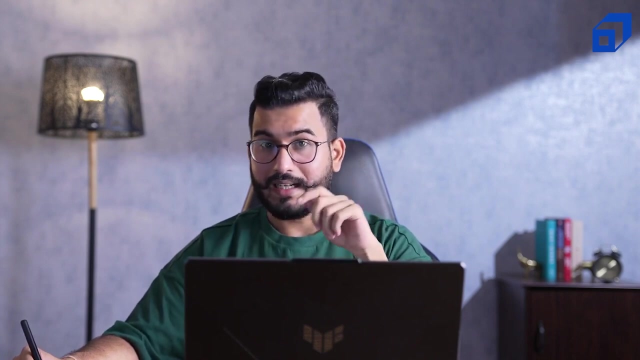 any of the event, it will have the equal chance of occurrence. for example, what is the probability that I will get the number one if I roll a die? it is simply 1 divided by 6. what is the probability that I'll get 2 again, 1 divided by 6- 3. 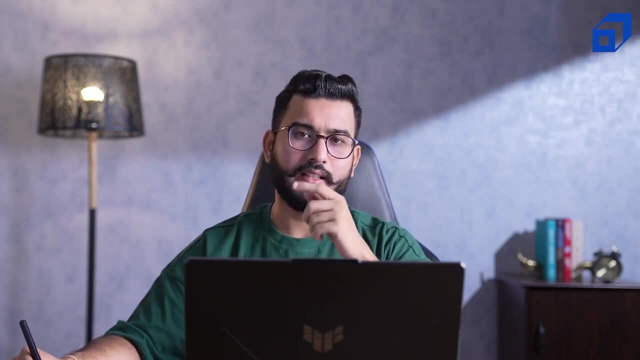 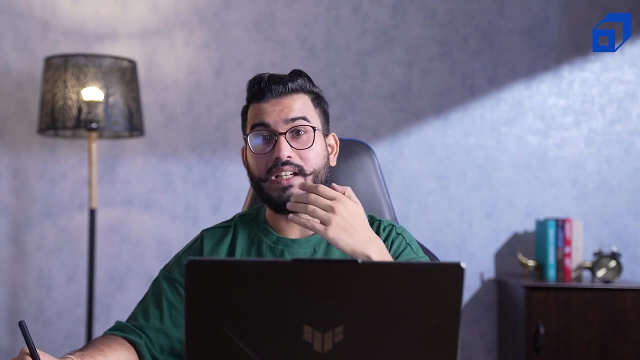 1 divided by 6, for 1 divided by 6, 5. 1 divided by 6, 6- 1 divided by 6. so all the events in this particular sample space are equally likely because each of them are having the probability equal to 1 by 6. 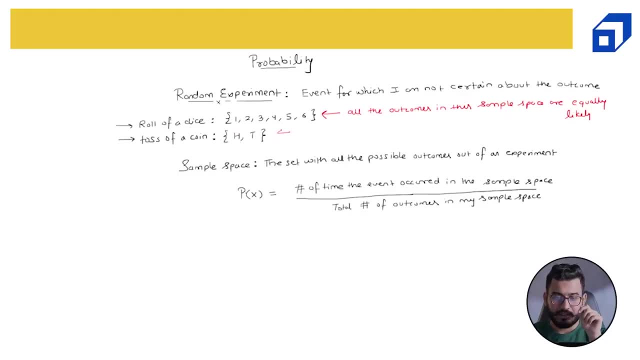 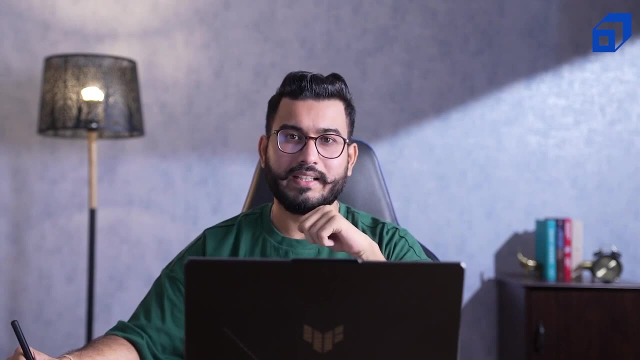 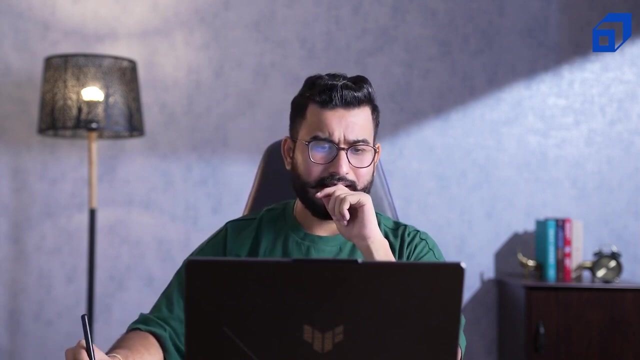 similarly, if I take this sample space- the sample is space is also equally likely. so what is the probability of getting head, 1 by 2? what is the probability of getting tail, again 1 by 2? so the probability of getting head and tail are equally likely. but now let's take example where I am tossing two. 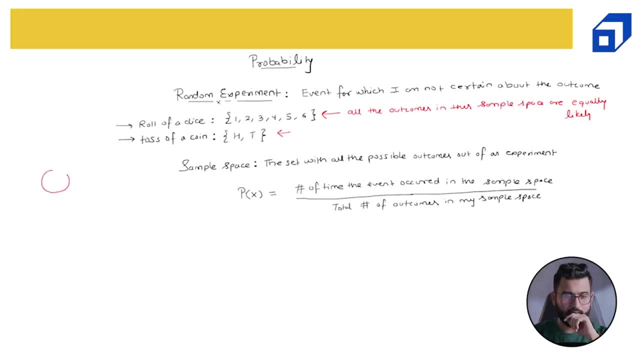 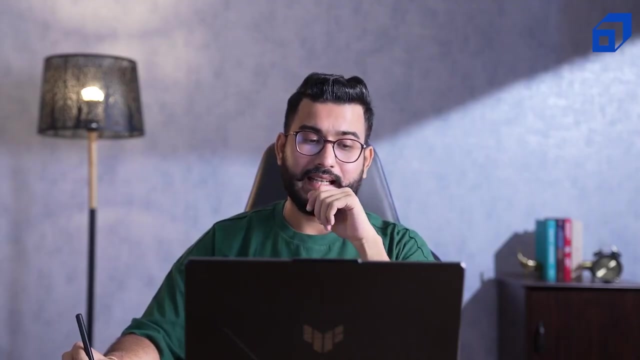 coins. so I am having two coins. my drawing is really good, so I'll use my skill over here. so let's say these are my two coins. now, what are the possible outcomes? I might get a head head, a head tail, a tail head or a tail tail. right now, what is the probability that I'll? 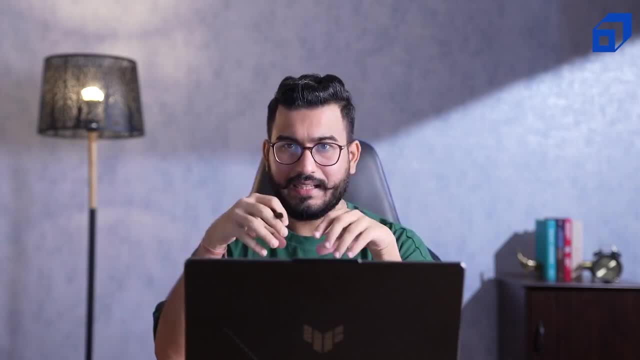 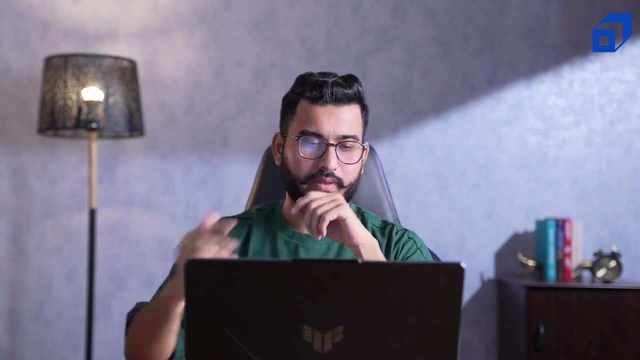 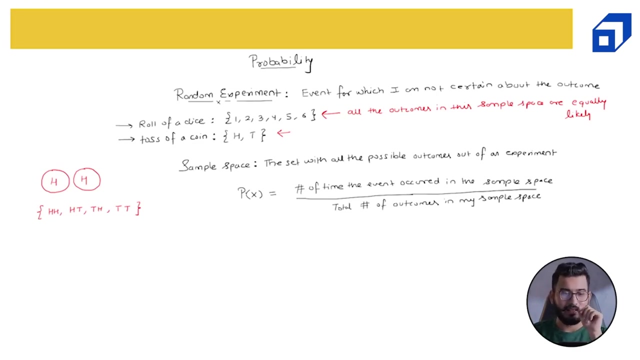 get a head and a head like both coins land into a both coins land with the face head and head. this is 1 divided by 4, because here I'm having total four outcomes and the probability of getting headed is is only one event is there, so the probability of getting headed is 1 by 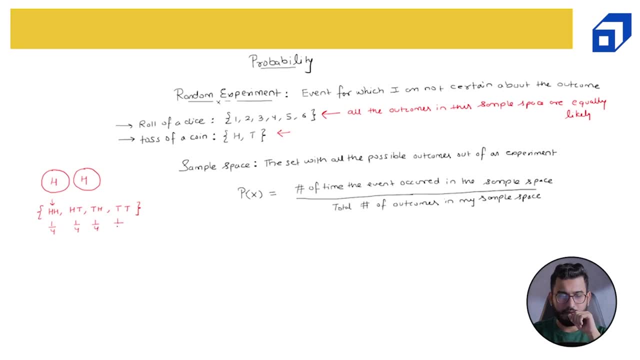 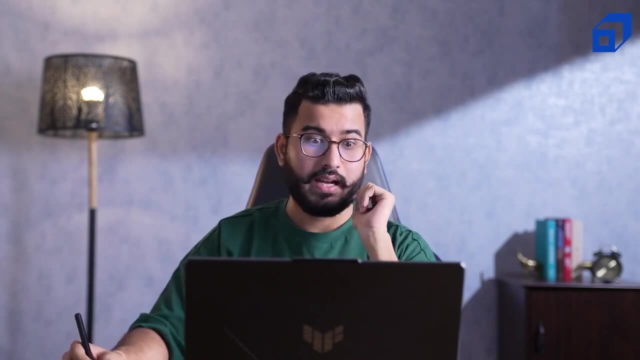 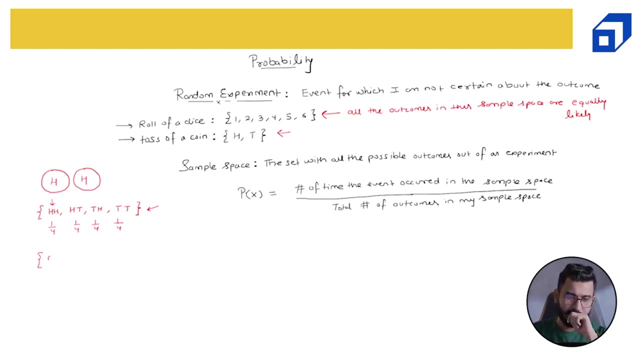 4. this is 1 by 4. this is 1 by 4, this is 1 by 4. so this sample space is also equally likely. can I write the sample space in another way? yes, we can. so let's say now: my sample spaces are the number of heads. so I can have zero heads and I. 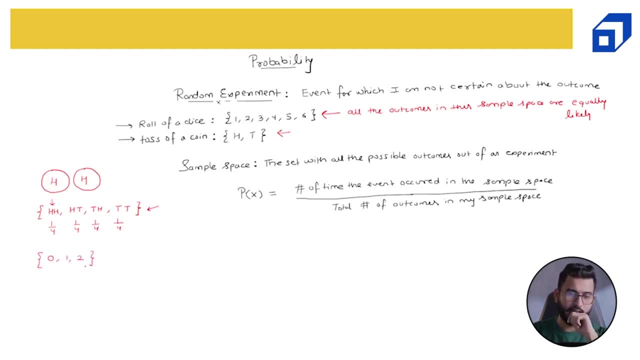 can keep just one and 2 heads. yes, so now I can write total: one heads and two heads. one head or two head. this is also a sample space, but there is a difference. this sample space is not equally likely. this sample space is not equally likely, so the probability of getting zero head is. one by four. and please remember, here each number represents one or two heads. so 4 is 1 & 4 is even. 4 is equal to 0. head of 0 is equal to 0. head of 1. head 1 & 4 is equal to 0. head of 1 & 4 is equal to 1 & 4 is equal to 0. head of 1 & scrub his name. seven half sunt導. 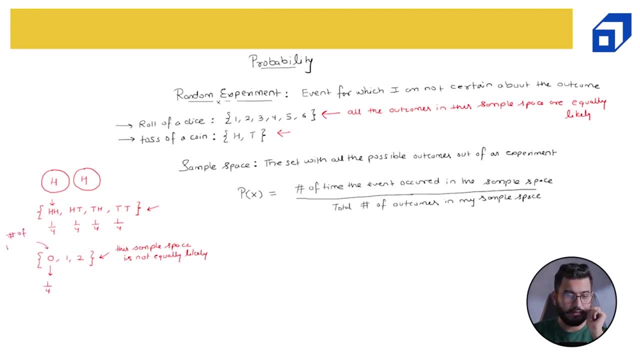 represents the number of heads. so the probability of getting zero head is 1 by 4. probability of getting one head is this plus this, so it can be either head, tail or tail head. so 1 by 4 plus 1 by 4 it is 1 by 2, and probability of getting two head is again 1 by 4. so here you can see that the 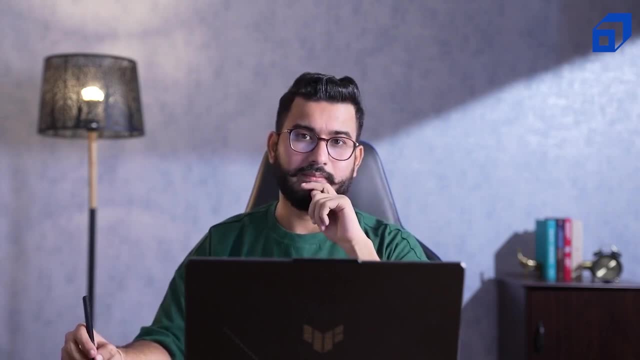 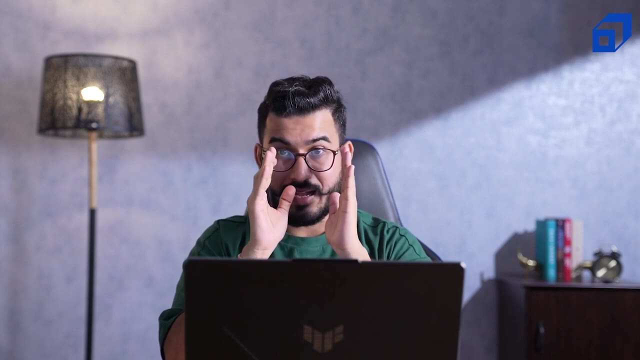 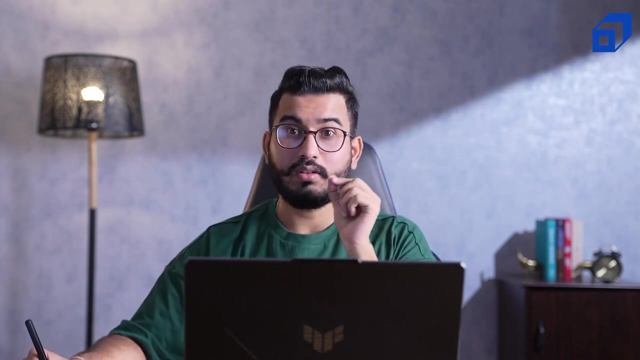 probability of each event is not equally likely. so whenever you are calculating probability, you have to make sure that your sample is sorry. your sample space should be equally likely. if it is not, then you have to carefully calculate your probability. I hope this is making sense. so now let's talk about some of the rules of probability. so I hope every one of you are. 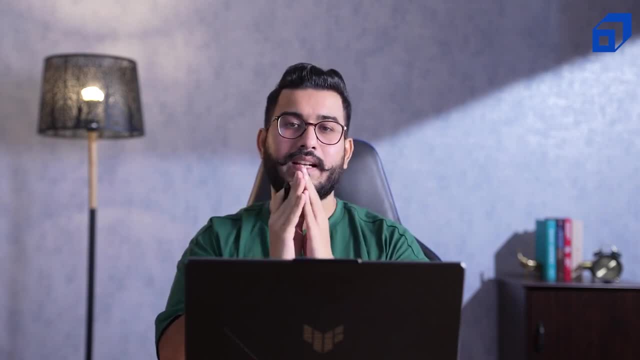 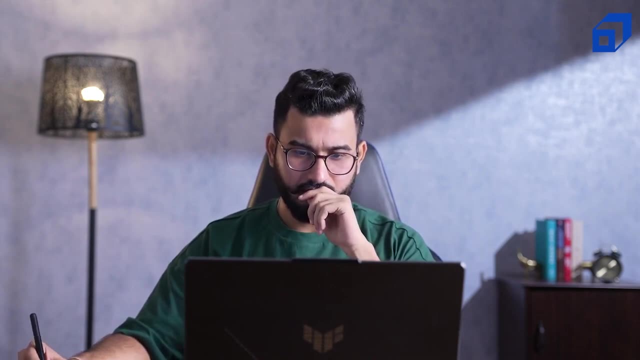 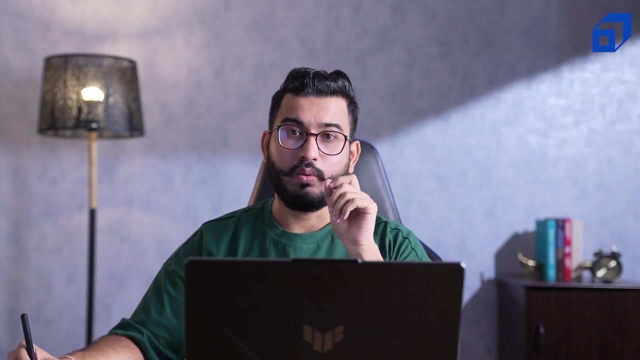 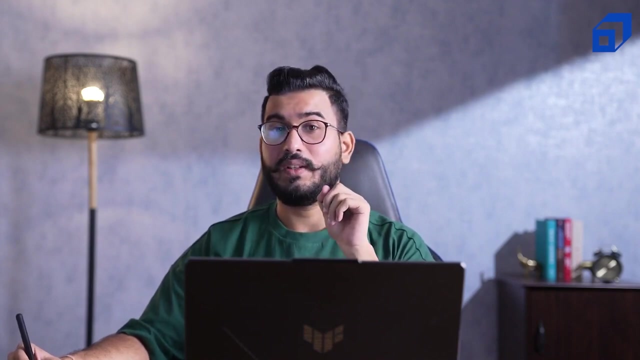 clear with the idea of Random experiment and the sample space. there is one particular term which is known as event. Now, what is an event? Any possible outcome or group of outcome out of an random Experiment or out of a sample space is known as an event. for example, if my experiment is: 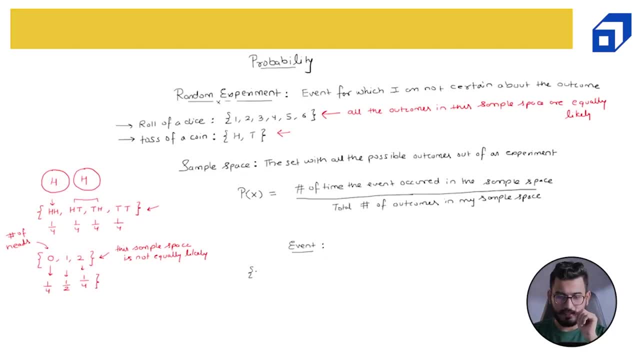 Toss of a coin, then I may get a head or a tail. So, out of this experiment, getting a head is an event, getting a tail is an event. Similarly, if I am tossing two coins, I may get head, head, head, tail, tail, head and tail tail in this case. 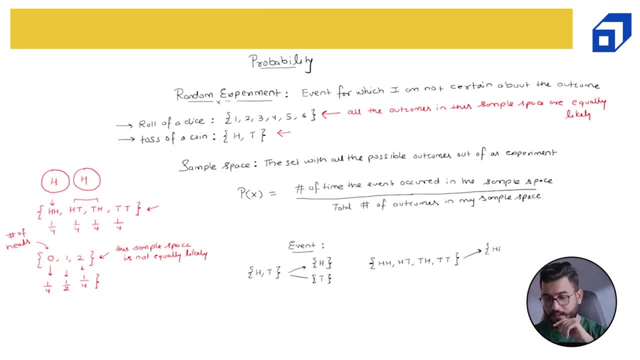 Getting two heads is an event, Getting one head is an event. Getting no head is an event. so all of these are my events. so event is nothing but a particular outcome or group of outcomes out of a sample space. so outcome or Group of outcomes or group of outcomes. 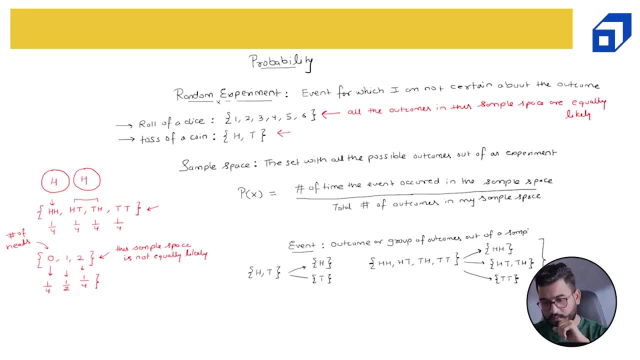 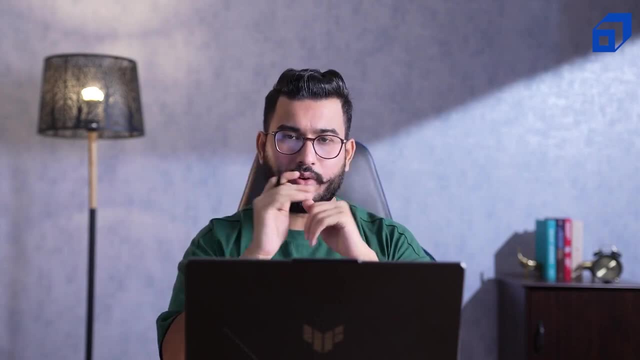 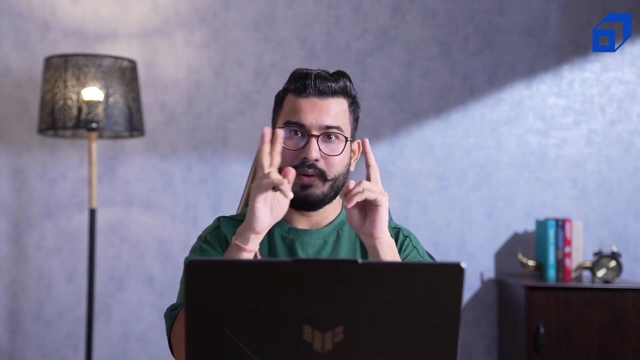 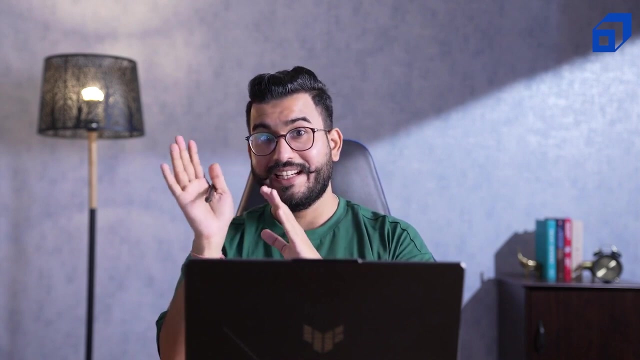 out of a Sample space. This is my Event. so how, what? what all we have talked about? number one: random experiment. number two is Sample space and the two ways in which we can write the sample space. one is equally likely sample space, Other one is not equally likely. the third topic: 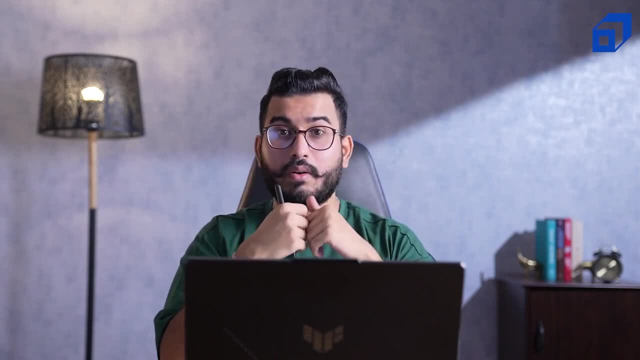 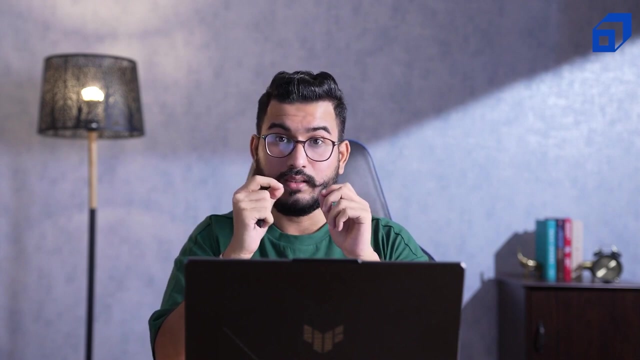 Which we talked about was event now. Now let's talk about the rules of probability. So when you are using probability as a measure or as a tool to basically calculate the possibility of probability of a particular event, there are some rules which we have to keep in mind. 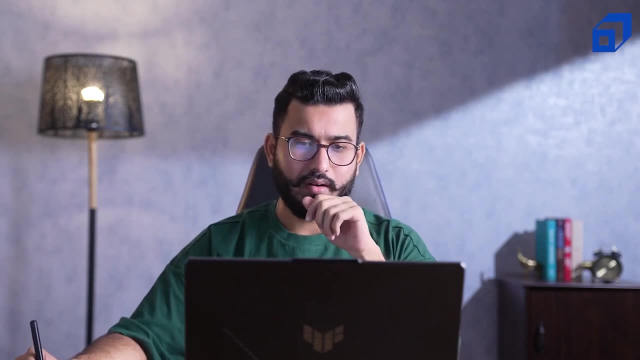 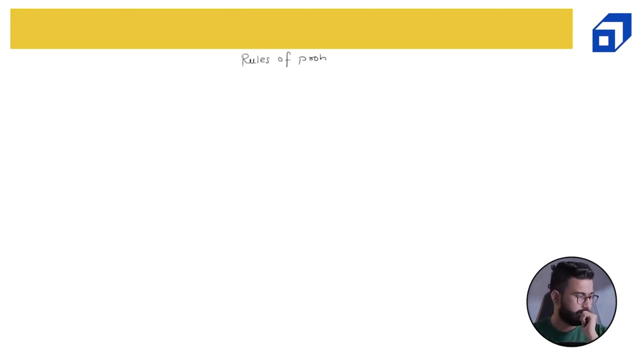 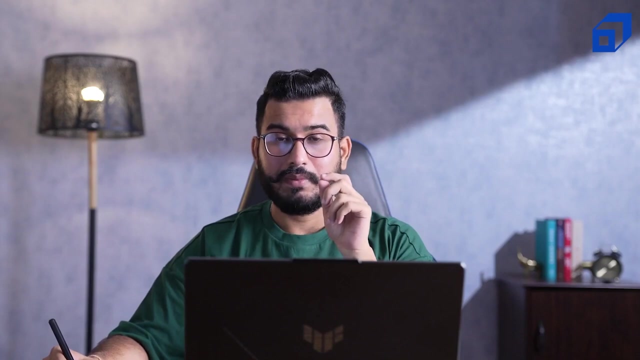 So let's talk about them. They are also known as the exams of probability. I'll just simply write it as rules of probability. So, rules of probability. The very first rule is: given a sample space, the probability of each outcome will always result to one. 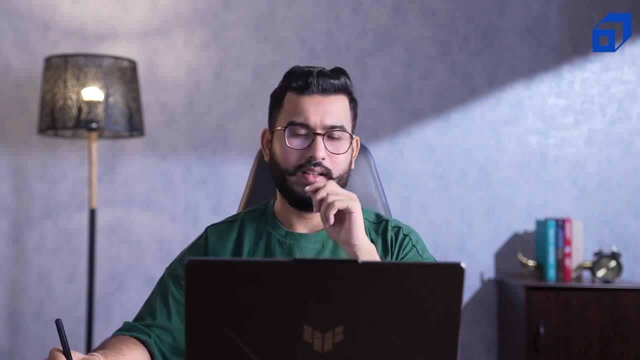 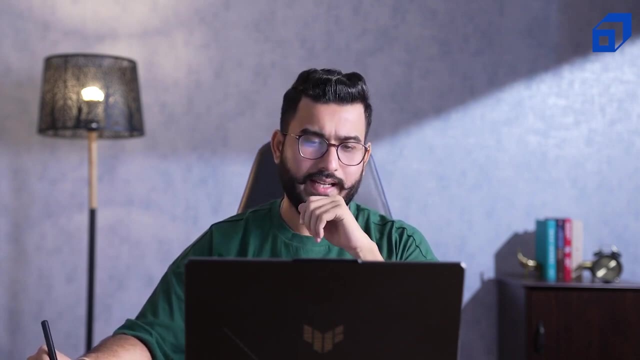 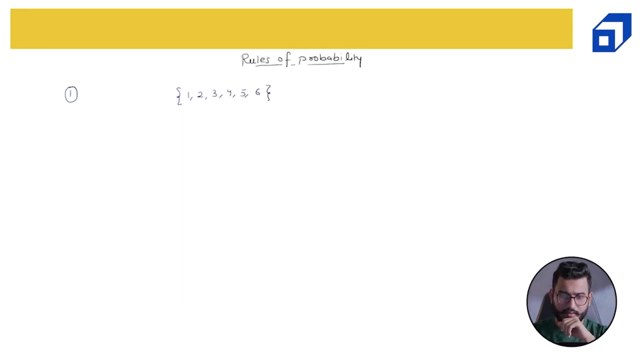 The total probability is always equal to one. Let's try to understand it. Let's say I'm given with a sample, a sample space of roll of a dice. So when I roll a dice I may get one, two, three, four, five or a six. 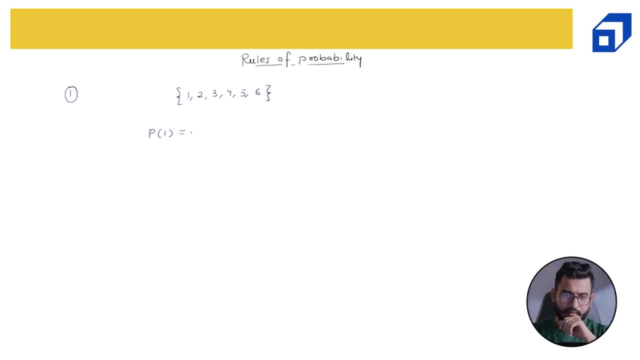 We know that the probability of one is one by six. So what is the probability of getting one in the dice? is one by six. What is the probability of getting two? It's again one by six. Probability of three: again one by six. 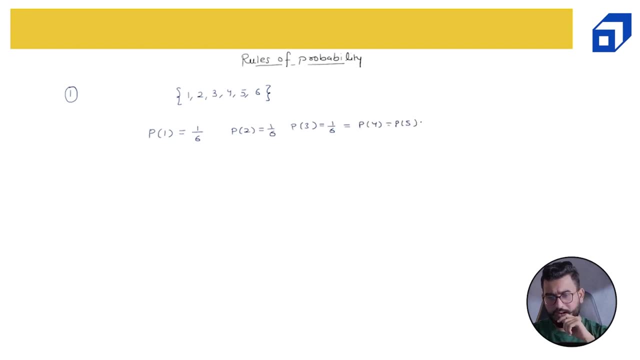 And this is equal to probability of four, probability of five and probability of six. All is one by six. Now, if I take the sum, probability of one plus two, plus three, plus four, plus five plus six, If you do the quick math you will find out that it is equal to one. 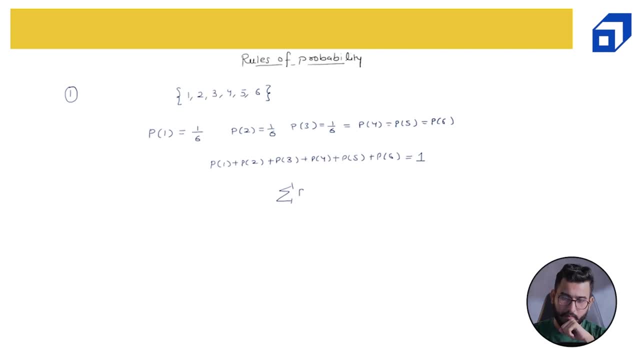 That is my first rule. So summation of pi, where i is running from one to n Or Pi is over my sample space. So I'll just simply write where i belongs: to my sample space. The sum of all the probabilities is always equal to one. 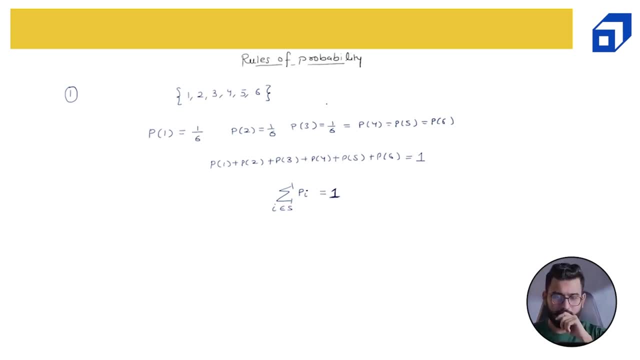 This is my first rule Let's talk about, So let me just formally write it down so that you guys are having all these notes And whenever you prepare for your interview. if you just read all the note, it will be very easy for you to. 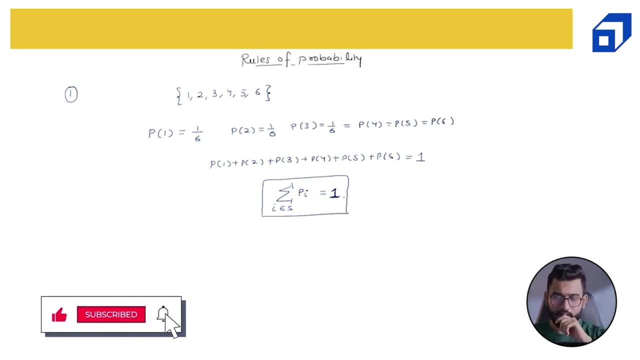 To pass your statistics around. So the sum of all probability over the sample space or the sample space is always equals to one. This is my first rule. Now let's understand the second rule, Which is known as the rule of sum or addition probability. 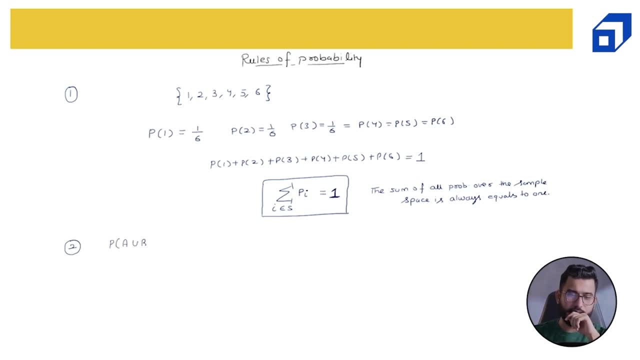 It says that the probability of A union B is equal to probability of A plus probability of B if A and B are disjoint event. So there is a condition if A and B are disjoint. Now, don't need to worry, I'll just write it down. 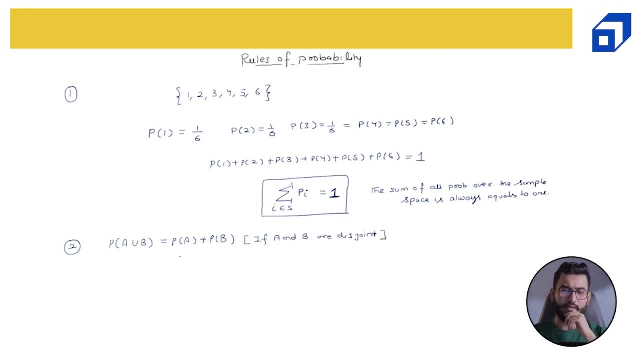 Don't worry, I'm not talking anything in German. This is very simple to understand. Let's take one simple example. Let's say I'm tossing two points. So when you toss two points, you might get two heads, two tail. one head, one tail and 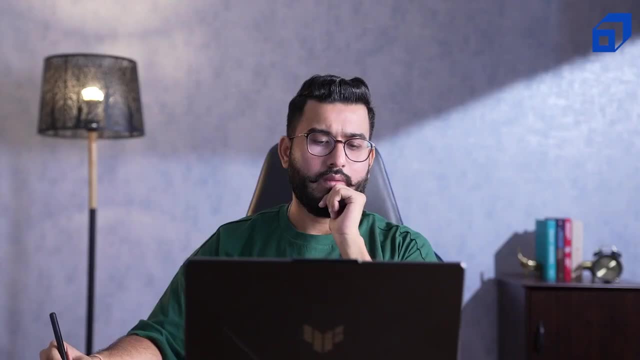 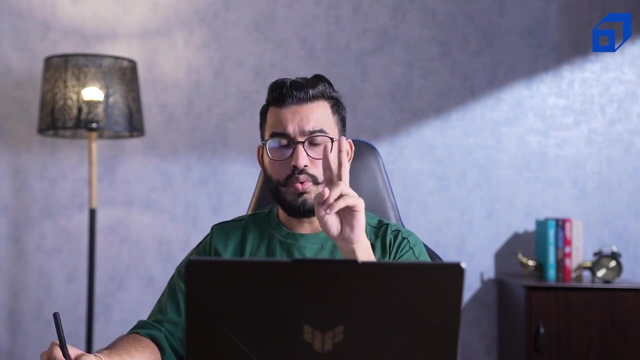 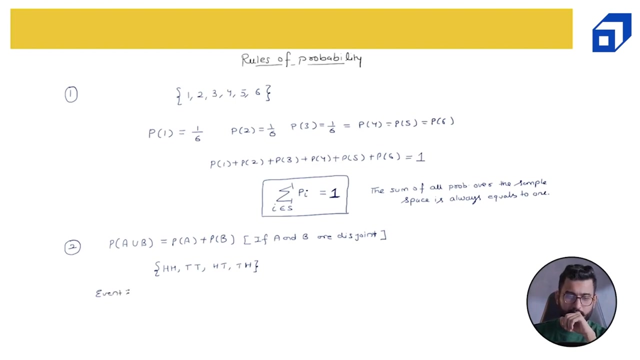 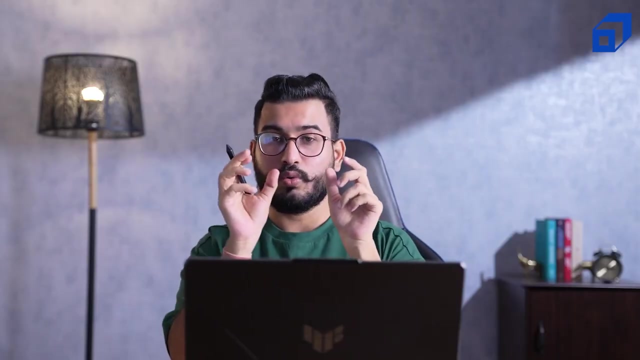 one tail, one head. Now, if I ask you what is the event of getting two head or so, let's take what is a. what is the event of getting two different outcomes? Let me write it down. What is the event Of getting both coins with different outcome, which basically mean both coins land into. 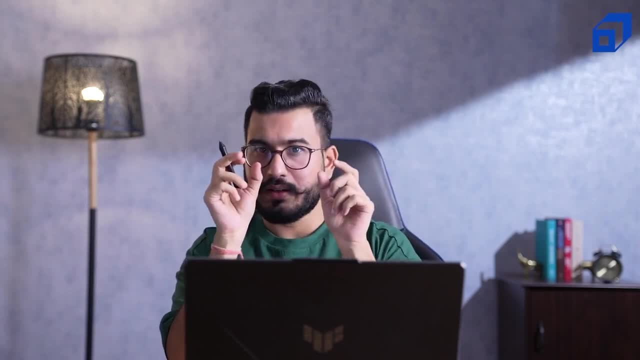 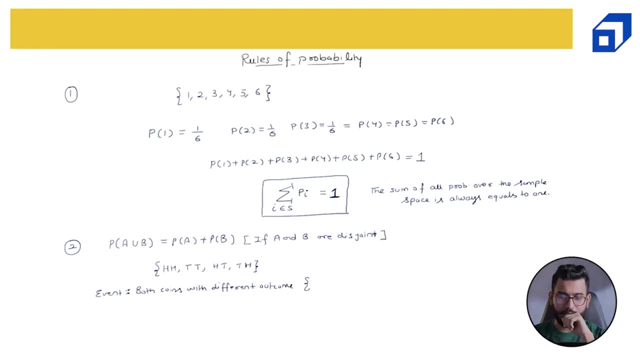 a different outcome. So one is head, So another one will be tail. If one is tail, another one will be head, And we already know that there are only two possibilities, So my event would be: head, tail or tail, head, Right. 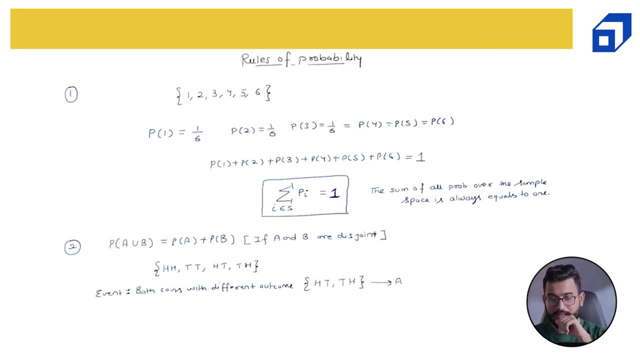 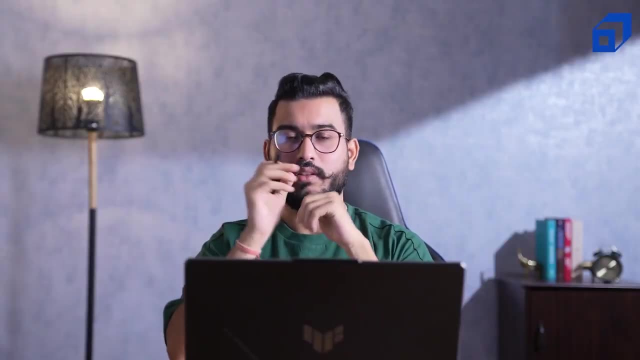 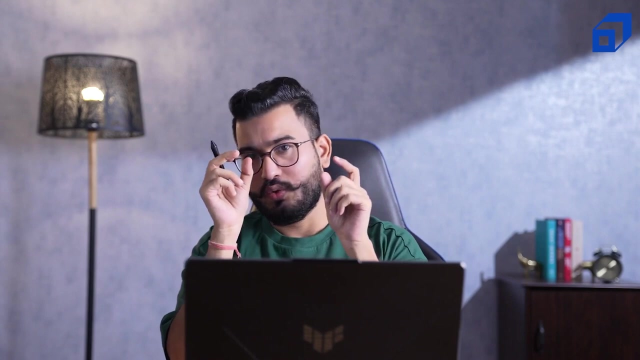 Let's call this as. let's call this event as event A. Now we have another event where both coins lands into same outcome, which basically means, if coin one is head, coin two is also head. If coin one is tail, coin two is also tail. 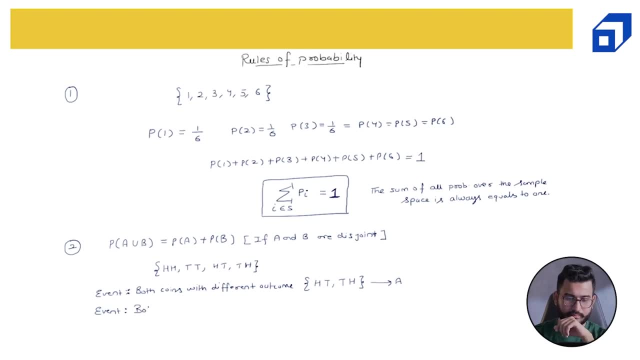 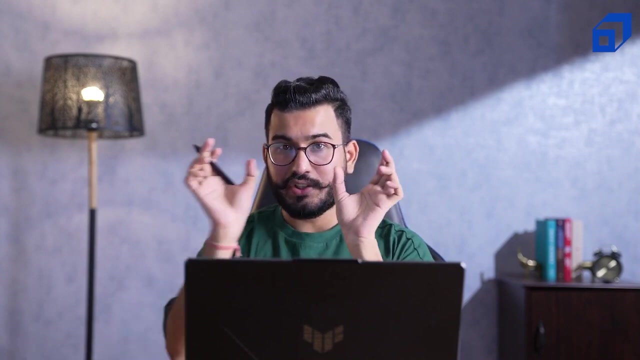 So this is same outcome. So both coins, both coins with same outcome. Okay, And that would be head, head, tail, tail. And this is my event B. Now, if I take the union, union means addition. If I take the addition of these two set, then according to the rule, it is the sum of individual. 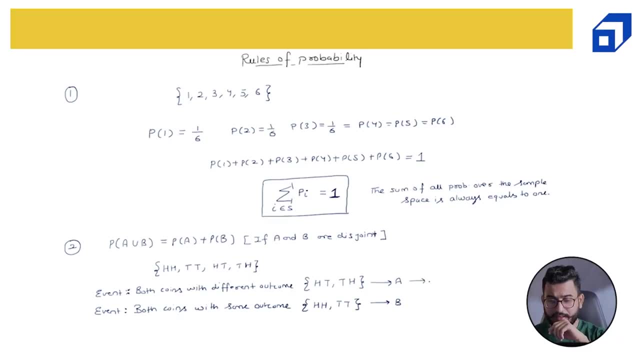 probability of the event. So what is the probability of event A? If you guys have understood, you can simply answer this And you can add your answers in the comment section. So the probability of A is there are two outcomes with which matches my condition. 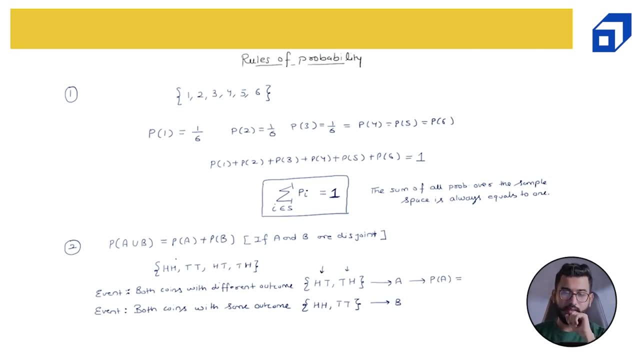 So head, tail and tail head. there are total of four outcomes in my sample space. So the probability is one, sorry two divided by four, which is simply one divided by two. Similarly, probability of B is also two divided by four, which is one divided by two. 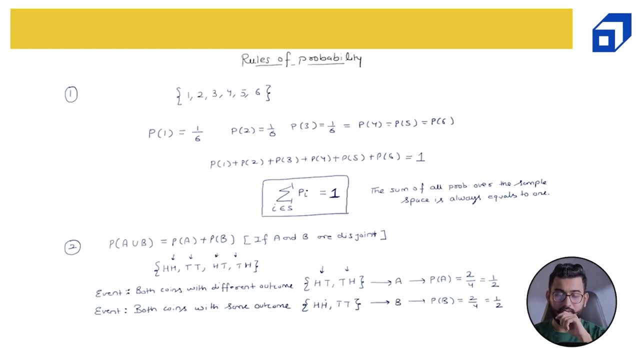 Now if I take the sum or if I take the union of these two events. so what is the union of A union B? A union B means I will combine all the events in my sample space. Now, since we do not have any common element, my union would simply be head, tail, tail. 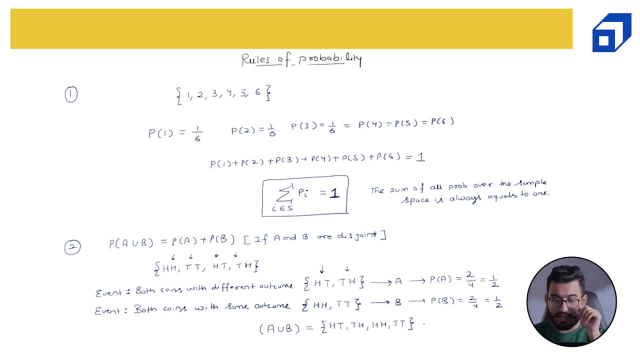 head, head, head and tail tail. And if I ask you what is the probability of A union B, You will just simply say it is Four divided by four, which is one. Now if I add these two probability- probability of A plus probability of B- you can simply: 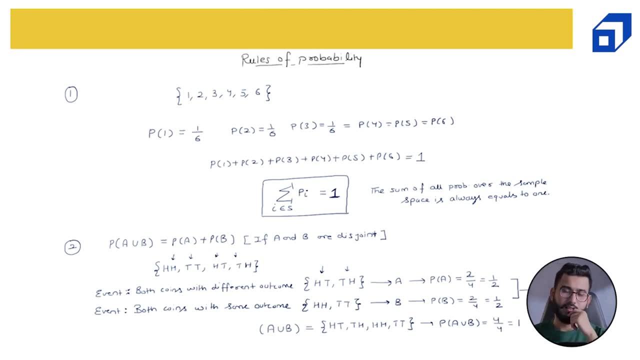 add one by two plus one by two. This is also one right. So that basically mean, if two events are disjoint. So here you can see, event A and event B are disjoint. Why am I calling them as disjoint? Because they do not have any common event. 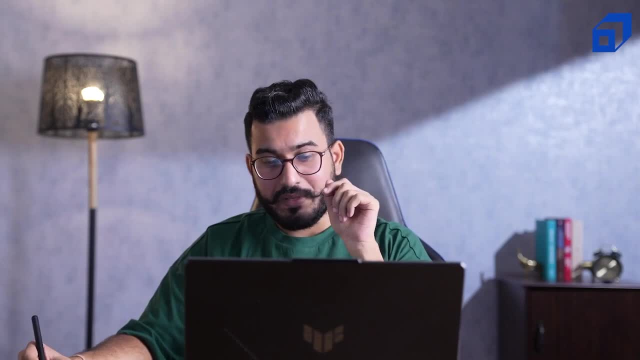 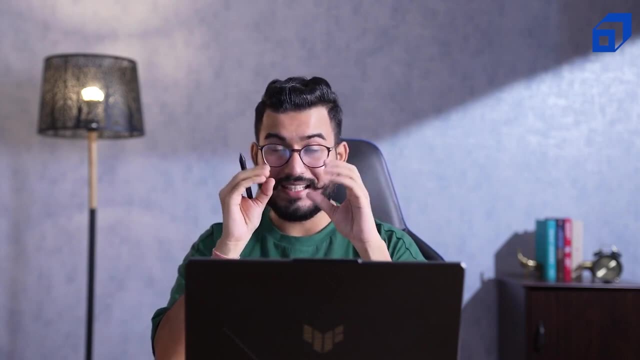 You can see that in event A I'm having head tail, In event B I'm having head, head, tail, tail. There is no common event. So when two events- A and B- are disjoint, they do not have any common event. then the probability 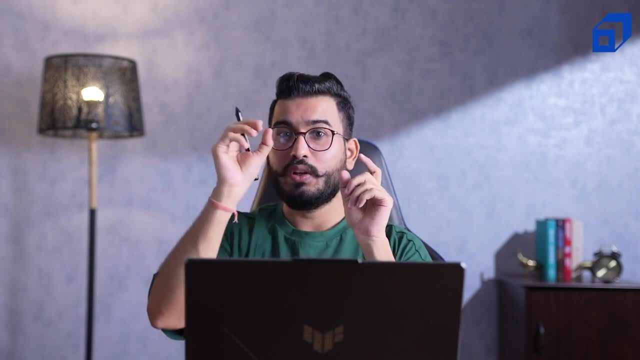 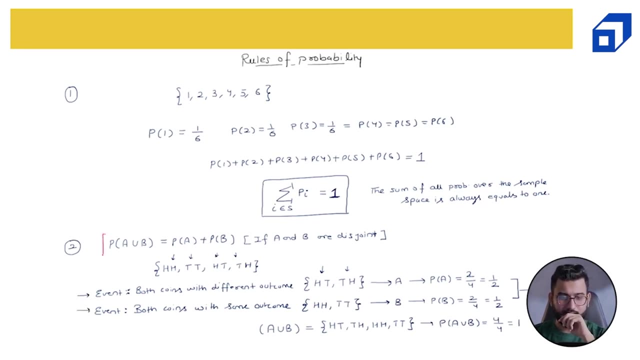 of the union is always equal to the individual sum of probability, And this is what we were trying to prove. So let me just quickly highlight this, And this is my second rule of probability. This was my first rule, This is my second rule. 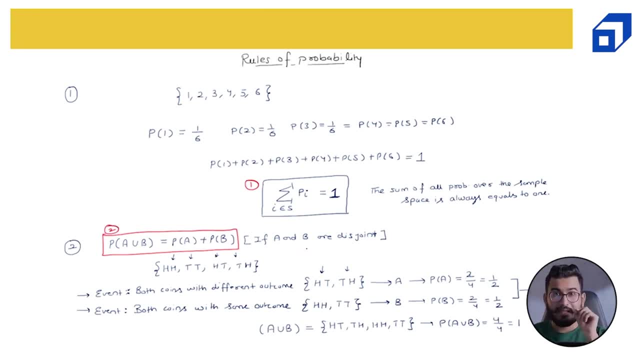 And this rule is only applicable when your two events are disjoint. where we have taken this example, A and B are disjoint because it is. it does not. it does not have any common event. It is a common event among them. Now let's understand the third rule, and third rule is also very much closely associated with 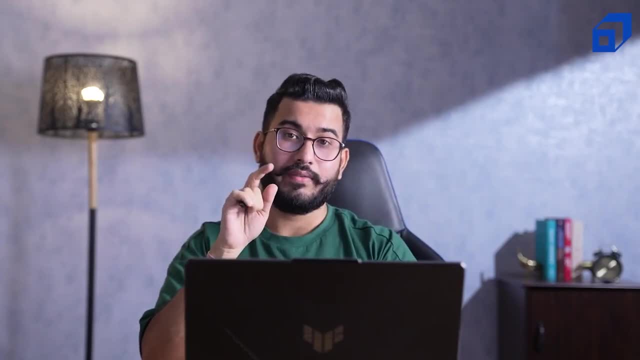 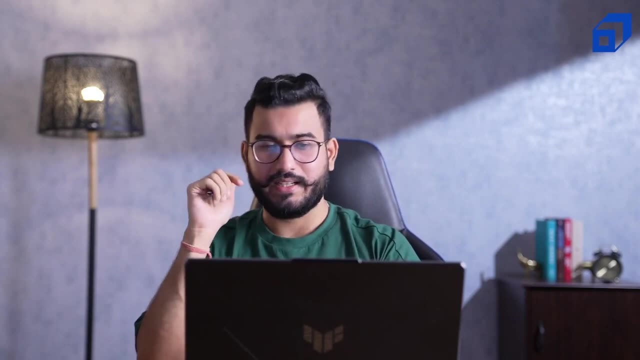 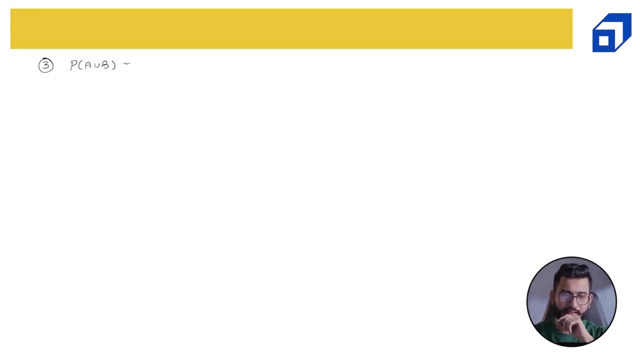 the second rule where we proved that probability of A union B is always equal to the probability of A plus probability of B if A and B are disjoint. Right Now there is one more rule: If they're not disjoint, Then A union B is probability of A plus probability of B minus probability of A intersection B. 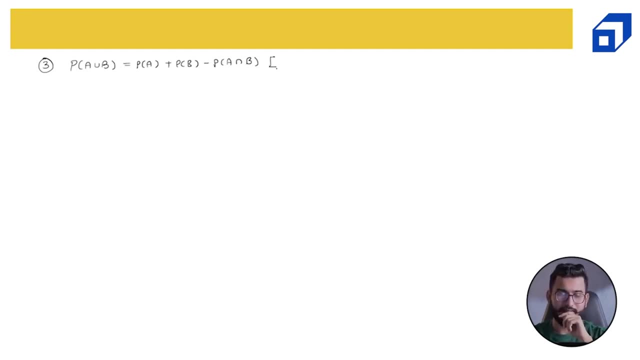 Again, you guys would be thinking that it is something German, but not. Let's try to understand it. In order to understand it in a better way, we will take the example of playing cards. playing cards, And I hope most of you would be aware about the playing cards. 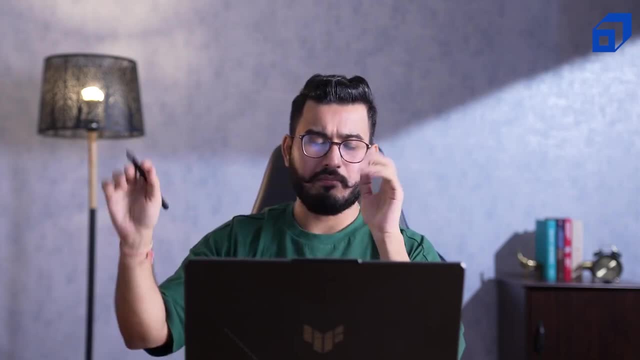 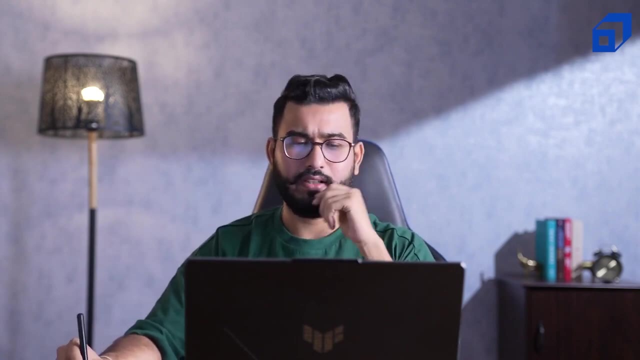 but if you are not, no need to worry, Let's try to write down the complete details about how many playing cards we have, what are the various suits and everything. So in total, a playing card or a deck of playing cards comes with 52 cards. 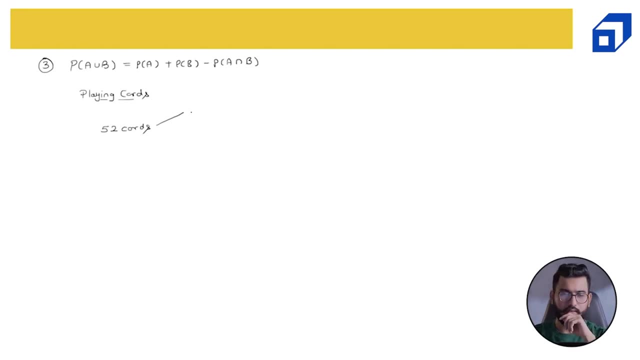 With four suits. So we have club, spade, heart and diamond. Now, if you guys are aware about it, then you can easily point it out that club and spade these are two black cards, while heart and diamond these are my red cards. 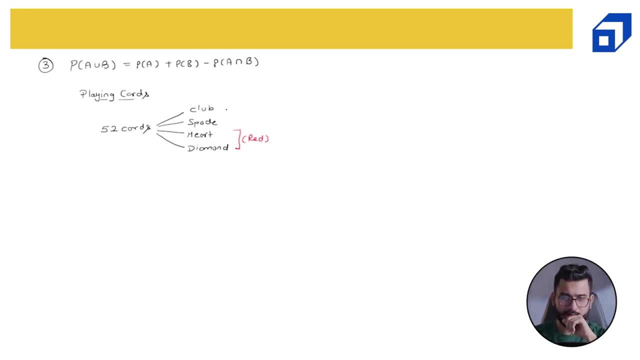 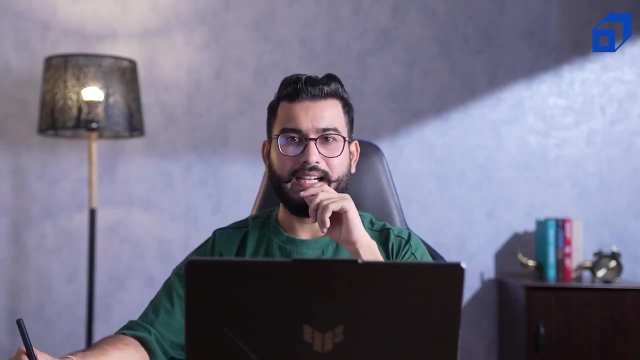 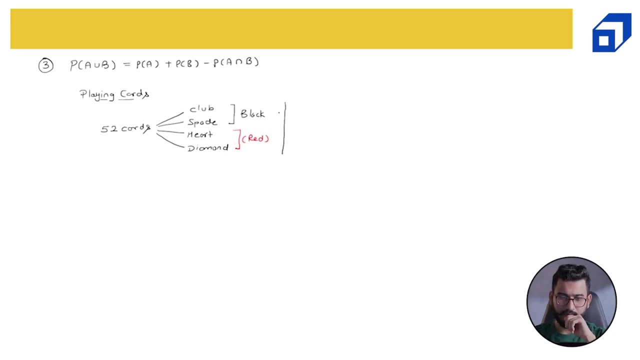 So club and spade are my black cards. Now club is having 13 cards, spade is having 13,, heart 13, and diamond 13.. So each of them is having 13,, 13 cards. Now, which all 13?? So let's write down the complete structure. 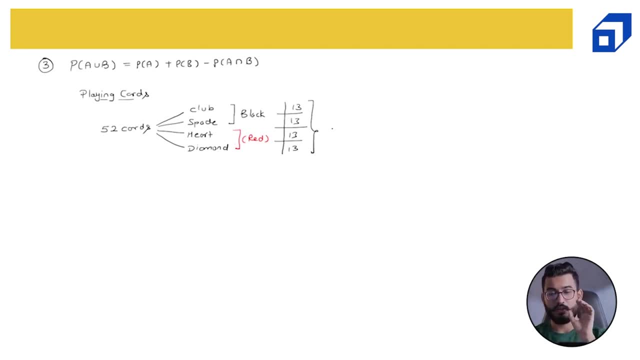 So each suit comes with a total of 13 cards, which starts with ace, a card of ace, then two, three, four, five, six, seven, eight, nine, 10, and then three cards which are known as the jack, queen and king. 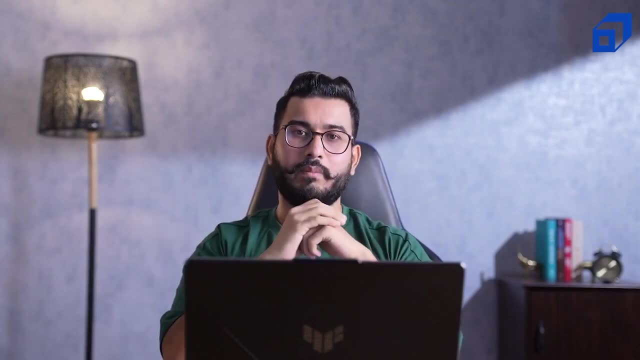 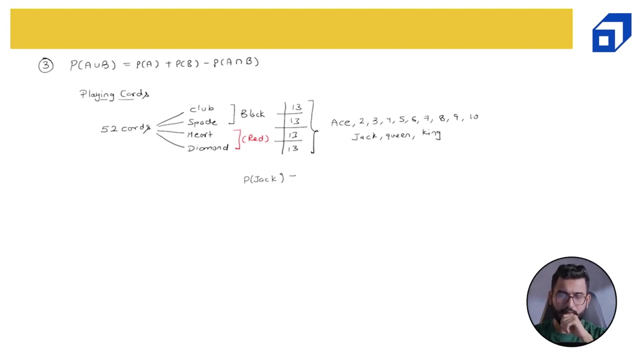 Now this is the complete portfolio of your playing cards, or the deck of playing cards. Now let's try to calculate some probability of some events. So what is the probability of getting a jack? What is the probability of getting a card which is a jack card? Now we already know. 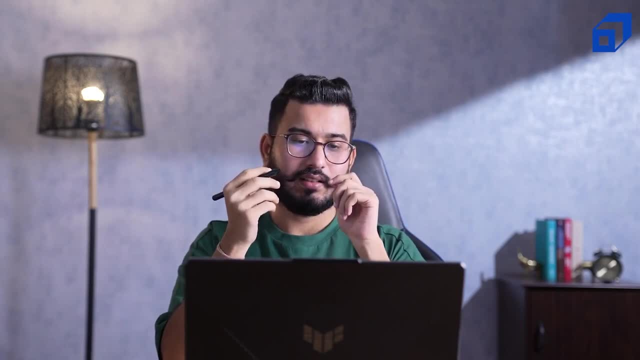 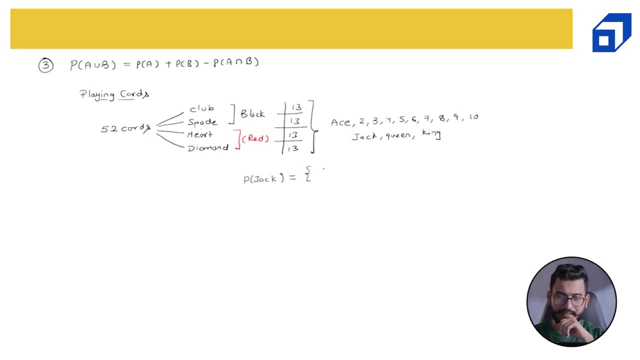 that a jack or card of a jack can come from any of the suit. So I may have a jack from club. so I'll write cj, club of jack or jack of club. you can say anything. Then we have a spade. 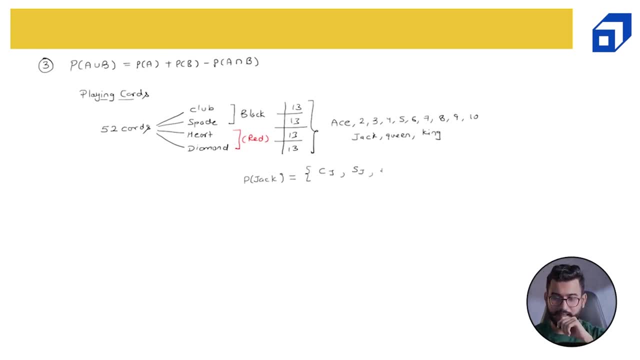 I can get a jack from a spade, I can get a jack from heart. I can get a jack from diamond. right, These are the total four outcomes, or total four favorable outcomes, while the total number of outcomes or total number of events in my sample space is 52, because each card is a outcome. 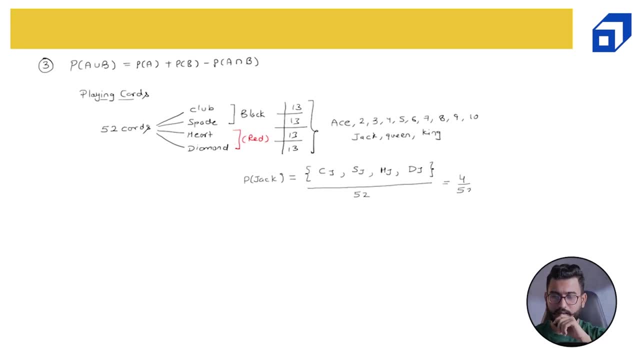 right. So the probability of getting a jack is four divided by 52. Right. What is the probability of getting a black card? now? we already know that club and spade. or let's simplify the question so that I can demonstrate you the rule that we were. 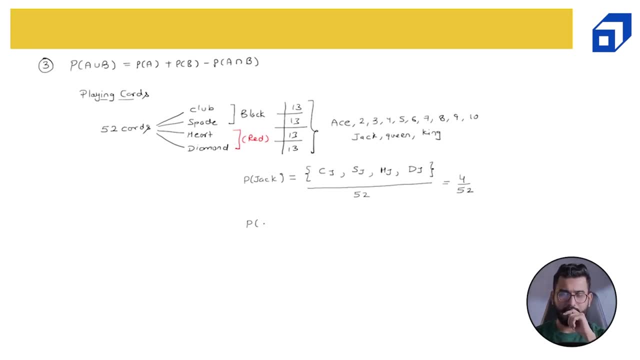 trying to prove. so what is the probability of getting a heart? now we know that there are total of 13 hearts. total of 13 hearts because heart it itself is a suit. so we have 13 cards belong to heart and total are 52. so the 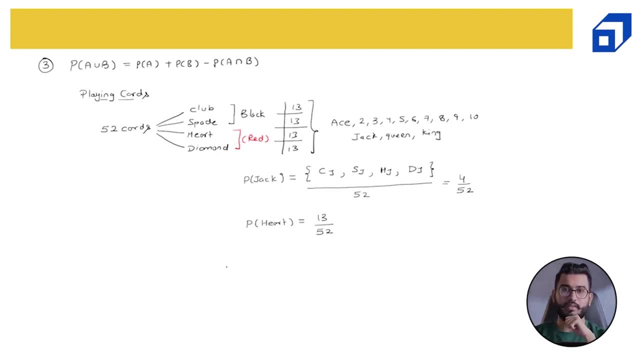 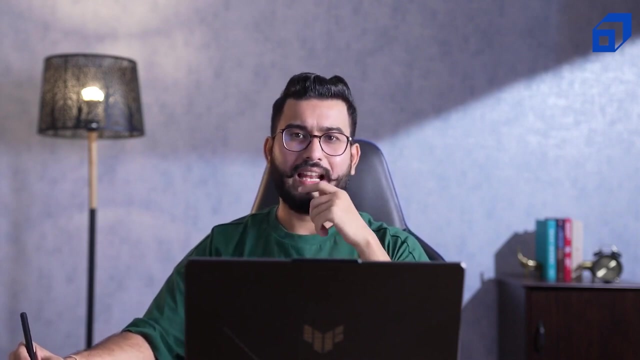 probability of getting heart is 13 divided by 52. what is the probability of getting Jack and heart? now, before we jump to the answer- I know you, most of you- would have already calculated the answers. let's try to note down all the outcomes. which matches this question. 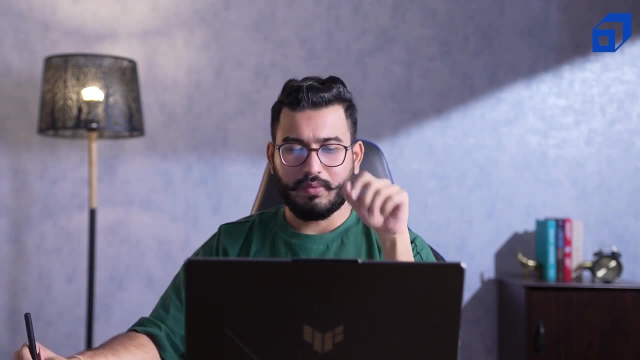 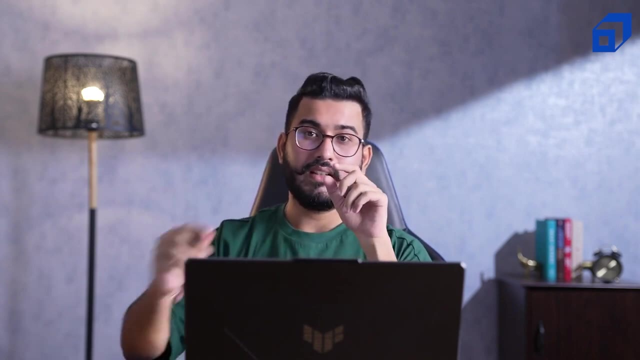 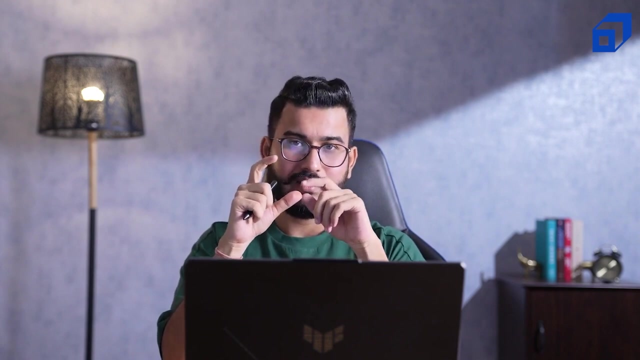 condition, and then it will be easy for us to understand if we are going to in the right direction or not. Jack and heart, which basically means the card need to be a Jack card and the card should be a heart. now, if you closely try to understand this problem, you will find out that it is only one card that can. 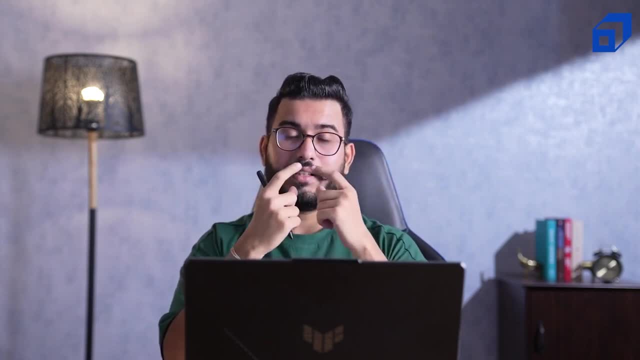 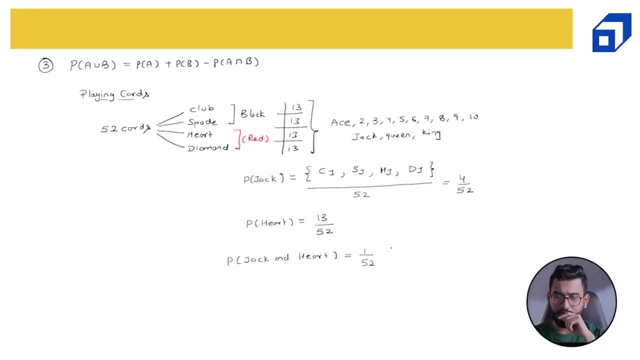 be a card which is Jack plus it also, it also belongs to a heart. so the probability is 1 divided by 52, because I will have only one card which is heart of Jack or Jack of heart. now what is the probability of Jack or heart now all? 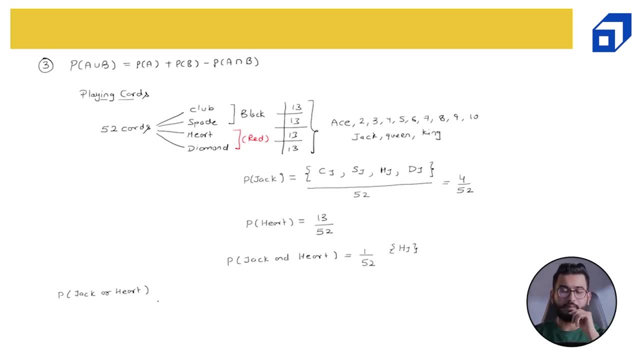 means nothing but the addition. before we calculate this probability of Jack, or a Jack or a heart, what is the probability of Jack or a heart? now, all means, nothing but the addition. before we calculate this, Let's write down all the outcomes, or all the events. So it will be: heart of Ace, heart of one, heart of two. 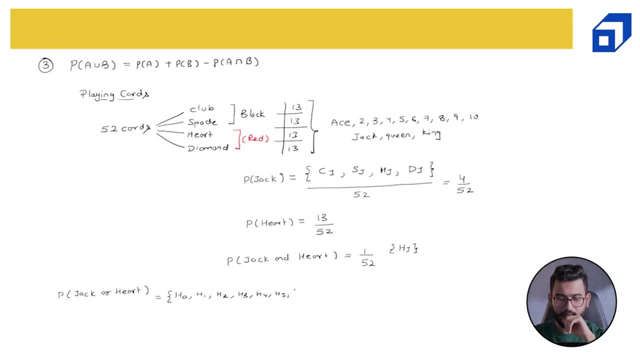 heart of three, four, five, six, seven, eight, nine, Ten, then heart of Jack, heart of Queen and Heart of King. These are all. my heart There's all. these are all the cards that belong to the suit heart. Now let's write down all the jack cards so I can have a jack. 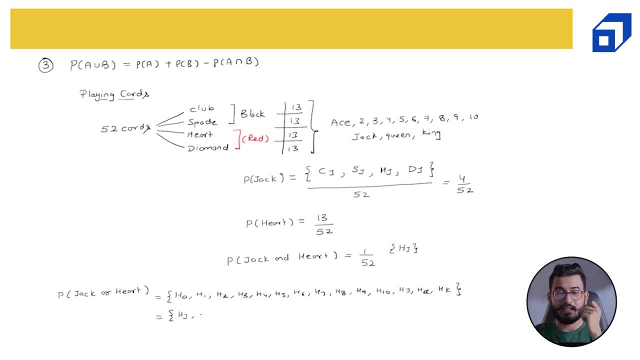 From heart, so HJ. I can have a jack from club, So CJ. I can have a jack from speed, so SJ and then DJ. Now if I combine them, if I take the union of them, So let's call this as event, be this event A if I take A union B. A union B means I have to create a set which is having the all the. 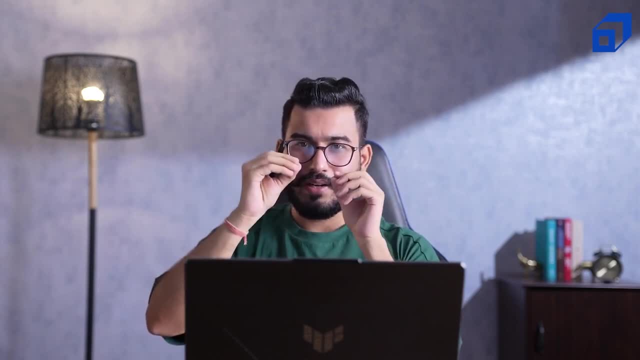 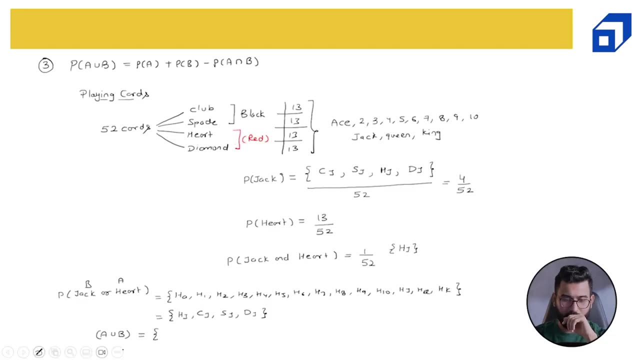 events from A and all the events from B, But if there is an event which is replicating for two times, I have to only pick one of them right. So if I combine them, you will find out that there is one event which is common in these two set, and this is this card. Let me just quickly circle it. 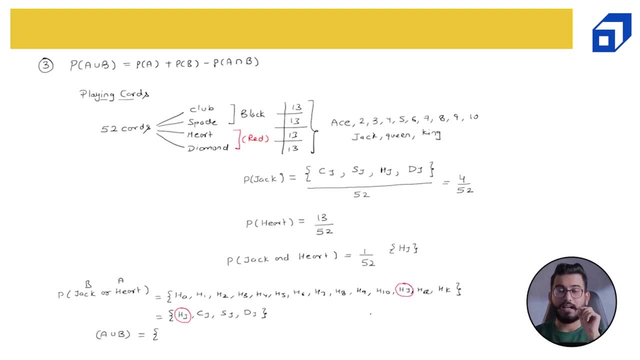 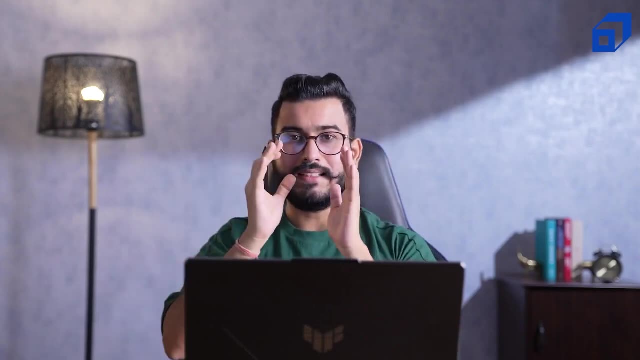 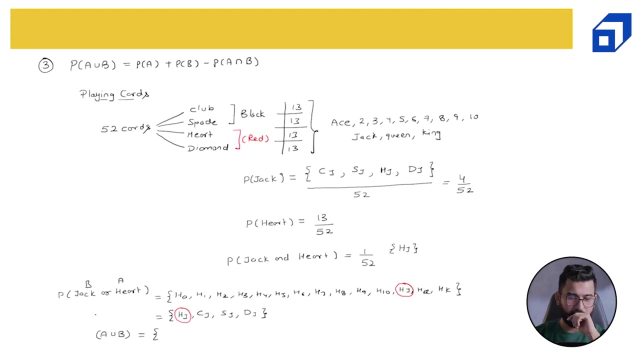 So, heart of Jack, this card is available in both the set right, And if I have to combine these two set, I have to count this particular card only for one time. So if I write down all the combined event, it will be from heart of Ace, heart of one, heart of two, heart of three, four, five. six, seven, eight, nine, 10,, 11,, 12,, 13,, 14,, 15,, 16,, 17,, 18,, 19,, 20,, 21,, 22,, 23,, 24,, 25,, 26,, 27,, 28,. 33,, 33,, 34,, 35,, 36,, 37,, 38,, 39,, 40,, 41,, 42,, 42,, 43,, 44,, 45,, 46,, 47,, 49,, 40,, 42,, 43,, 44,, 45,, 46,, 47,, 49,, 40,. 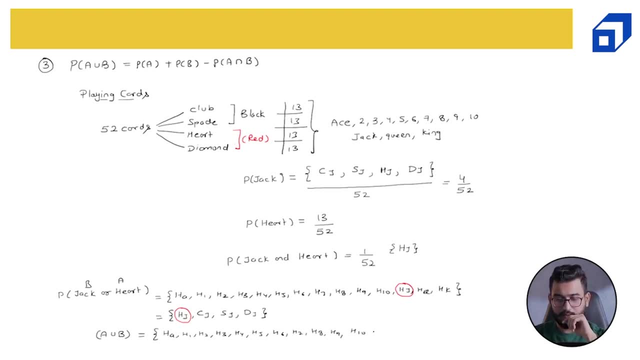 50,, 51,, 5,, 5,, 6,, 7,, 8,, 9,, 10.. Then heart of Jack- Now I have counted it already for one time- Then heart of Queen, heart of King, And then I will write down these three cards, which is C, J. 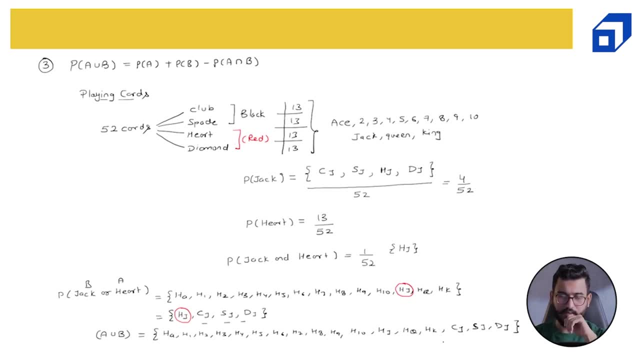 S J and D J, Now how many events I'm having in this. So one, two, three, four, five, six, seven, eight, nine, ten, eleven, twelve, thirteen, fifteen, sixteen, twenty, twenty. 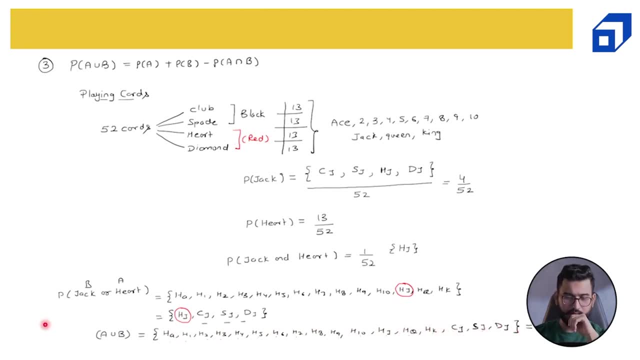 twelve, thirteen, sixteen, seventeen, nineteen, twelve, thirteen, twenty seventeen, twenty, twenty, forty, sixty, twenty ninety, twenty, fifty, ninety. one, two, three, 13, 14, 15, 16, 17. the mistake is this is not h1, this is h2. so after ace it starts from 2. 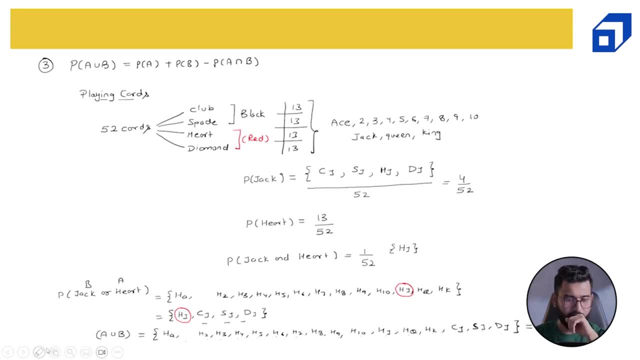 so I haven't read. I should not be writing this. in that case, my outcome will be 16 divided by 16, divided by 52. probability of Jack or heart is simply 16 divided by 52. now, if I go with the formula, what is the probability of getting hard? it is 1, 2, 3, 4, 5, 6, 7, 8, 9, 10, 11, 12, 13. so this is 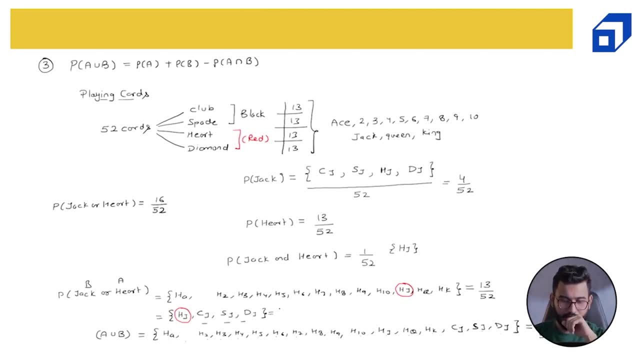 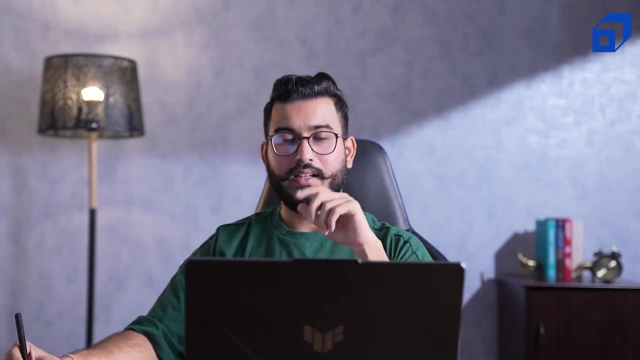 why 13 divided by 52, this is 4 divided by 52, right? if I add them without subtracting this common event, I will be basically counting this card for two time, which is wrong. right, if I have to add these two said, I have to make sure that I am. 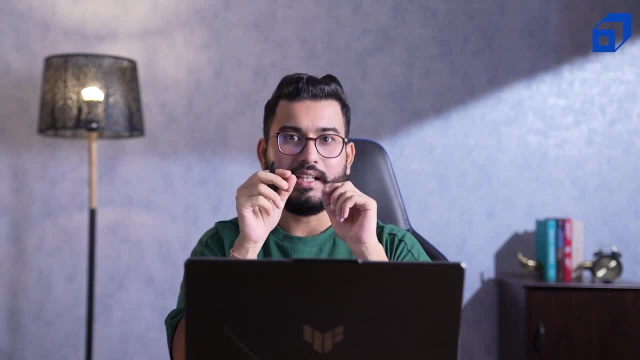 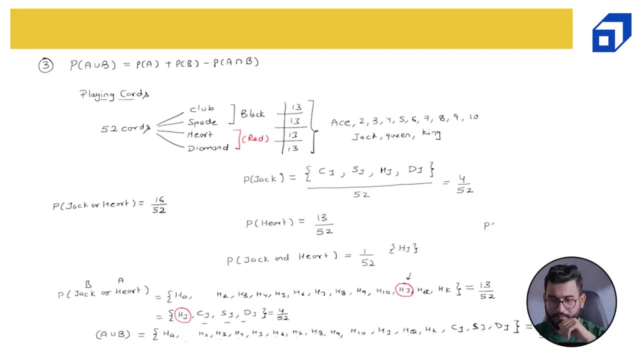 just counting this card for one time because logically I have only one card right. so that is the reason when I am combining them. I will write probability of a plus probability of B minus the common card or common event which occurs in these two set. so a and B. now, if a and B is 0, a and B can only be 0 when the two 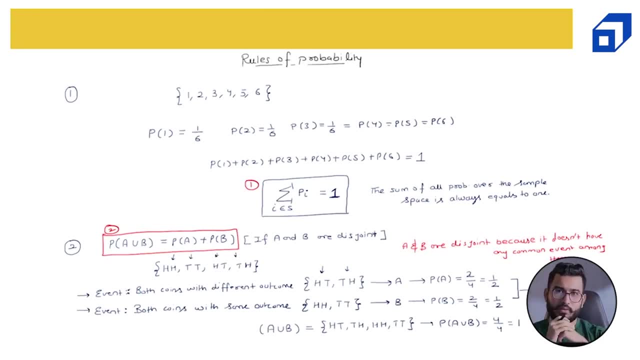 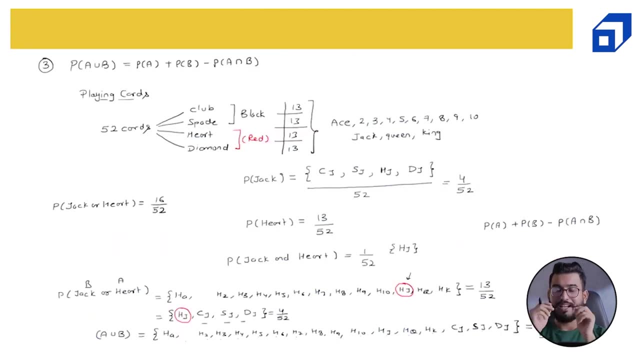 sets are disjoint. I will go back to my rule number two. so if a and B are disjoint, probability of a intersection B is 0. when a and B are joint basically mean they have a common event. then my probability of a or B pay a union B. 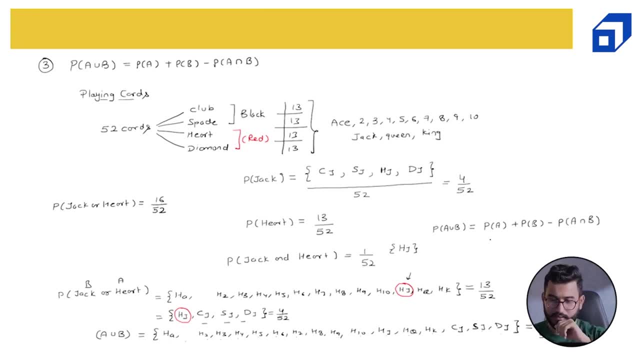 is equal to probability of a, which is 13 by 52 plus 4 by 52 minus 1 by 52, because I am having one card which is common and I have calculated it over here. so this will be total of 16, sorry, 17. 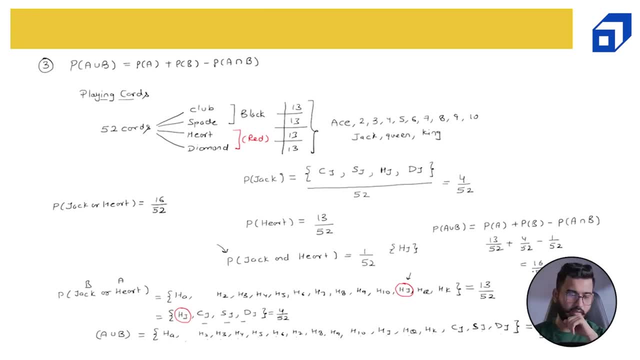 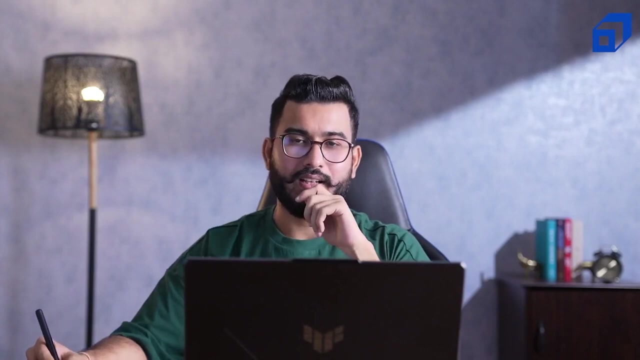 minus 1, which is 16 divided by 52, which is my third rule of probability. I hope everyone of you are clear with this. this is my third rule. now let's look at the one final rule, which says probability of a plus, probability of a complement, is always equal to one. 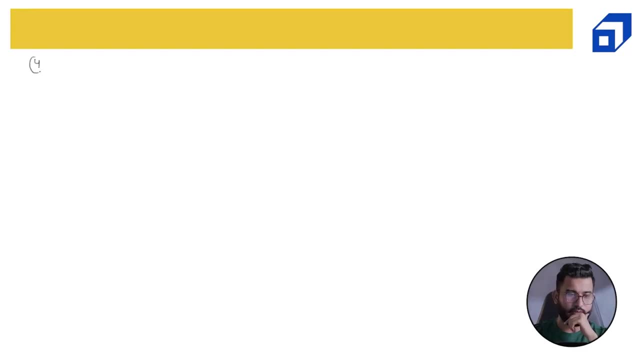 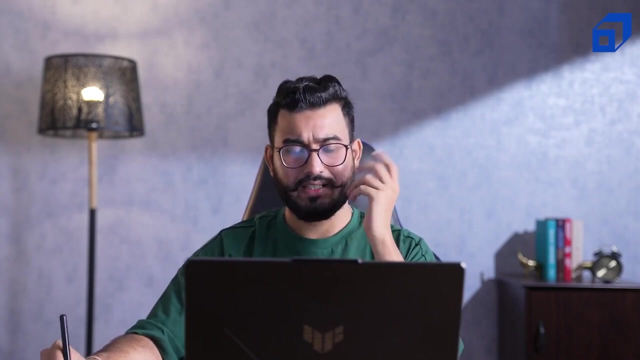 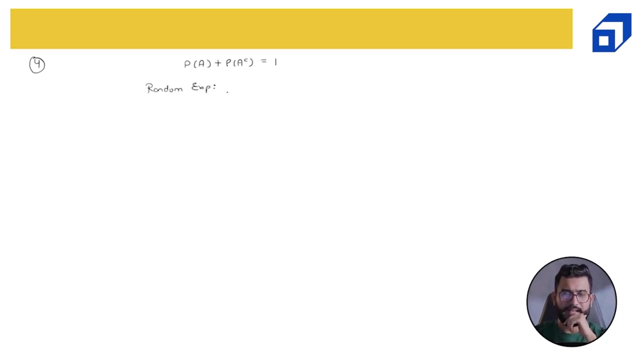 let's try to understand that. now. the fourth rule and the final rule is probability of a plus, probability of a complement is equal to one. what is the meaning of this? we have already seen this, but let's try to understand it again. let's take an event or let's take a experiment, the random experiment where 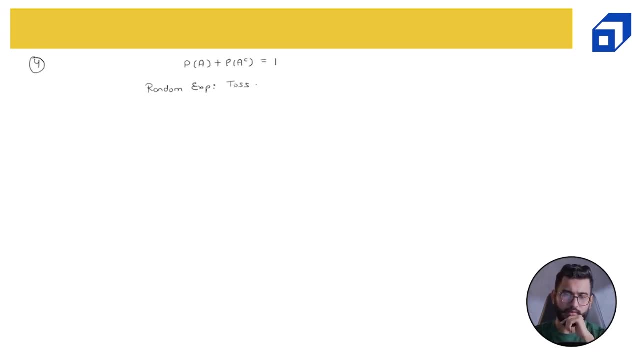 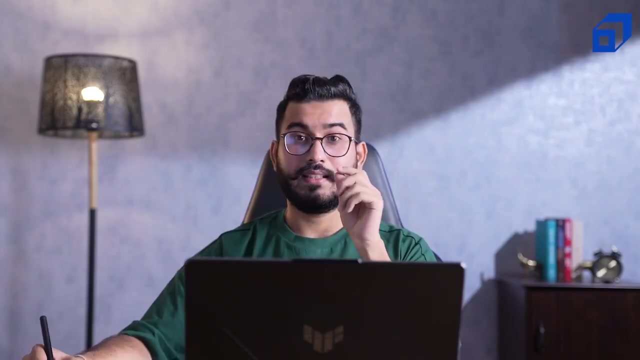 I'm tossing two coins, so toss of two coins, and I hope all of you are able to now build the sample space, which is we will get two heads, one head, one tail, one tail, one head, one tail and one head and then two tails. this is my sample space and this is a 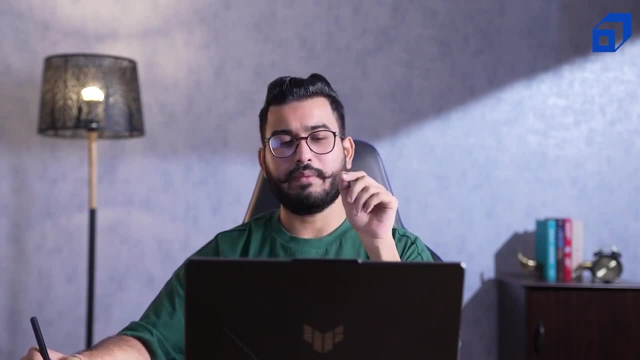 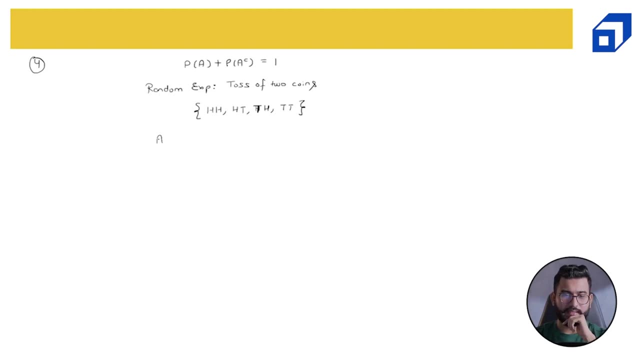 equally likely sample space. right, because each event is having same probability, right. okay, now, if I ask you so, let's say: event a represents both coins. both coins lands lands up with same outcome. both coin lands up with the same outcome. what is the complement of this? what is the meaning of complement, the opposite of this, this: 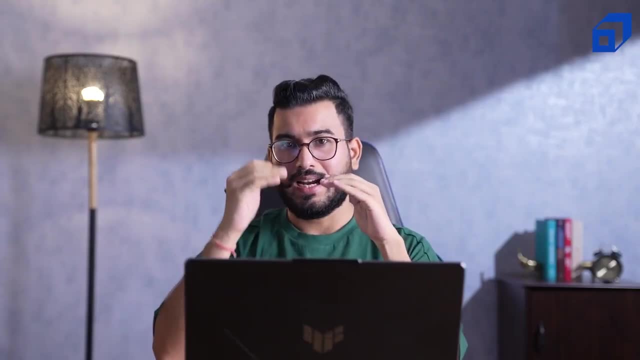 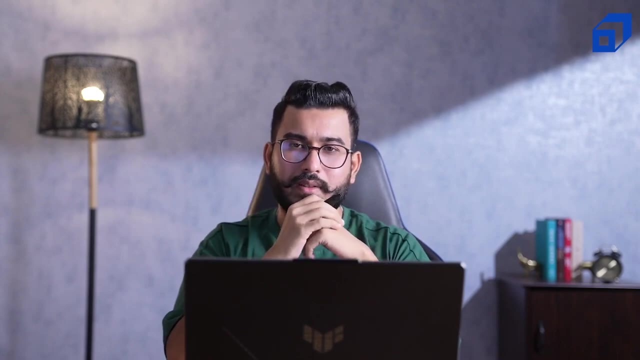 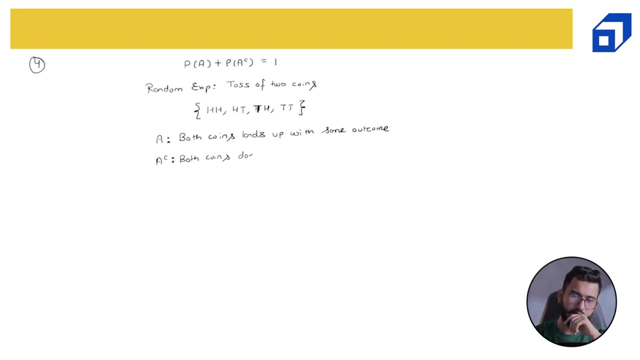 this statement. so I'm saying both coin lands up with same outcome. so the opposite of this is both coins did not or does not lands up in the same outcome. so let's write the complement: both coins does not lands up with the same outcome. now, what is going to be the sample event? 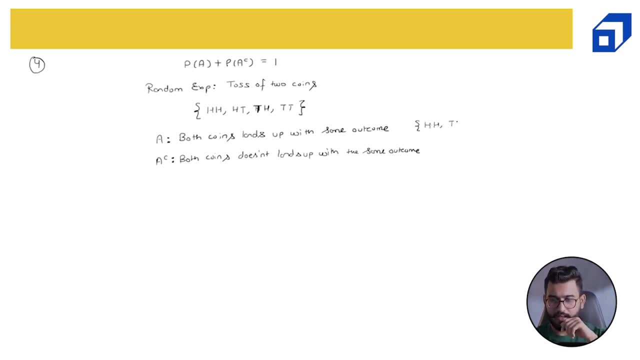 for a, it will be H, H and tail tail. the complement of this will be H, tail head, tail and tail head. now if I add these two probability, so probability of a is 1 by 2. probability of a complement is also 1 by 2. so probability of a plus, probability of 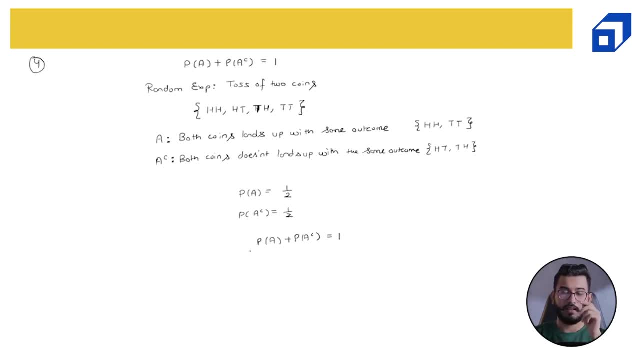 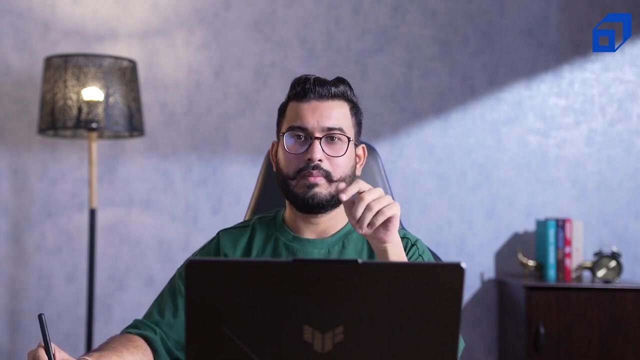 a complement is also equal to 1. this is a very important rule because sometimes you need to calculate the probability of a sample space and you just know one event. then it is simply. you can use this probability rule and you will be able to land up in the probability that you are looking for. 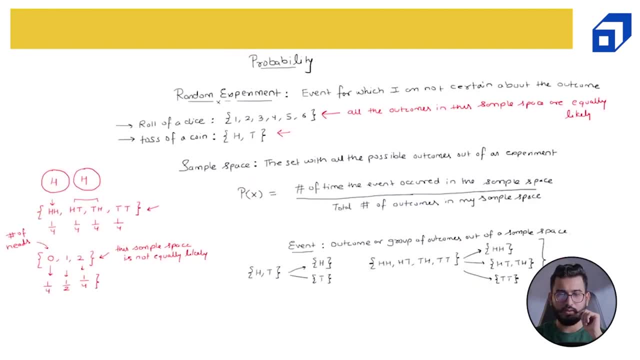 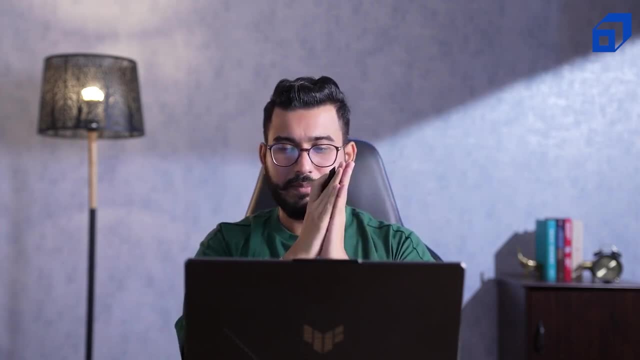 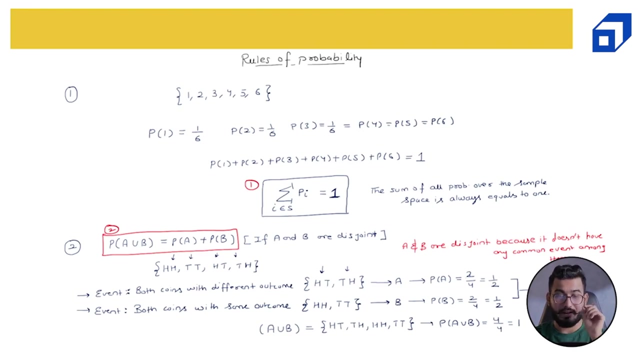 I hope all of you are now clear with all the four rules of probability. which is the addition of or the sum of all the probability over the sample space is always equal to 1 second. one is probability of a union. B is equal to probability of a plus probability of B if a and B are disjoint. if they are not. 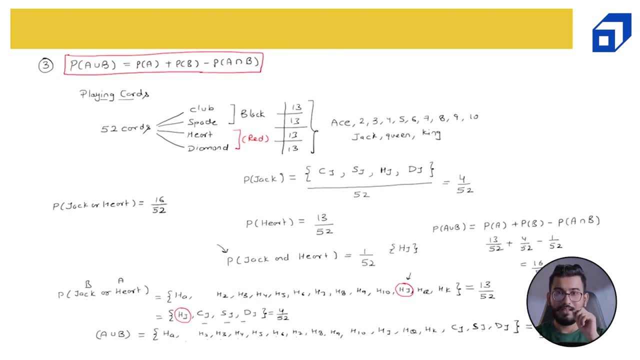 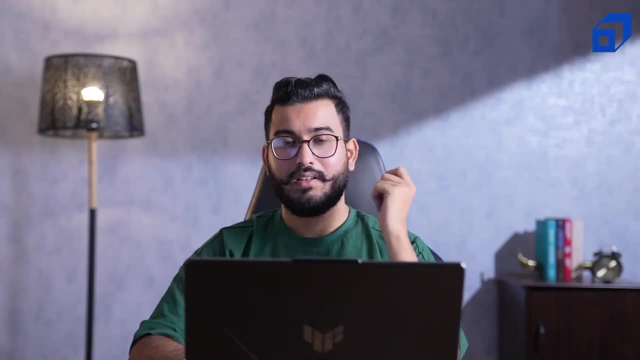 disjoint. then you have to subtract the probability of a intersection B and final one is probability of a plus. probability of a complement is always equal to 1. now let's try to understand the various types of events. a particular event or two events can be dependent or independent. then these two terms might: 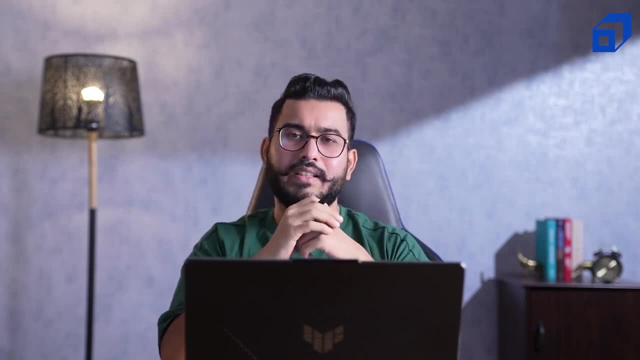 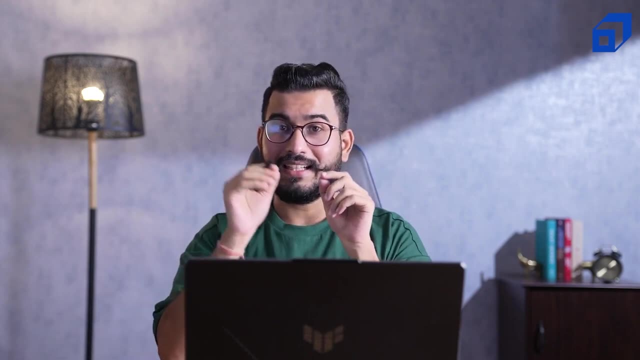 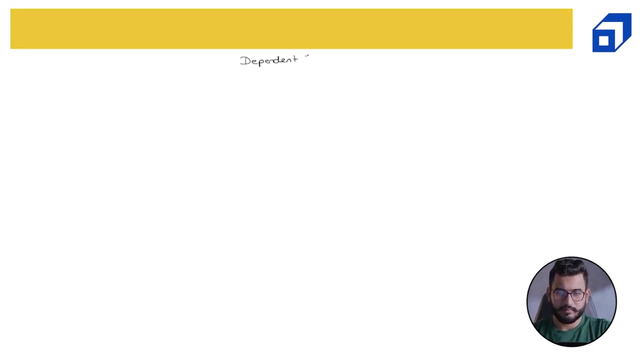 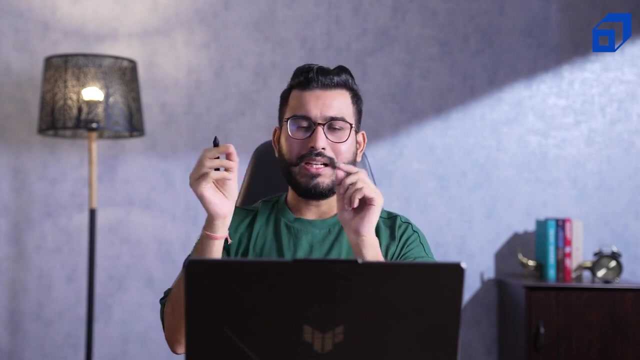 be familiar with you. but now let's try to understand them with an example. so now let's try to understand what is particularly dependent events and independent events dependent. first, we will try to understand the dependent events. when I'm saying events, I'm basically talking about two events or two or more events, right? so let's take 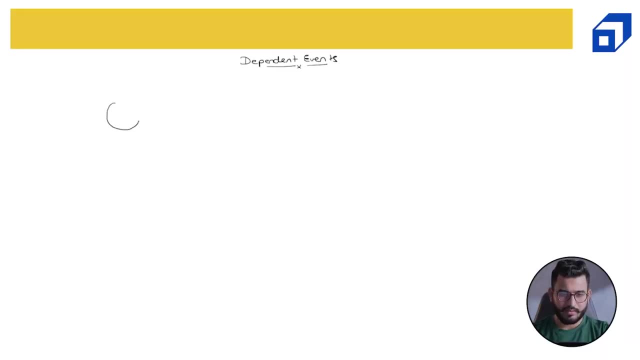 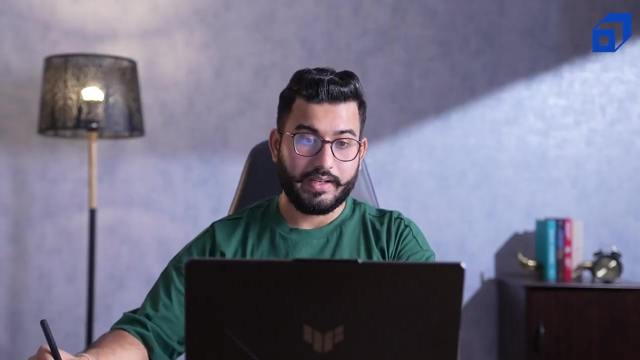 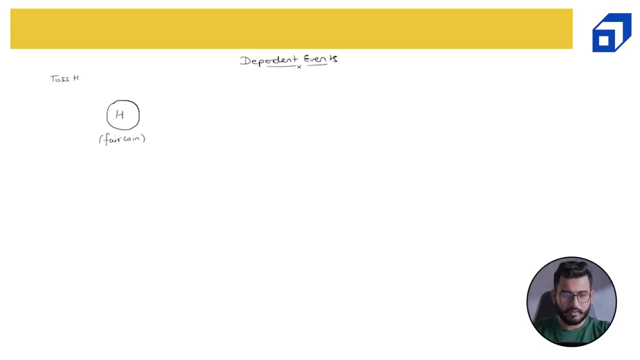 two events. I'm tossing a coin, so again my drawing skills. so this is, let's say, this is a coin and this is a fair coin. fair coin now, if I toss this coin for two times. so my experiment is to toss the coin for two times. now, when I toss, 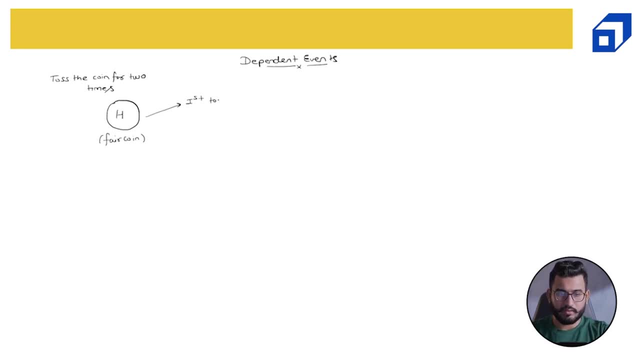 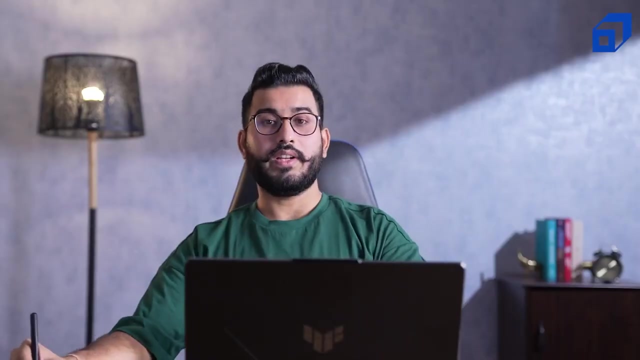 it for the first time, so this is my first toss. when I toss it for the first time and, let's say, heads appeared, so let me write it down. when I toss it for the, so let me write it down. when I tossed for the first time and heads appeared, so we 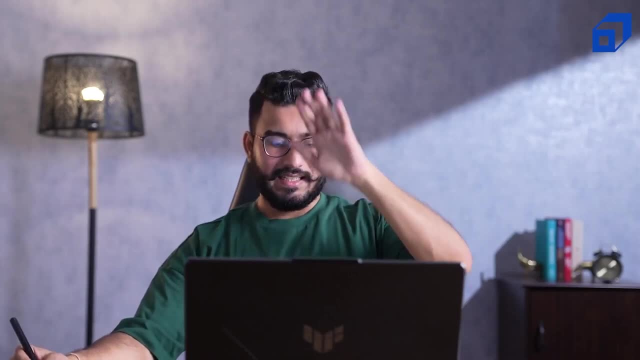 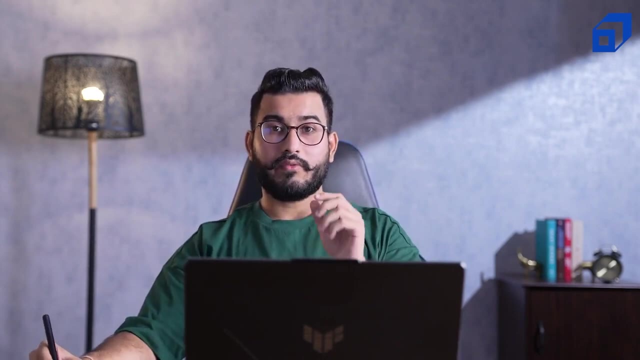 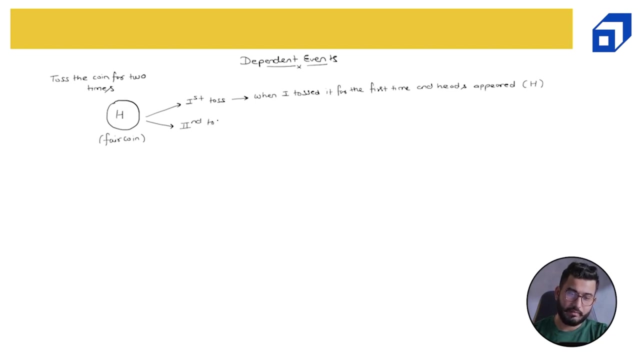 know that when I toss the coin and it lands up into head, you know this. so I let me write that the outcome of the first, first, the outcome of the first toss, is head now when I'm tossing the same coin for the second time. so second toss now. remember, the coin is same. I'm having the same coin but I'm tossing it for a 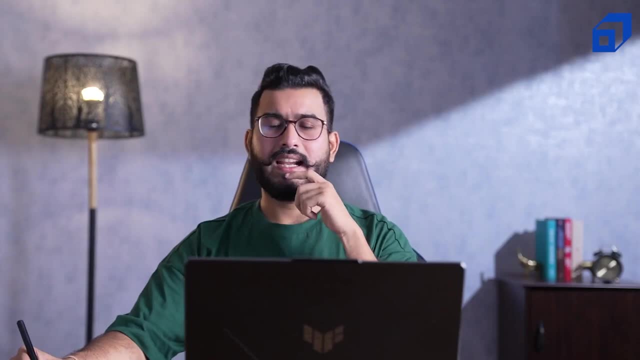 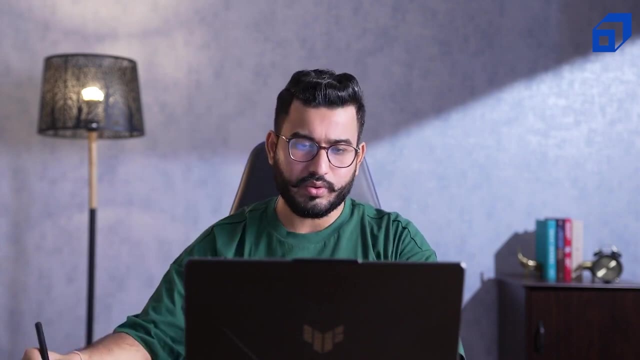 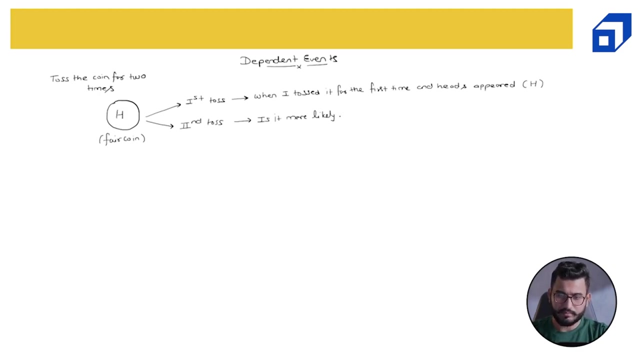 second time. now, when I toss it for second time, is it more likely that I would get a tail, because the first one was head. so my question to all of you is: is it more likely that we would get a tail, since the first outcome was a head? now all of you would say: 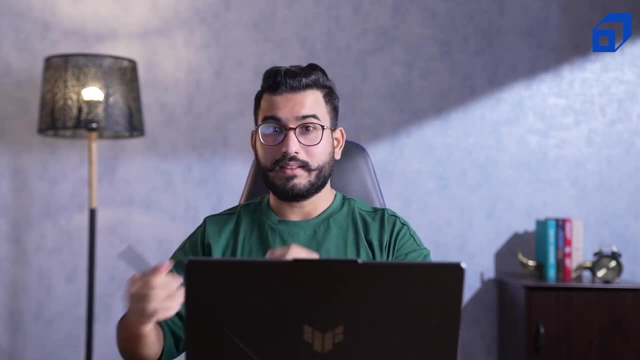 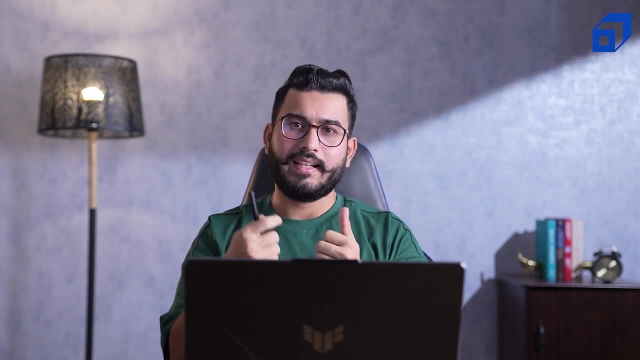 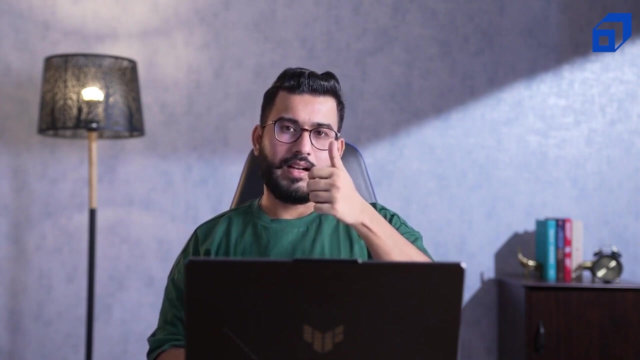 no, no I, because the next outcome can again be having the probability of getting head and tail to be equally likely, which basically means, if I'm tossing it for first time, I may either get a head or a tail. and what is the probability of getting head and tail? 0.5, 0.5, which is 1 by 2: 1. 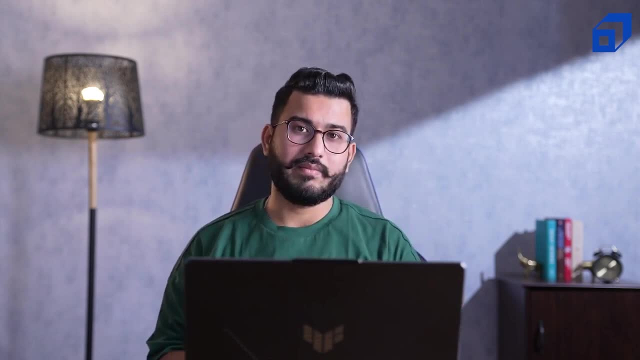 by 2. if I toss the same coin for the second time again, the probability of getting head and tail is 1 by 2. 1 by 2, which is 0.5, 0.5. so what I'm trying to say is: if I toss the coin for first, 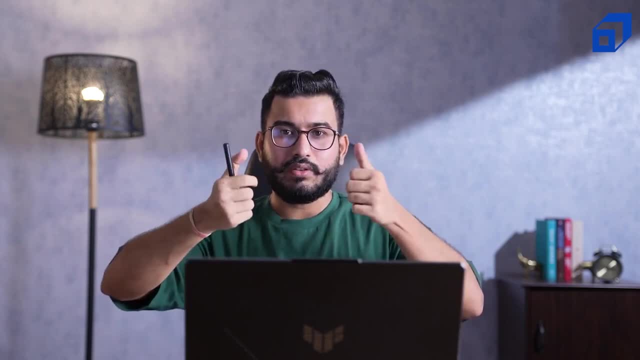 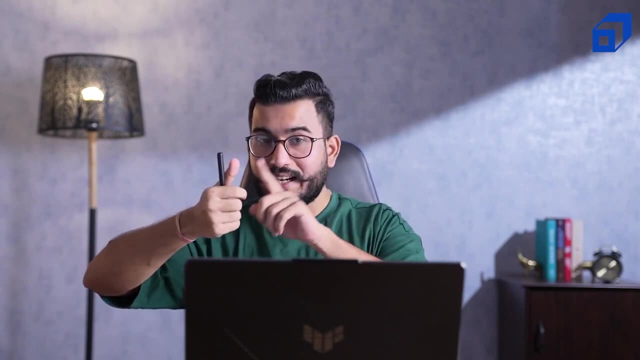 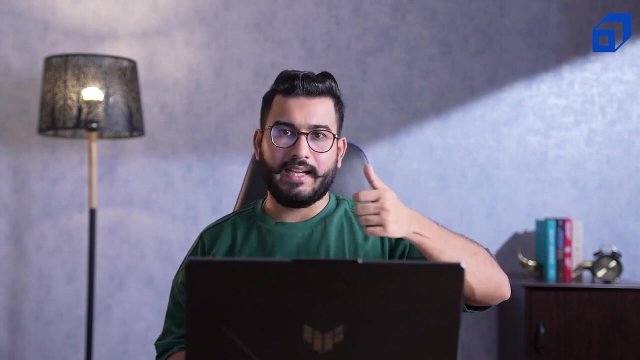 time and if I toss the coin for second time, these two tosses are independent of each other. the probability in my in the second toss is not getting influenced with the outcome of the first toss. if my outcome in the first toss is head in the second toss, it does it is. it is not influenced. 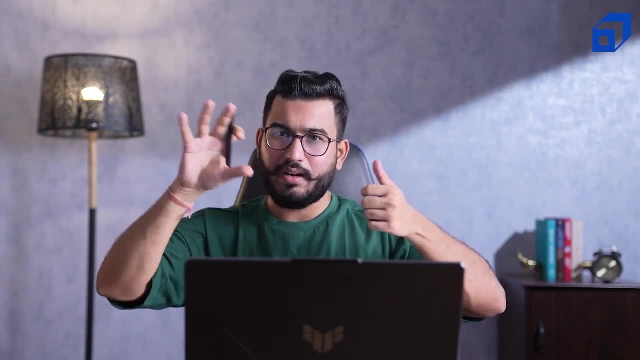 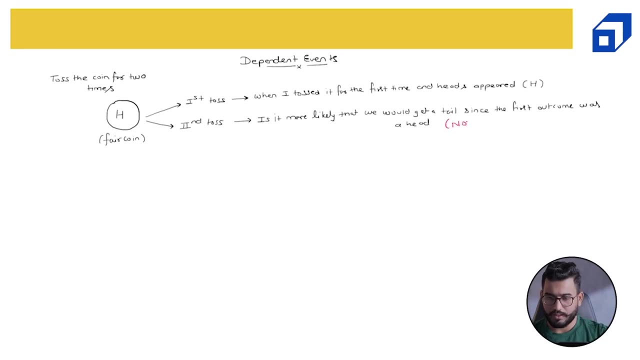 in right in the second toss it is, it can be still be head or tail. so in in simple words: first of all, the answer for this question is no, so I'll write a big no over here and the the rule is: the outcome of the first event is not impacting. 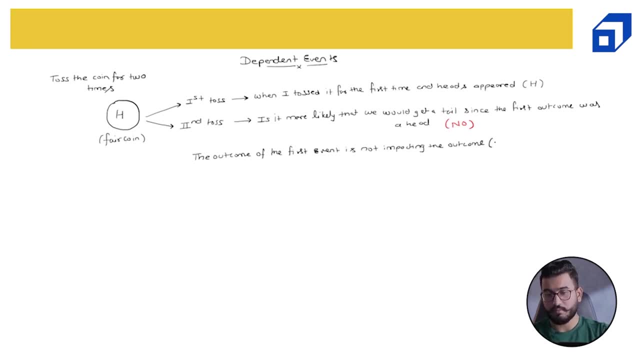 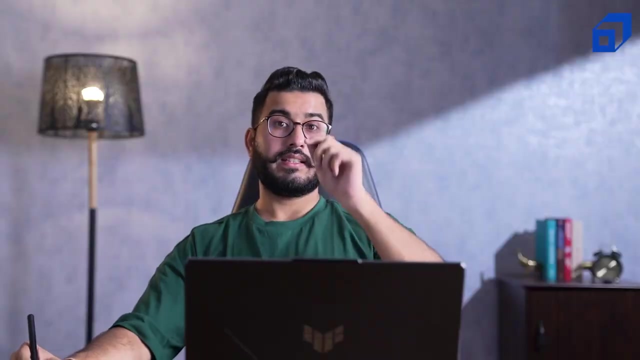 the outcome of the probability, the outcome or the probability probability of the second event or the second toss, and hence they are independent events. independent events. now there is a. there is a very good though. so in in probability theory, there is a very good. probability theory, there is a. 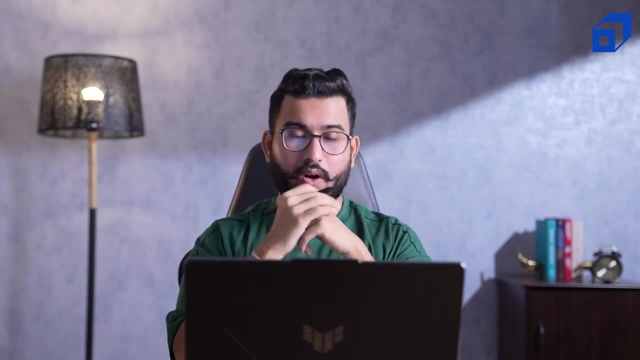 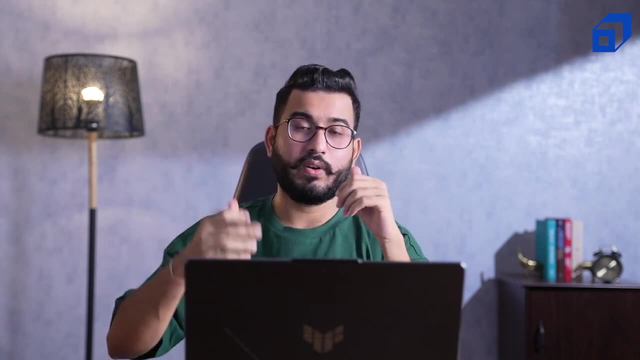 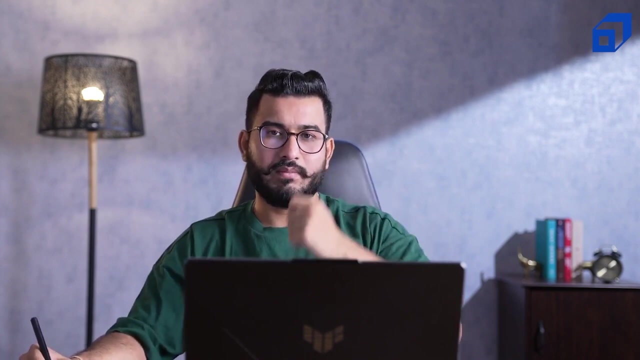 topic known as gamblers fallacy. what gamblers think that? if so, let's say, if the the game is of tossing a coin for 10 times, now, let's say there is a gambler who is given with the choice, who is given with the game to toss the coin for 10 times. for the first five times, let's say he. 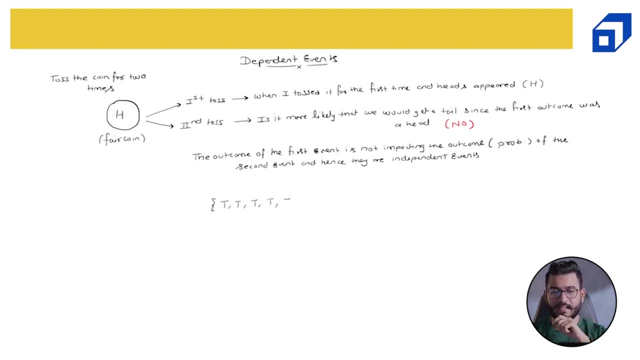 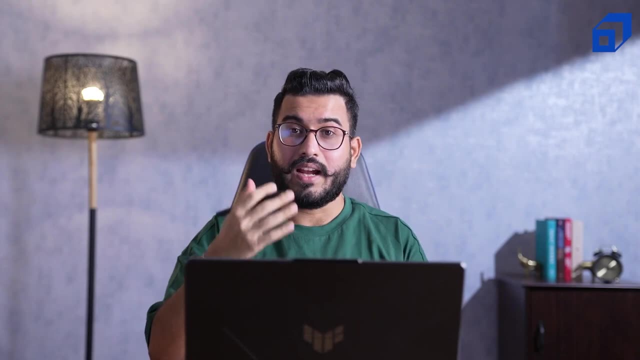 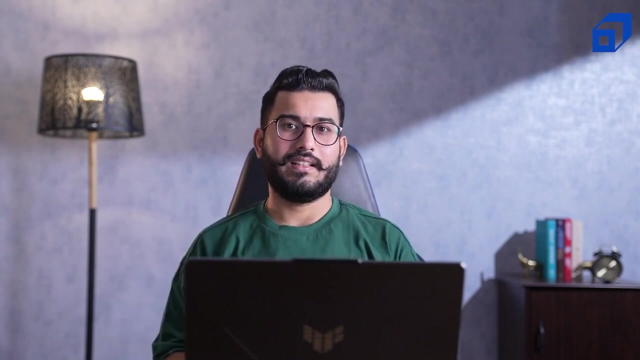 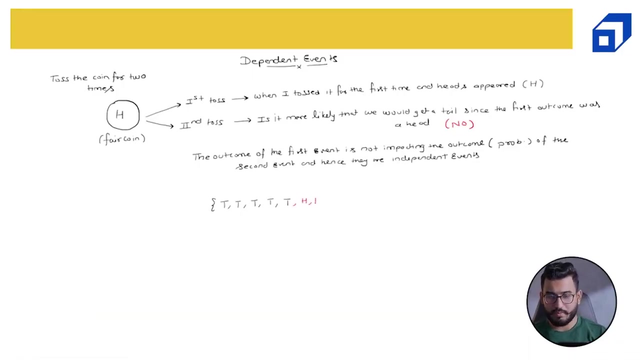 has got all tails. so tail, tail, tail, tail and tail. so for the first five times he has got all the tails. now what gamblers fallacy is that he will think that for the next five times he will get a head. so according to gamblers fallacy, the outcome for next five tosses should: 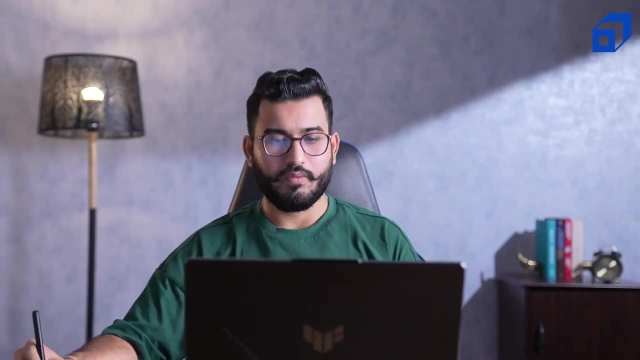 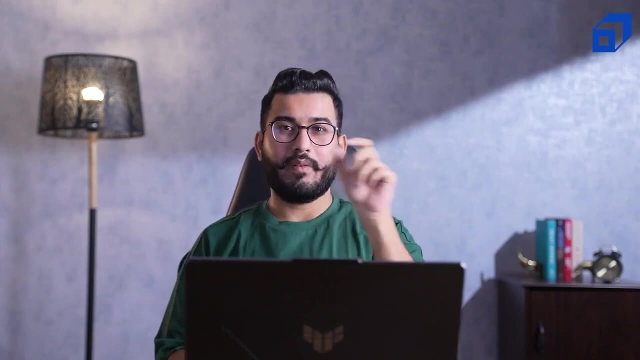 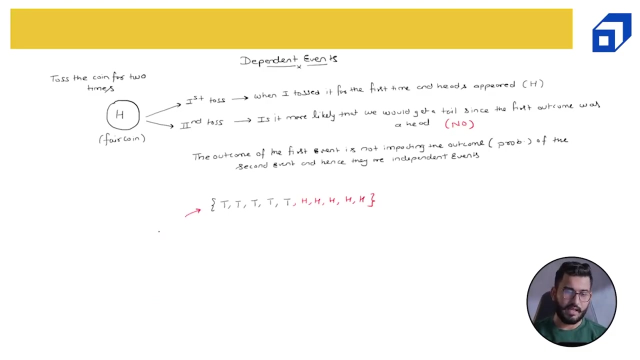 be head, head, head, head and head. why? because, according to the probability of head and tail, it should always be point five, point five. no, that's not wrong. it is only true when you are tossing the coin for very large time. that's known as the law of large number. so this is known as gamblers fallacy. this is wrong. this is wrong. this is. 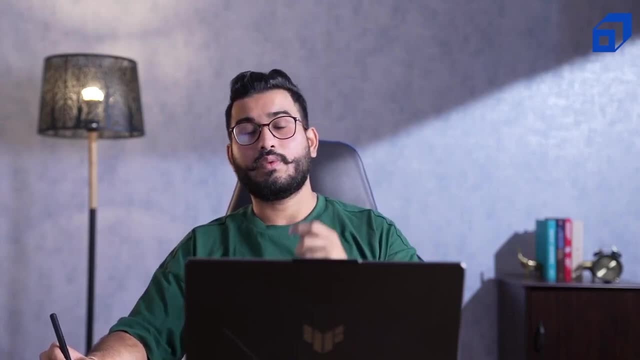 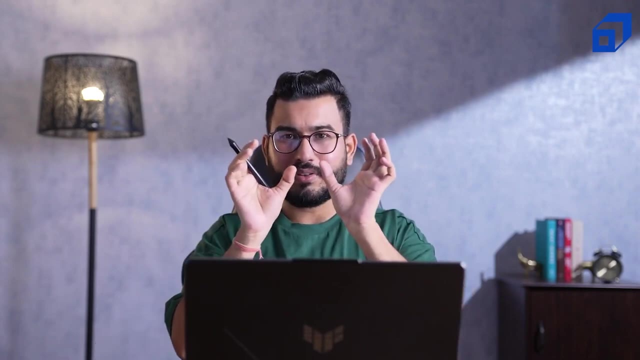 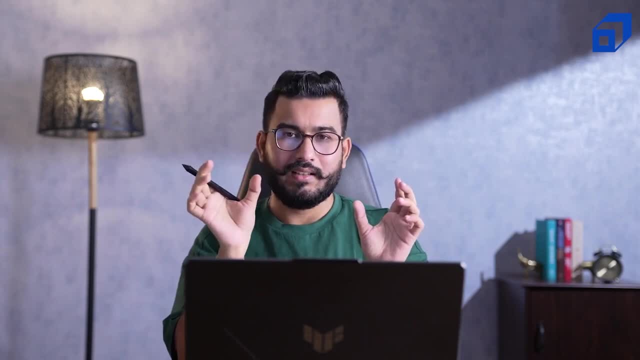 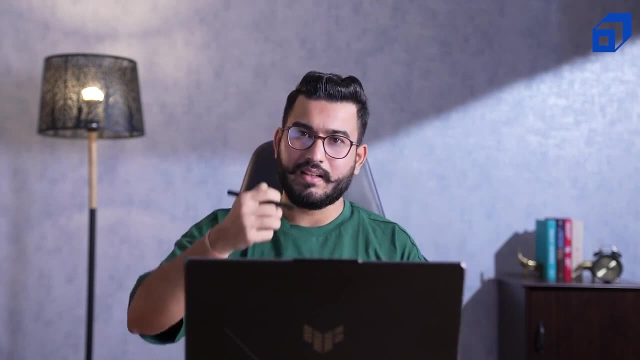 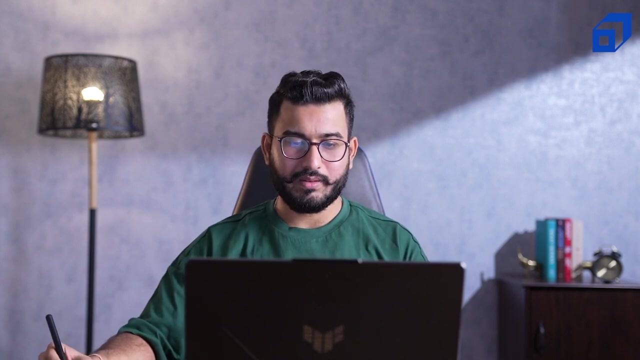 you obtained a head and five thousand time you obtained a tail. but if you are tossing the coin for two times and you expect that i will definitely get head for first time and tail for second time, that is wrong. that is the gamblers fallacy. so i hope you guys will not be landing into the gamblers. 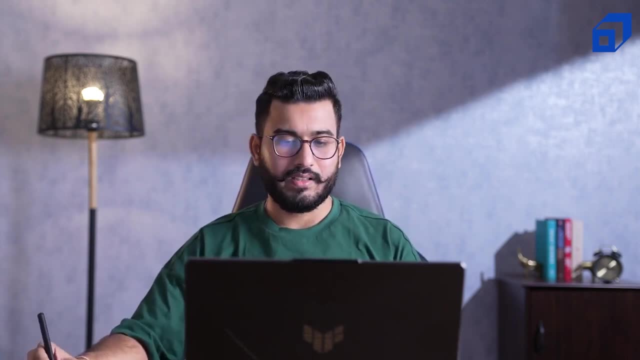 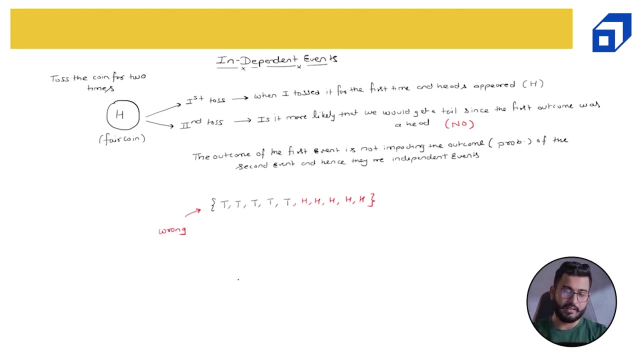 fallacy and i hope you are clear- with the dependent event independent, even independent. so when two events are independent, the probability of a and b is simply as probability of a multiplied by probability of b. so, for example, probability of getting head in first toss and probability of getting head in second toss. 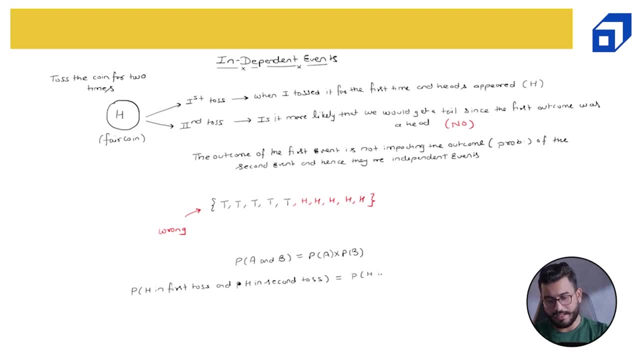 is simply can be written as probability of head in first toss multiplied by probability of head in second toss, and this will be equal to 1 by 2 multiplied by 1 by 2, which is 1 by 4.. i hope you guys are clear. let me just quickly show you. 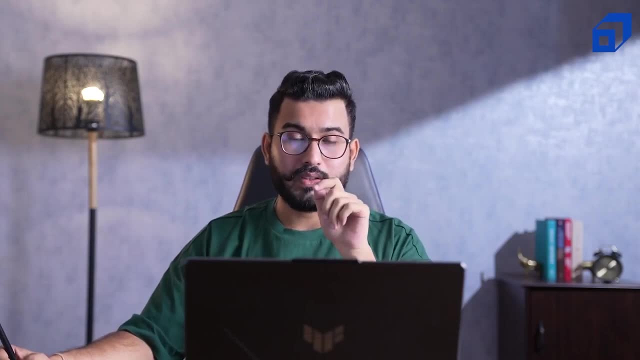 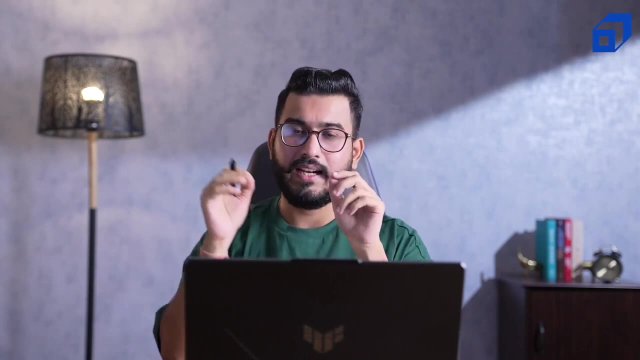 one example of gamblers fallacy which proves that when you toss a coin for very large time, then only the probability of head in first toss will be equal to head in second toss. the probability of head and tail will be closely or approximately be equal to 0.5 and 0.5. 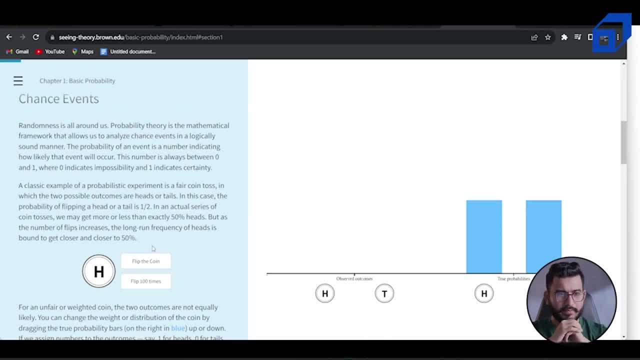 now here you can see there is a very cool website which is scene theory dot brown dot edu. this is an open source website. now it shows this is: these are the true probabilities. basically mean the probability of head is 0.5, for tail it is 0.5. now i can flip the coin, so the if i flip the coin for 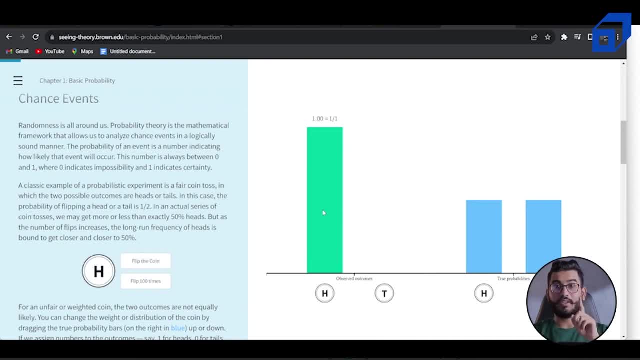 1 time. you can see that for the first time or i obtained a head, so my probability of getting head is 1 by 1 if i flip it for one more time. i obtained a tail, so 1 by 2, 1 by 2 if i flip. 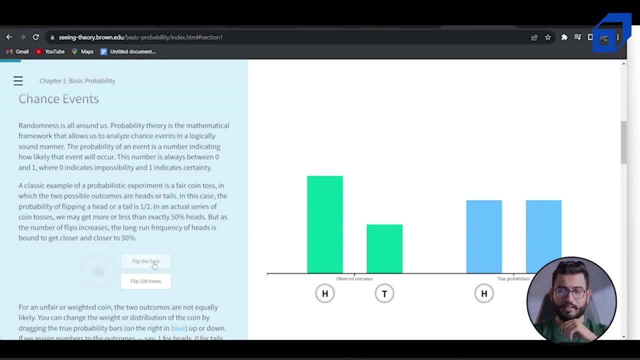 it for one more time. i obtain a head for one more time again ahead for one more time. a tail for one more time. a tail for one more time ahead. now, if i do it for hundred times, I obtained out of 107 times. head came for 57 times, tail came for 50 times. let me do it for. 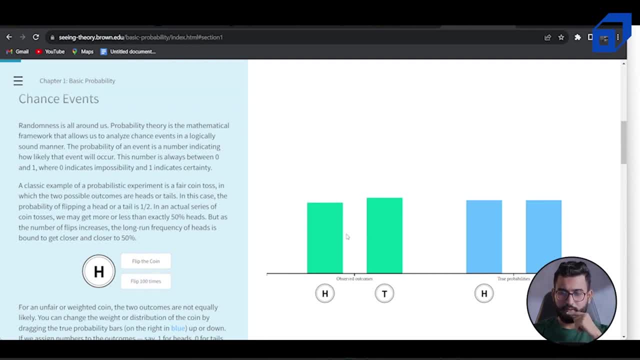 one more hundred time. now you can see that now the probability of tail is more than the probability of head if I do it for thousand times, so which basically means I have to hit this button for eight more times. so 1, 2, 3, 4, 5, 6, 7 and 8. now just look at this for point four, nine. 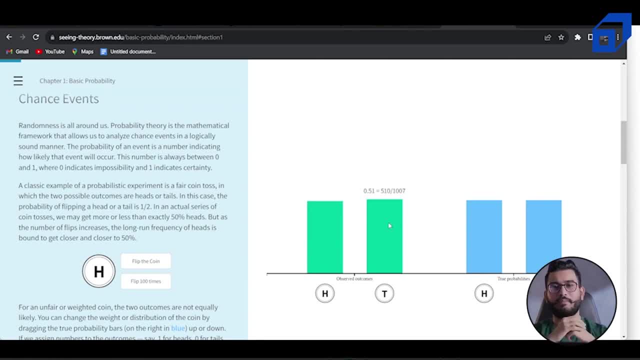 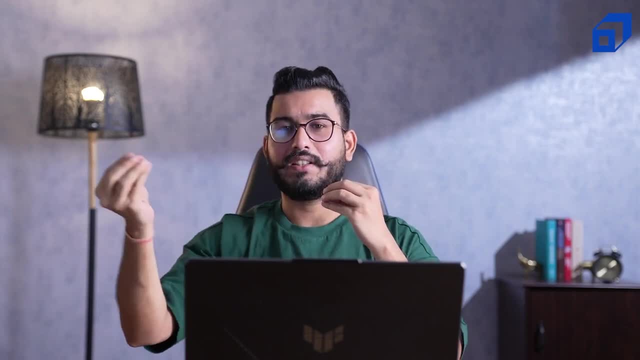 point five, one very close to point five and point five right. so this is point four. nine point five, one very close to point five and point five right. so this is the law of large number. if i perform the experiment for very large time, then my observed outcome or 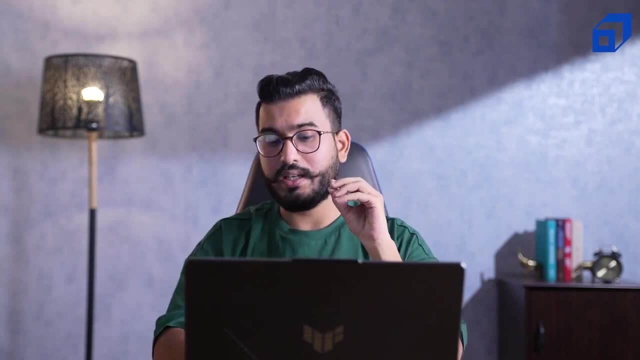 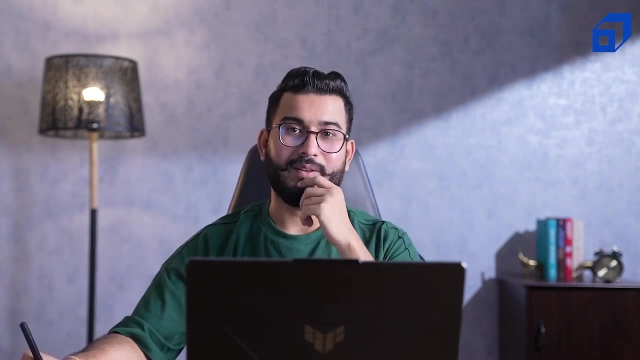 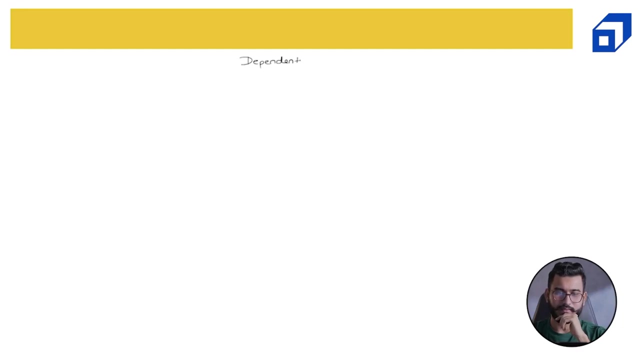 observed probability will be close to the true probability, which is 0.5 and 0.5. i hope this makes sense to all of you. so now let's talk about dependent events. so dependent events. now for dependent events. we will take a very simple example. let's say i'm having a bag. 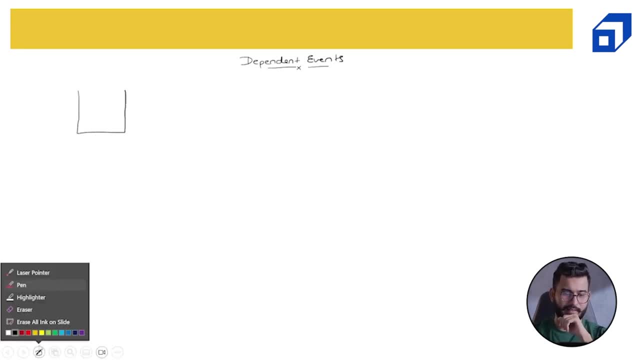 and this bag is having, uh, let's say, two orange balls. we have two orange balls and, let's say, some white balls. so for white balls, i'll draw it like this: one white ball, two white ball and three white balls, so total i'm having five balls, in which 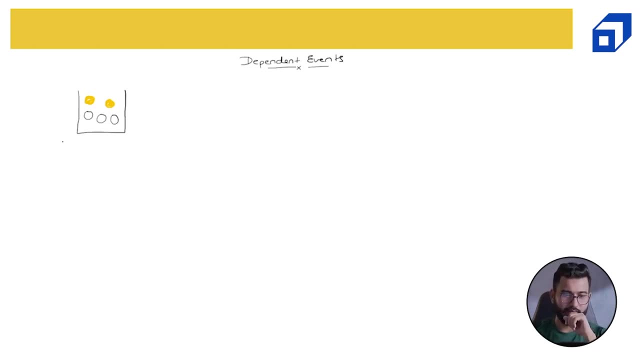 there are two orange, three white. so let me write it down: uh, two orange and three white. okay, now the experiment is: we take a ball out of the bag. so so, take a ball out of the bag. we have to note the color. so note down the color. 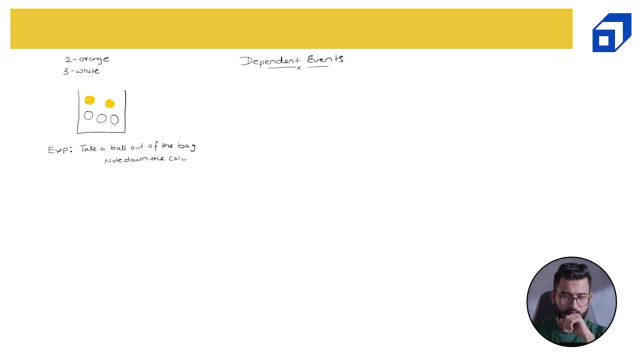 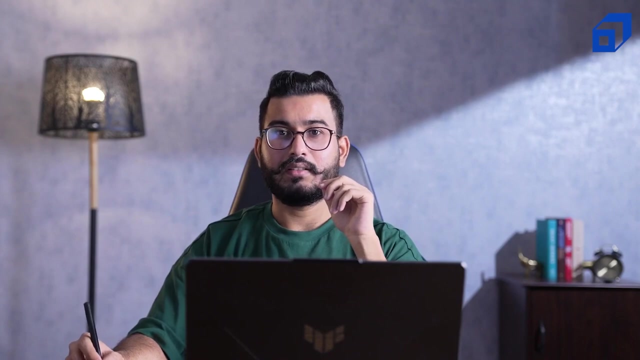 and we put another ball, we'll take out another ball out of the bag. so take one more ball out of the bag and then we note the color of that ball also. note down the color. now. please carefully remember that this experiment is without replacement, so let me just quickly. 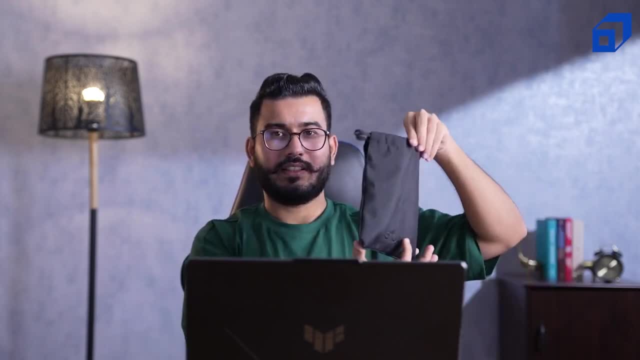 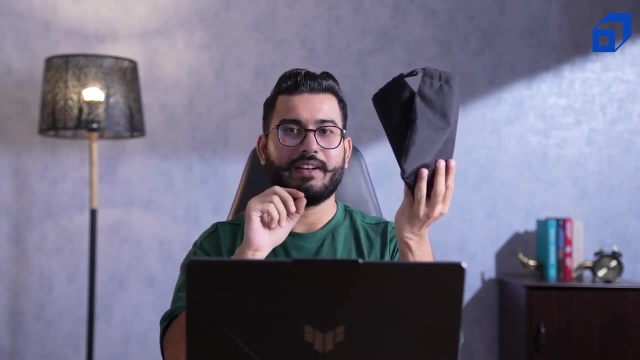 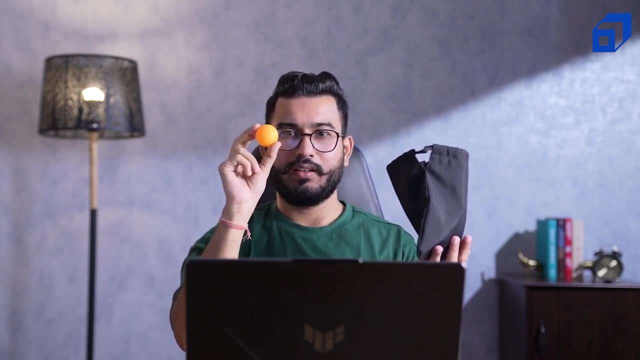 demonstrate this example. let's say this is my bag and this bag is having two orange balls and three white balls. now what is the experiment? I have to take a ball and let's ball out of the bag. so this is my orange ball and I note down the color. so we 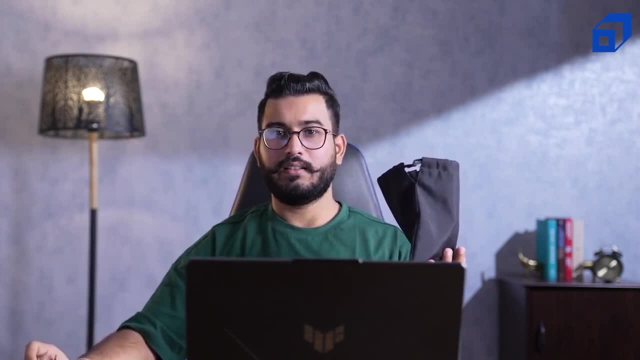 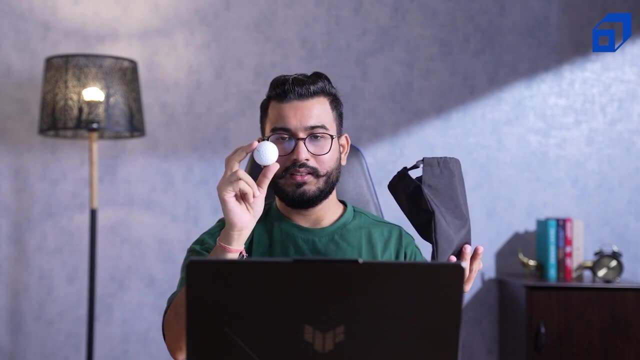 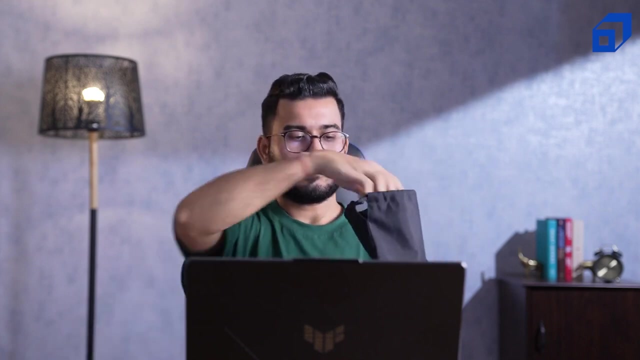 will write orange and we keep it outside. then we again take a ball out of the bag. this is a white ball. we will note down the color and we will keep the ball out of the bag. so this is what is my experiment. I hope everyone is clear now. 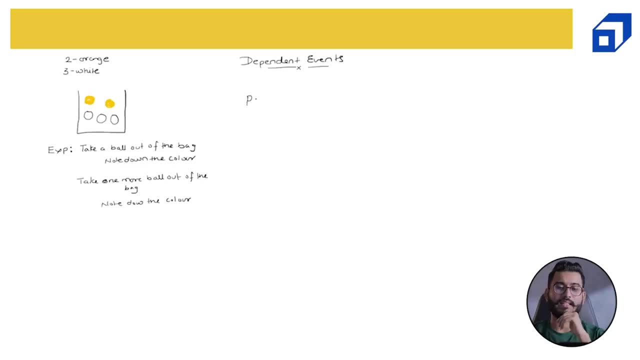 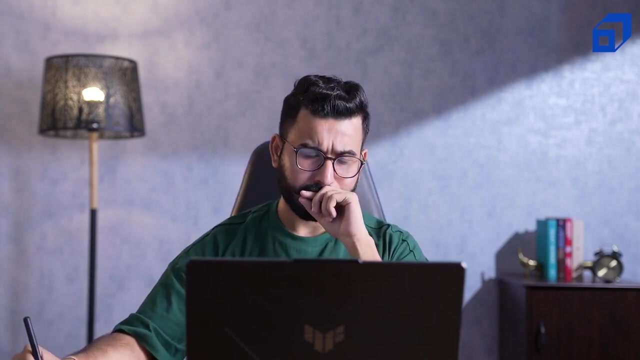 my question is: we have to calculate the probability that I get a orange, so O. so first ball happens to be orange, second ball happens to be white, so what is the probability that I will get first ball as orange and second ball as white? now let's solve this problem step by step. when I am taking out the first, 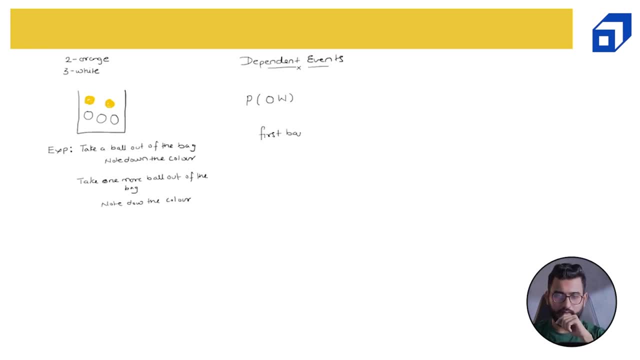 ball. I am having the following problems: that I am taking out the first ball, appreciate it. I'm getting silver and I'm taking out the orange middle and the. so this is my first ball, first ball. when I'm taking out the first ball, the bag is having. 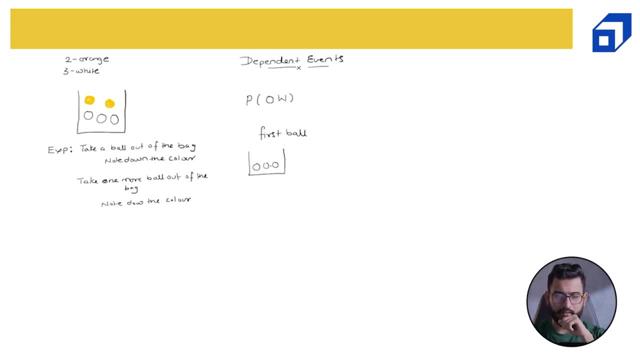 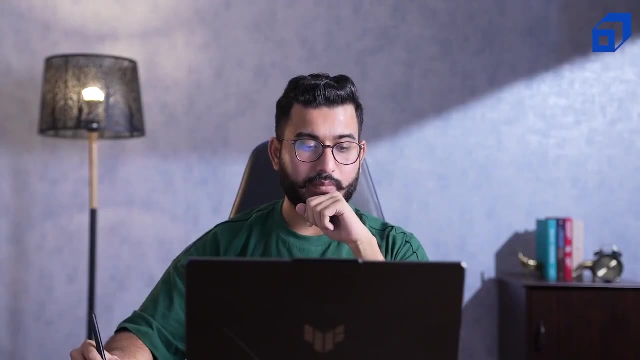 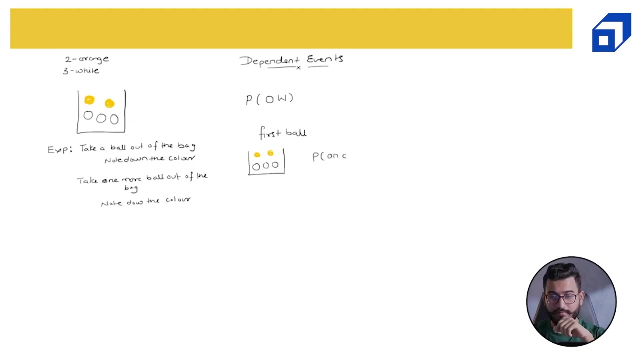 three white and two orange right. so initial is three white and two orange. now what is the probability of getting a orange ball or an orange ball? probability of getting an orange orange ball: this is simply we 2 divided by 5. why? because I have 2 orange ball and 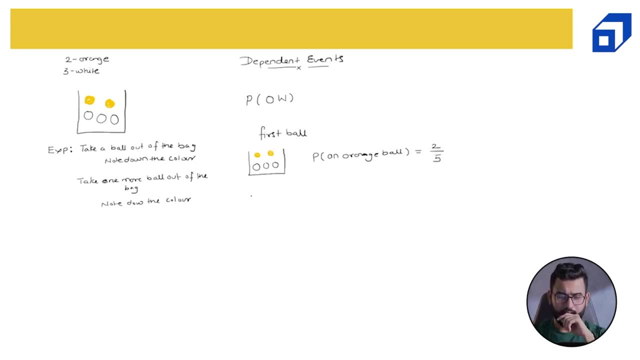 there are total of 5 balls. now I have taken this ball out of the bag, so the bag is now. so I will take this ball out of the bag. this ball is out of the bag now. now the bag is now your orange ball. orange" is left with one orange and three white balls: One, two, three. Now what is the probability? 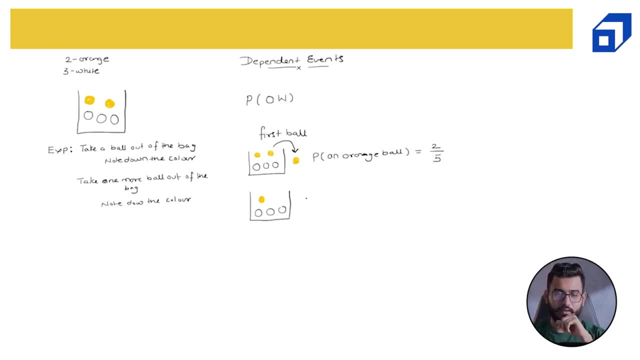 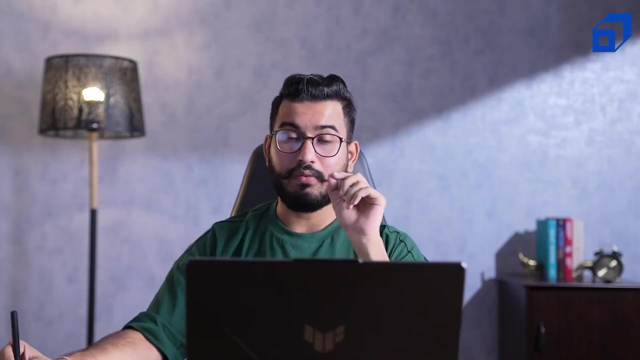 that my second ball is a white ball, So probability of second ball is a white ball, but there is a condition given to us. So given that, so this symbol means, given that the first ball was orange, So we know that first ball was orange. Then what is the probability that? 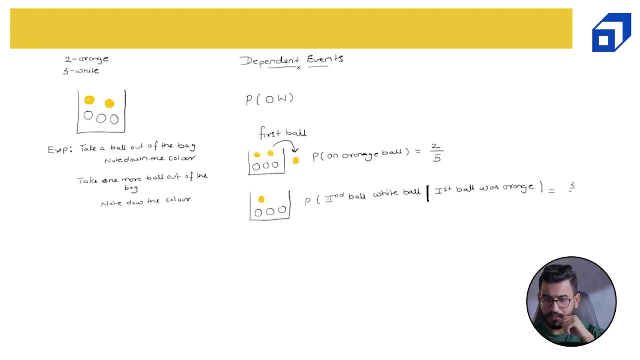 my second ball will be white. This will be three divided by four, Because we have three white balls and total are 4 balls. Now, if I ask you, what is the probability of getting orange and white? So what is the probability of first ball as orange and second ball as white? Now this: 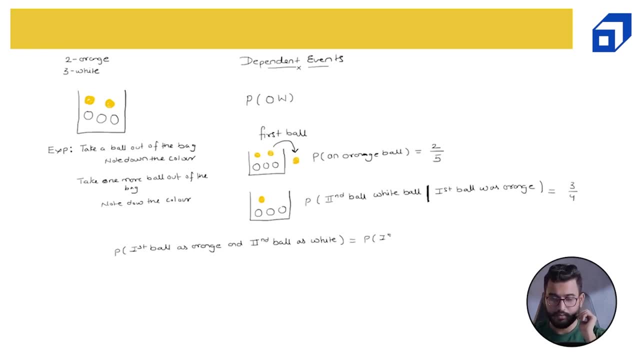 will be simply as probability of first ball as orange multiplied by probability of second ball as white, given that first ball was orange. So this would be 2 divided by 5 into 3 divided by 4.. So this will be 2 times. So this will be 3 divided by 10.. This is my probability of getting. 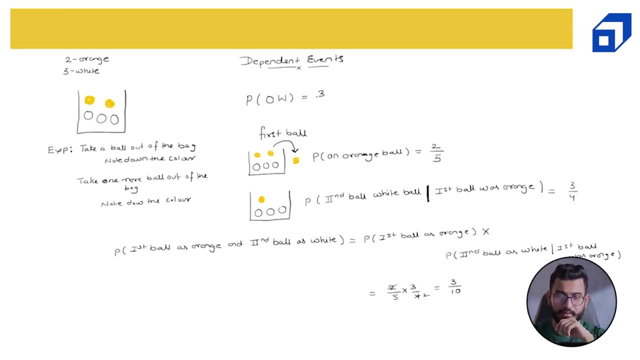 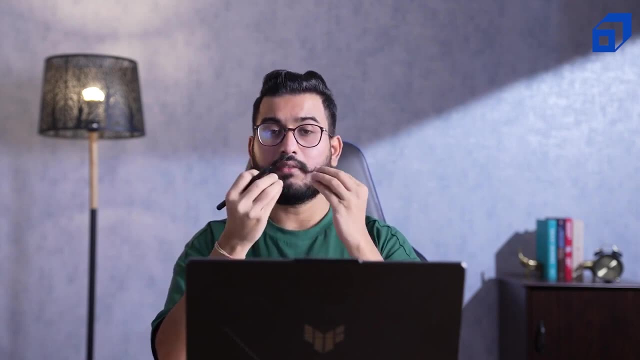 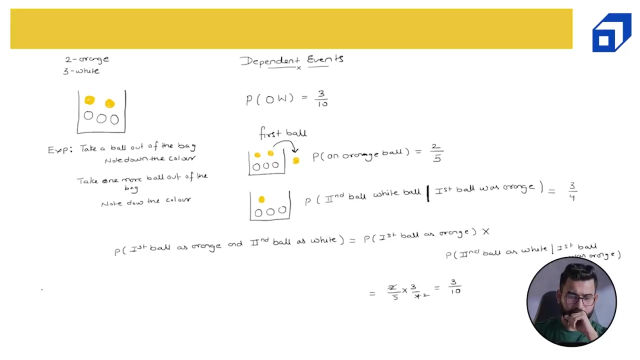 first ball as orange and second ball as white. So this is 3 divided by 10.. Now here, if you carefully understand the experiment, the probability of second ball is dependent on the outcome of the first trial. So here is a note: The probability. 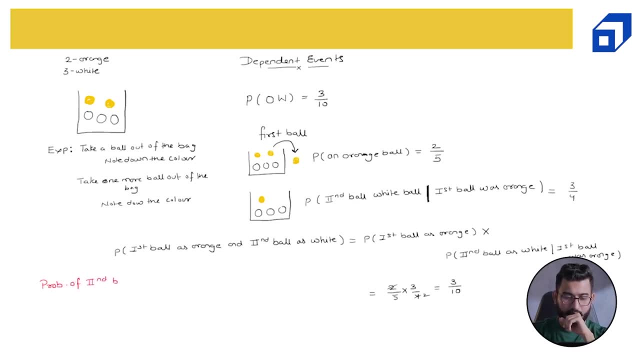 second ball is dependent on the probability or the outcome of the first toss, or first trial, or first. I would say first trial is a correct word. So this is what is my dependent event is dependent events. so when two events, A and B, are dependent on each other. if they are dependent, then the probability. 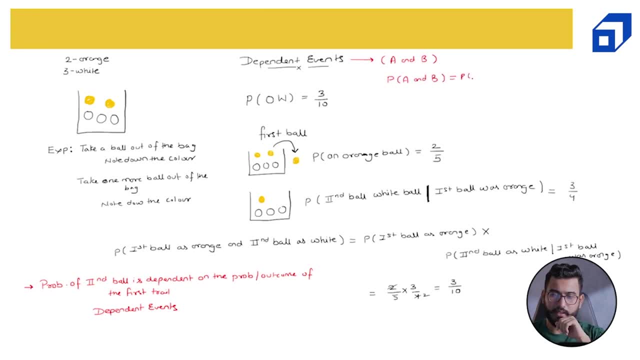 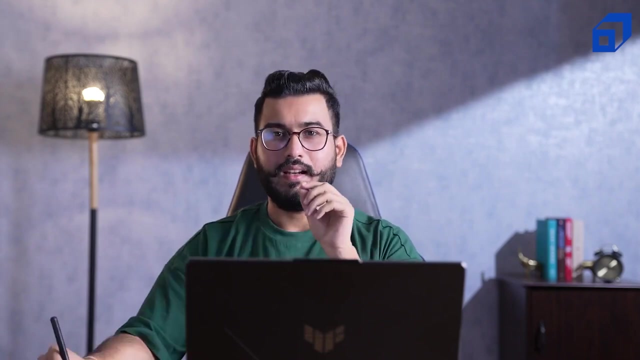 of A and B is given as probability of A multiplied by probability of B, given A has already happened. This is my probability of A and B. Now, this is the dependent rule, when two events are dependent on each other. I hope this experiment, this example, makes sense to all of you. Let's 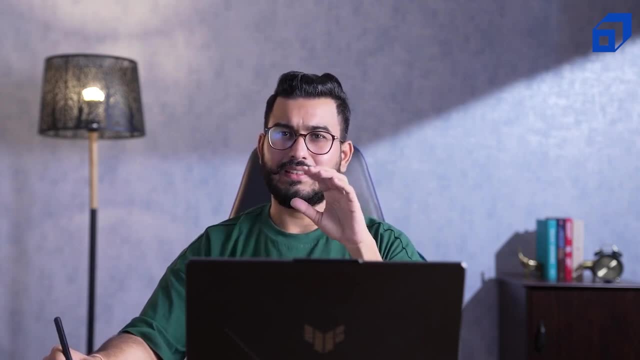 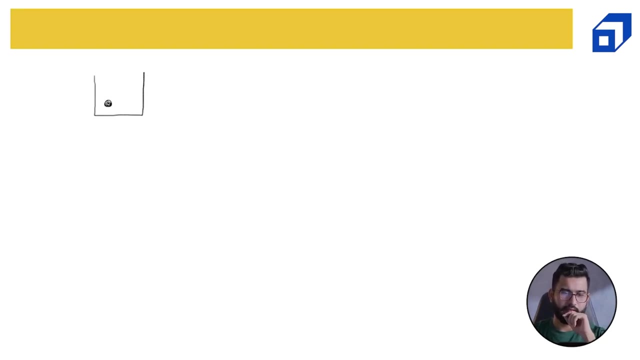 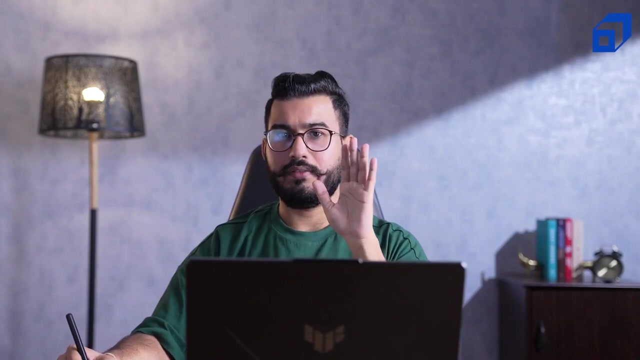 take one quick example to understand the dependent case in a better way. Let's say: I'm again having a bag. this bag is having three black and I want all of you to take out pen and paper and try to solve this. Pause the video, try to understand the logic and solve it. So the question is: the bag is 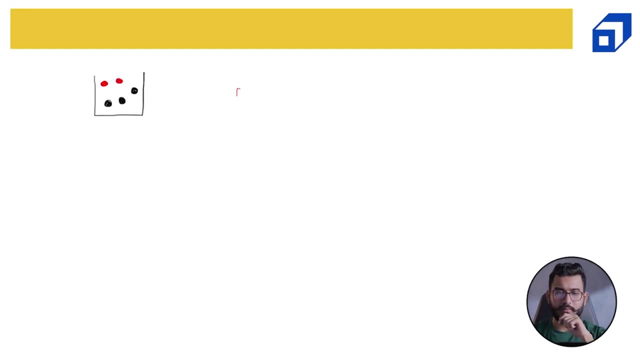 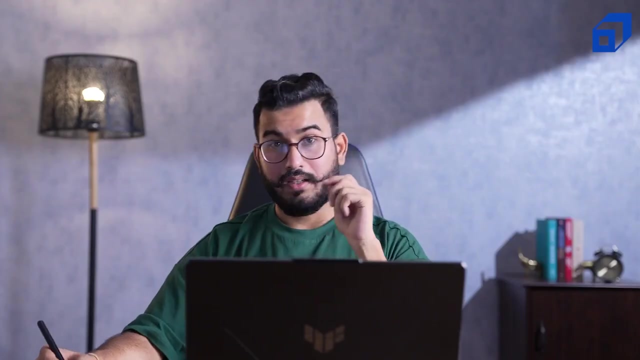 having three black and two red balls, What is the probability of getting red? red which basically means probability of red in first draw and red in second draw? This is my question. now let's try to logically solve it. I want all of you to pause the video and try to. 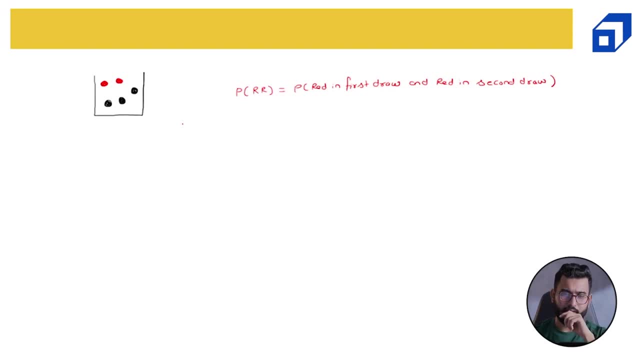 solve it by yourself. I hope you guys would have solved it already. So let's say initially the bag is having two reds and three black balls. Three black balls: Now the probability of the first ball being red is two divided by five. right Now, this ball is out of the bag. now. 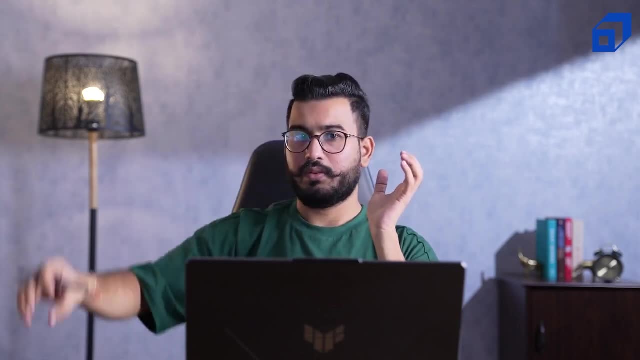 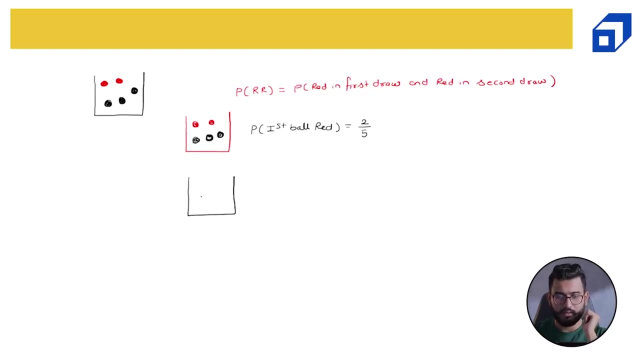 so I have taken out the ball. I have kept it outside, so the bag is now left with one red and three black, So one red and three black. Now what is the probability of getting the second ball as red, given that I have already taken out the first ball as red? given that 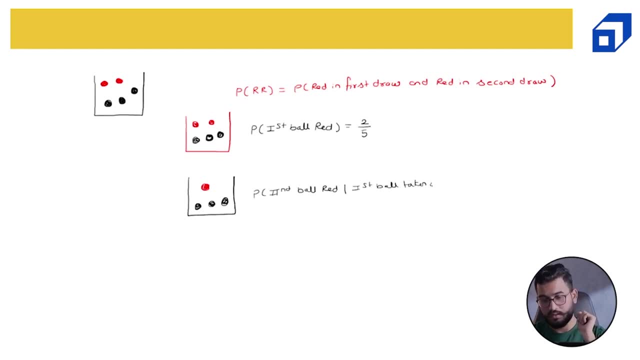 first ball taken out was red. Now this would come out to be 1 divided by 4, because I am left with one red ball and total balls are left are 4.. So what is the probability of getting a red red, which basically means red in first trial and red in second? This will be probability of 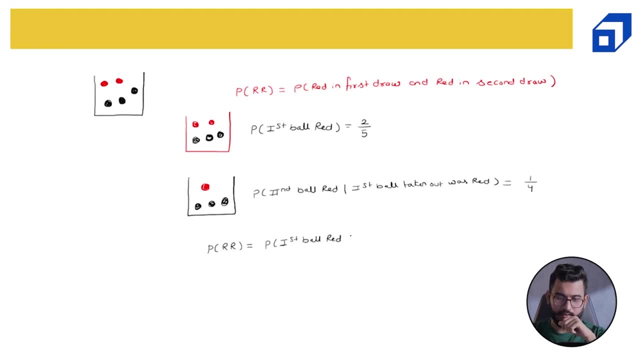 first ball as red, multiplied by probability of second ball as red, given first ball taken out was red. So this would be 2 divided by 5, multiplied by 1. divided by 4, this is 1 divided by 10.. I hope you guys were able to solve this question. Now let's talk about 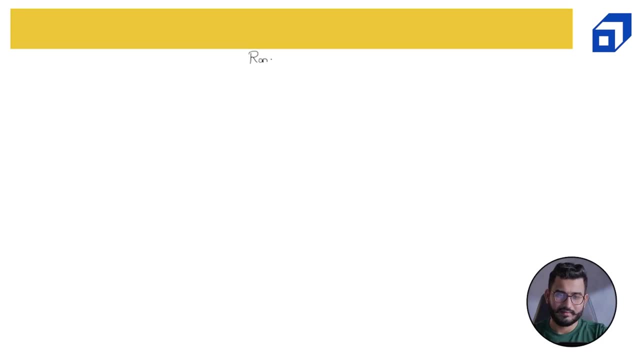 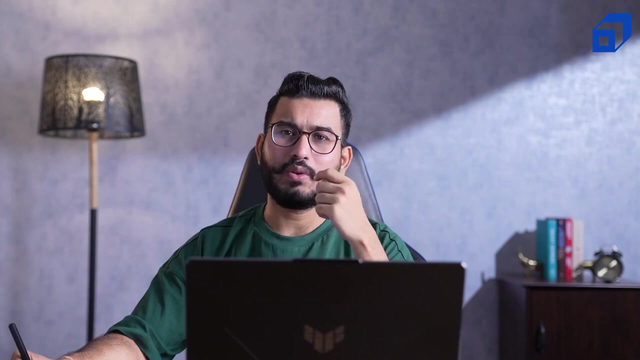 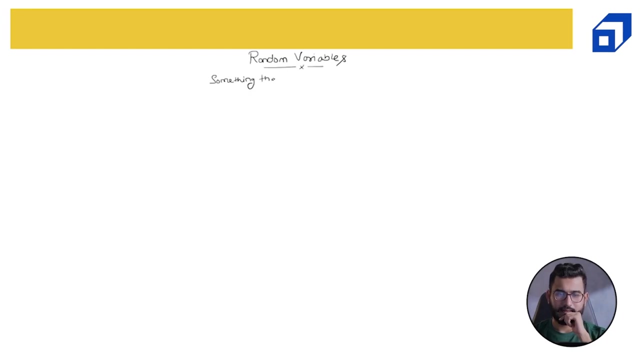 random variables. Now, random variables is something that quantifies the outcome of an experiment. something that quantifies the outcome of an experiment. Now let's try to understand it in a better way. So let's say, I am tossing two coins, So my experiment is toss of two coins. Now the 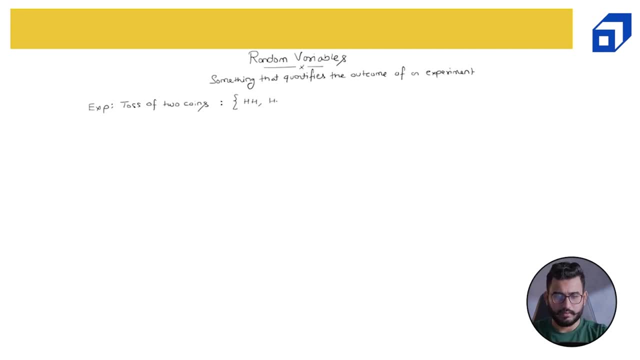 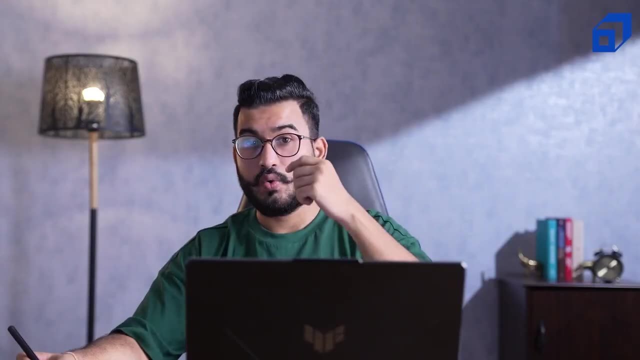 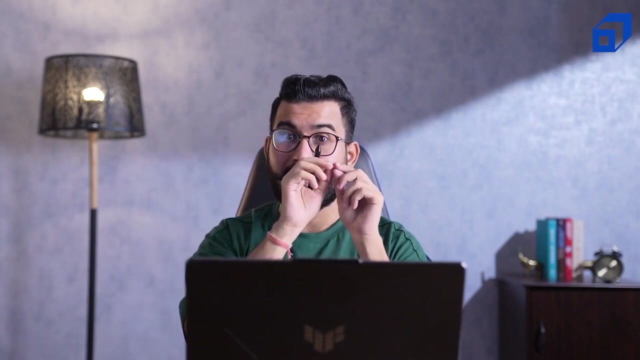 example, space for this would be comfortable. space for this would be two heads: head, tail, play ahead and T eject. Now how I can quantify the outcome. What is the meaning of quantification? converting the outcome into a number or mapping outcome into a number? so let's say, my random variable can be so. 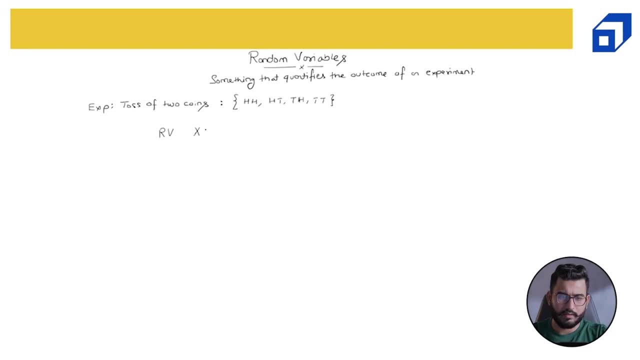 are we assigning the variable with the sign that sanie How to find a Α- owes the num. So my ex x, Good number of heads in a toss of two coin in a toss of two coins. now, this is my random variable, and 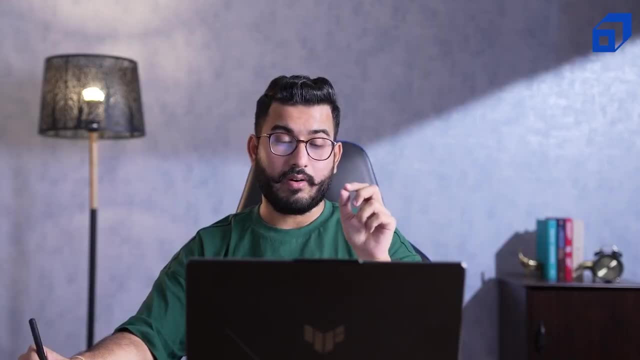 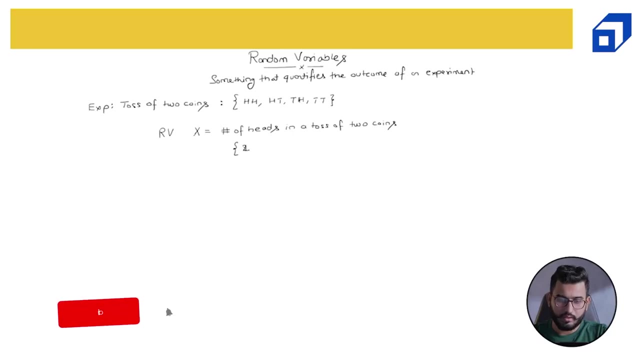 this will map the outcome of the random process, which was toss of two coins, into numbers. I will get two, one and zero. how so, if I write head, head, head, tail, tail, head and tail, tail, now this corresponds to two heads. so the number of heads when you toss two coins can be two heads this. 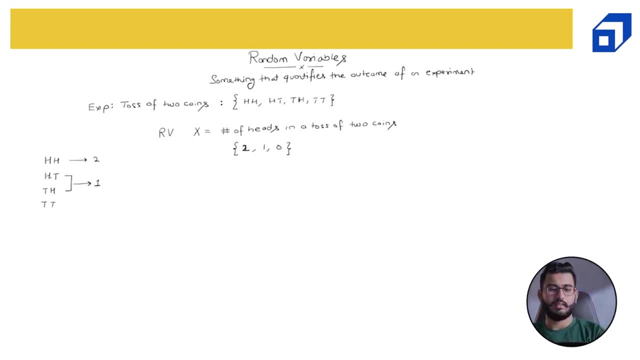 both quantifies to one, because in both of these outcome I am getting one head and this is mapped to zero because there is no head. so two, one, zero. this is my random variable X. similarly I can have a random variable Y with number of tails in a toss of two coin in a toss of two coins. so let's say: 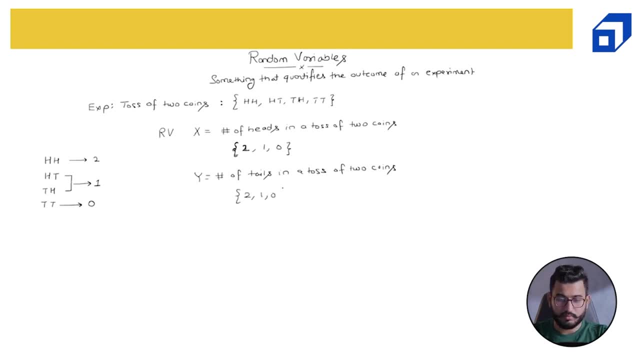 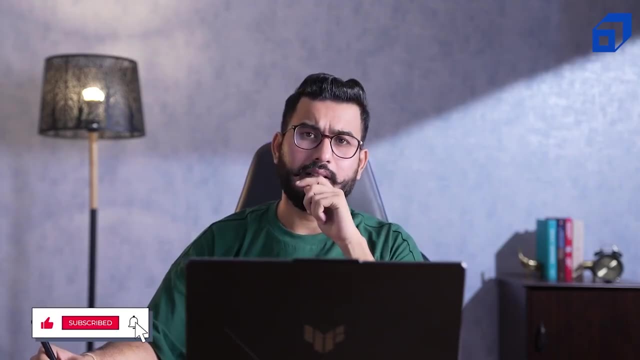 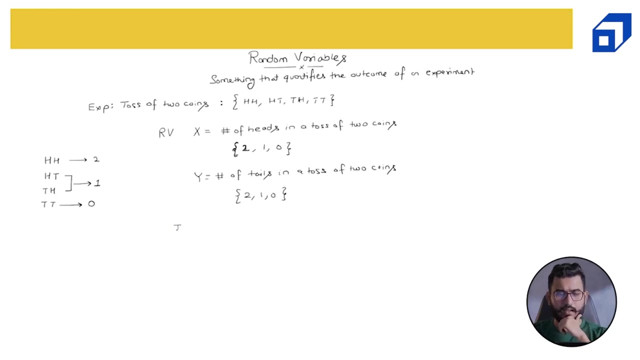 Y will also represent two, one, zero, right. I can have two tails, one tail or zero tail. I can also have a random variable, X, which is two tails, one tail or zero tail. I can also have a random variable where I, where I have taken a random number. for example, let's say I have stated that if you get so, 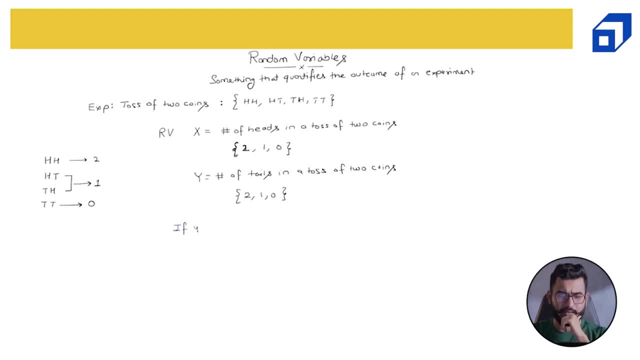 there is a game, let's say, there is a game which says: if you get two heads, I will give you ten rupees. so you know, you win ten rupees, you win ten rupees for any other outcome, for any other outcome you have to give me. you have to give me five rupees, so you pay five barrel. 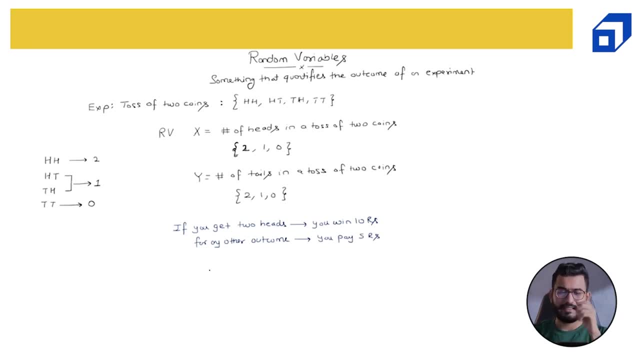 piece. now, in this case, let's say I am interested in the amount I can win, so X is my random variable. X represents the amount or the hour, the total price for the amount or the taste of everyone can win, and it can either be 10 rupees, so I like plus 10 because it is a, it is a gain for me. so 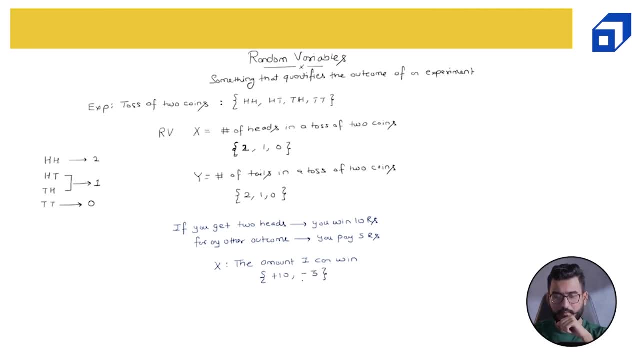 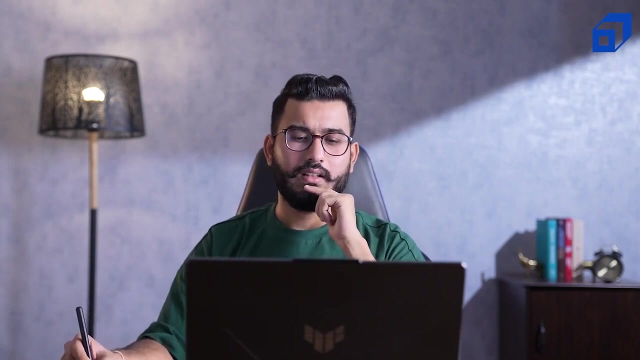 plus 10 and minus 5, because minus 5 represents loss. so here what I have done. if my experiment is having these four outcomes, then this is mapped to plus 10 and all of them are mapped to minus 5. this is also a valid random variable. now, random variables are essentially divided into: 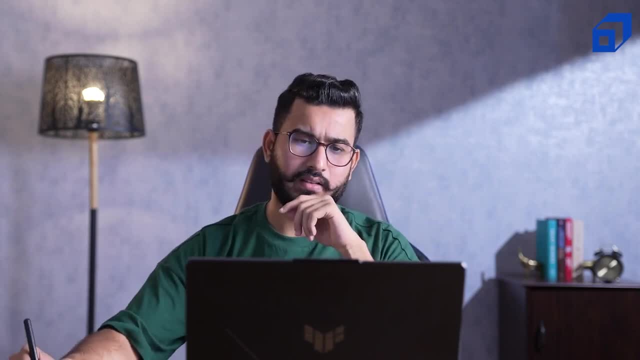 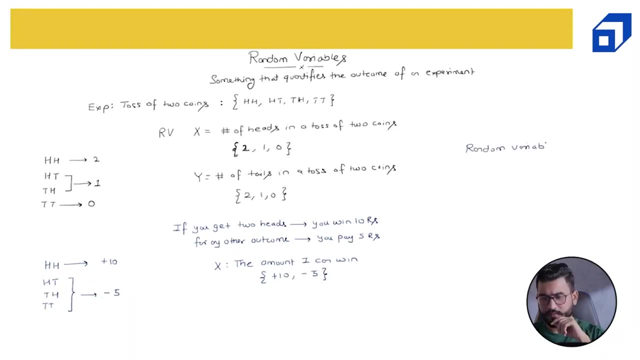 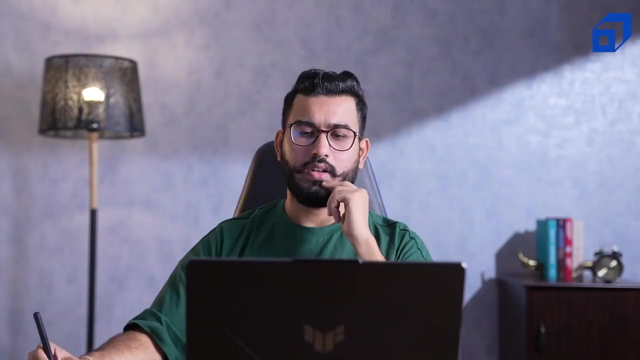 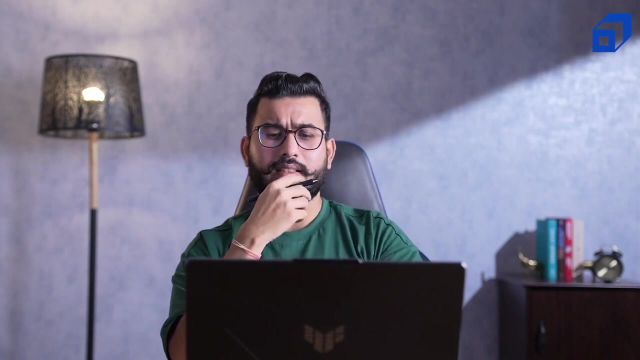 two categories: a random variable can either be a random variable or a random variable, or a random variable can either be discrete or it can either be continuous. Now, what is discrete random variable, or what are the discrete random variables? Well, discrete random variables are those variables for which the outcome can be quantified. 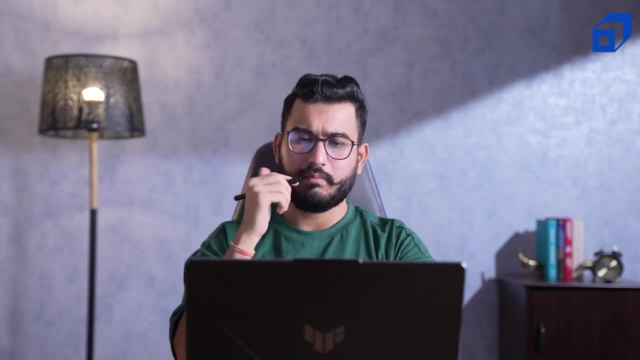 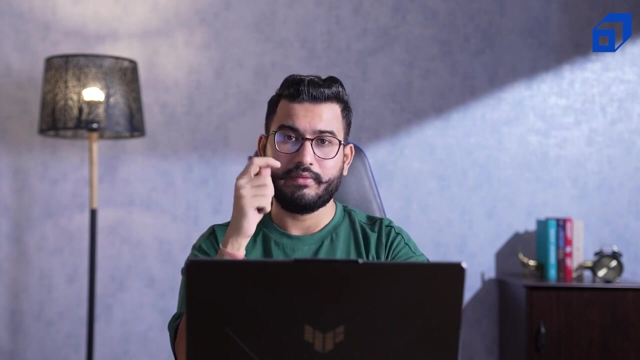 into integers which are countable, For example, number of heads in a toss of two coins. I know it can be either 0,, it can be either 1,, it can be either 2.. But if I ask you about you completing watching this video, 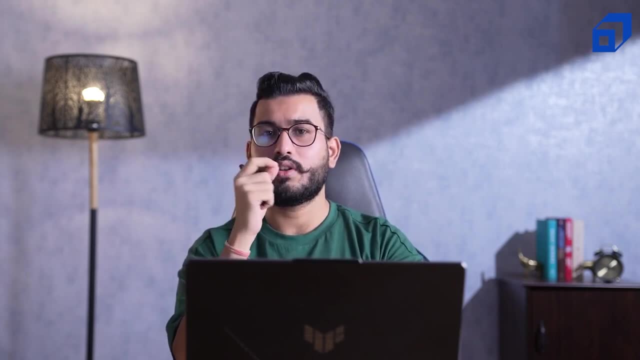 so how much time you will take to watch this video? Now, it can be anything from minus infinity to plus infinity. You can take 1 hour. you can take 1 hour 5 minutes. you can take 1 hour 5 minutes. 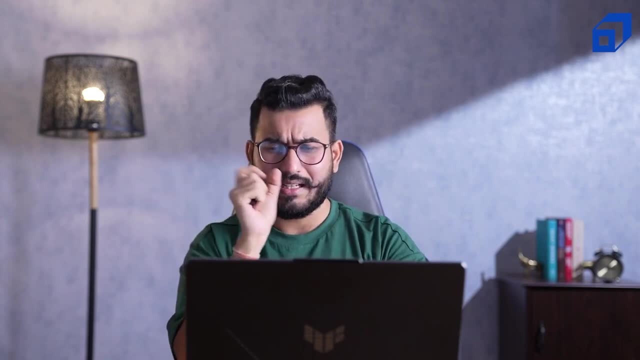 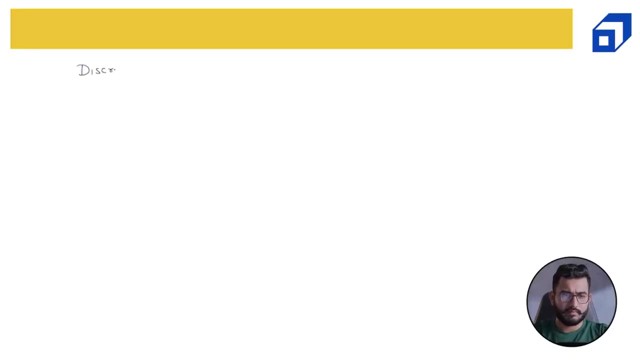 50 seconds. There are endless possibilities, right, Let's take a simple example. Let me just go to our next page For discrete. first of all, we'll take example For discrete: random variable, the outcome, the outcome are mapped to. 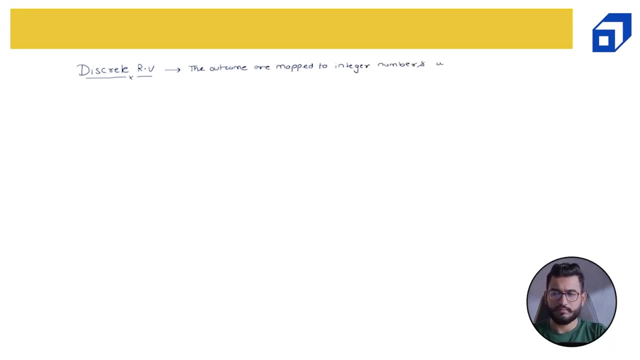 integer numbers Which are countable. We can simply count them. For example, number of heads in a toss of two coins. Or let's take one more example. Let's say there is a person who is trying to shoot a particular target. 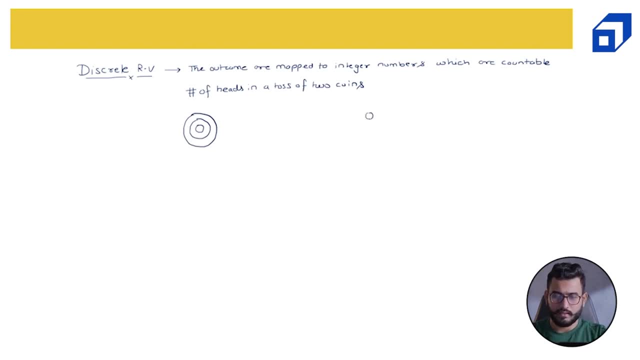 Let's say there is a person who is trying to shoot a particular target. So this is my target. Here I'm having the person And this person is trying to shoot the target. So here is the target. Now let's say this person is trying for 10 times. 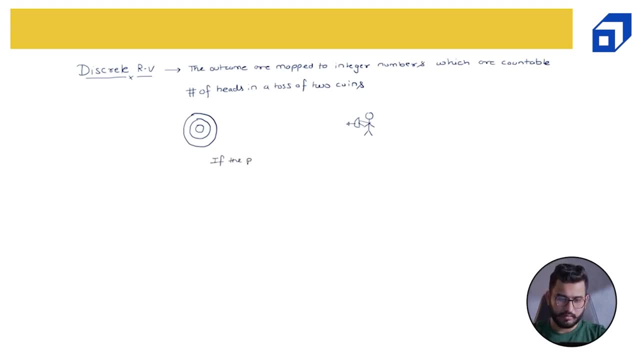 So if the person tries to shoot the target, So if the person tries to shoot the target for 10 times, then what can be my random variable? My random variable can be the number of times the person hits the bull's eye. 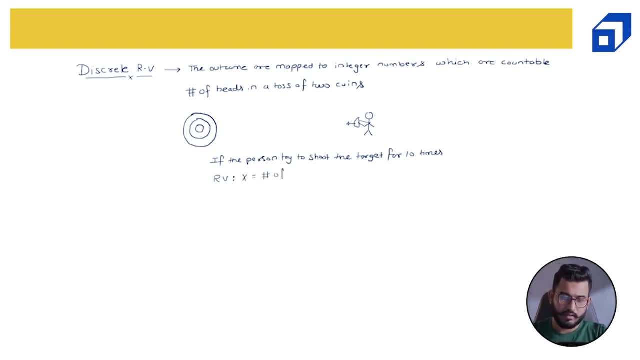 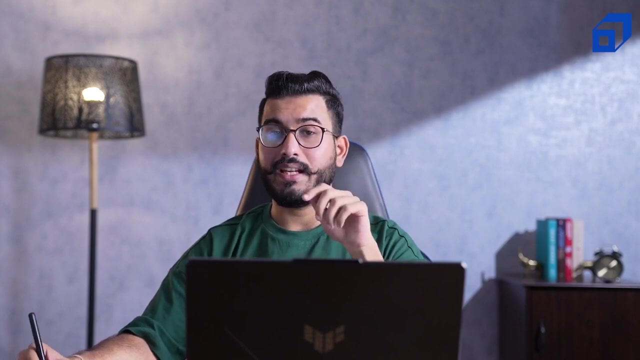 So my random variable, x can be number of times the person hits the bull's eye. Now, Now, if you closely observe, Now, if you closely observe, this can be. this can only take this random variable can only take integer numbers. 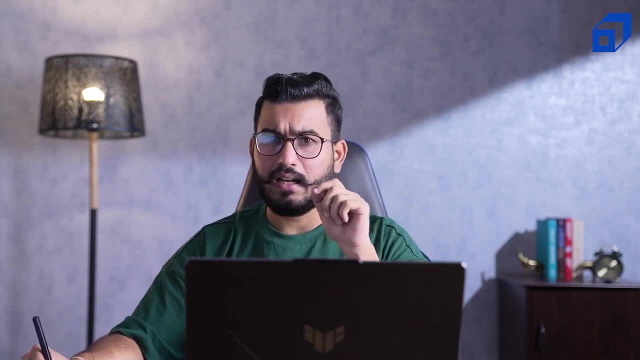 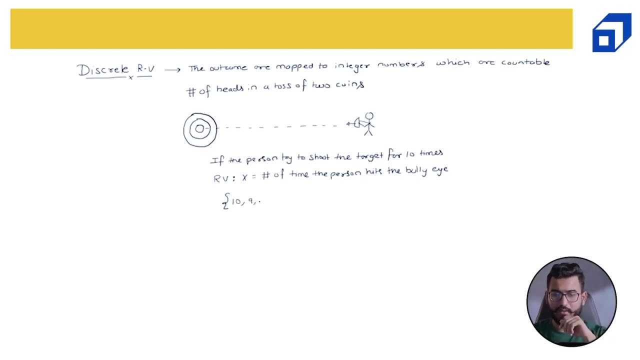 So I can only get. So. the person can either hit the target or hit the bull's eye for all the 10 times, maybe for 9 times, for 8 times, for 7,, 6,, 5,, 4,. 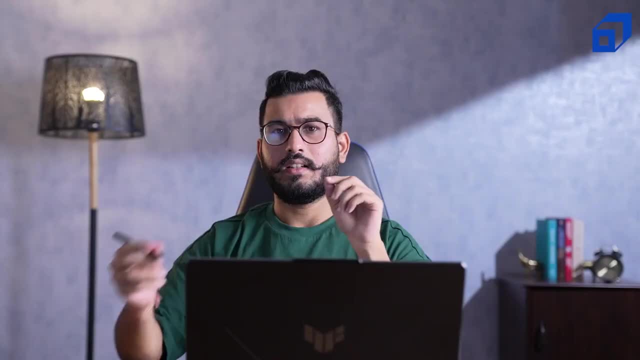 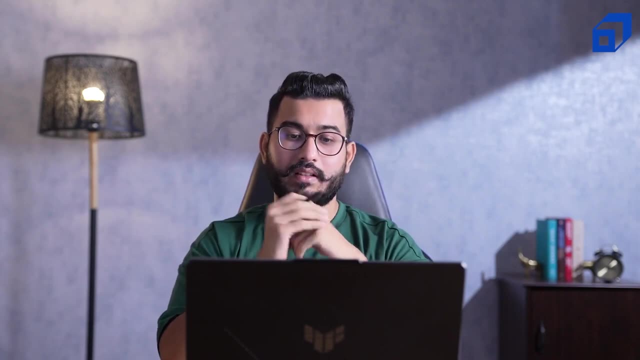 3, 2, 0.. 0 means the person was not able to hit the target for any time. This is my discrete random variable. Can this variable take any value other than all these possibilities that I have written? Can the random variable x that you can see on your screen? 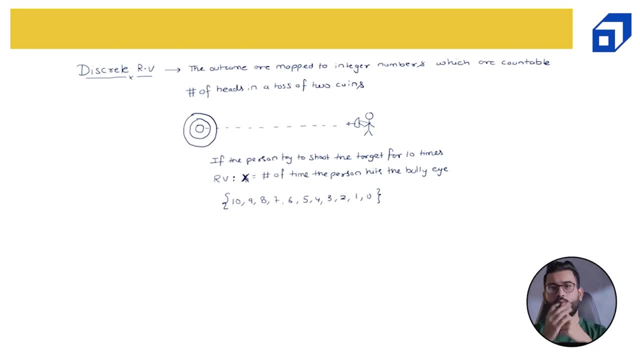 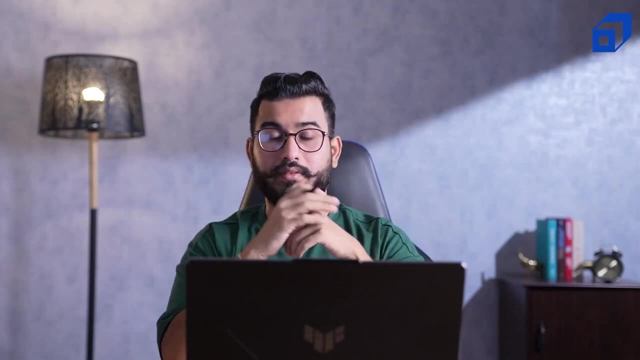 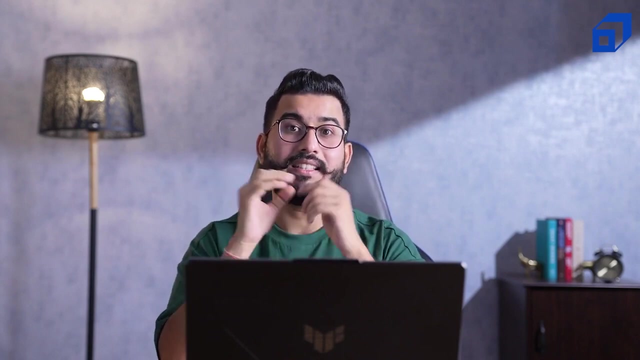 Can this variable take 1.7?? No, It cannot take 1.7.. Similarly, this random variable cannot take 10.5 or maybe 9.11.. So it can only take these limited numbers. So this is why this is known as a discrete random variable. 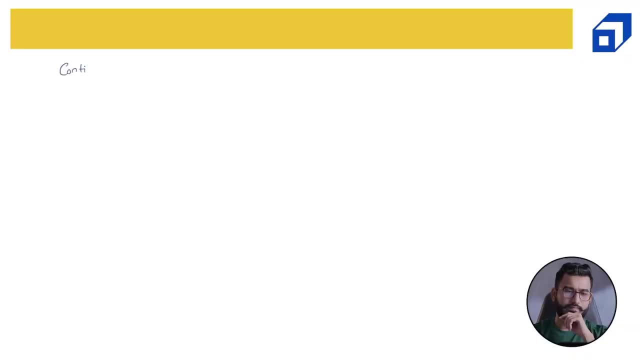 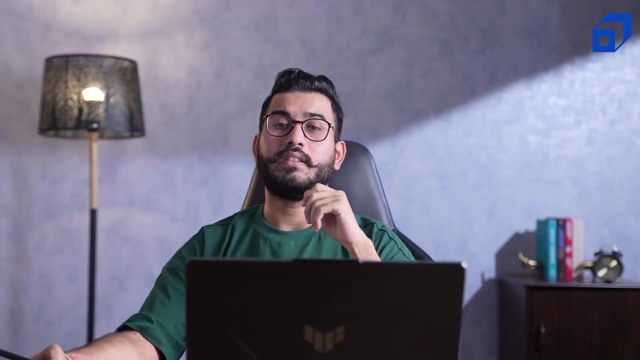 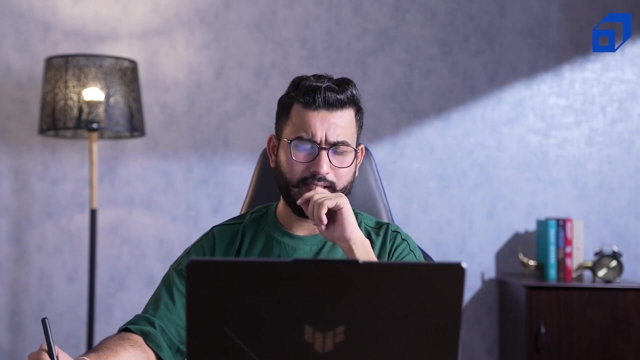 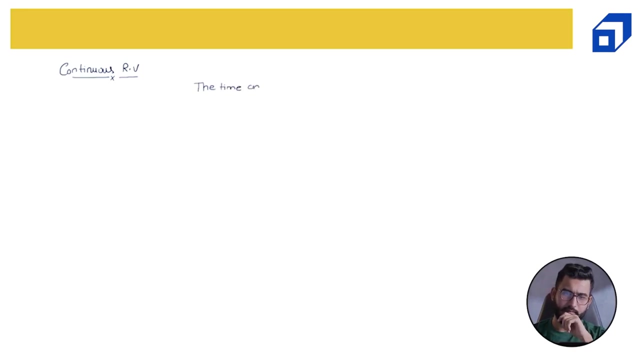 Let's talk about continuous random variable. Now, continuous random variable can take many values. The outcome are many possibilities. So, for example- let's take first of all an example- The time an employee takes to commute from home to office. Now this is my random variable x. 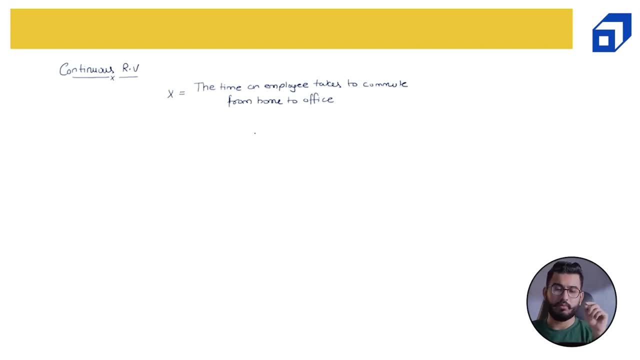 The time an employee takes to commute from home to office. Now, this can be anything. Let's say we have defined a range. Minimum is the person minimum takes 10 minutes. Maximum is, let's say, 1 hour. Or let's say we will keep the scale in minutes itself. 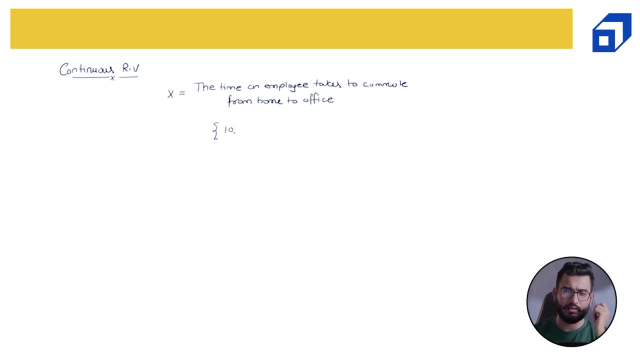 So we have written 10 minutes, So this is 10 minutes And the maximum is 60 minutes. Now, between these two minimum and maximum, between this range, I can have endless numbers, Endless Right. There can not be a particular point. 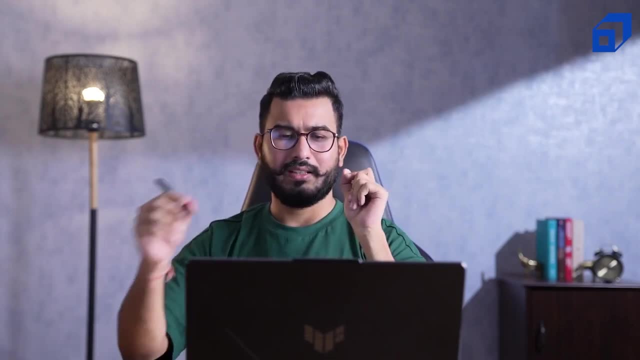 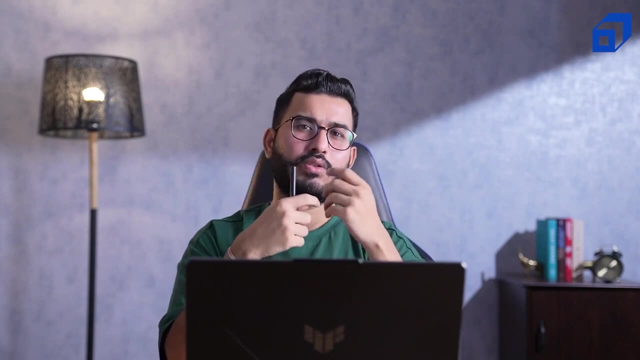 that I can pinpoint. I cannot say the person would take 10 minutes, 5 seconds, 3 milliseconds, 2 nanoseconds. It can be endless possibilities, right? So this kind of random variable is known as the continuous random variable. 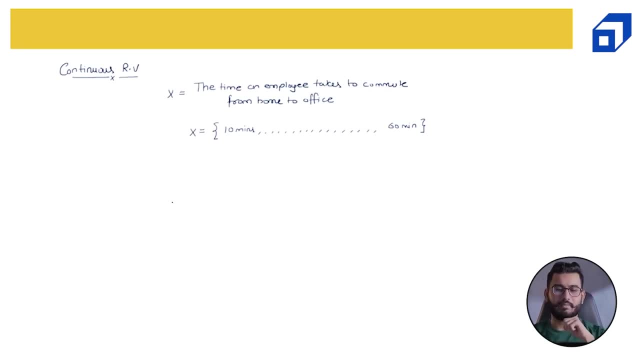 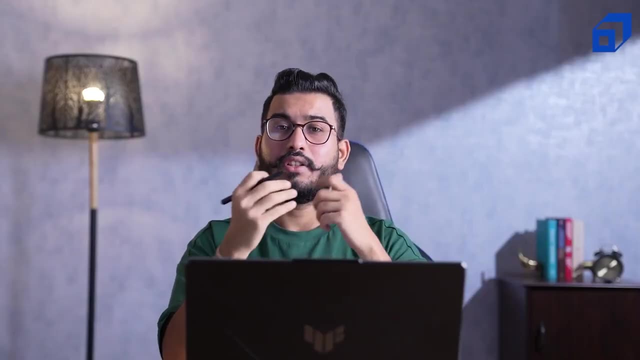 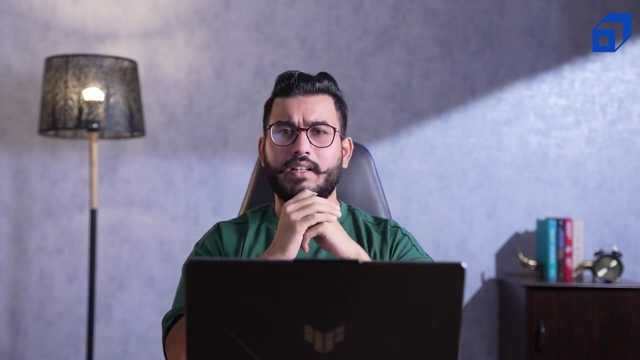 So here x represents my continuous random variable. When I talk about discrete random variables, there are some properties and distributions associated with them. Similarly for continuous random variable, the reason we are talking about it is because we wanted to generalize them. 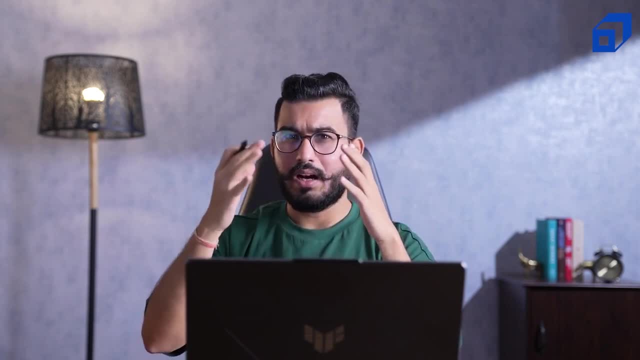 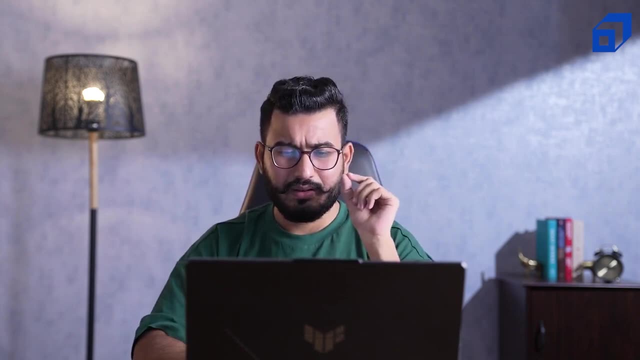 I will talk more about them. I will talk more about how we can generate a distribution out of them, But before that, let's briefly talk about a very important topic known as expected value, And we will take this example to calculate the expected value. 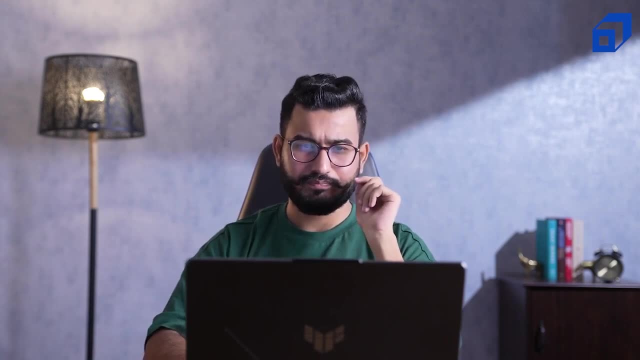 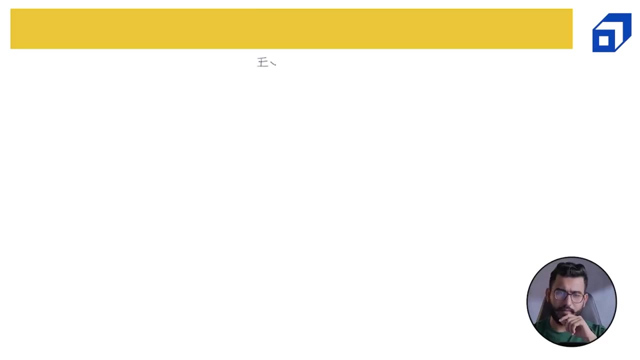 What is the expected value? So I am just taking a topic out of the random variable to talk briefly about expected value And then we will jump to distributions. So expected values. Now, when we talk about expected values, it is basically the average value of the random variable. 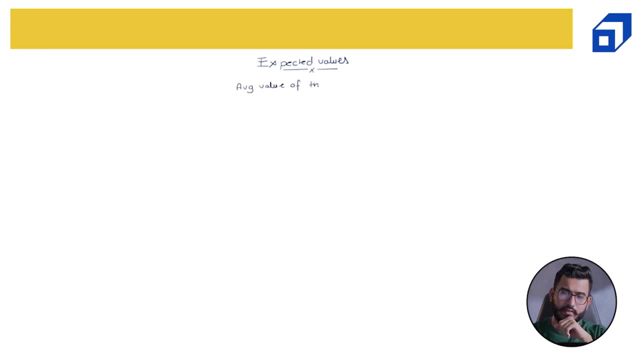 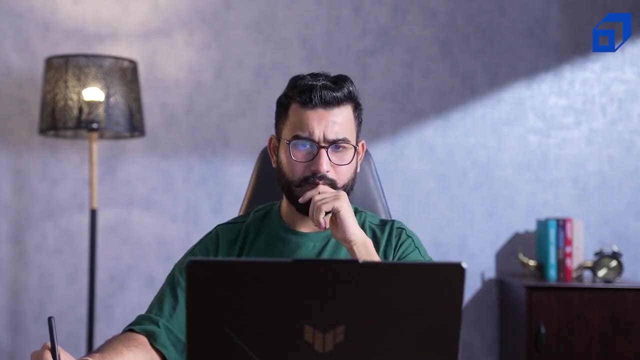 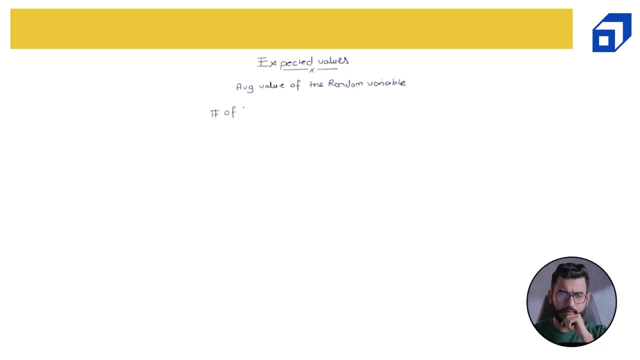 Average value of the random variable. Now let's say I am taking one example. Let's say the number of heads, The number of heads in a toss of two coins. Now this is my random variable x, And this random variable can take. 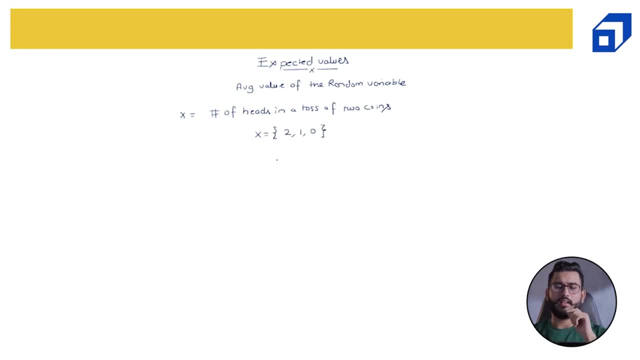 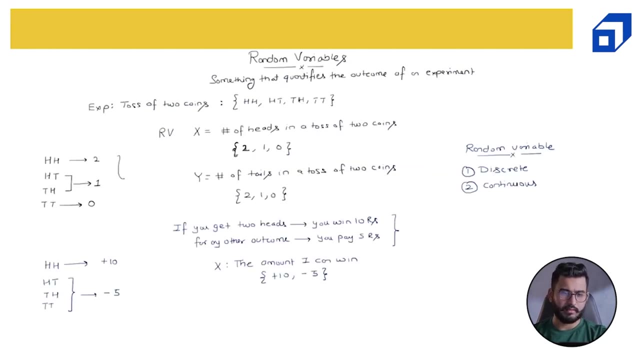 2, 1 and 0. So either I can get 2 heads, 1 head or 0 head. I have already shown you this. Please remember this. Now. what is the expected value of this random variable x? 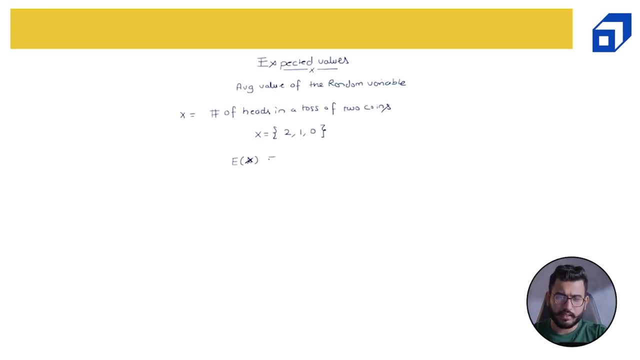 So what is the expected value of x? Expected value is nothing but given as summation of i over x, pi into x i. I would write it formally as x i into p. probability of x is equal to x i. What is the meaning of this? 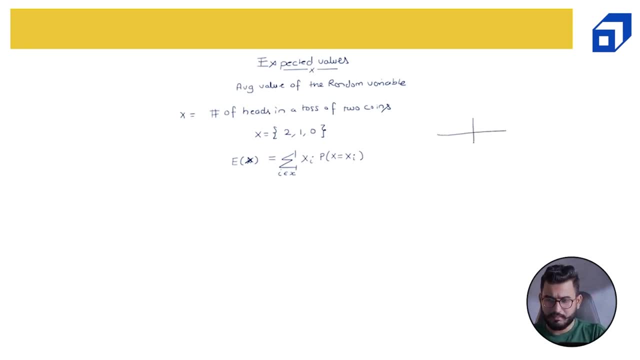 So let me just quickly create a table with the random variable x and the probability of x. So random variable x, probability of x is equal to x- i, So the random variable can take value 2, 1 and 0.. 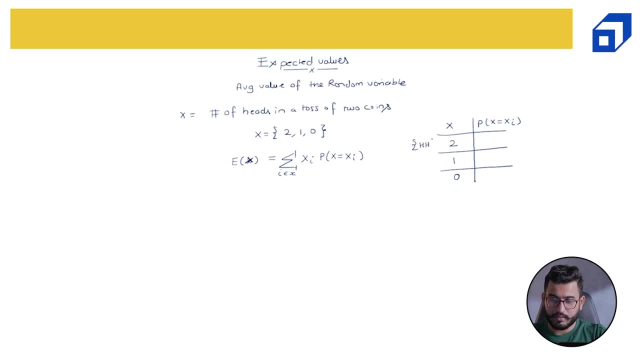 Now 2 can come out from this event: head-head. 1 is the event of head-tail and tail-head And 0 is the event of tail-tail. So the probability of getting 2 is 1 divided by 4.. 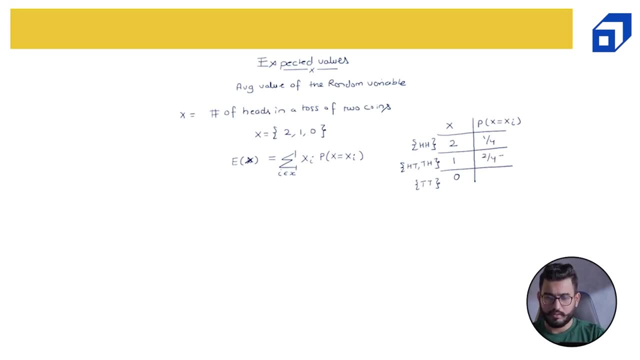 This is 2 divided by 4.. Which is eventually 1 divided by 2.. This is 1 divided by 4.. These are the probabilities. So the expected value of x is nothing but the random variable multiplied by the probability of that random variable. 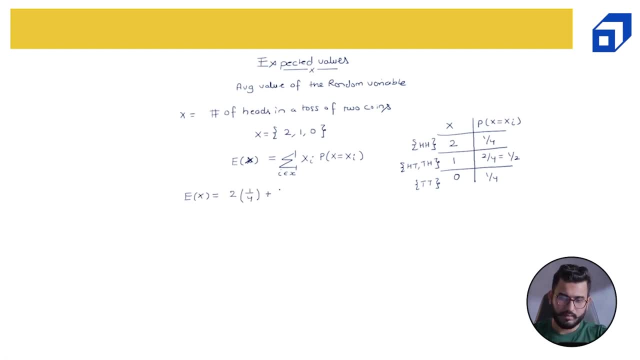 So 2 multiplied by 1 divided by 4 plus 1 multiplied by 1 divided by 2 plus 0 multiplied by 1 divided by 4.. So this will be 2 times. So I will get 1 divided by 2 plus. 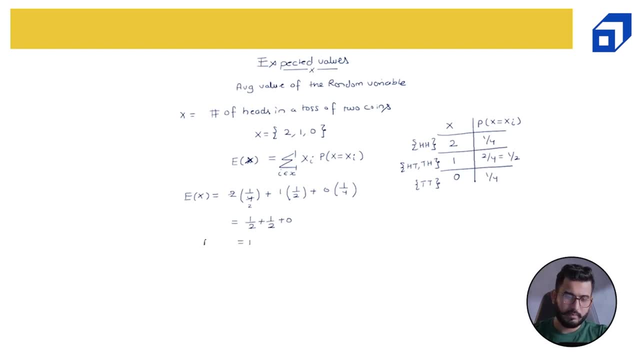 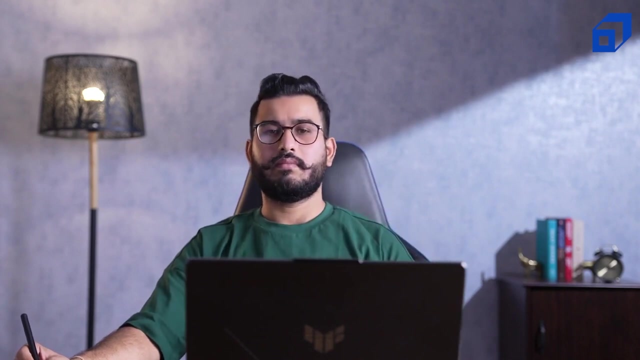 1 divided by 2, and this will be 0. So the answer is 1.. Expected value is 1.. What is the meaning of this? This means on a long run, if I perform this experiment, for very long time, if I keep on performing this experiment. 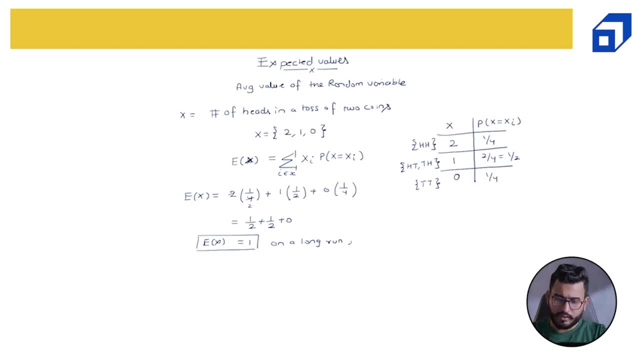 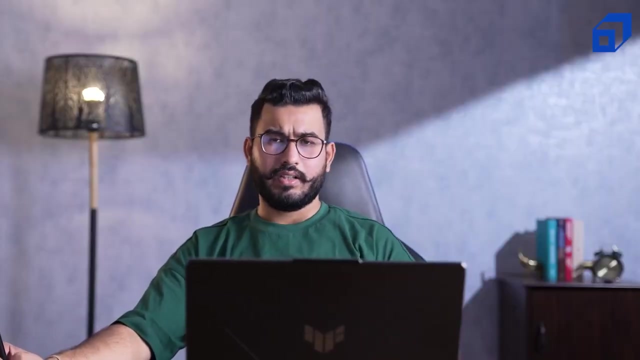 I am tossing 2 coins again and again on a long run. on an average, this experiment, this experiment, this experiment would result in 1 head. So, on a long run, you will observe that you are getting 1 head. This is the mean. 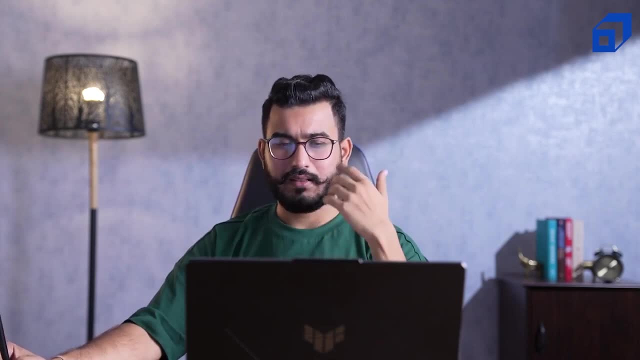 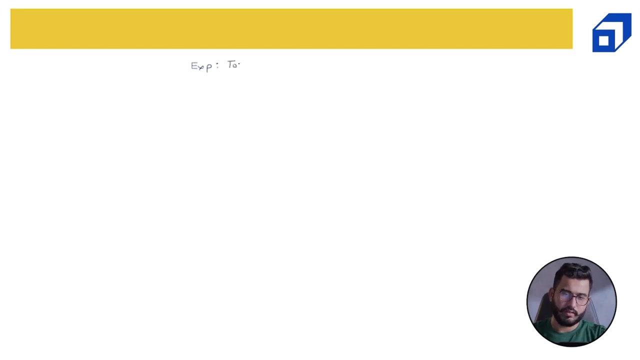 of this random variable. If this is not making sense, let's take an example in a game format, And then you will be able to connect with it. Let's say now I am having the same experiment. The experiment is toss of 2 coins. 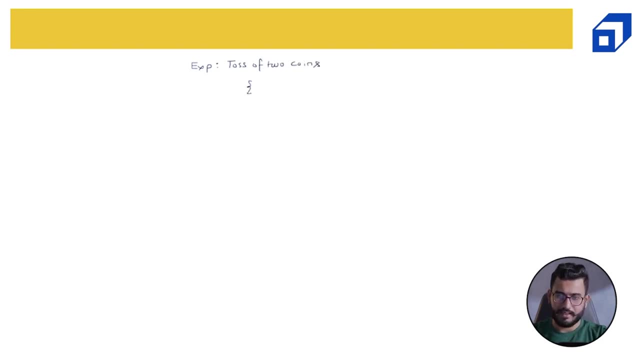 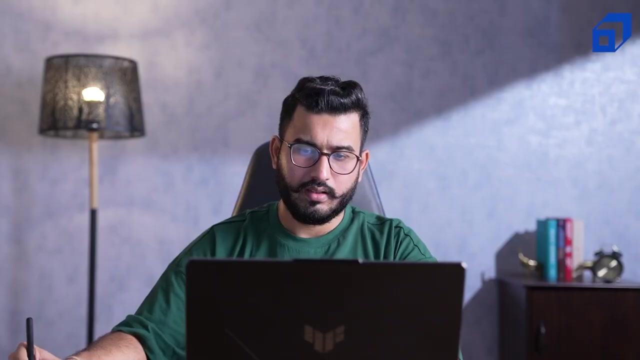 toss of 2 coins. I may either get head, head, head tail, tail, head and tail tail. Now we are mapping. so my random variable x is now the amount I can make, The amount I can win. The amount I can win, Let's say, 2 people are playing. 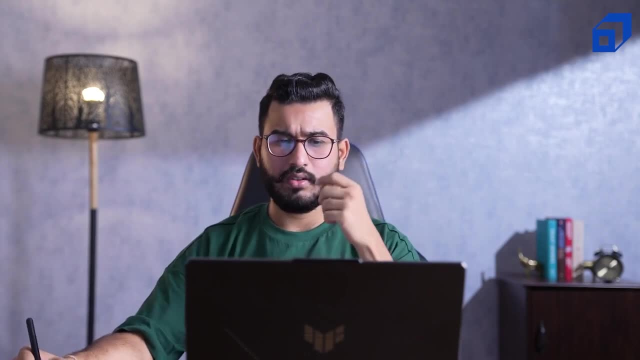 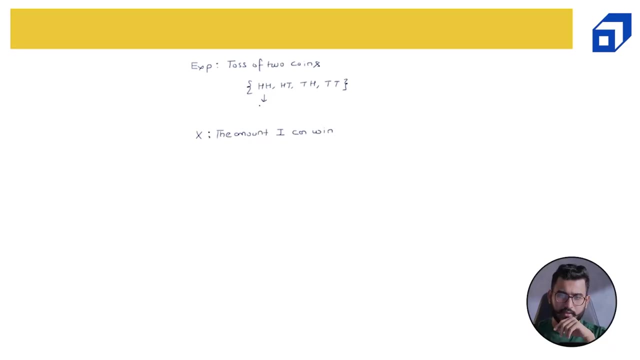 some game and the condition of this game is: if the person tossing 2 coins, or if the person tossing a coin for 2 times gets both of them are head, the person wins 10 rupees. For any other combination, the person has to pay 5 rupees. 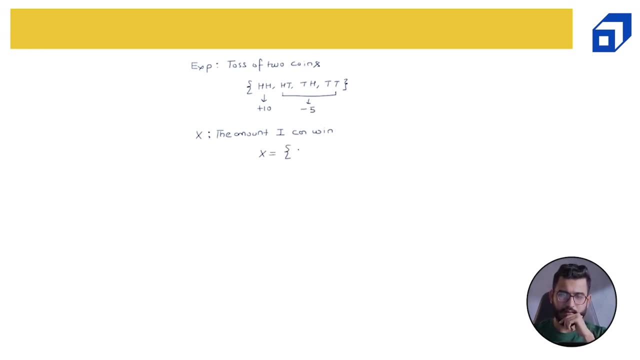 So the random variable x is plus 10 or minus 5.. Now I will quickly create a table. This is my random variable x i- This is the probability of x- is equal to x- i, So the person can win 10 rupees, so plus 10.. 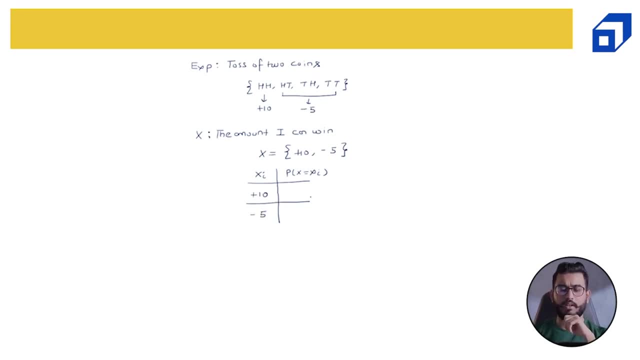 The person can lose 5 rupees, so minus 5.. What is the probability of winning 10 rupees? You can see the probability of winning 10 rupees plus 10 can only come when the person has obtained both head, which is 1 divided by 4.. 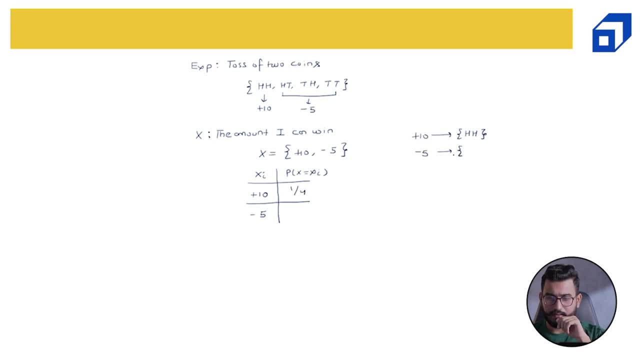 Probability of losing 5 rupees is getting either of the either of the event, which is head tail, tail, head and tail tail. So head, tail, tail, head and tail tail, And this is 3 divided by 4.. Now I will calculate. 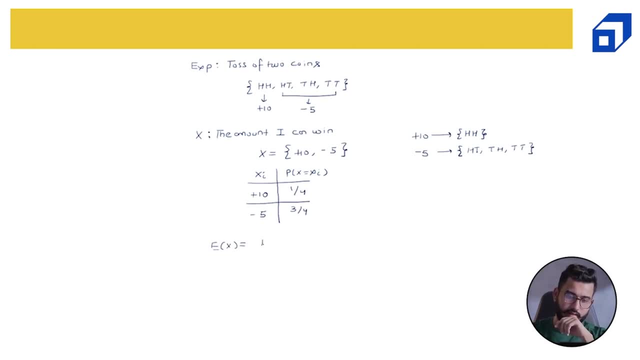 the expected value of x, which is 10: 1 divided by 4, plus minus 5, into 3 divided by 4.. Now this will be 2 times 2, 2 times 5.. This will be 5 divided by. 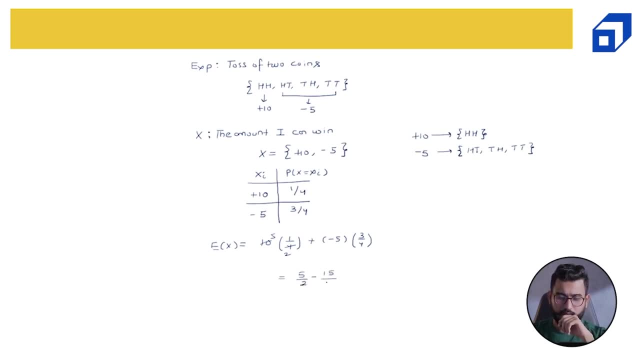 2 minus 15 divided by 4.. For easy calculation, let's keep them, let's, let's not cancel out the 4, because the numerator is denominator is both 4.. So I will get 10 divided by 4 minus 15 divided by 4.. 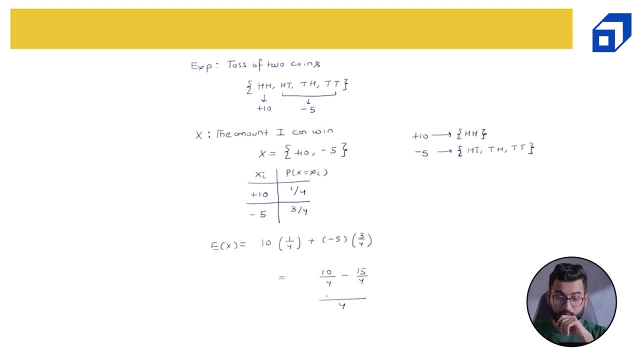 This would be denominator. denominator is 4.. 10 minus 15 is minus 5 by 4.. So minus 5 divided by 4, which is minus 1.25.. Now, what is the meaning of this value? This value basically mean: 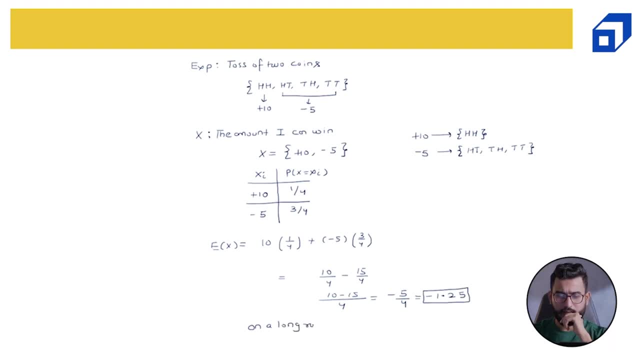 on a long run. if you play this game for very long time with your friend on a long run, on an average you would end up losing 1.25 rupees per game. So this is a loss for you. What was my random variable? 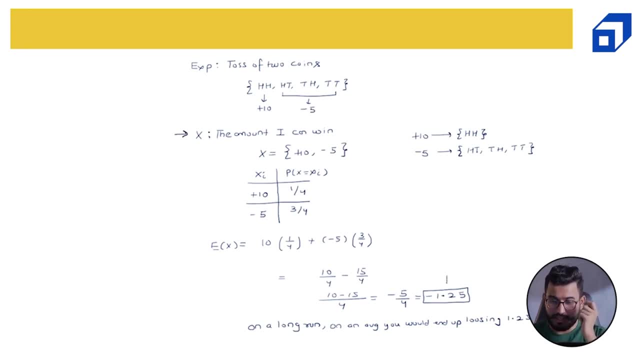 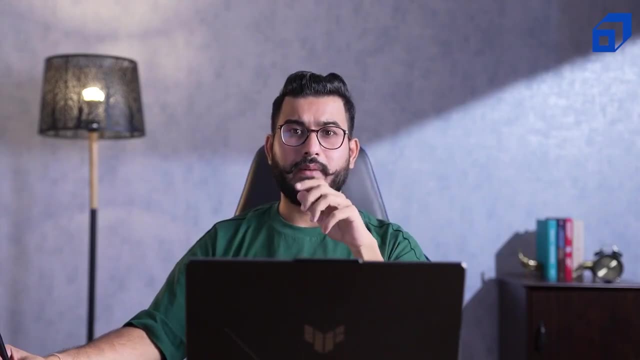 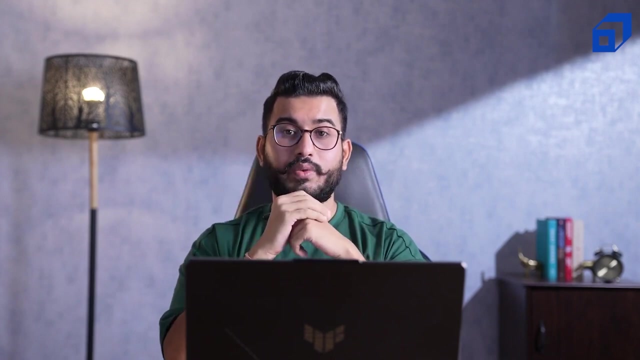 The amount I can win. the random variable ends up in a negative value, which is minus 1.25.. So on a long run, if you perform this experiment for a very long time and you play this game with your friend, then you will end up losing. 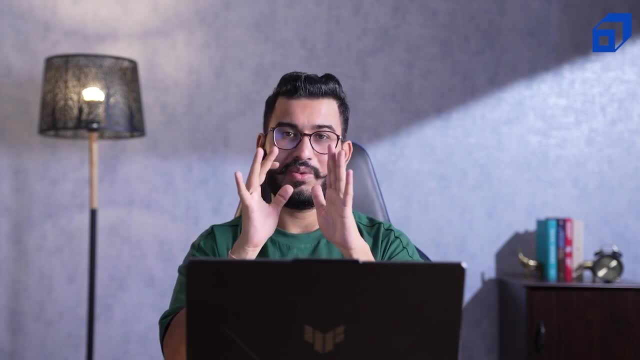 1.25 rupees per game, and that is what you should do. So when you are playing a game, please make sure the expected value should always turn out positive for you- and you would have heard about this term- the house always wins, Which basically means: 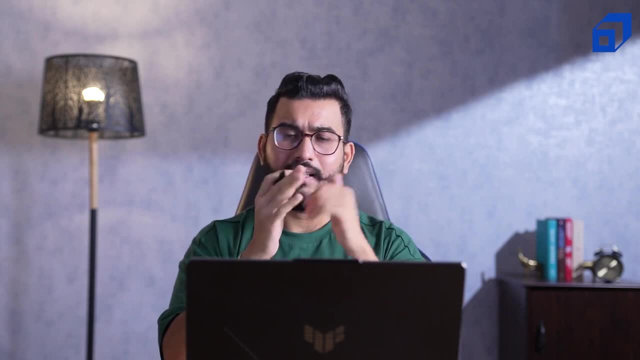 in gambling. whenever you go to any casino or any gambling house, they always win on the long run. So if so many people are playing the same game, some of them will win, while most of them will lose. So on a long run it is a profit for the. 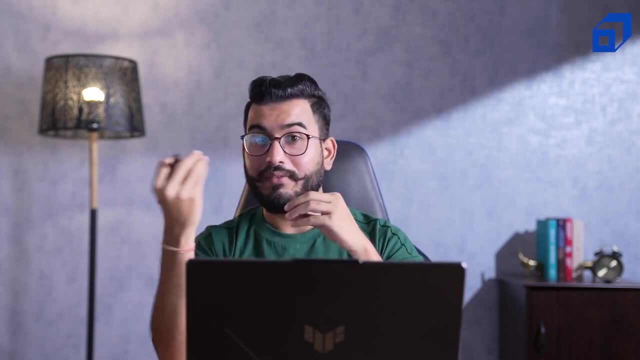 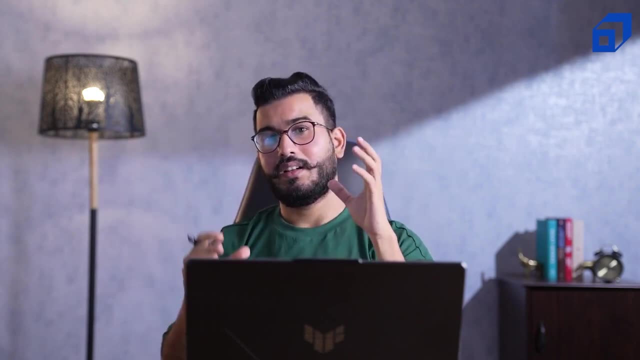 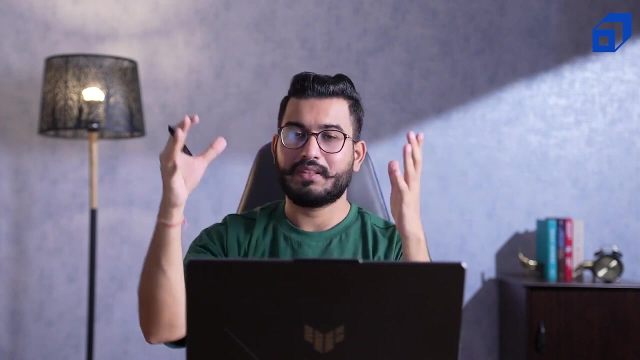 gambling house or for the casino. So some of them may win, but on a long run, when many people are playing the game in the casino, the house will always win, because their expected value is positive for them and negative for you, and all the games are made. 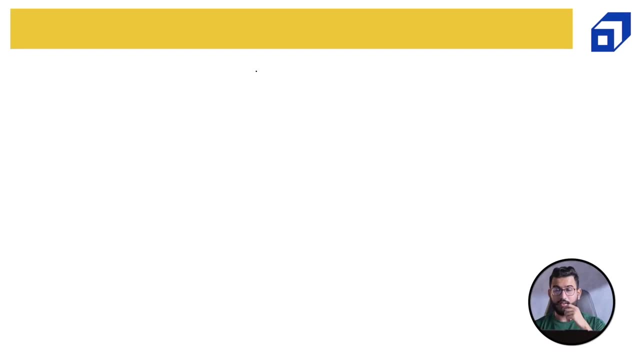 in such a way that the expected value is favorable to them. So now let's talk about distributions. What is distribution? So, when we have a random variable- I hope you already know a random variable can be of two types: either discrete or continuous. 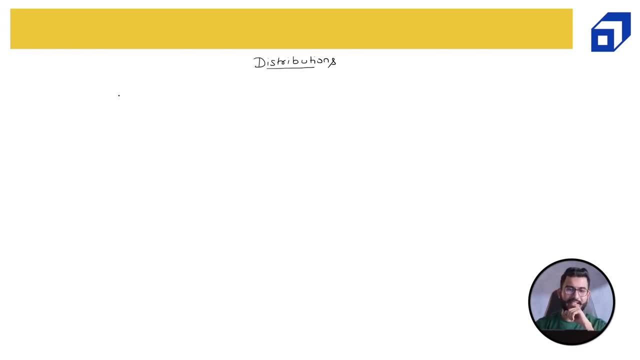 So let's say I am having a discrete, random variable and first of all we are talking about the distributions for discrete. I will take an example for both and then we will talk in detail about the variety of distributions we have. Distributions are very important. 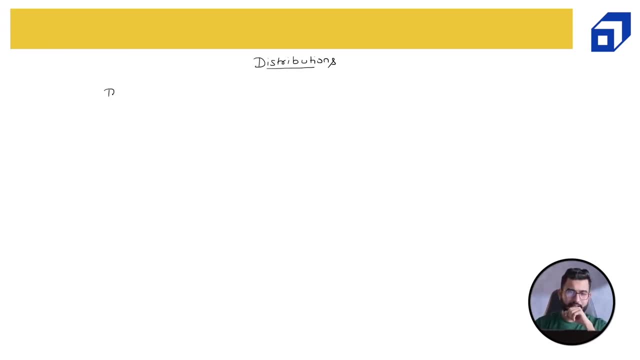 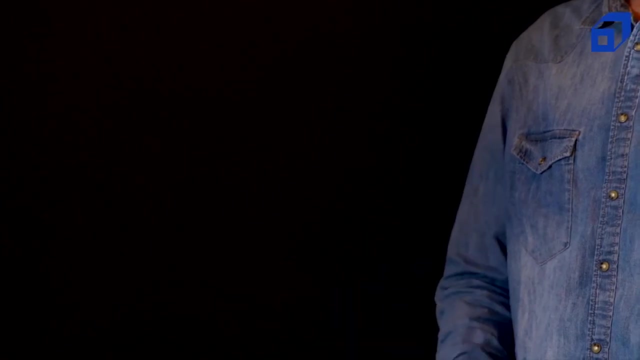 to understand the topic very carefully. So when we talk about discrete random variable, discrete random variable, we know that the outcome can be discrete, it can be integer. So let's take one example. let's take one experiment of two coins, and I have taken this experiment. 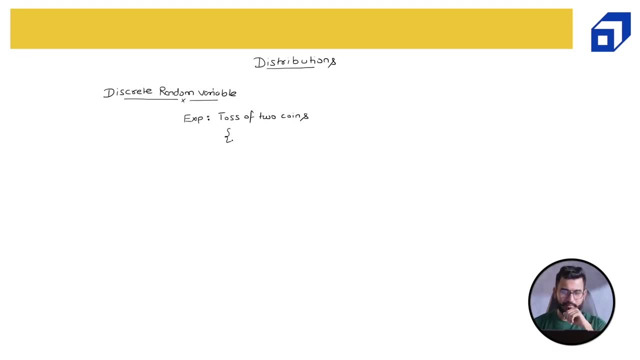 for so many times. So you already know that the outcome can be head-head, head-tail, tail-head and tail-tail right. The random variable can be: x can represent the number of heads, and it can be two head, one head or. 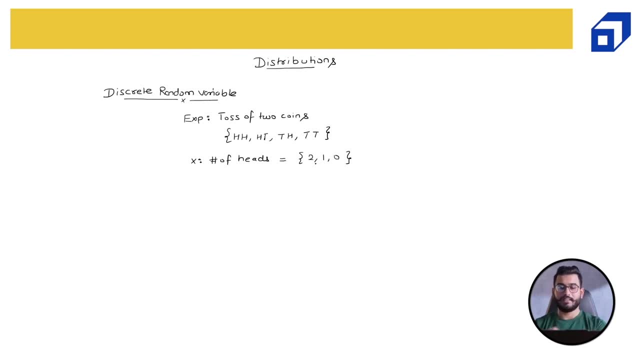 zero head Now if I plot this distribution. so I am having a plot in the x-axis, I am having the random variable and I already know this random variable can either take two: one or zero. Here I am having the count. So 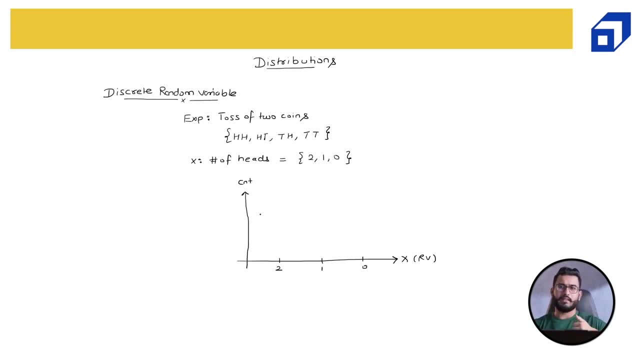 assume that you are performing this experiment of tossing two coins for many times and you have noted down the number of times you obtained two heads, the number of times you obtained one head, the number of times you obtained, let's say, no head. So let's say: 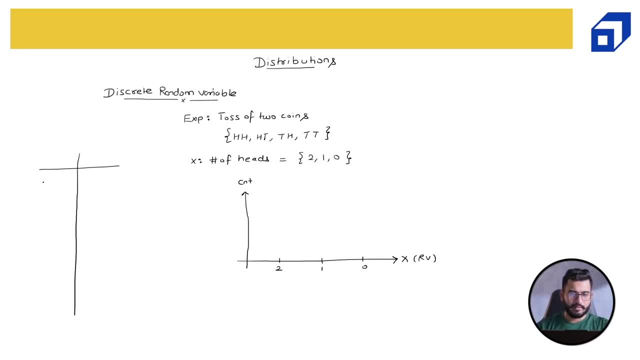 I am creating a table and let's say so, this is my trial number one, so I will write one over here. in the trial number one, you obtained head-head, so here I will write two. In trial number two, you obtained head-tail, so one. 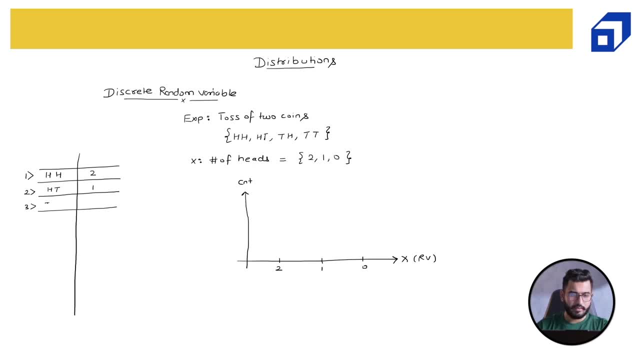 In trial number three you obtained tail-head, so again one. In trial number four: you obtained tail-tail, so again zero. In trial number five: you obtained tail-head, so one. In trial number six: you obtained tail-head, again one. Seven. 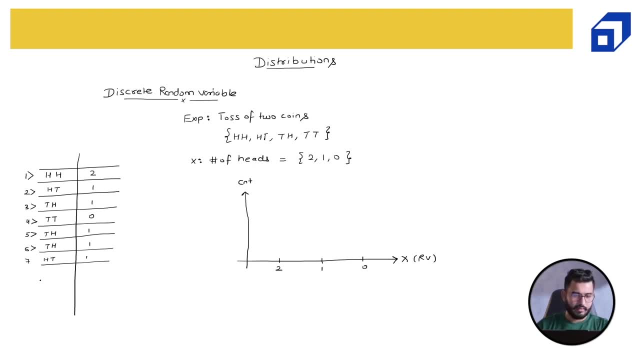 you obtained head-tail, so one. Eight you obtained head-head, so two. In trial number nine, you obtained tail-tail, so zero. In trial number ten, you obtained tail-head, so again one. Now this is my outcome, or random variable x. 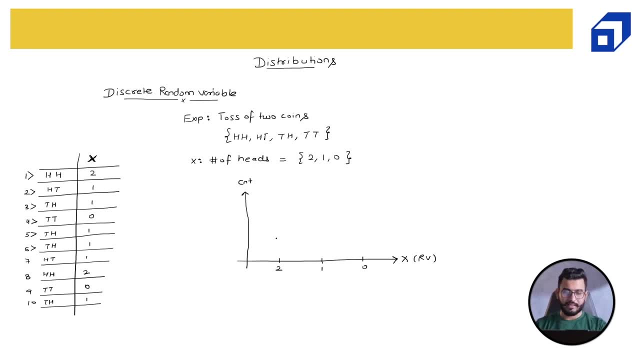 Now I will just count and create a plot. So how many times I have obtained two heads? So one time, two times. So I will assume that this is one, this is two, this is three, and so on. So for two times I have obtained. 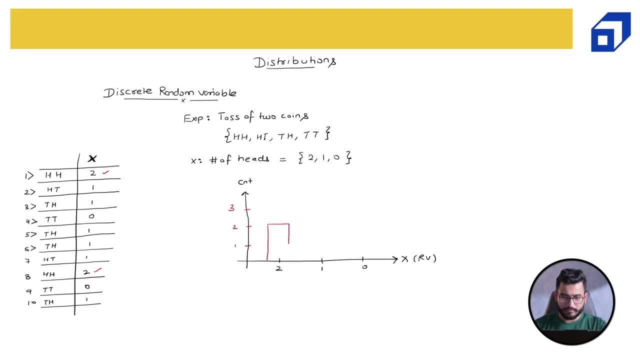 head-head, So I will create a bar over here. Then how many times I have obtained one head, So one time, two time, three time, four time, five time, six time, So six time, let's say represents like this: 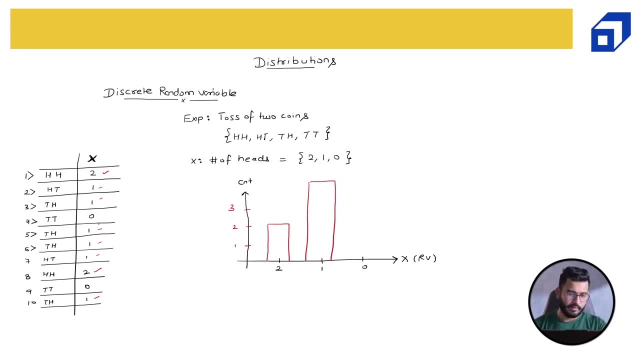 And then how many times I have obtained no head. So zero and zero, So two times. This is known as the distribution of discrete random variable and we have a very good name for this distribution, known as the PMF. This is PMF. This is known as the. 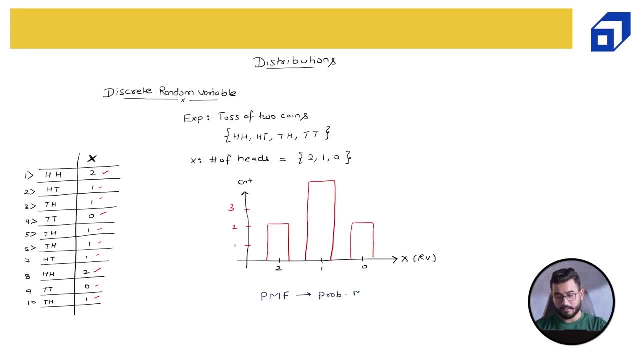 probability mass function. This is the probability mass function. Now, please remember this, that if I am tossing one coin, So let's say if I am just tossing one coin, and we have already created this probability mass function. I hope you remember. I have shown. 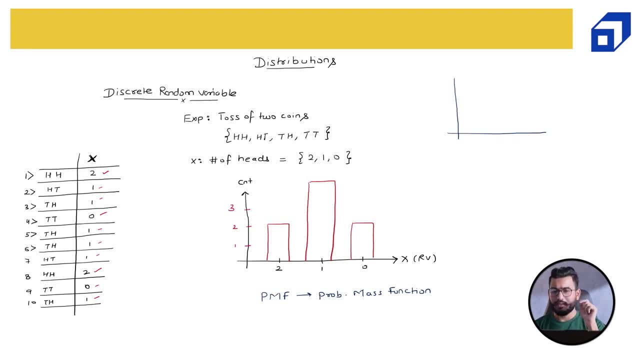 you one website, scene-theoryedu. In that website you have seen that for the true probability. So the true probability of getting head and tail when you toss one coin is half and half, One divided by two and one divided by two. The probability of mass function of 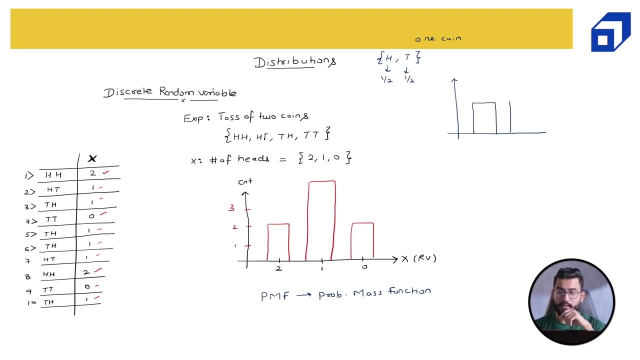 the true probability when you toss one coin will be 0.5, 0.5.. So this is head, this is tail: 0.5, 0.5.. But when you actually perform the experiment, this can change, This can be. 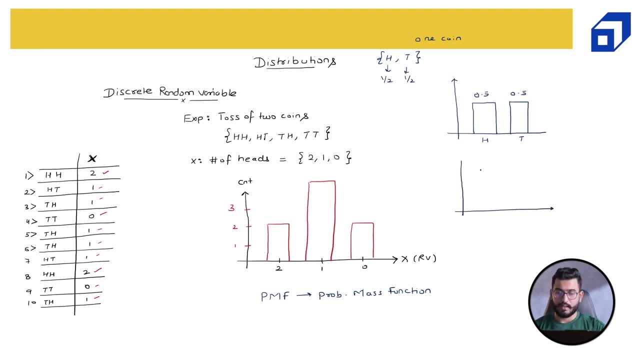 anything This can be. let's say I am having more head and less tail. Let's say this is 0.7,, this is 0.3, when you tossed one coin for 10 times, So 7 times, you obtain head. 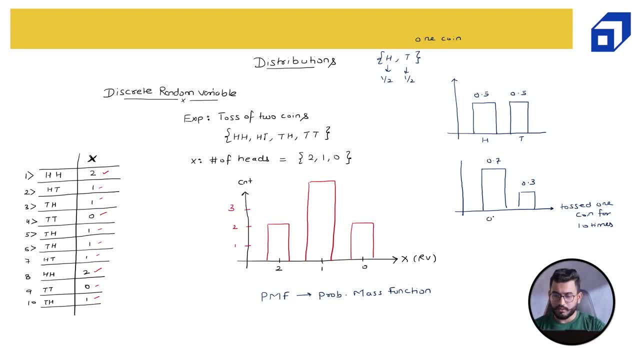 3 times you obtain tail Quite possible right. This is known as the observed. This is known as observed. This is known as true. Similarly, for this example: the true. So what is the probability of getting two heads? It is 1 by 4.. 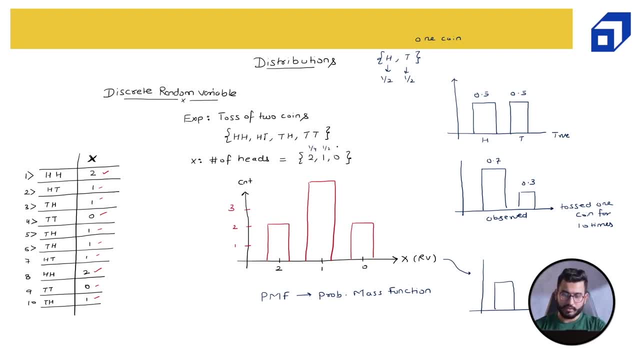 Probability of getting one head: it is 1 by 2.. Probability of getting zero head: it is 1 by 4.. How? Because I have mapped them. Please remember this probability is 1 by 4.. Probability of one head will be 1 by 4 plus 1 by 4. 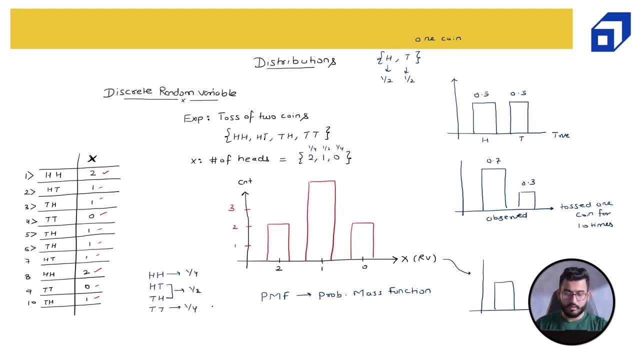 which is 1 by 2, and this will be again 1 by 4.. So the true PMF for this would look something like this, Where this would be 1 by 4, which is 0.25, 0.5. 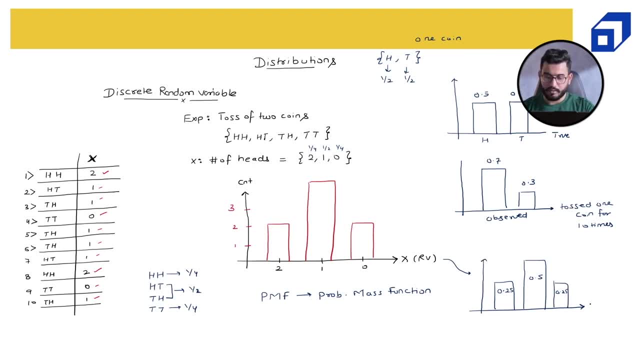 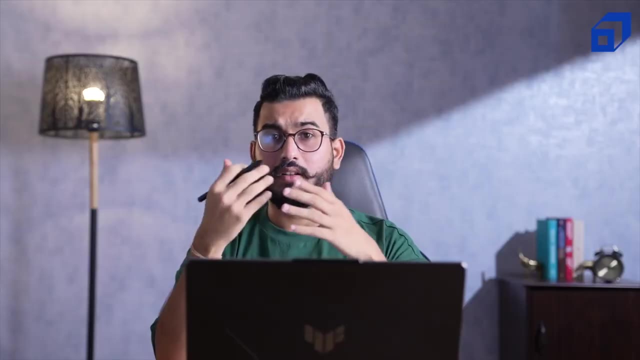 and again 0.25.. This is the probability PMF for my random variable X, which is a true, true probability. This is the PMF. This is for the discrete random variable. Now let's talk about the continuous random variable and how the distribution looks like. 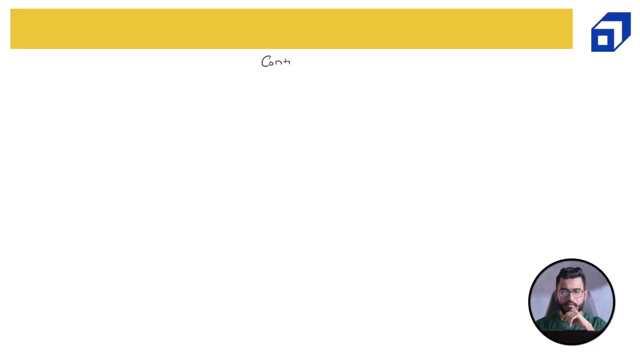 For continuous random variable. if you guys carefully try to understand the continuous random variable, we cannot have the discrete type values or integer values. but we can have range also. We can have range right. For example, let's say the random variable is times an employee. 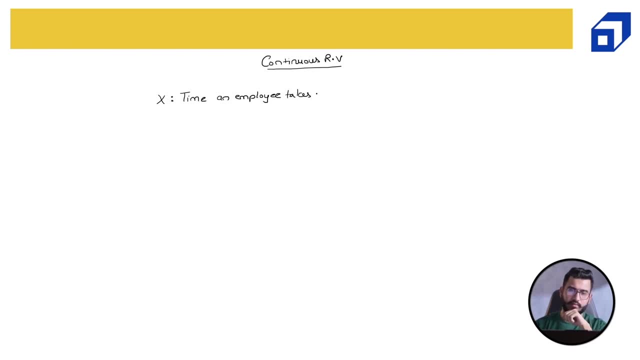 takes to commute between home and office. Now let's say we have defined the minimum and the maximum range. Let's say: minimum, the person takes 10 minutes. maximum, the person takes 60 minutes. Now I can have endless possibilities between these two numbers, right? 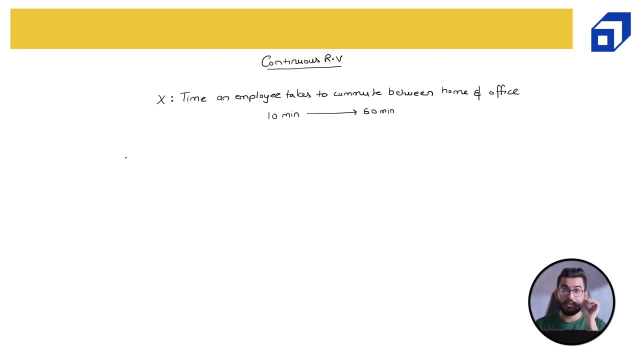 Let's say we have observed this. So let's say I have taken one employee. or let's say I have taken myself, and every day I am just taking down the number of minutes I took. So let's create a set over here. 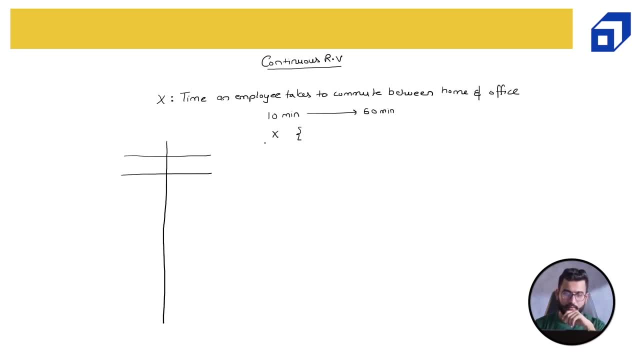 This is my observed set for X. So X observed set. The observed set for X is, let's say, in the first day I took 11 minutes. second day I took 32 minutes. then let's say 23 minutes. then let's say: 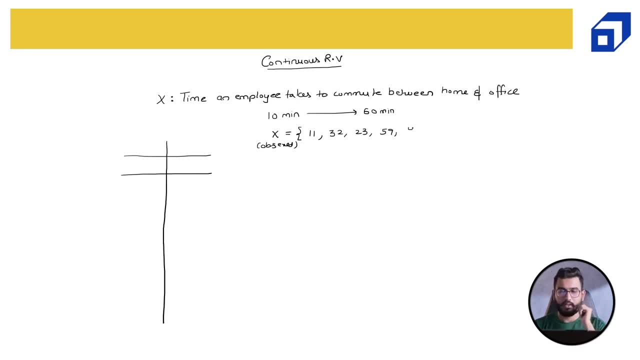 59 minutes, then let's say 43 minutes, then let's say 29,, 33,, 48,, 57, and 12.. So 1,, 2,, 3,, 4,, 5,, 6,. 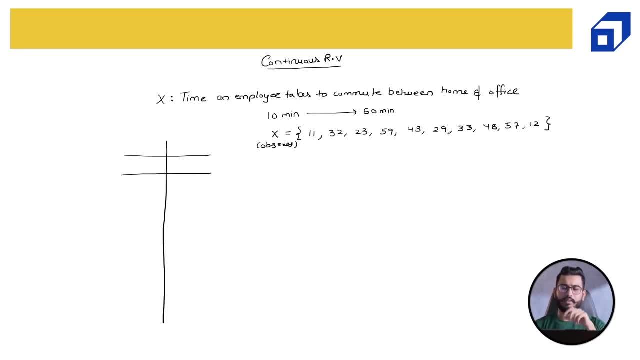 7,, 8,, 9,, 10.. For 10 days I observed the number of minutes I took. Now can I take each of them as a random variable? No, Because this is a continuous random variable. So my question to all of you: 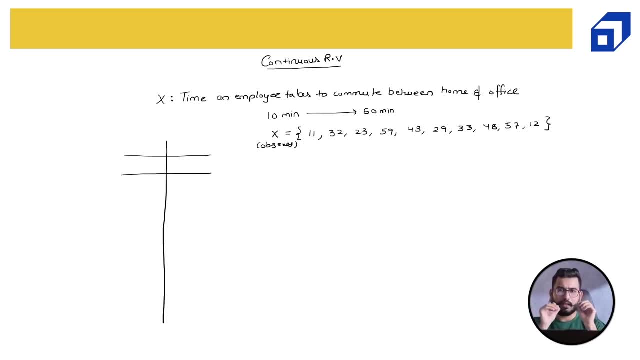 is that: are these the only possible outcomes which I can get from this experiment? No, We can have more outcomes. If I perform this experiment for another 10 days, I can get more values, Let's say some day. I took 23 minutes 2 seconds, So 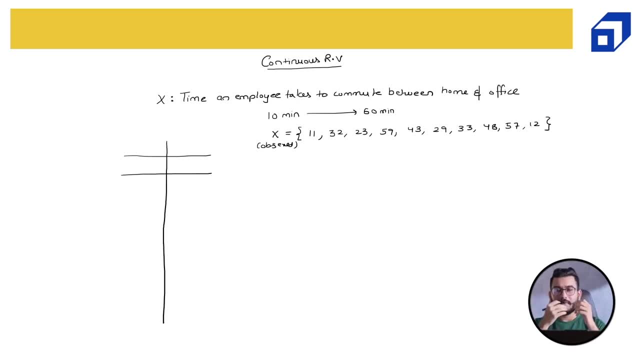 23.2.. Let's say some day, I took 11 minutes and 5 seconds, So there are endless possibilities, So I cannot take each entry or each outcome over here as one random variable. Then what is the solution? I would go with the rain. 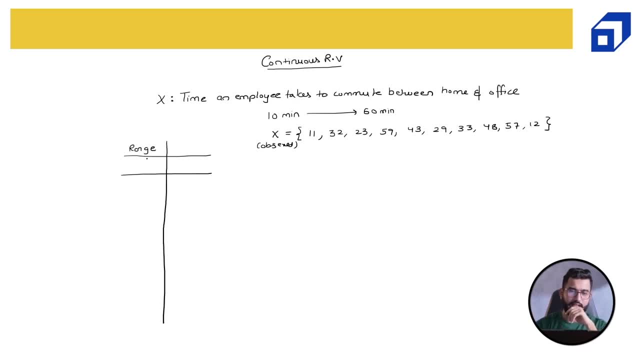 So let's define the range over here. So range would be, let's say, from 10 to 15,, 15 to 20,, 20 to 25,, 25 to 30,, 30 to 35,, 35 to. 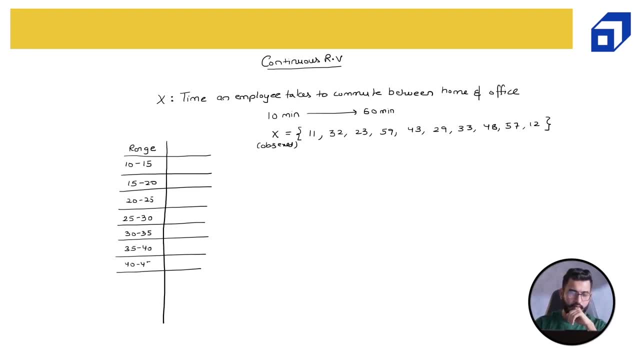 40,, 40 to 45,, 45 to 50,, 50 to 55, and finally 55 to 60. And I will now just write down number of times I observed a value between this range or in this range. 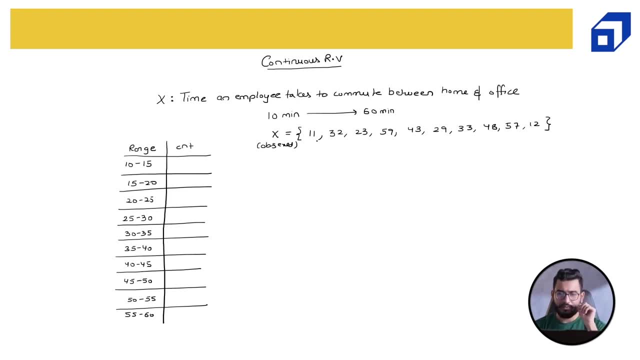 So let's write the count. So in between 10 to 15, I was having this value which is 11 and 12. So I write 2 over here Between 15 to 20, I don't have a value. 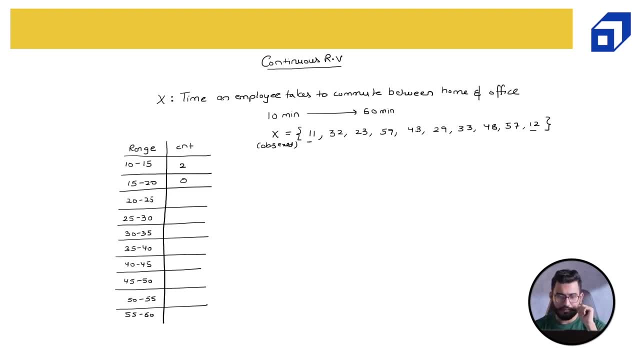 between 0.. 20 to 25,. 20 to 25, I am having 1 value, so I write 1 over here. 25 to 30,. 25 to 30, I am having 1 value, so I. 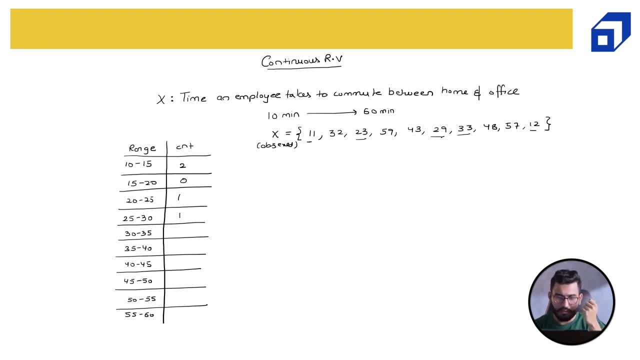 write 1 over here: 30 to 35, so 1 value over here. 1 value over here, So 2 values: 35 to 40,. 35 to 40, I don't see a value, So okay. 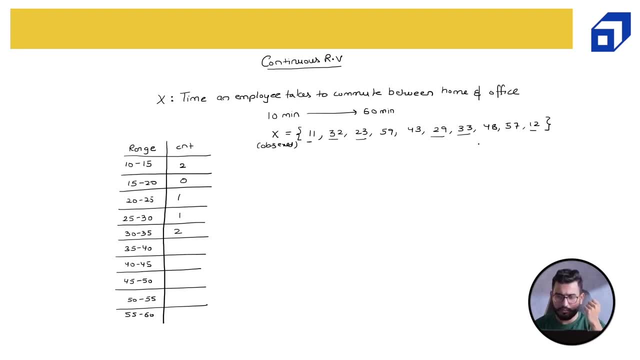 30 to 35,. I was having no value, So I should write 0 over here. 30,, no 35,. I am having 33 and 32.. Yeah, 2.. This was correct. Ignore if I am doing. 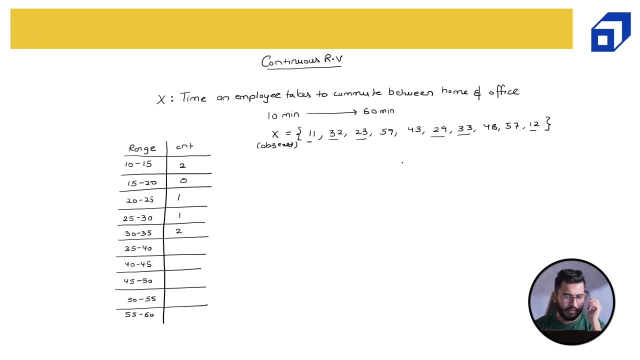 something wrong because I am just trying to quickly fill this table. 35 to 40,: 0.. 40 to 45,. 40 to 45,- 1 value over here, So 1. 45 to 50,. 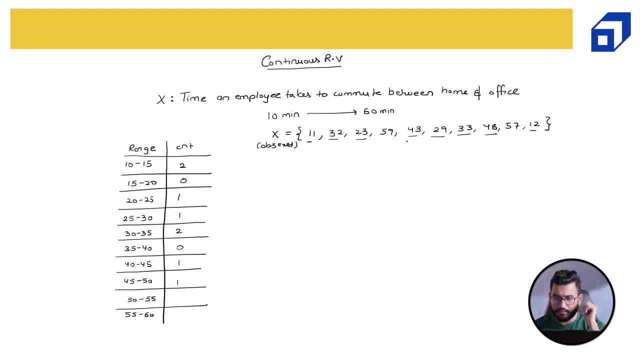 1 value over here. 50 to 55, I don't see a value 50 to 50,, 55 to 60, 1 value over here, 1 value over here, so 2 values. Now, when I plot this: 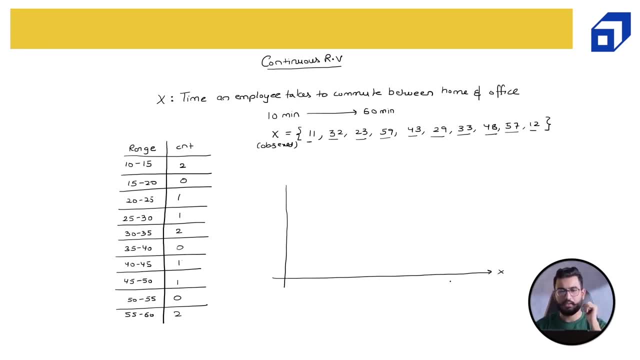 I will plot it as a range. So my x is over here, which is again the time taken by an employee to commute between office to home. Here I am having the same count, but here I will have the range, So starting from 10,. 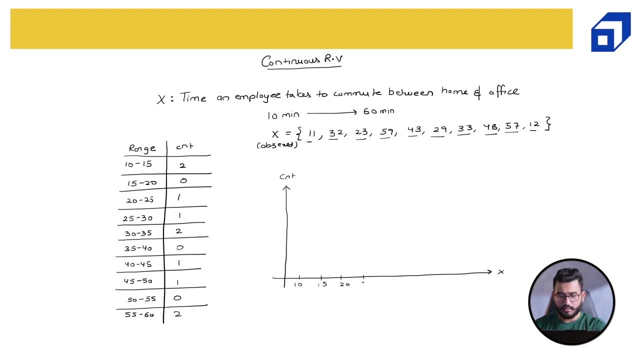 15,, 20,, 25,, 30,, 35,, 40,, 45, and so on till 60. And then I will have this bars, which is known as the histogram. This is not the bar chart, this is the histogram. 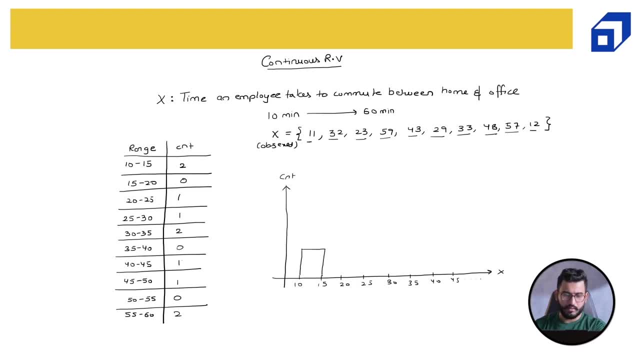 So 10 to 15,, let's say 2, like this, Then 15 to 20, I am having 0.. So a line like this: Then 15,, 20 to 25, I am having 1 and then 1.. 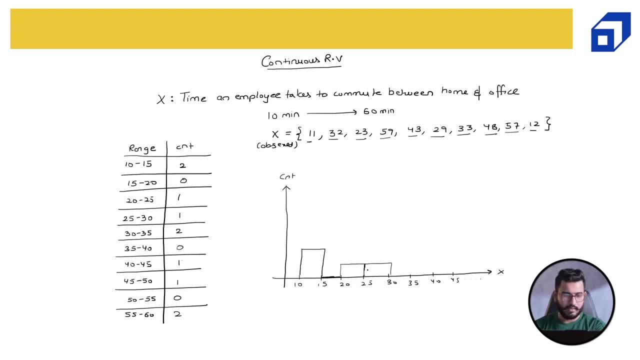 So let's say like this: And then then again I am having 2. And then again I am having 0. Then again 1 and 1. And so on. Now, this is basically my probability density function. PDF. 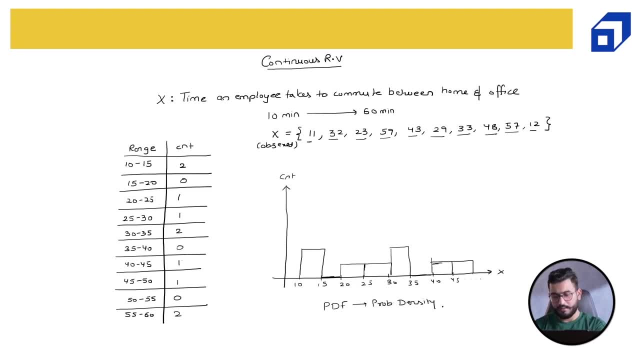 Probability density function. Now why I am calling it as a density? Because if I ask you what is the probability of a person takes the time between 10 to 15 minutes. I am not talking about one point, I am talking about a range. 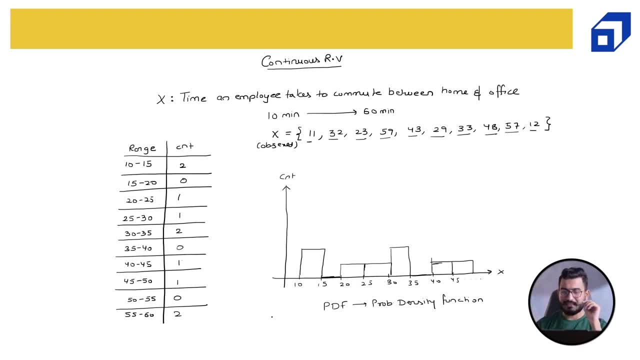 which is density. So that is the reason. here the distribution is known as the density And please remember, the probability of a one point, one point in a continuous distribution or continuous random variable is always equal to 0.. If I ask you what is the? 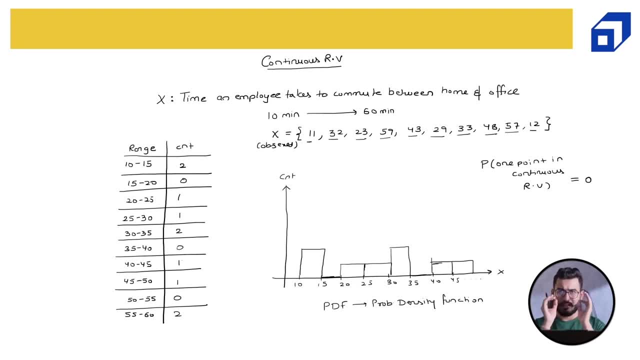 probability that a person will take 10 minutes. That would be 0.. The probability is 0.. The reason is: we cannot calculate it. We cannot calculate it because the way we are calculating the continuous random variable is by using a measure. Here we are using a measure. 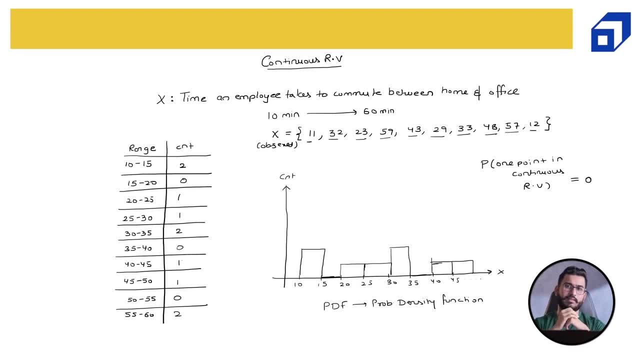 as the time taken by a person, And 10 minutes is something that a person can take endless number of time, So we don't know how many times a person can take 10 minutes divided by we know So how many times a person can take 10 minutes. 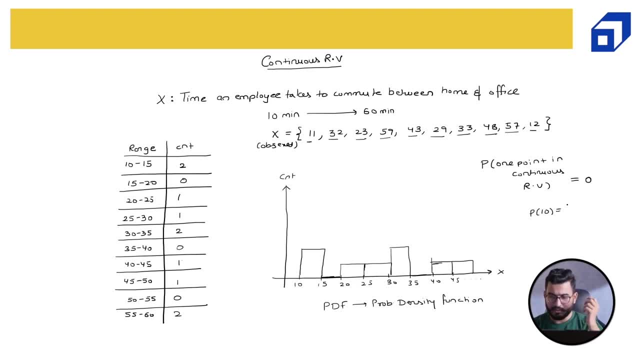 The probability of 10 minutes would be number of times the person takes 10 minutes divided by total, total total time, So total time. we know Total time is 60 minutes, But how many times the person has taken 10 minutes I don't know. 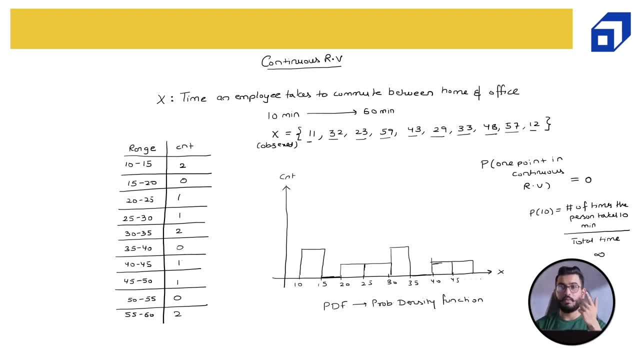 The answer. this can be infinity also, right? I don't know that. So the probability will end up becoming 0.. The probability of a point in a continuous random variable is 0. And the reason we call it as a probability density function is: 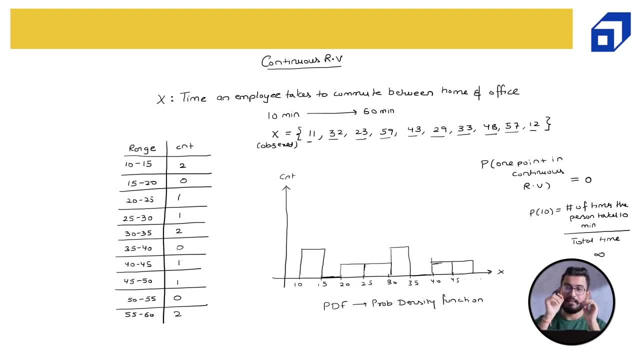 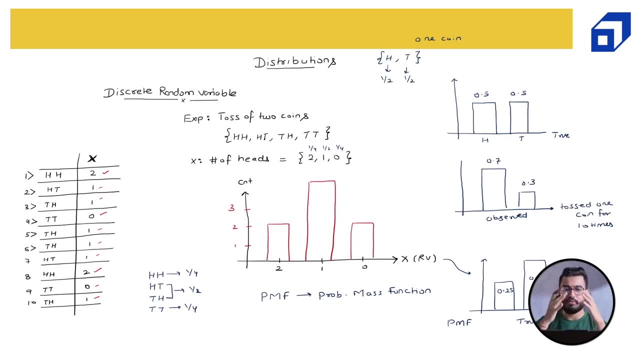 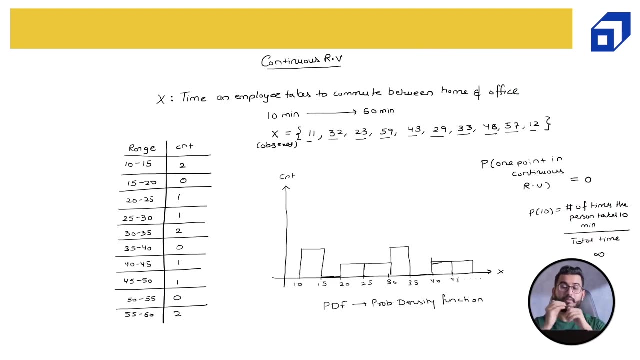 because we are not talking about one point, probability. We are talking about a range Now, within discrete random variable, the distribution for discrete random variable and the distribution for continuous random variable. we have some very general distributions, Some standard distributions that are very important in the 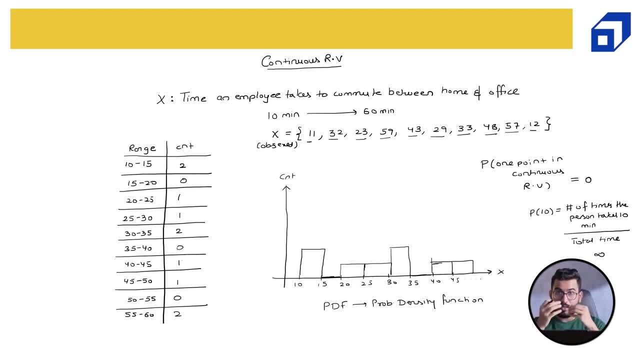 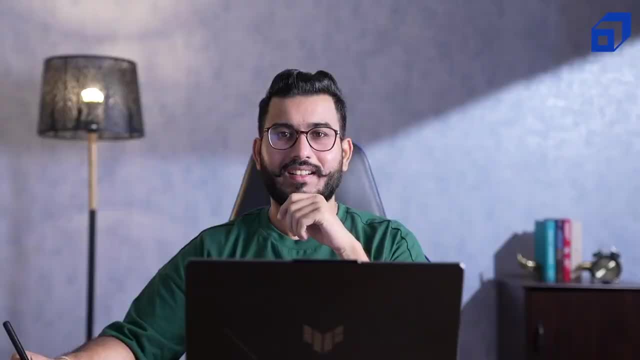 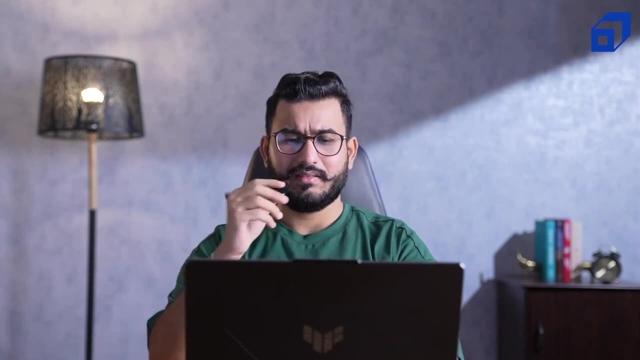 field of statistics and probability. So that is what we are going to learn. next, The various type of standard distribution. that comes under both discrete and continuous. So we have talked about discrete random variable and continuous random variable And we have seen very simple example of how. 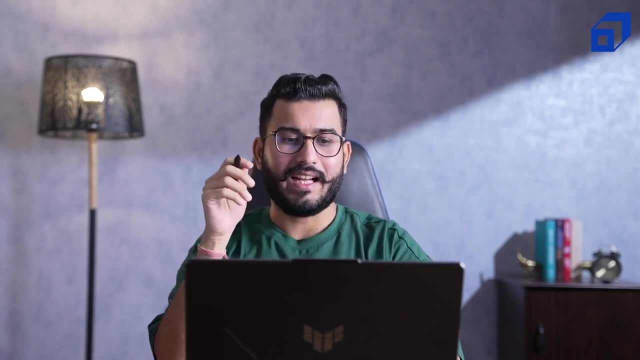 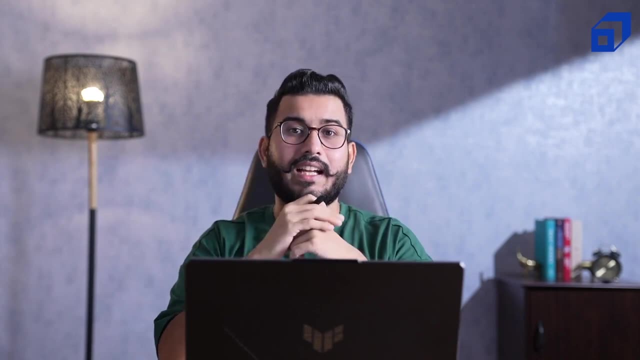 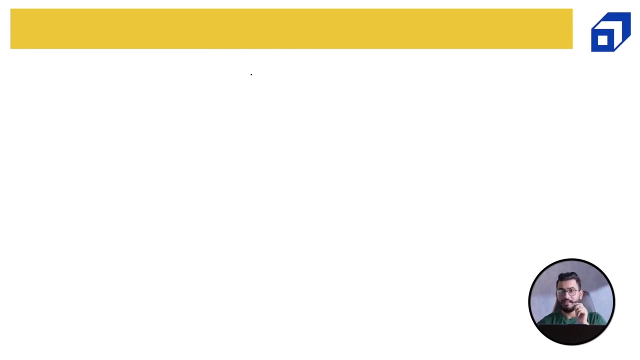 we can create distributions for discrete and continuous. Now there are some standard distributions that comes under discrete and continuous. So what we are going to do, we are going to talk about these standard distributions. So the very first we will first talk about 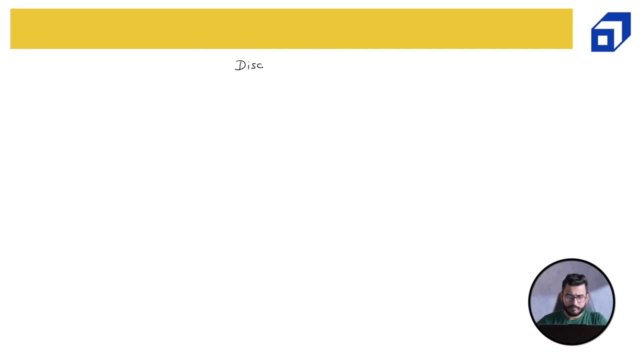 discrete. So within discrete, the discrete, random variable. we have two very important distributions: One is known as Bernoulli and the second one is known as Binomial. So Bernoulli distribution and Binomial distribution. Now, what is the? 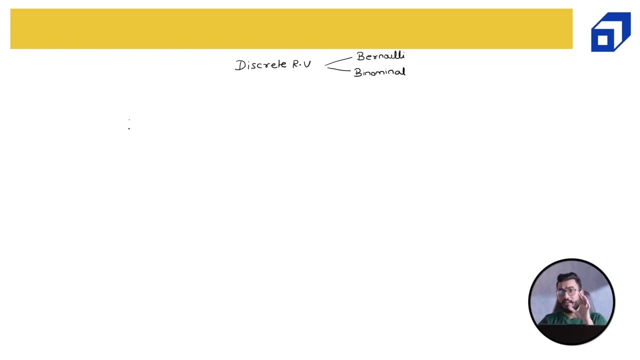 Bernoulli distribution. We will first talk about the Bernoulli experiment. So when we talk about the Bernoulli experiment, the Bernoulli experiment is a particular experiment in which number one, the outcome, is always binary. So the outcome is: 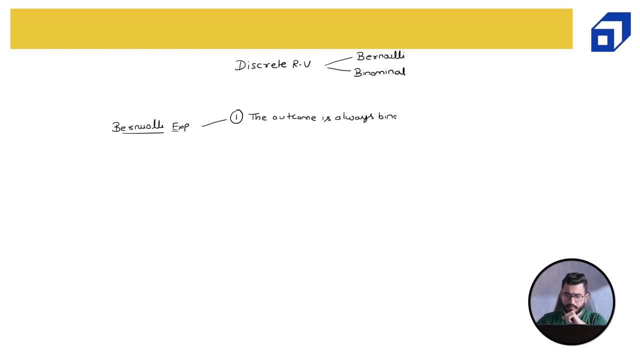 always binary, Which basically means the outcome is either head or maybe win or loss, head or tail. So let's say head or tail, or loss, or maybe one or zero. So it will always be binary. The second one is the number. 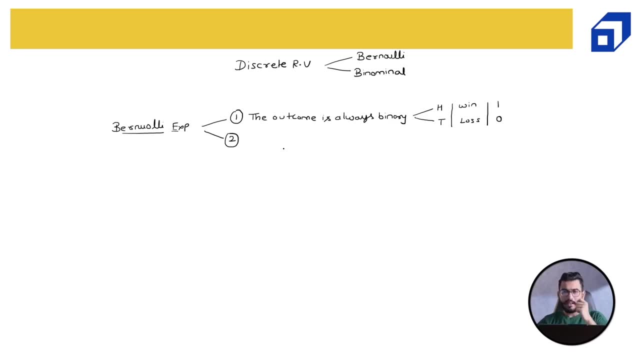 of trials is only one. So we are just performing the experiment for one time. So the the number of trials is only one. So, for example, let's say I am having a coin and I tossed this coin for one time. So 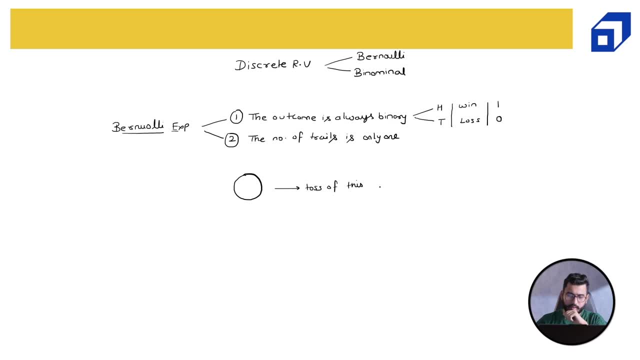 toss off this coin for one time. Now, can I consider this as a Bernoulli experiment? Yes, Why? Because when I toss this coin, I may either get a head or a tail, So the outcome is binary. Now, since the outcome is, 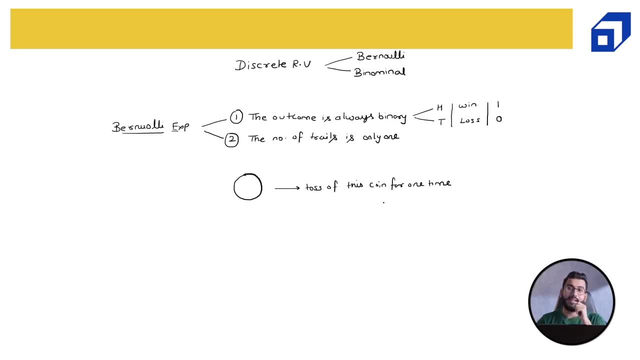 binary. this experiment is the Bernoulli trial. So why I am calling it as a trial? Because I am performing the experiment for one time, So I can either get head or tail. So the Bernoulli distribution looks like very simple. 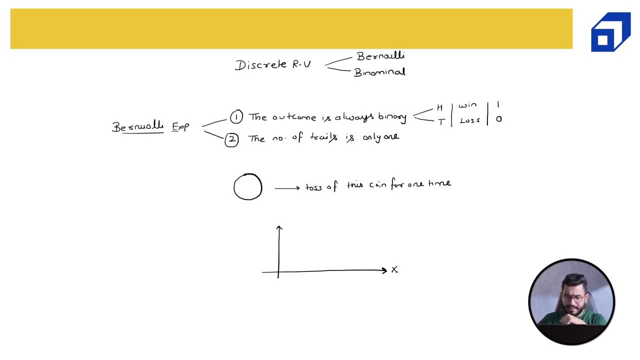 We have already seen it, but I am drawing it again. Let's: x represent the number of heads when you toss a coin for one time, So you may either get a head. So let's say I obtained a head and for tail, 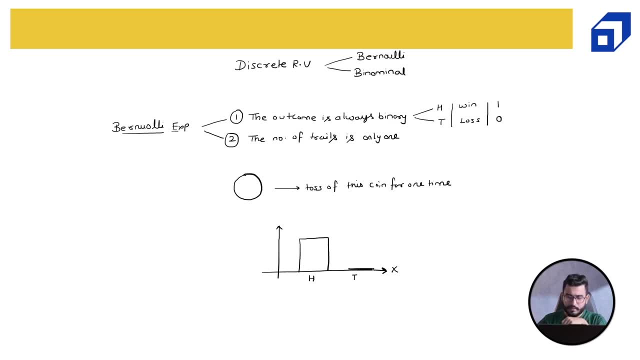 it is nothing. So this is basically my Bernoulli distribution. Bernoulli distribution. Now, please remember one thing: There is nothing difficult to remember about Bernoulli distribution. It is just a particular experiment which is having binary outcome and one trial. 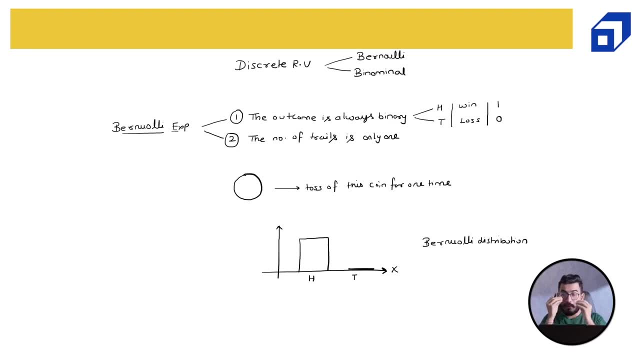 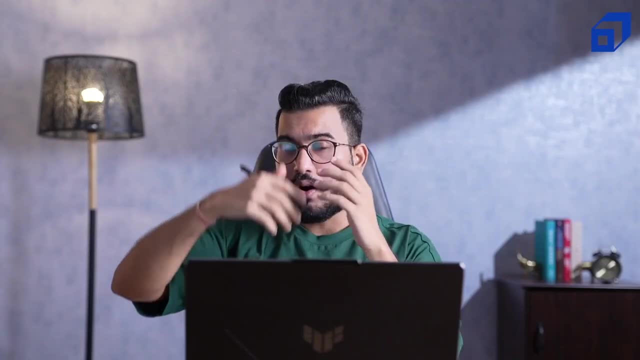 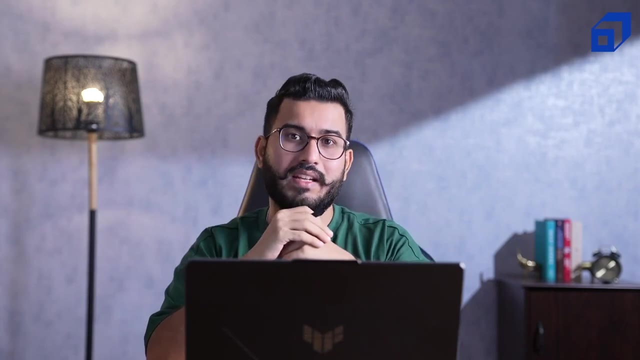 Binary outcome: one trial. Now, binomial is something very much associated with Bernoulli. So when I perform the Bernoulli experiment for n number of times, then we get a binomial experiment. So what is binomial? 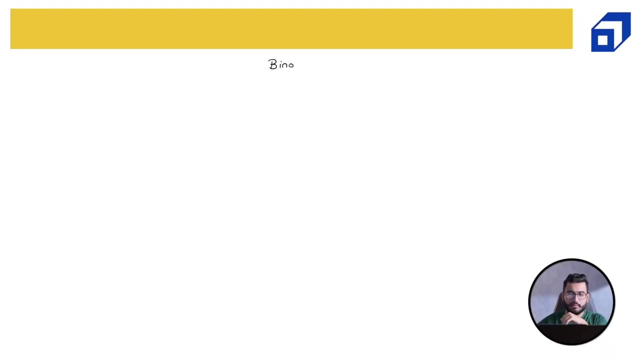 Binomial, binomial, binomial, binomial, binomial. So when the Bernoulli experiment, when the Bernoulli experiment is performed for n times, we get binomial experiment, We get binomial experiment. This is my binomial experiment. Let's take one example. 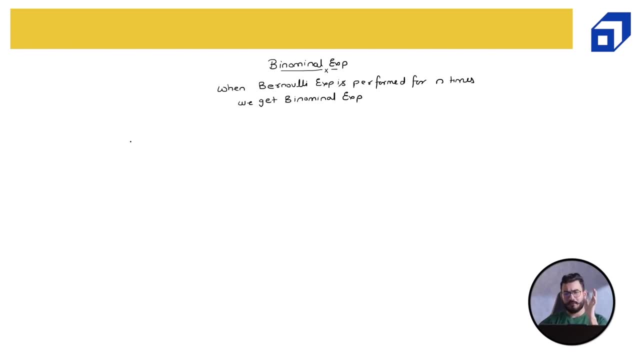 Let's say we are having a bag and we will try to understand the binomial experiment. Binomial experiment is nothing, but when I am performing the Bernoulli experiment for n times it becomes binomial Again. the outcome of each trial in 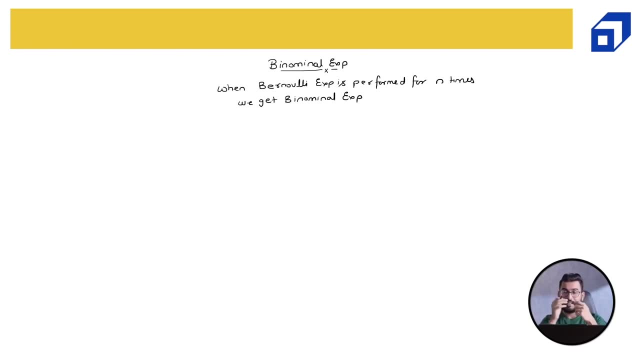 binomial experiment is binary. So again, assume that you are having a coin and you are tossing it for 10 times. Since I am tossing it for 10 times, it becomes binomial, But the outcome of each trial is going to be either head or tail. 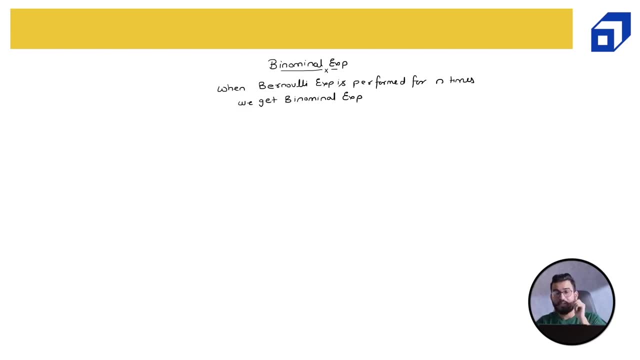 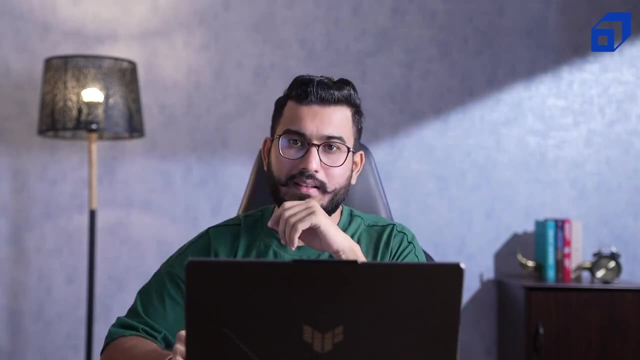 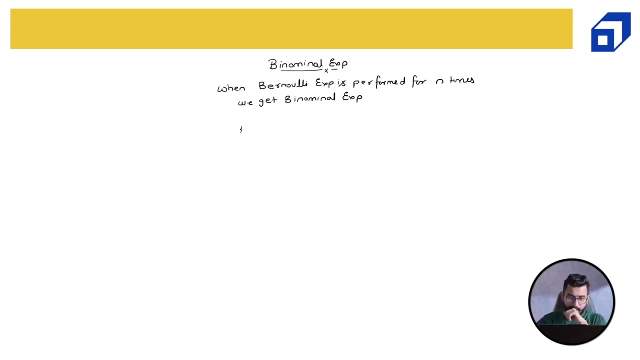 which is binary, and that is the reason it is a binomial experiment. So we have n Bernoulli experiments. When I combine them it becomes binomial. Now let's understand how to calculate the probability of binomial experiment. So probability. 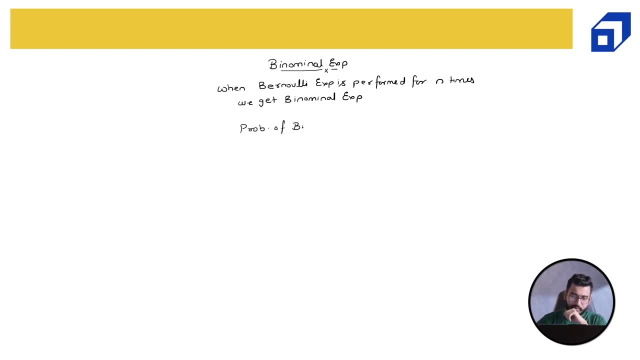 of binomial experiment. Okay, Now let's say I am having a bag and this bag is having, let's say, two orange balls. So two orange balls. So let's say the bag is having three orange balls and two white balls. 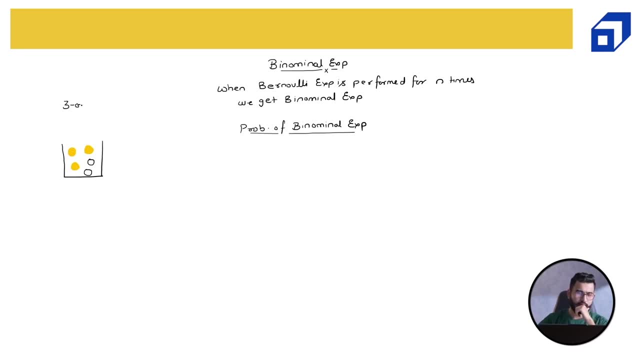 Two white balls, So three orange and two white. Now my random variable x is the number of heads. Oh sorry, My random variable x is the number of orange balls I may get out of this bag. Number of orange balls I may get. 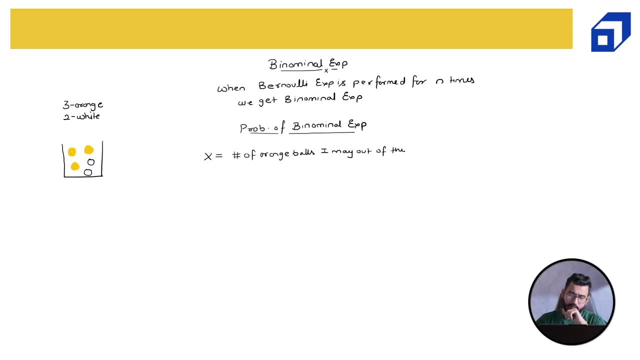 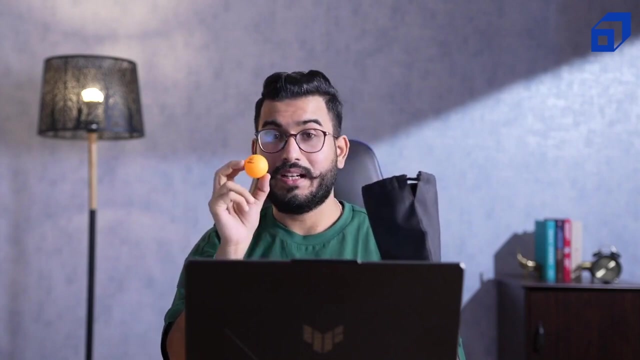 out of this bag if, if the experiment is performed for three times. Now, if you are not able to understand it, let's try to take the example. So the experiment is: we have to take the ball out of the bag. note down. 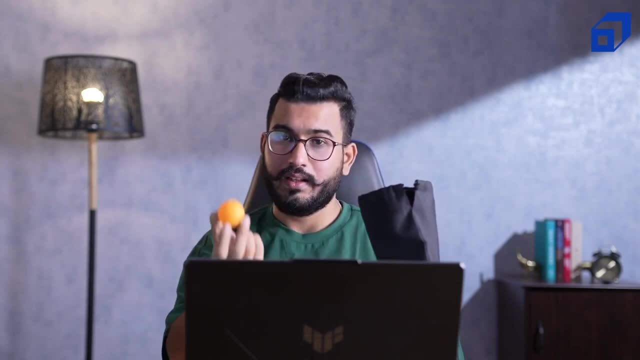 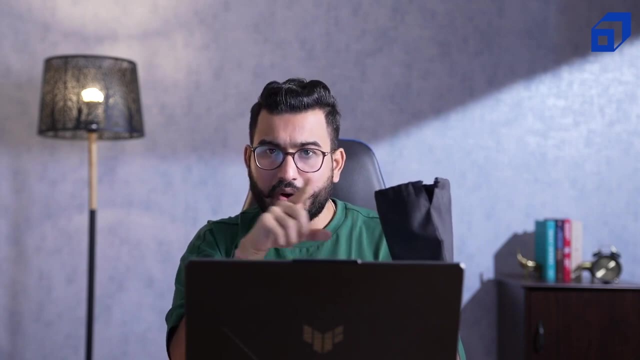 the color. So what's the color Orange? We will note it down and put the ball back to the bag, And I will do this for three times. Now is this a Bernoulli trial When I am taking the ball out of the bag for? 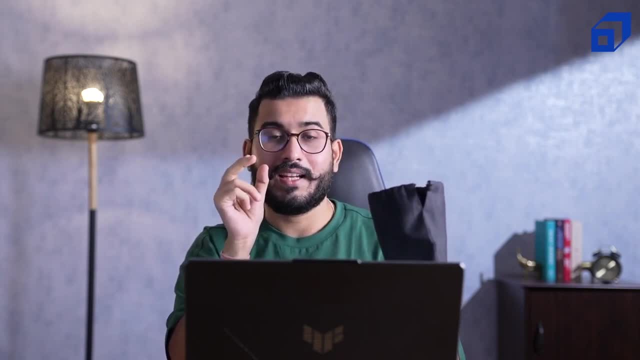 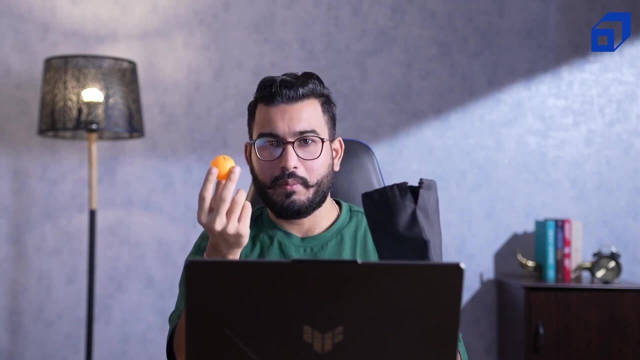 one time. is it a Bernoulli trial? Yes, Why? Because I can either get an orange ball or not get an orange ball. So first time I obtained an orange ball, This is my one Bernoulli trial And I placed the ball back. 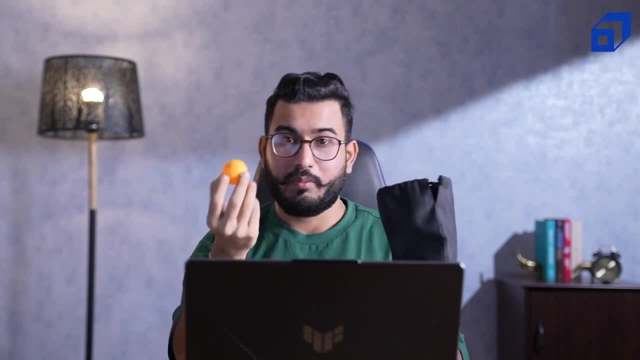 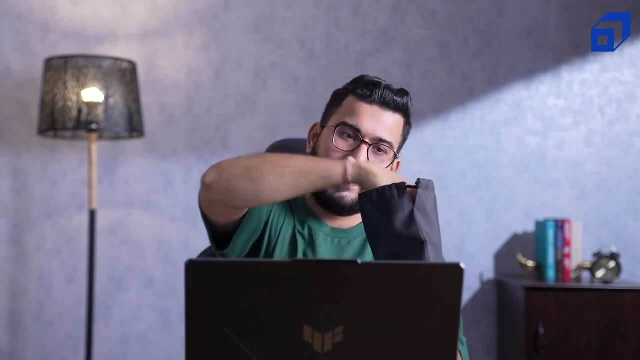 to the bag Again. I did the experiment. I obtained again an orange ball And I note down the color. I put the ball back to the bag And I did it again. I again take a ball out of the bag It came out to: 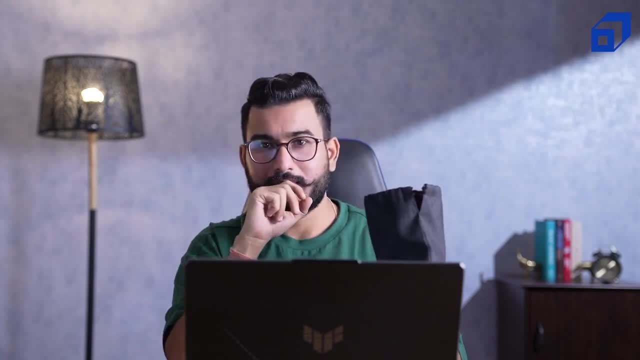 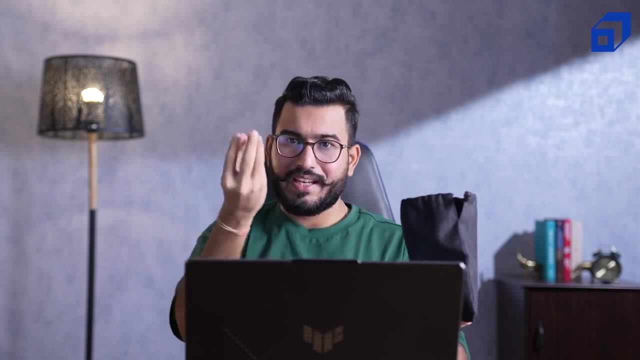 be orange. I note the color and I put the ball back to the bag. Now what is happening? I have performed the Bernoulli experiment for three times, So each time I was taking the ball out of the bag, it was a Bernoulli trial. 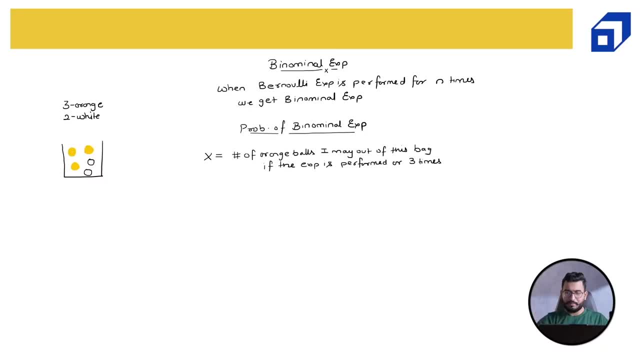 And I have performed the Bernoulli trial for three times, So let me just note down the outcomes. First of all, let me note down the experiment. The experiment is: take a ball out of the bag, Then note down the color of the. 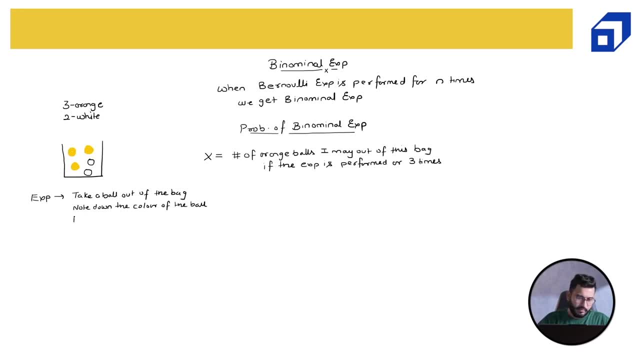 ball And then put the ball back to the bag. Back to the bag. Now we have to perform this experiment for three times. Now we have understood the experiment. right Now, let's say I am interested in finding out the probability. 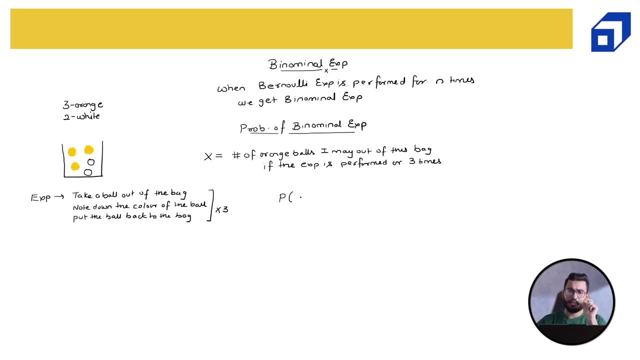 that I will get exactly two balls when I am performing this experiment for three times. So two orange balls, Two orange balls in three trials. Now what are the possible combinations in which you can get two balls or two orange balls? Let's note it down. 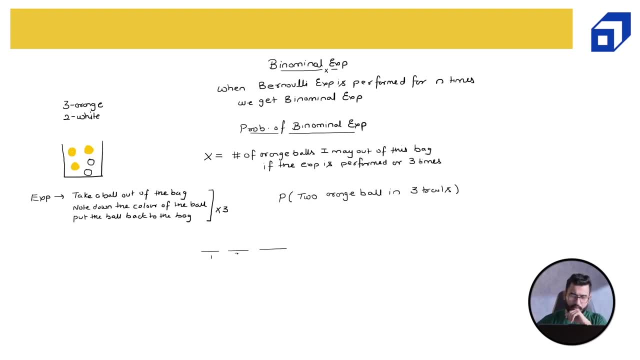 So this is my trial number one, two and three. Let's say, for the first two trials I obtained orange, So let me write O, O. And then you obtained a white ball. So white Then, for the first you. 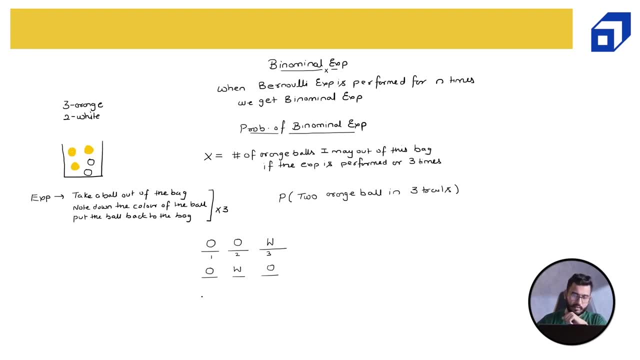 obtained orange, Then white, Then orange, Then, for the third, you obtained white, Then followed by orange and orange. So now these are the three possible combinations I may get out of this experiment. Now, what is the experiment? I am taking a ball out of the bag, noting 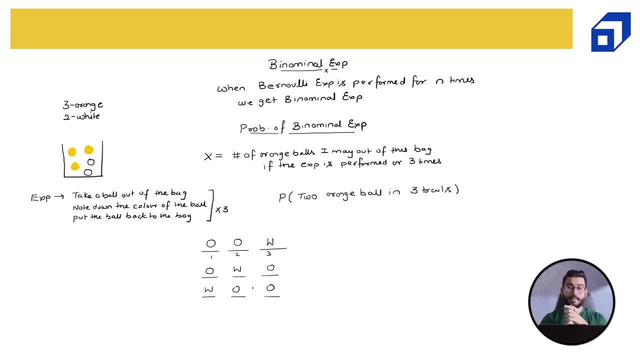 down the color, putting the ball back to the bag, performing this experiment for three times. My objective is to find out the probability that I will get two orange balls in three trials when I am performing this experiment for three times. These are the three possible combinations. 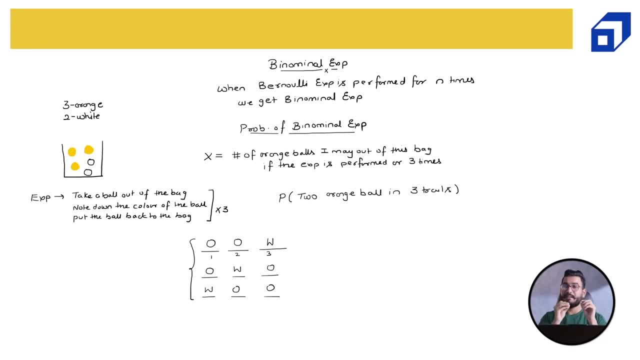 Now, if you carefully observe, each trial is independent of the other, because every time I am taking a ball out of the bag, the bag is still having five balls, because we have a total of five balls, right? So what is the probability of? 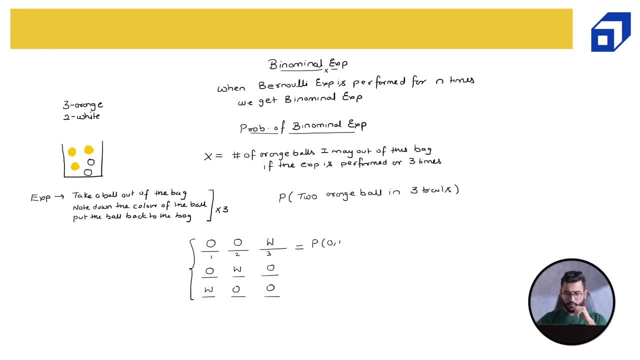 getting orange, orange white, It will be simply probability of orange multiplied by probability of orange, multiplied by probability of white. Similarly, for this orange white orange would be probability of orange multiplied by probability of white, multiplied by probability of zero. sorry orange. 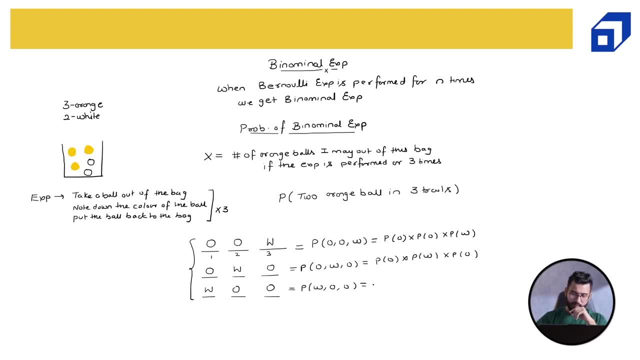 Then white orange. orange would be probability of white multiplied by probability of orange, multiplied by probability of orange. Now, probability of orange is three divided by five. Probability of orange is 3 divide by 5.. Probability of white ball is 2 divide by. 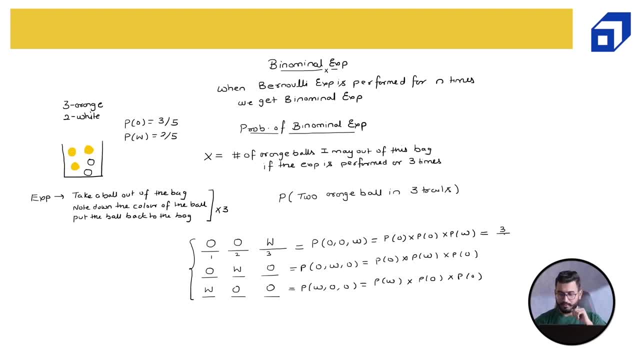 5.. So this will be 3 by 5 into 3 by 5 into 2 by 5.. This will be 3 by 5 into 2 by 5 into 3 divided by 5, and this will be 2 by 5 into 3 by 5 into 3 by 5.. So if you carefully observe, 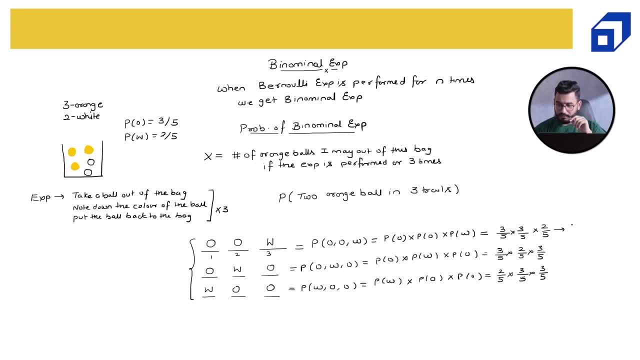 I can write each of them as 3 by 5 to the whole square into 2 by 5.. I can even write this as 3 by 5 to the whole square into 2 by 5.. I can write this as 3 by 5 to the whole square. 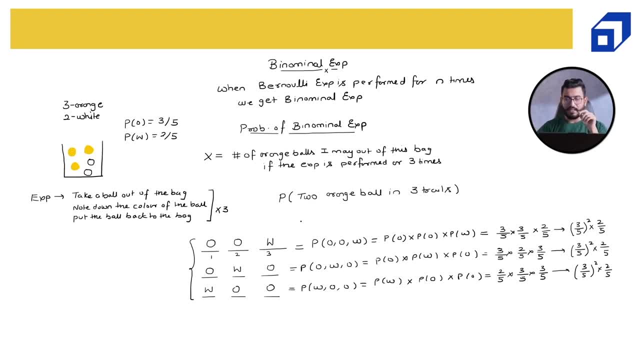 into 2 by 5.. Now what is the probability of getting to orange ball in three tiles? I'm having three possible combination, So it can be either this or this or this. So when I'm having an all term, that basically means I have to add all of them, right? 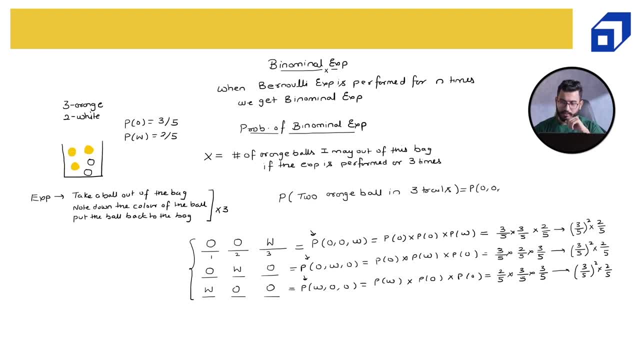 So to probability of O comma O comma white, which is plus probability of orange comma white comma orange, plus probability of white comma orange comma orange. Now we have already calculated everything. So it is- I'm just taking it over here- So it will be um. 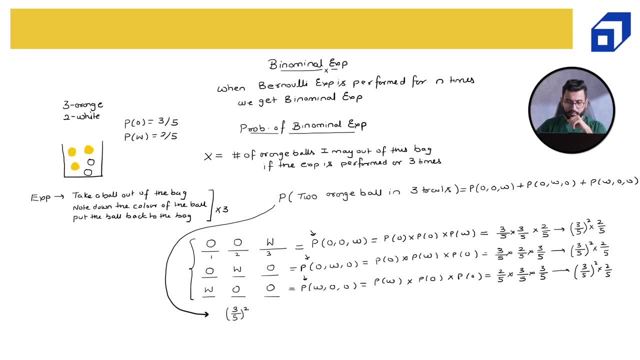 three by five to the whole square into two by five, plus three by five to the whole square into two by five, plus three by five to the whole square into two by five. Now all the three terms are similar, so we can just simply write it as three times of three by five to. 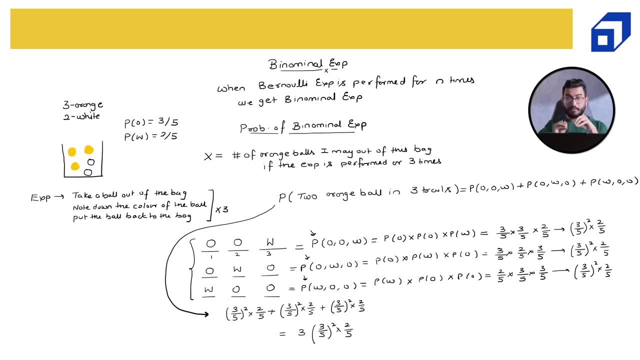 the whole square into two by five. Now this particular equation can be generalized for any binomial experiment. How Let's see. The generalized equation is N, CX, PX, Q to the power N minus X. This particular equation can get you the probability of any binomial experiment. 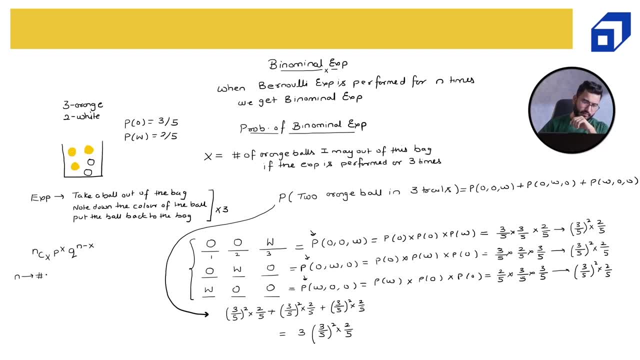 What is N? N is the number of Bernoulli trials. Bernoulli trials, X is the number of success in N trials, P is the probability of success and Q is the probability of success. What is Failure? So failed. So if I try, 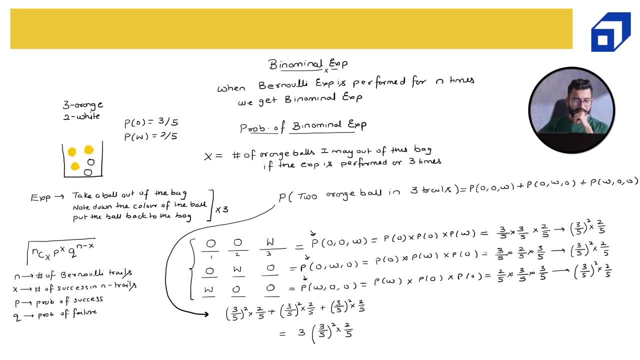 to map this equation for this particular experiment, where I have calculated the probabilities three times of three by five to the whole square, to two by five. um, let's try to do it in the next slide. So the formula is NCX, PX, Q to the power N minus X. Now I've delivered. 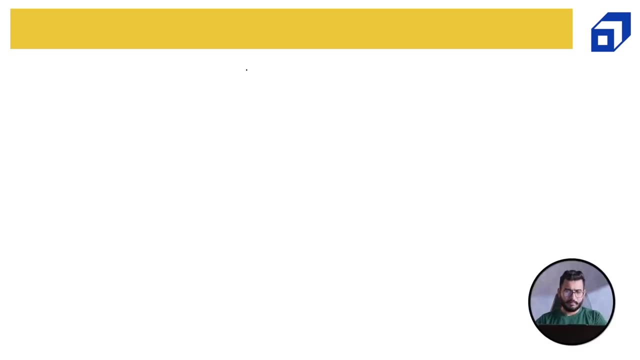 this problem here already, as we were lasts diseases, uh numbers. so now what I'm going to figure out is: what is I'm going to see? a بPB up to n minus X? In the last experiment we were performing the trials- Bernoulli trials- for three times. 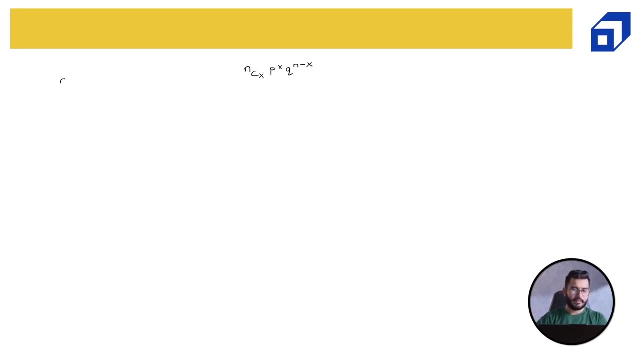 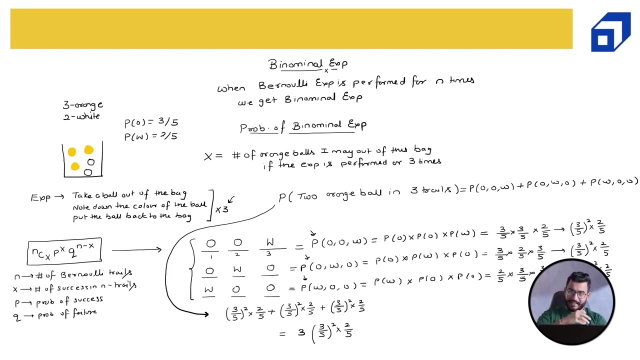 Here I have written it right. So my value of n is 3.. Now, what is x? x is the number of success. Now, if I consider getting an orange ball as a success, then I was interested in getting two orange balls right. 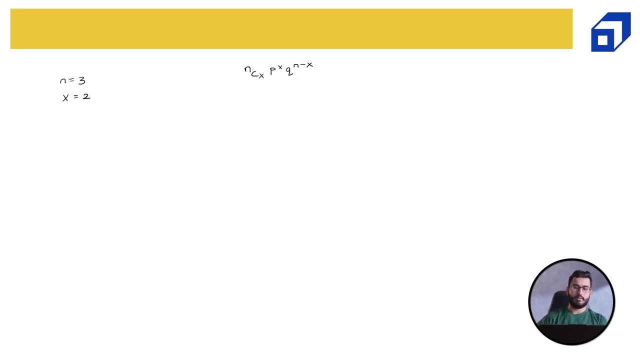 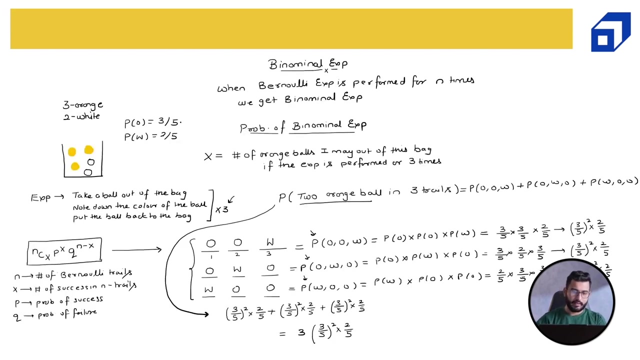 So my x is 2, because I am interested in getting two orange balls. P is probability of success, which is nothing but probability of orange, And orange probability is 3 by 5.. And Q is the probability of failure, which can be also written as 1 minus P. 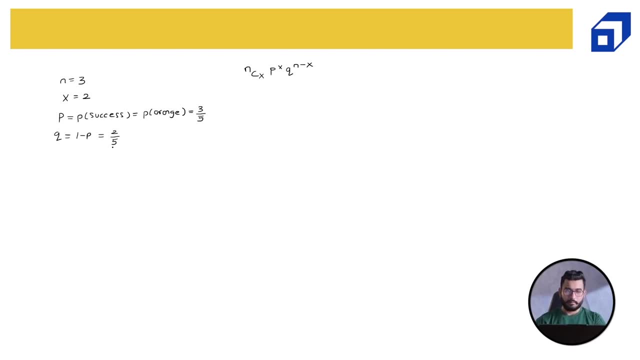 This is given as 2 by 5.. Now, if I put everything on the formula, this will be 3C2,: 3 by 5 to the 2, into 2 by 5, into to the power of 3 minus 2, which is 1.. 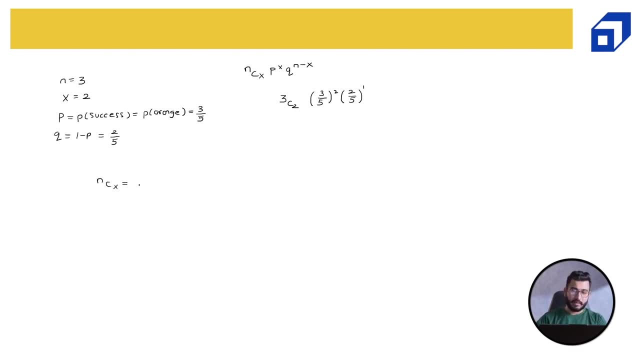 Now the nCx factorial. this particular term can be expanded as n factorial upon x factorial, n minus x factorial. So 3C2 would be 3 factorial upon 2 factorial, 3 minus 2 factorial, which is 3 into 2 factorial. 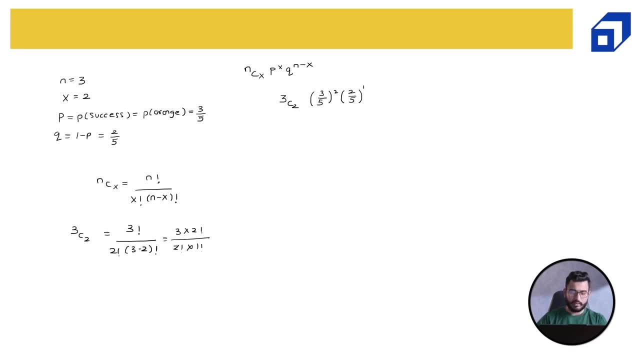 divided by 2 factorial into 1 factorial. 2 factorial will cancel out 2.. So we'll be left with 3.. So 3 times of 3 by 5 to the whole square and 2, 2 by 5.. 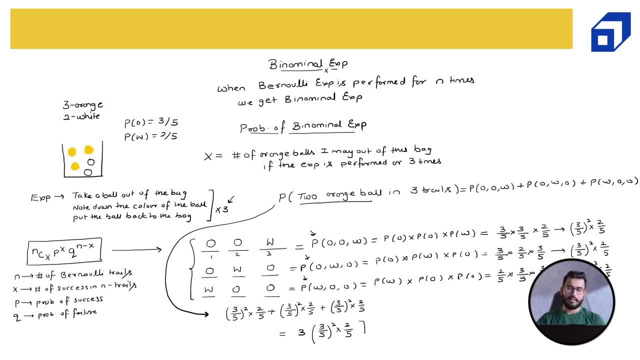 And here you can see we have already done this manually. So using this formula you can find out the probability of the number of success in n Bernoulli trials, The number of success which is x in n Bernoulli trials Which becomes binomial right. 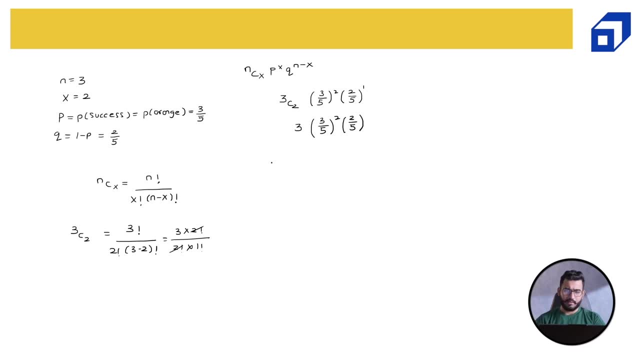 Let's take one more example, a quick example, to help you understand this. So I'll just create a portion over here. So let's say there is a person who is trying to shoot a target. Here we have a person. this person is trying to shoot a target for for 10 times, for 10 times. 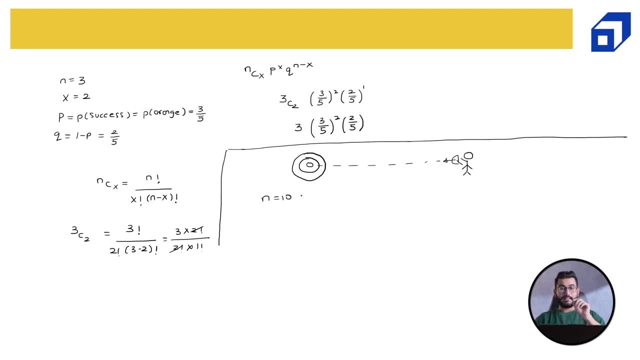 So n is 10.. Now is this: is this particular experiment consists of a Bernoulli trial? Yes, Because when the person is trying to shoot the target, it will either hit or miss. So it is a binary experiment, which is the outcome is binary. 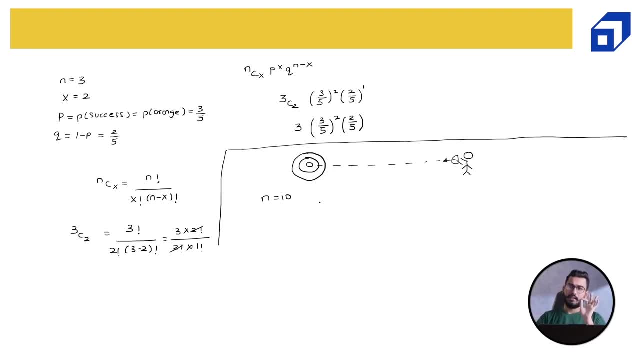 And if I consider the experiment to be performed for one time, it is a Bernoulli trial. Since I'm performing this experiment for 10 times, it becomes binomial experiment. So let's say the person is trying to hit the target for 10 times. 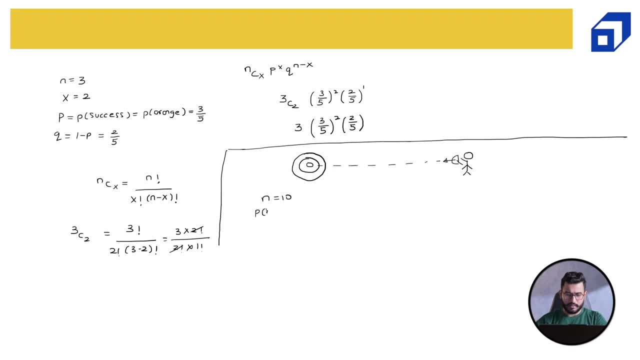 The probability that he will make a head is point, let's say, um 0.4.. So there are 40% chances that if a person tried to tried to make a head to the target, it will hit the target 40% of the time. 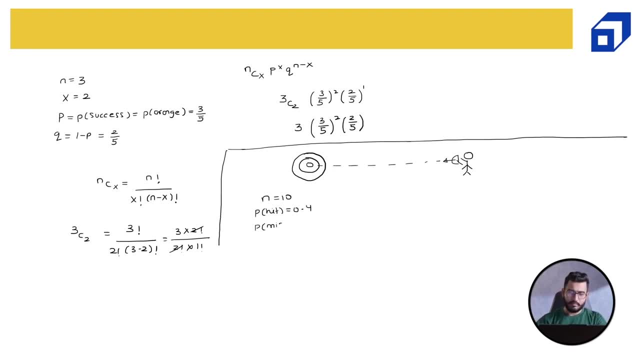 So the probability of miss will be 20%. So this is the probability. So the probability of miss will be 20%. So you will hit a target for 10 times. The probability of miss is 40%. It is a binary experiment. 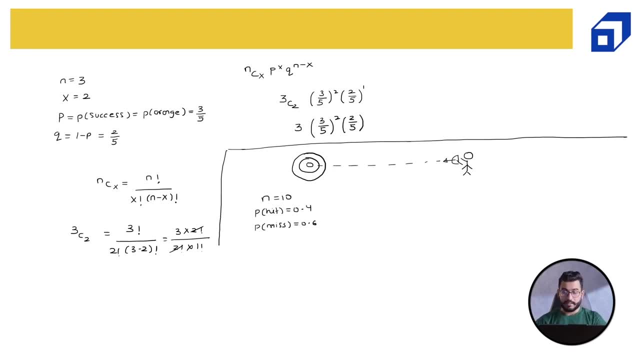 So you will hit a target for 10 times 0.6.. Now I'm interested in probability that he hits the target exactly for five times. So I'm interested in five success in 10 Bernoulli trials. So my X value will be five. I quickly apply the formula and CX, P, X, Q to the power and minus X. 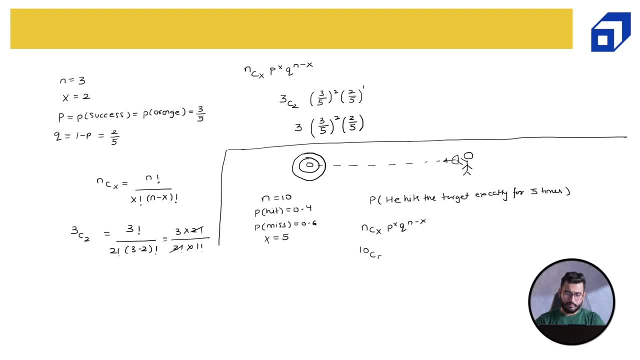 and is 10 C. five Probability of hit is 0.4 to the power of five and then 0.6 to the power of five. You can solve this and you will get your answer. What is the probability that, if the person is? 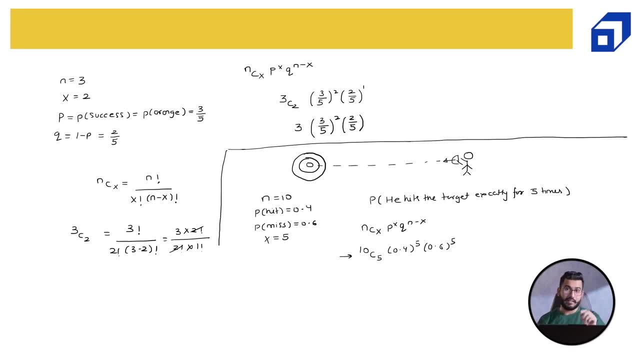 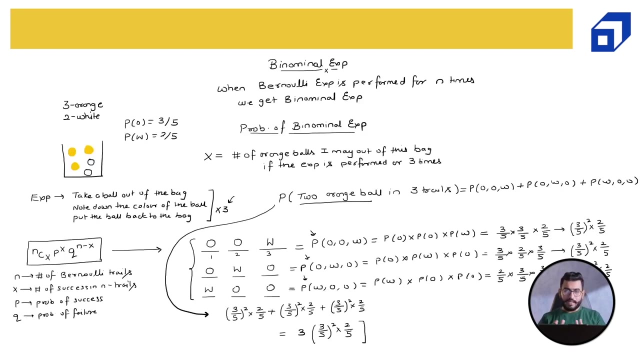 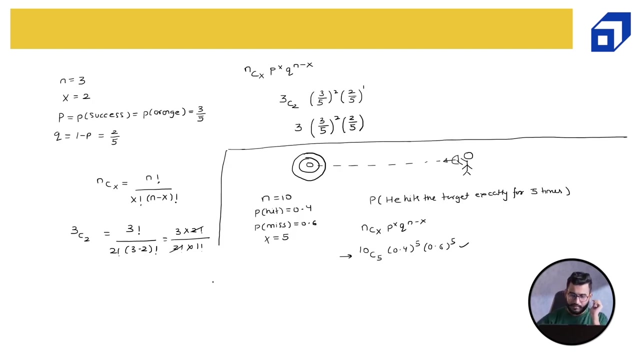 trying to hit the target for 10 times, he will make a hit. He will make an exact hit For five times and this will be your probability. This is the binomial probability. Now, if I calculate all the probability for all the random variables in this case, in the case, 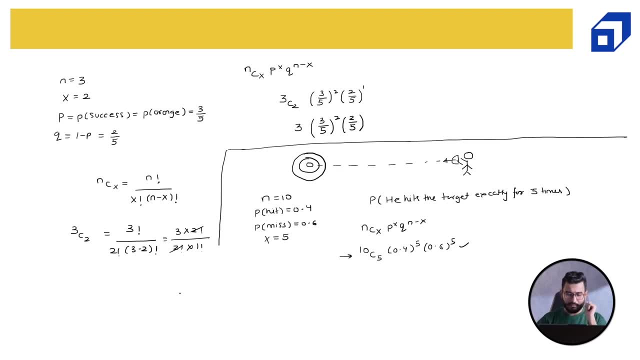 of hitting the target. what is my random variable? My random variable X is the number of times this person makes a hit makes a hit. Now the person can make a hit for all the 10 times, for nine times, for eight times, for seven times, six times or maybe for zero times. So these are all the random. 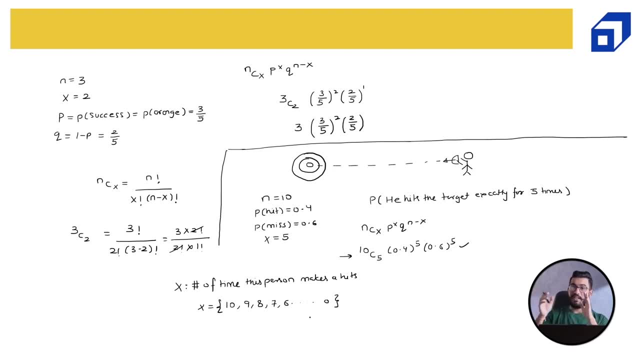 variables now against each random variable is why calculate the probability? and I plot them. So let's say: here I'm having X, here I'm having probability of X is equal to X side. And if I calculate all the problem probability, what is the probability that he will hit the target for exactly 10 times? 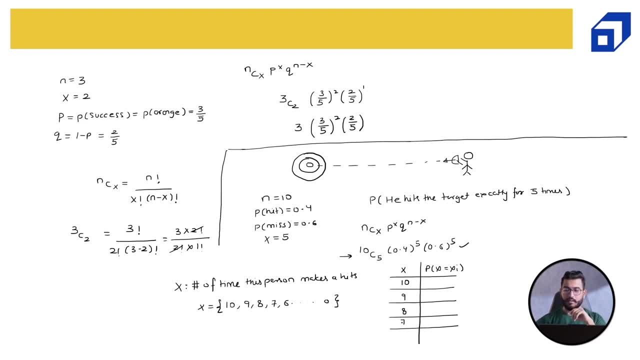 for nine times, for eight times, for seven times and so on, And if I plot it in our mass function. so here I'm having X, here I'm having, let's say, probability P of X is equal to X I, then this will become my 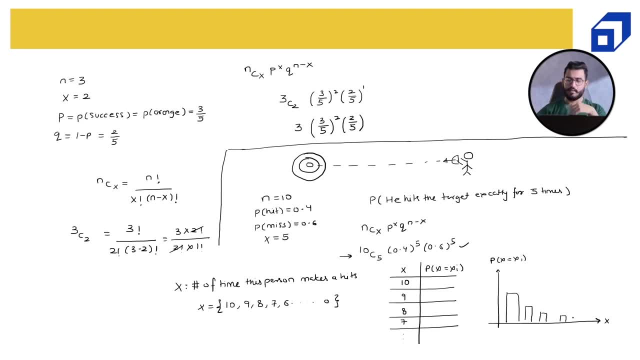 this will basically become my PMF of binomial probability or binomial experiment. I hope everyone is clear about this. We can have a quick Excel example to demonstrate you how this particular PMF looks like. So let's look at it. Excel example. 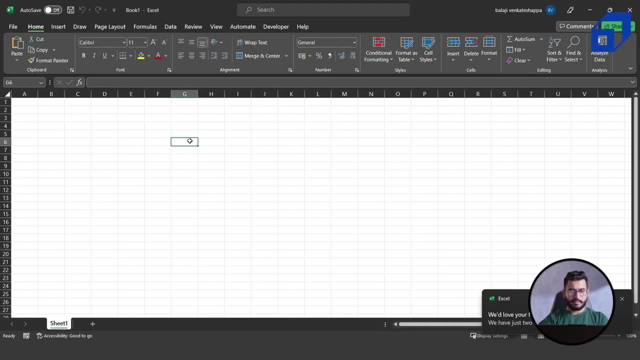 Now, here I'm having a Excel worksheet. Let's say, this is my X, which can be a zero: one, two, three, four, five, 6,, 7,, 8,, 9, and 10.. What is the meaning of one? Uh, zero. That basically means person was not able to make. 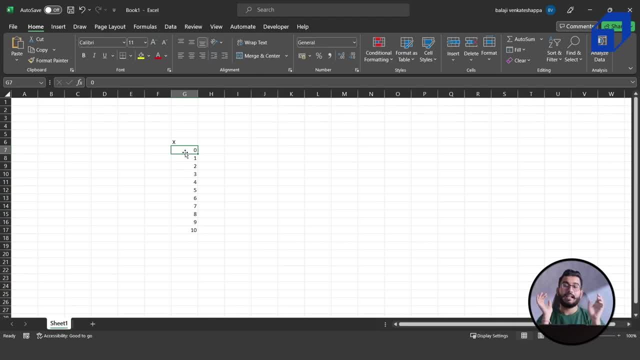 any corrected. So if the person was trying for 10 times, he was not able to hit for any time. the, the, the. the number of successful hits was zero. What does it meaning of one? 1. 1 basically means when the person was trying to hit for 10 times, or maybe shooting for 10 times. 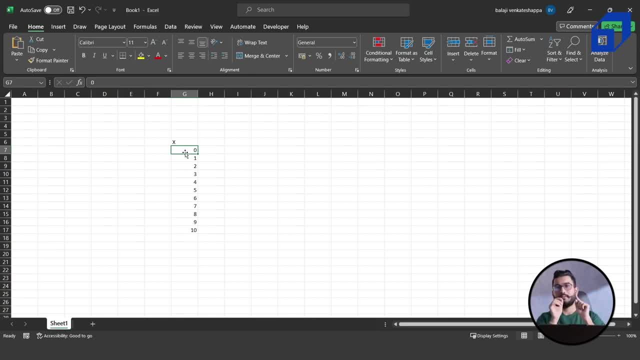 he was able to hit the target only for one time. So that's what my X is. I'm now interested in calculating the probability of X is equal to Xi, So let's do that. We will use the formula um, the combination formula. So combine is the combine is the function that we have in Excel. 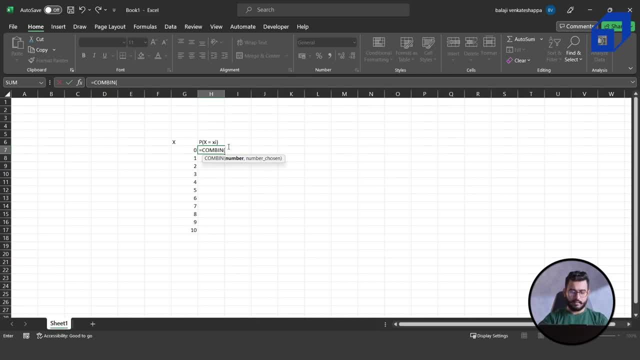 And, uh, the total number of trials are 10. X is this multiplied by? So NCX probability of success was 0.4, 0.4 to the power of X, 0.4 to the power of X- And I'll put this in a bracket so that nothing is getting wrong- And this is multiplied by um. 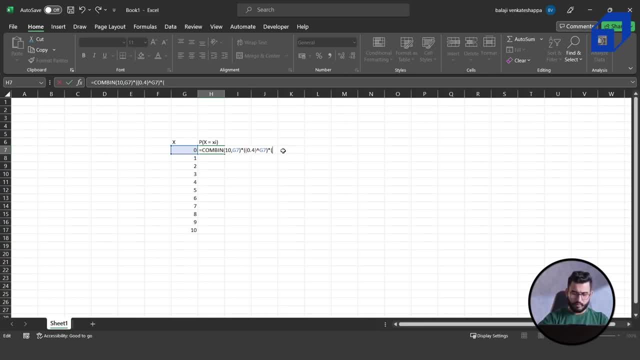 failure. So Q, so 0.6 to the power of N minus X, So 10 minus X and I close the bracket and I think everything is fine. Let's expand this. I have the probabilities Now let's plot it. So I'll go to insert, I'll choose a chart. 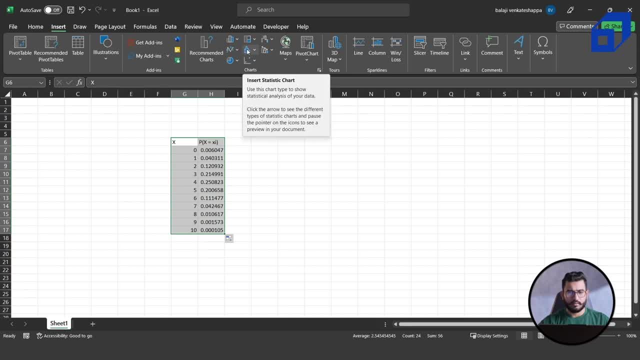 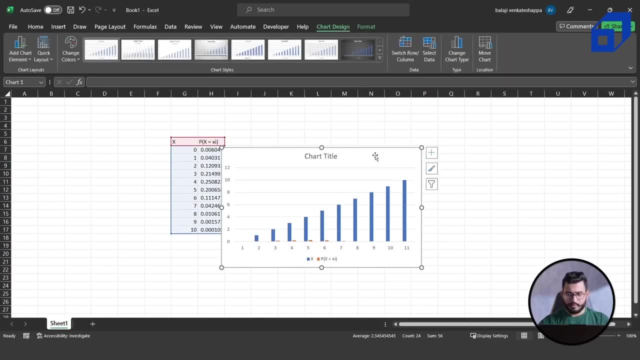 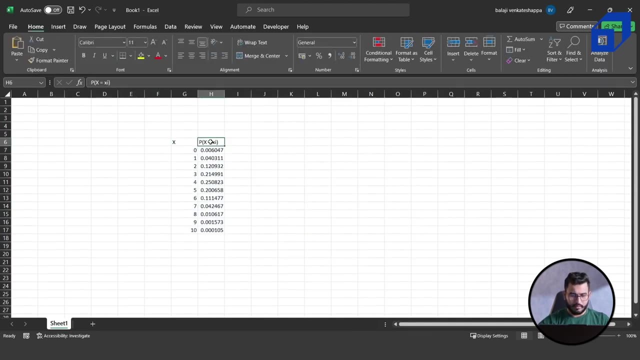 maybe a column chart, And here we have the probability, which is wrong. Actually, it is plotted very wrong, Um, and I should choose only I think, if I choose this also, let me try it for one more time, Otherwise we have to manually do it. Okay, That is not. 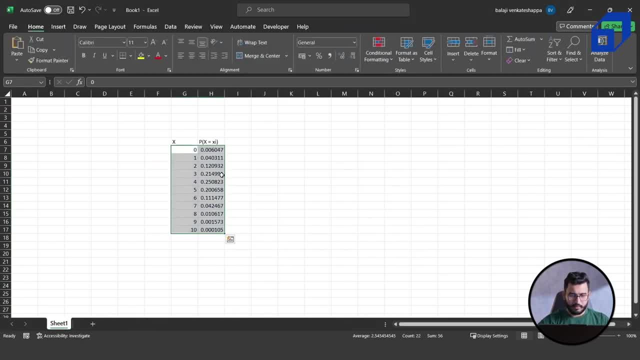 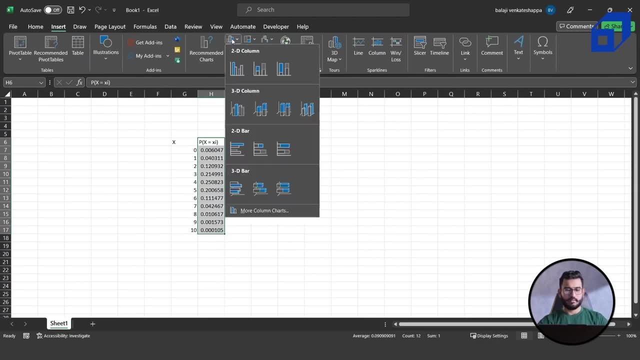 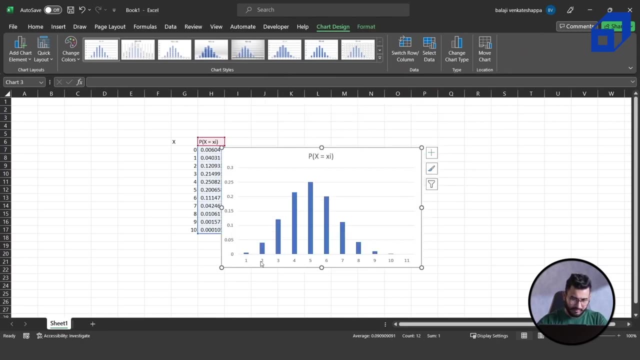 coming correctly. So let's choose only this one. uh, in salt. and the start. Now here: um, first of all, this is not one. This will be zero. This will be one because, um, we have haven't selected the X, So assume this is zero, then this is one, and so on. Now you 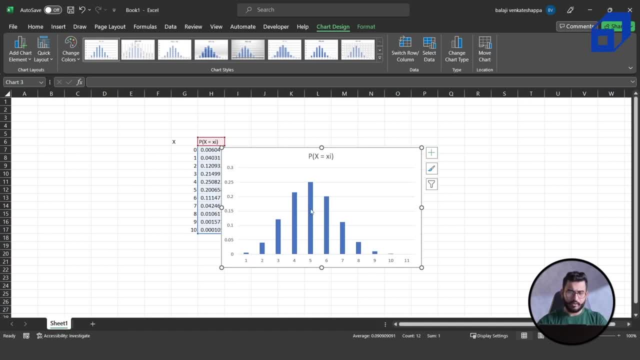 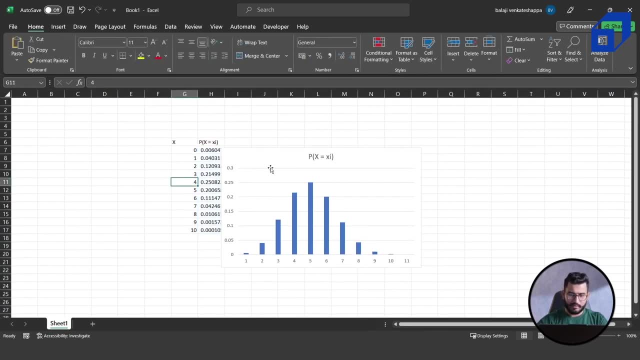 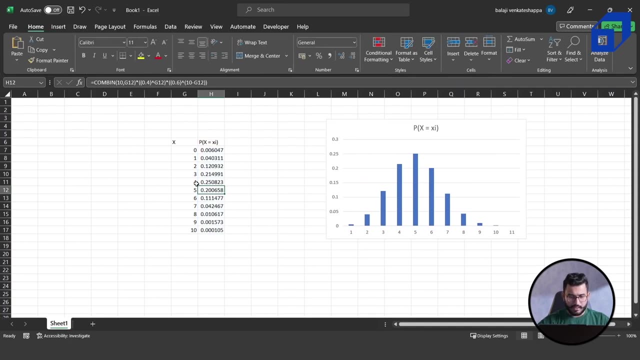 can see that the probability that a person will hit for four times is highest. four times is highest And here you can see in the, in the result also, that the person hitting the target for four times is highest. And then as we move forward it becomes lower and lower. 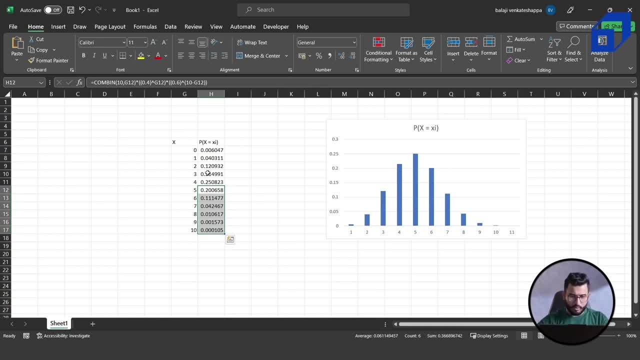 and lower And if I go below four it is becoming lower and lower and lower. So using the probability mass function of any discrete random variable, we can answer a lot of questions. So if I ask you, what is the probability that the person will be able to hit, or the person will? 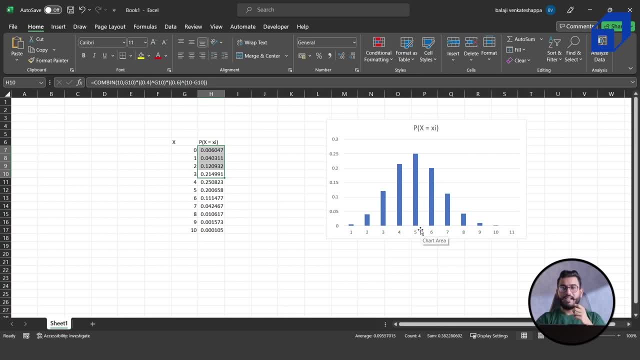 be able to make at least five. at least five correct hits, or at least five correct hits, Five successful hits. So at least five means I'm interested in the probability of X greater than or equal to five, which basically means I'll just simply take the summation of all. 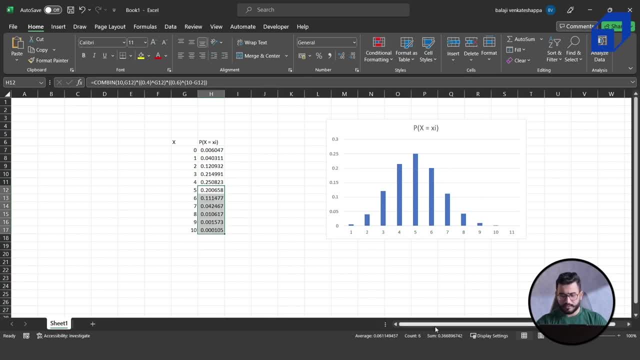 these probabilities, which is equal to 0.36.. So there are there are 36% chances that the person will hit at least four or five times. What is the probability that the person will be able to make the correct hit at most? five times at most means less than five. 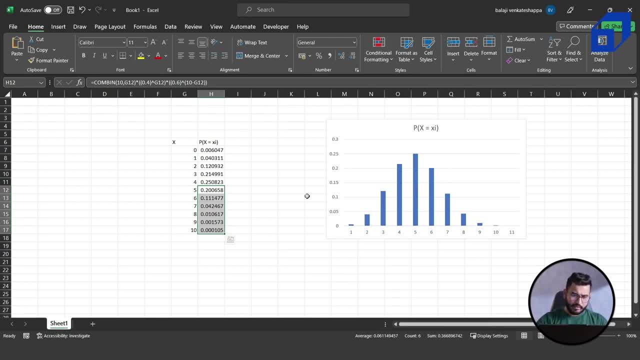 Or equal to five, which basically means I'm interested in all these probabilities, which is 83%, which basically means the person will be able to make at most five correct hits, 83% of the time, right Now, using this PMF of various distribution, various discrete. 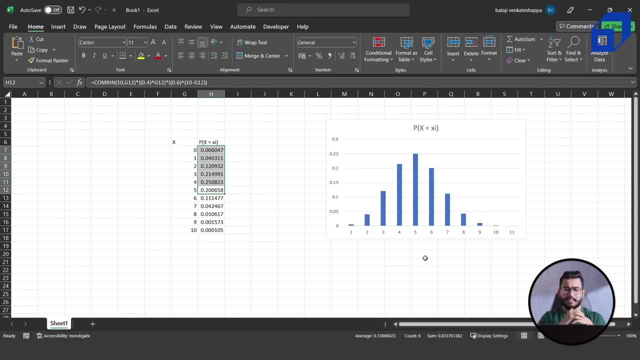 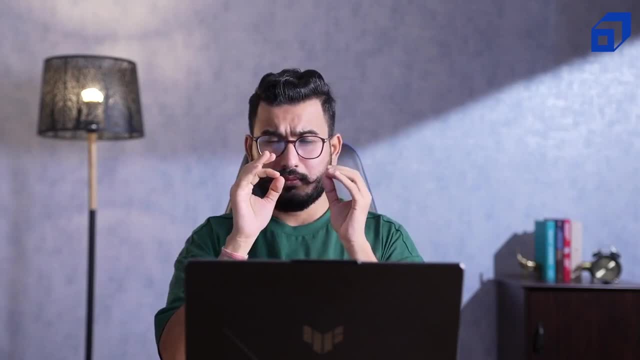 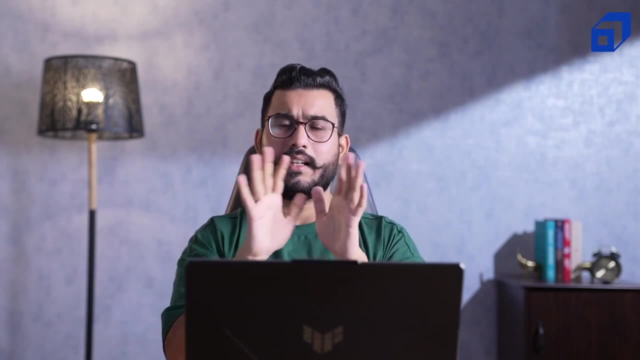 random variables. we can answer a lot of questions right, And that is the reason these distributions are created. But we are interested in one such distribution, that is the. I would say that is a very important distribution in the entire statistics and entire machine learning. That is known as the normal distribution, which comes under 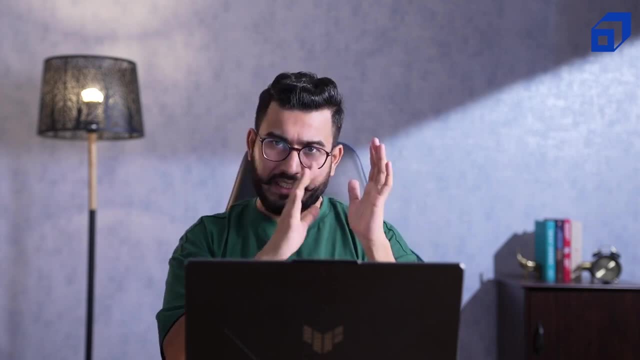 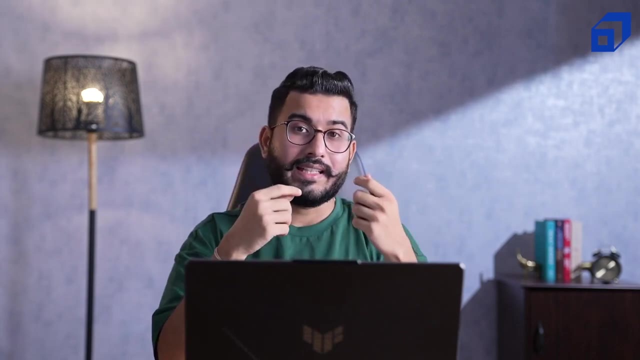 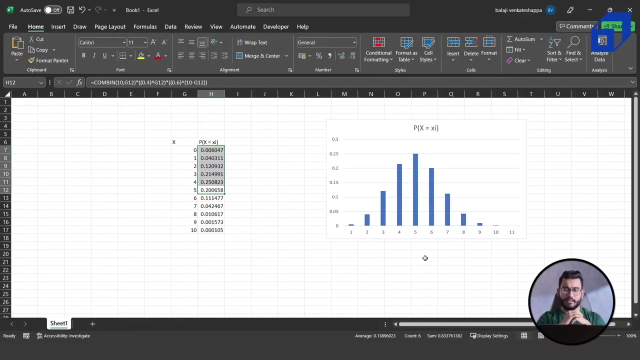 the continuous random variable. So we have completed a discussion around a discrete random variable, under which we talked about Bernoulli experiment and the Bernoulli distribution, then binomial experiment and the binomial distribution, And this is Now let's talk about the continuous random variable And within that, the most important. 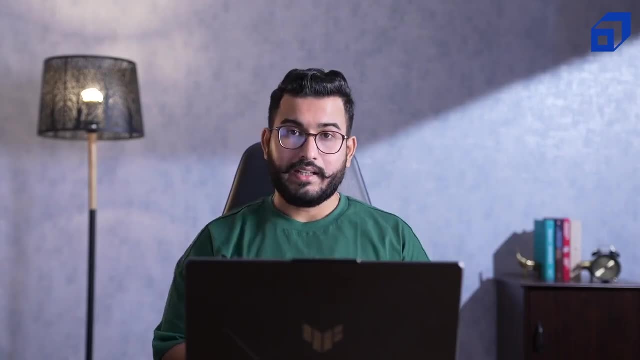 distribution is normal distribution. If you guys are targeting for any data science job and you have to, or you have to attend your interview for the data science field, then this topic is one such topic that you will a hundred percent find out in your interview. 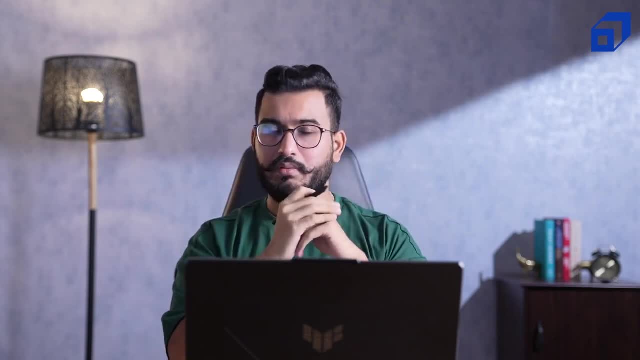 It can be in any way, but it will be around. You want to make sure we get a lot of information around this topic, So please listen to me very carefully, because this is really important. Then, when it comes to data science interviews. 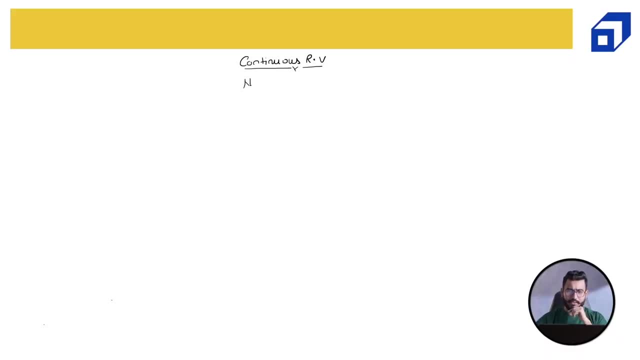 So, when it comes to continuous random variable, we have our distribution, known as the normal distribution, And normal distribution is something that looks like a bell shaped curve, Something like this. I want you to appreciate that. I want to get your attention. Yeah, Okay, Thank you. 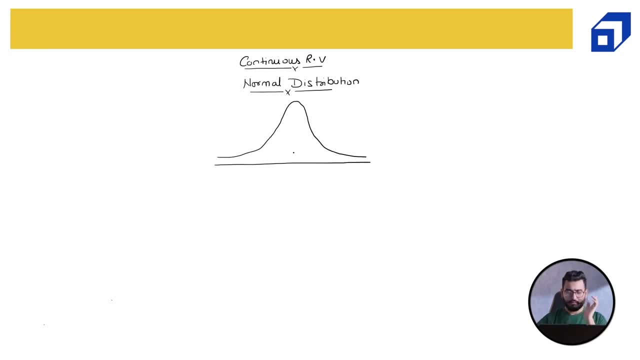 Now, what is the meaning of this? So if I, if I assume that the X axis represents income and the Y axis represents the count or the probability, then within this range, within this range I have highest number or the highest occurrence of the observations. So I have. 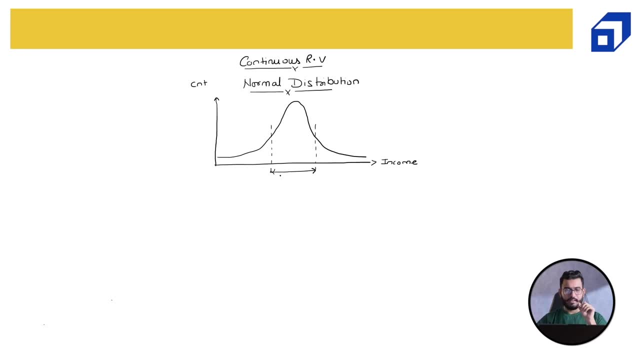 maximum number of people in the in the mid range, in the mid income range. This is known as the center of my distribution. Now, what I have drawn right now is a normal distribution, but in reality, normal distributions can be of variety of shapes. As of now you can see, it is a very symmetrical shape, but in reality, 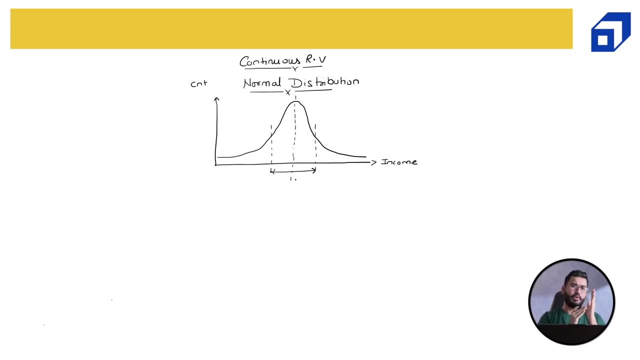 you might get a very symmetrical shape of a normal distribution or you might not get. So, in order to understand whether your data is following our normal distribution or not, we have something known as the standard normal distribution. Now why we have a standard normal distribution. a standard normal distribution will help you. 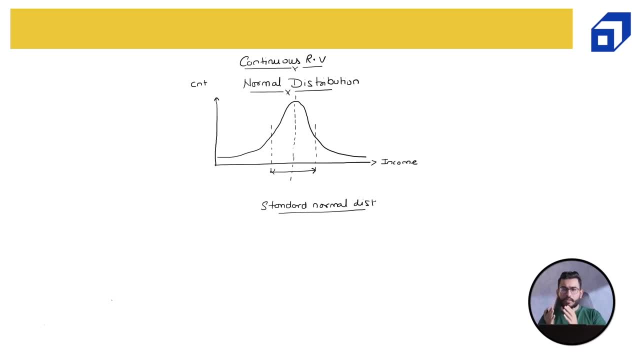 to compare few properties in your original data. So let's first of all, let's first of all understand what is a standard normal distribution, What are the properties of standard normal distribution, And then we will try to compare our data with the standard normal. 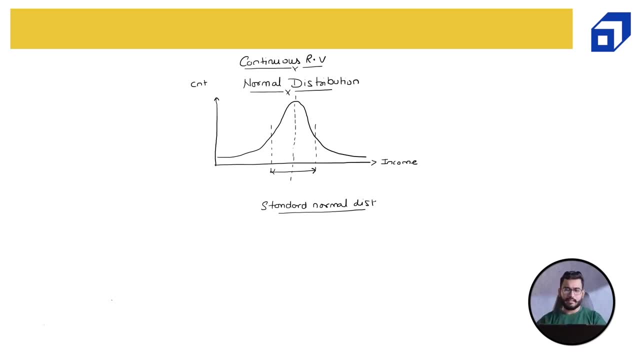 distribution to generate some insights. Let's try to understand the standard normal distribution. Now, here I'm having a particular standard normal distribution. The advantage of standard normal distribution is that it is perfectly symmetrical, which basically means this is my center, This is my center, which basically means this is having the mean, This is my 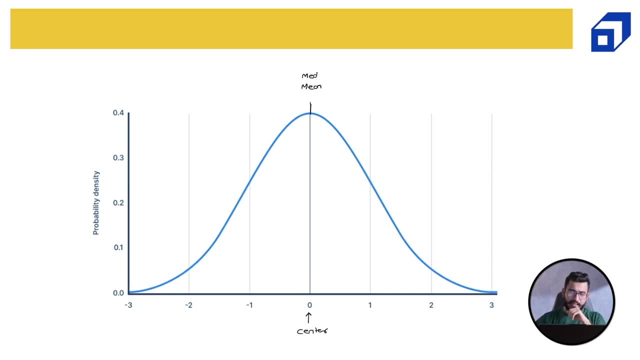 meme point. So mean, median and mode, all the three quantities fall in the center. I'm having 50% data below this, 50% data above this. So it is perfectly symmetrical, Half here in the left side, half here in the right side. Now the numbers. you look into the X-axis. 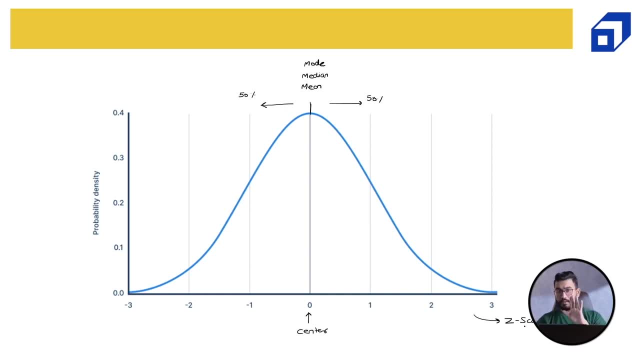 are as the Z scale. We will talk more about it. Don't worry, I will explain you everything. What is Z scale, How we got these numbers? Don't worry, as of now, just try to understand what is the standard normal distribution. So number one is the mean is the mean and. 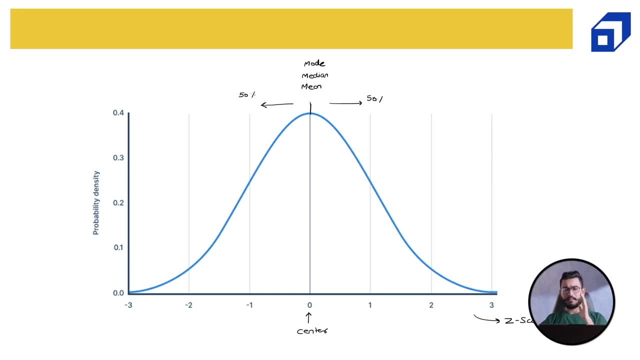 the median and the mode. All these three properties lies in the center. It is perfectly symmetrical: 50% on the left, 50% on the right, which basically means 50% data is on the left, 50% data is. 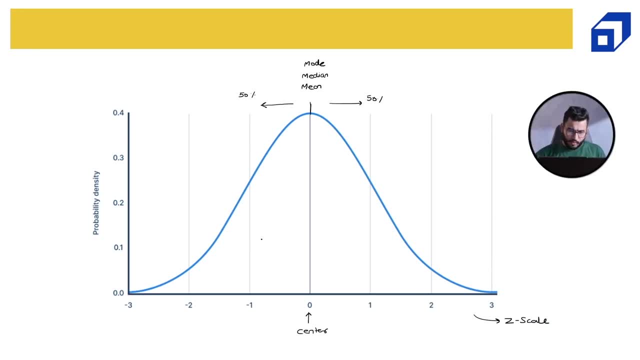 on the right. According to the standard normal distribution distribution property, 68% of the data lies between plus minus one standard deviation, 95% data lies between plus minus two standard deviation and 99.7% data lies between plus minus three standard deviation. 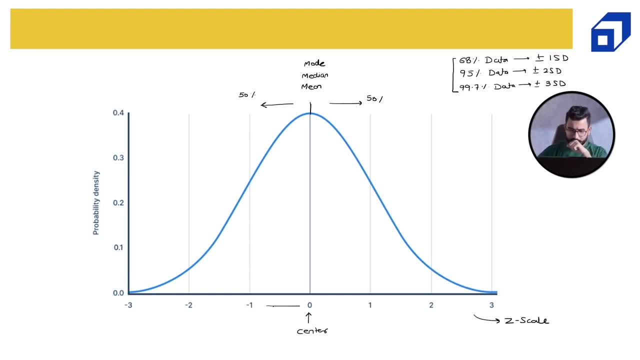 Now, what is this? This is one standard deviation, one standard deviation below, one standard deviation above. So between these two points, I'm having 68% of the data. Between these two points, I'm having 95% of the data, and between these two points, from this point to this point, I'm having 99.7% data. 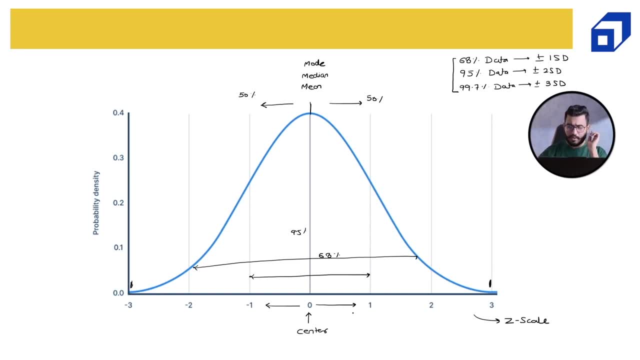 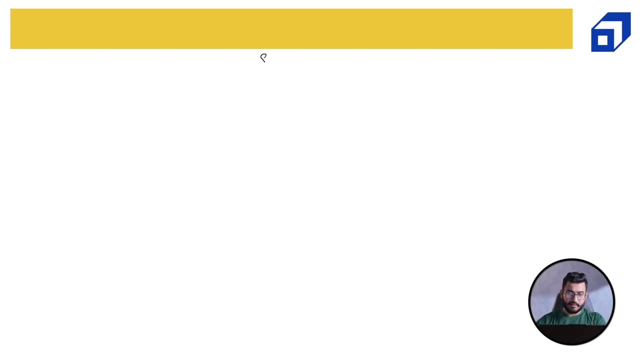 If you're not able to understand how I obtained the Z scale and what I'm talking about in 68,, 95,, 97, let's try to understand it with a real example. First of all, let's try to understand the Z scale. So what is Z scale? For this we have to jump into topic of scaling- Scaling Now. 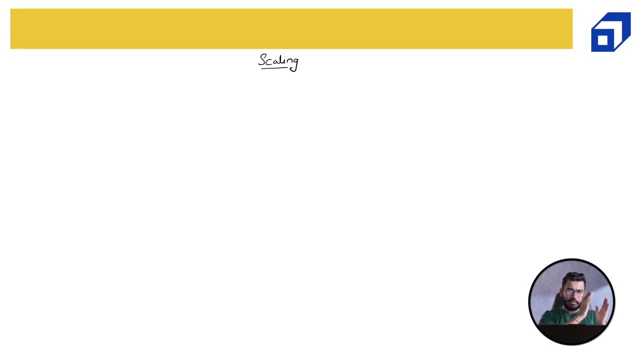 don't worry, We have a topic which we are talking about, which is normal decision distributions. We have talked about standard normal distribution. We have looked into some of the properties, but there is one confusion. The confusion is: what is Z scale and what? 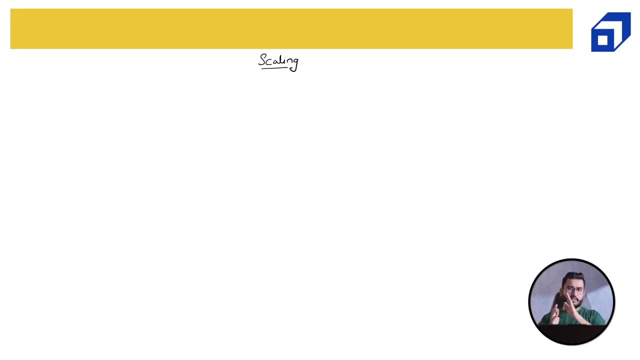 how we have obtained these numbers and what is one standard deviation below, one standard deviation above. So we will pause this topic as of now, just just create a barrier over here. We'll try to understand. this is small topic which is scaling and the Z scale. 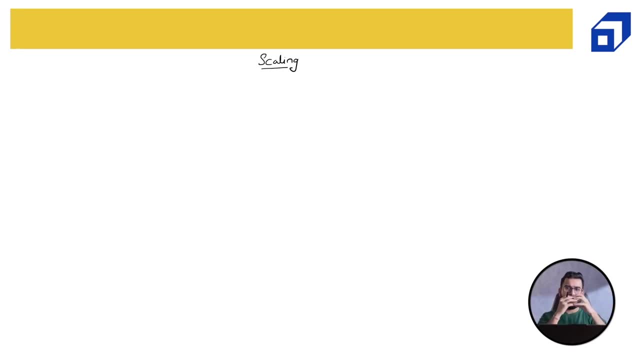 Once we are clear with this, then we will bind everything and you will be very much clear. So stay with me for another 10 minutes and you will be clear with everything. So what is scaling? Now? the problem is: let's say I'm having two variables: age and income. Let's say age is a person is 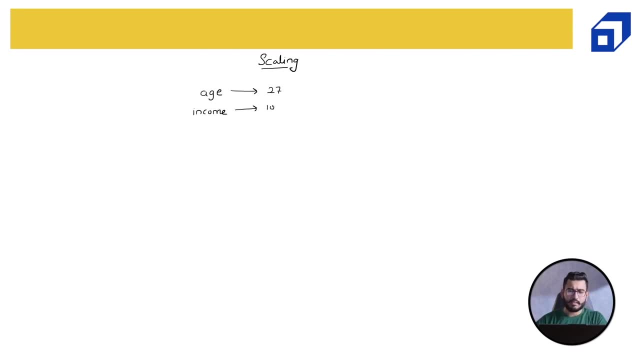 having age of 27 and income of thousand dollars, something like that. Now can I compare these two values? Can I say this is a very low value and this is a very high value? No, essentially we can not. Why, Because both of them are having a different scale. Age isn't. the age is in the scale of year, while 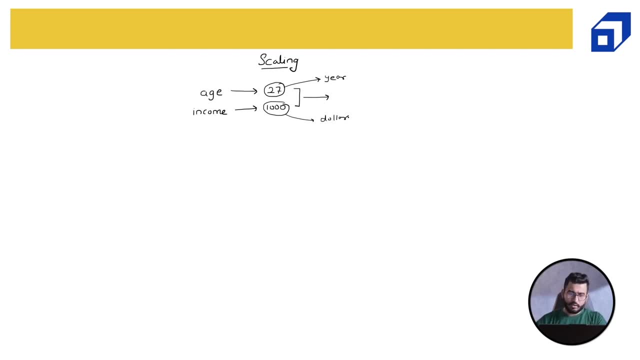 income is in the scale of dollars, So I can not compare these two values. They are, they belong to two different scales and we can not compare them Right. But what? if I want to compare them, then we have to compare them. So what, if I want to compare them, then we have to compare them. 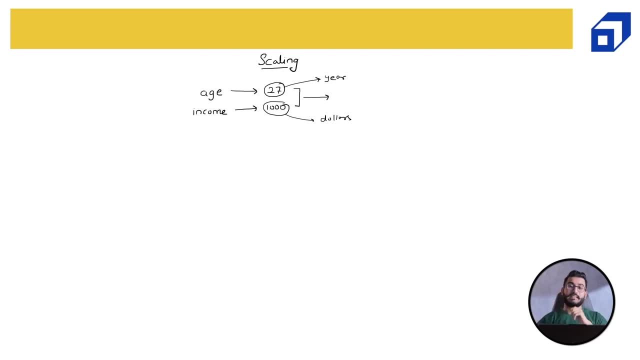 We have to make them into a common scale, right, And that is what scaling is known as. So scaling is a process of converting the data into one common scale using which I can compare various values. There are two common approach which we fall in scaling. One is known as the min max. 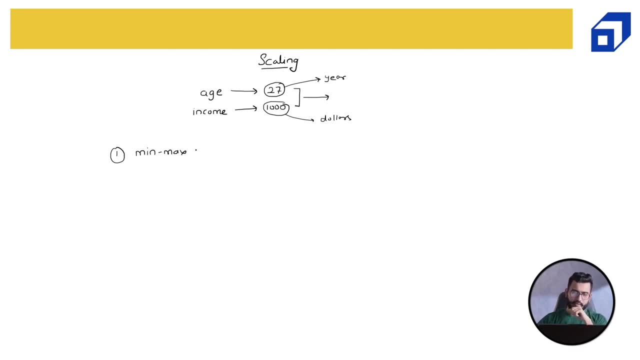 scaling, also known as the normalization scaling. The second one is known as the standardization or the Z scaling, the Z scaling In the min max scaling. I try to convert the complete data into a scale of zero to one where minimum is zero, maximum is one. The formula is very simple: X minus. 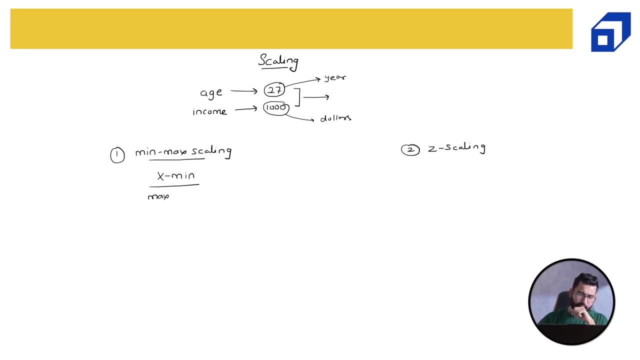 min divided by max minus min. I'll show you. I'll show the show you the example in Excel. As of now, just look into the formula where X is the value I want to convert. So X is zero. So X is zero, So X. 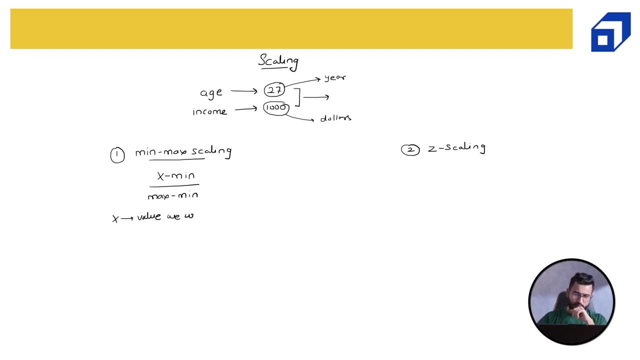 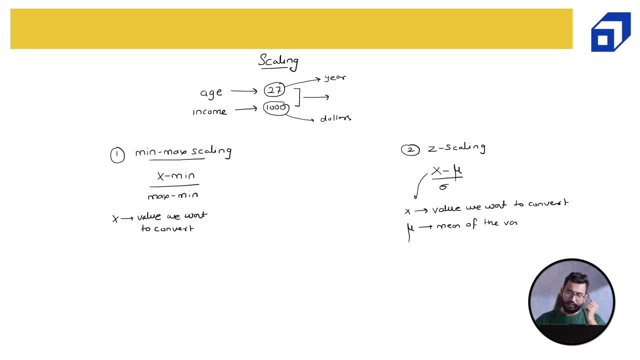 is the mean of the variable And sigma is the standard deviation of the variable. So we have this formula. Now let's try to apply this formula in the actual data in the Excel file, to make sense out of it, And then you guys will be very clear about how we obtained this y axis. This is the major question, right? We have the. 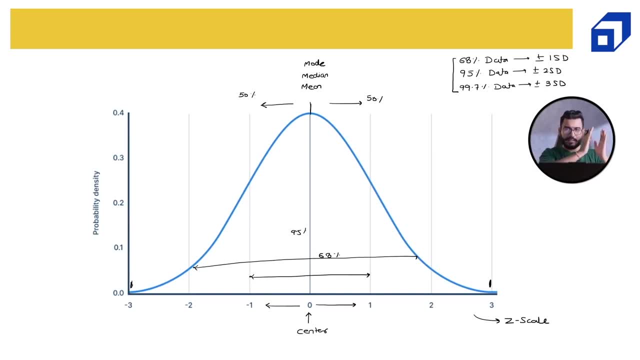 normal distribution, a standard normal distribution topic parked as of now. We are trying to understand the scaling And the main question that we are trying to answer right now is how this Z scale came into picture. And once we are clear with this, then this standard normal distribution. 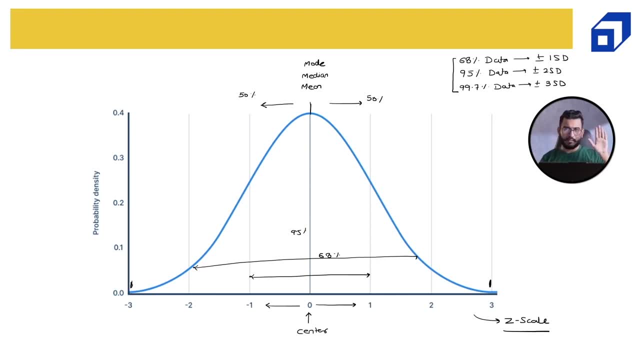 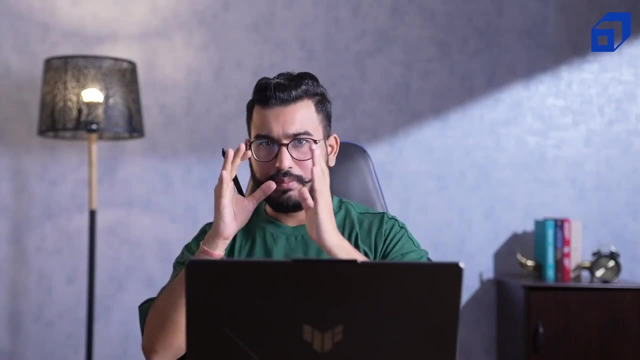 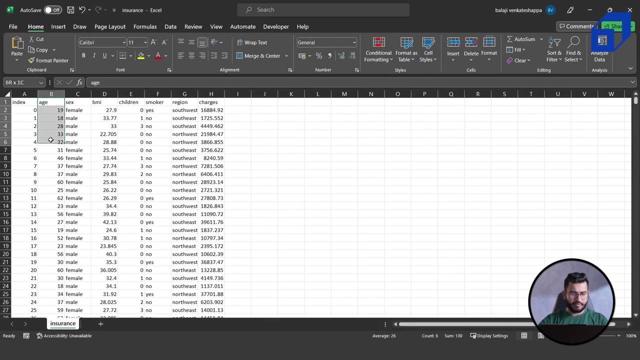 will make more sense to you, right? So keep this topic parked. We are talking about this topic And now we are moving forward to understand the scaling topic in Excel with particularly a data example. So let's do this Now. here you can see, we have a data which is having age: BMI. 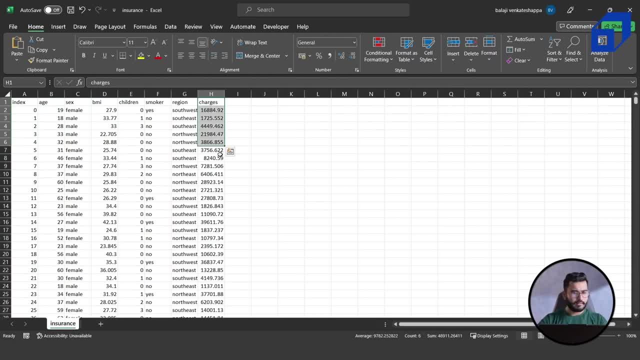 and charges the insurance charges. I cannot say that this value is very low. This value is middle and this value is very, very, very high. Why? Because age is in year. BMI is in kg per meter square. If you know, BMI unit is kg per meter square and charges are in year. So this is. 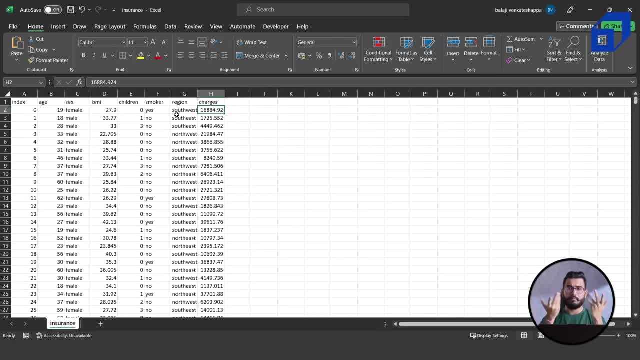 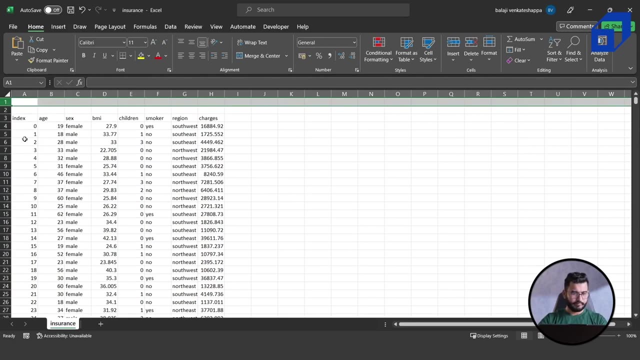 the minimum value, And these three are in dollars. These all three are in different scale. I cannot compare them right. Let's try to use min max scaling. So for min max scaling I need the minimum value. So let me insert quickly some rows. So let's say: here I'm having minimum maximum. 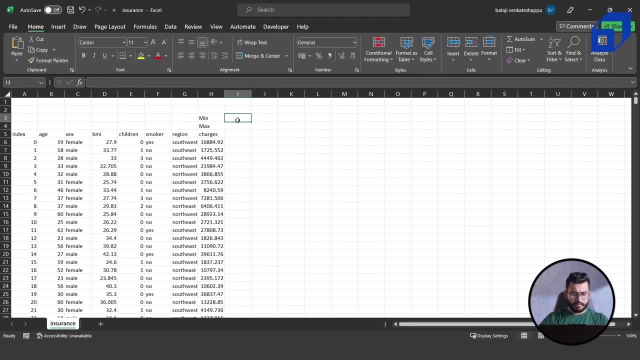 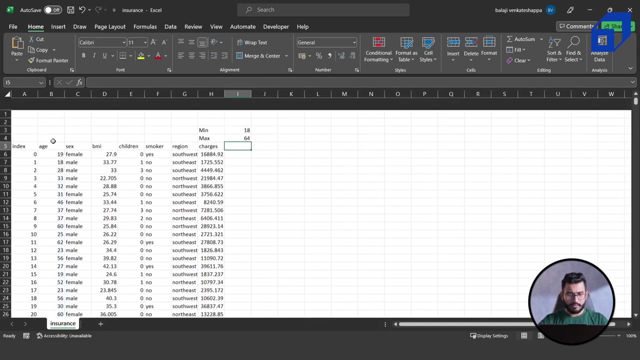 So I'm kind, I'm just calculating the minimum for age, or sorry, is equal to the minimum of the column age. So I'm having the minimum value to be 18, then calculate the maximum of the column age. The maximum value is 64.. Similarly, I'll call this column as age Underscore. 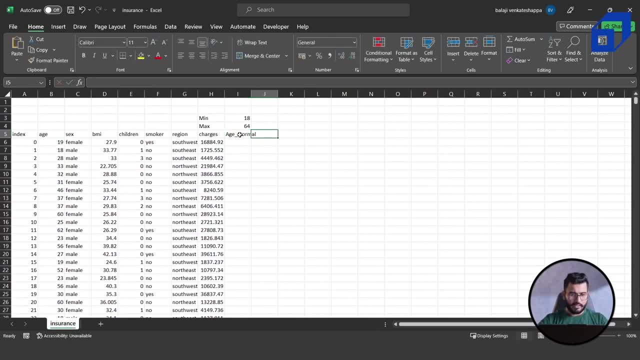 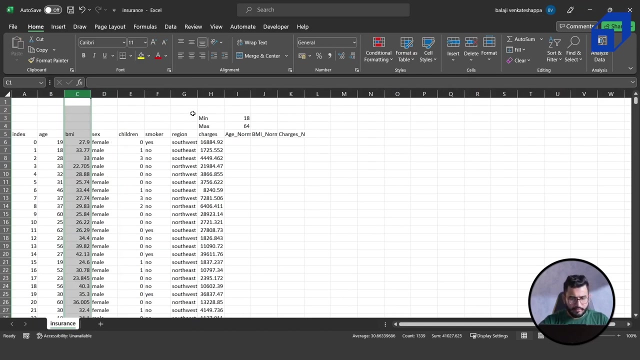 Similarly, I'll do it for BMI- BMI underscore normal- and then for charges- charge underscore N. I'll just find out the. so let's quickly do one thing: Let's shift these columns. Let's shift this column also, so that I can simply just 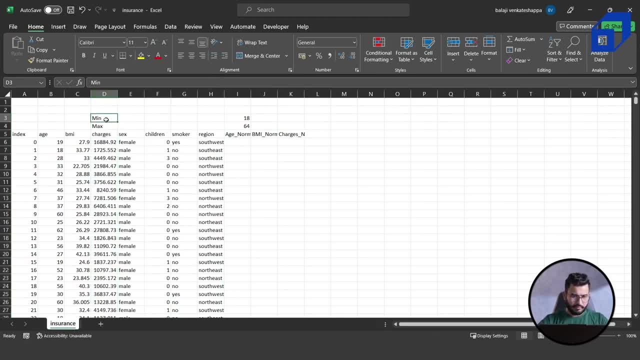 extend the formula and I do not have to write it again and again. Now, if I just simply extend this formula, I get the minimum of age, BMI and charges and this will give me the maximum of age, BMI and charges, because age, BMI and charges are one after the other. 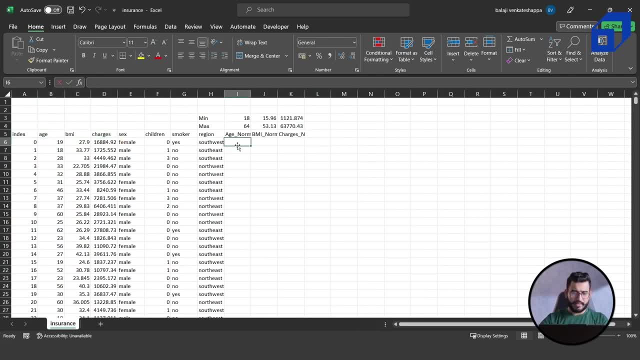 So I just extended the formula. right Now, let's apply the formula. it is equal to X, which is this value I want to convert, minus minimum. So I'll just freeze this value. So I want, I will put a dollar. 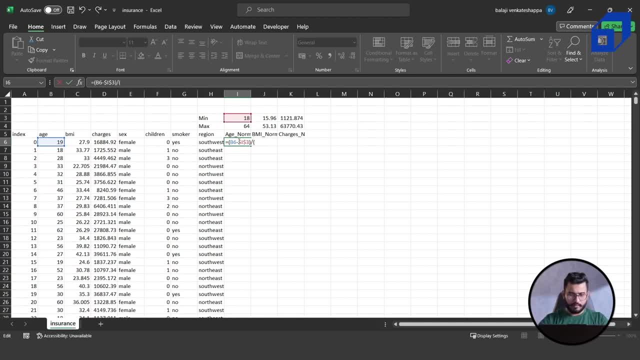 X minus min, divided by the value of max and then minus and then min, And I will put: change $ K. take what is jorn orange, correct, Okay, Okay. so let's do one thing: let's not freeze i, so that if i extend the formula this is not getting. 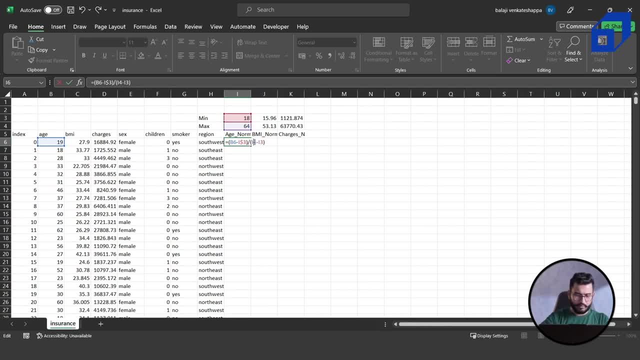 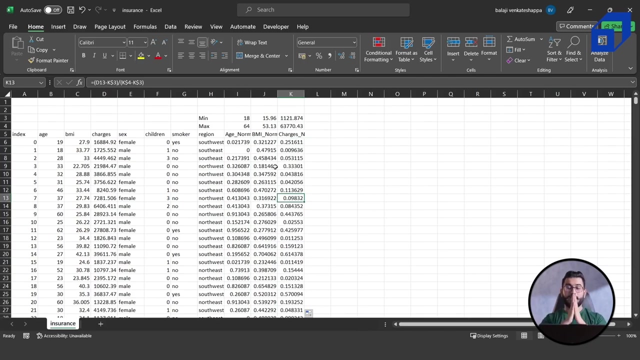 fixated. i'll just fix the row dollar four and dollar three and let's enter, let's try to apply it on the entire column and let's try to extend it to bmi and charges also, and let's try to extend it to all the rows now. now, all these three columns are in a scale where minimum is zero, maximum is one. 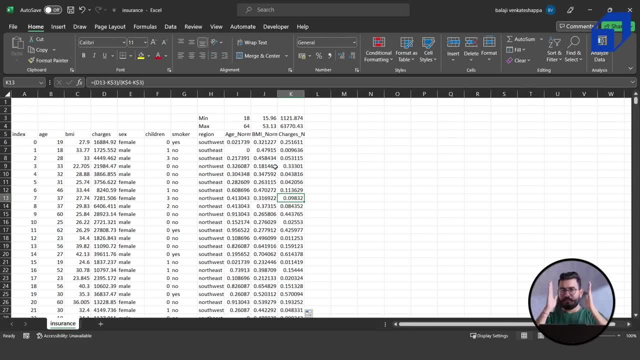 so assume that you have a number line: minimum is zero, maximum is one. now the middle point will be point five, so the mean is point five. so any value which is close to zero, you can assume that the value is close to zero. and let's try to extend it to all the rows now. now, all these three columns. 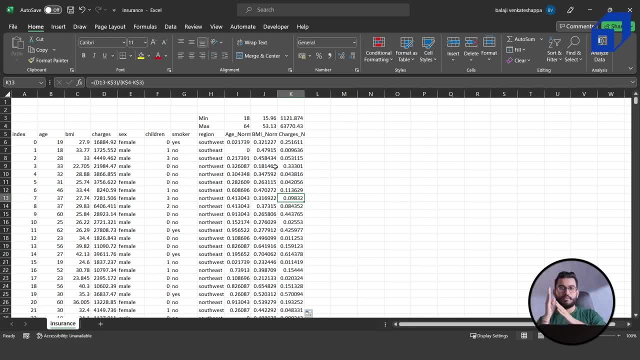 value is very low. Any value which is close to one, you can assume that the value is very high. Any value which is around 0.5 is the average value. right Now the scale is very clean and all these three columns- age, BMI and charges- are now in this scale: the normalized 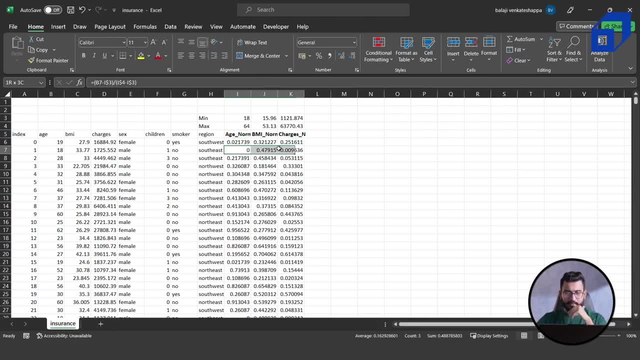 scale. Let's try to compare the value. If I look at this person, the age of this person is zero, which basically means this person is the person who is having the lowest age. in my data, The age is zero means the person is having the lowest age, the minimum age. 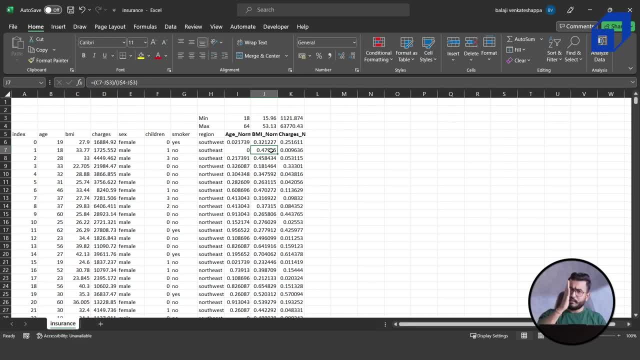 Then 0.47 is the BMI, which basically means the BMI is around. mean, As I told you, 0.5 is the middle, 0.47 is near to 0.5, right? So BMI is around average, While the charges. 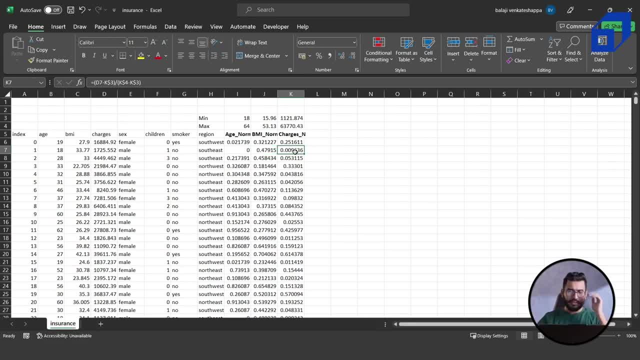 are zero. BMI is around average. So BMI is around average, While the charges are zero- 0.009, which is very close to zero, right? So what I can conclude for this person? this person is a young person, very young, having average BMI and very low charges. right, Let's. 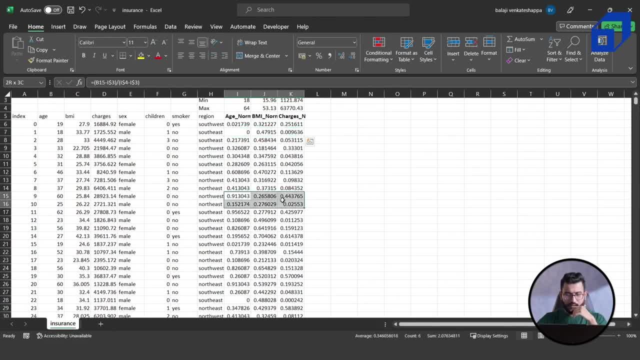 take one more person, Let's say this person. the age is 0.91, which is close to one right. 0.91 is close to one, So age is 0.91.. BMI is 0.26, close to one, So BMI is close to. 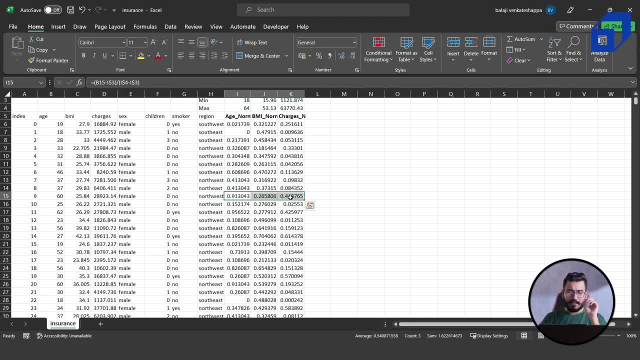 one 0.1, so 0.26.. And then charges are 0.4, which is close to the middle value. So if I talk about this person, this person is having very high age, not very high BMI. So BMI is. 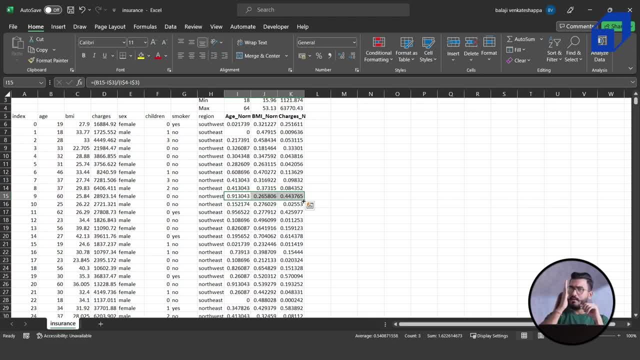 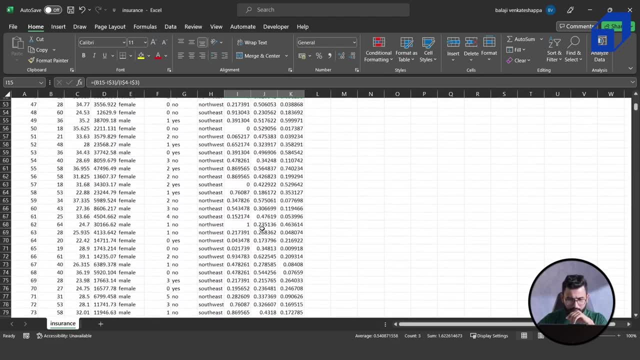 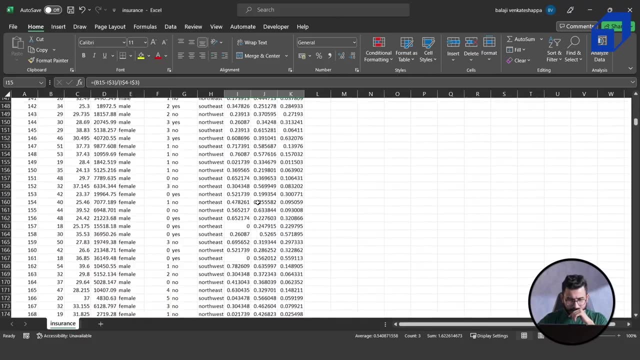 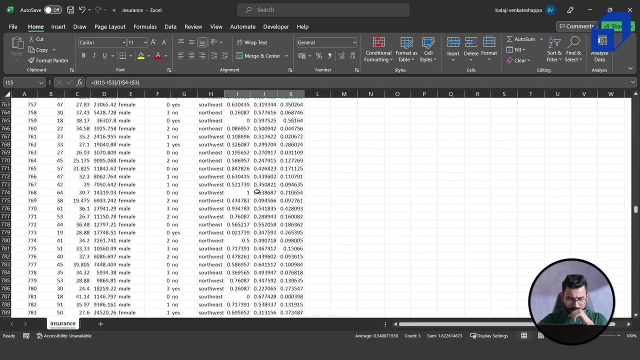 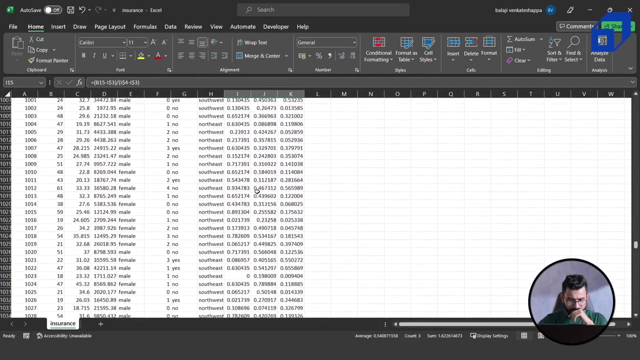 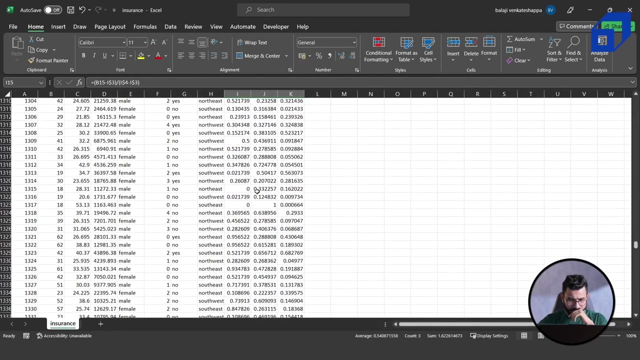 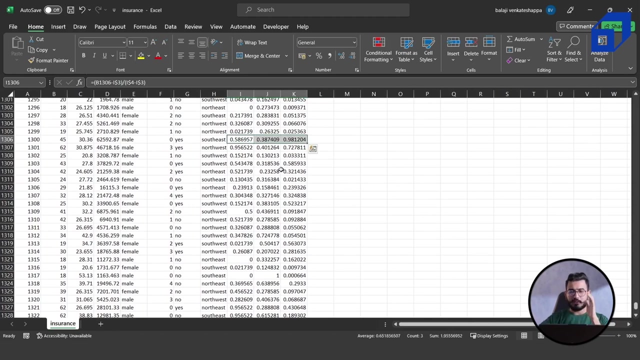 below average, but charges are around average. right, Let's talk about a person who can be a outlier or something. Let's see if I can find out some interesting value so that it makes some real sense. Okay, If I look at this person, this person is having 0.5 as age, middle age. the BMI is 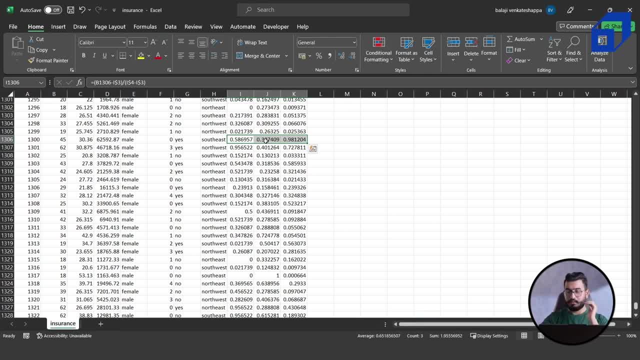 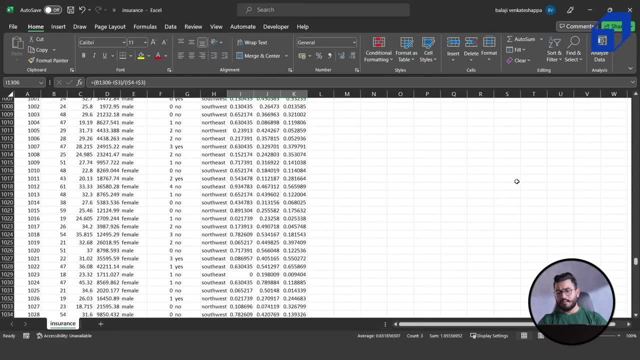 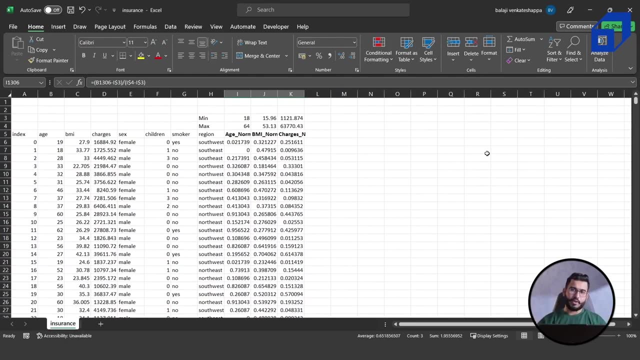 for this person is below average, but the charges are very high for this person. You can see this person right, So I hope now you guys are able to understand how to read values in a normal scale. The normal means minimum is zero, maximum is one And the formula is x minus min divided. 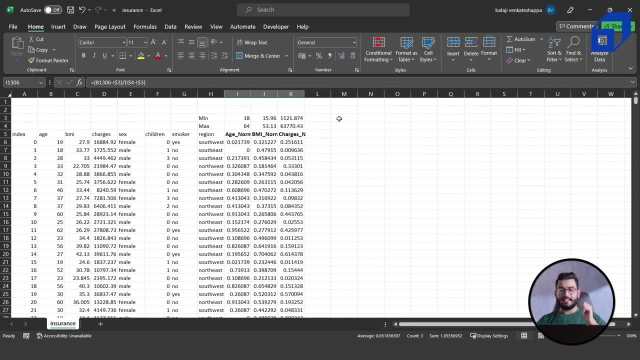 by max minus min. Hmm, Yeah, The reason why does it cut out? Okay, Okay, scaling, which is a standardization. we need the average, we need the standard deviation, And once I do this, let's do this first of all. So this will be my 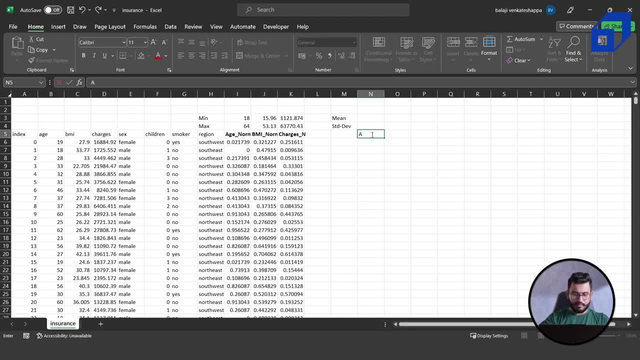 age-z, and this will be my BMI-z and then charges-z. Now let's apply. the formula is equal to. so first of all we have to calculate. the mean is equal to average. I need average of the age column. I will just extend this formula to the next cell, next two cells. 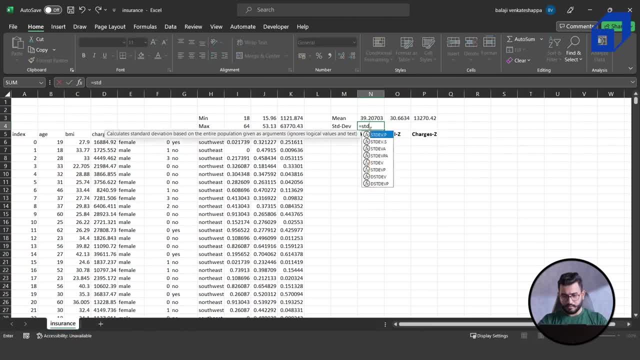 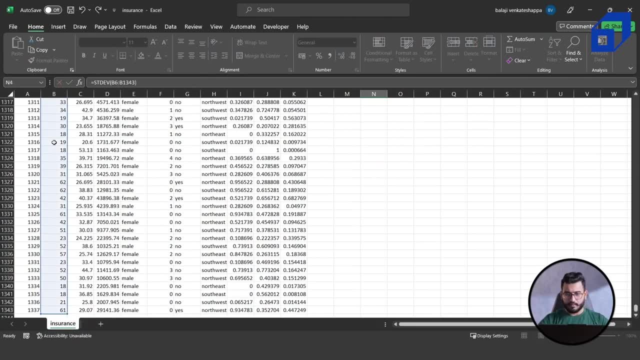 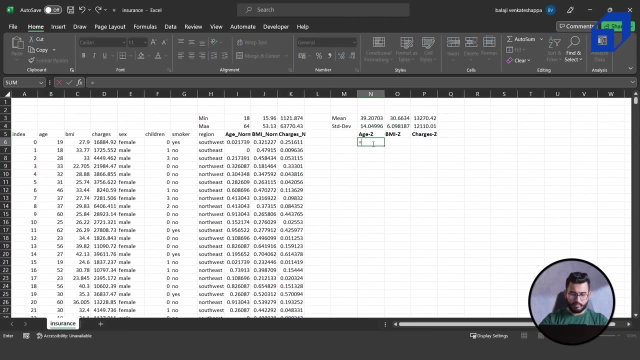 Then I need the standard deviation. So I'll just use this standard deviation of the BMI age column. Then I will extend this to the next cell And now we will apply: the formula is equal to X. X minus mean, so X minus mean, and I will again just freeze the row X minus mean. 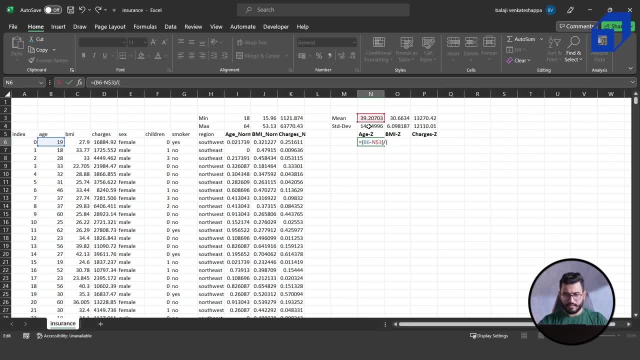 divided by standard deviation. This is my standard deviation. I will freeze the row and enter. Now let's extend it to all the rows. I don't know why it's not happening. Let me try it one more time. Okay, I don't know why it's not happening, So I have to do it manually. 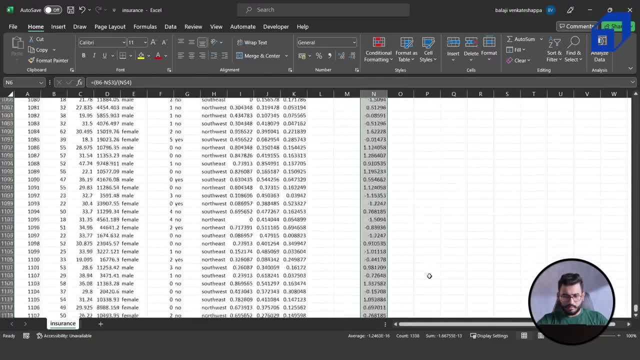 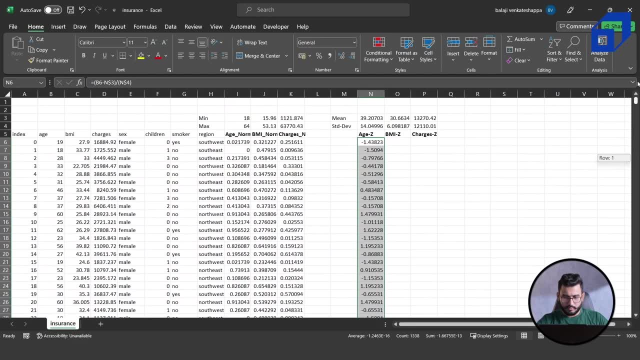 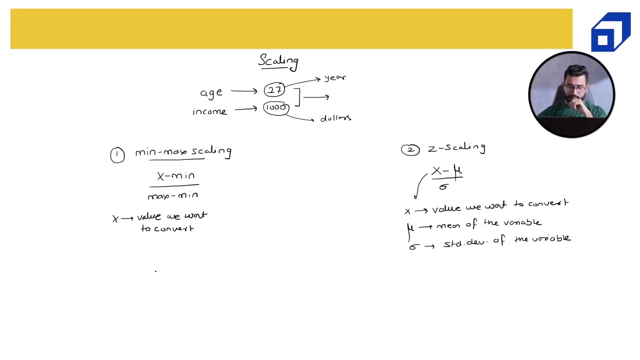 And then I will extend this formula to the next column also. So let's do it like this, And this one also. Okay, Now in the Z scale, in the Z scaling, my middle point is zero, Then I'm having minus one, minus two over here, plus one plus two and plus three over here. 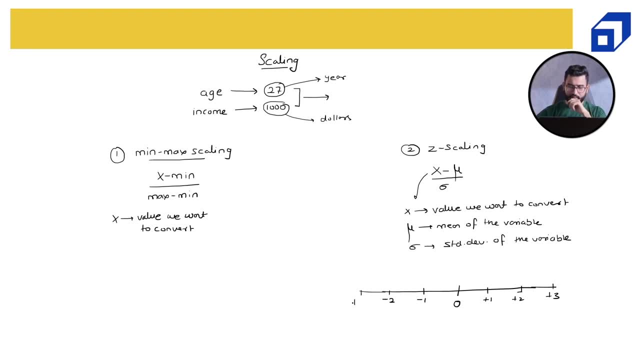 And minus three over here. What are these values? These are known as my standard deviation. this is my mean. So standardization or Z scaling, will convert your data in such a way that now the data is having a mean of zero and the standard deviation of 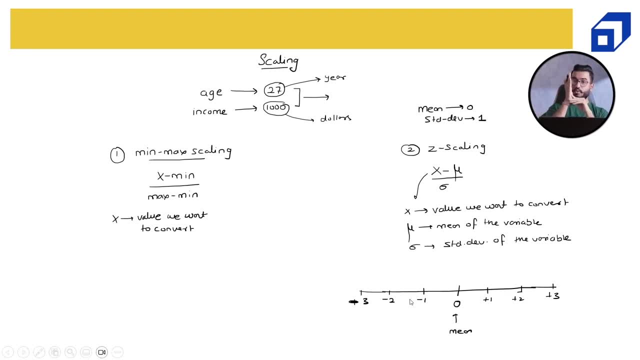 one. So if you get a value close to zero, that basically means you are an average. If you go on the positive side you are moving above average, and the higher you move, that many standard deviations you are above the average. So let's say the value is plus 1.2,. 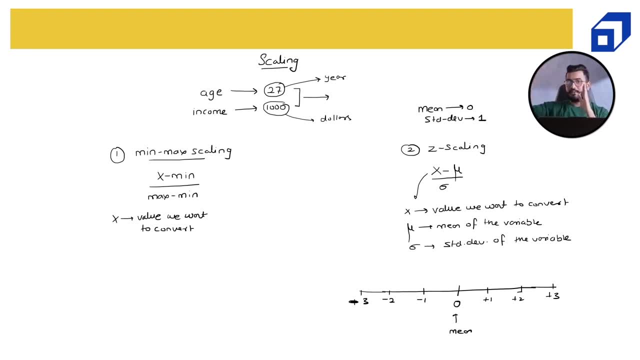 which basically means you are one standard deviation above the average. If, let's say, the value is minus three, that basically means you are three standard deviations below the average. So Z scaling will convert your complete data into a scale where the set enter becomes zero, The mean becomes zero and the standard division becomes one unit. 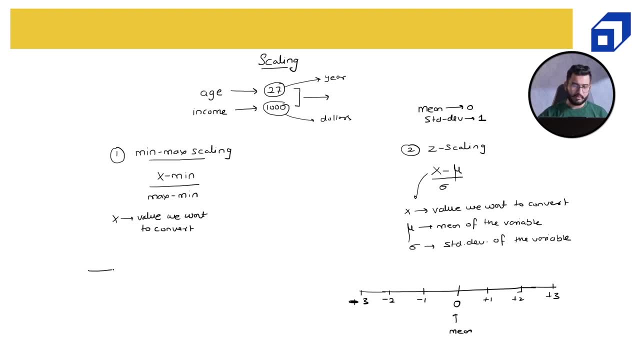 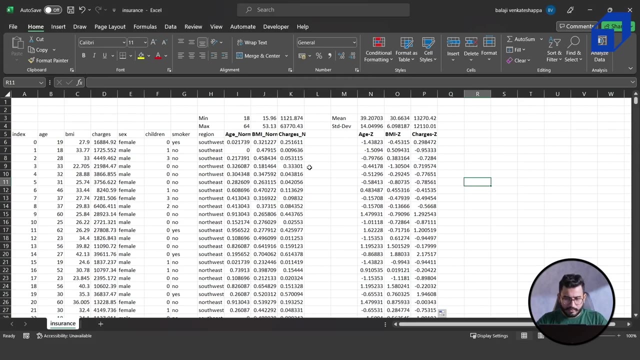 one unit on either side For min max scaling. it was something like this: 0, 1 and middle is 0.5.. Right, Let's quickly compare it and try to check the Z scale. So here, if I look into this person, this person is having BMI of 0.5. 0.5 means very close to zero, right. 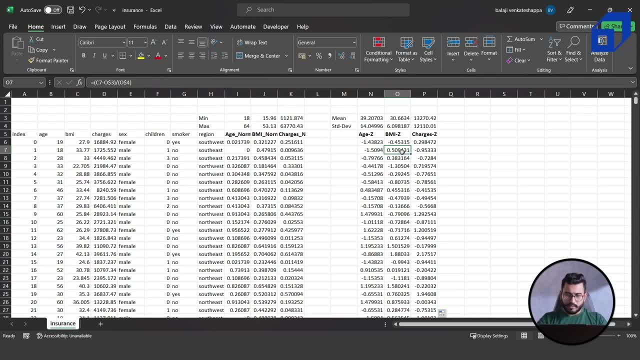 So zero is the middle, 0.5 is very close to zero. Then minus 1.5 is the age, which basically means from zero the person is 1.5 standard deviation below the mean, then minus 0.9 charges. 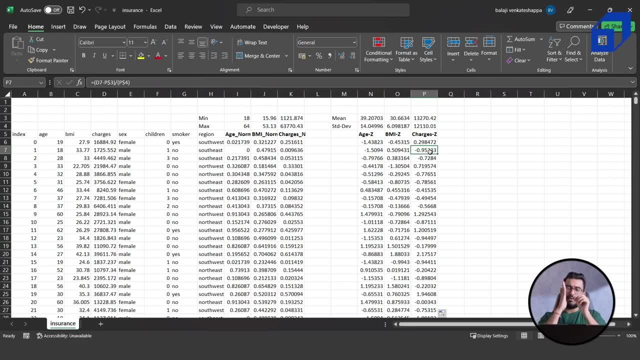 from the mean. The person is 1.9 is standard deviation below the mean. So this person is having normal BMI because the value is close to zero, very low age and very low charges because both the values are on the negative side. So you can see that with standardization- since I'm having positive, 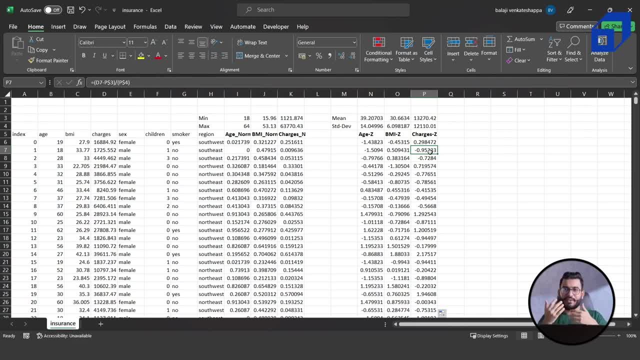 negative sign and middle is zero, it becomes very easy for interpretation. If the value is positive, I know this is above average. If the value is negative, I know this is below average. If the value is positive, which basically means it is close to zero. That is the advantage. 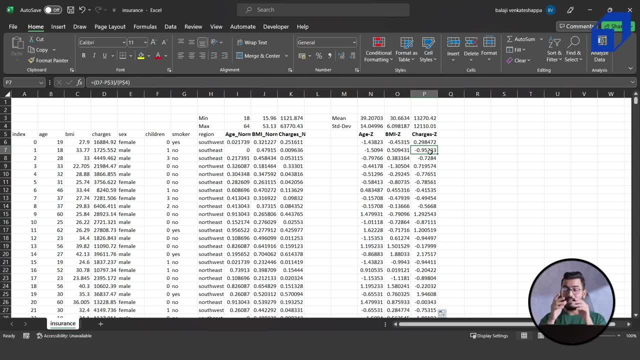 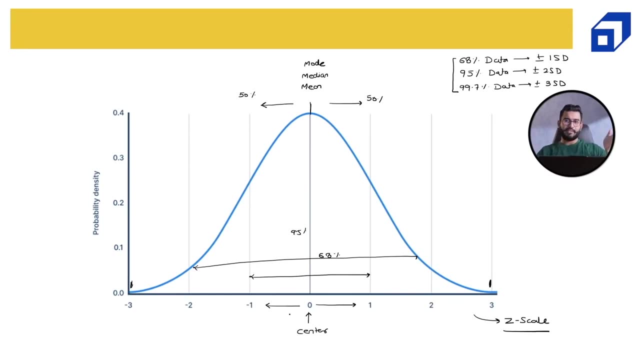 of standardization. Now this is the Z scale which you guys can find out in my standard normal distribution. So if I go back to my standard normal distribution, this is what the Z scale is. So the middle is zero. I have one standard deviation below the mean one. 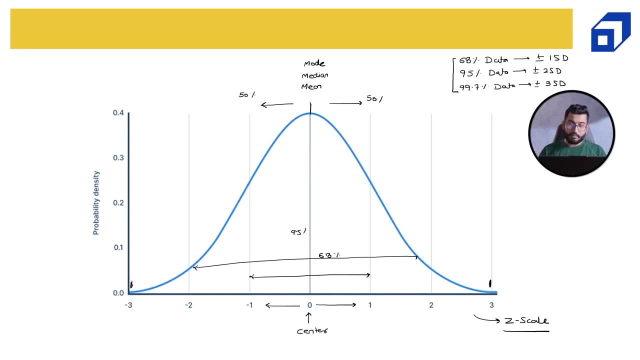 standard deviation above the mean, and so on. Now, according to the property of a standard normal distribution, It states that 68% of the data is plus minus one standard deviation above or below the mean. 95% data is plus minus two standard deviation. 99.7% data is plus minus three standard deviation. 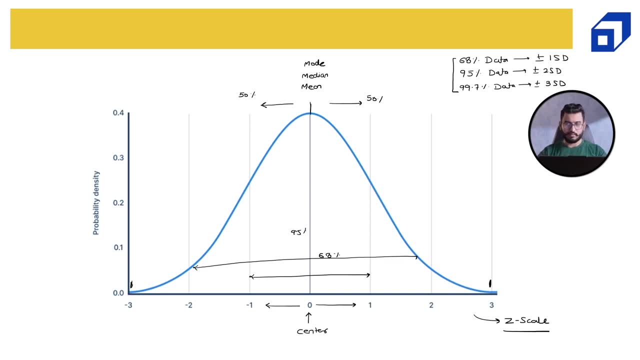 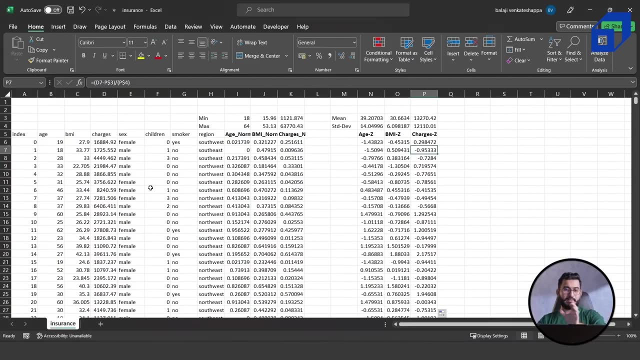 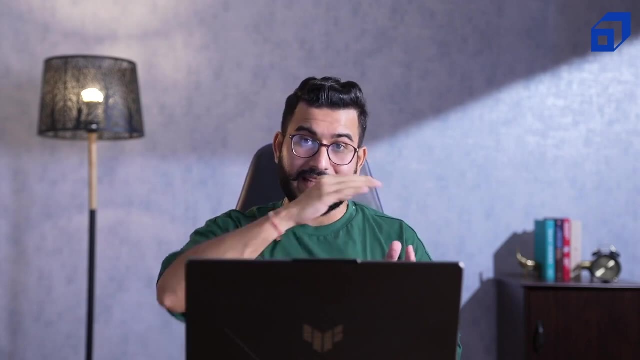 Let's try to quickly prove it. Let's let me prove it. for that, First of all, we have to check which particular column among age, BMI and charges follow normal distribution. So I already know that BMI follows a normal distribution, which basically mean when a 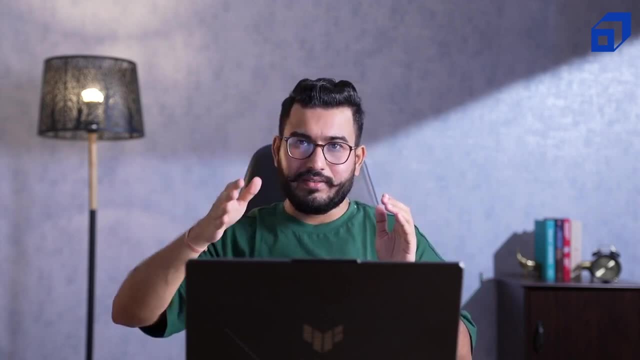 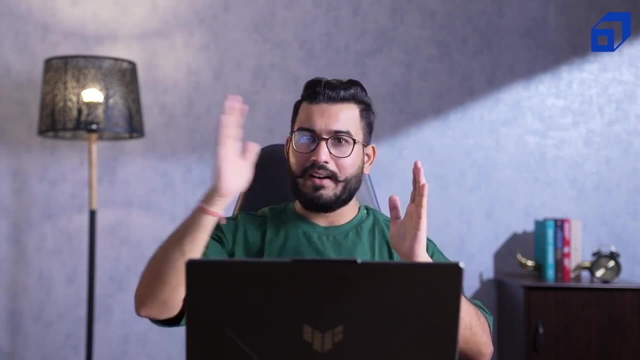 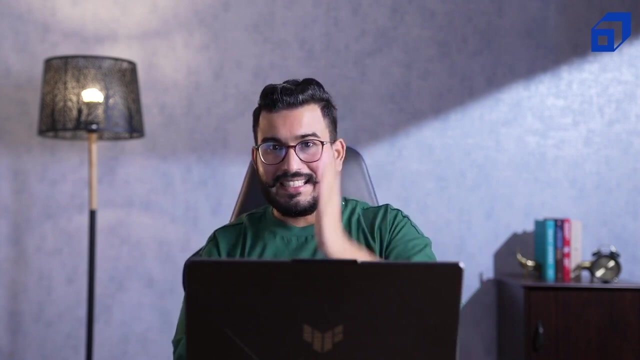 lot it. it would resemble a normal curve, a bell shaped curve, which is symmetrical. you will get half data from below the centre and half data above the centre. And since I have converted the BMI column completely into a Z scale or standard scale, 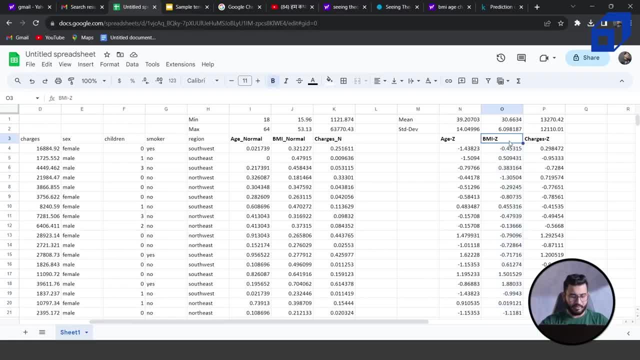 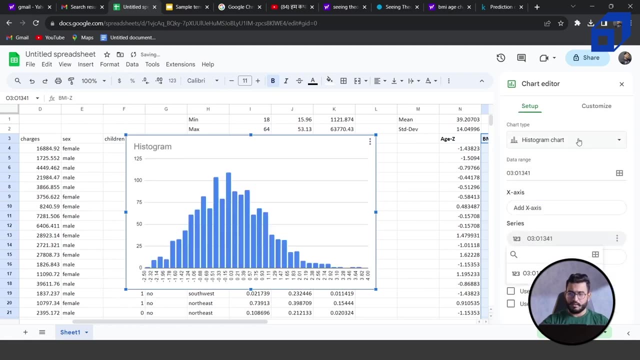 Now just see the magic. I have selected the BMI column And now we will go to the insert option in this Google sheets, go to chart and we will select the histogram. Now, if you closely observe this histogram, you can see that this: 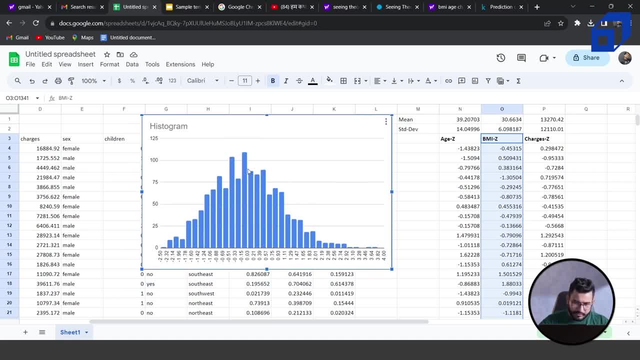 point is the center, 0.03 is the center, and below this value, I'm having negative points. above this value, I'm having positive points. Now you can see that the data is spread around minus two standard deviation, which basically means below- uh it will. it is distributed. 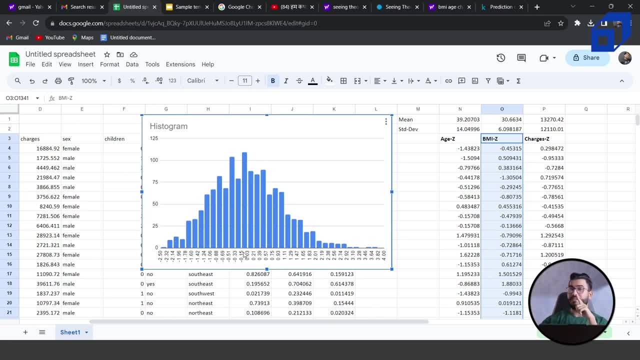 to standard deviation below the mean and four standard divisions above the mean. Now you can. you can see that it is not perfectly distributed to standard deviation below for a standard division above. So here I'm having less data, here I'm having more data, or the. 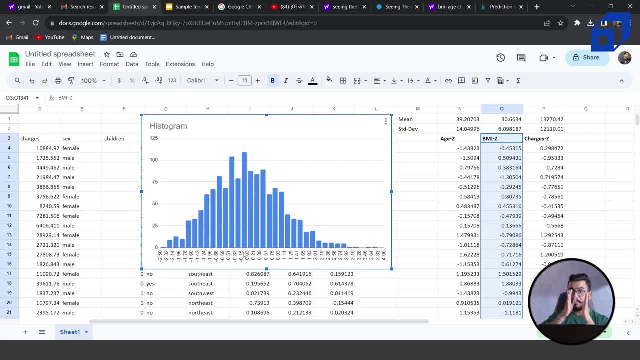 spread. It is more on this side, the positive side. This is one thing we can understand. This is a normal distribution, but this is not standard normal. So in order to compare this distribution with something, we need a standard thing, right, Let's say, if I have to compare, 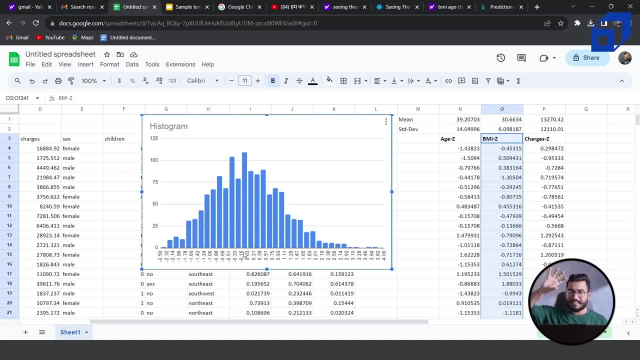 my performance in any exam, I need some standard score right. Standard score is hundred, So maximum is hundred, The best is hundred. So whenever we try to compare something, we need a standard right. Similarly, in order to compare the distribution of a continuous random variable, which appears to be normal, 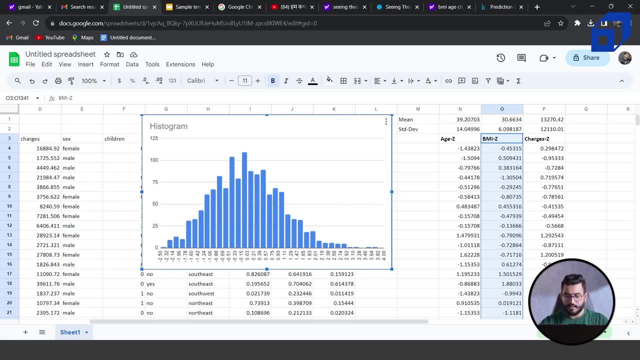 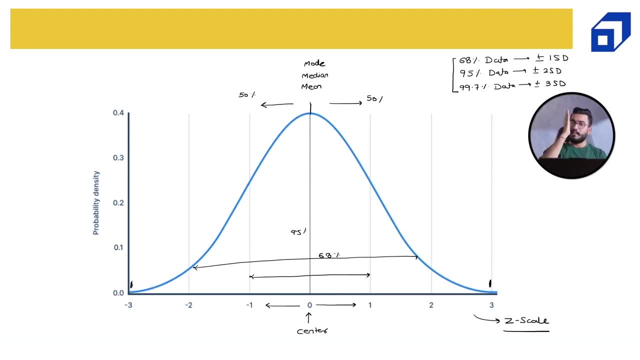 I need a standard normal distribution And this is where my standard normal distribution comes into picture. This is my standard normal distribution, or standard normal distribution says that your mean, median and more will lie in the center. And if it is not lying in the center, if your mean is not equal to mode, is not equal to median, your distribution. 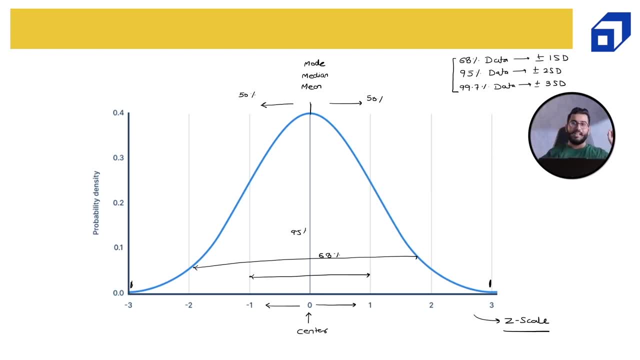 is not a standard normal distribution. It will be either left skewed or right skewed. These are the two terms which I'm introducing. I will explain to you as we move forward, Don't worry. But as of now we are trying to understand the properties of normal distribution. 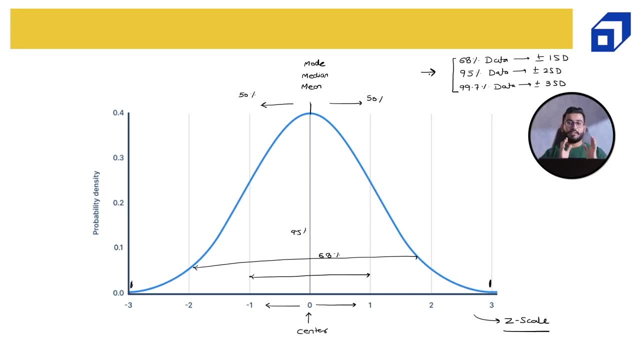 And here I've already written the three properties, which is 68% of the data lies across one mind plus minus one standard deviation above or below the mean. Similarly, in 99.9% of the 95% to standard deviation above or below the mean and 99.7% data lies across plus minus. 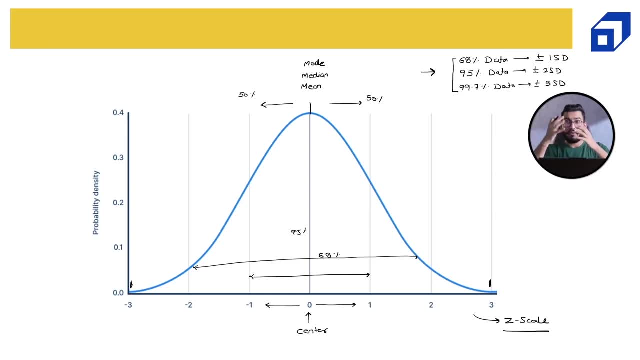 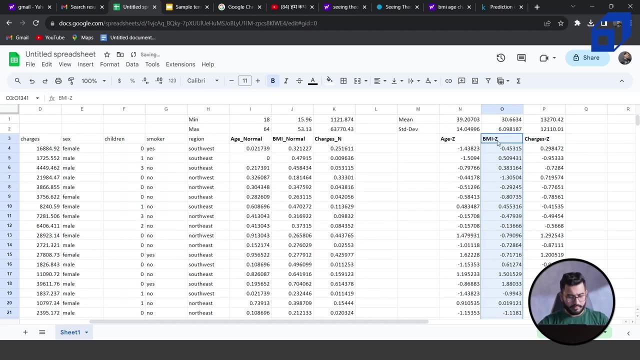 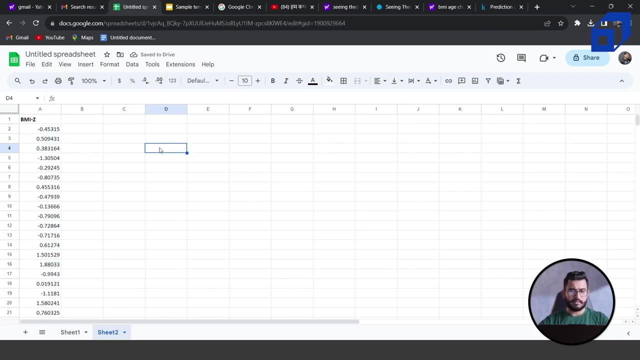 three standard deviation right Now. what we are going to do, we are going to quickly prove it. So here we have the data. I'll just quickly close this. I'll copy this data into a new sheet over here. Now we will calculate the mean, median and mode And, for simplicity, 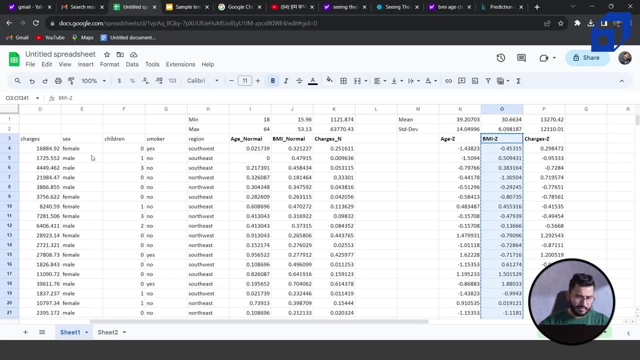 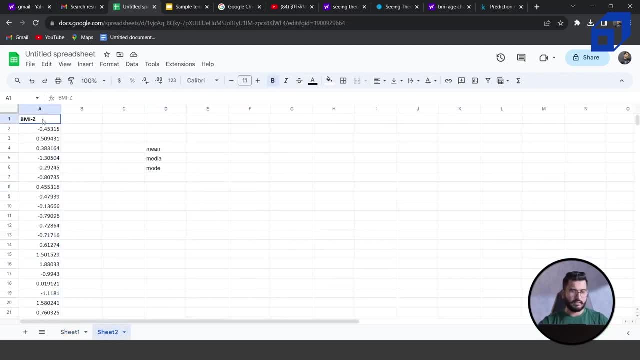 purpose. let's not use the Z scale, let's use the original scale, so that you guys are able to understand this. So I'll just replace this column with the original data: BMI. What is the average? BMI is equal to average of this column. What is the median? So, median. 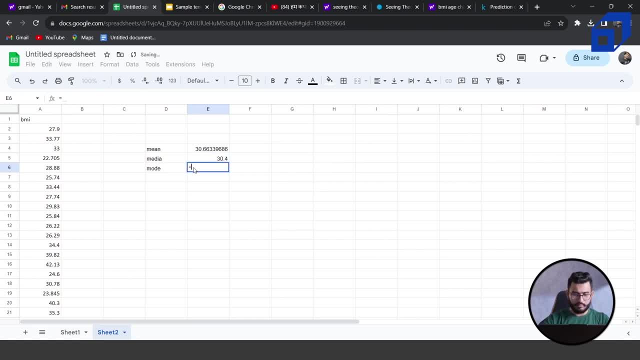 of this column and what is the mode and mode of this column? And here we have. so now you can see that mean is 30.6,, median is 30.4, mode is 32.3.. These values are approximately close to each other, not exactly the same. So first impression about this distribution: 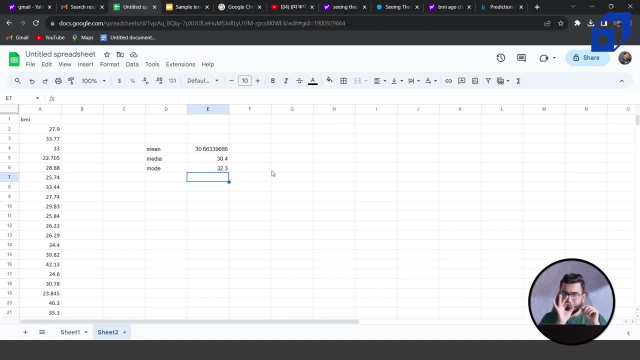 is that it is not standard normal distribution, but it's something close to standard, right, But how much close? Let's try to understand that. First we will prove the property. The property is that 68% of the data falls across. 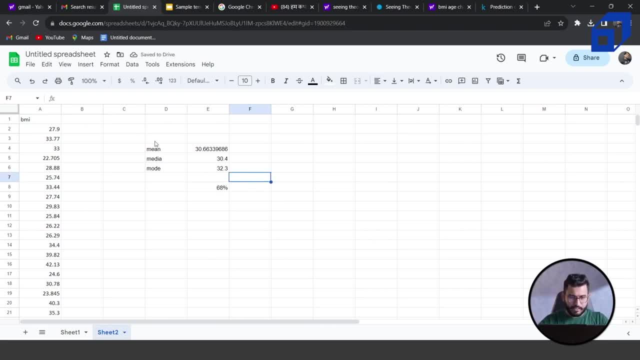 plus minus one is standard deviation, right? So let's quickly find out the standard deviation. So STD DEF is equal to STD. So this is my standard deviation of this data. It is 6.09 standard deviation If I go plus one standard deviation below the mean. so let me create. 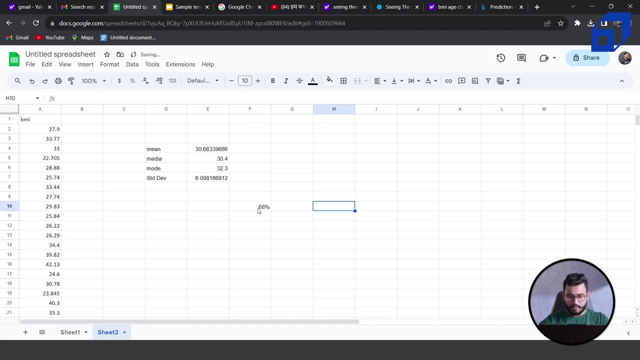 a table over here: 68% I go. so this is my mean minus. Let's say this is my lower limit, This is my upper limit. I'll explain you everything. Don't worry, Don't get overwhelmed. And this is my count, This is my total, And let's write. 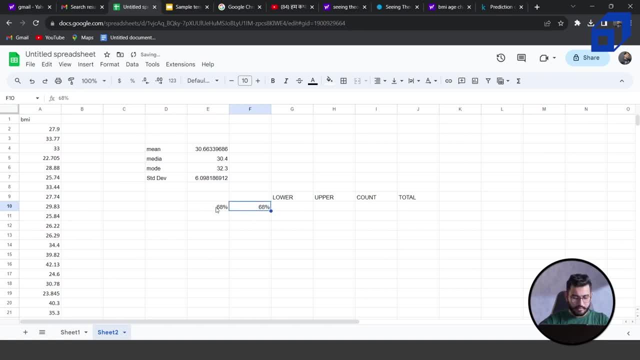 68% over here, And this is mean, So one is standard deviation. So now what we are going to do? we are going to take mean and subtract: one is standard deviation, So one is standard deviation. So mean minus one is standard deviation. The 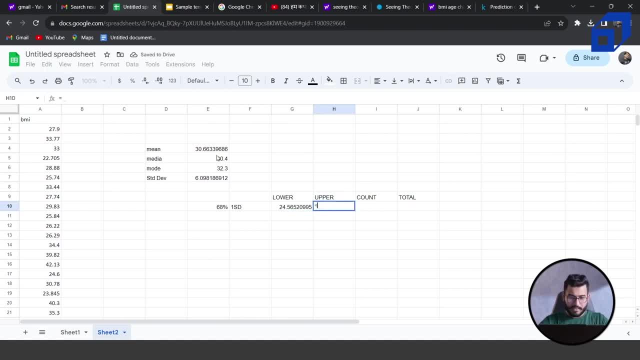 lower limit is 24.5.. Then mean plus one is standard deviation. The upper limit is 36.. Now I will count how many values are falling in this range, because my objective is to find out the percentage. So I'll quickly apply this. 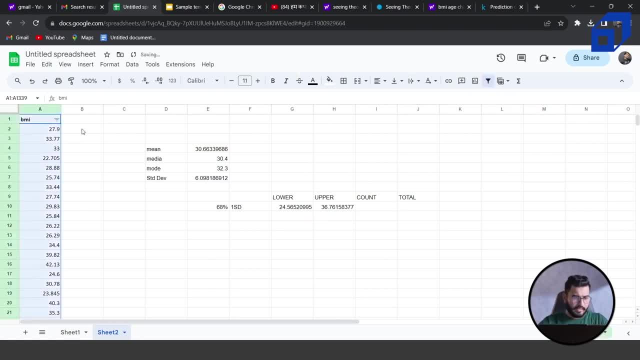 Okay, So I'll apply a filter over here and I will create a filter by condition, And my condition is: is between: is between: the lower value is 24.5 and upper limit is 36.7.. And I'll just quickly create a filter. Now, I'll just simply count it. 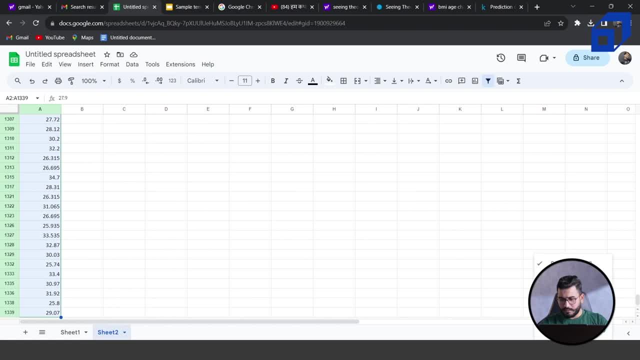 If you carefully look over here, the count is 900.. So there are 900 values. that falls in this range. What are the total number of values? for that? I have to remove this filter, So I'll say none, I'll say okay And I will calculate. So 1,338 is my total. So 1,338.. 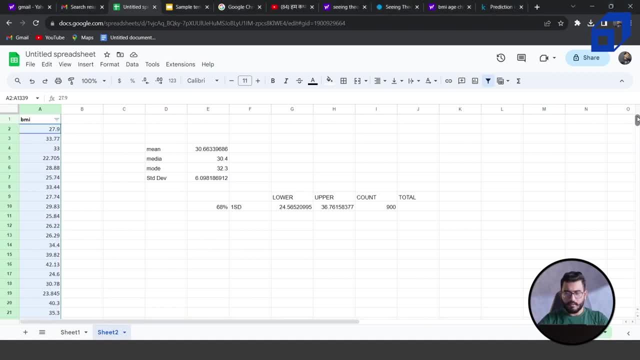 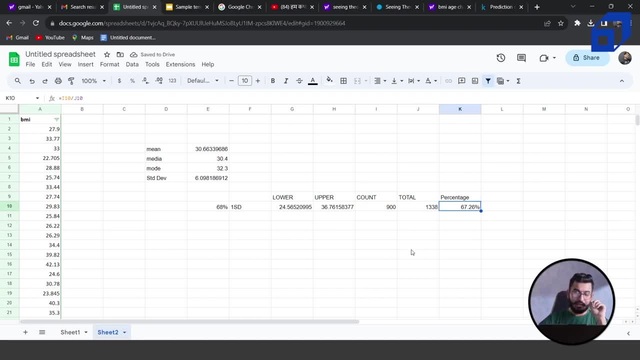 this into percentage. it is 67.2%. The standard value is 68%. My data- My data- is resulting in 67.2%. This is the first proof of the first property. The first property says that 68% data lies. 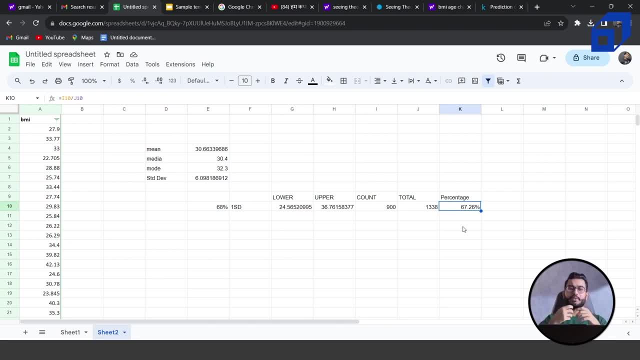 between plus minus one is standard deviation. I'm getting 67.2 because it is not a standard normal right. The second property is 95%. So 95% data lies between plus minus two standard deviation. Let's check the lower limit. So is equal to mean minus. 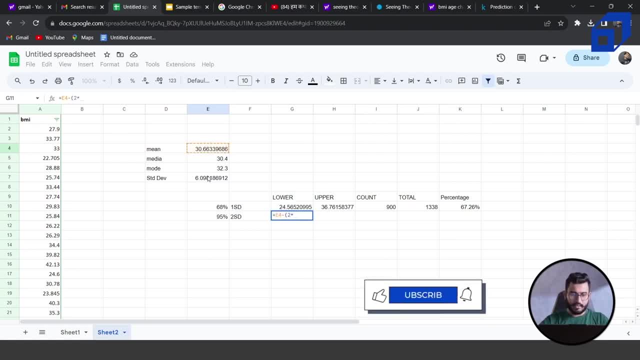 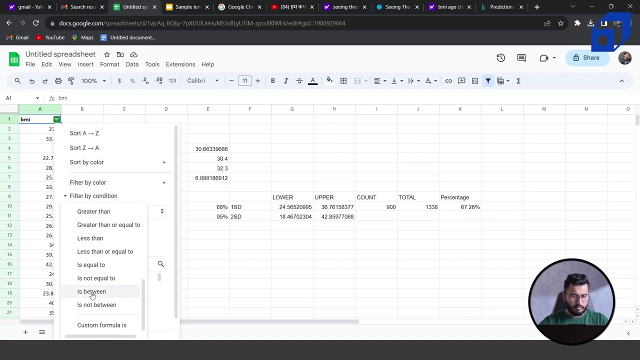 Minus two times of the standard deviation then is equal to mean plus two times of standard deviation. And now I will count, So I will go over here. My condition is between: my lower limit is 18.4.. Upper limit is 18.4.. 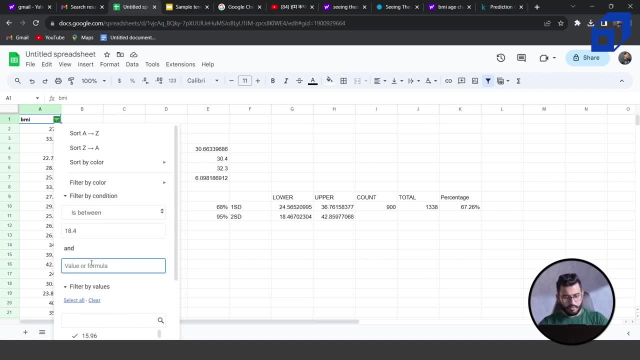 So I will go over here. My condition is between: My lower limit is 18.4.. My limit is 42.8.. I'll click okay And I will now count. The count is 1,281, data points: 1,281.. 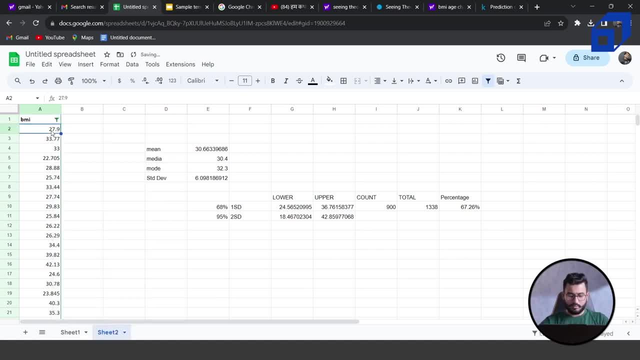 So let's quickly write it down over here: 1,281.. 1338 is my total. I'll just extend this formula to the next, the below cell: 95.74.. So this is my total. I'll just extend this formula to the next, the below cell. 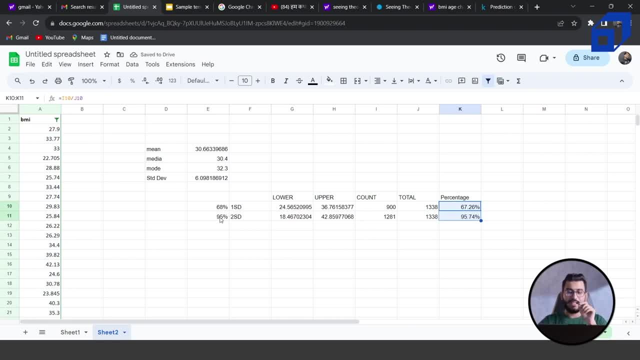 95.74.. What is the standard value? 95%. What I'm able to achieve: 95.74.. Why there is a difference? Because BMI is not my standard normal distribution. According to the standard normal distribution, around 95% values in my data point will lie. 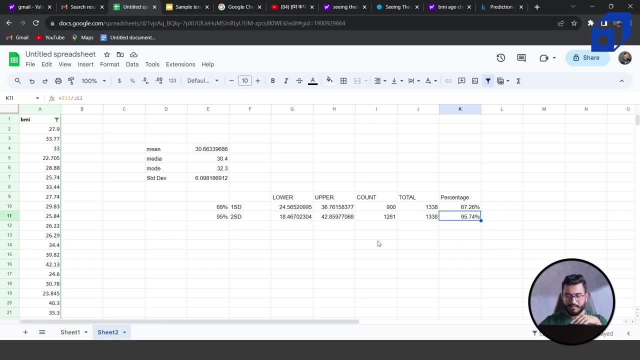 between plus minus two standard deviation- And here you can see final one- is 99.7% of my data falls between plus minus three standard deviation. So it's equal to mean minus three times of standard deviation is equal to mean plus three times of the standard deviation. 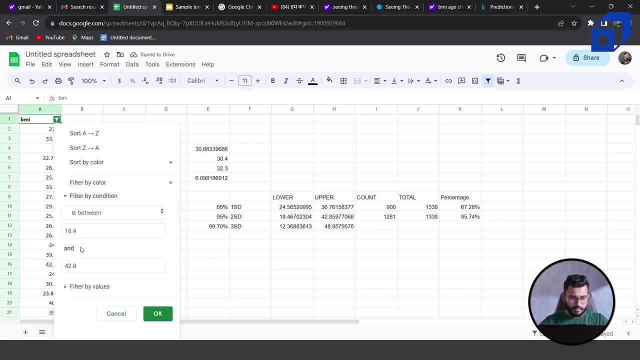 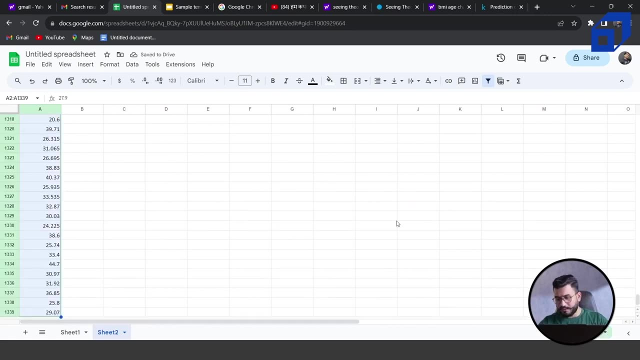 Now I'll calculate how many data points I'm having in this range, So 12.3,, 12.3 to 48.8.. And I'll click. okay, I'll just quickly count. It is 1334 and total is 1338.. 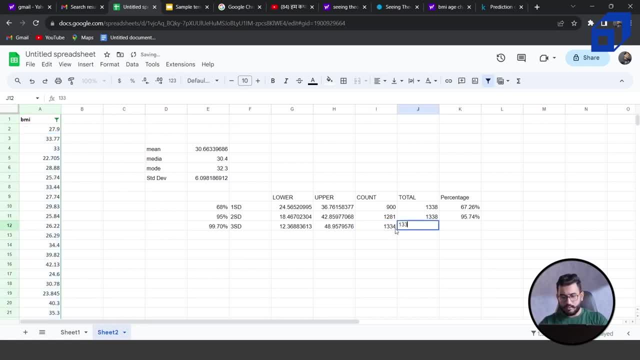 So 1334,, this is 1338, and I will extend this formula to the next row And I'm getting 99.7, which is exactly the same right. So this is the proof of these three properties, That 68% of the data. 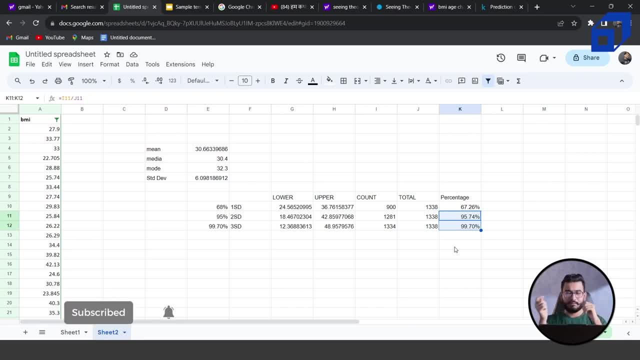 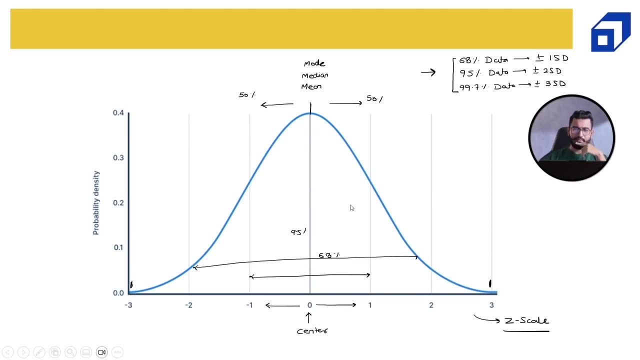 Lies between plus minus one standard deviation, 95%. plus minus two standard deviation: 99.7 in plus minus three standard deviation. Now, if I am given with a particular value- so let's say I'm given with a particular value- how I can find out that? what is the probability at that point? 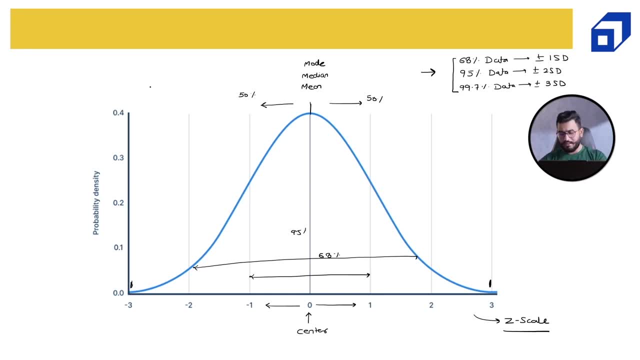 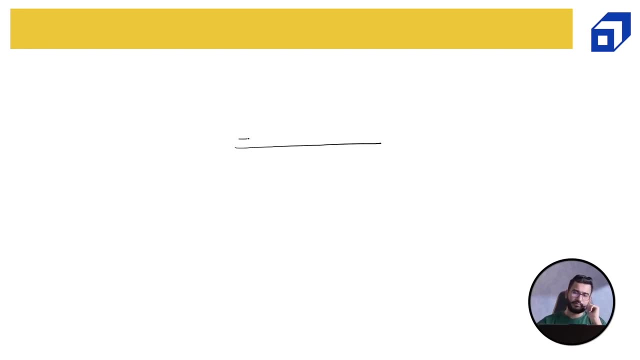 If you're not able to understand my question, Don't worry at all. Let's try to. let me try to make you understand what I'm asking you. This is my standard normal distribution. This is my middle point, which is zero. zero means the mean is zero. 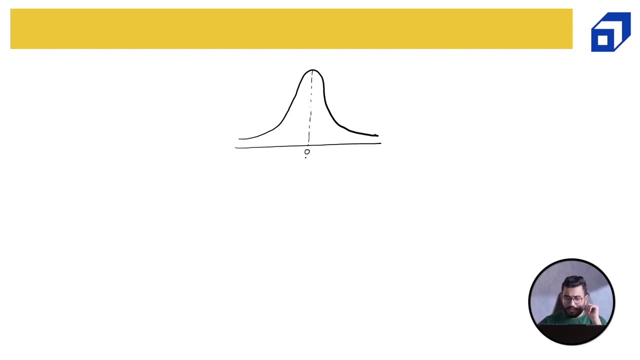 What is the probability that a data point will lie below this point? What is the probability at this 0.5? And above this point, at this 0.5, because, as you already know that if I'm having a, if I consider the complete probability, so what is the probability that a data point? 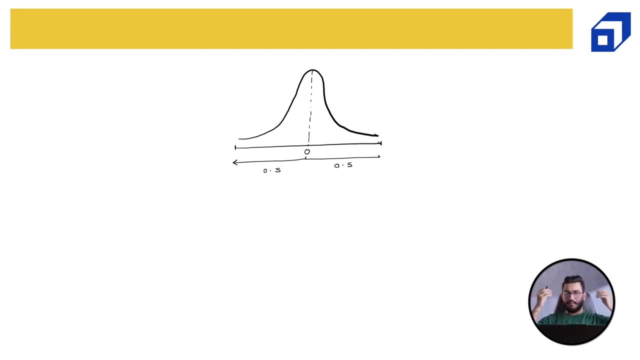 will lie anywhere in this particular range. It is one right. We know the minimum range. We know the maximum range. I know the probability that my data will lie somewhere in the middle, So I know it is going to be one. What is the probability that it will lie below? 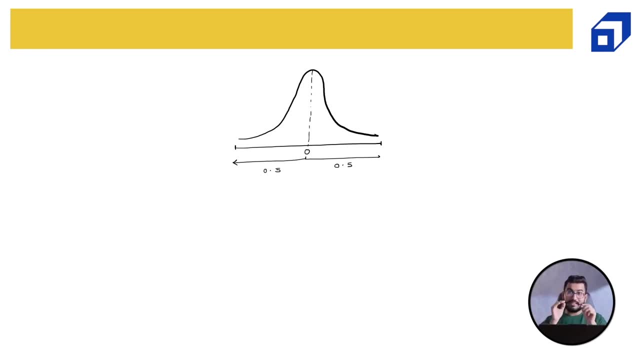 Mean 50% Above mean 50% If it is a standard normal distribution. So in order to find out the probability at any point from the left, we have something known as a Z table. Z table is basically a standard normal distribution table. 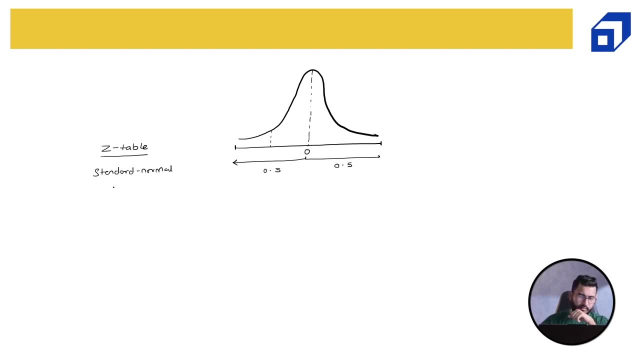 Standard normal distribution table. Okay, Which helps us to find out the cumulative probability from lower point to this point. If I ask you what is the probability that a data point will lie below this point? So using the Z value. so let's say the Z values over here is minus one. 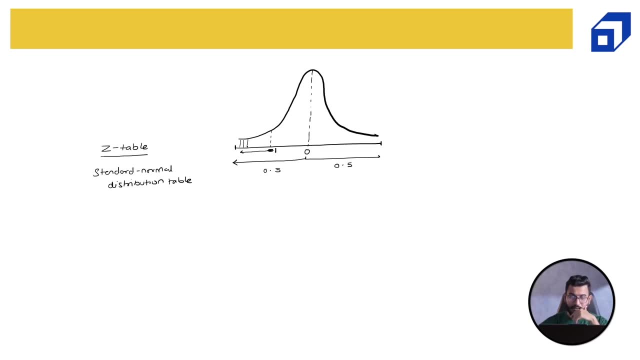 So, using the Z table, we can find out this probability, which is the area under the curve. Now let's see one example. Let's say a set of biology marks in a class are normally distributed with a mean of 70 and a standard deviation of six. 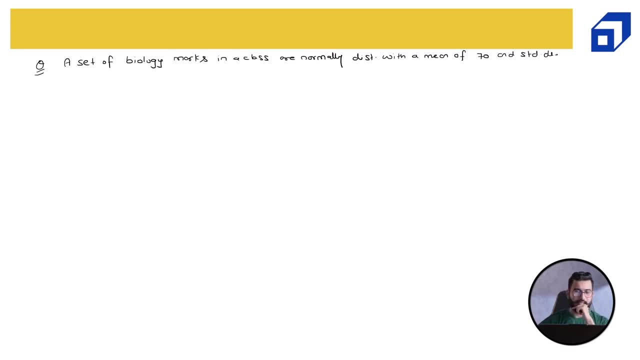 Okay, Okay. So what would happen if we find out the probability of a standard division of six points? What would happen if we find out the probability of a standard deviation of six points? Now, let X represents the score on randomly selected person. 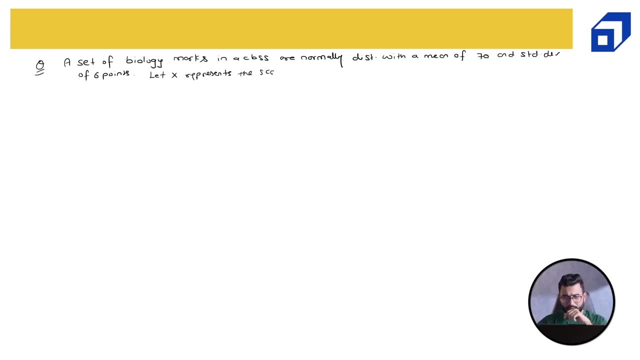 So let X represents the score of a randomly selected person. Okay, Okay, Okay, selected student. Then what is the probability that the marks of this student would be between 64 to 79.? Now, this question is very simple to solve. We just need the properties that. 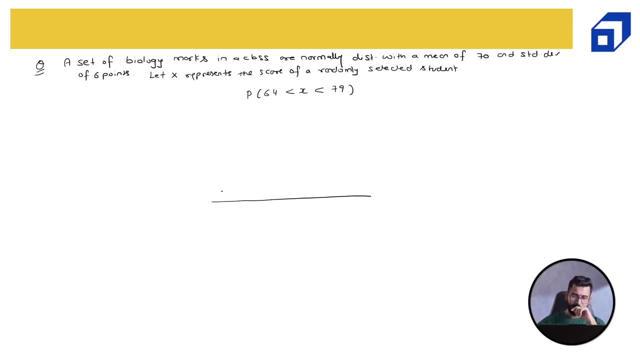 we have learned. Let's create the normal distribution first of all. This is my normal distribution. The mean is 70.. The standard deviation is 6, which basically means I'll go one standard deviation below, so I'll get 64.. One standard deviation above, so I'll get 76.. Two standard 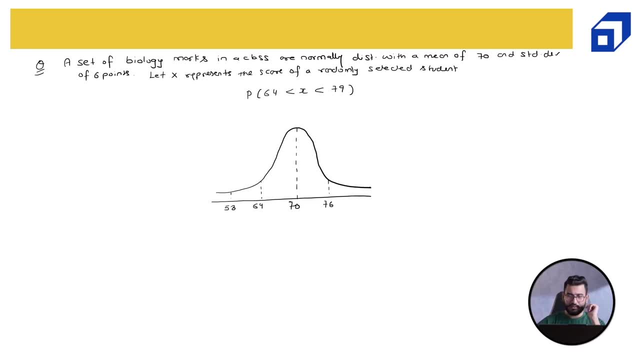 deviation below 58.. Two standard deviation above 82.. Now what I need? I need the probability between 64 and 79.. 64,, which is this point. 64,, which is this point to 79,, which is between 76 and 82.. 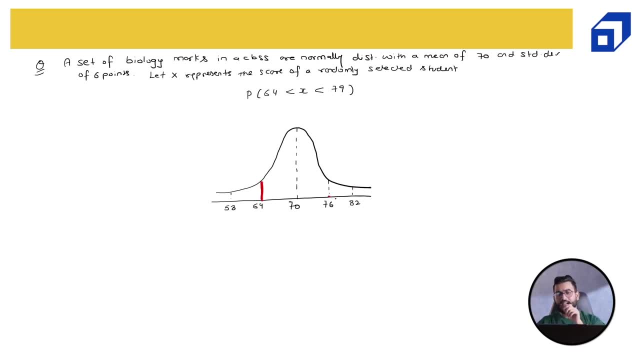 So from 76, if I go half standard deviation above, this will be 79. So this is the area which I'm looking to find out. Let me just highlight the area. This is what I'm looking to find out. I hope you guys are able to look at the area. It looks like I'm coloring a book, but I hope. 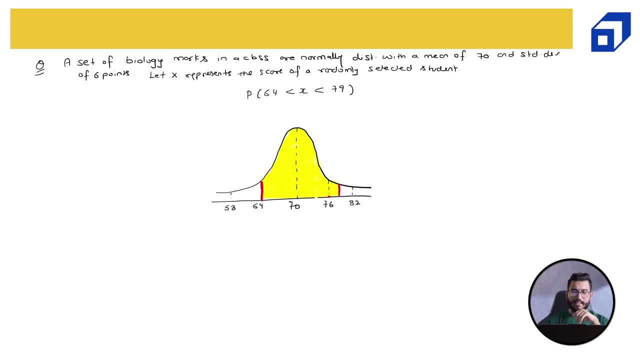 this makes sense. Now, this is the area which I'm interested in. Now, if I go with the logic and the properties that we have learned, So from this point till this point, my, the percentage of data point, so the probability of a data point, between 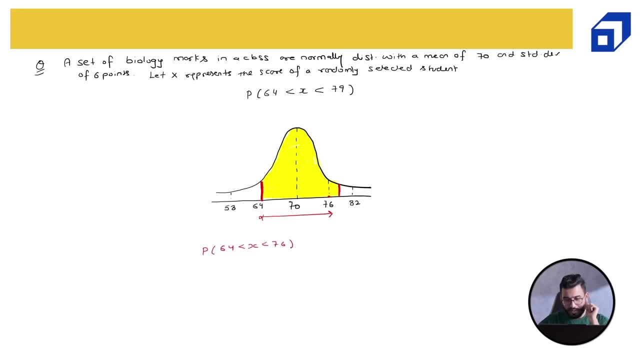 64 to 76 is 0.68, so 68%. we know the property right Now. from this point till this point, from this point till this point, from this point till this point, What is the area under the curve? So, if this is 68,, then this point will be, or let us not. 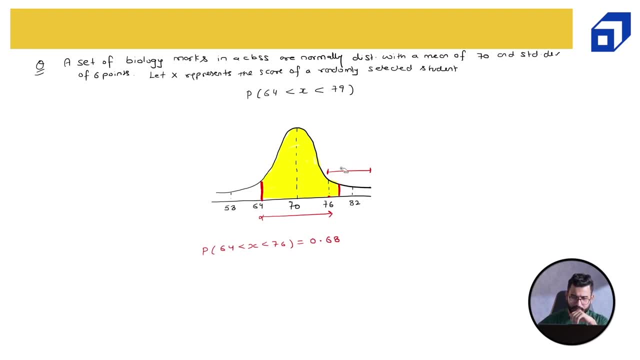 look at the complete curve. Let us look at the middle portion only. So from 58 to 82, from 58 to 82,. so probability of data point between from 58 to 82 is 0.95, 95%, right, If I? 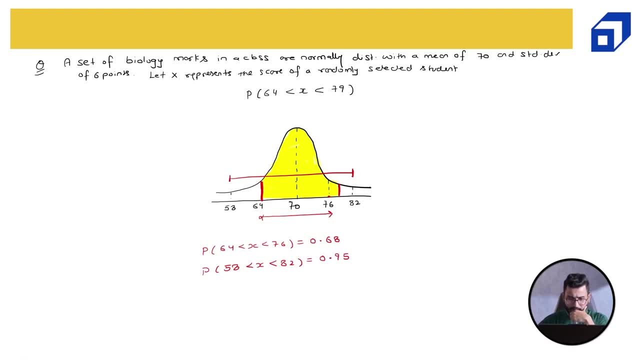 subtract this middle portion, this point, I will get this portion and this portion and I need the half of this portion. So from 58 to 82, I will get 0.95.. So probability of data between from right, As we know that this part and this part is going to be exactly the same right. So let's. 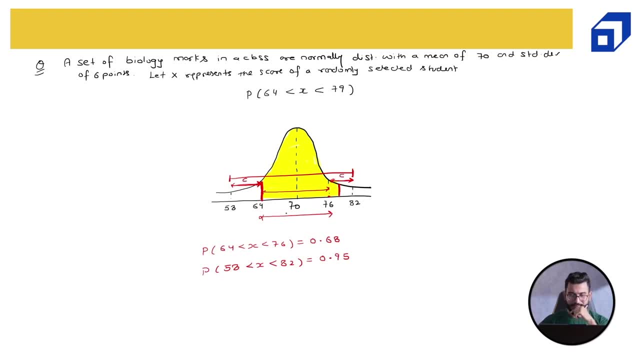 call this as C. and let's call this as C. Let's say: 0.68 plus 2C is equal to 0.95.. So 2C is equal to 0.95 minus 0.68.. C is equal to 0.95 minus 0.68 divided by 2.. This will give me C, this part. 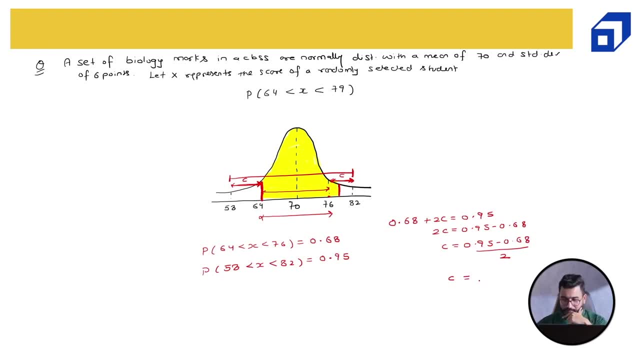 right? So let's calculate C, So this will be 0.135.. Now I'm interested in half of it, right? So my final answer will be probability of a data point between 64 to 79.. I'm interested in this. 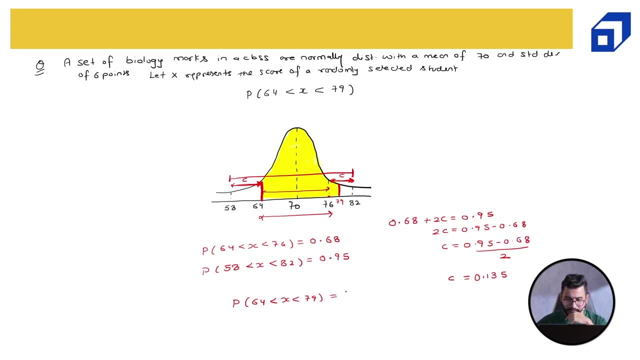 point Will be 68, which is 0.68 plus 0.135, divided by 2.. So 0.68 plus 0.675, which is 0.7475.. This is my final answer. So there is there are 74.7% chances that a person who is randomly selected 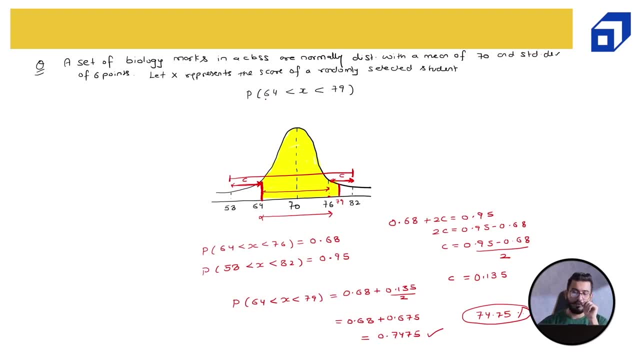 in the class will have the marks between 64 to 79.. Now, in order to solve this question, we have used just the property of a normal distribution, which is states that 68% of the data lie between plus minus one standard deviation, 95% between plus minus two and 99.7% plus minus three. I hope this. 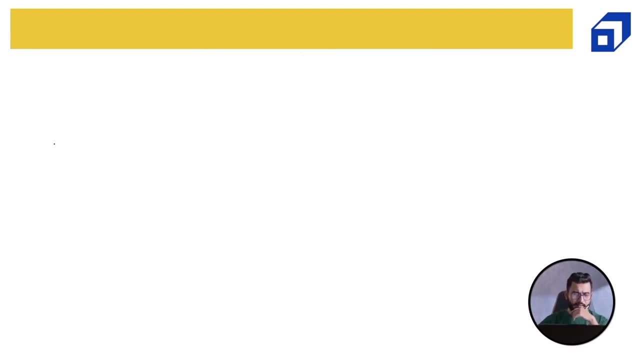 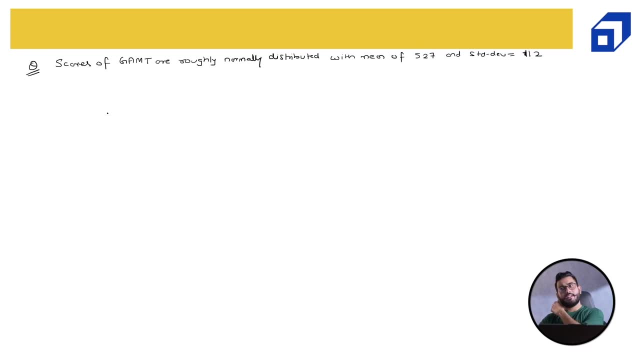 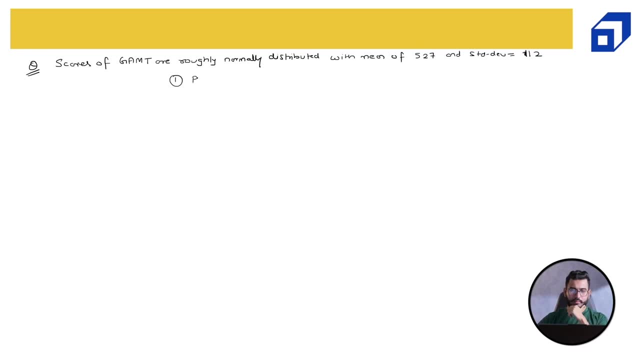 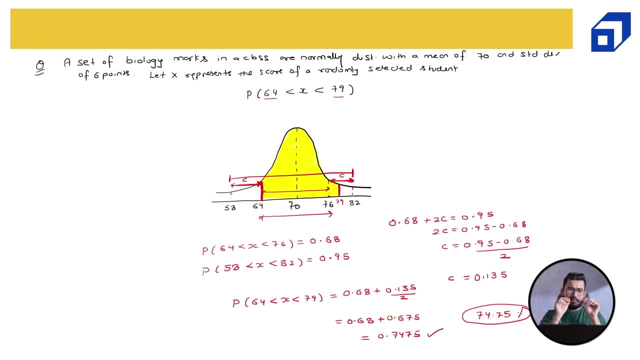 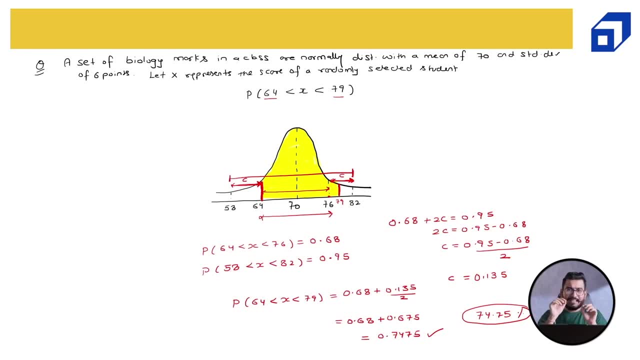 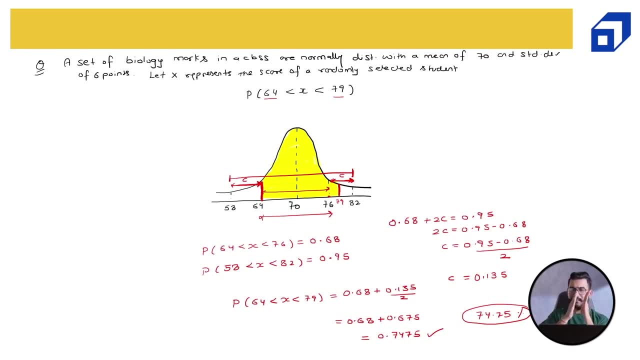 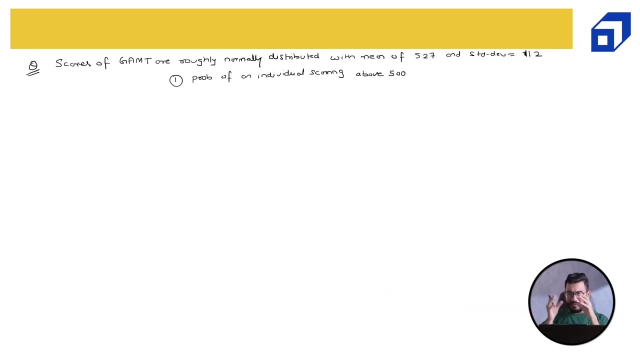 0.675.. 0.675. 0.675., 0.675. 0.675.. given the minimum and the maximum range in such a way that I was able to make calculations. I was able to use elementary math to get to the point right, But now we are not able. 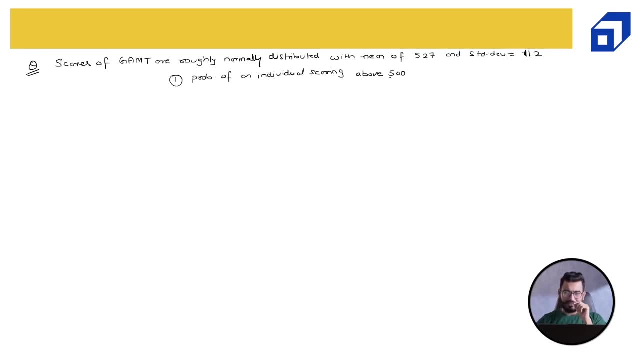 to adjust it, because 500 and then standard deviation is 112.. It is really difficult to use the logic and use elementary math to get it done. In this case, Z-tables are very useful. Let's solve this question. I know that the ZMAT scores are normally distributed with: 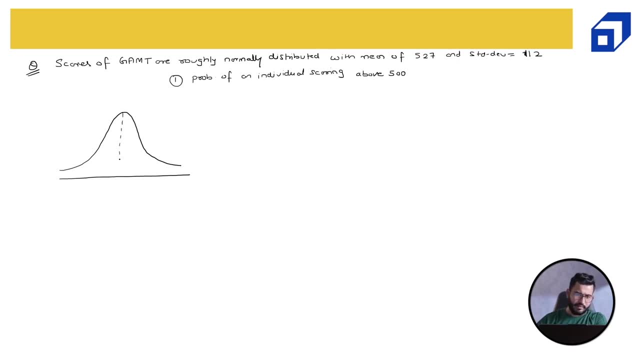 the mean, which is 527, and standard deviation is 112.. Now I will find out how many standard deviations. now I will find out how many standard deviations above or below this value is lying at. So we'll use the standardization formula, We will find out. 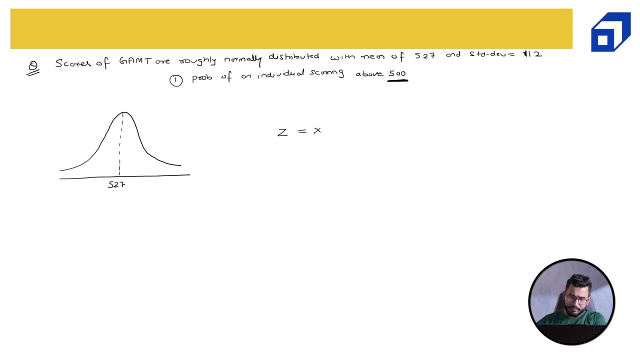 the corresponding Z value, which is nothing but X minus mean, divided by sigma X is 500, the value to be scaled minus mean, 527, divided by 112, which will be minus 0.24.. So if I consider the Z scale, this value will be 0 and minus 0.24 is over here below me, minus 0.24.. Now 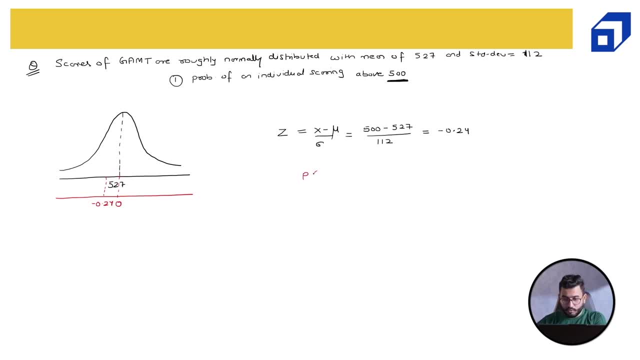 what is the probability that the person will be able to score above 500, in which area I'm interested in. So if this point is minus 0.24, then I'm interested in the area above 500.. So if this point is minus 0.24, then I'm interested in the area above 500, then I'm interested in the area above. 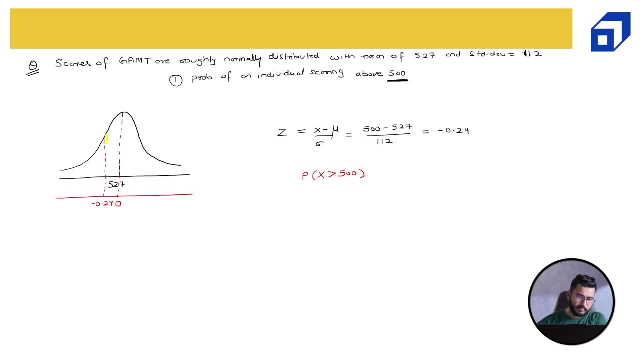 this, which is this area: The probability that the person will be able to score above 500, so I'm interested in this area, this particular area. Now, how we will find it out? So, using the Z table. Z table will provide me the area under the curve from this point all the way up to this. 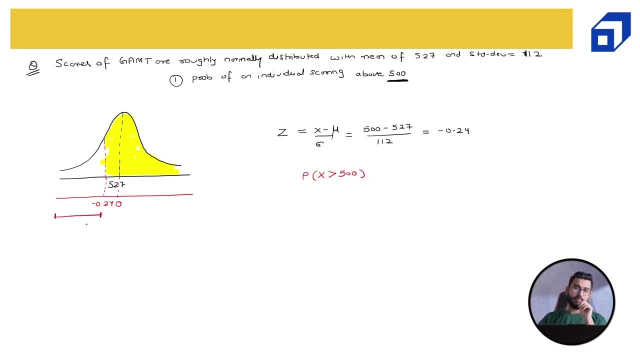 point. Remember AUC that you will get from the Z table will always be from the left to the left. So once I have the area, which is the probability, from this point all the way up to this point, I'll subtract it from one and I'll get my required answer. Let's 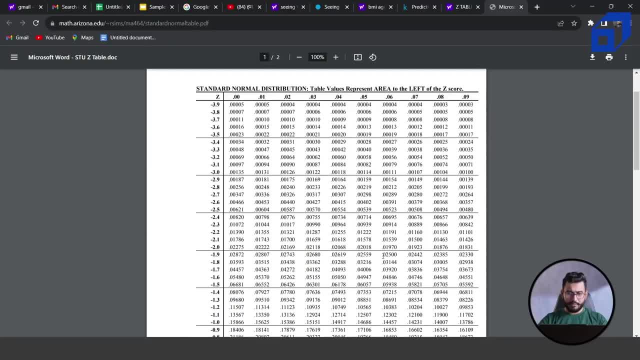 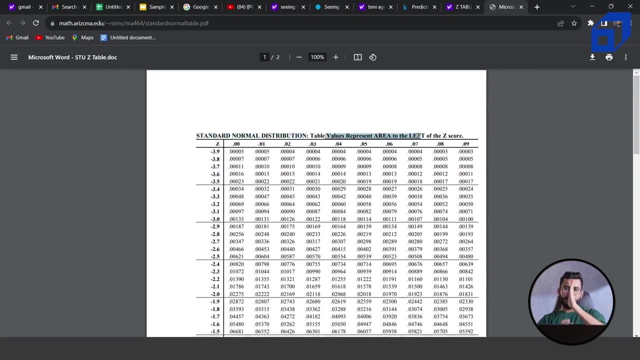 check the Z table. Now here we have the Z table And if you read, this is the standard normal distribution table. value represents area to the left of the Z score. So if I, if this is my Z score, left of the Z score, I'm interested in the value which is minus two. 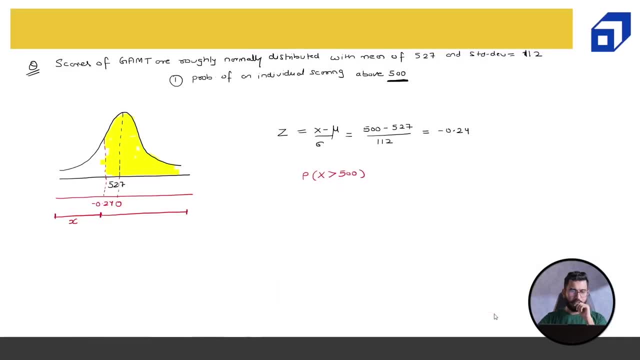 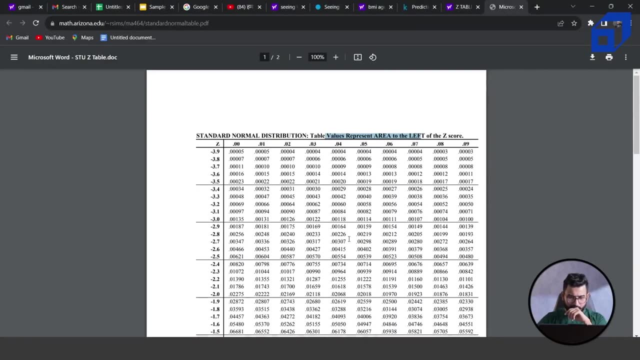 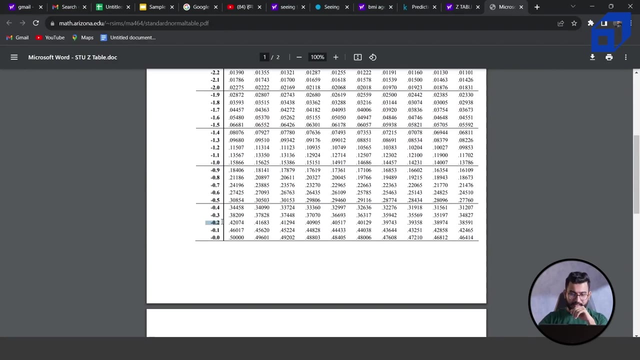 or let me just cross check it: minus 0.24.. Let's check the area under the curve. So minus this is 0.2.. So my we have to first read the row and then the column. so minus 0.2.. 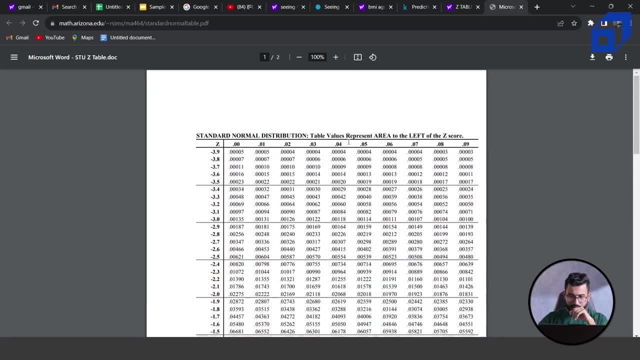 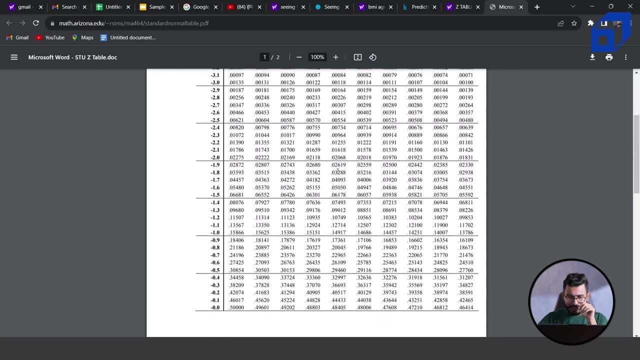 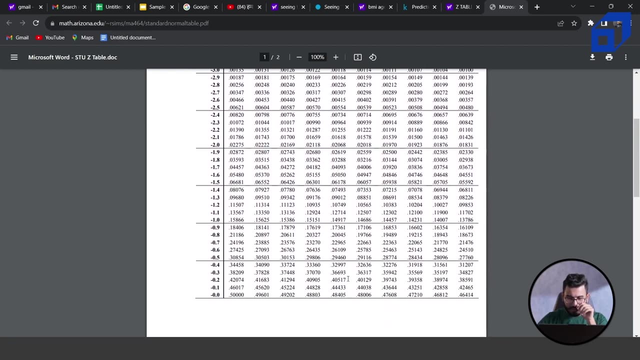 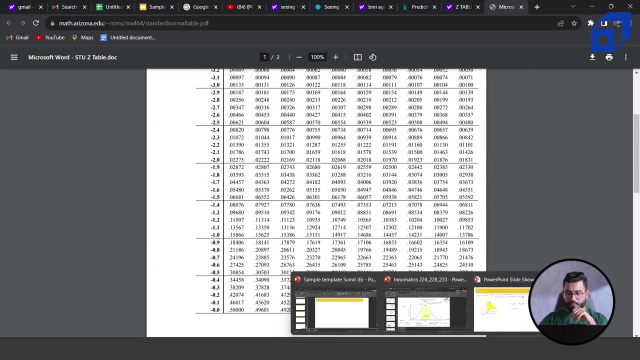 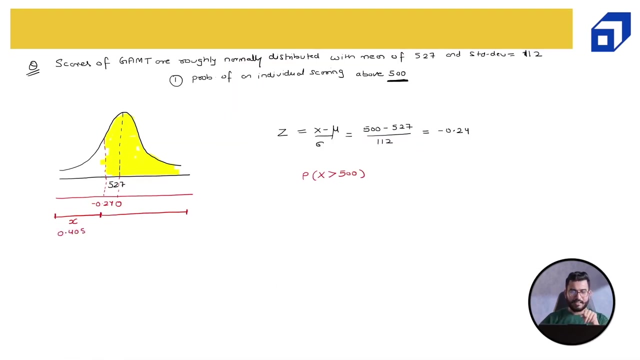 And then for this value Over here, so minus 0.24.. The intersection of these two values will lie over here, I think Yes. So this is 0.40517, 0.40517.. So this x is 0.40517.. I'm interested in this. So what it will be is equal to 1 minus probability. 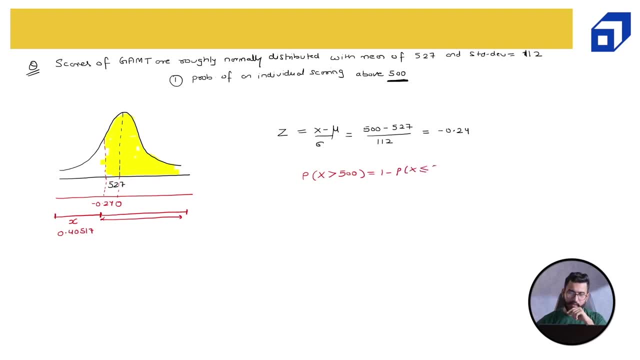 of x less than or equal to 500, which is 1 minus probability of 0.40517.. The answer will be 0.59.. There are 59% chances. Let's say there is one more question In the same in. 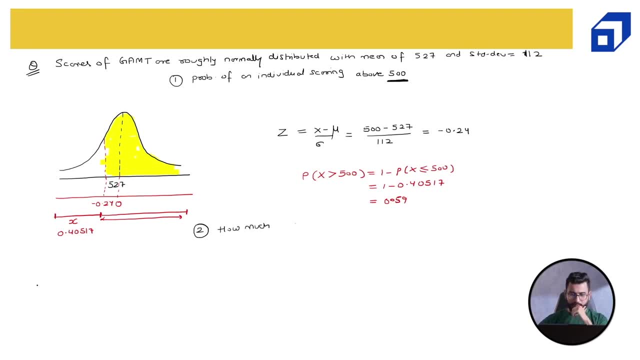 the same example: how much minimum marks should the individual score in order to be in the top 5%? Now, this is a very interesting question And if you guys can understand it, you have understood the complete normal distribution: Top 5%. If this, 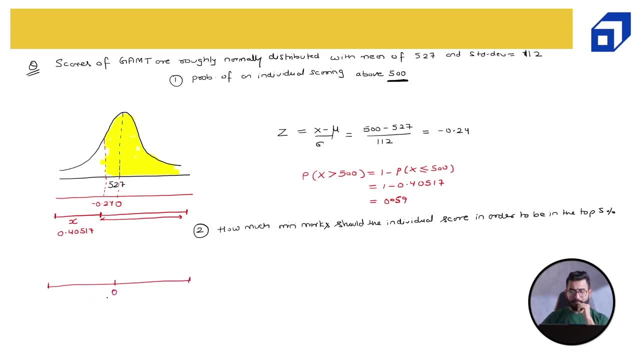 is my middle value. top 5% means below me or below that point, 95% data is there. So if I draw the normal distribution and below, so let's say this is the point which I want to find out and below this point I'm having 95% of my data Right. So I know that I want to find out the 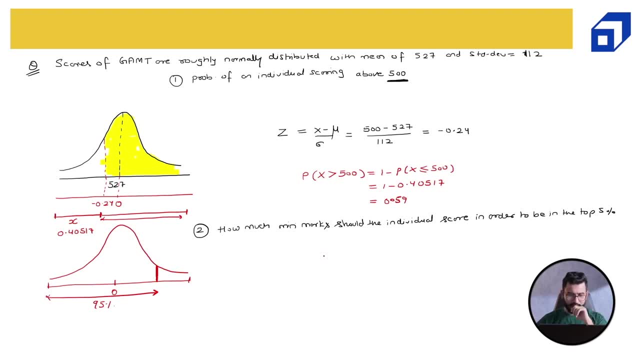 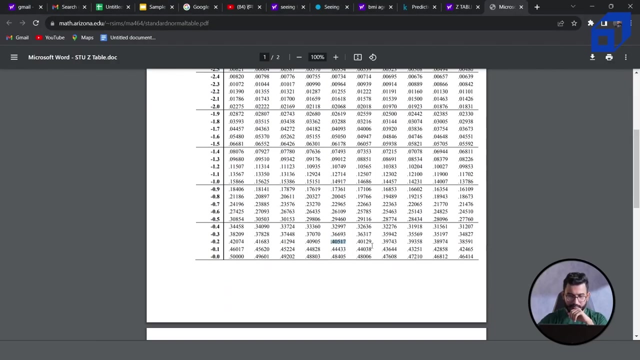 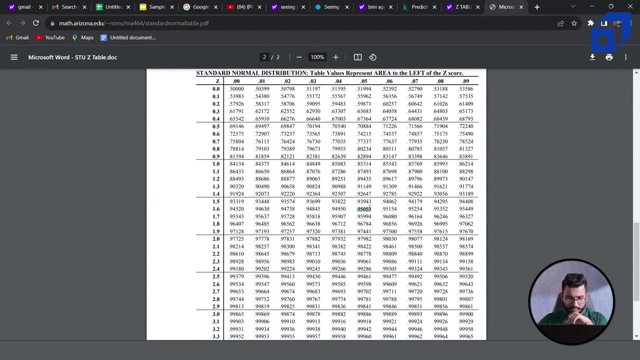 next column, the next colon, the next column: 있지만 out is over here: This is 1.6 and 5.. So 1.65 is my z value. So the z value over here is plus 1.65.. 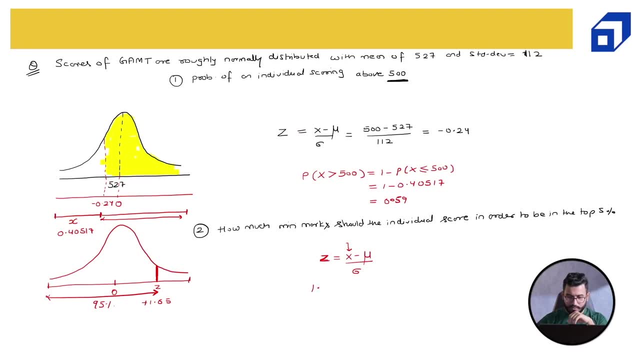 So I know the z value plus 1.65 is equal to x minus mean is 527 divided by standard division is 112.. Again, the elementary math 1.65 multiplied by 112 is equal to x minus 527.. My x will be 1.65 multiplied by 112 plus 527 and this would be 710.6, which basically mean. 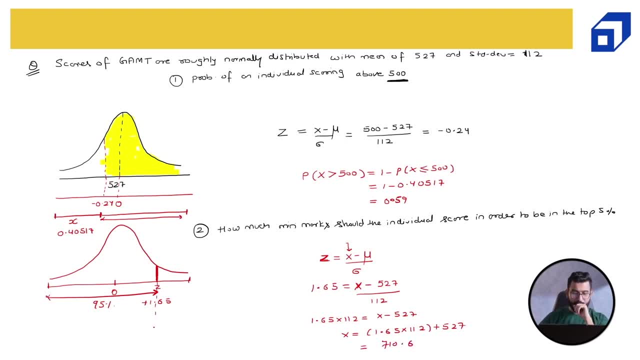 the person has to score a minimum of 710.6 so that the person can lie in the top 5% and below that person, I am having 95% of the observation. Now, this is the application of z table. How z table can help you to find out the z values. 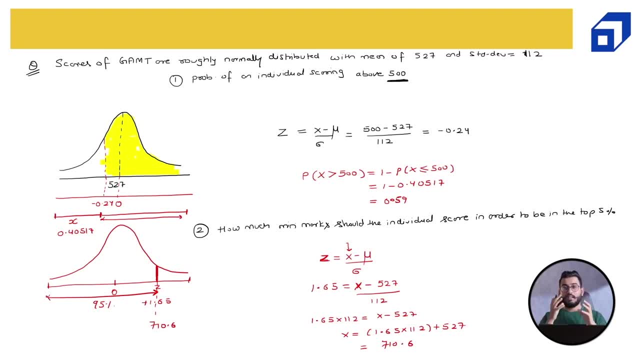 and how z table can help you to find out the area under the curve, which is essentially the probability. What is the probability that I will have a data point below this point, below this z value? That's what the application of z table is. 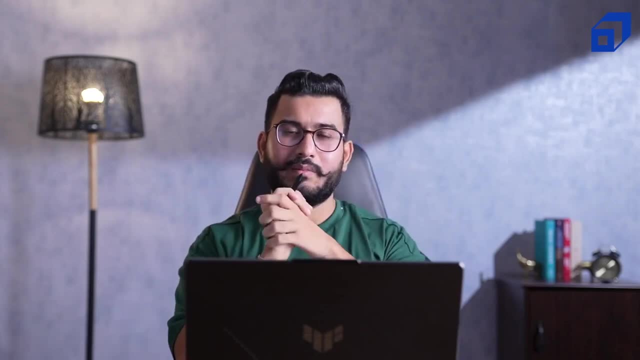 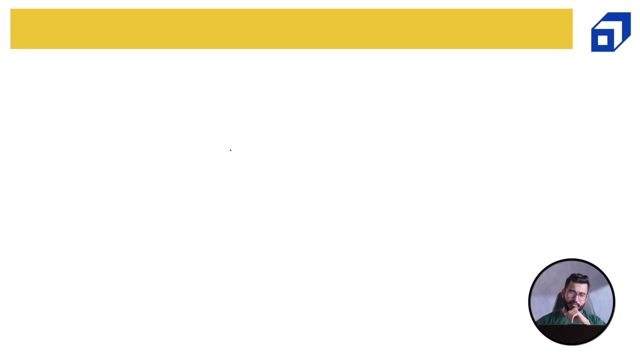 Now we have learnt a lot about standard normalization, Normal distribution. Right Now, what we are going to do, We are going to learn last property of standard normal distribution, which is the analysis of skewness. We know that a standard normal distribution looks something like this: A bell-shaped curve which is symmetrical. 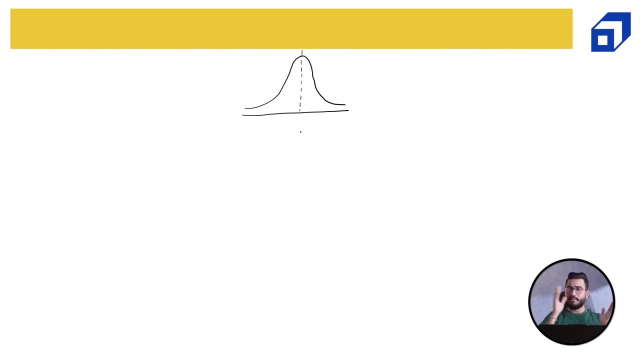 which basically means 50% data below mean, 50% data above mean. but this is the standard And in reality, very difficult or close to impossible to find out a random variable, a continuous random variable, which appears to be a standard normal distribution. So we use standard normal distribution. 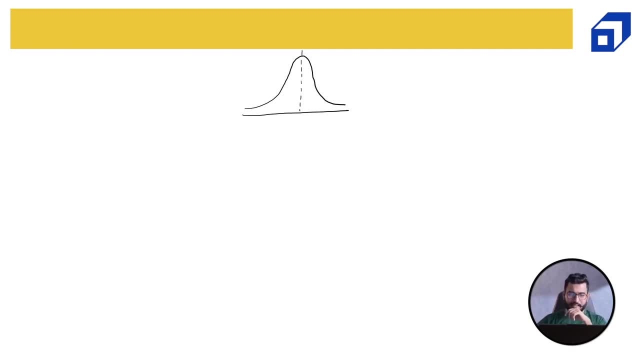 as a benchmark, But in reality you may get a distribution which is either left skewed, right skewed, or no skewness or near skewness. Let's look at all the three types. This is known as the left skewness. I apologize, This is known as the right skewness- Right skew. Why I'm calling. 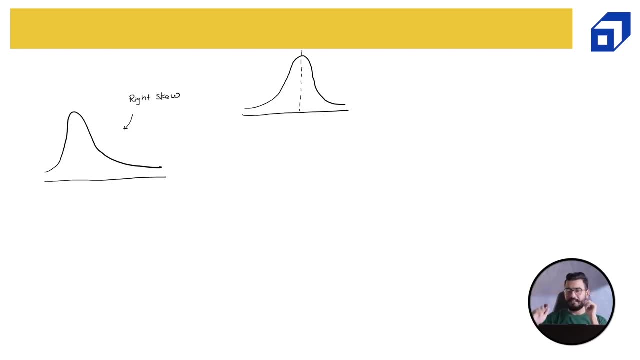 it as right skew Because the skewness is on the right side. So right skew In the case of right skewness, this tail happens to be because of the presence of outliers: The presence of outliers, Presence of outliers, While most of my data is on the lower side. So here I will get the mode. 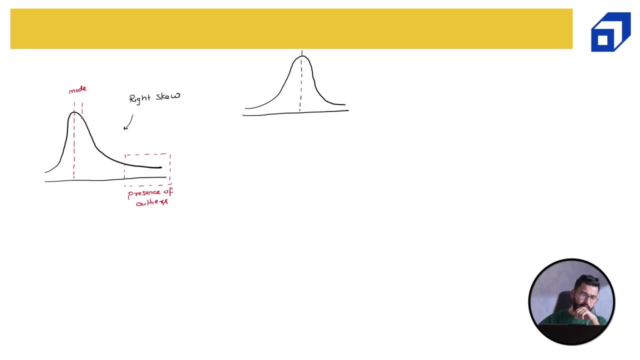 followed by the median And then I will have the mean. So I hope you guys remember that when we were talking about the descriptive statistics, we have learned that if I'm having outliers on the higher side, my mean will shift to the higher end, And that is the reason you can see that the mean has shifted. 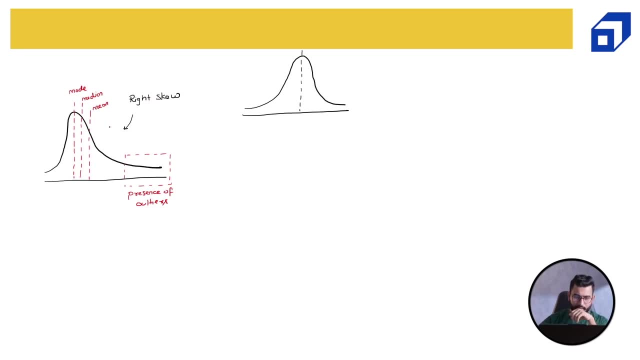 to the outliers or towards the outlier. Now, below this point, below the median, I will have the 50% of my data, And above this, I will have 50% of my data. This is known as right skewness. I can also get our distribution, which is left skewed, Something like this: 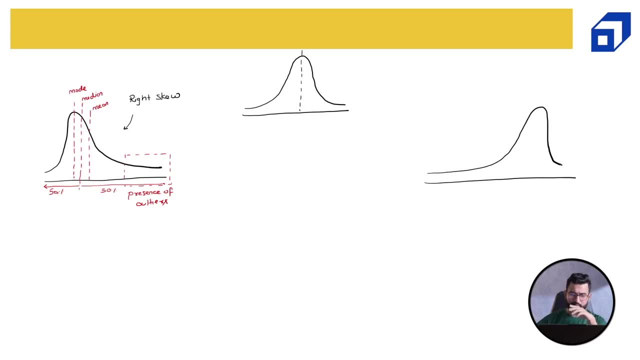 Now, here again, you guys can easily understand This tail is because of the presence of outliers, Presence of outliers, And then again, this is the mode, the mode We have the median somewhere around here, the median somewhere around here, And finally the mean. So mean again shifted towards the outlier. 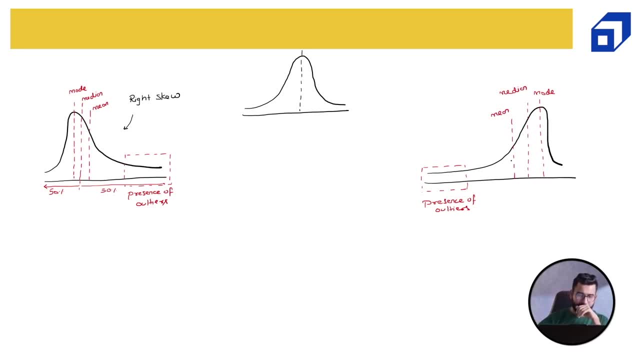 Now, here, most of my data is on the higher side. If I consider this X axis to be my income, then this left side graph represents that most of the people are having low income, While in the left skewed graph, or left skewed distribution, we can understand that most of the people are. 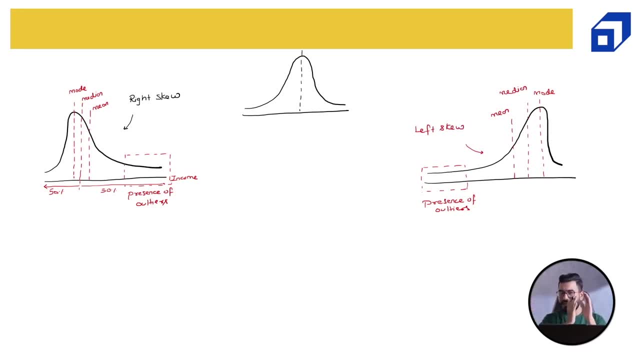 having high income, but due to the presence of few people who are having low income or very low income, the graph has been on. the distribution has been skewed and we obtained a left skewed graph. Now, in the case of right skewness, my mean is greater than median. 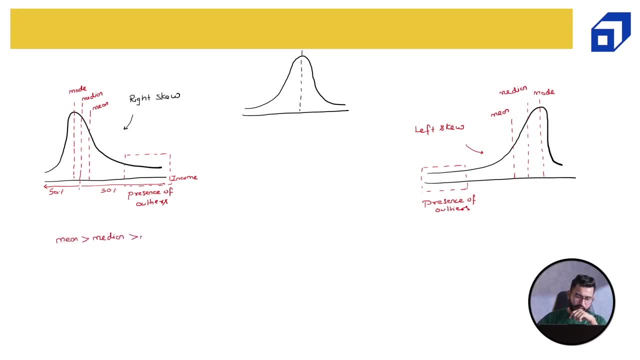 is greater than median. This represents the presence of right skewness in the left skewness. My mode is greater than median, is greater than mean. This is the presence of left skewness And in the case of no skewness, mean will be equal to, or approximately equal to, median. 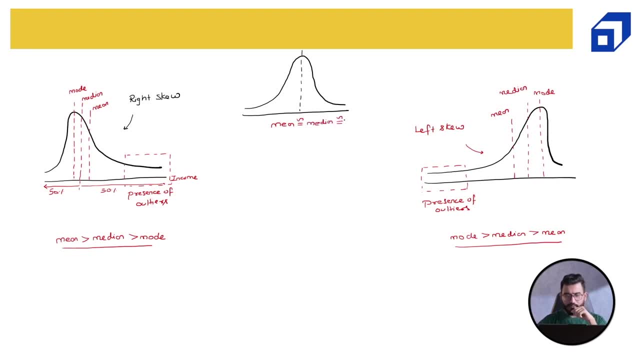 will be equal to, or approximately equal to, mode. If you are getting something like this, you can say your distribution is close to normal distribution. close to normal distribution. Now please remember the properties that we have learned: 68%, 95%, 99.7%. 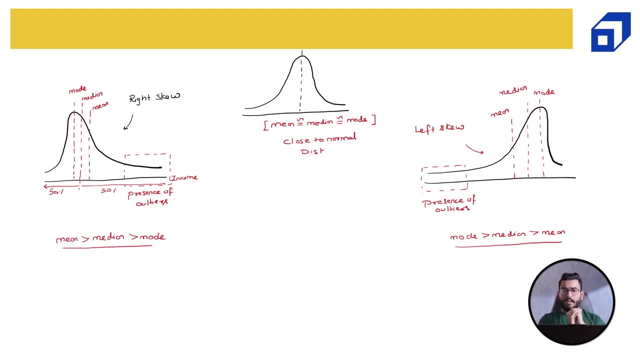 which is also known as 123 rule. It will be best applicable if your distribution is close to normal distribution, While if your distribution is having left skewness, right skewness, well, those properties will not be 100%. true. It will be close, It will be very. 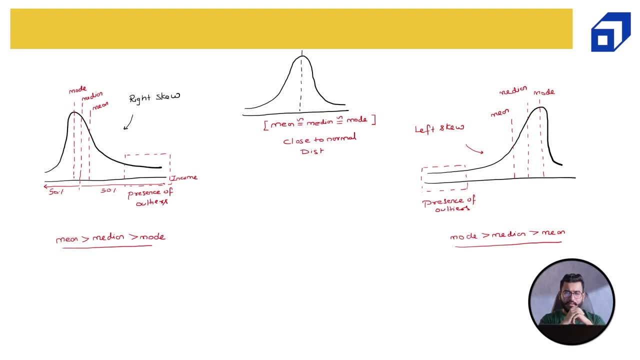 close It. sometimes it will be very different. So whenever you are applying the property, please make sure that your distribution is close to normal distribution. The example of BMI that we have seen was close to normal distribution and we can just go back to the same same sheet. So 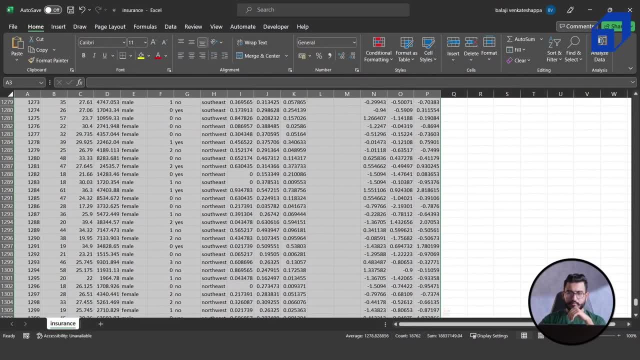 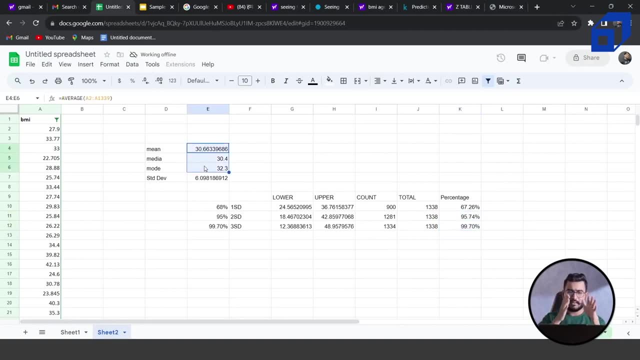 let me go back to the same sheet. Here we have the data And here you can see that the mean, median and mode were very close to each other. So this distribution was close to normal. it was not perfectly normal, it was close to normal And that is the reason these properties. 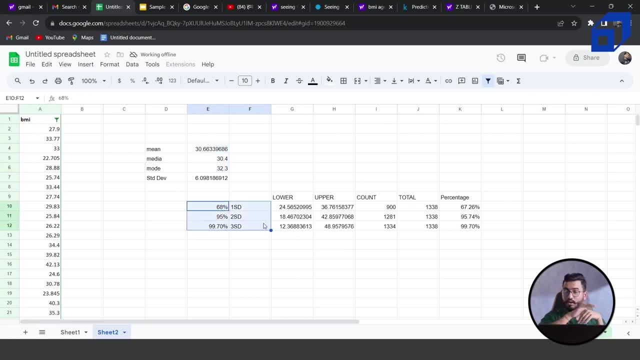 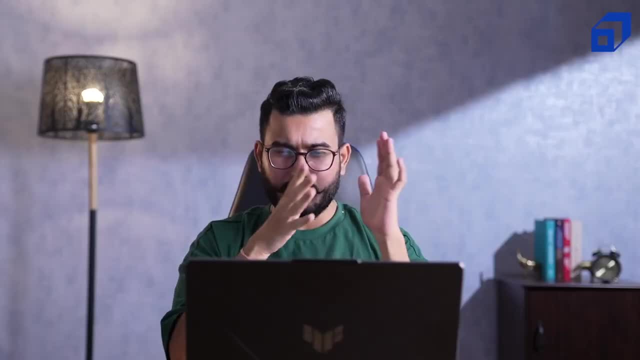 hold true. Otherwise, if this distribution was not normal, this properties would not have held true. I hope this makes sense. So we have covered a lot of topics and the most important topic that we have covered till this point was the normal distribution. 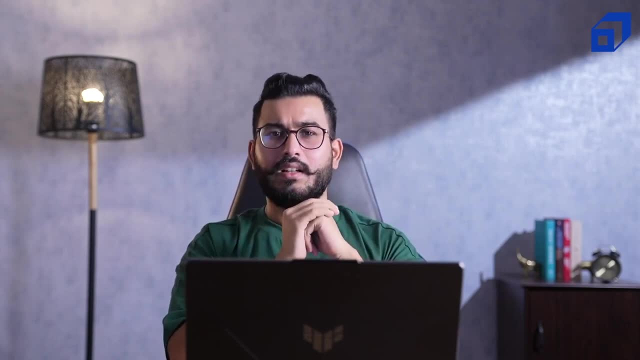 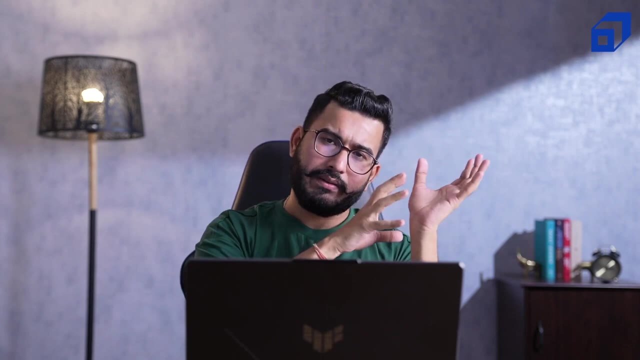 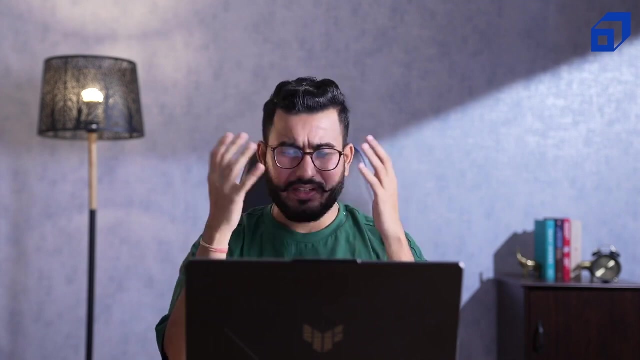 the analysis of Z table, how to read a Z table, how to make use of Z table to find out the probability values, And we have also learned about descriptive statistics and a bunch of probability: the random variables, continuous expected value. We have learned a lot. right Now we are going to start with the second, very important topic. 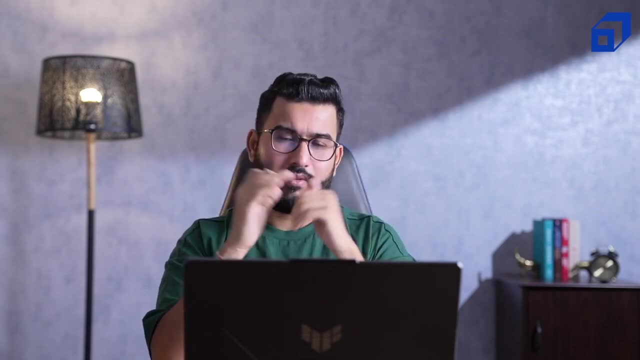 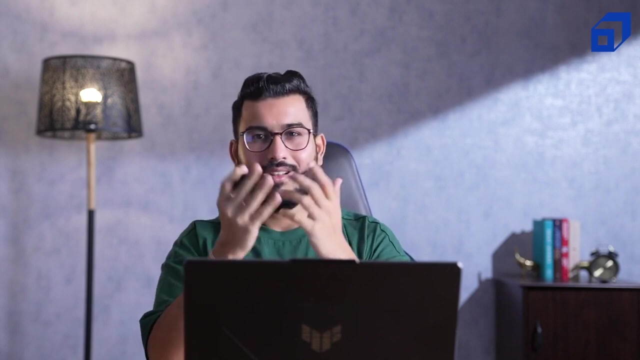 which is under our statistics and probability framework, which is inferential statistics. I have already given you the essence of what inferential statistics is and why we need it, when we were discussing about descriptive statistics, But now we are going to understand it completely And also we are going to utilize the power of inferential statistics to make 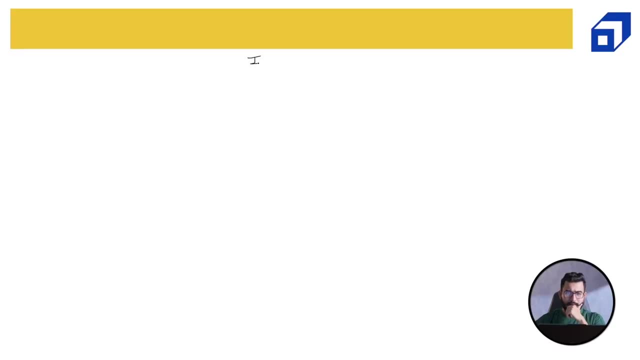 estimations. So let's start our discussion. So let's start our discussion In order to understand inferential statistics. we will take one example. Let's say you work for a marketing company And your manager wants you to, wants you to find out on an average. 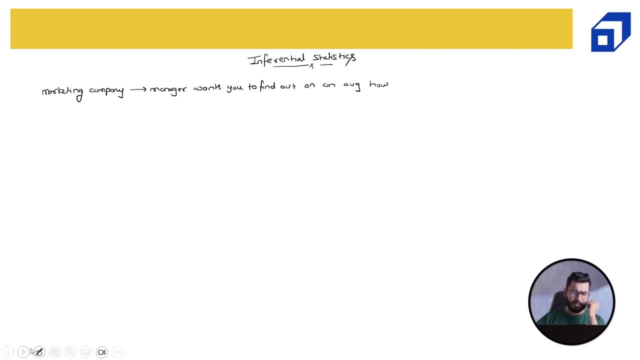 how many recharge, or maybe the average recharge. So your manager wants you to find out the average internet recharge, the average internet recharge done by an individual, from an individual made by the Indians. So I'm talking about the complete India in the Indians. 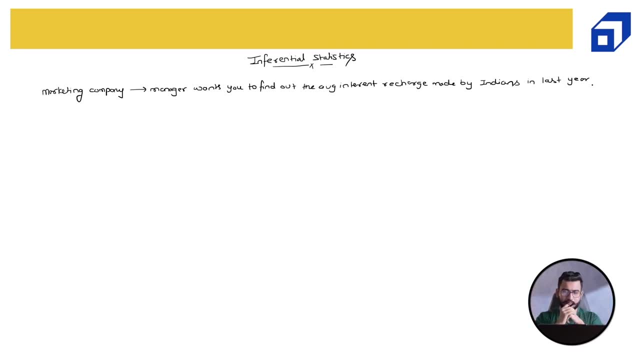 in last year. Now just look at the scope of the problem. we are talking about complete India And your task is to find out the average, the average internet recharge that was done by in last year. It's a very big, challenging problem, right? So let's assume that we have. 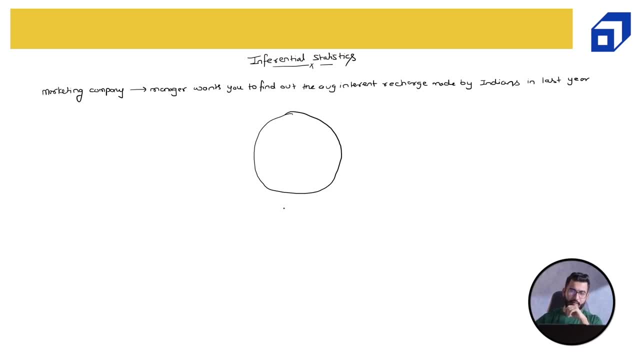 the circle representing the complete Indian population. So population and now, in order to find out this answer, what you will do? So let's say: this is you, this represents you. You will basically reach out to each and every individual. You will collect the. 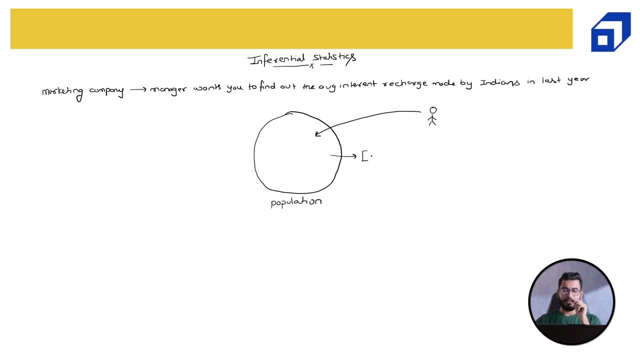 data. So let's say the recharge done by person number one. So let's say the recharge done by person number one is R1,, then R2,, then R3, and so on till R3. Let's say 150 crore. Now, first of all, it is impossible, or not impossible, to near to. 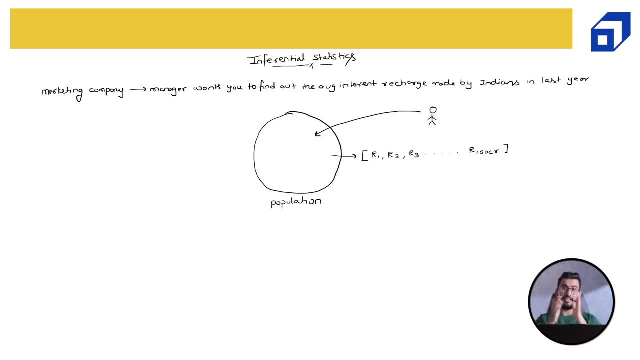 impossible for you to collect the data of this much size And it will be impossible for you to perform survey in such a large scale. So what is survey? Let's say, if I'm having a group of people and I want to ask whether they prefer tea or coffee and they 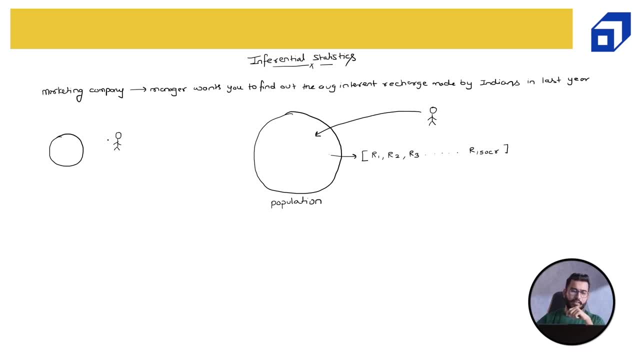 prefer coffee. So what I will do? I will perform a quick survey. I'll perform a survey. So survey basically mean I will go to each and every individual. So reach out to each and every individual, then ask them about their opinion. So ask the question, ask the. 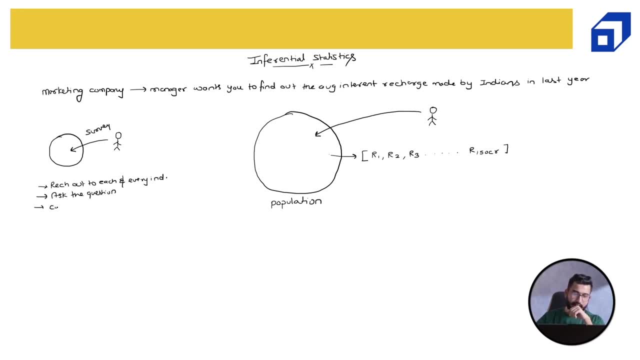 question, Then collect the data, collect the data And finally, we perform the estimation. So estimation estimation means we- uh, we- calculate the average minimum, maximum, whatsoever you want to calculate. This is the process of survey. Now, if I have to perform the same, 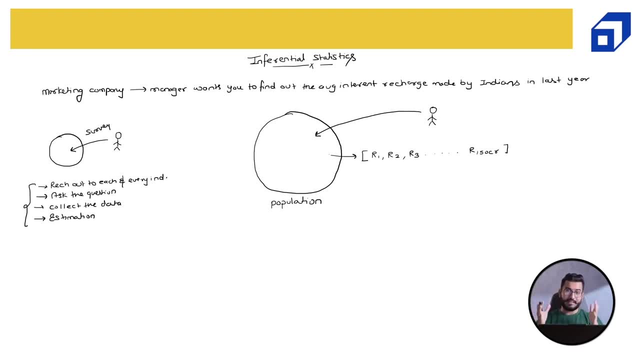 thing on a population which consists of 150 plus car or people, don't you think it's going? for a individual like you, it is near to impossible, not impossible to near to impossible And the I would say it is impossible even for me, or even for a government organization. 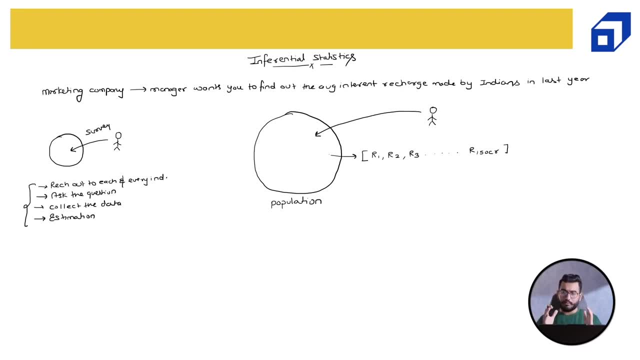 it is impossible for anyone to perform a survey in such a large scale. Even if it is possible, even if it is possible by a government organization, it will take a lot of time, a lot of time and it will take a lot of investment. 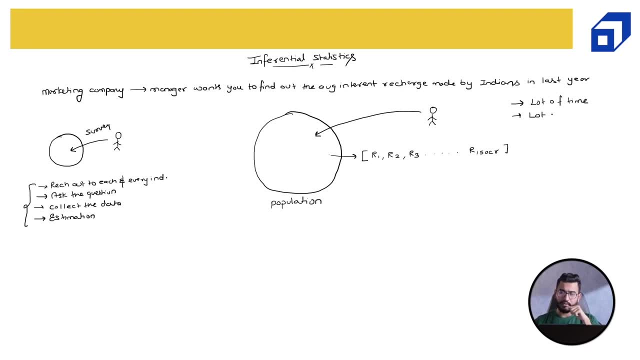 Lot of investment. Lots of money is required, A lot of people is required. So lots of investment, investment. Now, what is the better solution for this? We have already discussed about it. Solution is: I'll take a small sample. We call this as a random sample. Now I'll talk about what. 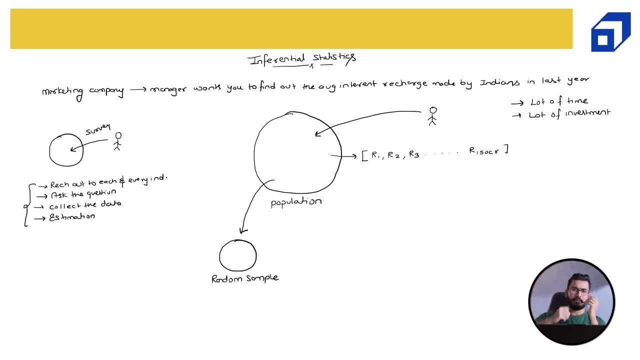 random sample is all about. but we take a small sample, We take random people. Let's say I have taken one lack random people, one lack random people from the population of 150, car or plus people. Now, as an individual, it is quite possible for you to perform survey. 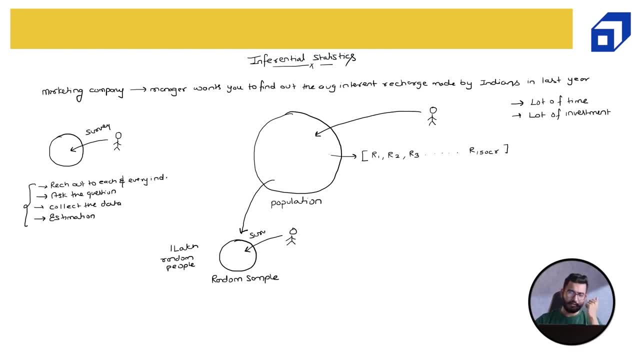 on one lack people. So you have performed a survey, you calculated or you collected the data, So R1, R2, R3,, R4,, R5,, R6, R7, R8,, R9,, R10,, R11,, R12,, R13,, R14,, R15,, R16,, R17,, R18,, R19,, R20,, R21,. 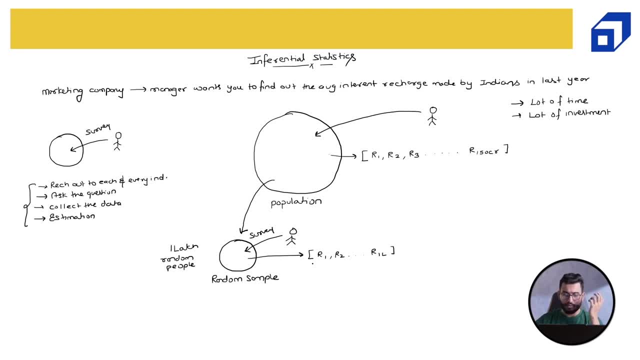 R22, R30, R24, R23, R24, R24,, R29, R30. Then you have to leave. leave all these сол mean we will try to approximate the population parameter, a population mean, And this is: 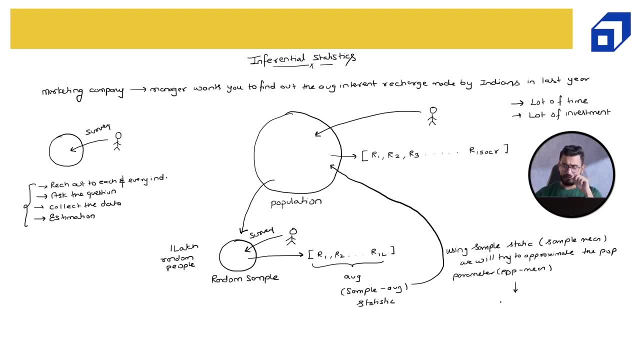 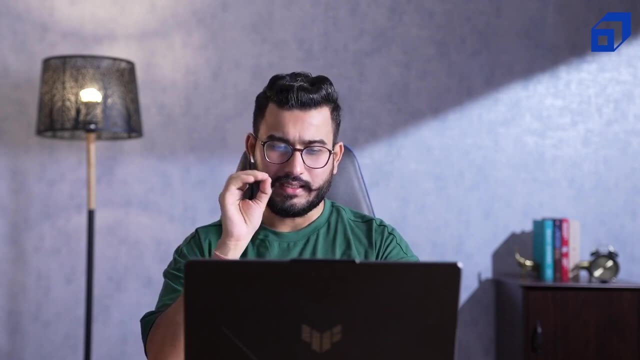 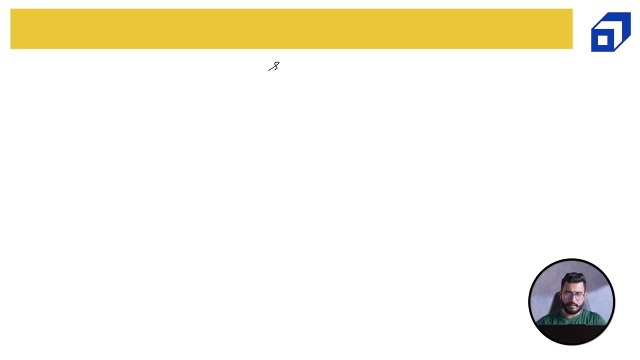 basically known as your. this is basically known as your inferential statistics, inferential stats. Now, before we talk about how to estimate the population parameter, let's try to quickly understand what is sampling and random sampling. So, when we talk about sampling, 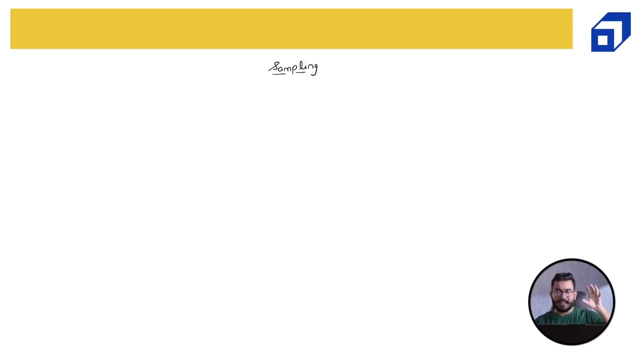 it is basically the procedure of collecting few observation from a bigger subset, or you may say population. So I'm having a population, I'm having a population And now I want to collect a smaller sample of smaller group of observations. This is another sample. Now this process is known as sampling. 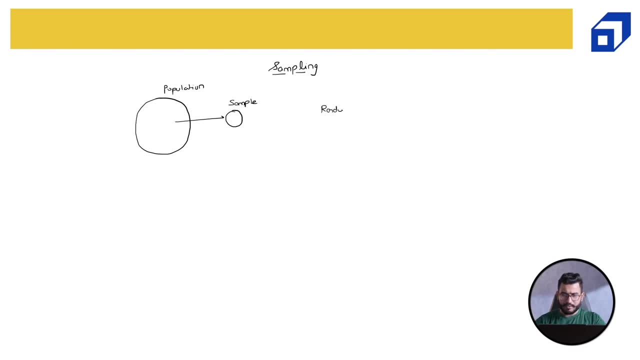 There is one very popular sample sampling technique which is known as random sampling, And this is a very important interview question. What is random sampling? Random sampling is nothing but assume that if I'm having a population, having, let's say, numbers, 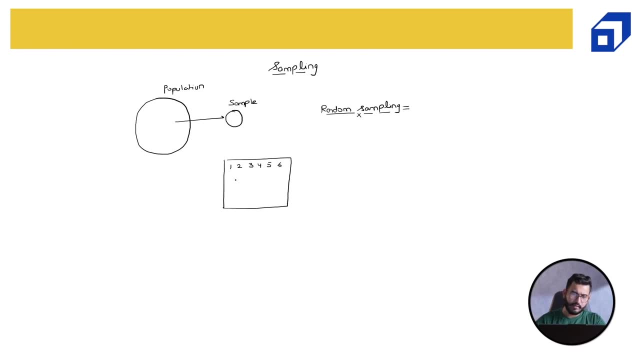 one, two, three, four, five, six, seven, eight, nine, 10,, 11,, 12,, 13,, 14,, 15,, 16,, 17,, 18,, 19, and 20.. 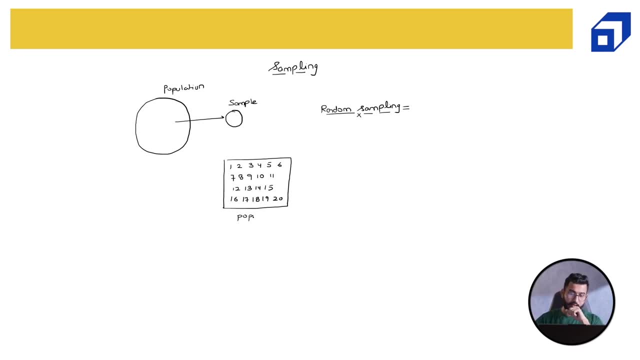 So I'm having a population which is having 20 people And the rule number of 20 peoples are written over here. Now, if I have to select a random sample of five people, so select random sample of five people. so what we will do, we will. we can kill. select any five people, but 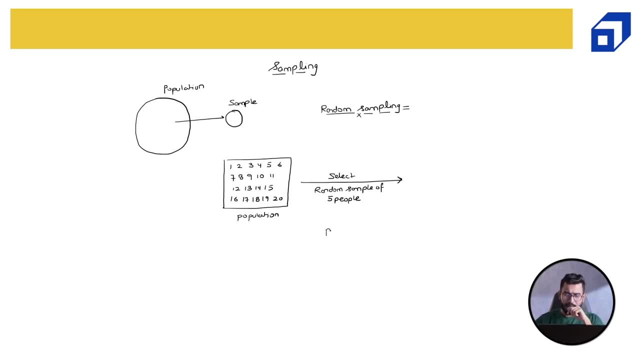 according to the random sampling, the probability of selecting any observation is equal to one by n. so probability of selecting one is 1 divided by 20. probability of selecting 2 is 1 divided by 20, and this is same for selecting any number is 1 divided by n, which basically means, in simple: 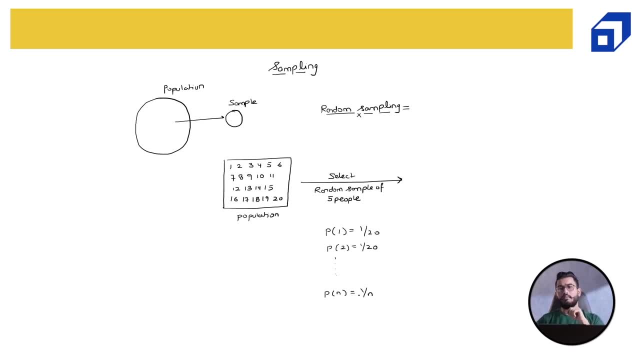 random sampling. there is no bias. we will just randomly select any observation from a population, and the probability of selecting any observation in my population is 1 divided by n, which is the same probability for every observation. so each observation in my data comes with same probability of. 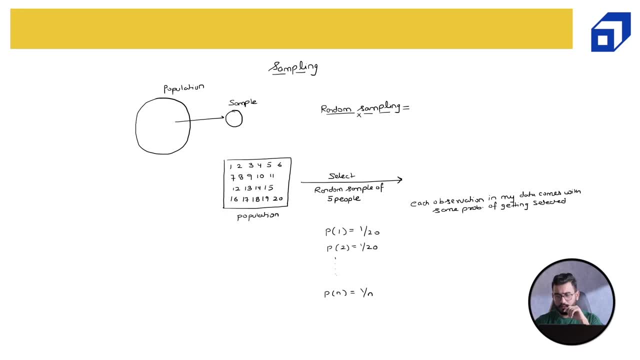 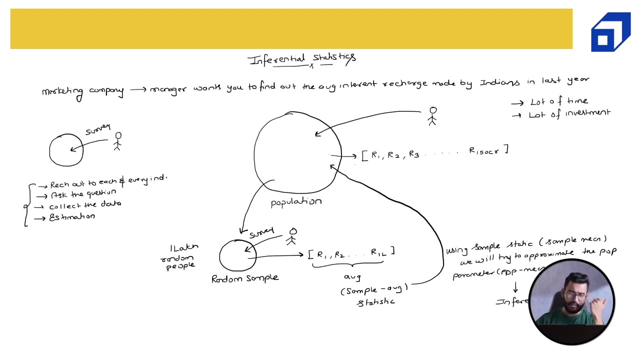 getting selected into the sample. so here my sample can be five, nine, two, seven and ten. now why I have written five, why I have written nine: I have just randomly selected these five numbers. so this is simple, random sampling, and that is what I was talking about here: the simple, random sample. okay, now let's. 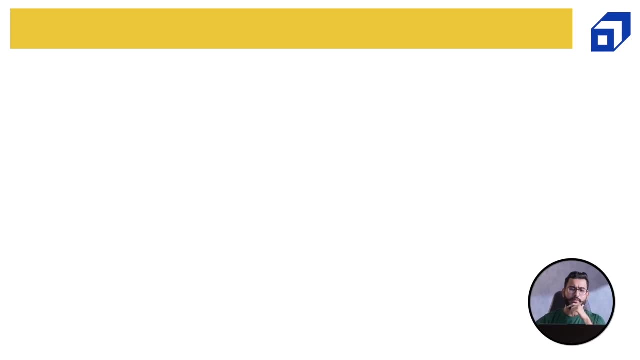 talk about how to perform estimation. in order to perform estimation, we use a particular algorithm: central limit theorem. central limit theorem. now what this theorem talks about? this theorem states that if I'm having a population- let's say this is a population of Indian people, let's say I took one simple random sample of one lakh people. now, when I calculated the average, 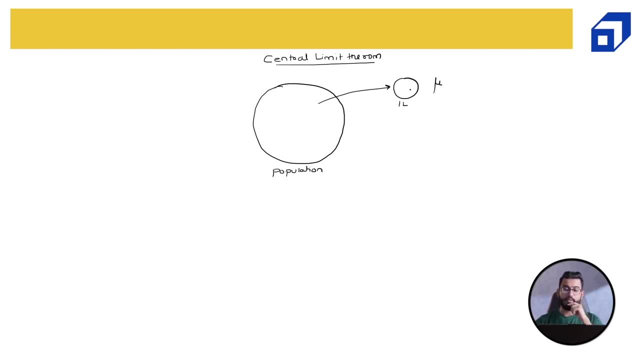 the average recharge amount for these one lakh people for sample number one came out to be, let's say, 250 rupees. for again, I took another sample, sample number two, of another one lakh people. the average came out to be, let's say, 220 rupees. I again took one more sample, sample number three. 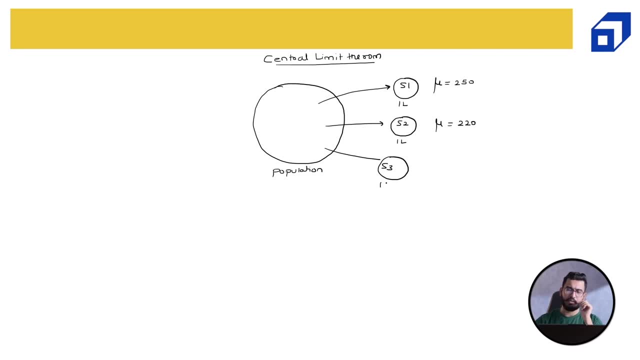 again, with one, one lakh random people, the average came out to be, let's say, 210 rupees. and like this: if I keep on doing, if I take enough simple random samples from my population and I quickly plot them in a particular histogram, I'll get a normal distribution like this: 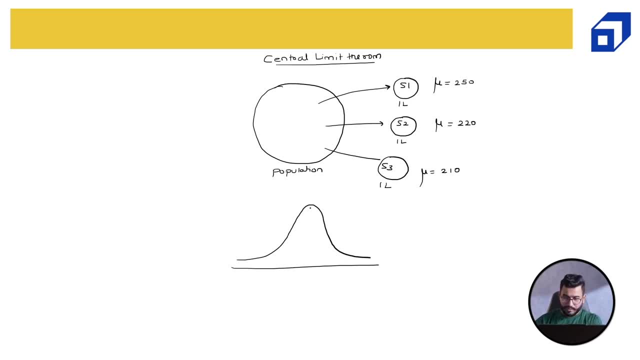 I'll get a normal distribution where the average of this normal distribution is my population average and the standard deviation is given as sigma divided by root of n. so the first property of central limit theorem is the average of all of all sample average. sample average will be: 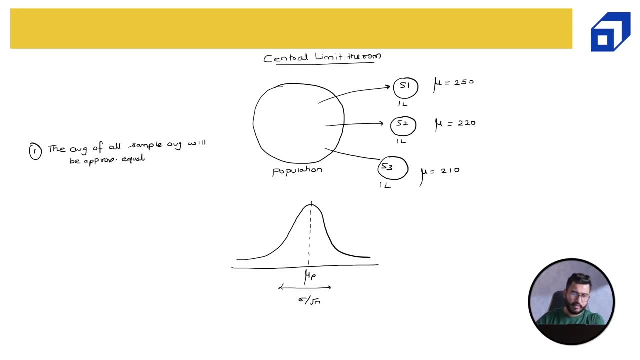 approximately to the population average. The second property is the standard deviation of the sampling distribution is given as sigma divided by root of n. Now these are the two properties of the central limit theorem and using these two properties we can estimate the population range. Let's try to understand how we can estimate the population range. Let's say this: 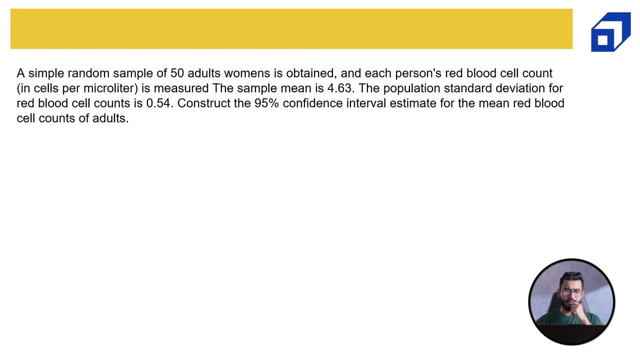 is the question that is given to us. in a simple random sample of 50 adult woman is obtained. So I have a simple random sample. This sample is having. n is equal to 50 women And when the red blood cell count was measured for them? 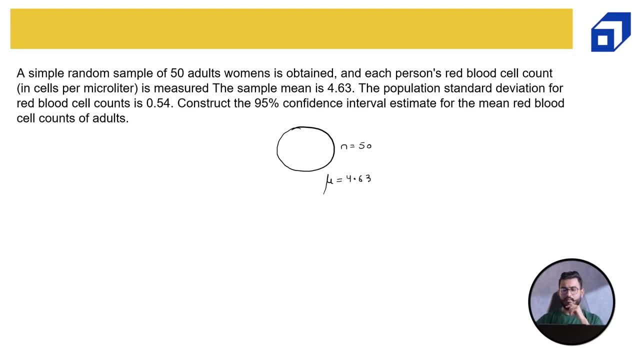 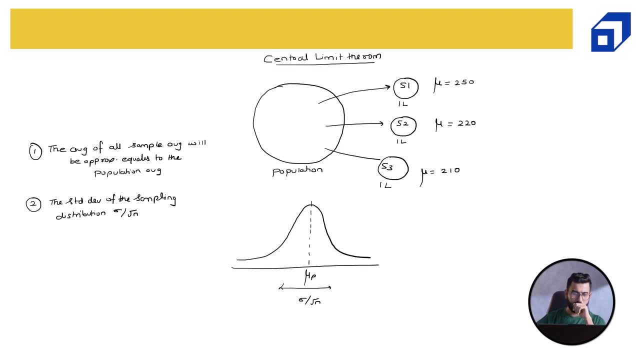 This sample average came out to be 4.63.. The population is standard deviation is 0.54.. Now let me go back, and I was. I did not specify that this Sigma represent population standard deviation and this n represents the number of observations in the sample. So in this, 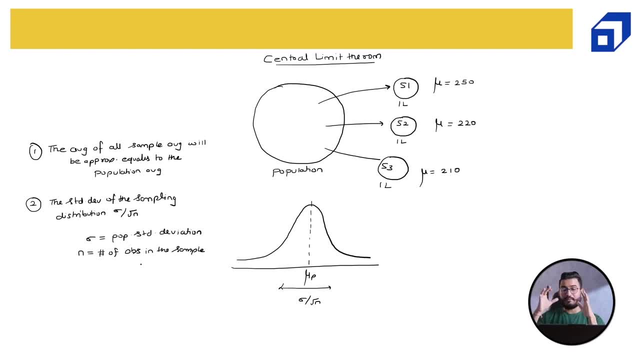 case it would be one lack. So central limit theorem states that the average of all these sample average. So I've taken multiple sample of sample. I have taken multiple samples from my population. These are my multiple samples. These are my multiple samples: one, two, three and so on. And if I take the average, 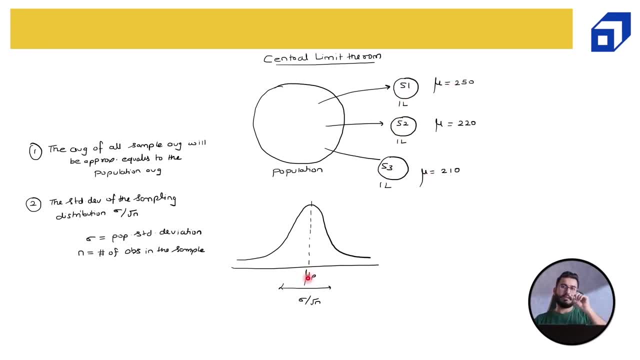 of all these sample average. it will be closely equal to the population mean, a population average. And if I plot them, if I plot all these sample means in a distribution, in a, in a histogram, it will closely resemble in normal distribution And the this, this is this distribution. 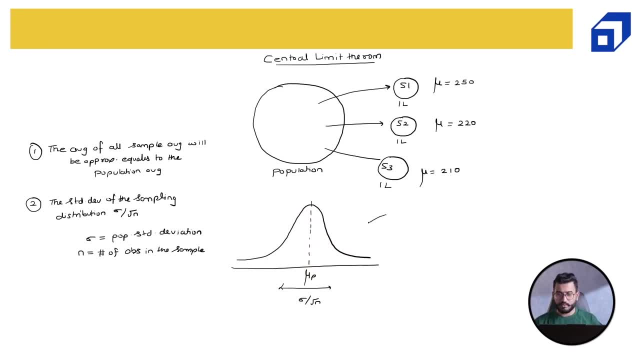 is known as the sampling distribution. This distribution is known as the sampling distribution by sampling distribution because we have obtained it using the sample means. So these are mine: Sample means. Sample means Now: central limit theorem states that the average of all these sample mean will be closely. 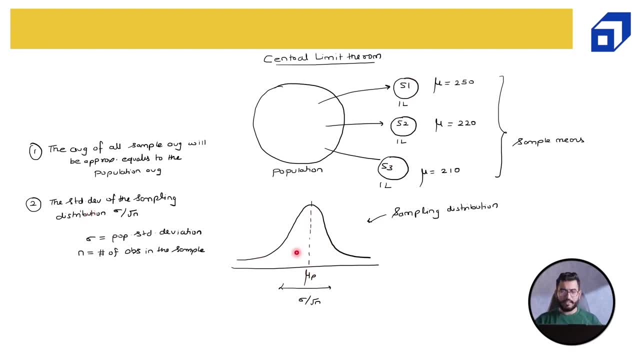 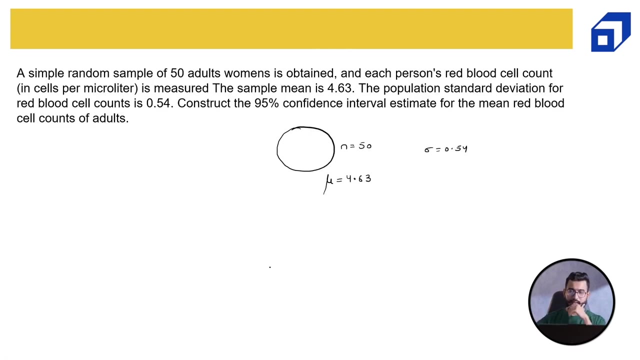 equal to the population mean And the standard deviation of the sampling distribution is Sigma divided by root of n, where Sigma is a population standard deviation and is the number of observations in the sample. Now this property is very important and very useful to estimate the population range. So 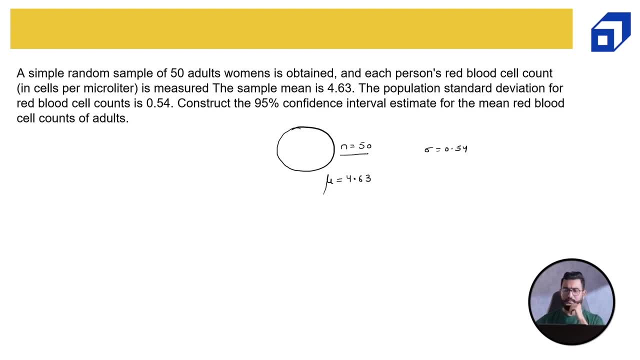 I'm given with n as 50.. My Sigma population standard deviation is 0.54.. My average sample mean is 0.4, 0.6, 3.. Now I have to construct 95% confidence interval estimate. We already know that is sampling. 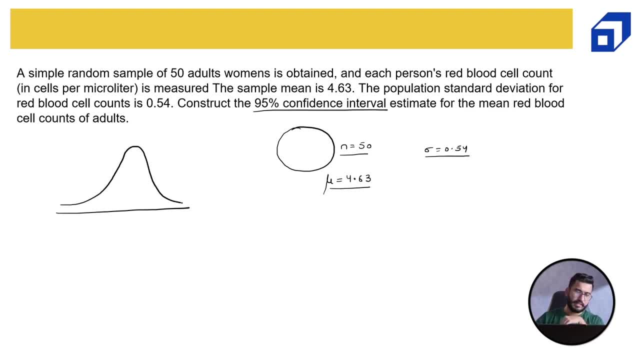 distribution follows a normal distribution. This is my sampling distribution for this particular uh, for this particular event. So I know that my sampling distribution follows normal distribution. Let's say this is my new, which is sample mean, And I want to estimate this range- lower value, upper value- in such a way. 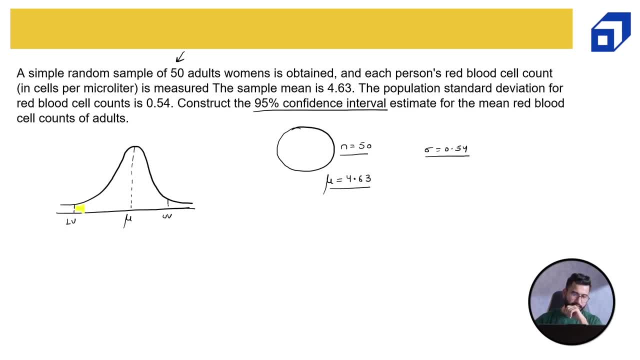 that between these two, I get. between these two, I get 95% of my data. Now, don't worry, I'm not rushing. Don't worry, I'll explain everything, But this is my, this is my problem statement. I have to estimate the lower value and the upper value in such a way. 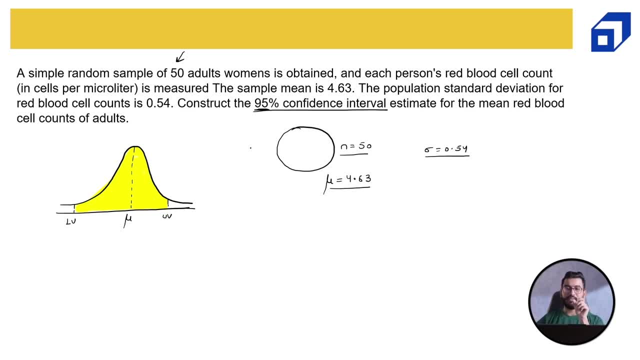 that between this I have 95% confidence. Right now we are using the word confidence, but as of now you can use the term that I need lower value and upper value in such a way that 95% of my data, percent data, is between these two values. Now we already know this, actually, that from the mean 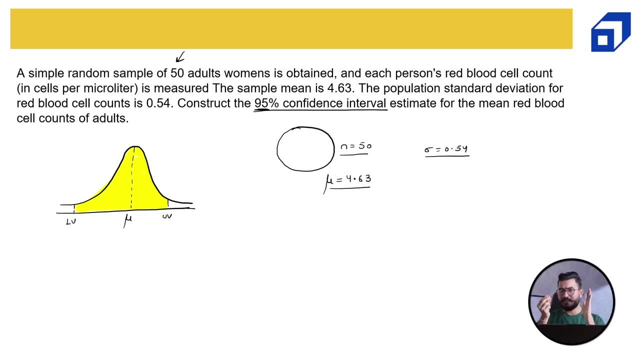 if I go below two standard deviation and above two standard deviation, I can get 95% of my data using the second property of my normal distribution right. But that is not exactly two standard deviation below the mean. I'll just tell you. assume that. assume that this is my standard. 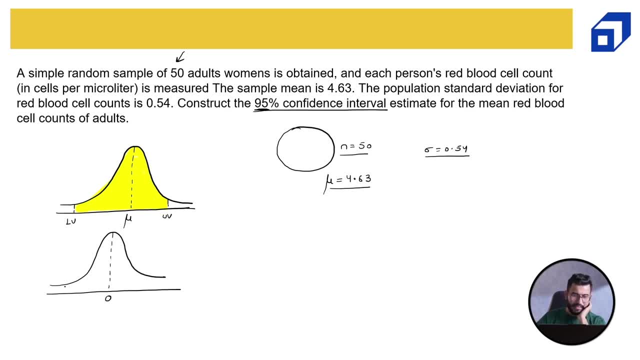 normal distribution means zero. And I have to find out. I have to find out the Z value over here. What is the Z value over here And what is the Z value over here, Z1 and Z2.. And assume that between Z1 and Z2,. 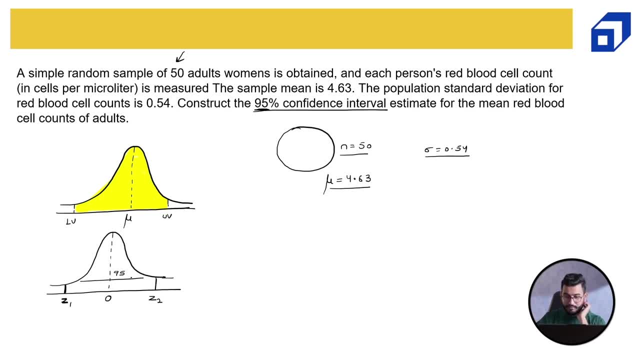 that is the standard, normal distribution, And I have to find out. the Z value over here Area is 95. So if the area is 95 between Z1 and Z2, this area, this black color area, what that will be, What that will be. So the total sum of these two black area will be 5%. 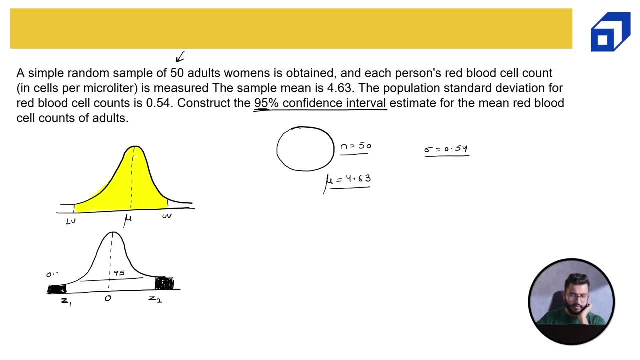 So this will be 0.025 and this will be 0.025.. How So total is one between these two data points, Z1 and Z2, my area is 0.95.. So I'll subtract, So I'm left with 0.05, sorry, 0.05.. 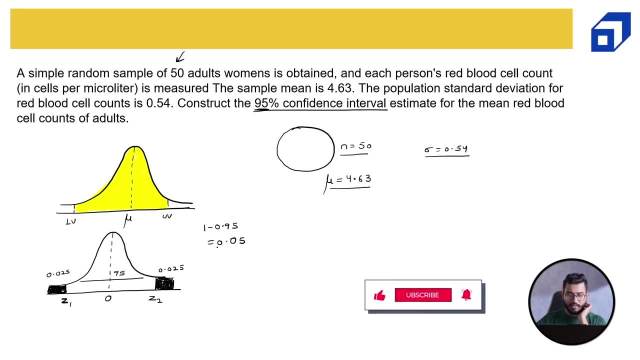 Now, since I'm having two shaded regions, I will divide it by two, So I'm left with 0.025.. So half is over here and half is over here. Now I have to find out the Z value over here. So from here to here, the area under the curve is 0.025.. Let's quickly use our Z table. So. 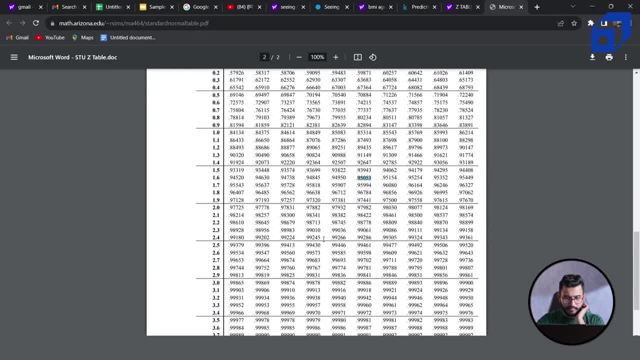 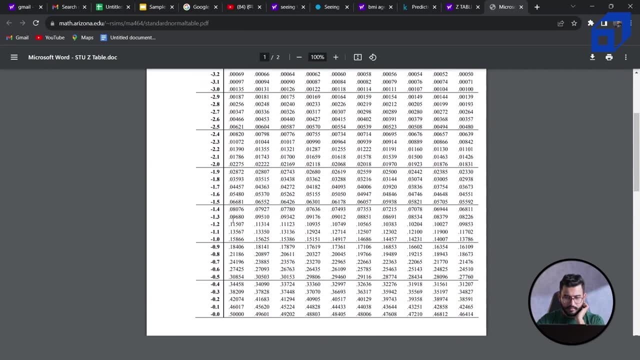 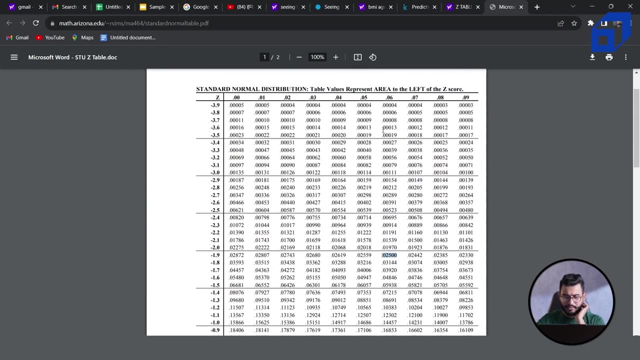 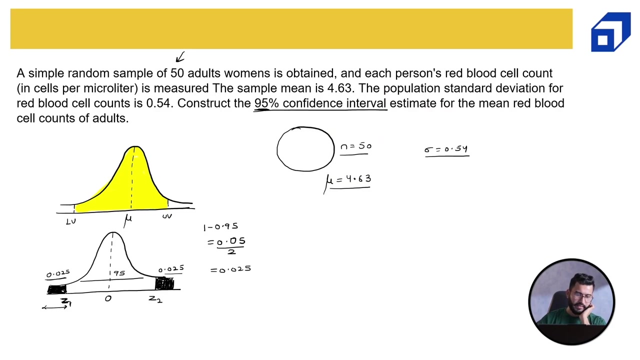 0.025, I have to go on the negative scale. 0.025 is over here and this is minus 1.9 and six. You can see it is not exactly two, it is minus 1.96.. So this is this point: Z1 is minus 1.96.. Similarly, to find out Z2, I have to 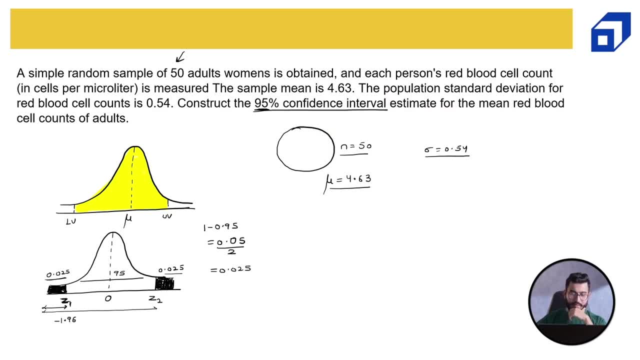 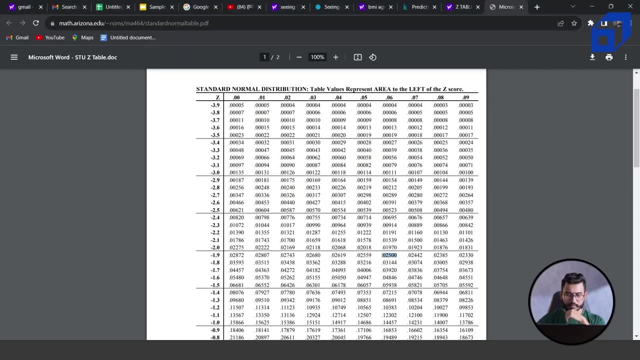 go from here all the way up to here, So that will be 0.95.. This is middle region plus 0.025.. So that will be 0.975.. So let's look at 0.975.. So 0.975,. 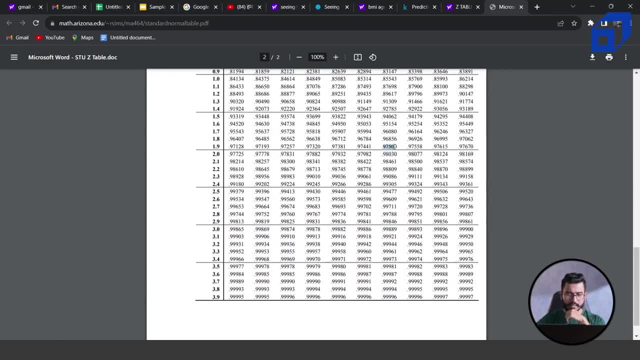 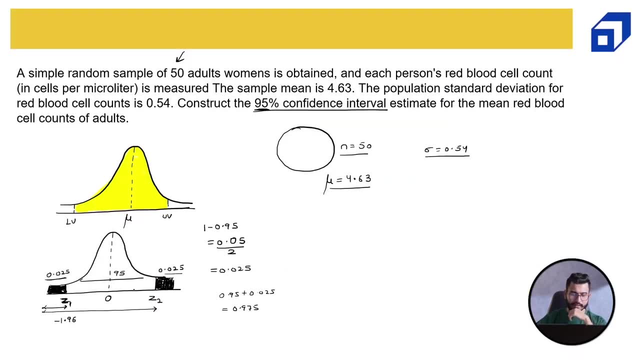 975 is over here. This is plus 1.9 and six We have plus 1.96.. Now we have the lower Z value and upper Z value From the sample mean to estimate, to estimate population range or population parameter range. 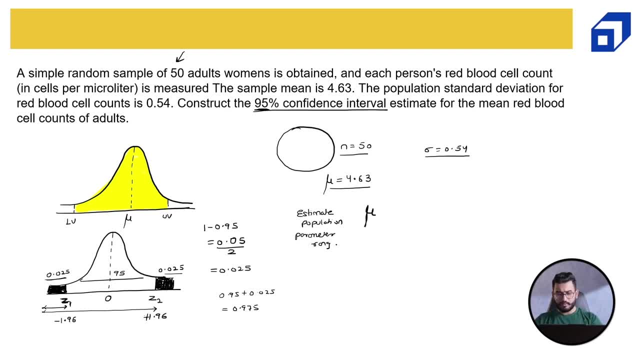 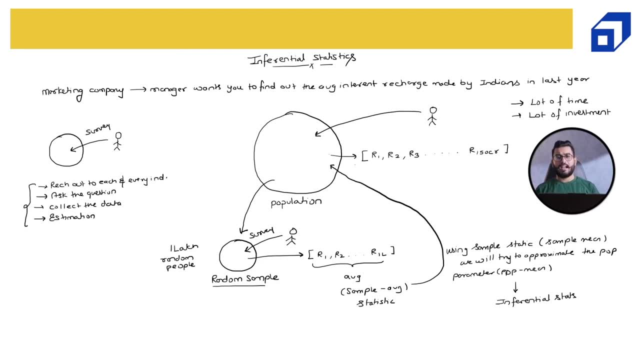 Why I am estimating range. because if my manager is asking me to find out average recharge made by the Indians, And anyways, if I'm using sample mean, I'm not 100% sure right, So I can not tell my manager that the sample mean was for. 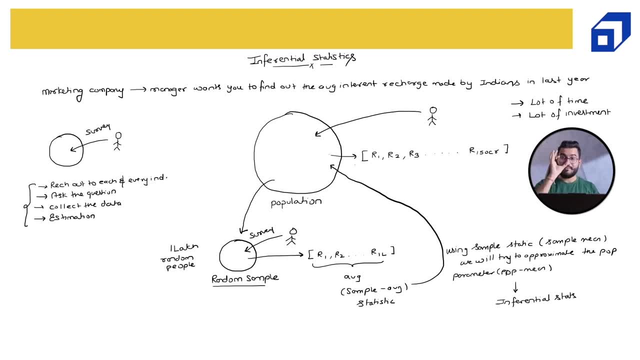 let's say 280 rupees, because I have just analyzed one sample, I have just surveyed one sample, So I have to tell my manager with a range that I can tell to my manager that. okay, sir, I don't know exact value. 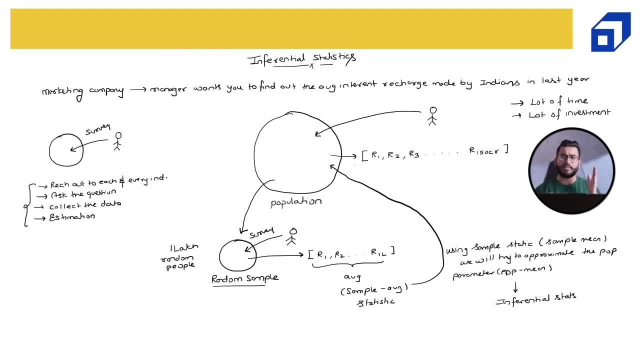 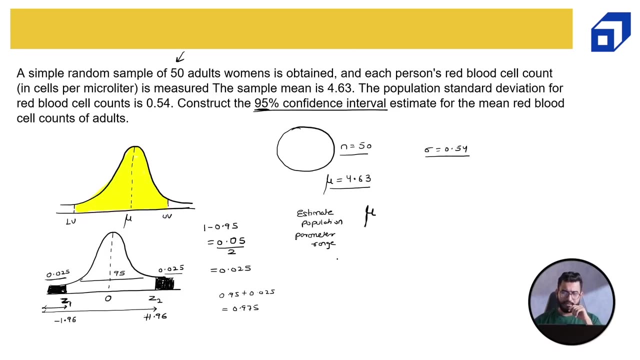 but I'm sure I'm 90% confident. so I'm 95% confident that my population mean lies somewhere between these two values. So that is what we are trying to estimate. So, if I go back to my question, to estimate the population parameter range, 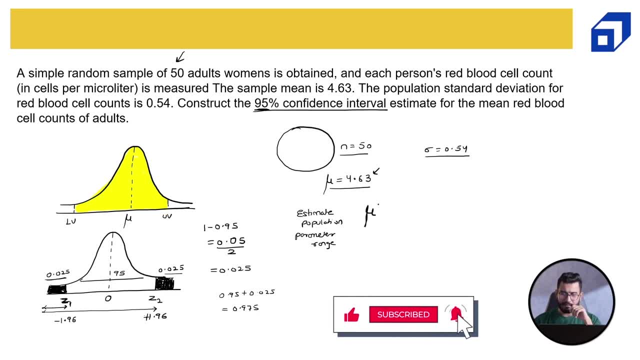 in my sample mean. this sample mean, we will add and subtract the z times of sigma divided by root of n, What is z. So from this value I'm moving 1.96 standard deviation below the mean. 1.96 standard deviation above the mean. 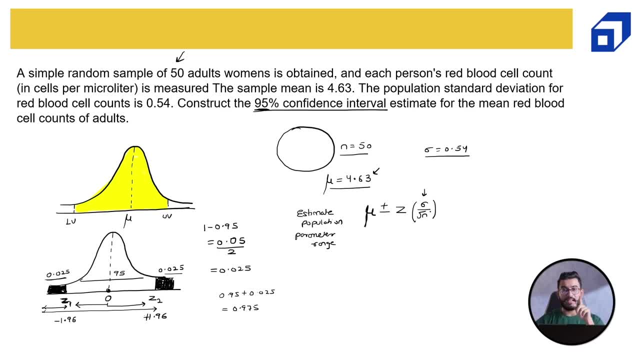 of the standard deviation, of the standard deviation of my sample. So essentially what we are trying to do from the mean, from the sample mean, we are just moving below and above, below and above, so to get this lower value and the upper value. 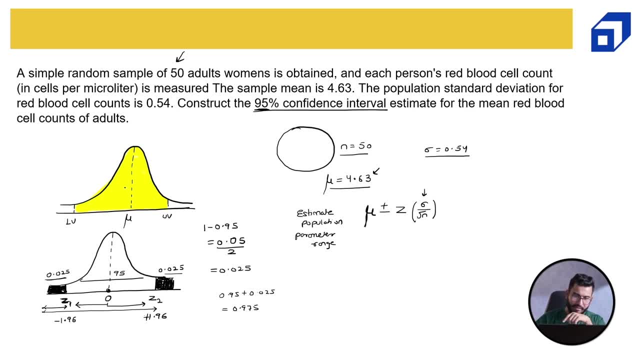 So this is my mean: In order to get 95% confidence, I will move minus 1.96 standard deviation below, plus 1.96 standard deviation above the mean, and that will get me the population range. So mean is 4.63, plus minus 1.96,. 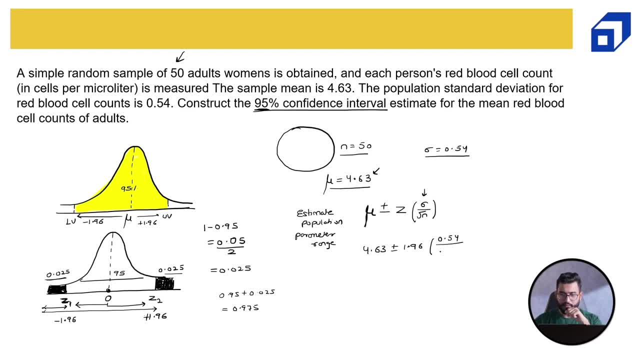 standard deviation is 0.54, divided by sigma of root, 50.. If I solve this, 4.63 plus minus, so this will come out to be 0.149.. So this will come out to be 0.149.. 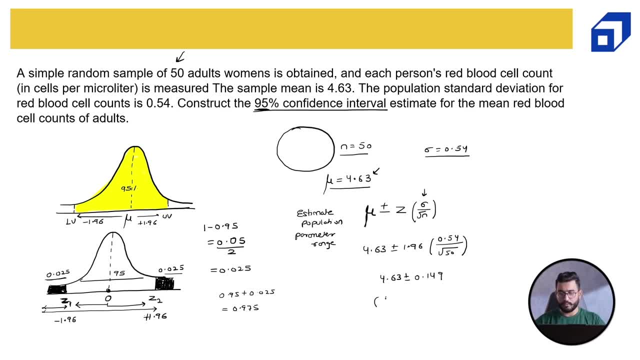 So this will come out to be 0.149.. And the range would be 4.481, 4.779.. And the range would be 4.481, 4.779.. And the range would be 4.481, 4.779.. 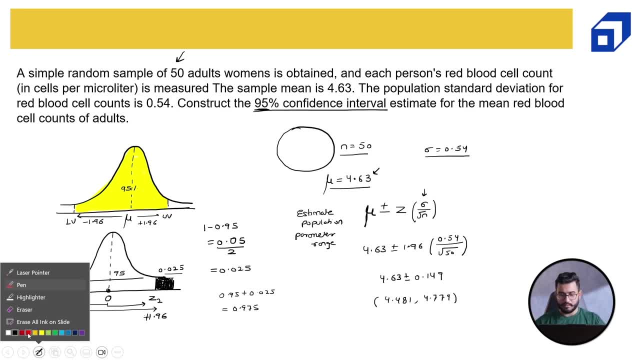 What is the meaning of this? This basically means that there are 95% chances that the actual population mean. that the actual population mean would lie somewhere between 4.481 to 4.779.. that the actual population mean would lie somewhere between 4.481 to 4.779.. 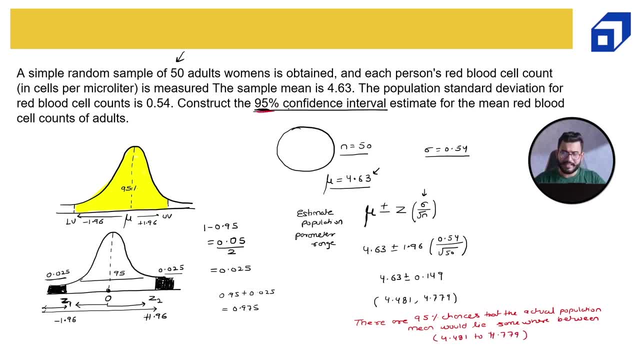 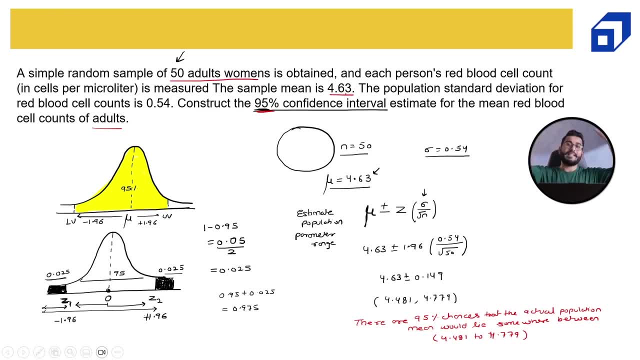 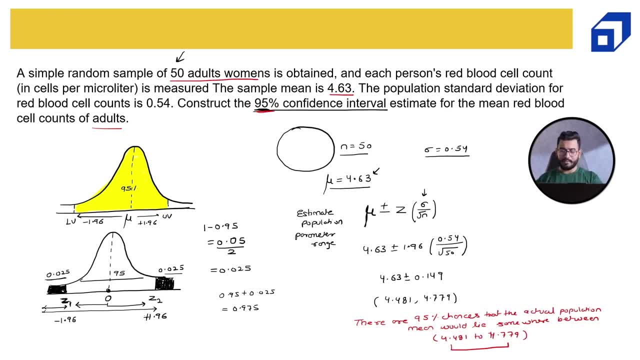 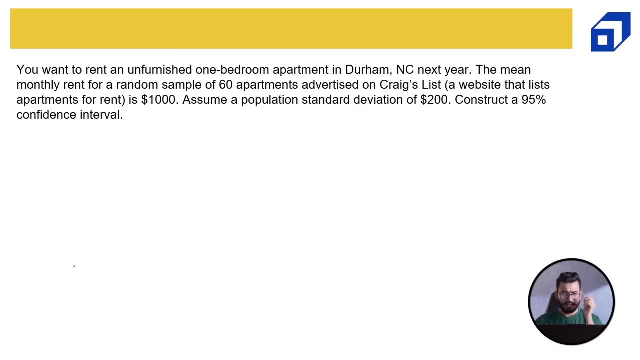 That is what this range is. Let's look at one more question and then it will clear all your doubts and it will be very clear to all of you. So the question says: you want to rent an unfurnished one-bedroom apartment in New York City. 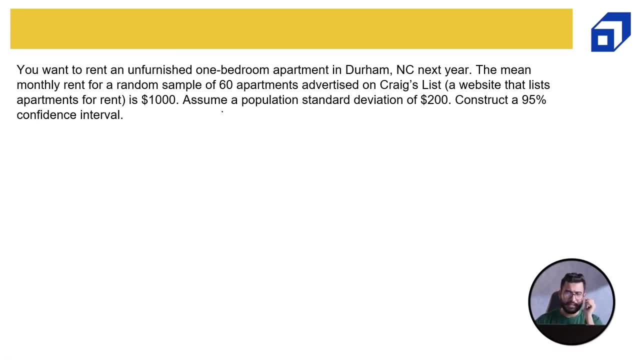 The mean monthly rent of random sample of 60 apartments advertised in some website came out to be $100.. So what you did? you were trying to estimate what is going to be the average one-bedroom cost, or average one-bedroom cost or average one-bedroom rent in New York City. 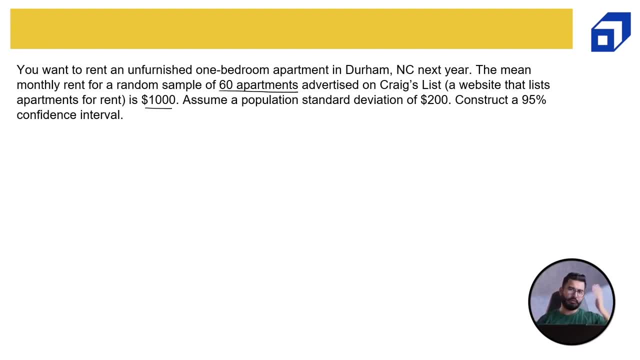 So what you did? you Googled and you searched through some website. you sampled 60 apartments in the same city. So 60 apartments, my N is 60. And after looking at all the rent, the average of the sample came out to be $1,000. 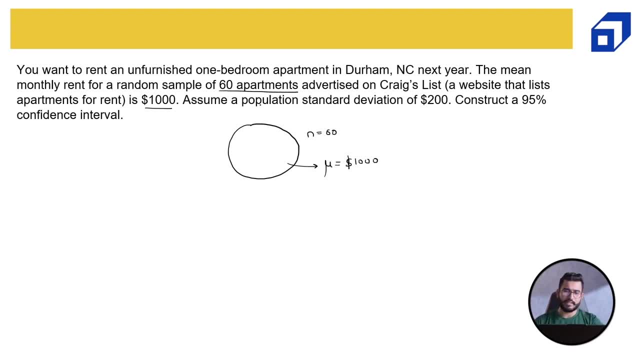 And the standard deviation was. you assumed that the population standard deviation to be $200.. So this is just an assumption. Population standard deviation is $200.. This is population. Now we have to construct 95% confidence interval Again for 95%. 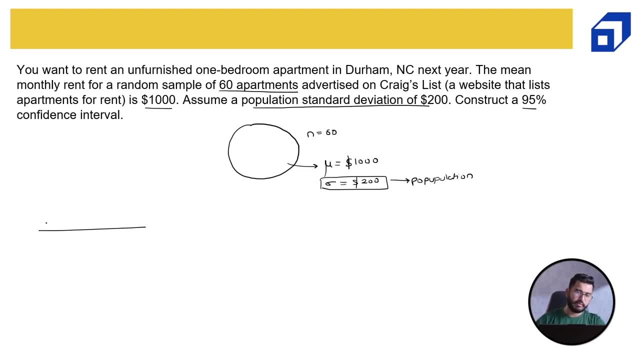 we have already calculated the Z values. So the Z values is minus 1.96 plus 1.96.. So we will just apply the formula mean plus minus Z times of 60.. Sigma divided by root of N mean is 1000 plus minus 1.96.. 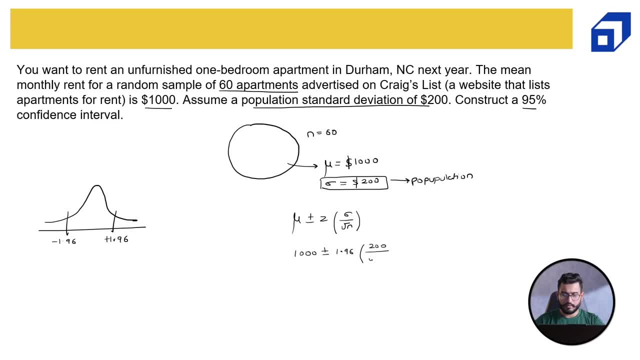 Sigma is 200 divided by root of 60. And if I just quickly solve this, it will came out to be 949 comma 1050, which basically mean there are 95% chances that the average rent is going to be $1,000.. 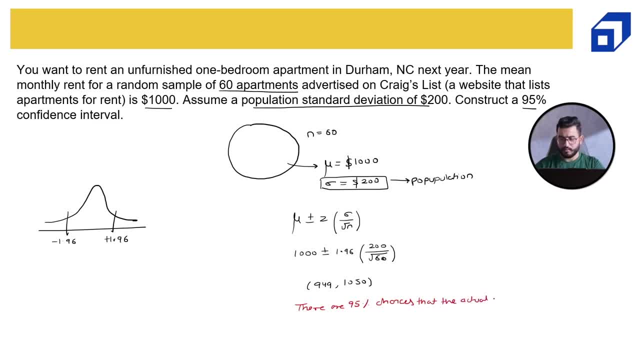 that the actual rent of one bedroom, one bedroom apartment in New York City would be somewhere between $949 to $1050, and this is what the application of inferential statistics is. I hope you guys are able to connect all the dots and able to understand how we have arrived. 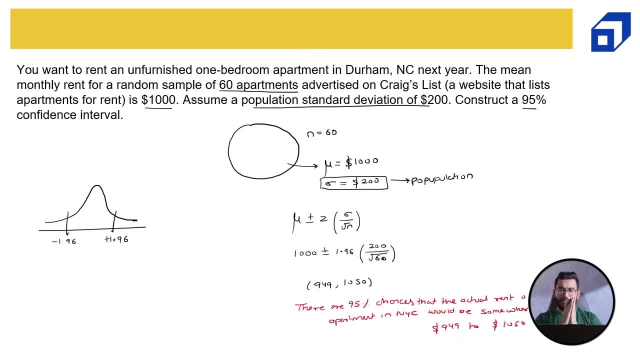 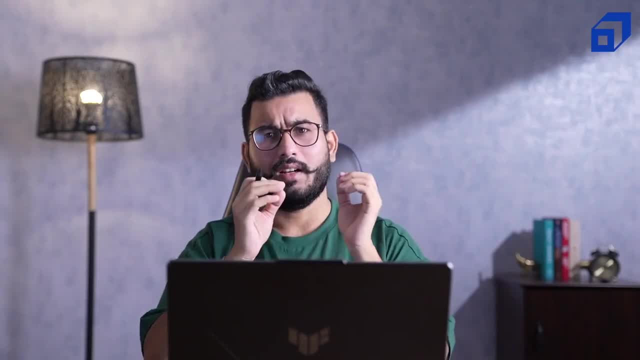 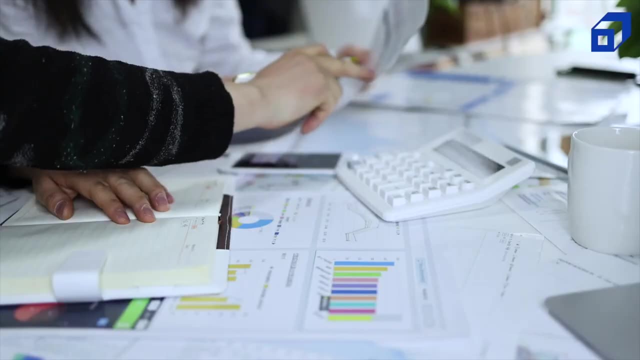 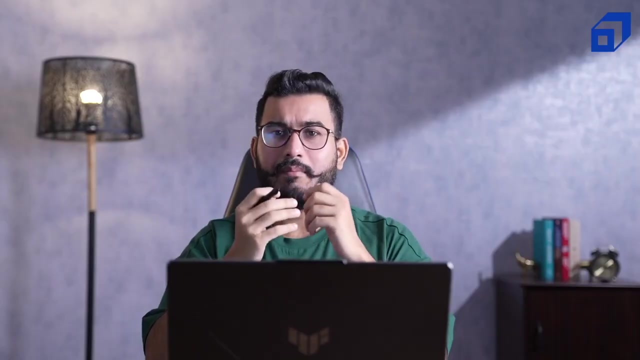 to this particular point Now. this concludes our discussion in inferential statistics. So till now we have talked about descriptive statistics, we talked about probability and we have also looked at how we can use inferential statistics to approximate the population parameter, given the sample statistic. So this is all what we have covered. 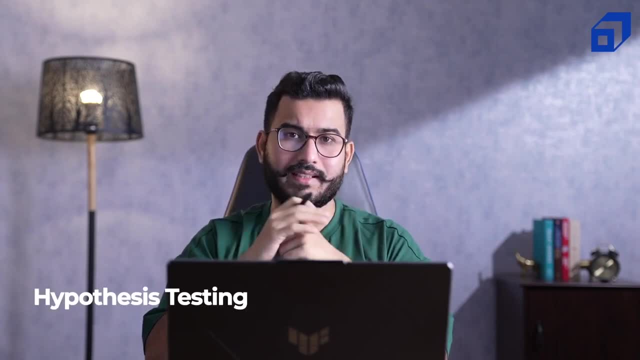 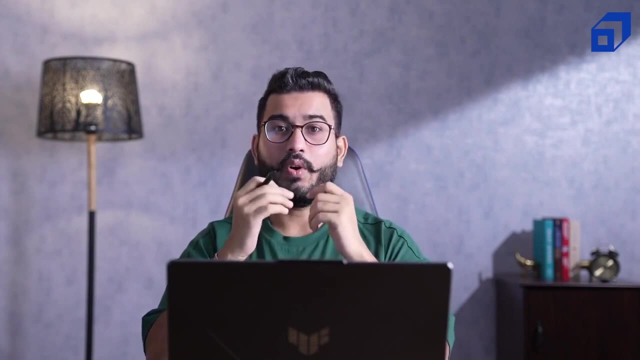 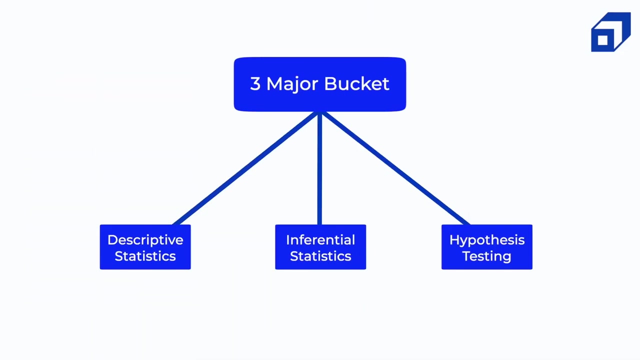 Now we are going to start with hypothesis testing. Now I have already given you a brief idea behind what hypothesis testing is. So when we started this video, we briefly discussed about all the three major buckets: What is descriptive statistics? What is inferential statistics? 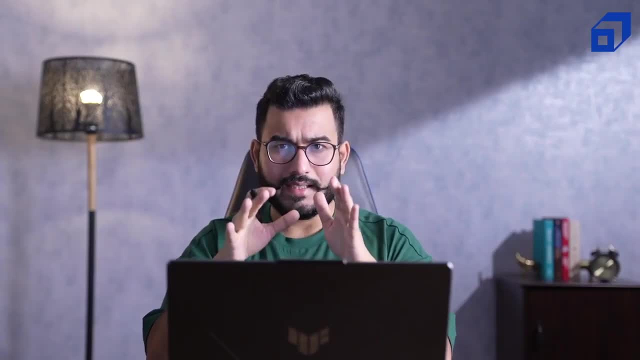 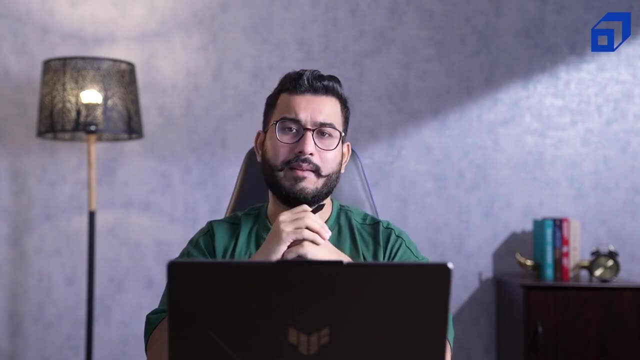 What is hypothesis testing? But in this section, we are going to have a detailed conversation regarding what exactly is hypothesis testing and how this can be useful when it comes to data science or when it comes to data analysis. So let's get started. So let's start this discussion Now to understand hypothesis testing. 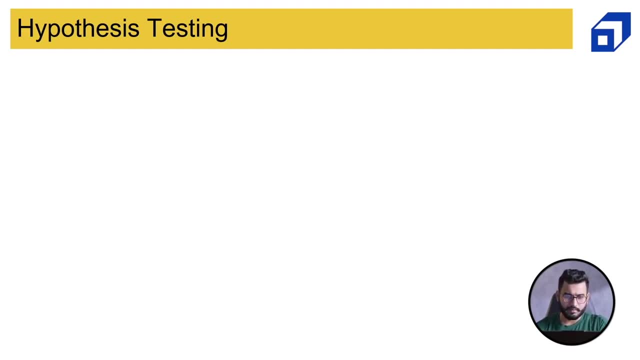 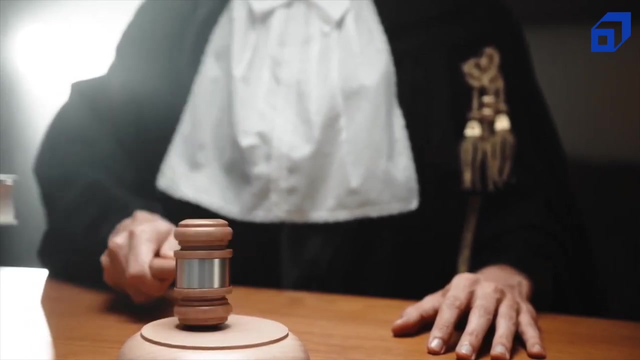 we will take one example. So let's say there is a court, So let's say this particular person is the judge sitting in the court. So judge in the court, and we have two lawyers and we have the person sitting in the court. So judge in the court. and we have two lawyers and we have the 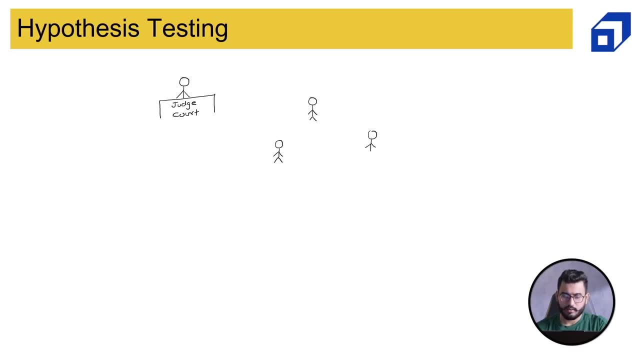 person who has been convicted. So this person has been charged, charged for some crime. Let's say, this person is talking in favor of the convicted person and this person is the against the person. Now, if I ask you, what would you say about the person who has been convicted? 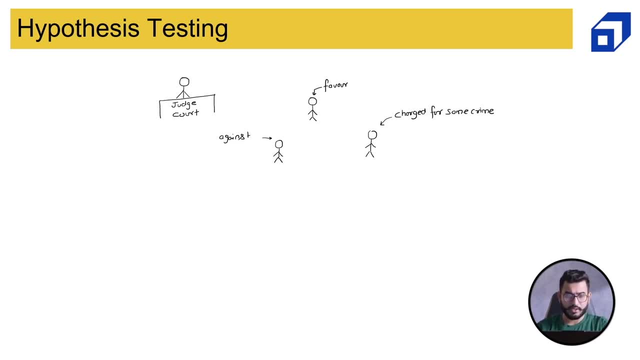 What would you say about the person who has been charged for some crime? So the judge will be the thought process this judge will be having in his or her mind regarding this particular person who has been charged for some crime. You guys can easily say that the judge will be having two assumptions, or maybe two hypotheses. 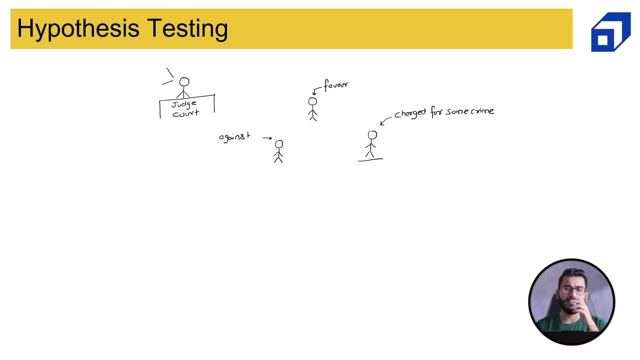 or two thought process, If I tell you like, if we think in general English, it would be two thought process. Either the person is guilty or the person is innocent, right? So that is what the judge will also be having in their mind. So either the person is guilty or the person is innocent. 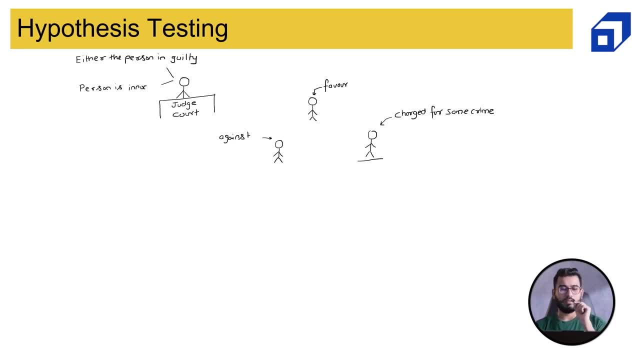 Now the judge will decide after listening to both the lawyers: the particular lawyer who is talking in favor of the charged person and then another lawyer who is talking in favor or in the against the charged person. So the judge will listen to both these parties and then. 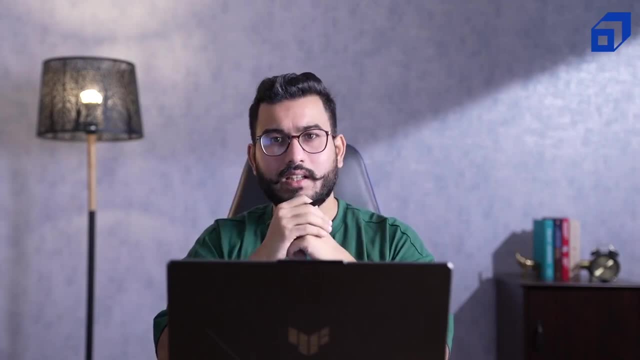 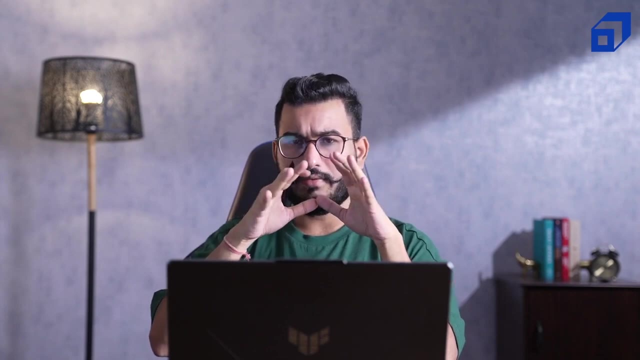 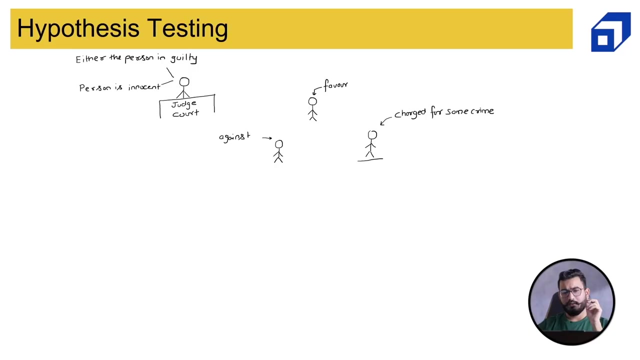 they will declare or they will come to a particular conclusion right Now. this is basically the framework of what hypothesis testing is. So in hypothesis testing we have two thought process, two assumptions, and we try to conclude, we try to prove one of them. This is a very raw definition. 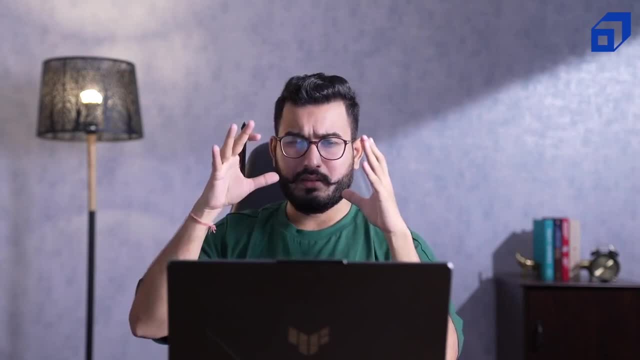 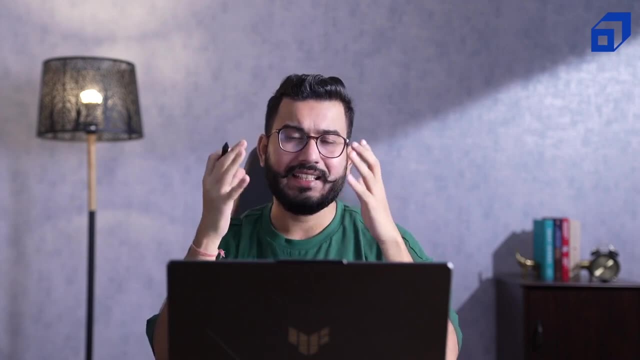 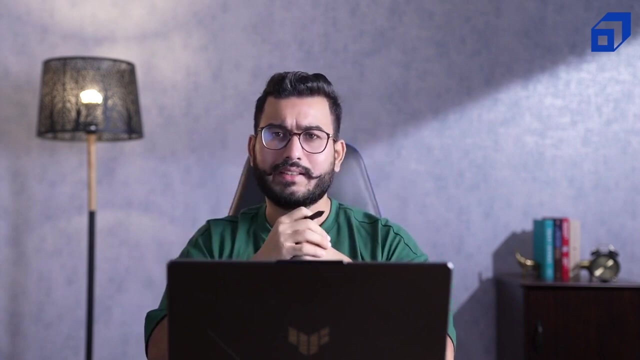 This is not 100% correct, But the reason I am talking in this way is because I wanted to create a create a base of what exactly is hypothesis testing. So just keep this example in your mind and whenever somebody is asking you what exactly is hypothesis testing, you can just: 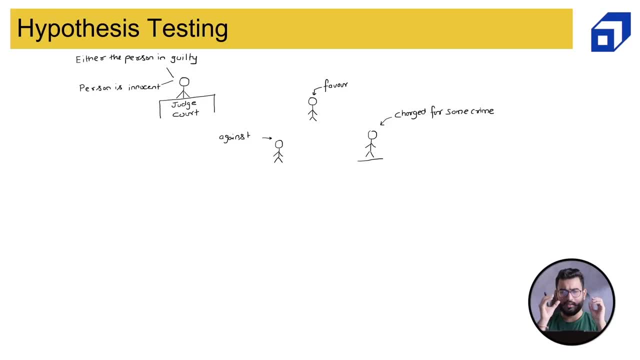 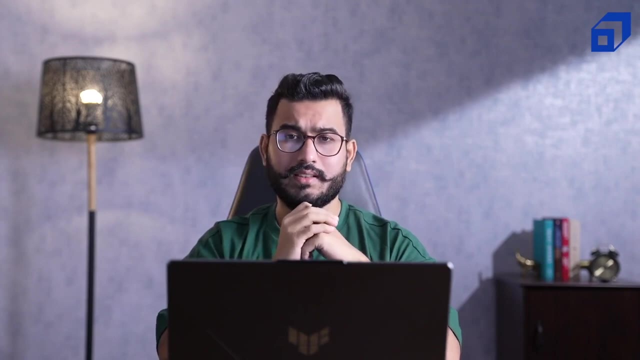 generate this picture in your mind: that there is a courtroom, there is a judge who is listening to both the lawyers- one in favor and one in against- and there is a convicted person. Now either the person is guilty or the person is innocent. these are the two hypotheses. 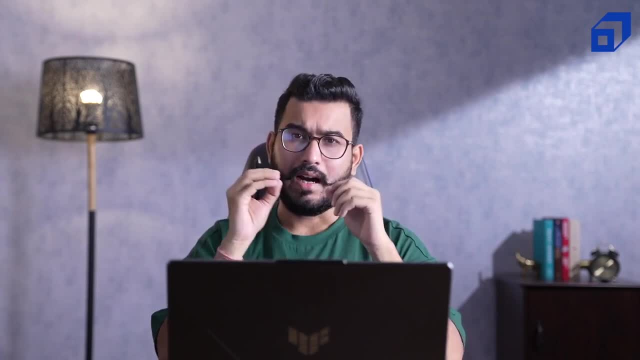 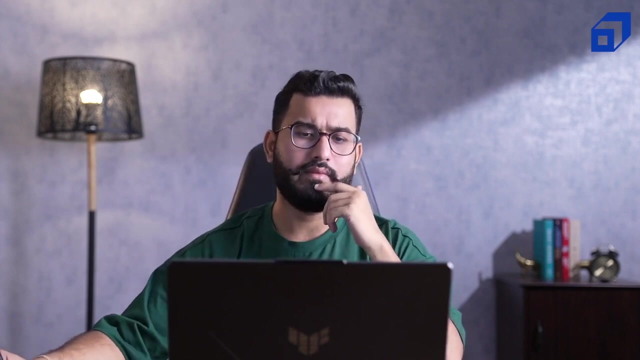 that the judge will be having in their mind. After listening to the whole conversation between these two lawyers, the judge will come to a conclusion, and that is what the conclusion which we are trying to achieve. right, So the complete hypothesis framework is having two stages. Number one is to formulate the hypothesis. 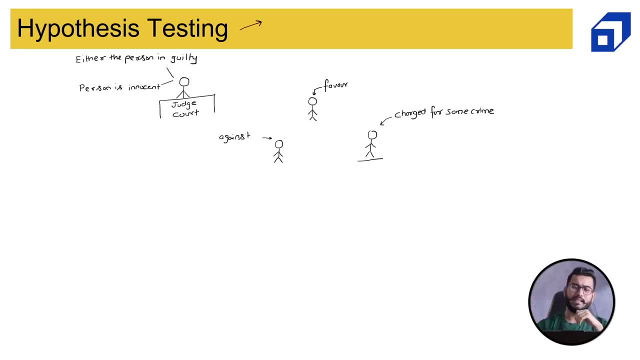 So, given a problem statement, we have to formulate the hypothesis. So formulation, Formulation of the hypothesis. And number two is the test. So we will perform the test to reject or to fail to reject one of the hypotheses. Now, please don't worry about the term which I 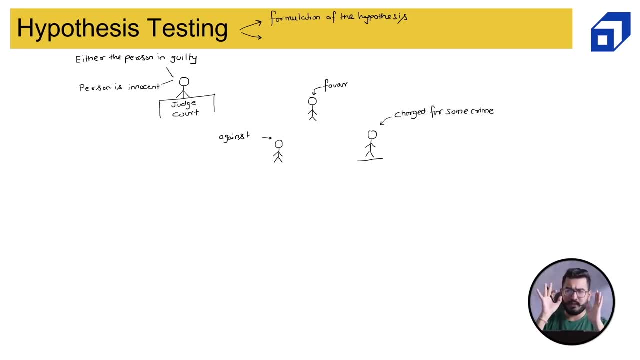 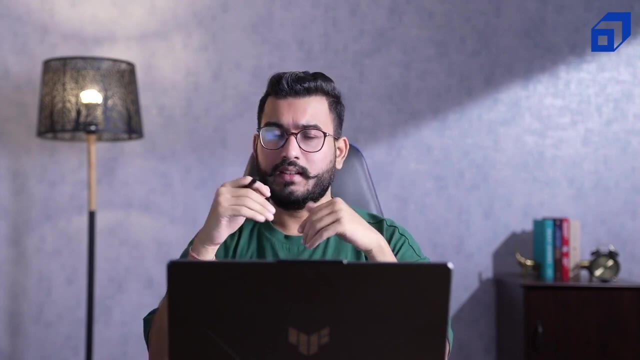 have just said Reject, Reject, Reject, Reject or fail to reject. But just remember that we will first formulate the hypothesis given a problem statement. So let's say your manager has given you a problem statement, You will first formulate the hypothesis and then you will perform the test Based on the 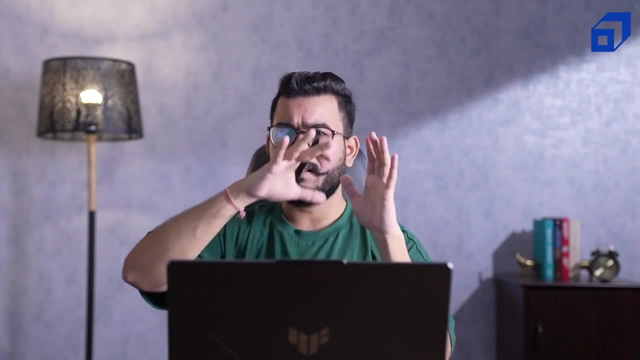 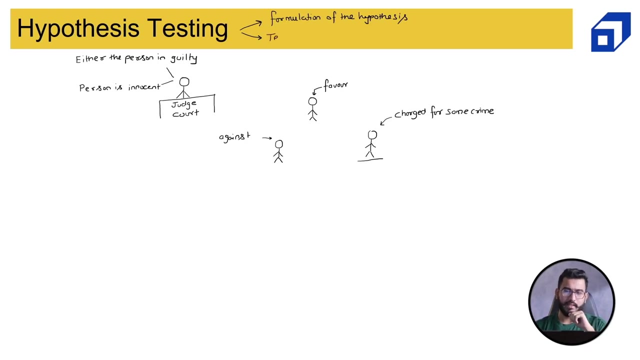 test result, you will make some conclusions. So this is the simple process of hypothesis testing. So the next step is testing or performing the test. So the next step is testing or performing test. So the next step is testing or performing test, and then, finally, conclusion. 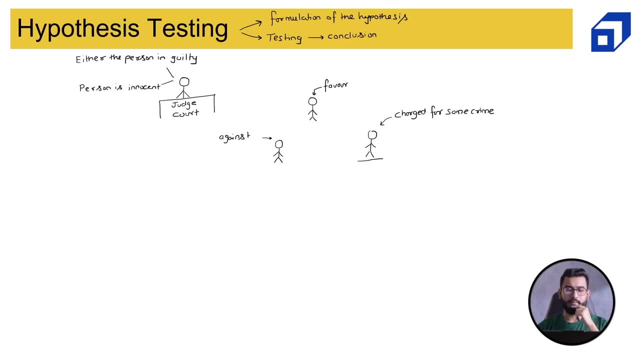 Now let's understand the formulation of hypothesis, As I have just told you that this judge would be having two thought process in his mind or in their mind. Either the person is guilty or the person is innocent. Now there is a formal word or there is a formal name given. 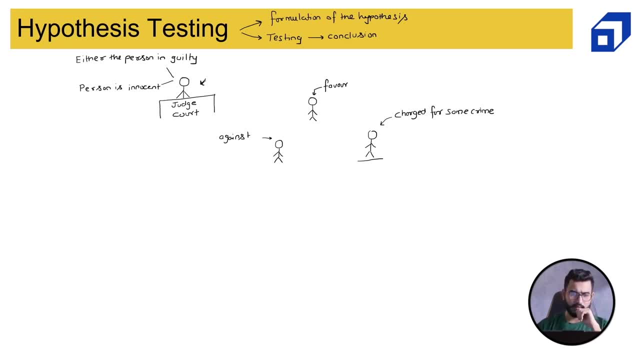 these two thought process. One is known as the null hypothesis and another one is known as the alternate hypothesis. Null and alternate hypothesis. Now, what is null hypothesis? Now, if I ask you, before this person was charged for crime, before this person was taken to, 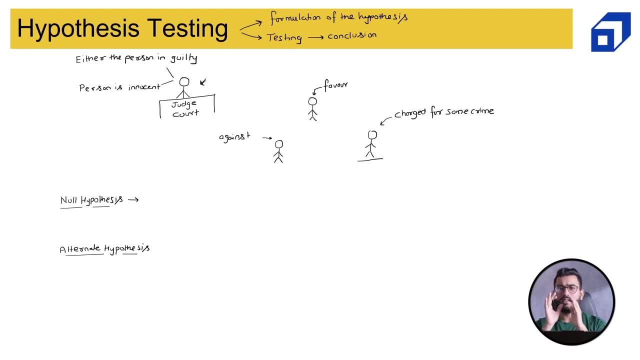 the court. Initially this person was innocent, right? So Null hypothesis talks about the initial state of anything, Or initial state of the particular item or particular case that we are trying to test. So Null Hypothesis is basically the initial state of the case we are trying to test. So the initial state. 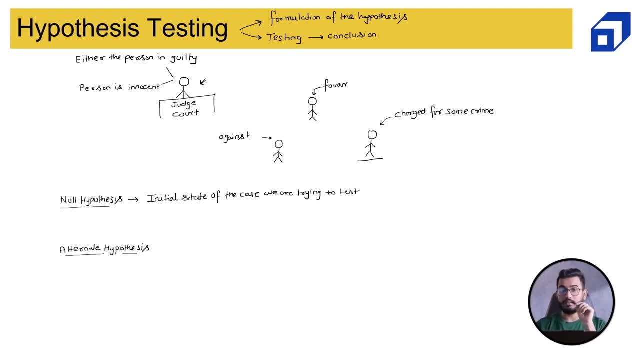 of this person is that this person was innocent before this person was taken to the court, before this person was charged for some crime. this person was innocent before anything happened to him. he was innocent. So my null hypothesis is: the person is so H naught, so null hypothesis. 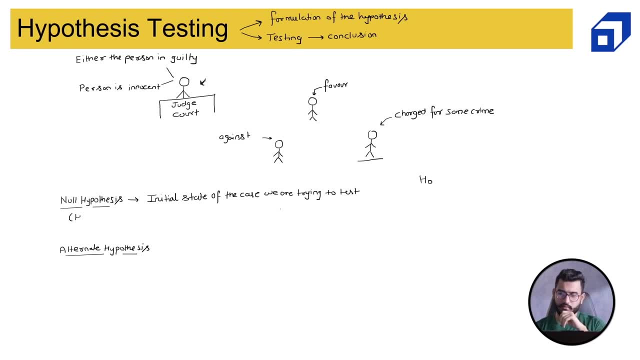 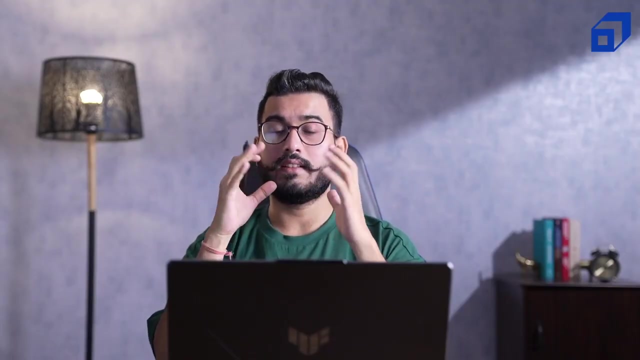 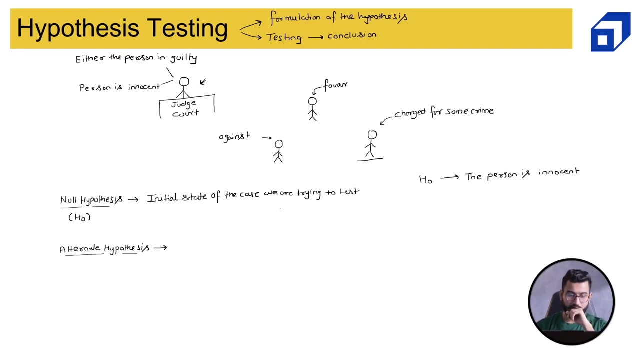 can also be represented as H naught. The person is innocent. Now the alternate hypothesis is: what new thing has been happened, what new we are trying to prove? the new thing that has happened to this person is: this person has been charged for crime now. So this is the new thing, or new state, or the claim, or 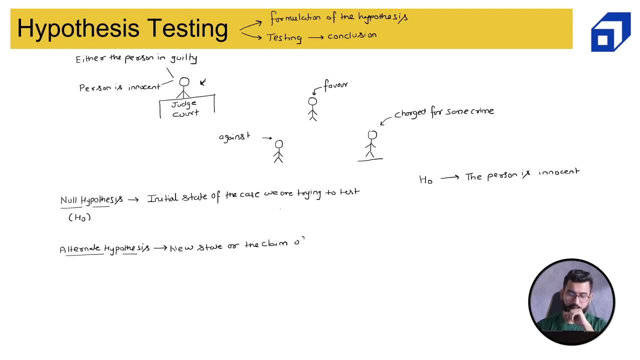 the case we are trying to test, We are trying to prove. So H- alternate hypothesis can be represented as H and in this case it will be: the person is. the person is guilty. So this is how we can formulate the hypothesis. Please remember. 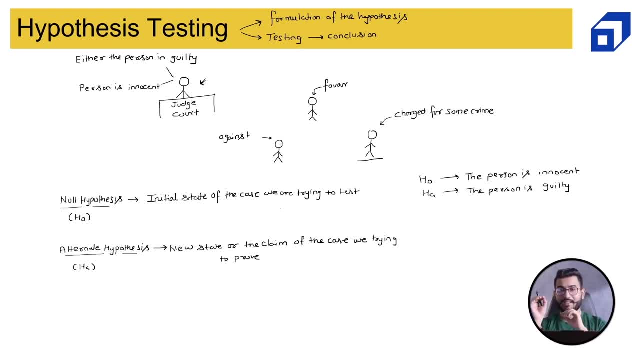 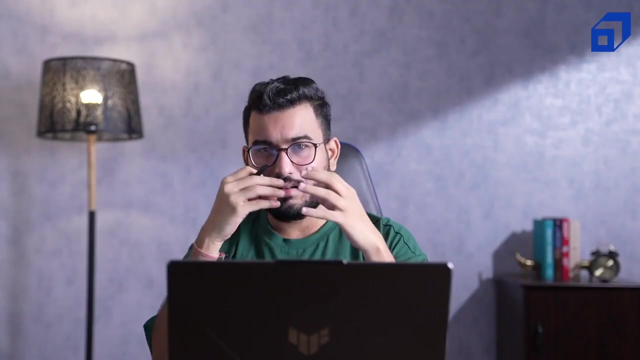 null hypothesis represents the initial state of the person or initial state of the case which we are trying to test, and alternate hypothesis is basically the new finding, the new thing- or maybe not the new happening which for the particular case which we are trying to prove or which we are trying to test now let's take few examples just to understand how we can. 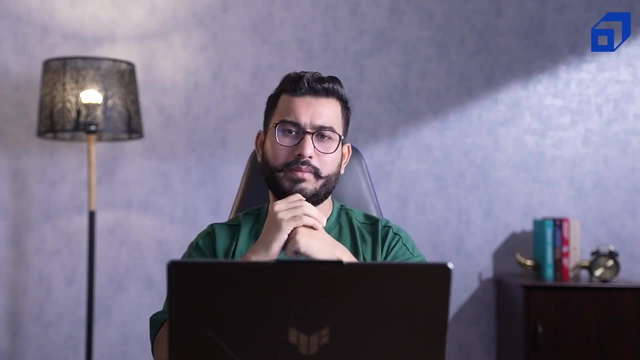 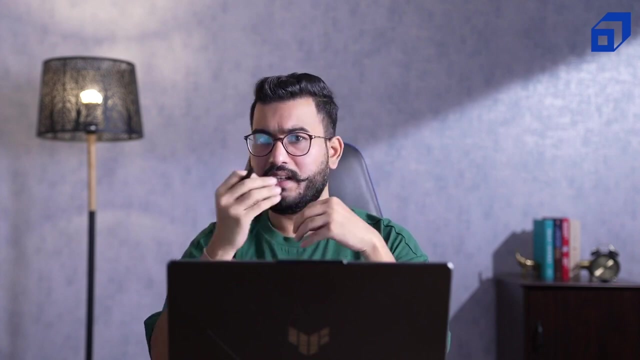 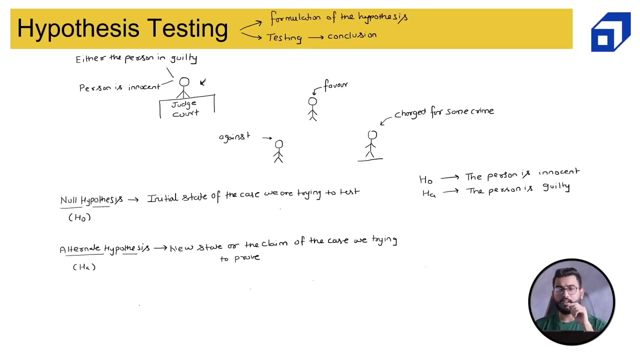 formulate hypothesis given any problem statement. so right now this was not the problem statement. this was a very plain example. but now we will be looking at some problem statements which will have some sample, mean, population, mean, standard deviation, to understand how we can formulate the hypothesis now before we talk about some business examples to better understand. 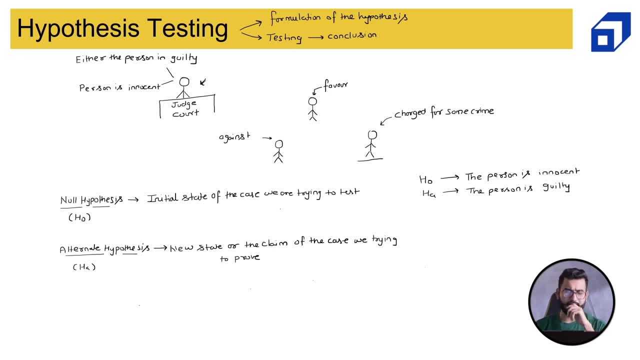 how we can formulate the hypothesis. we can formulate the hypothesis to formulate the null and alternate hypothesis. we will understand a very small topic which is really important when we conclude. So whenever we conclude the hypothesis testing during conclusion, we say that we reject null, or either we say that we fail to reject null. 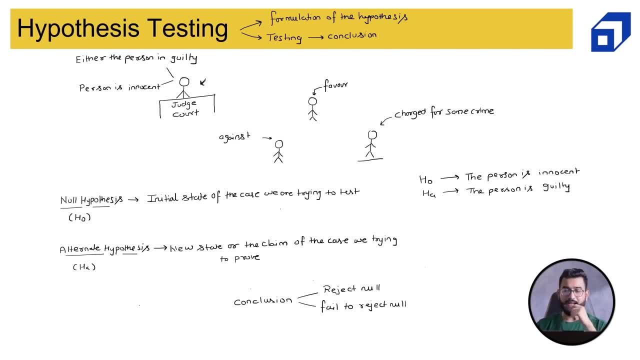 Now we never say that we accept null or we accept alternate. So what we never say, we never say, we never say we accept null or we accept alternate. Now there is a reason for this. So this is the something which I should mark in red color, because this is wrong. 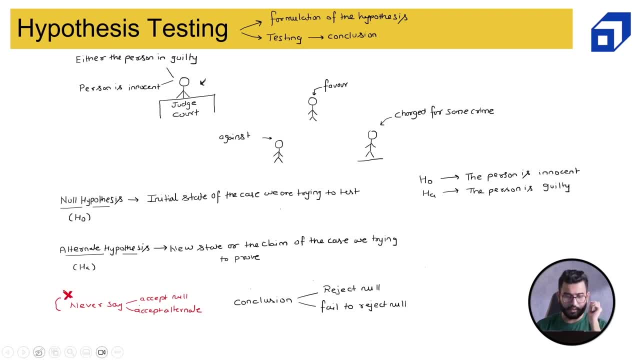 We never say this. Now, the very first thing that we should understand is: why are we only rejecting null and fail to reject null? Why it is only null, Why it is not alternate? Well, the reason is because null hypothesis is something that we know, that we certainly. 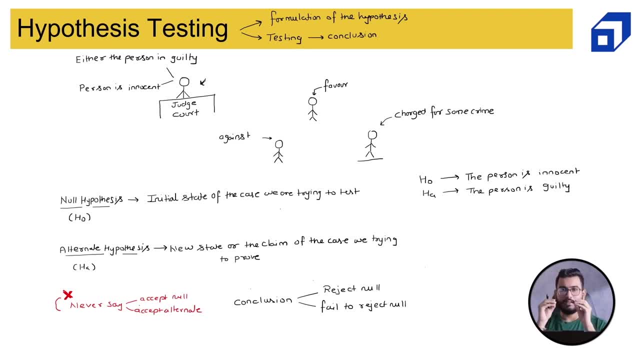 know, We are 100% sure that this person was innocent before committing crime or before the person was charged for the crime which in the court, somebody is trying to prove. So the reason we conclude on the null hypothesis is because null hypothesis is the statement. 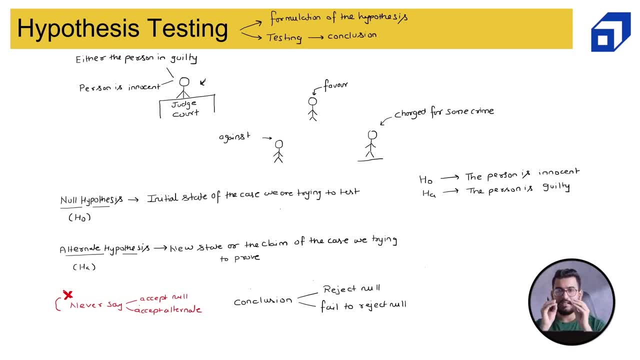 which we are certain about. We know that, initially, this is something which actually is null. This is something which actually happened. The person was actually innocent and we are certain about it. We are 100% certain about it. Now, why we don't say: accept null. 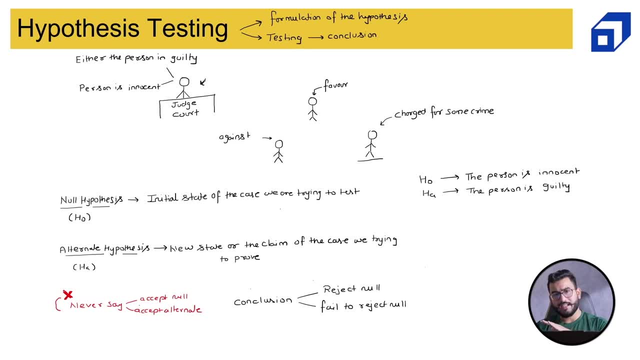 If I say accept null, we are completely ignoring the fact that the person was guilty. Now it might be because of the lack of evidence. So if I say I accept null, I am 100% sure that the person was guilty. So if I say I accept null, I am 100% sure that the person was guilty. 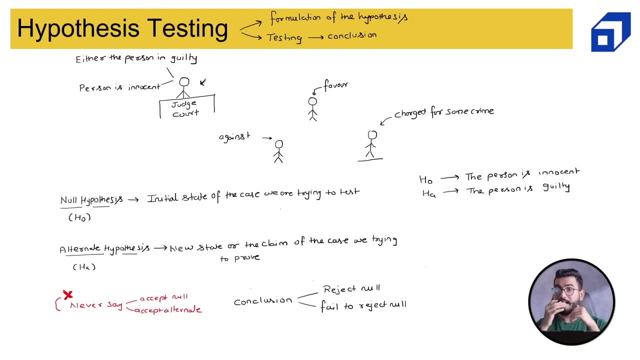 Now, it might be because of the lack of evidence. It might be because- so let's say, this person who is talking against the charged person- he was not able to present enough evidence against the court, due to which he was not able to prove that the person is guilty. 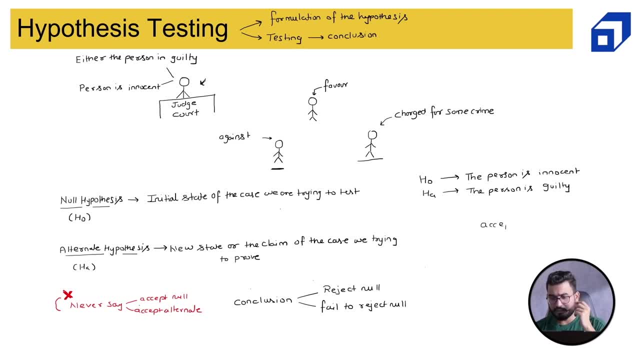 So when I say that I accept null, I accept null. Okay, So I am basically ignoring the fact, and I'm 100% certain that this person is innocent, and I'm ignoring the fact that this person is guilty, which is not true. 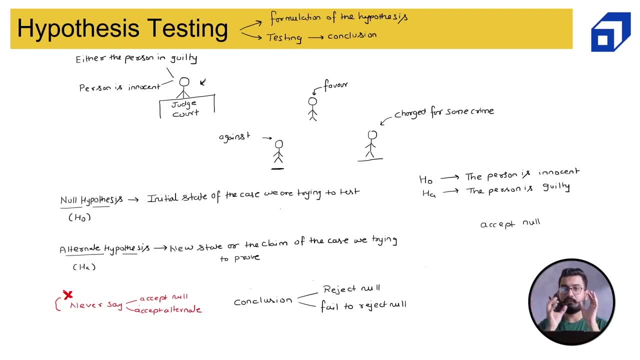 We have to be uncertain, We have to keep some uncertainty. So the uncertainty is the lack of evidence. When we say that I reject null, I'm saying that I'm rejecting null, but I'm not saying I'm accepting null. Rejecting null means I'm accepting null. 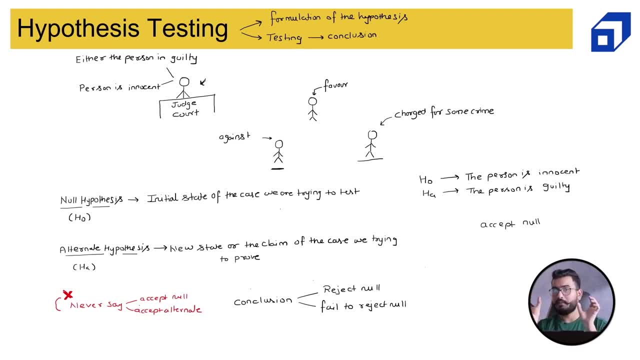 I'm not 100% sure and it might be because of the lack of evidence. Now, when I say accept alternate, the reason why I don't say accept alternate, so accept alternate- basically mean that I'm 100% sure that the person is guilty. 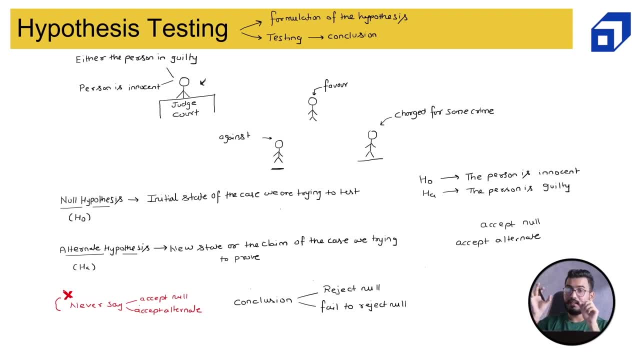 Now, again, there might be the lack of evidence. The person who is talking in favor of this person was not guilty, Okay, Okay, So again, we are not able to collect enough evidence to prove that this person was innocent or this person is innocent. 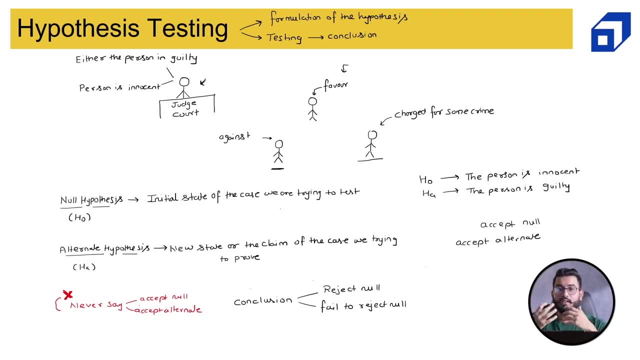 So, again, when we say we accept alternate, we are completely ignoring the fact that there is some uncertainty that can happen. So, in order to make sure that while we are concluding something, we have the uncertainty in our decision and there are chances, There are chances or there are possibilities of other thing happening because of the lack. 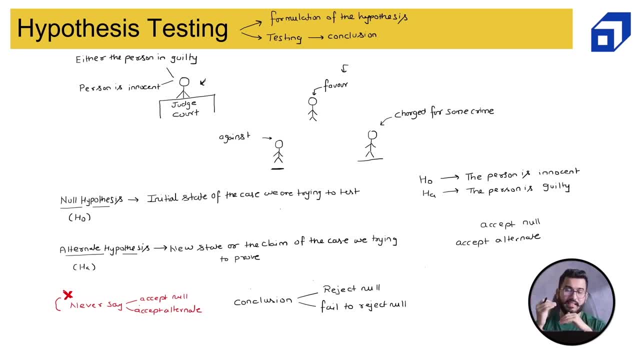 of evidence. We only say that we either reject null or we fail to reject null. I hope this makes sense. If it is not making sense, just remember one thing: we only say reject null or fail to reject null. We only use the null hypothesis because we are a hundred percent sure that null was a 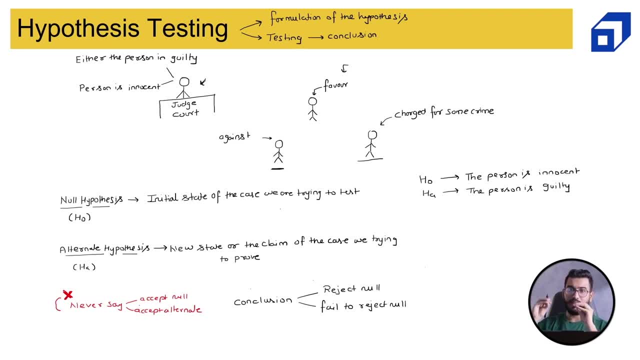 fact That null was true. Null happened. Null happened in reality. This person was innocent in reality. That is the reason we use null. The second reason why we do not say accept null or accept alternate is because there might be lack of evidence due to which I was not able to prove the statement. 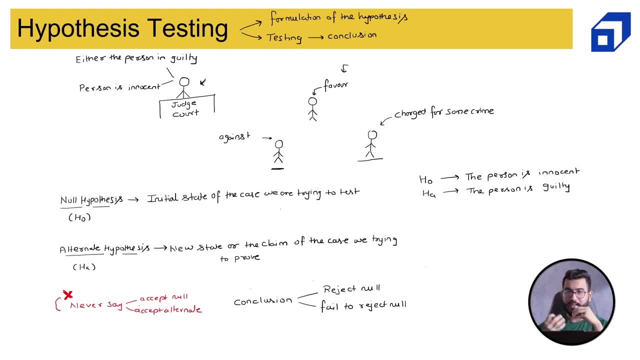 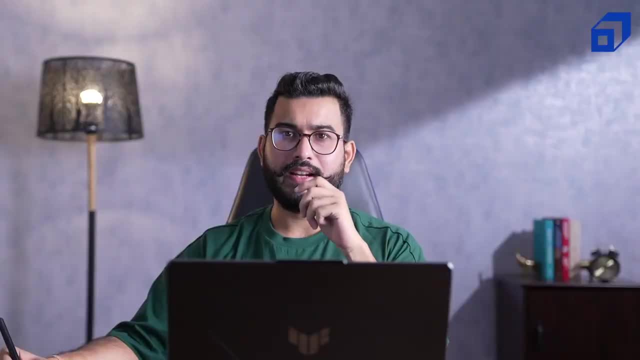 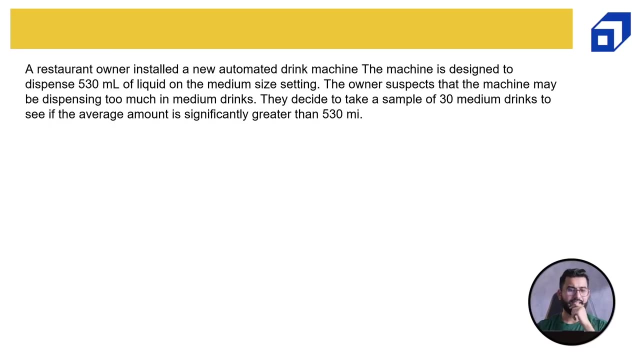 So, in order to include the uncertainty in my conclusion, Okay, In conclusion, we only reject or fail to reject null. I hope this makes sense Now, given a particular problem statement how we can formulate the null and alternate hypothesis. So in this particular question, it states that a restaurant owner installed a new automatic. 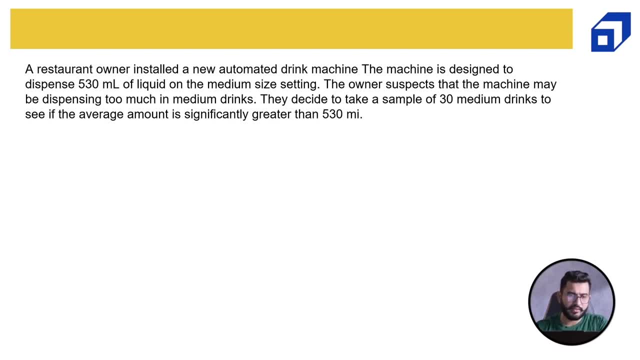 drink machine. The machine is designed to dispense 530 ml of liquid on medium size setting. Now, what is the initial state of this machine? So we know that the machine was designed to dispense 530 ml. This is the initial state of the machine. 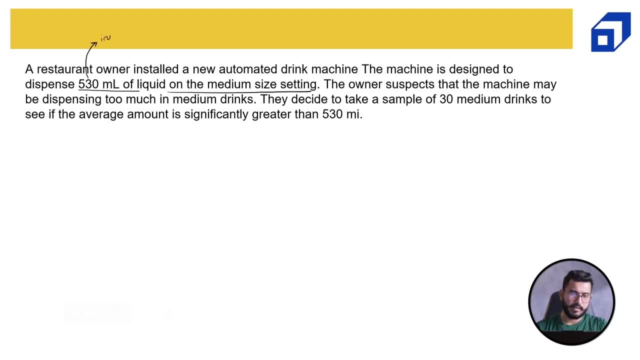 So let me just highlight this. This is the initial state of the machine. The owner suspects that the machine may be dispensing too much in medium drink. They decide to take a sample of 30 medium drink to see if the average amount is significantly. 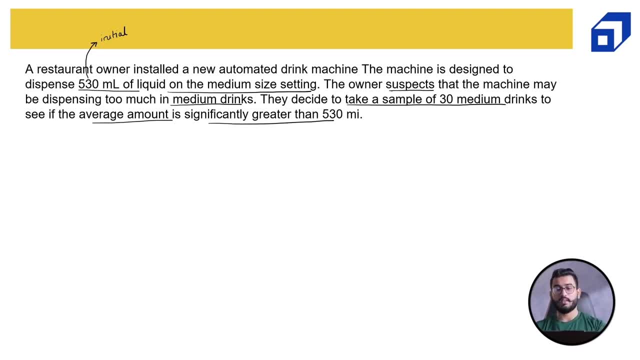 greater than 530 ml. Now what The owner wants to test if the average amount is greater than 530 ml. So this is the new finding, New finding. So my alternate hypothesis is that the average amount is greater than 530 ml. 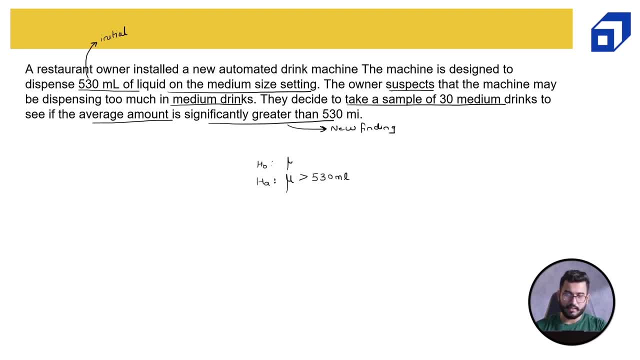 My null hypothesis will be: the average amount is less than or equal to 530 ml. Now why I am using less than or equal to 530 ml. Okay, So I am using less than or equal to 530 ml. Now, please remember, in the question it says the machine is designed to dispense 530 ml. 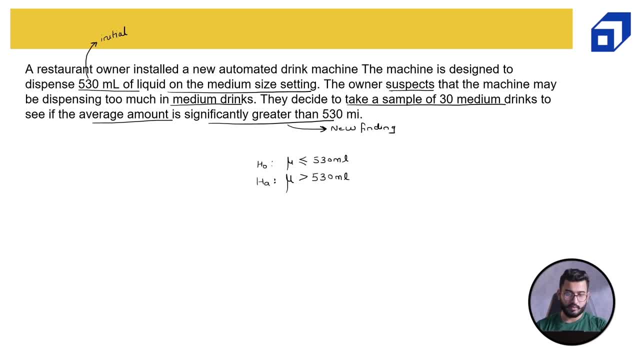 of liquid, So I should have written null, as average is equal to 530 ml. But please remember one thing: I hope you guys remember when we were talking about continuous random variable and the distribution of continuous random variable, we know that the point probability is zero. 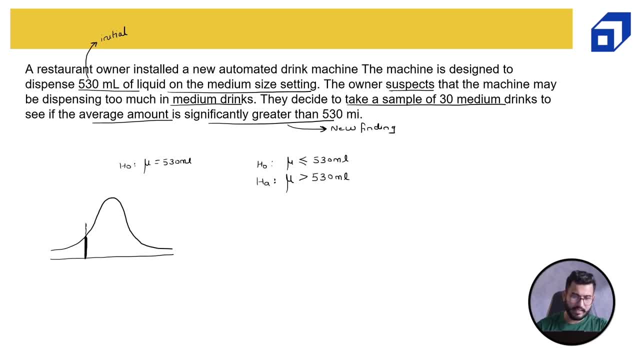 So is equal to 530 ml. let's say this line, this line is 530 ml. Now, greater than 530 ml, is this region Above the line? everything is greater than 530 ml. right, This is greater than Now. if I use alternate as greater than 530 ml and null as is equal to 530 ml, I will. 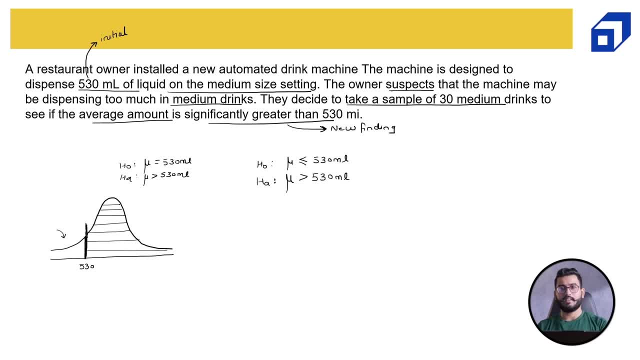 never be considering this region, This region, the lower region, and that would not be helping us to arrive at a conclusion. So, for example, if I'm getting a value which is lying below 530 ml, then in that case, if I do not consider this area, I would not be able to conclude anything. 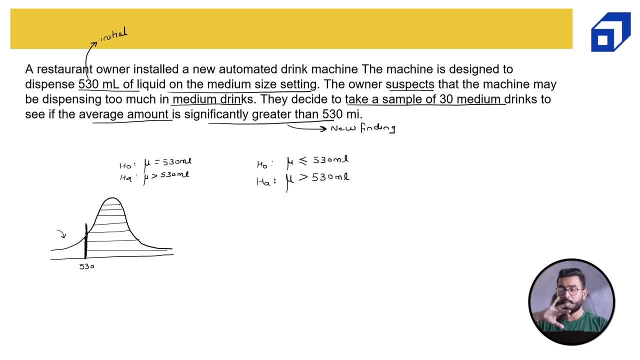 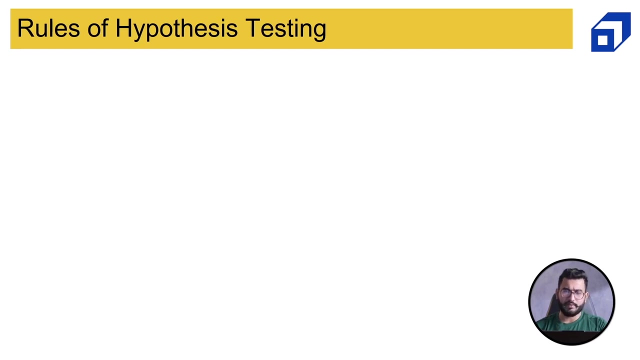 So that is the reason, in order to make sure that I'm covering up the complete distribution, we use less than or equal to, So we get this part also, And then we will be able to cover up the complete area under the curve. There is one rule also, the rule of hypothesis testing- that when we talk about or when we 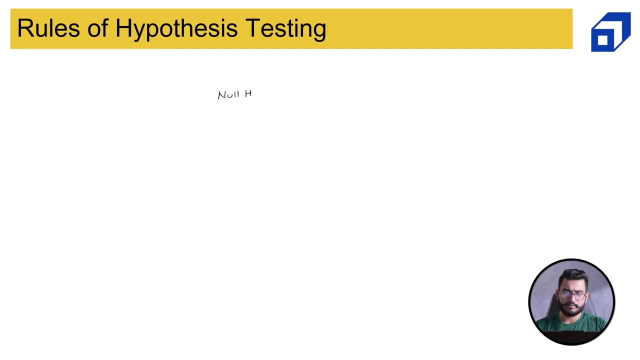 formulate the null hypothesis. the null hypothesis always have. they will always be higher than 530 ml. So we are having less than equal to sign, greater than equal to sign or equal to sign, While alternate will always have less than greater than or not equal to. 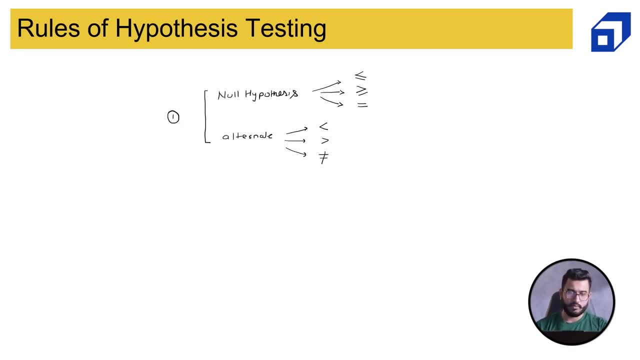 This is rule number one. Rule number two is null and alternate are 100% opposites, Right Opposite to each other. So null and alternate are 100% opposite to each other. which basically means: if, in my hypothesis formulation, if I get my alternate as less than this will be greater than equal. 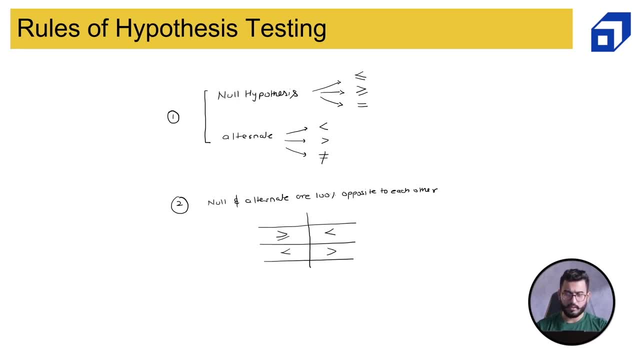 to. If this is greater than, this will be less than or equal to Right. If this is equal to. if this is not equal to, this will be equal to. This is my alternate. this is my null. The third rule is: always start by formulating alternate. always start by formulating alternate. 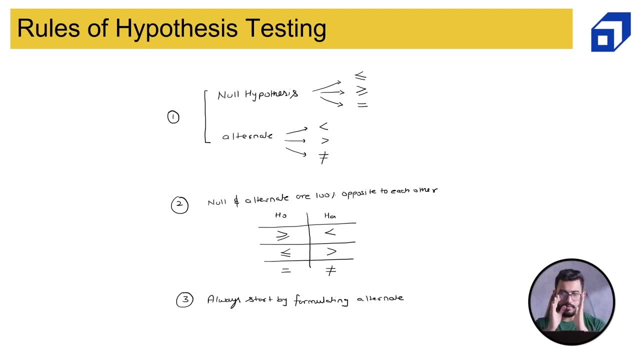 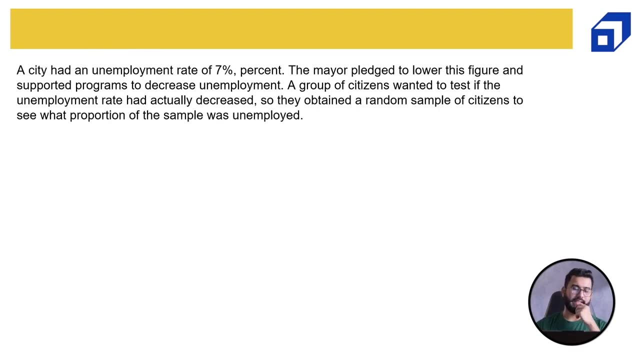 Now, these are the three rules which, so if you remember them, you can formulate the hypothesis for any given problem. Let's try to look into set the second problem. A city had an unemployment rate of 7%. Now, this is my initial estate. 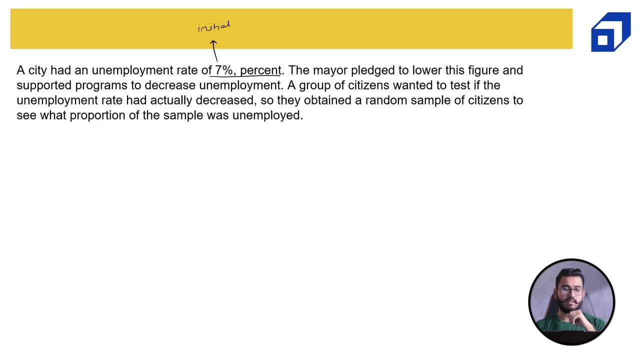 This is something which is initially given to us, that we all know in the in the complete city that unemployment rate is 7%. The mayor placed to lower this figure and supported program to decrease unemployment. The group of cities and want to test it. The unemployment rate is 7%. The Maher blessed to lower this figure and supported program to decrease unemployment. A group of citizens won't to test if the unemployment rate is less than or equal to 0.7.. Point number three: Like Bombay if we look at Indian two suggesting unemployment rate change eight percent of the sentence in Act No 1,. 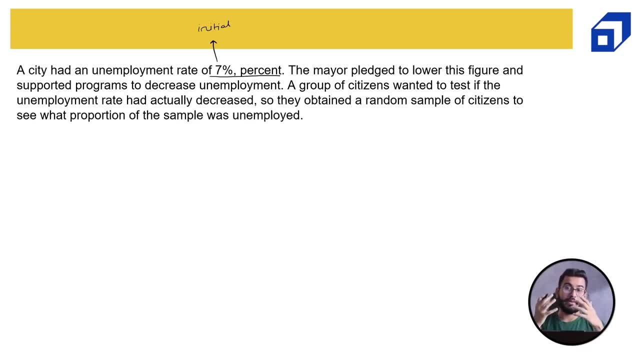 rate has actually decreased. so now what we want to test, or what is my new finding? now, new finding is that the unemployment rate has to be decreased, it has to go down or it has to go below seven percent. so i will start by writing my alternate hypothesis, which is: average, less than seven. 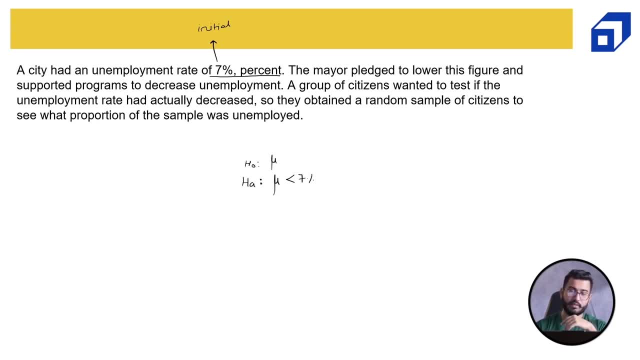 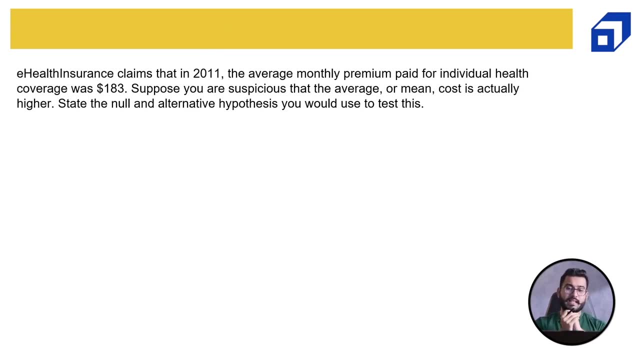 percent. the opposite of this average, greater than or equal to seven percent, would be my null hypothesis. let's take one more example. e-health insurance claimed that in 2011, the average monthly premium paid for individual health coverage was 183 dollar. this is the initial statement made by the company. so this is my initial claim, or initial state. initial. 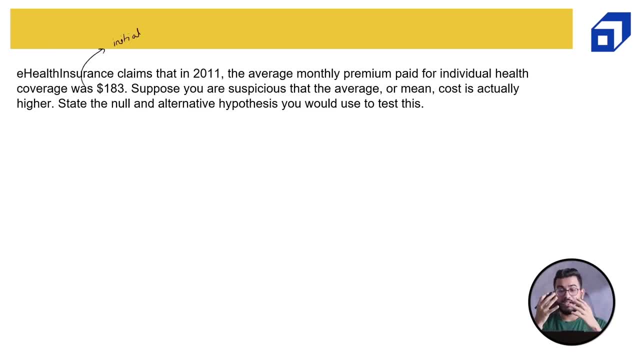 suppose you are suspicious- that the average or mean cost is actually higher. now the new finding, the new thing that you wanted to test, is you wanted to test the average monthly premium paid for individual health coverage was 183 dollar. the average is actually higher than this number. so my alternate: the average is greater than 183. 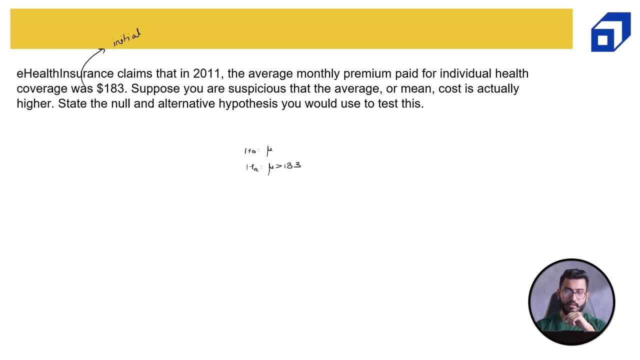 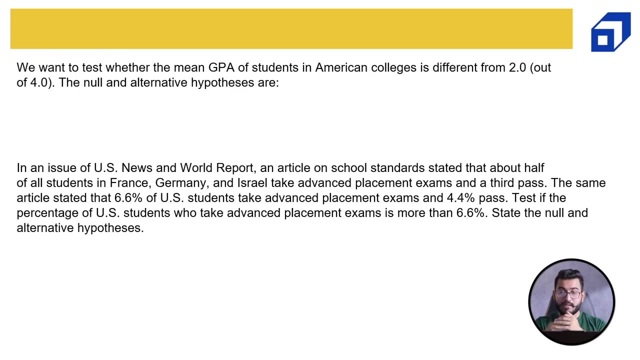 dollars null. the average is less than or equal to 183 dollar, simple. let's take one more example. we want to test whether the mean gp of students in american college is different from 2.0. now, this is what we want to test in this question. we are not given with the initial state. 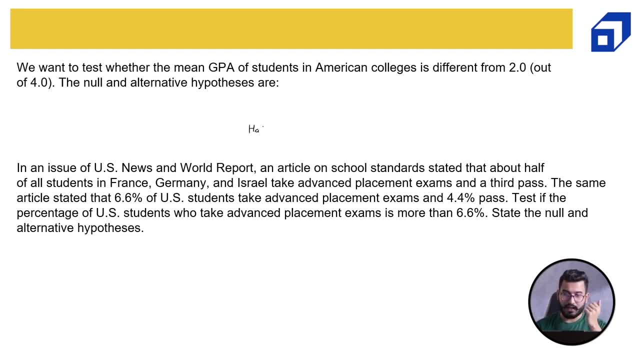 so we know the alternate: that average is not equal to 2.0, null will be the average is equal to 2.0. in an issue of us, in an issue of us news and word report, an article on school standard stated that about half of the students in france, germany and israel take advanced placement exam. 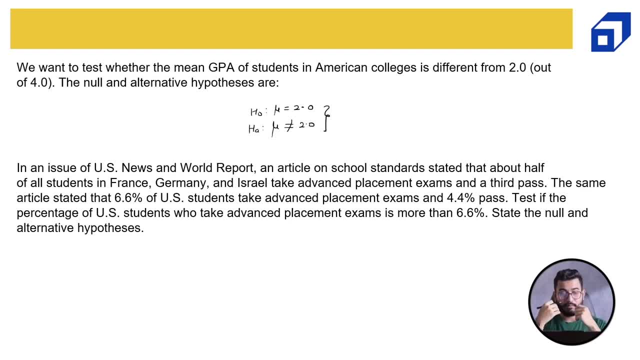 and third pass the same article state that 6.6 percent of us students take advanced placement exam and 4.4 percent of students take advanced placement exam and 4.4 percent of students take 6.6 percent pass test. if the percentage of us student who take advanced placement exam. 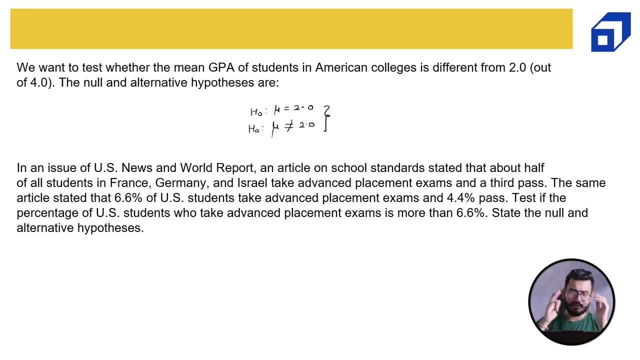 is more than 6.6 percent. so there is a magazine or there is some report which already stated that 6.6 percent of us student take advanced placement exam. you want to test that if this number is more than 6.6 percent. so what you are interested in testing, the alternate will. 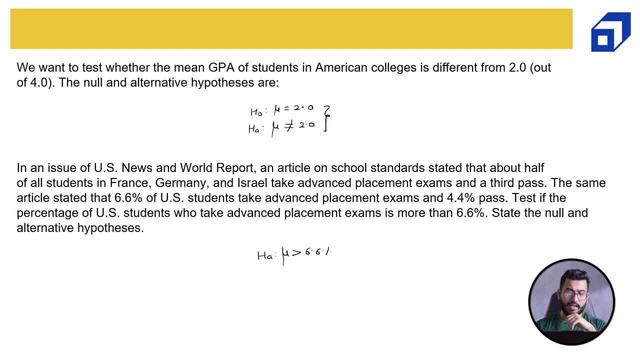 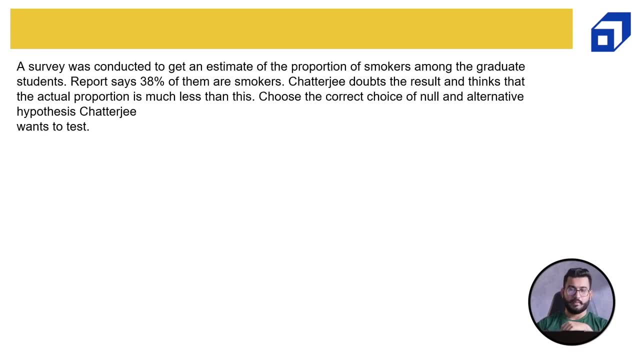 be average is greater than 6.6 percent, while null is average is less than or equal to 6.6 percent. okay, last question. a survey was conducted to get an estimate of proportion of smokers among the graduate student. report says 38 percent of them are smokers. so there is a report which says 38. 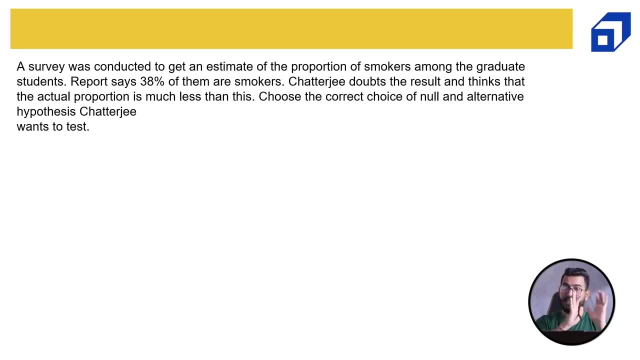 percent of the graduate students are smokers. now this is the initial state. this is already given in the in some report. this is already proven. but now chatalji doubts the risk of smoking over time. Now we have a new finding. This person is suspicious. The person says Chatterjee doubts. 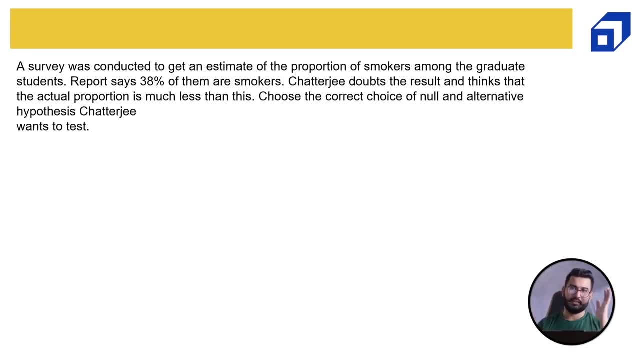 the result: thinks that the actual proportion is less than this. So there is a benchmark: 38%. There is a new finding in the Chatterjee. Chatterjee is thinking that the actual proportion is less than 38%. So what is alternate? That the average is less than 38%, which is what? 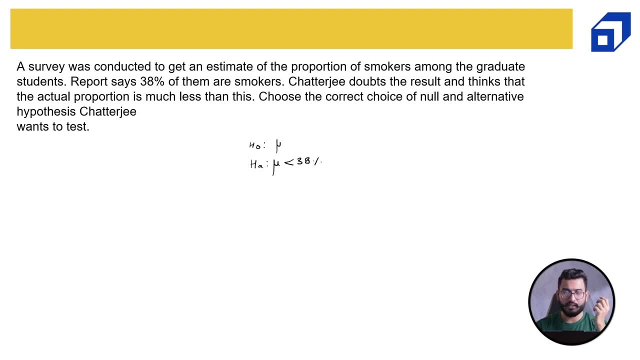 Chatterjee thinks, While the report says it is greater than equal to 38%. This is my null and alternate hypothesis. So I hope now you guys are clear with the first stage of hypothesis testing, which is how to formulate the null and alternate hypothesis given a particular 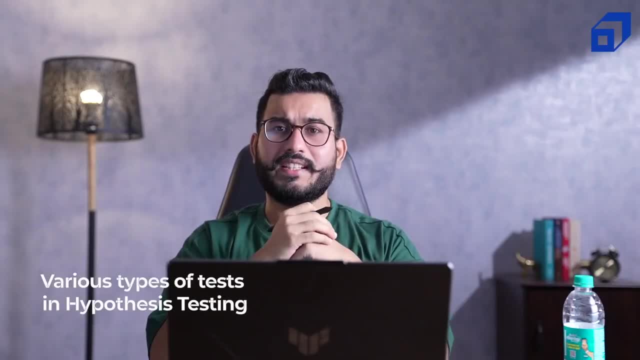 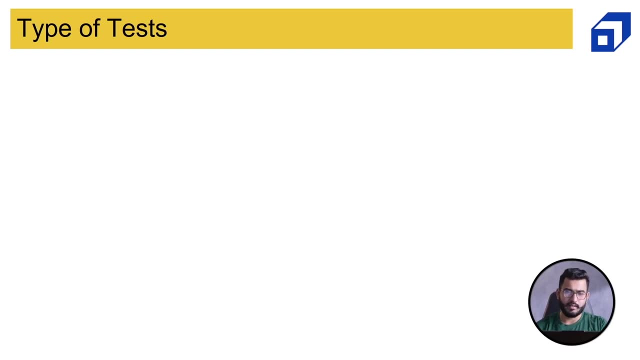 business statement. Now let's try to understand what are the various types of tests we have in the hypothesis testing topic. There are two kinds of tests. Number one is known as the z-test. the second one is known as the t-test. Now, within z-test, we have two. 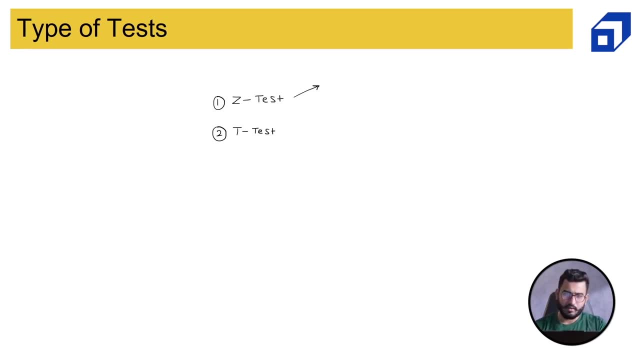 methods. One is known as the confidence interval, confidence interval estimation or confidence interval test, also known as the z-test or the z-value method. Then we have significance test, also known as the p-value method. So within z-test we have z-value method and the p-value method. Within t-test we have three types of tests. 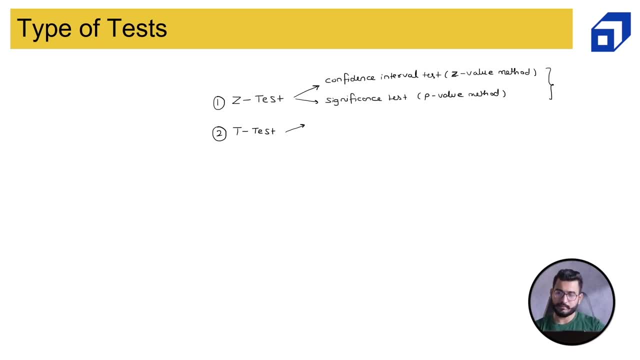 So these are the two methods to perform z-test, But within t-test we have three types of tests based on the problem statement. Number one is one sample t-test, second one is paired sample t-test and the third one is independent sample t-test. 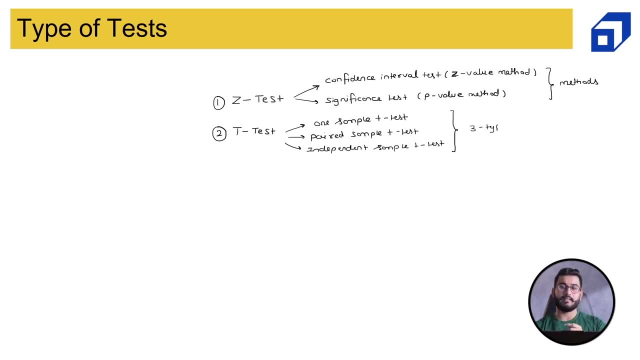 So these are the three types of tests within the t-test. If I have to perform t-test, we have three types of tests based on the business or problem statement. So three types of tests based on the problem statement. Now when to use z-test, when to use t-test. So I will first talk about when to use z-test. 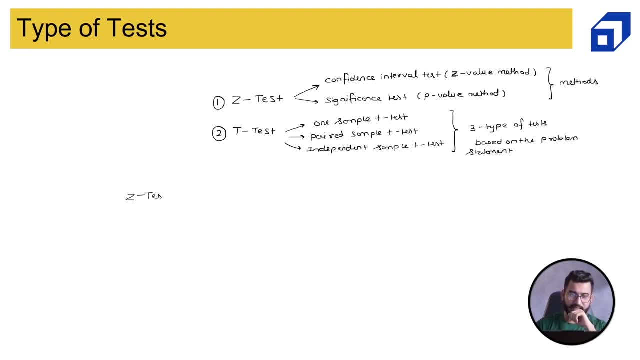 test And when we will be starting the D test. I will talk more about when to use D test. So when to use Z test, you have to check for two things. Number one: the number of observations in your sample. in the sample should be more than 30. And the second condition is the population. 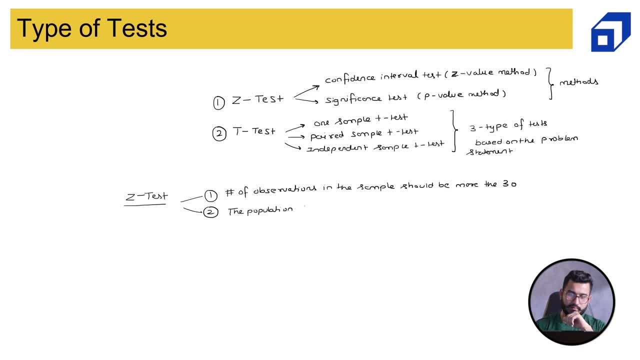 is standard deviation is known Now be FRP. Remember very important interview question, a very common interview question, about what is the difference between Z test and T test. I'm just talking about Z test. as of now, when we start the T test, I will show you the rules of when to use a T test. but 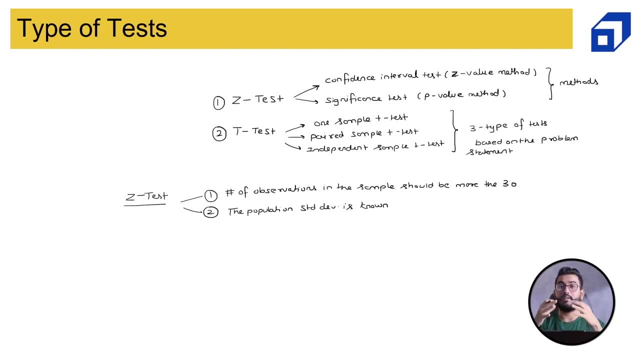 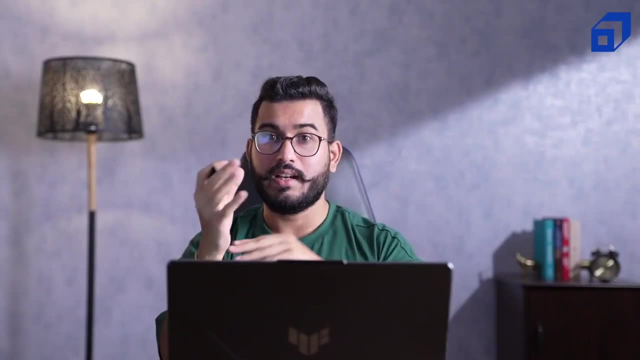 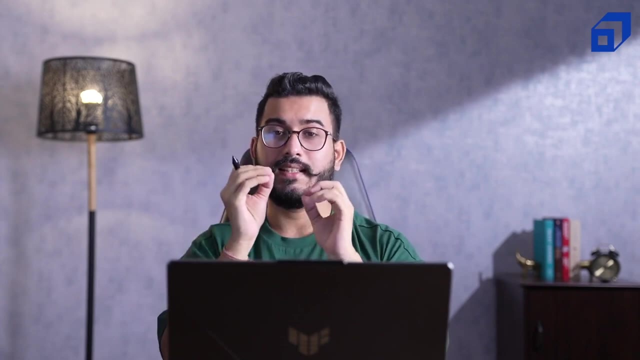 please remember this is a very important topic. this is a very common interview question: the difference between Z test and T test. so if I do not know the population standard deviation and I know the sample standard deviation but my sample size is more than 30, then still Z test is applicable now directly. 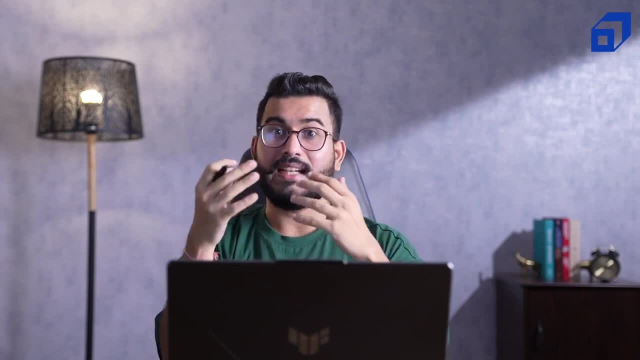 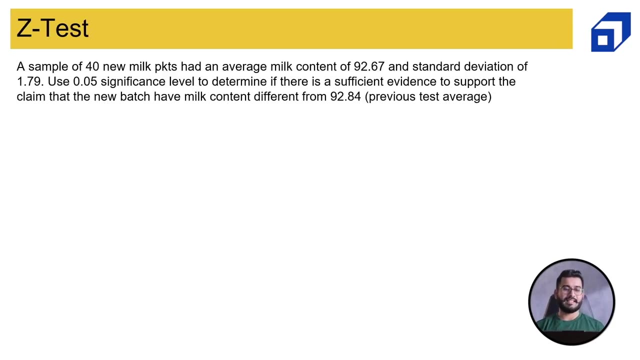 jump to a problem statement. let's formulate the hypothesis, apply the Z test and let's try to conclude in this question. we are given with a sample of 40. new milk packet had an average milk content of 92.67. so within a milk packet you will find out some quantity of milk and some quantity of water. so it has. 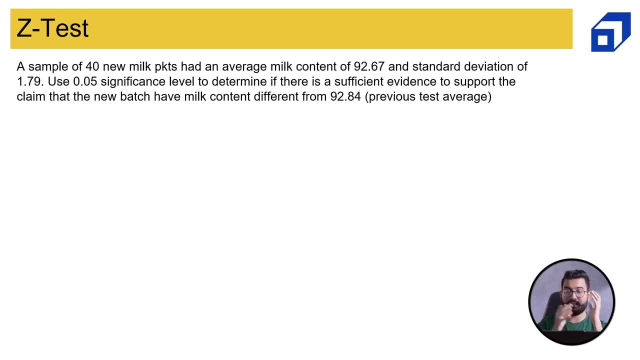 been given that a sample of 40 new milk packet had an average milk content of 92.67 with a standard deviation of 1.79. so this standard deviation is the sample standard deviation. now, since my sample size is more than 40 Z test is: 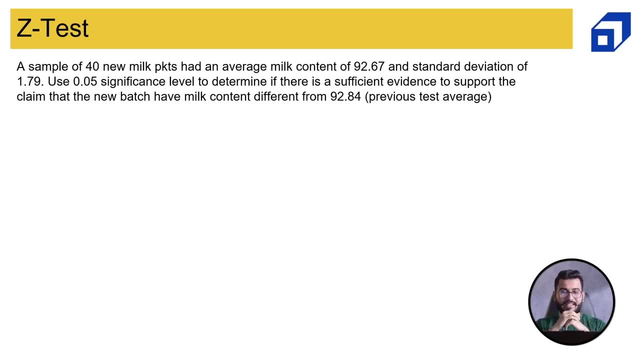 applicable over here. use 0.05 significance Z test is applicable over here. use 0.05 significance Z test is applicable over here. use 0.05 significance level to determine if there is sufficient evidence to support the level. to determine if there is sufficient evidence to support the claim that the new batch have milk. 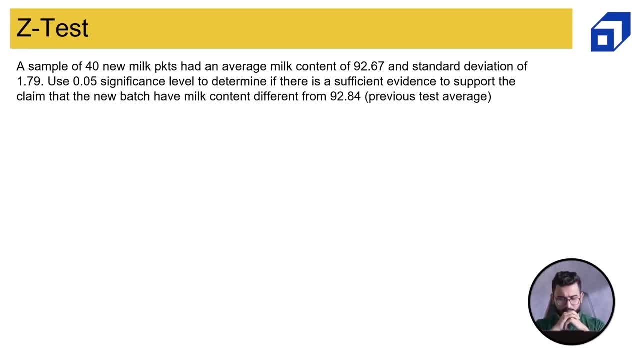 claim that the new batch have milk content different from 92.84. now, as of content different from 92.84. now, as of now, the complete question may be sounding really now. the complete question may be sounding really German to you, don't worry about it. 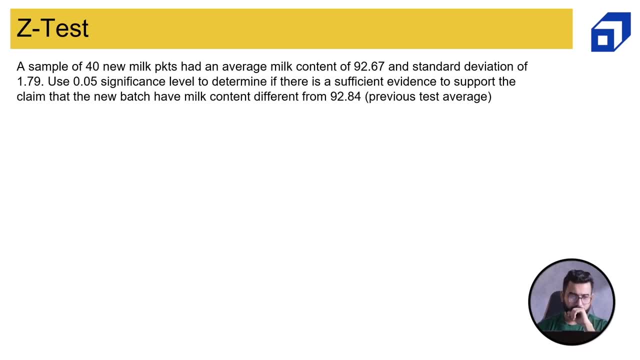 German to you. don't worry about it, let's try to decode this particular problem. so, let's try to decode this particular problem. so assume that you work as a quality test. you work. assume that you work as a quality test. you work as a, let's say, as a scientist in the quality test. 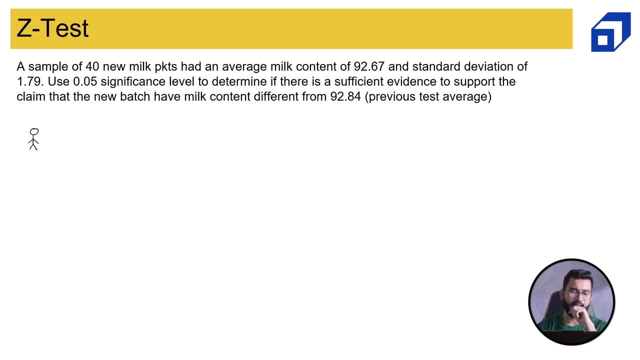 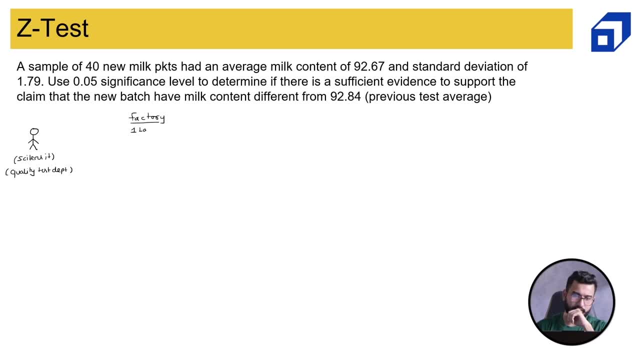 and on the daily basis. let's say, this factory, on the daily basis, is producing 1 lakh milk packet- 1 lakh milk packets. so, on the daily basis, this factory is producing 1 lakh daily packet, now as 1 lakh milk packets. so, on the daily basis, this factory is producing 1 lakh daily packet now as 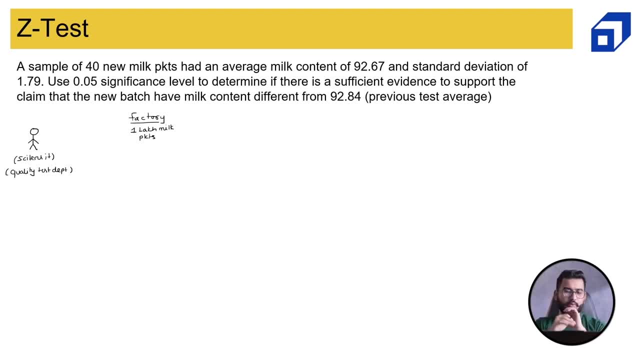 1 lakh milk packets. so, on the daily basis, this factory is producing 1 lakh daily packet. now, as a scientist, it is a scientist, it is a scientist. it is completely impossible for you to test all, completely impossible for you to test all, completely impossible for you to test all the milk packet, right? so what is the? 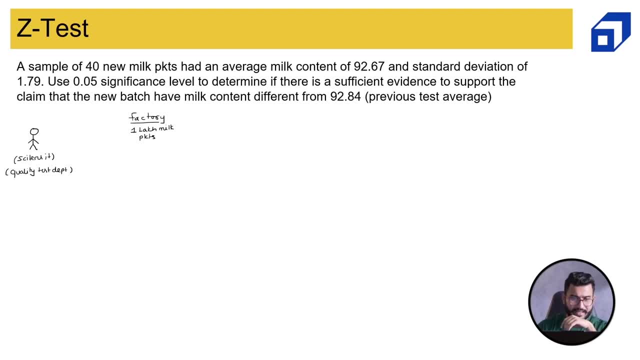 the milk packet right. so what is the? the milk packet right. so what is the correct procedure? we have already learnt correct procedure. we have already learnt correct procedure. we have already learnt about it. we will take a sample out of it about it. we will take a sample out of it. 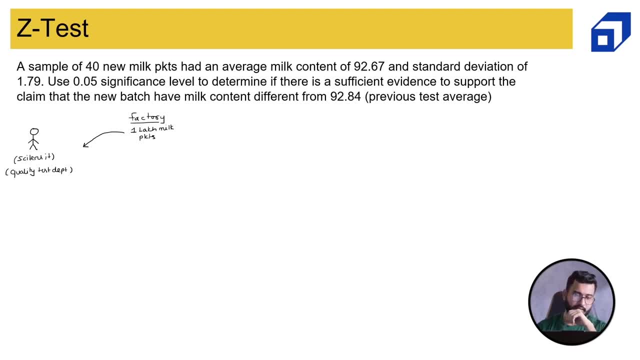 about it. we will take a sample out of it. so let's say, on the daily basis you are. so let's say on the daily basis you are. so let's say, on the daily basis you are taking a sample of 40 milk packet. so taking a sample of 40 milk packet, so 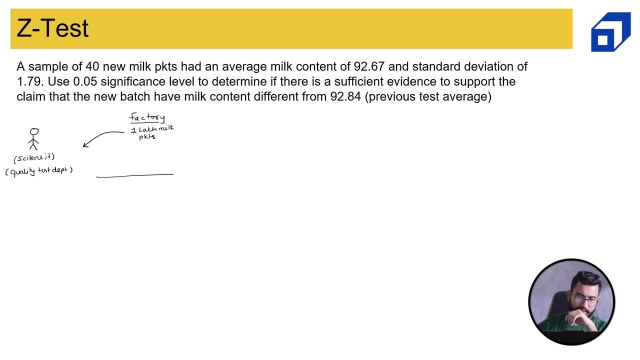 taking a sample of 40 milk packet. so let's say I have just drawn a table on. let's say I have just drawn a table on. let's say I have just drawn a table on my screen, my screen, my screen, let's say this represent the day in the 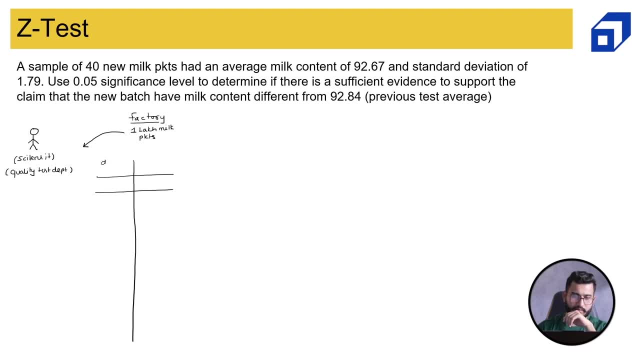 let's say this represent the day in the. let's say this represent the day in the month. so day of the month on this month, so day of the month on this month, so day of the month on. this represents the average milk quantity. so represents the average milk quantity. so 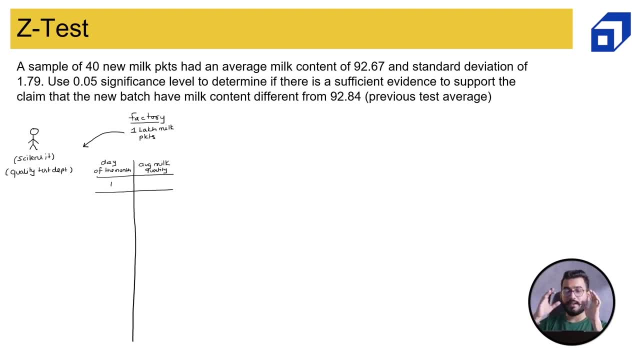 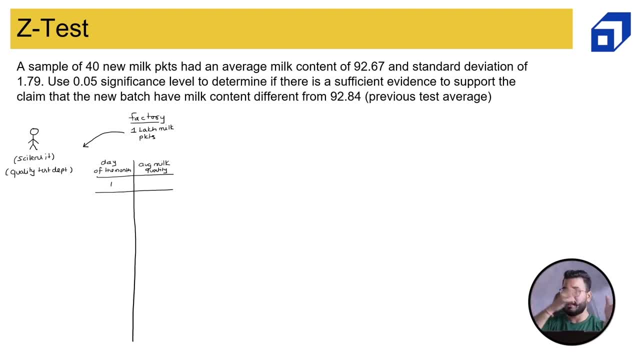 1 lakh milk packets out of the population of 1 lakh milk packet that was produced on packet. that was produced on packet that was produced on that particular day. you sampled out 40. that particular day, you sampled out 40. that particular day, you sampled out 40 random milk packets. after performing the 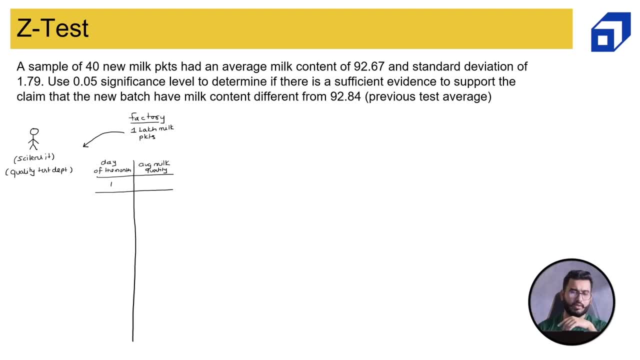 random milk packets. after performing the random milk packets, after performing the test on all those 40 packets, the average test on all those 40 packets, the average test on all those 40 packets- the average milk content came out to be less than milk content came out to be less than. 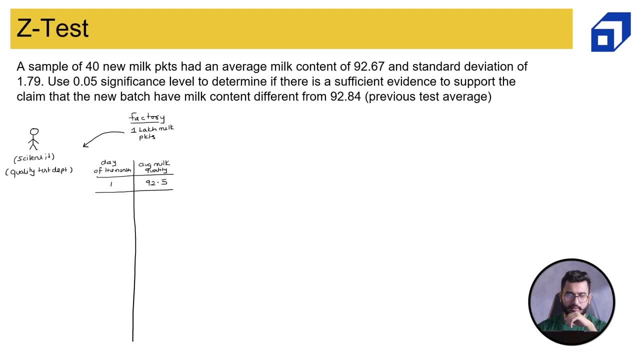 milk content came out to be less than 92.5. then on another day, the average came 92.5. then on another day, the average came 92.5. then on another day, the average came out to be ninety two point seven, on out to be ninety two point seven on. 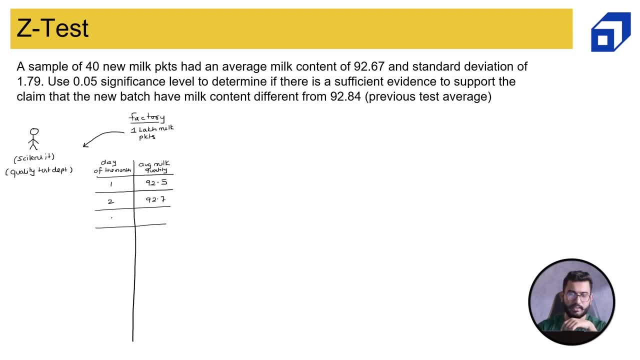 out to be ninety two point seven. on another day, the average came out to be: another day, the average came out to be. another day, the average came out to be, let's say, ninety two point. let's say, let's say ninety two point, let's say, let's say ninety two point, let's say eight. on another day, the average came. 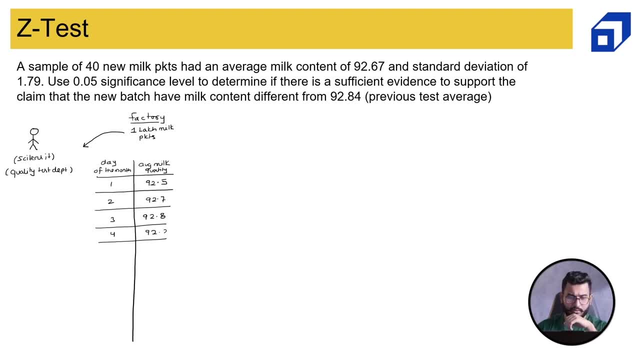 eight. on another day, the average came eight. on another day, the average came out to be, let's say, ninety two point out to be, let's say, ninety two, point out to be: let's say, ninety two point two, seven. and you have been doing this: two, seven and you have been doing this. 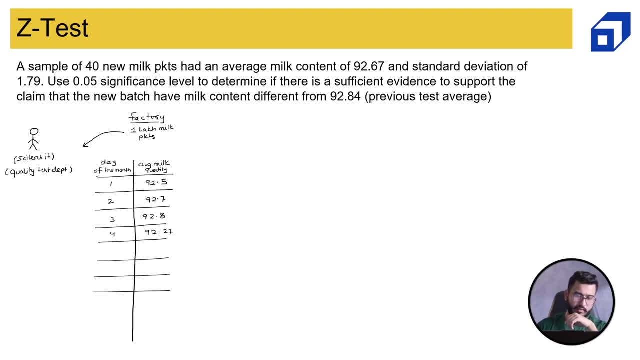 two, seven, and you have been doing this thing. let's say for last one month, so thing. let's say for last one month, so thing. let's say for last one month. so let's say on day 30, so I'll just put. let's say on day 30, so I'll just put. 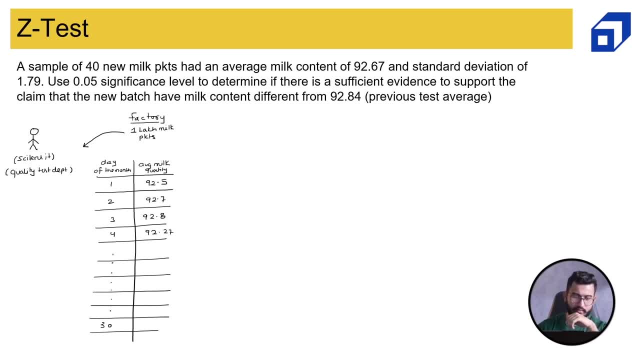 let's say on day 30. so I'll just put dot dot dot in this in this table on day. dot dot dot in this in this table on day. dot dot dot in this table on day thirty. the average came out to be ninety two thirty. the average came out to be ninety two. 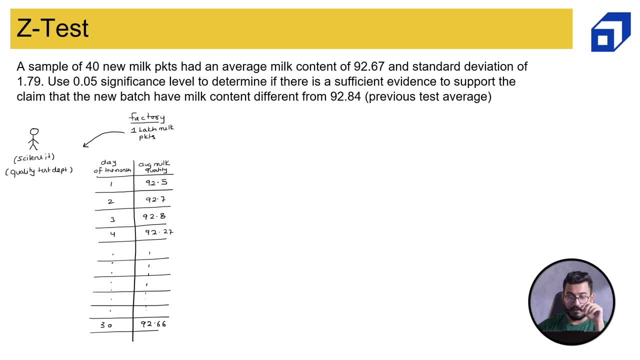 thirty. the average came out to be ninety two point six six. now, when you looked at point six: six. now, when you looked at point six: six. now when you looked at the month average, the complete month, the month average, the complete month, the month average, the complete month average, the monthly average was ninety. 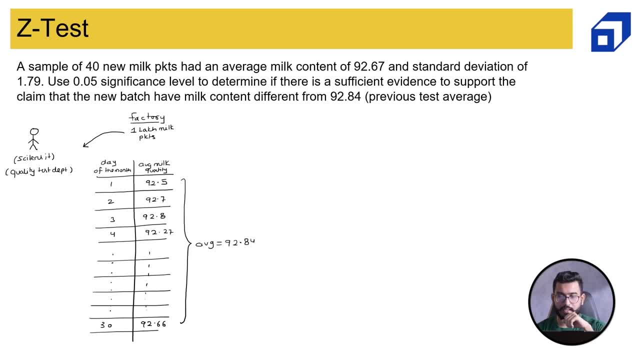 average: the monthly average was ninety. average: the monthly average was ninety. two point eight four now. this is what two point eight four now. this is what two point eight four now. this is what has been given to us, so another day has been given to us, so another day. 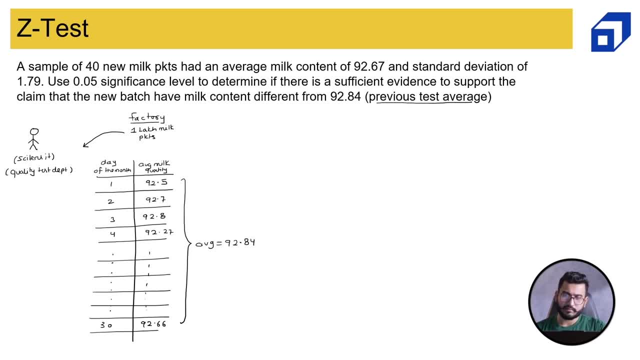 has been given to us. so another day, let's say another month, another day when let's say another month, another day when let's say another month, another day, when you are testing forty new milk. you are testing forty new milk. you are testing forty new milk packet, forty new milk packets. 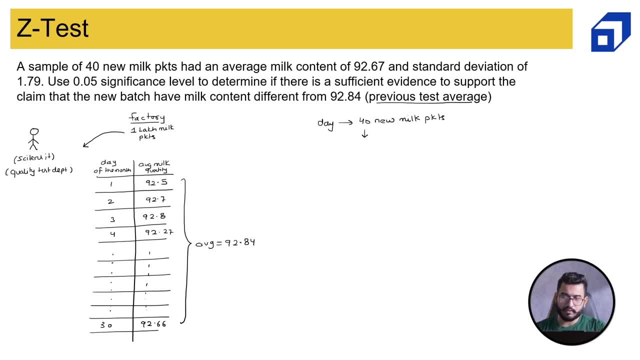 packet forty new milk packets. packet forty new milk packets. your average came out to be ninety two. your average came out to be ninety two. your average came out to be ninety two point six, seven point six, seven point six, seven. so I hope this, this complete picture is. 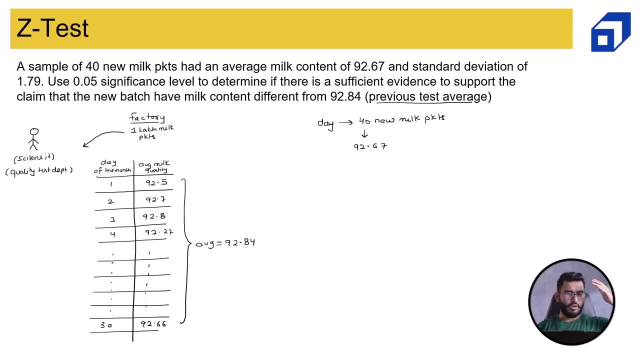 so I hope this, this complete picture is so I hope this, this complete picture, is making sense. you have been doing the making sense. you have been doing the making sense. you have been doing the test for all the days, from day one to day. test for all the days, from day one to day. 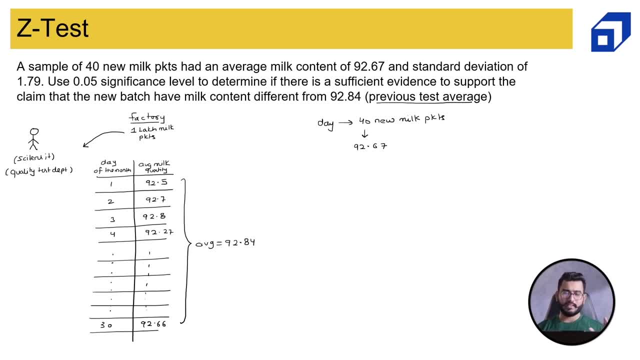 test for all the days from day one to day thirty from last one month and the thirty from last one month and the thirty from last one month, and the average was ninety two point eight four. average was ninety two point eight four. average was ninety two point eight four. and this is, let's say, you can see that. 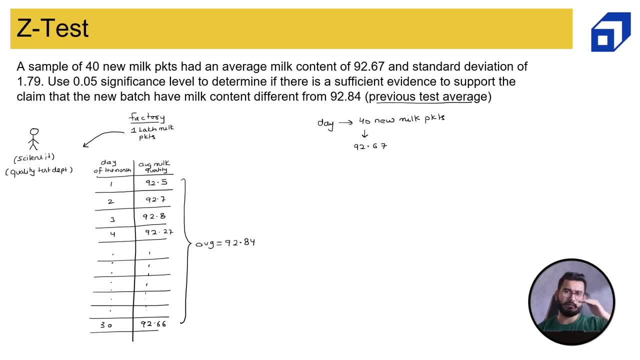 and this is let's say you can see that, and this is let's say you can see that this is above the quality of the quality, this is above the quality of the quality, this is above the quality of the quality cutoff, but on one particular day after. 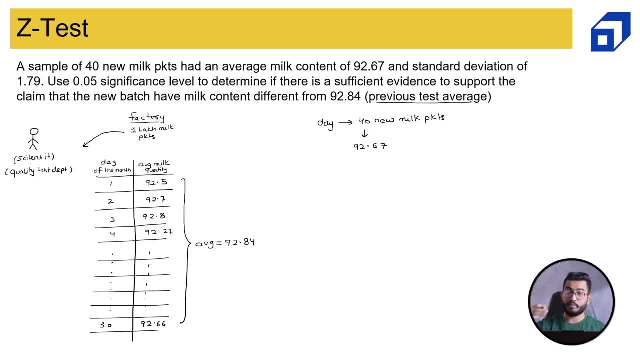 cutoff, but on one particular day after cutoff, but on one particular day after testing this forty new milk packets. the testing this forty new milk packets. the testing this forty new milk packets. the average came out to be ninety two point. average came out to be ninety two point. 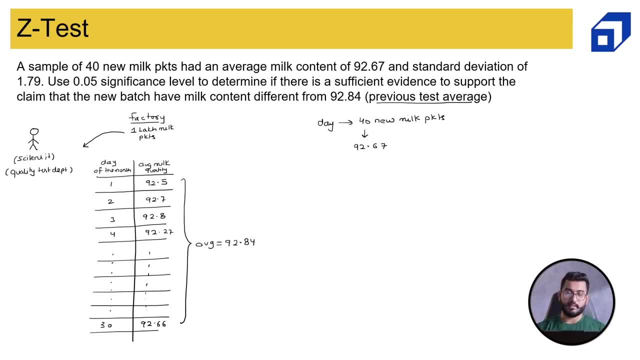 average came out to be ninety two point six seven. now you want to perform the six seven. now you want to perform the six seven. now you want to perform the test to check if this number, the new test to check, if this number, the new test to check, if this number, the new mean, the new sample mean, is in the 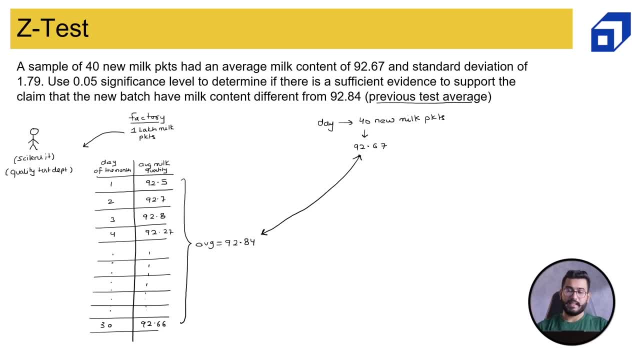 mean. the new sample mean is in the mean. the new sample mean is in the significance range or is? is this number significance range or is? is this number significance range or is? is this number is ninety two point six seven is. is ninety two point six seven is. 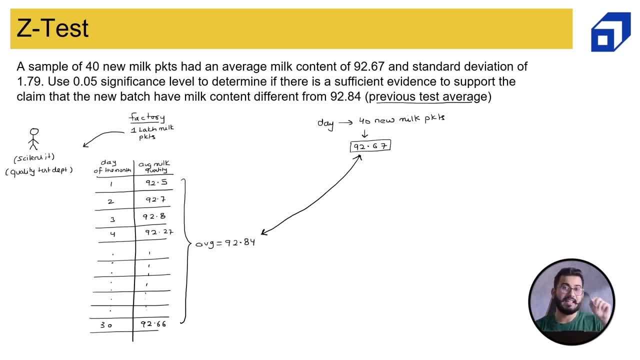 is ninety two point six, seven is statistically significant or statistically significant. or statistically significant or statistically same as ninety two point. statistically same as ninety two point. statistically same as ninety two point. eight, four or not. so what we want to. eight, four or not so what we want to. 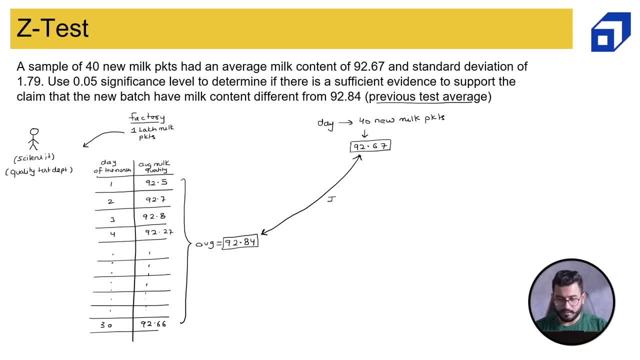 eight four or not. so what we want to test is ninety two point six seven. test is ninety two point six seven. test is ninety two point six seven, statistically same as ninety two point eight four or not, as ninety two point eight four or not, as ninety two point eight four or not. this is what we want to test. so if these 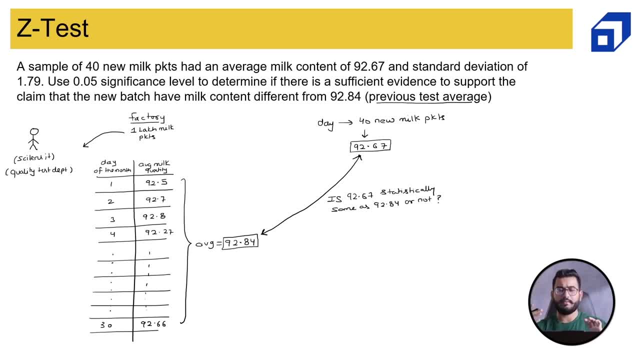 this is what we want to test. so if these- this is what we want to test- so if these two numbers are statistically same, then two numbers are statistically same, then two numbers are statistically same, then we will approve this, this, this batch. we will approve this, this, this batch. 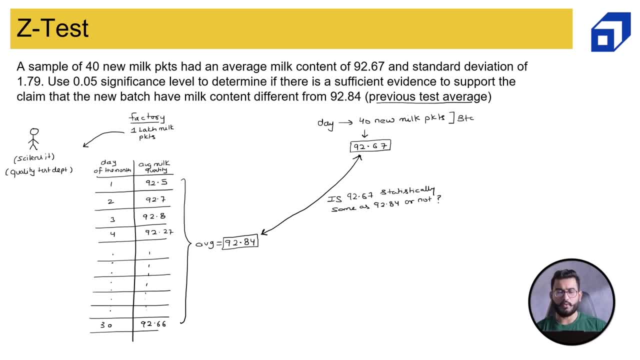 we will approve this, this, this batch, this batch of new 40 milk packets. if this batch of new 40 milk packets, if this batch of new 40 milk packets, if they are different, if they are, they are different. if they are, they are different. if they are statistically different, we will reject the. 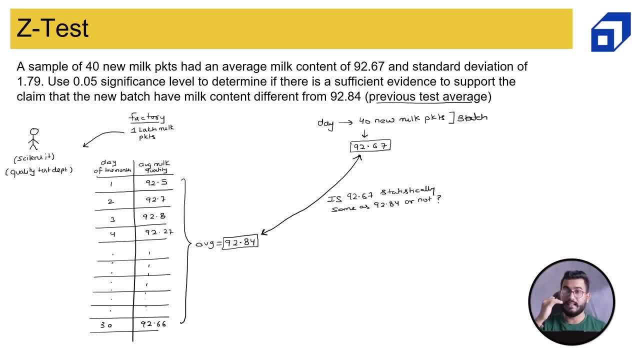 statistically different. we will reject the statistically different. we will reject the complete lot because the milk content is complete. lot because the milk content is complete. lot because the milk content is less than the acceptance. this is what, the less than the acceptance, this is what, the less than the acceptance, this is what the complete scenario is now the number one. 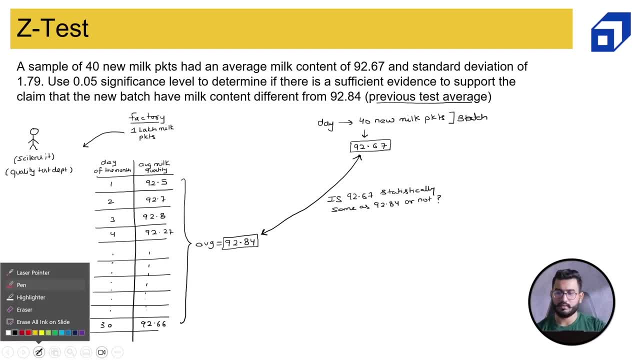 complete scenario is now the number one. complete scenario is now the number one. thing that we will do is to formulate. thing that we will do is to formulate. thing that we will do is to formulate the null and alternate hypothesis, so my. the null and alternate hypothesis, so my. 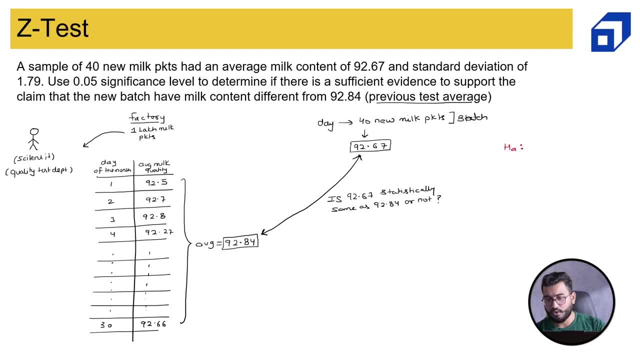 the null and alternate hypothesis. so my alternate hypothesis will be that the alternate hypothesis will be that the alternate hypothesis will be that the average is not equal to ninety. two point average is not equal to ninety. two point average is not equal to ninety two point eight. four why I am using ninety two. 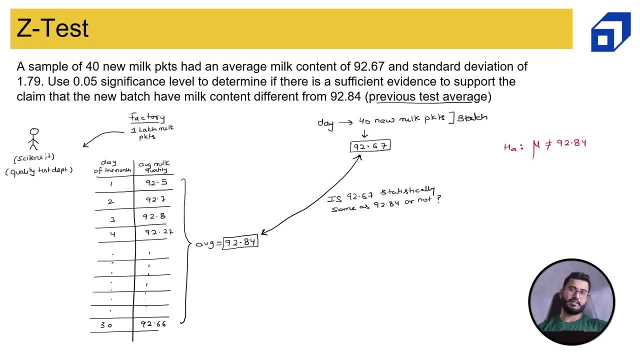 eight four. why I am using ninety two eight four. why I am using ninety two point eight four over here. because that is point eight four over here. because that is point eight four over here. because that is my previous or previous proven value. my previous or previous proven value. 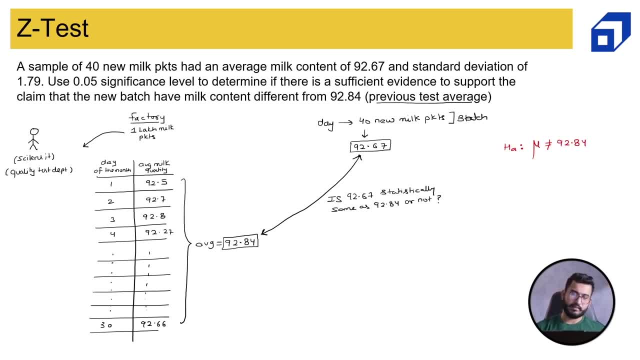 my previous or previous proven value. this is my initial value right initial. this is my initial value right initial. this is my initial value right initial. now alternate or sorry, null will be the now alternate or sorry, null will be. the now alternate or sorry, null will be. the average is equal to ninety two point. 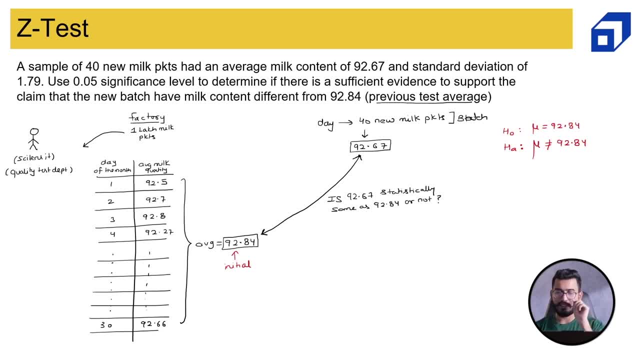 average is equal to ninety. two point average is equal to ninety two point eight four. okay, now, please remember one. eight four. okay, now, please remember one eight four. okay, now, please remember one thing: whenever we have a not equal to thing, whenever we have a not equal to 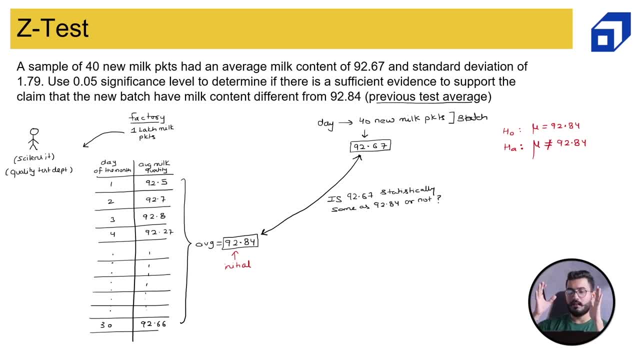 thing: whenever we have a not equal to sign, this basically mean I have to sign this basically mean I have to sign this basically mean I have to perform the test, perform the test, perform the test. oh, oh, oh, oh, oh oh, which will be our two-tailed test. so 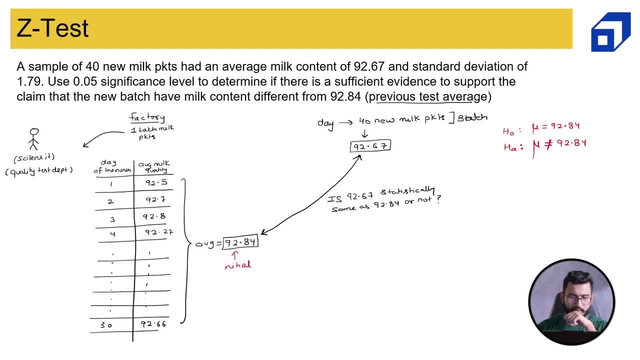 which will be our two-tailed test. so, which will be our two-tailed test? so let's quickly understand this part. if let's quickly understand this part, if let's quickly understand this part, if I'm having not equal to sign in my, I'm having not equal to sign in my. 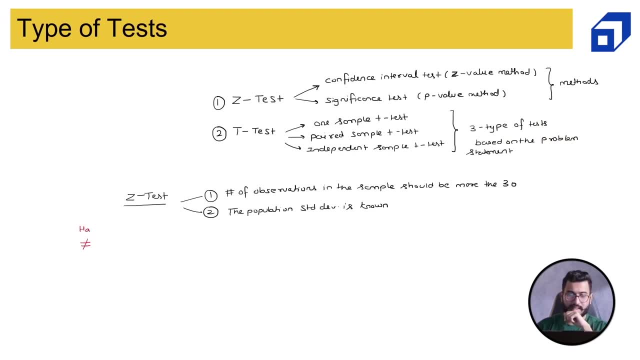 I'm having not equal to sign in my alternate hypothesis, then my rejection. alternate hypothesis, then my rejection. alternate hypothesis, then my rejection. region. so what is rejection? what is region, so what is rejection? what is region so what is rejection? what is acceptance? we will talk about it, don't. 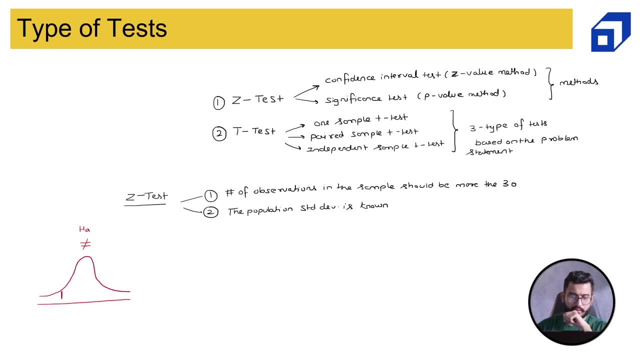 acceptance: we will talk about it. don't acceptance: we will talk about it, don't worry, but my rejection will region will worry, but my rejection will region will worry, but my rejection will region will be on both the side. so this is my: be on both the side. so this is my. 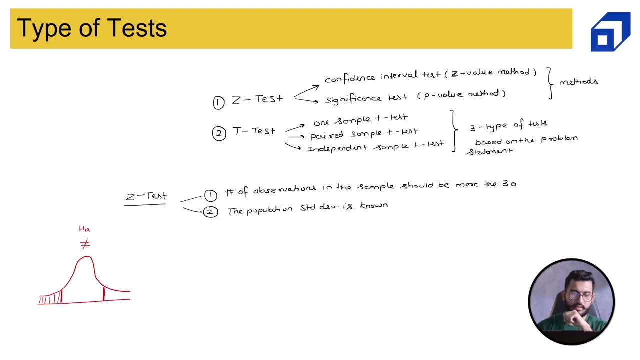 be on both the side. so this is my rejection region. this is my rejection rejection region. this is my rejection rejection region. this is my rejection region if I am having less than sign in region. if I am having less than sign in region, if I am having less than sign in my alternate hypothesis, then my 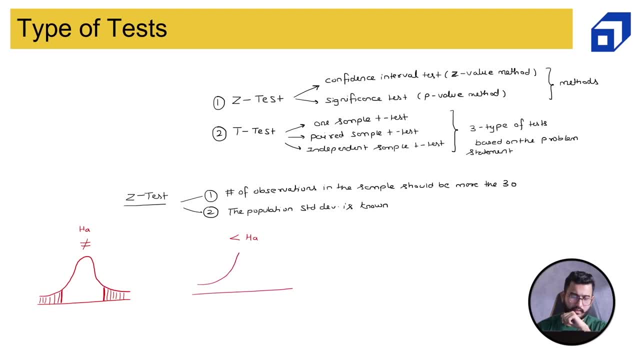 my alternate hypothesis, then my, my alternate hypothesis, then my rejection region will be on left side. rejection region will be on left side. rejection region will be on left side, this side, so just see the arrows. so the this side. so just see the arrows. so the this side. so just see the arrows. so the arrows pointing on the left. so my. 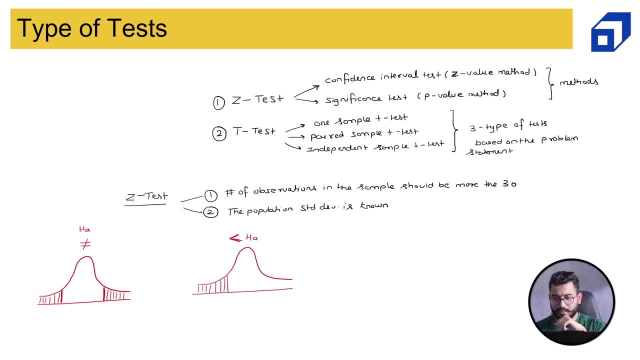 arrows pointing on the left, so my arrows pointing on the left, so my rejection region is on the left. if I'm rejection region is on the left. if I'm rejection region is on the left if I'm having greater than sign in my alternate. having greater than sign in my alternate. 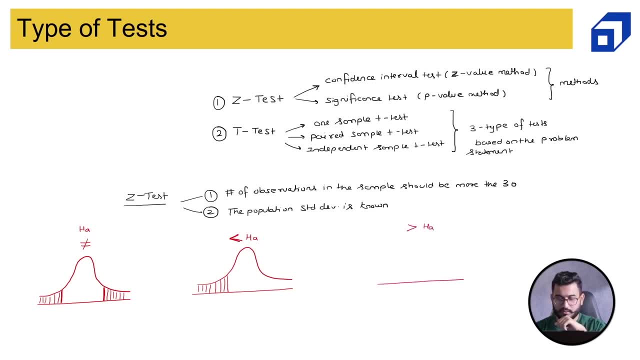 having greater than sign in my alternate hypothesis, then my rejection region will hypothesis, then my rejection region will hypothesis. then my rejection region will be on the right, which is on the this be on the right, which is on the this be on the right, which is on the this side. so just see that arrow. arrow is. 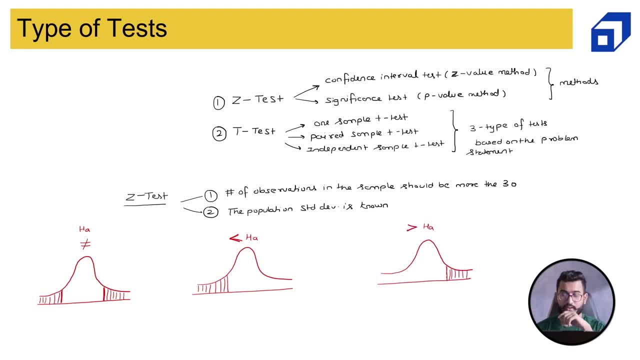 side. so just see that arrow arrow is side. so just see that arrow arrow is pointing towards the right. so my pointing towards the right, so my pointing towards the right. so my rejection region region is on the right. rejection region region is on the right. rejection region region is on the right now, since I am having not equal to sign. 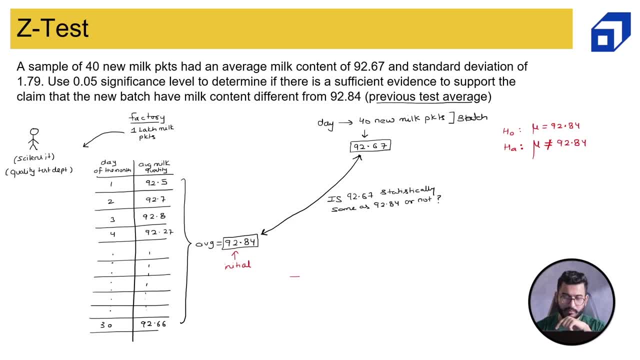 now, since I am having not equal to sign now, since I am having not equal to sign in my alternate my, that this particular in my alternate my, that this particular in my alternate my, that this particular test would be a two tail test. so this test would be a two tail test. so this: 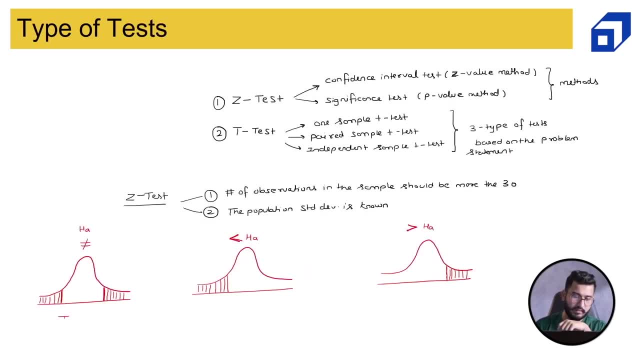 test would be a two tail test, so this is known as a two tail test. this is is known as a two tail test. this is is known as a two tail test. this is known as a left tail. this is known as a known as a left tail. this is known as a. 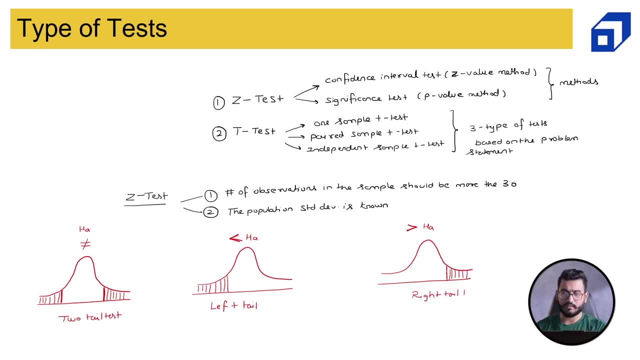 known as a left tail. this is known as a right tail test. so this is my two tail right tail test. so this is my two tail right tail test. so this is my two tail test. so my rejection region is on the test. so my rejection region is on the 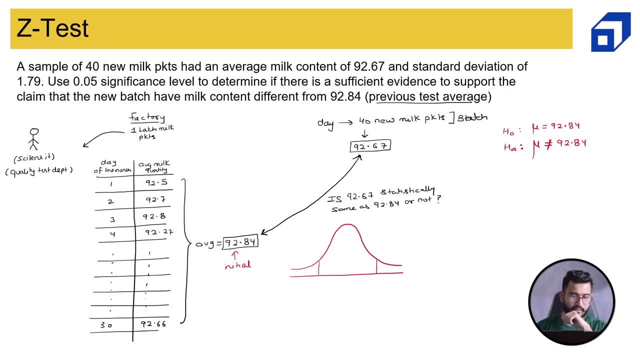 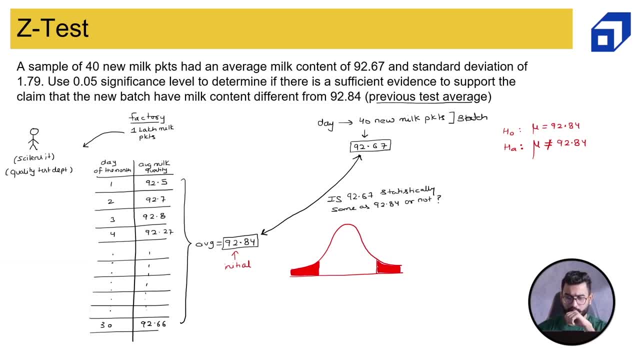 and this is my rejection region now, and this is my rejection region now- what we are going to do. we are going to what we are going to do. we are going to what we are going to do. we are going to find out this particular value lower. find out this particular value lower. 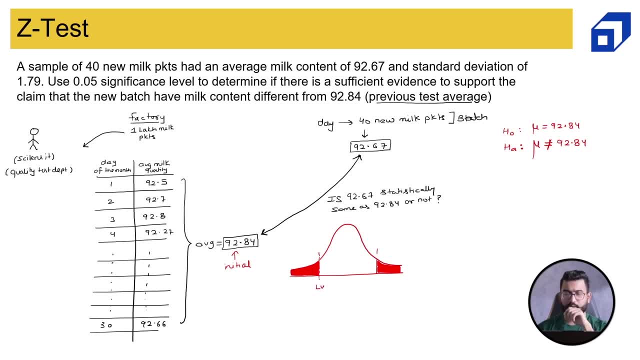 find out this particular value- lower value and the upper value now I hope you value and the upper value now. I hope you value and the upper value now. I hope you guys remember that we have already done guys, remember that we have already done guys, remember that we have already done this using confidence interval. 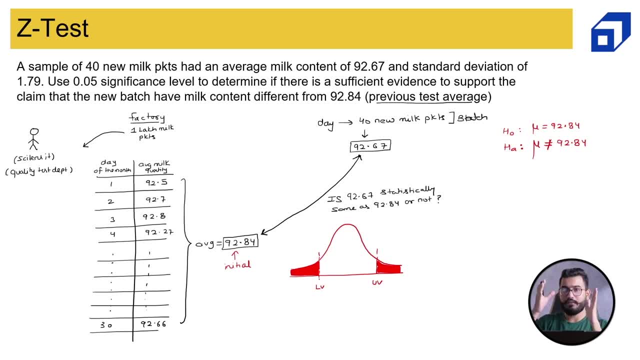 this using confidence interval. this using confidence interval estimation in inferential statistic. we estimation in inferential statistic. we estimation in inferential statistic. we have already found out the limit. the have already found out the limit. the have already found out the limit, the lower limit and the upper limit. right so 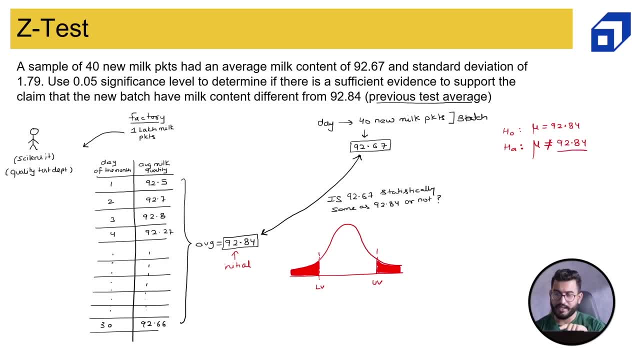 lower limit and the upper limit right. so lower limit and the upper limit right. so we have the average the. so here we call we have the average the. so here we call we have the average the. so here we call this as a population average. so we have. 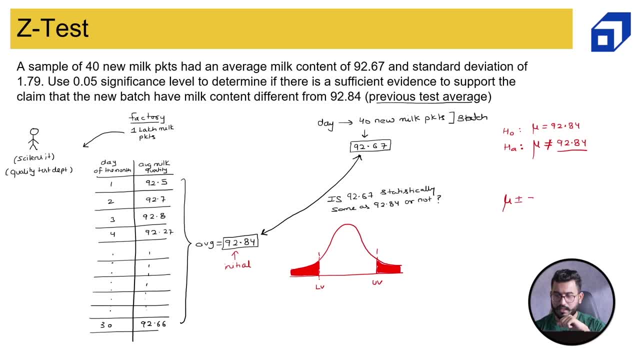 this as a population average. so we have this as a population average. so we have the average plus minus Z times of Sigma. the average plus minus Z times of Sigma. the average plus minus Z times of Sigma. divided by root of n- now what is going. divided by root of n- now what is going? 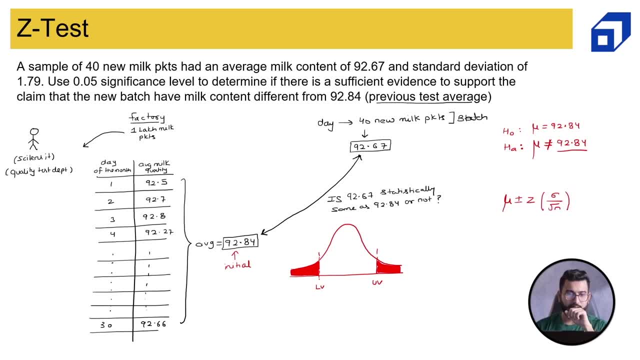 divided by root of n. now, what is going to be my Z value now? for that we have to to be my Z value now, for that we have to to be my Z value. now for that we have to use this significance level, significance. use this significance level, significance. 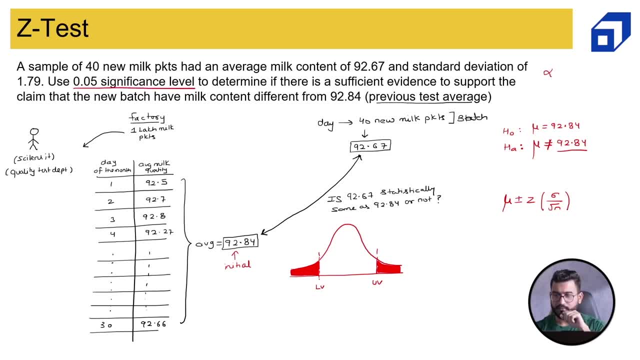 use this significance level. significance level, also known as alpha level, also known as alpha level, also known as alpha, is basically my area of rejection, which is 0.05. so out of the rejection, which is 0.05, so out of the rejection, which is 0.05, so out of the complete area, which is 1. 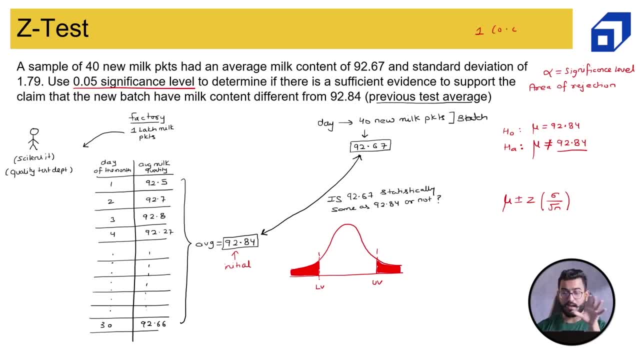 complete area, which is 1. complete area which is 1. 0.05 is the area of rejection now, since 0.05 is the area of rejection now, since 0.05 is the area of rejection now, since I'm having area of rejection or. 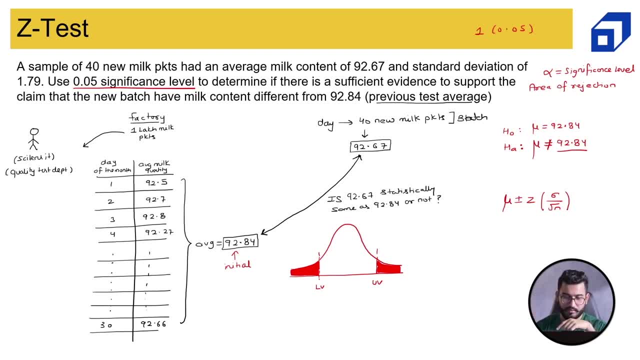 I'm having area of rejection or I'm having area of rejection or rejection region. these are my rejection rejection region. these are my rejection rejection region. these are my rejection regions, regions, regions, rejection region, rejection region, rejection region. this is also my. this is also my. this is also my rejection region. 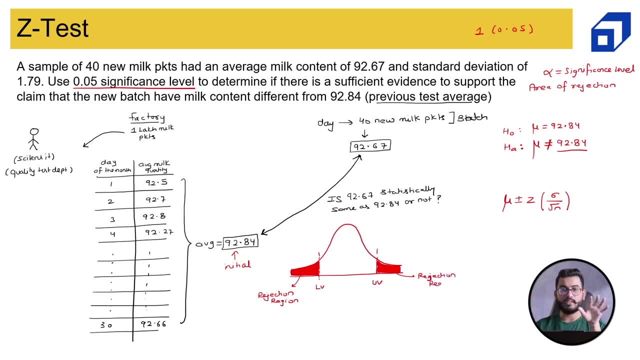 rejection region. rejection region since my, since my rejection region is on both the end. rejection region is on both the end, rejection region is on both the end. I have to divide this significance or area. I have to divide this significance or area. I have to divide this significance or area of rejection by 2, so 0.05. 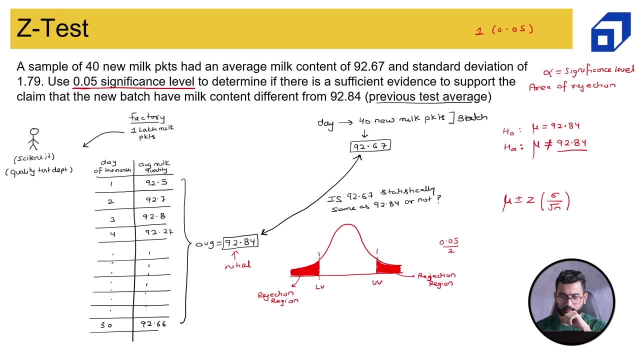 of rejection by 2, so 0.05 of rejection by 2, so 0.05 divided by 2 will be 0.025. so from here, divided by 2 will be 0.025. so from here, divided by 2 will be 0.025. so from here to here, the area is 0.025. 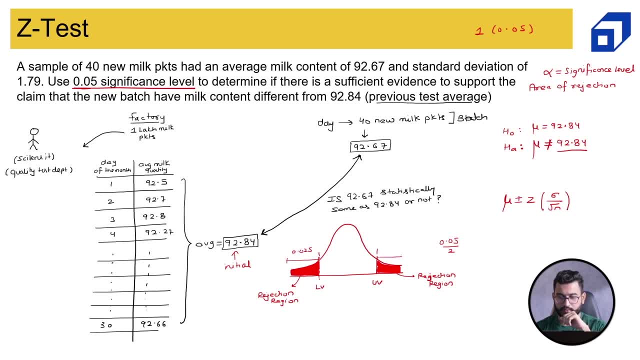 to here, the area is 0.025 to here, the area is 0.025. from here to here, the area is 0.025. from here to here, the area is 0.025. from here to here, the area is 0.025. now, what is the Z value over here? what is? 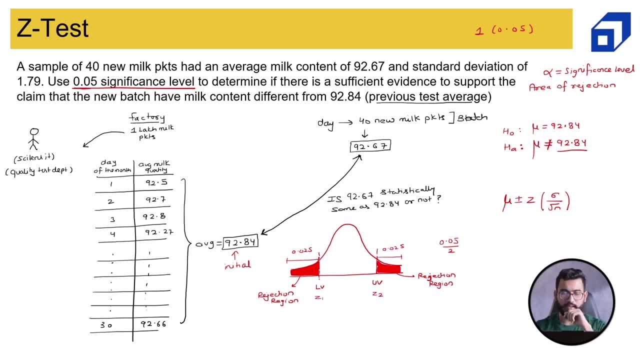 now? what is the Z value over here? what is now? what is the Z value over here? what is the Z value over here? we already know the Z value over here. we already know the Z value over here. we already know this. but let's quickly find out the Z. 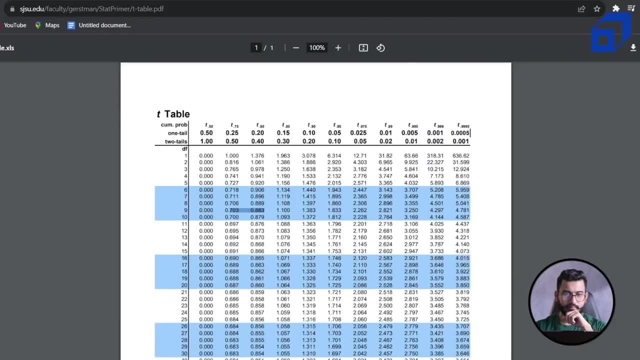 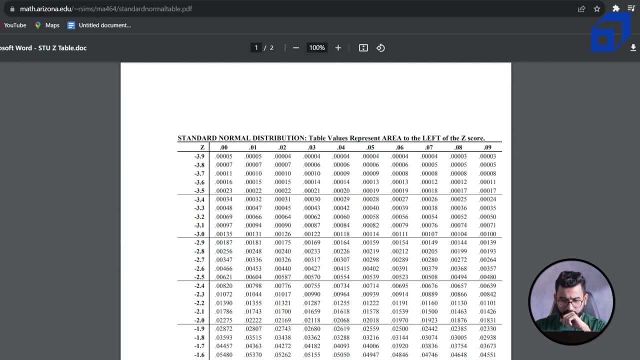 this, but let's quickly find out the Z- this, but let's quickly find out the Z: value at 0.025, so 0.025 over here, and value at 0.025, so 0.025 over here, and value at 0.025, so 0.025 over here, and the value is minus 1.9 and 6. similarly. 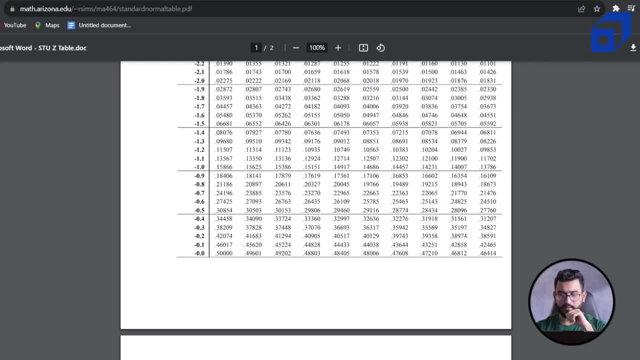 the value is minus 1.9 and 6. similarly, the value is minus 1.9 and 6. similarly, for the positive side it will be plus. for the positive side it will be plus. for the positive side, it will be plus 1.96. so this is minus 1.96, plus 1.96. 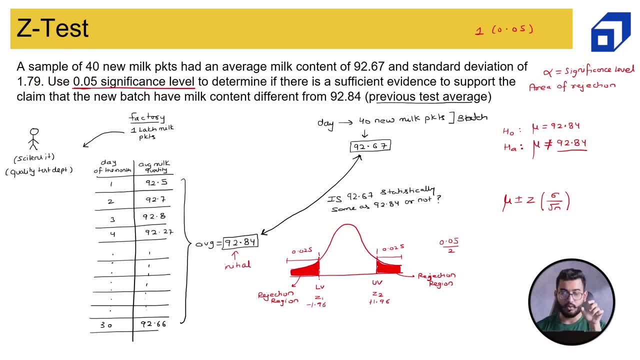 1.96, so this is minus 1.96 plus 1.96. 1.96 so this is minus 1.96 plus 1.96. now, using this, we will find out the. now using this, we will find out the. now using this, we will find out the lower value and upper value. so 92 point. 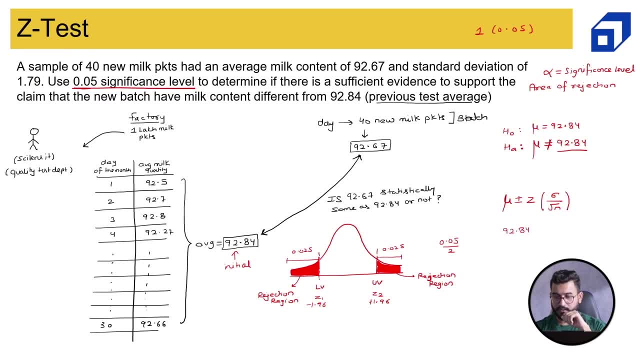 lower value and upper value, so 92 point. lower value and upper value, so 92 point. eight four plus minus 1.96 Sigma, which eight four plus minus 1.96 Sigma, which eight four plus minus 1.96 Sigma, which is standard division, is one point nine. 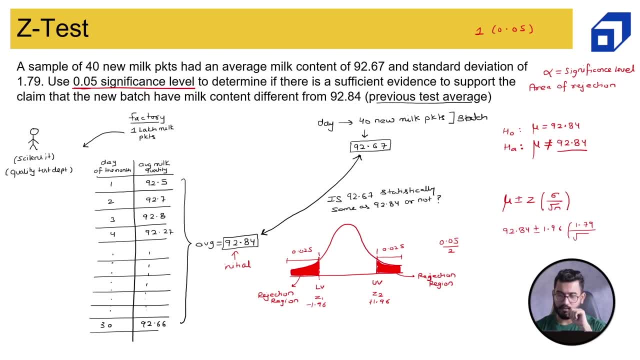 is standard division is one point. nine is standard division is one point nine. seven, nine divided by root of 40, so we seven, nine divided by root of 40, so we seven, nine divided by root of 40, so we will get ninety two point two, eight, six. 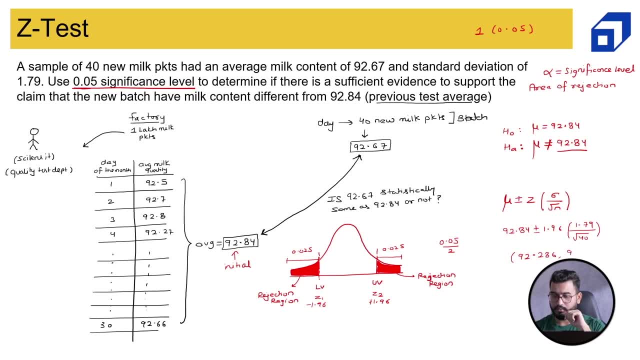 will get ninety two, point two, eight six will get ninety two, point two, eight six comma. ninety three, point three, nine four comma. ninety three, point three, nine four, comma. ninety three, point three, nine four, so here, so here. Here we will have 92.286,, here we will have 93.394. 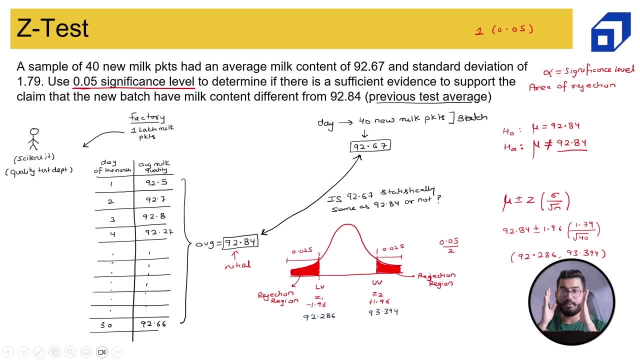 Now, this is the range which has been given to us or which we have derived using the population mean. So now, if my sample mean, this is my sample mean. If my sample mean lies between, or maybe in, the acceptance range, this is my acceptance. 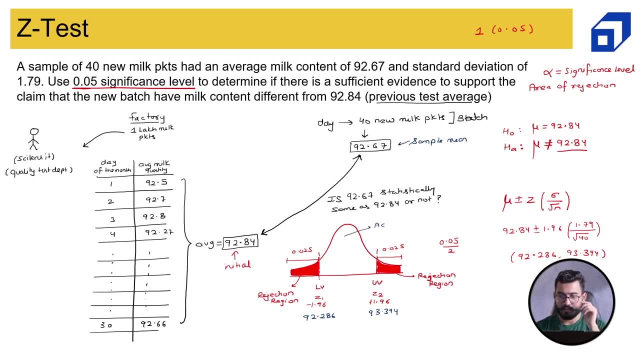 range. So if my sample mean lies in the acceptance range, we say that we fail to reject null. So 92.67 will lie somewhere between this over here, since it is lying in the acceptance range. So if sample mean lies between lies in acceptance range, we conclude that we fail to reject null. Otherwise, if it is, 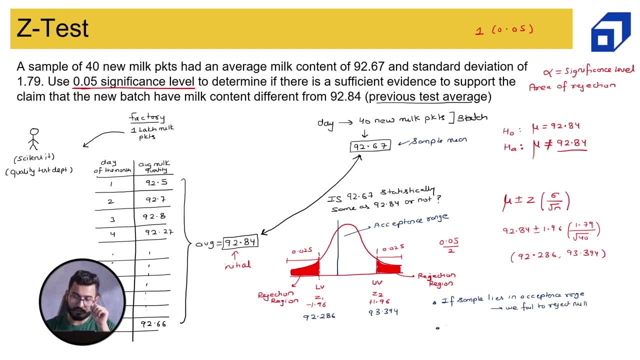 in the rejection region. if sample mean- so I forgot to write- mean false or lies in the rejection region, we reject null. We reject null. So, as of now, what conclusion we will derive? The conclusion will be: we fail to reject null. Why? Because the sample mean. 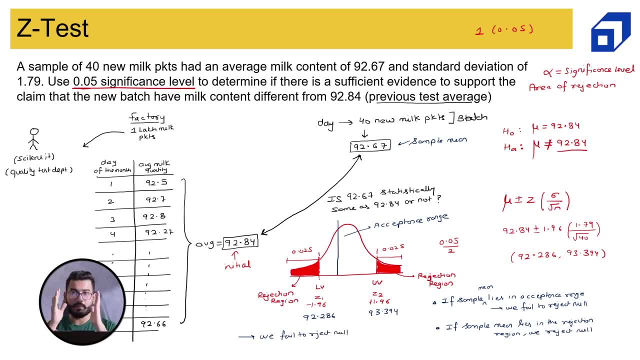 is within the acceptance region or within the boundary which we have derived using the population mean. This is also known as the hypothesis. The reason hypothesized mean is because we hypothetically call it as a population mean, but it is not the true population mean. So if you're getting confused, just be very clear. 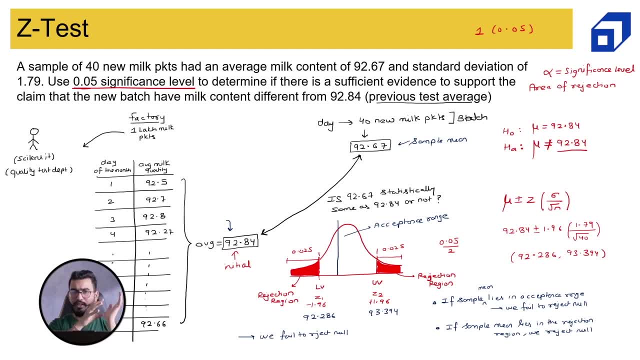 This is a sample mean. 92.67, 92.84 is my population mean And using the population mean we have derived a range. If my sample mean fall within this range, we fail to reject null. If it is outside the range, we reject null. I hope this question makes sense. 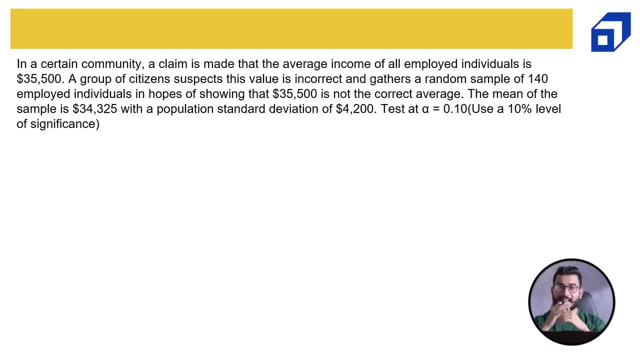 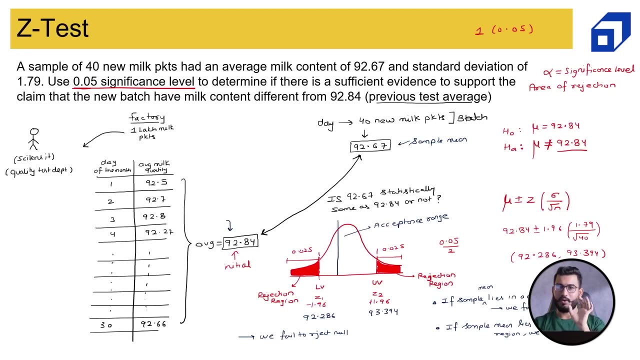 If it is not, let's take one more example. Now let's try to solve this particular problem, And I would advise all of you to pause this video and try to solve this problem by yourself, Because we have already seen one example. You have to just follow the steps and try. 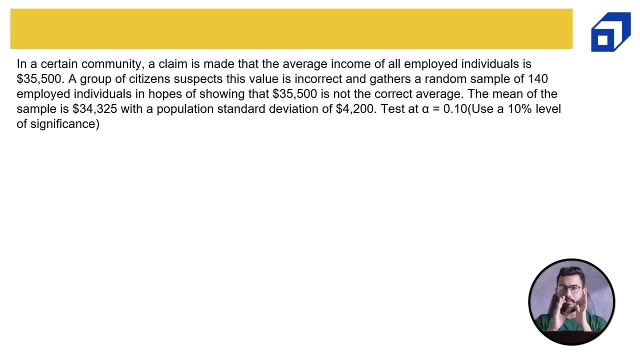 to solve this problem And try to pause the video and just try to solve it by yourself. I assume that you guys would have solved it by yourself. If not, let's try to solve it together. Let's try to solve it. The question says: in a certain community, a claim is made. 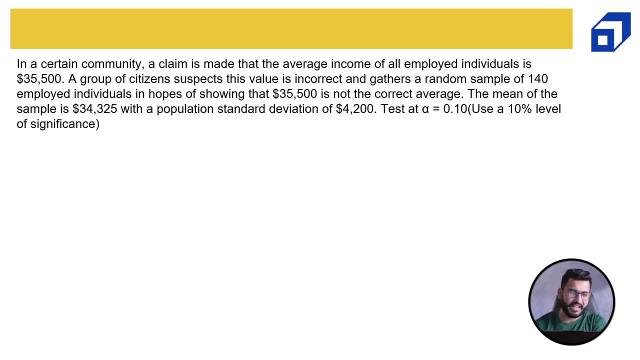 that the average income of employed individual is $3,500.. Now again, there is some initial statement which has already been proven, that the average income is $3,500.. So this is my initial statement. Initial statement: A group of citizens suspect. that a value of $3,500 is $3,500.. A group of citizens suspect that a value of $3,500. A group of citizens suspect that a value of $3,500 is $3,500.. A group of citizens suspect. 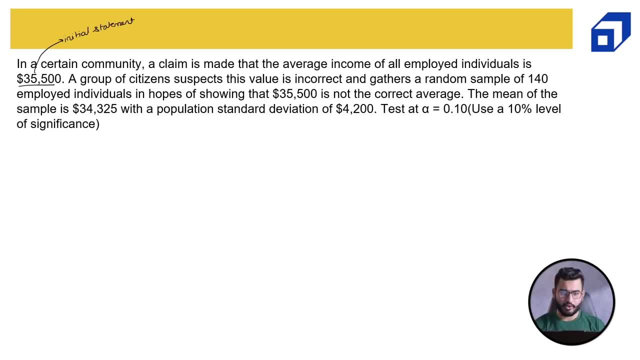 that a value of $3,500 is $3,500.. A group of citizens suspect that a value of $3,500 is $3,500 and gather a random sample of 140 employed individuals in a hope of showing 35,500 is not the correct average. The mean came out to be 34,325.. So what the 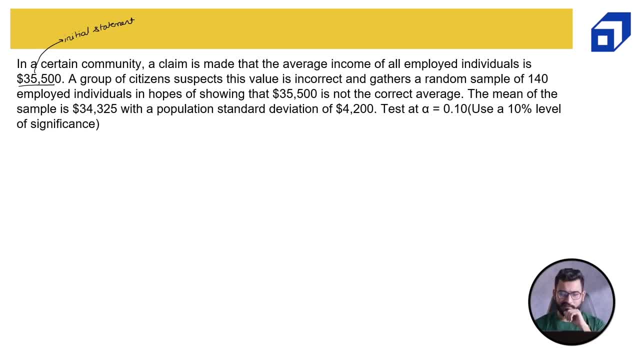 group of citizens did. they collected a sample of 140 people and they obtained the sample mean to be 34,325 with the population standard deviation, The population standard deviation standard deviation. so this is not sample standard deviation. so here we have been given with the 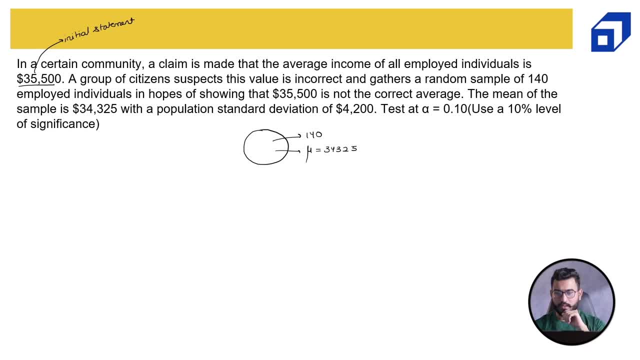 population standard deviation of four thousand two hundred and two hundred dollars. the alpha, alpha. what is alpha? the area of rejection. area of rejection is given as 0.10, which is 10 percent. now let's start with the formulation of the hypothesis. my alternate hypothesis is that the average is not equal to 35 500. 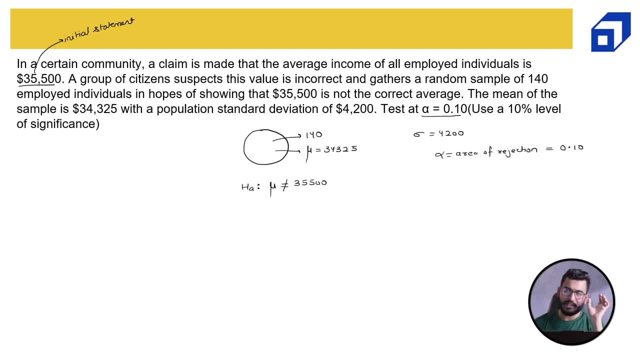 because 35 500 is the initial value, initial state. so group of citizen wants to prove that 35 500 is not the correct average. so that's my alternate. null will be opposite of this. mean is equal to 35 500. now what is my second stage? i will find out the lower critical. 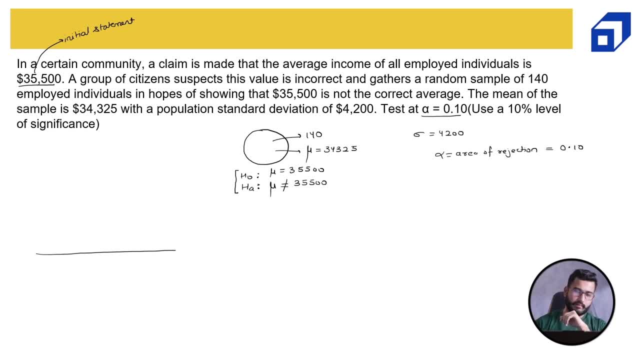 value and the upper critical value. so here is my normal distribution, since i am having not equal to sign in my alternate hypothesis. it is the two tail test. my area of rejection is on both the end, so this is also area of rejection and this is also my area of rejection. 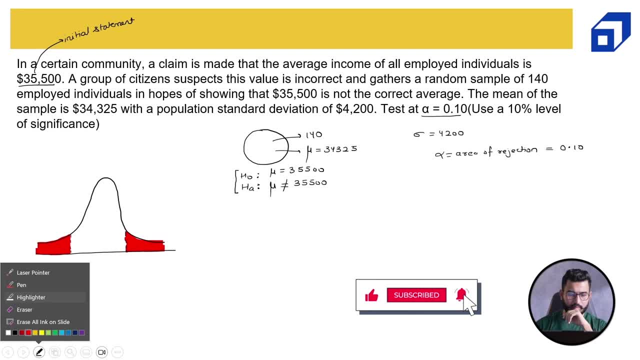 now we have to find out the lower critical value and the upper critical value. before that, we are given with the alpha of 0.10. since i am having rejection region on both the ends, my alpha will be divided by 2, so 0.1 divided by 2. so this will be 0.05 from here all the way up to. 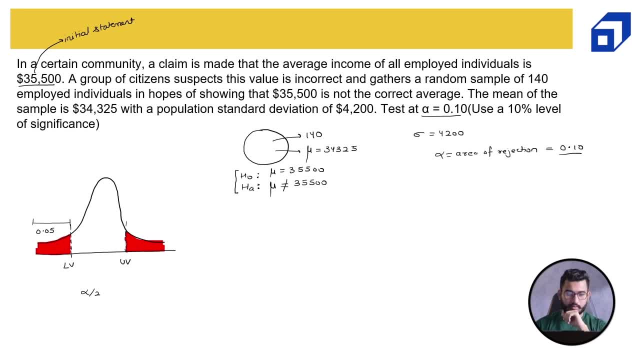 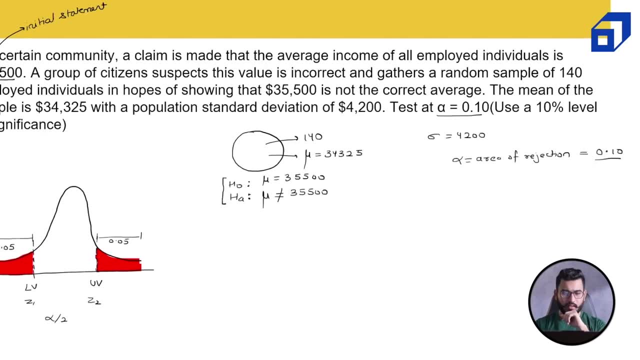 here, and this will also be 0.05. so this will be 0.05 from here all the way up to here, and this will also be 0.05. so what is the z value over here? again, we will use the z table, so we have to look at 0.05. 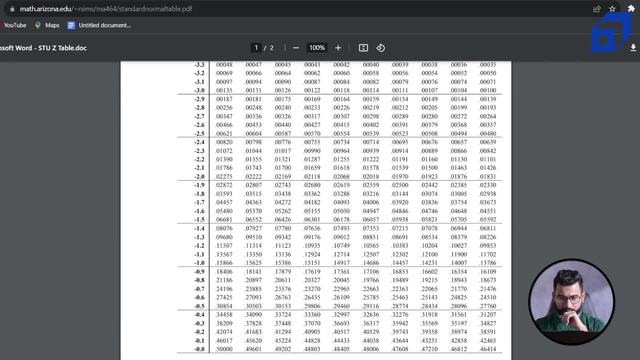 0.055. okay, over here maybe we can take this one or maybe this one. so minus 1.64. or 6: 5, you can take any one. so i'll go with minus 1.64. so this is minus 1.64, this is plus 1.64. now i have the z value. i have all the values. i have also the z values. so now 1.06 neurienen also, by the way. 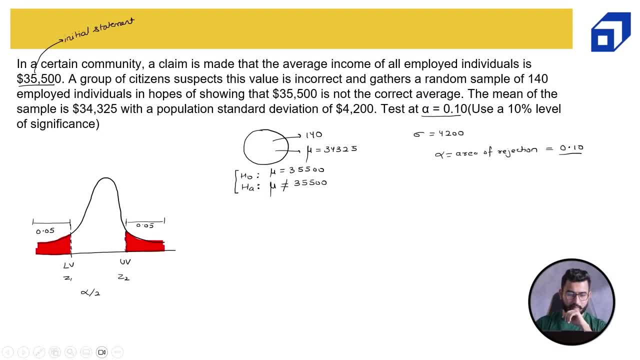 0.06 neurienen. also, by the way, t bis f drinking plus 1.64. example: let's calculate the range Mean plus minus z times of sigma divided by root of n. My mean is 35500 plus minus 1.64.. Standard deviation is 4200 divided by root of 140.. So the range would be. 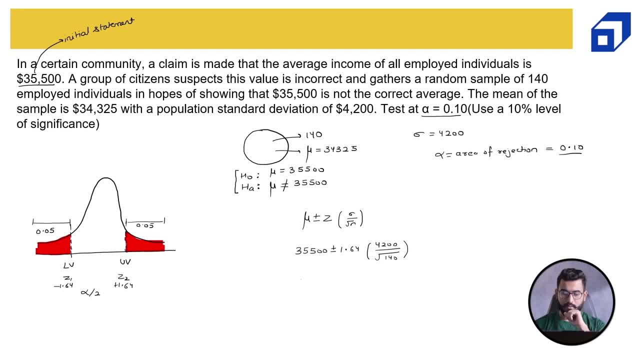 34917.76, comma 36082.24.. So this value lower value is 34917 and the upper value is 36082.. Now where my sample mean is lying at 34325.. So my sample mean is 34325.. So my sample mean is 34325.. So my 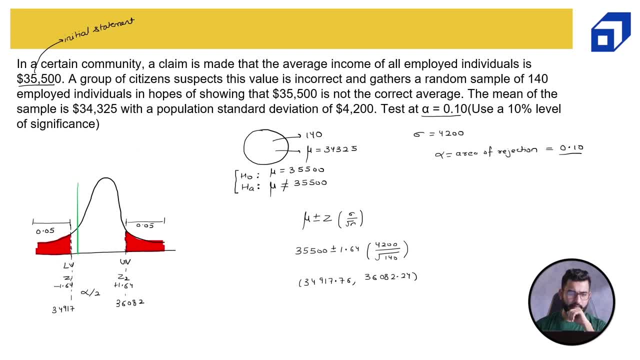 sample mean is 34325.. So my 34325 will lie somewhere over here, 34325 in the acceptance region. Since it is falling in the acceptance region, we conclude that we fail to reject null And that basically means the claim that was made was correct. 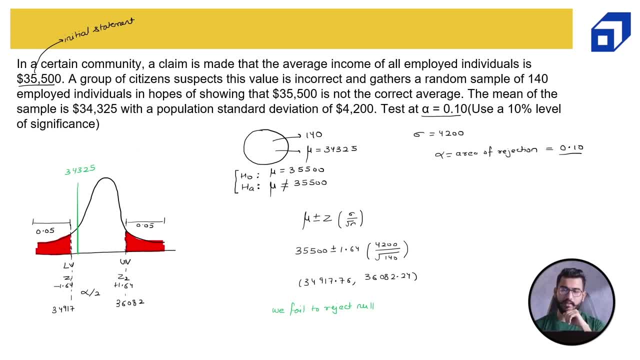 which basically means this null is actually true. Now I'm just saying we fail to reject null, but maybe because the sample size was less or because the sample collection process was biased, due to which the citizens were not able to prove that 35500 is a wrong average. 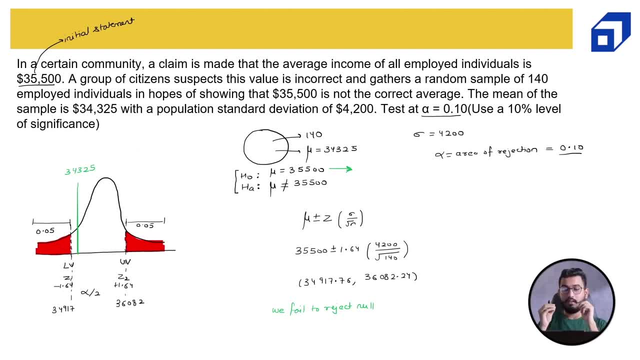 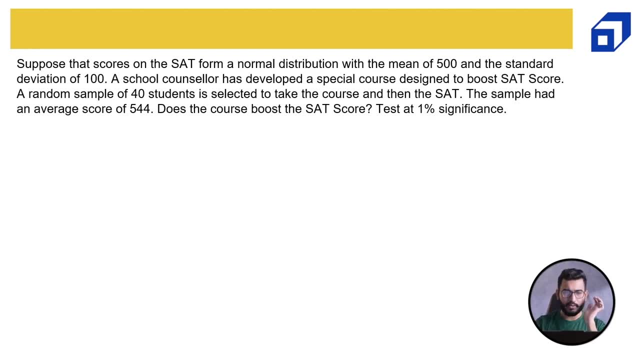 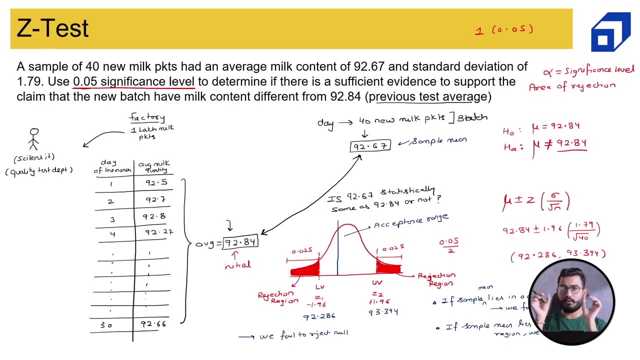 But as of now, using the test result, we fail to reject null. I hope this makes sense Now. here we have one more example. So we have seen two examples where we use two tail test where the rejection region was on both the end. But now let's take one example. 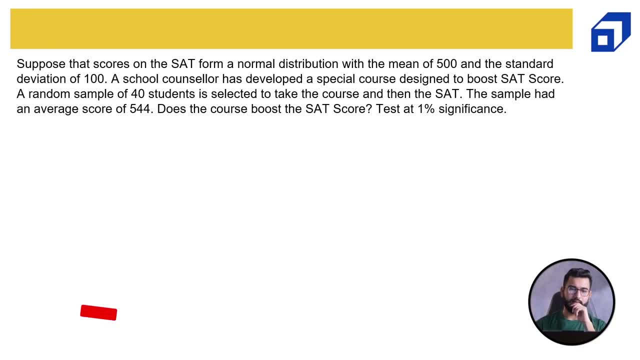 where I'm having a one tail test, either left or right. So the question says: suppose the scores on the SAT? so SAT is one of the examination form, a normal distribution with mean 500 and standard deviation 100.. The school counselor has developed a special course designed to boost SAT score. 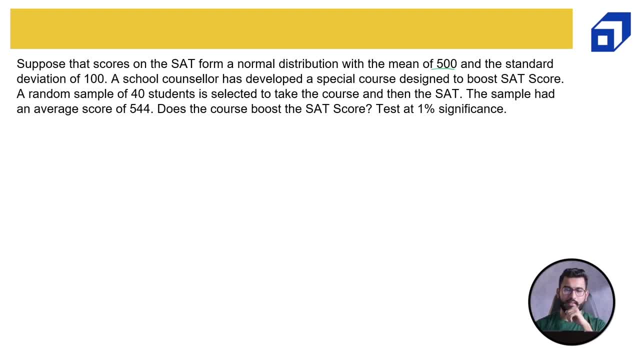 The school counselor has developed a special course designed to boost SAT score. The school counselor has developed a special course designed to boost SAT score. a random sample of 40 students is selected. So we have a sample of 40 students and the sample average came out to be 544 after they have gone through the course and they have attempted the SAT. 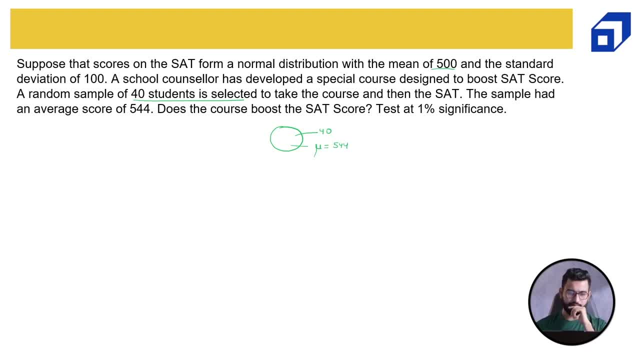 examination. The question already states that the SAT score is having a normal distribution with mean 500 and a standard deviation of 100. So this is my population parameter. You may assume these are the population parameters. Now, does this course boost their score? 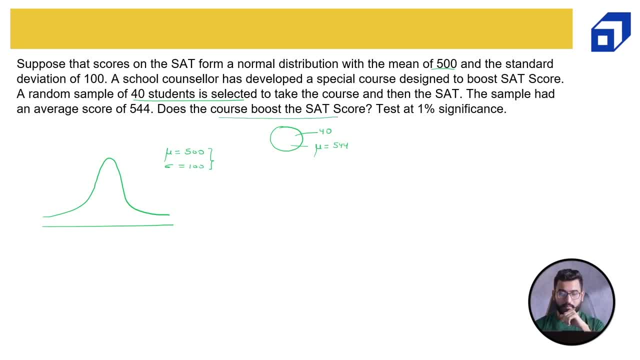 The does the course boost the score? So my alternate hypothesis is: does the average is greater than 500?? Because if the course boosts the score, it should be greater than the population average, which is 500,. right Null is it is less than or equal to 500, right Now greater. 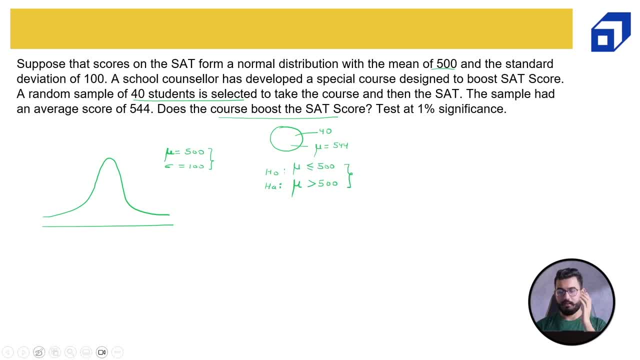 than 500 basically mean it is: the arrow is pointing on the right side, so it is a right tail test, So my rejection region will be on the right end. This is my rejection region. Now, what we have to do Again, we have to find out the Z value over here. So let's find 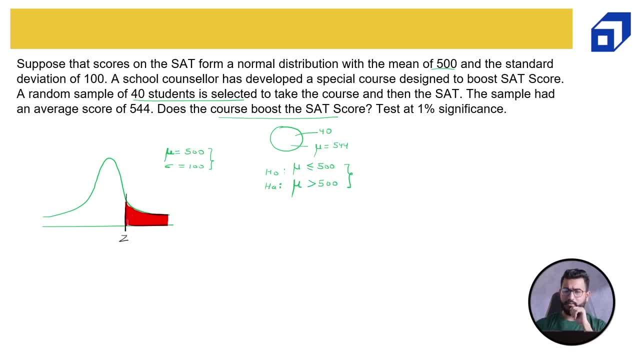 out the Z value over here Now, to find out the Z value, the area of rejection alpha is given as 1%, which is 0.5.. Okay, Okay, 0.01.. So this area, from this point all the way up to the end, is 0.01.. So what is the? 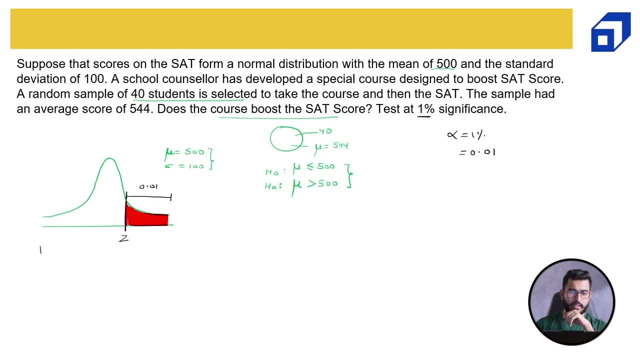 area from this point all the way up to this point, It will be 0.99.. So now we will use the Z table to find out the Z value at the AUC of 0.99.. So let's use the Z table. So. 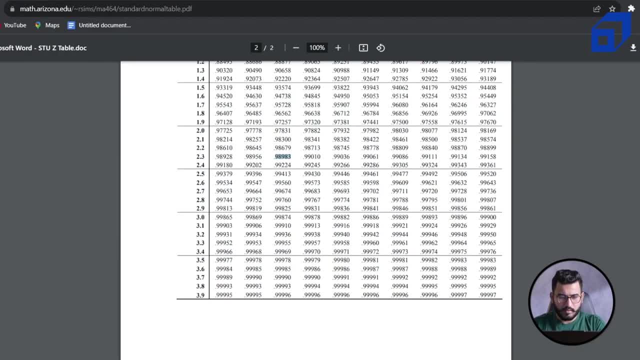 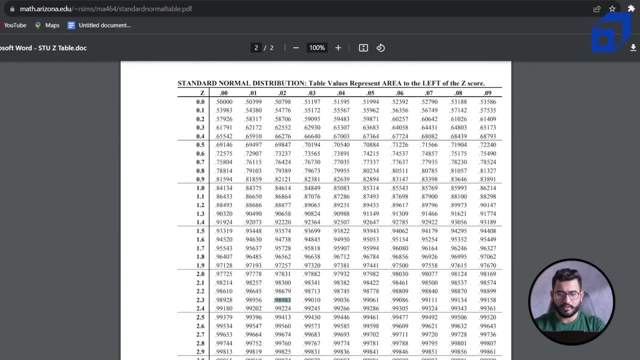 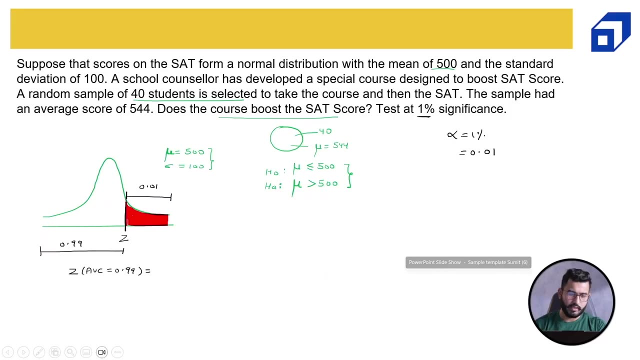 0.99.. What is the Z value? So either we can go with this value or we can go with the Z value. So this is 2.32 or 2.33.. So I'll go with 2.32.. So Z value is 2.32 and this is. 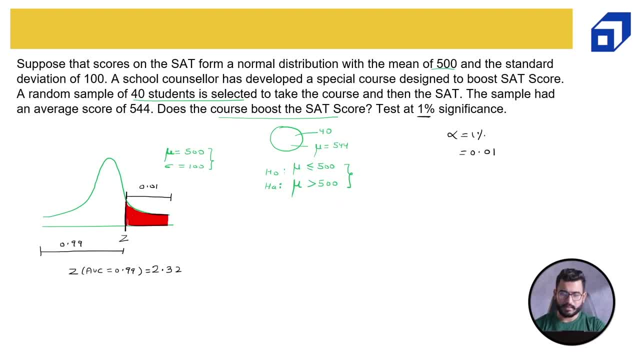 plus. Now let's apply the formula mean plus Z times of sigma divided by root of n, Remember the lower value will now be minus infinity. We have to just find the upper value. So mean is 500 plus 2.32.. Sigma is, which is the standard deviation, is 100.. So this will come out to be 36.6.. 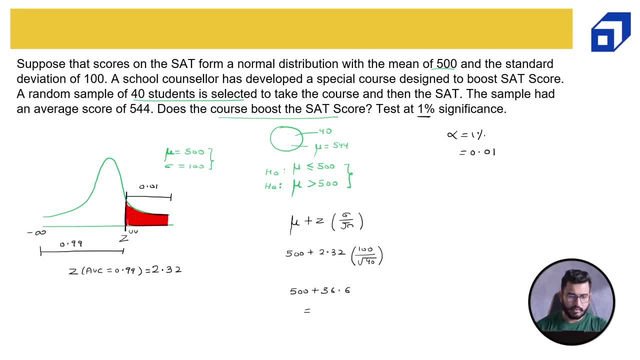 So the total is 536.6.. So this value over here is 536.6.. Now where my sample mean is lying at. My sample mean was 544.. 544 will lie on this side, right On this side, So 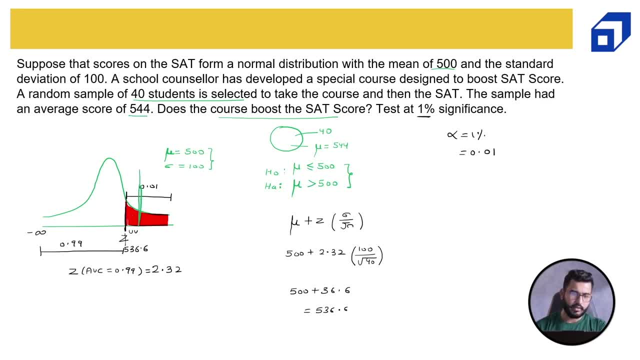 the rejection side, this side. So this will be 544.. So since my sample mean is lying at the rejection region, we conclude that we reject null. So if I reject null, that basically means the course does increase the SAT score. The course does increase the SAT score. So 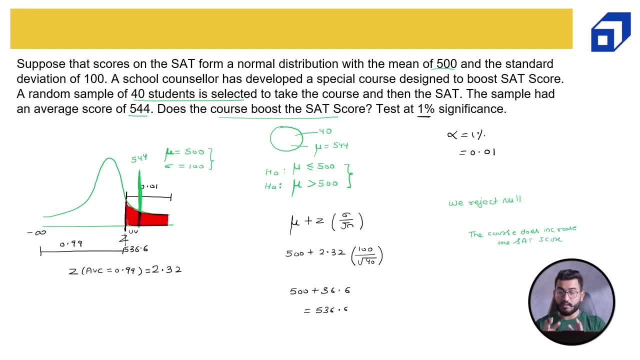 now, please remember this statement is based on this particular sample. I'm not saying it will always increase the SAT score. Based on this sample, the conclusion is that course does increase the SAT score, but it might be because of some uncertainty. It might be. 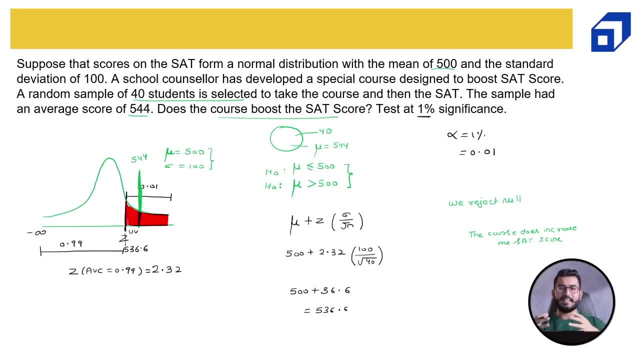 because when we were, when we were selecting the students, we have only selected the intelligent students with higher IQ, And that is the reason we obtained the average, which is greater than the population average. So it might be because of the uncertainty also, So that is. 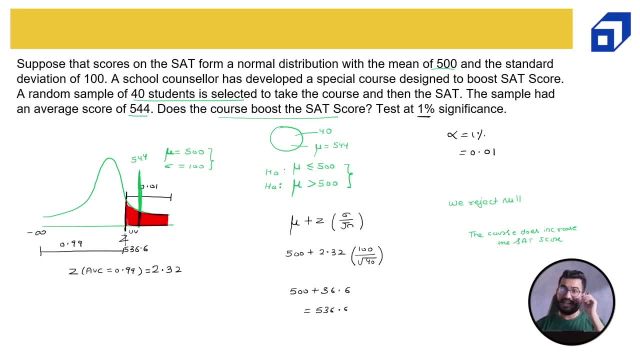 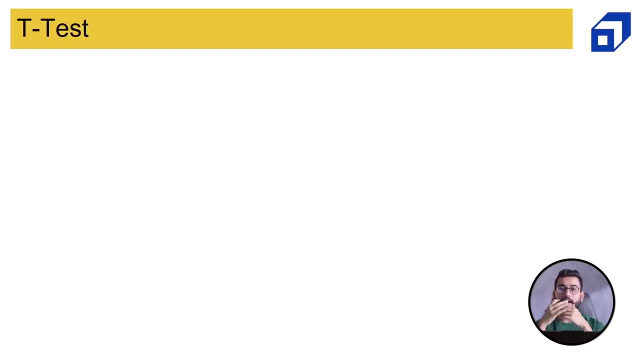 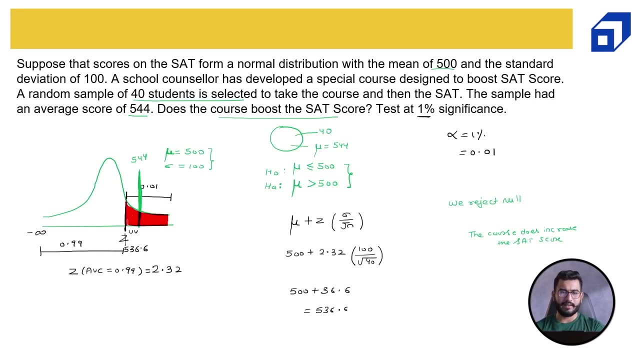 the reason we say we reject null, We are not saying we accept alternate. We will not say that. I hope now the thing is making more sense. So now let's talk about t-test. We have already seen a z-test in very much detail. 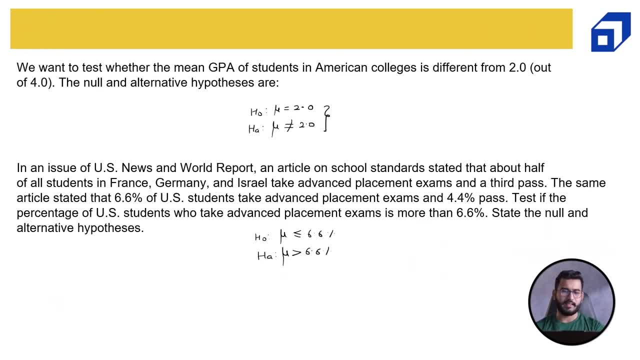 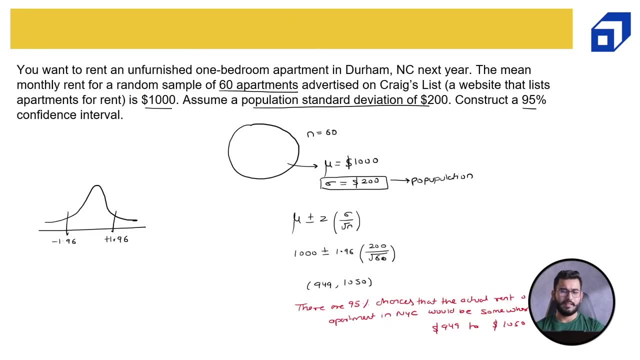 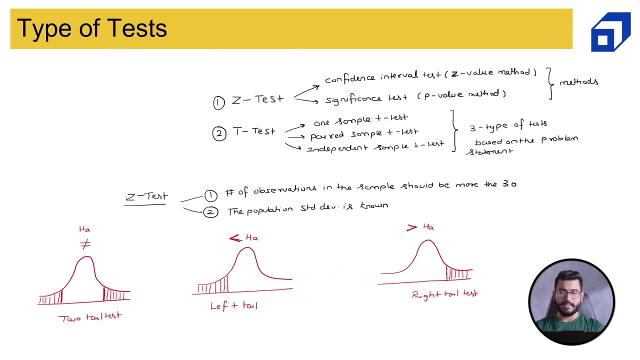 We have solved three problems. Now let's talk about t-test. And before we jump into solving few problems using t-test, let's first of all understand when to use a t-test. So we have already talked about z-test, Now let's write down the conditions for t-test. So I 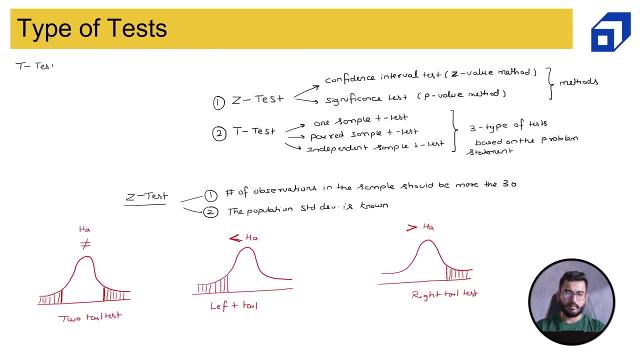 will write it over here: t-test. So we use t-test condition number one when the initial number of observations in the sample is less than 30. So the number of observations is less than 30.. This is my first check. The second check is population standard deviation. 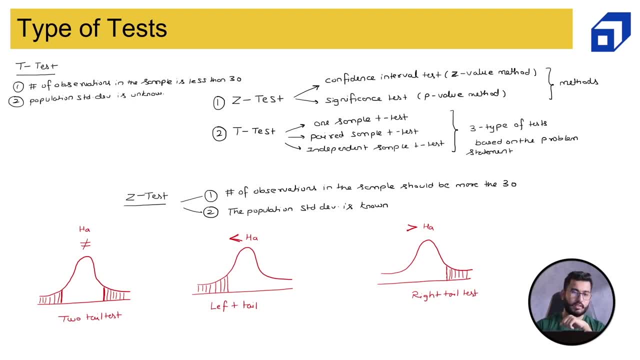 is unknown. The third check is: the sample has been taken out from a population which is known to be normally distributed. The sample has been taken out from a population which is known to be normally distributed. Now, what is the meaning of the sample has been taken out from a population which is 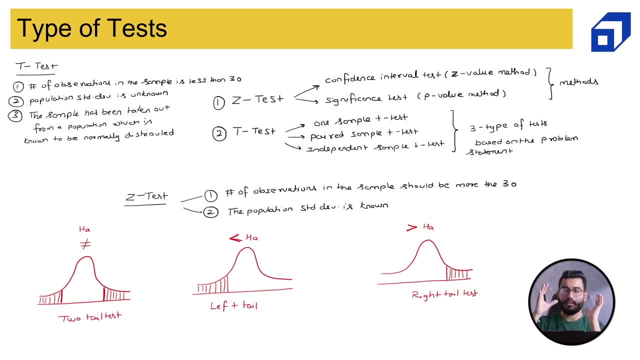 known to be normally distributed. So let's say I take example of income. I know that in India the income is normally distributed. Now, if I take a sample of five people now, this sample will satisfy the t-test condition. t-test. 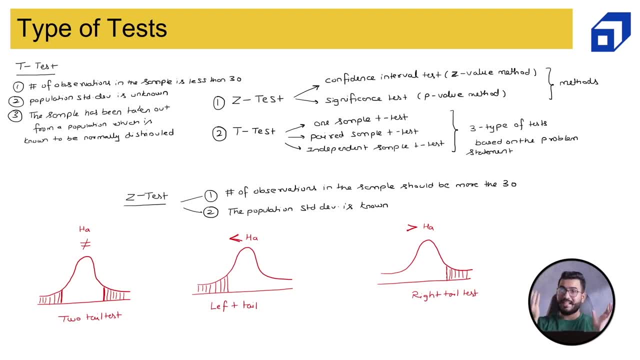 t-test parameters because I know that it has been taken out from a population which is normally distributed, The number of observations in the sample are less than 30 and the population standard deviation is unknown, So I don't know what is the standard deviation of the. 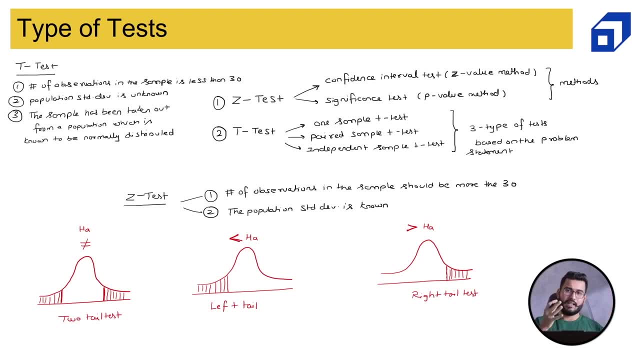 income in my Indian population, because the population is really large, right? So before we apply t-test, we have to check these conditions, We have to check these parameters. Now let's solve a problem. to understand this, As I've already told you that t-test can be performed, 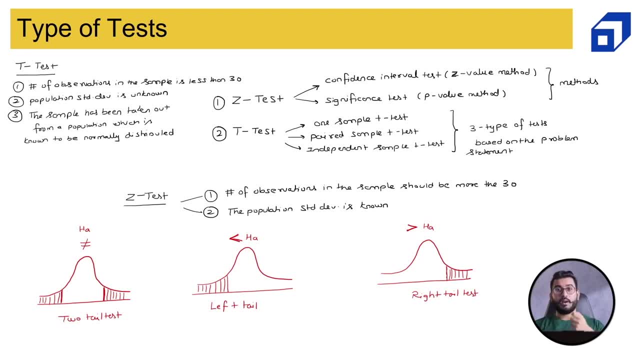 or there are three types of t-test based on the problem statement. So let's try to understand them very briefly: about what kind of problem statement satisfy which kind of t-test? Now, there can be three types of t-test: One sample t-test. 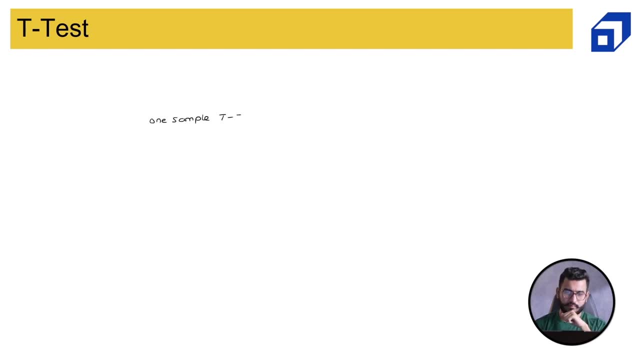 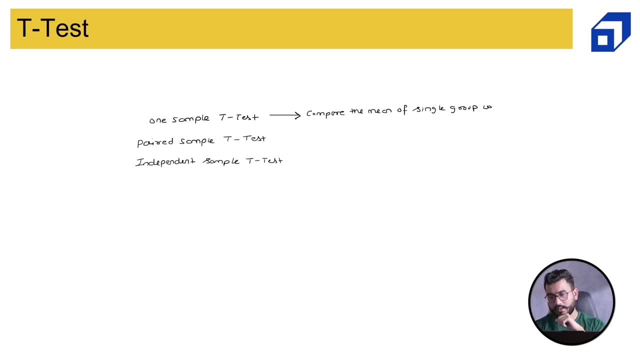 single group with known mean. now, if it is not making sense, don't worry, we will when we will be solving a problem. then i'll better explain you this paired sample t test. here we compare the mean of the same group at two time, or two time two different time, so at two: 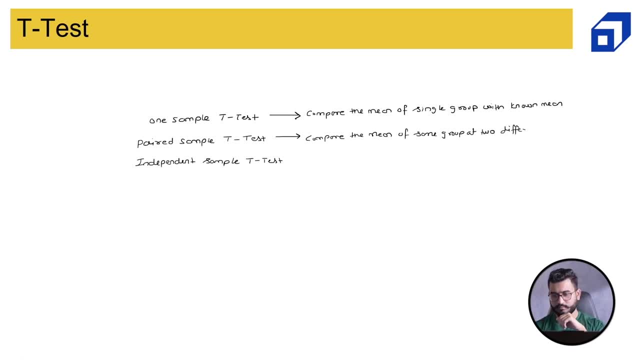 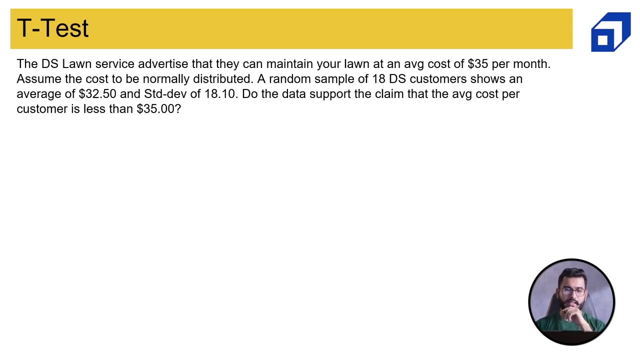 different time. in independent sample t test we compare the mean of two different groups. now, if it is not making sense, don't worry, we will take example of each one of them and then it will make more sense. let's start with one sample t test. so a ds lawn service advertise. 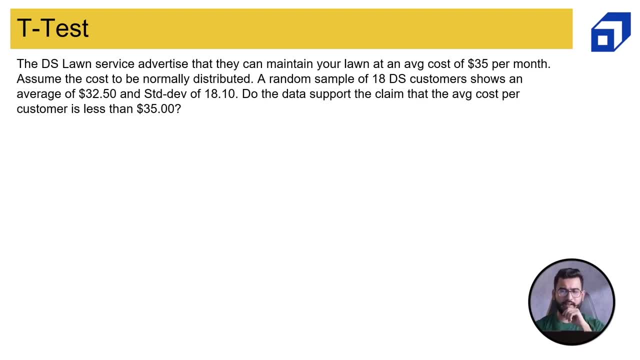 that they can maintain your lawn at an average cost of 35 dollars per month. now, this is what their a proven value is: the initial value that they have given. assume the cost to be normally distributed. now, this is a very important sentence. the population is normally distributed. that has. 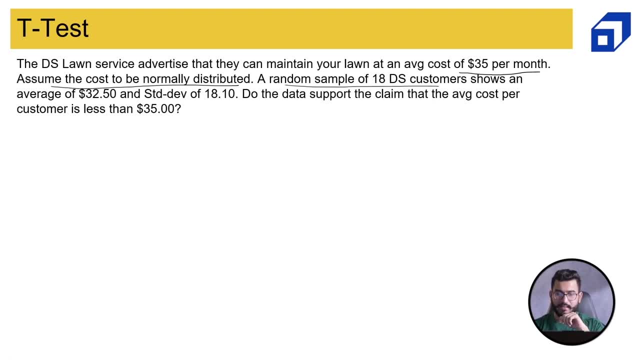 been given to us. a random sample of 18 ds customers shows the average of 32.50, so we have taken a sample. the sample is having the mean of 32.50 and the sample is be 18.10.. Now we know that this sample has been taken from a population, from a population. 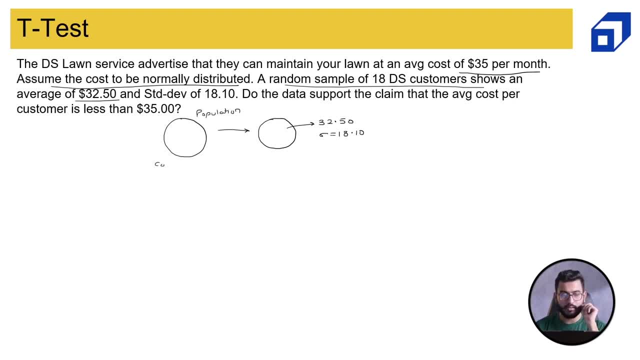 in which the cost was normally distributed. Cost was normally distributed. So first of all let's check whether this question or this particular problem satisfies the condition of t-test or not. The very first condition is: the number of observations in the sample should be less than 30. Here my n is 18.. So yes, first condition is satisfied. Second, 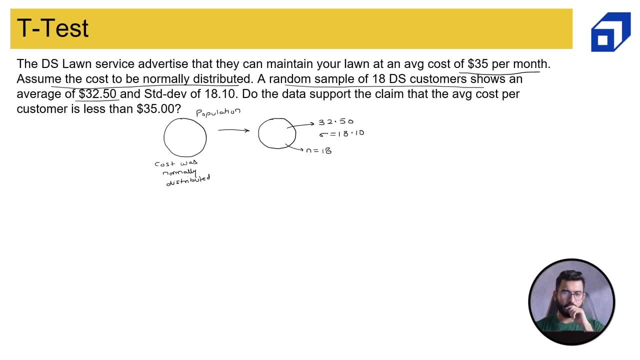 condition is the population standard deviation is unknown. Yes, we do not know the population standard deviation, but we know the sample standard deviation. And the third one is the sample has been taken out from the population which is normally distributed, So this particular sample has been taken out. 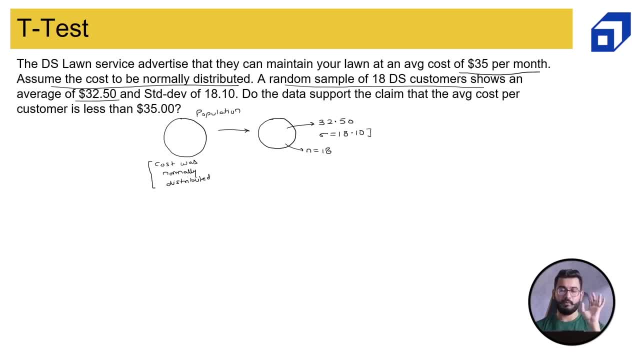 From a population where the cost was normally distributed. So all the three conditions are satisfied. Let's try to see the procedure now. Number one: we have to formulate the hypothesis. So my alternate hypothesis would be that the average average cost is less. 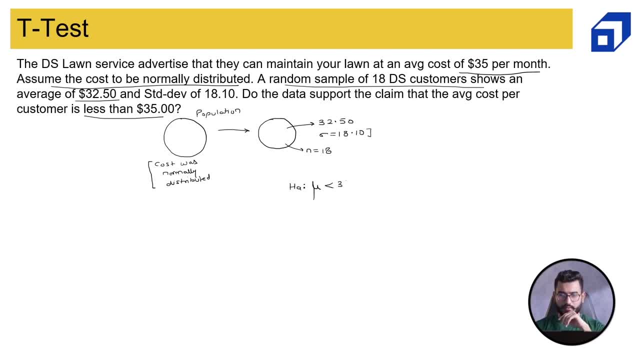 than 35.. So this is what we want to test. So average is less than 35.. Null will be: average is greater than or equal to 35.. This is my null and alternate hypothesis. Again, since I'm having less than sign in. 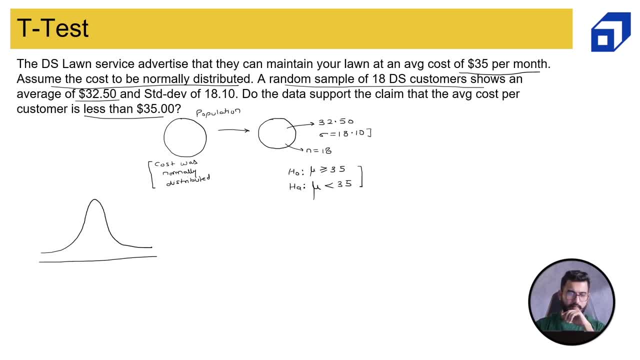 my alternate. it is a lower tail test, So lower tail test. Now we will find out the t-critical. Now t-critical formula is similar to z-value: X minus mu, divided by sigma, divided by root of n. I hope you guys remember the z-value formula when we were talking about 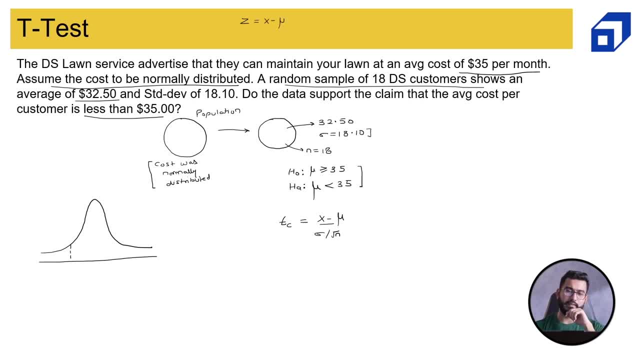 the z-scaling. The z-value formula was: x-minus mu, x-minus mean divided by sigma. Now here I'm using sigma divided by root of n is because this distribution is a sampling distribution and the standard deviation of the sampling distribution is given as sigma divided by root of n according to the central limit theorem. 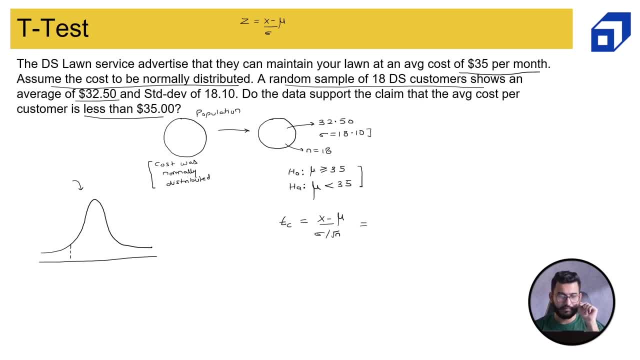 Now, what is x? X is my sample mean, which is 32.50.. Mu is my population mean, which is 35 divided by sigma, 18.10 divided by root of 18.. What is the value? You guys can quickly calculate it. 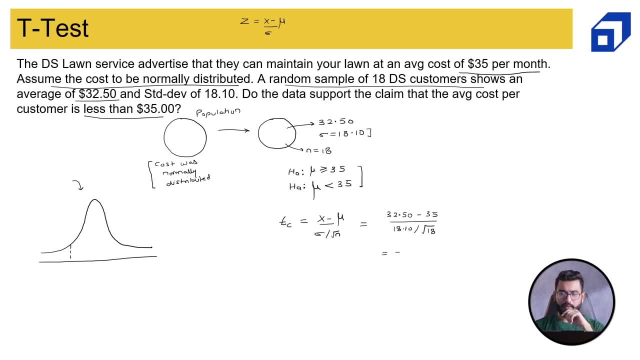 I have already calculated it, So this will be minus 1.30.. Sorry, there is a one correction. This is not t-critical, this will be t-estimated, So t-estimated is 1 minus 1.30.. Now we will. 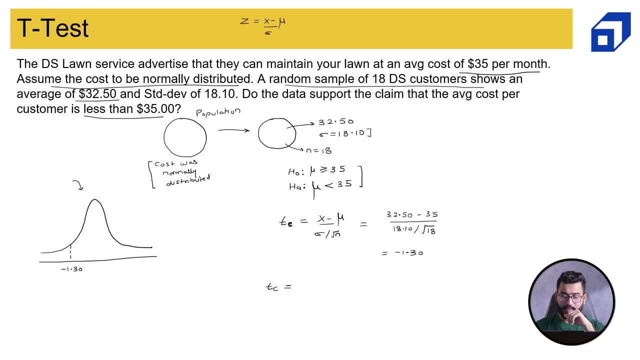 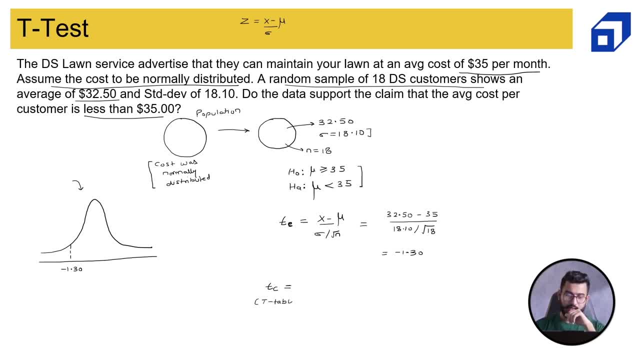 using the T table, and T table requires your alpha, which is given as. so okay, I haven't written alpha, So let's assume alpha to be 0.05.. So alpha is 0.05 and degree of freedom? Now, degree of freedom is given as n minus one. but what is degree of freedom? What is? 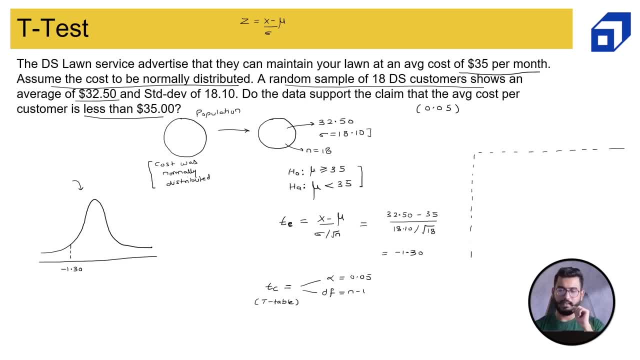 degree of freedom. So let's understand degree of freedom. Now, let's say there are three people: one, two and three. These are the three people. and let's say these are A, B and C, and this is Sumit. Now, what I have. 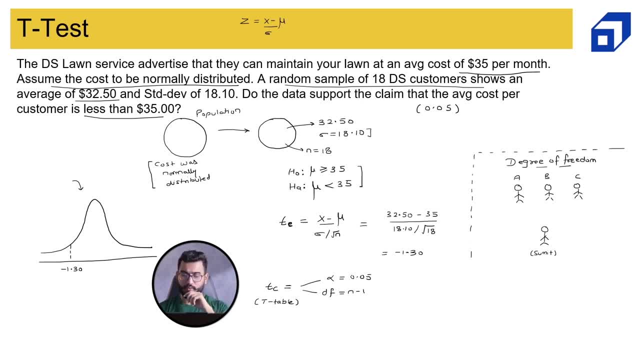 what I'm asking A B C to do. I'm asking A B C to choose one number in such a way that the total is 10.. Now, let's say so. let's write down A, B, C and the total. Now we already. 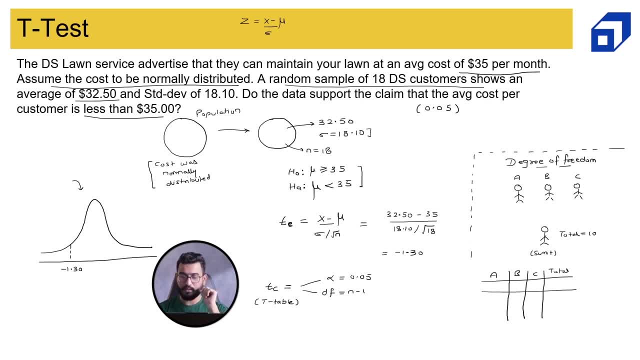 know that the total in all the cases would be equal to 10.. So let's say A has chosen five, B has chosen three, Then C is bound to choose two. Let's say A has chosen five, B has chosen five, then C is bound to choose zero. Let's say: 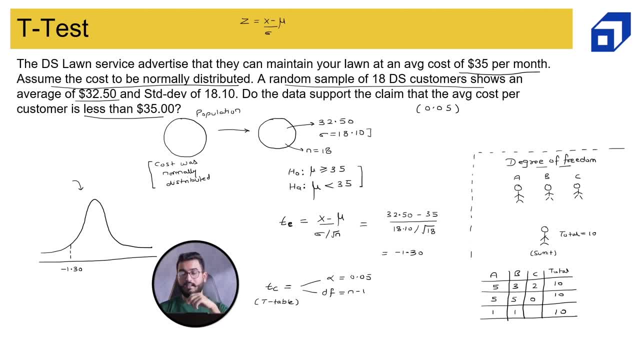 A has chosen one, B has chosen one, Then C is bound to choose eight. Now you hear, you guys can see that component, or the third data point in my summation, is not free to choose a value when we already know the total. So there are only two values, A and B, which are free to choose any value. 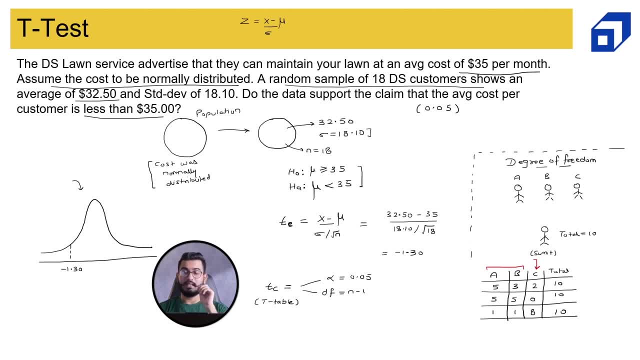 of their choice, but C is always bound. C is always bound to choose a value that is left out. So degree of freedom talks about how many observations in our data are free to choose a value- the number of observations in the data that are free to choose a value. 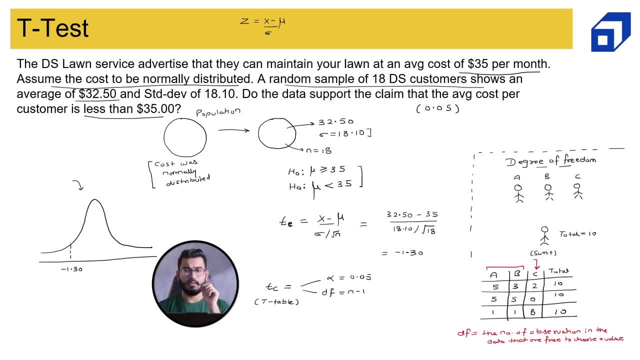 Now here, since we know the sample average, Since we already know the sample average, the degree of freedom will always be n minus 1, because there will be always one value which will be bound to choose, a value that can make the average to come out to be what we are given with. So here, 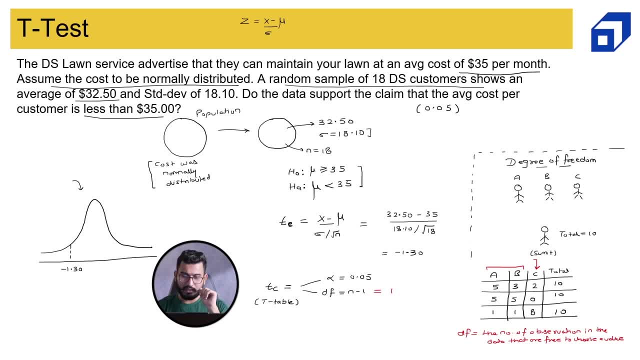 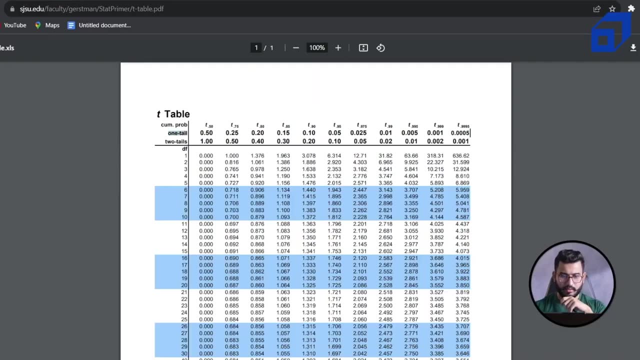 degree of freedom will be n minus 1, n is 18, so 18 minus 1 is 17.. Now we will use the t table with these two parameters to find out the t critical value. So let's use the t table. So this is a one tail test with the significance of 0.05 and the degree of freedom. 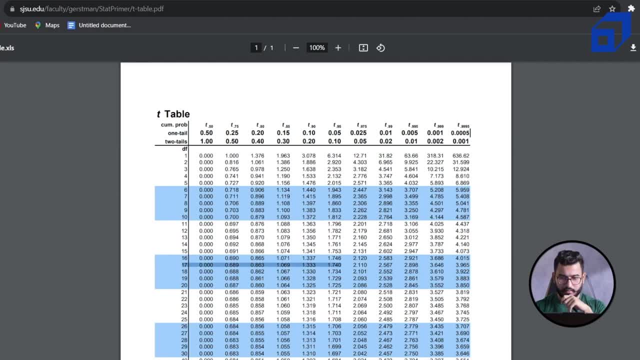 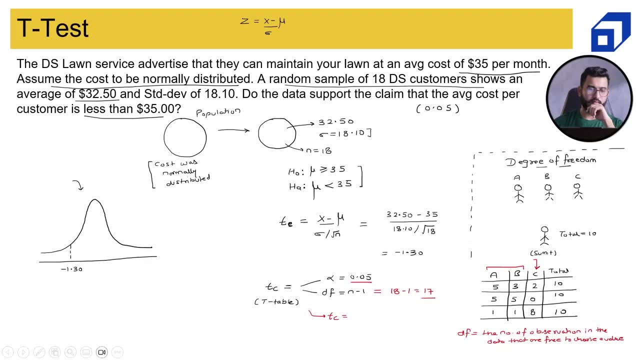 to be 17.. So here, so correct value is minus 1.74.. Okay, So t critical is minus 1.740.. Now I'll quickly delete this because I do not have to write this first. First of all, we will write the t critical minus 1.740.. Now where this minus. 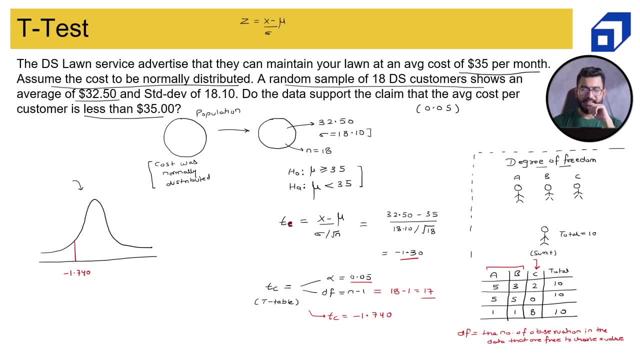 1.30 will lie t estimate. T estimate will lie, let's say so, minus 1.3.. Okay, So minus 1.3 will lie over here. So this is my rejection region which is below the t. 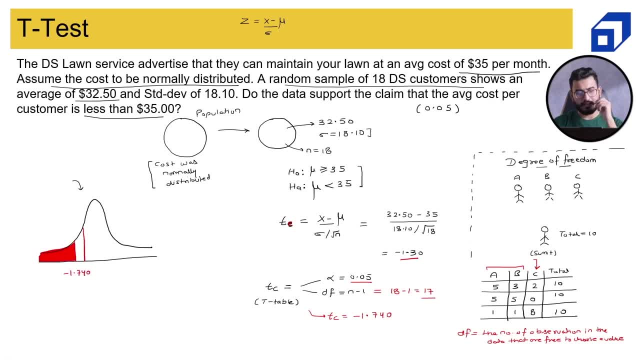 critical value and my t estimated is beyond the t critical. So this is the boundary t critical And this is my t estimate. Now, since t estimate is on the acceptance side, we say that we fail to reject null, which basically means that this statement it is greater than or. 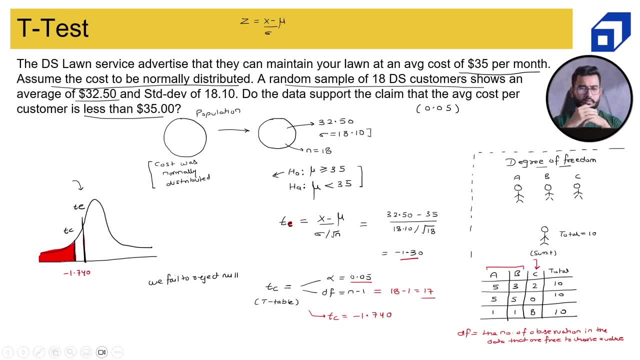 equal to 35. That basically means those people or those people who were doubting, who were having the doubt. Okay, Regarding this DS lawn service, they were actually correct that, based on this sample, we can conclude that the average cost that this DS lawn service charges for maintaining 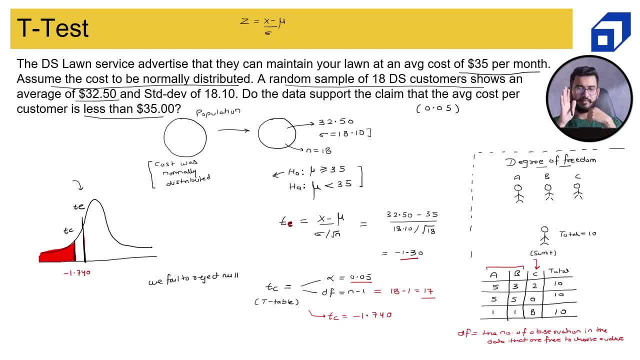 your lawn is not 35 or less than 35. It is more than 35. I hope this is making sense. This was one sample t test, One sample t test. Now, the reason it was one sample t test is because we have one group. 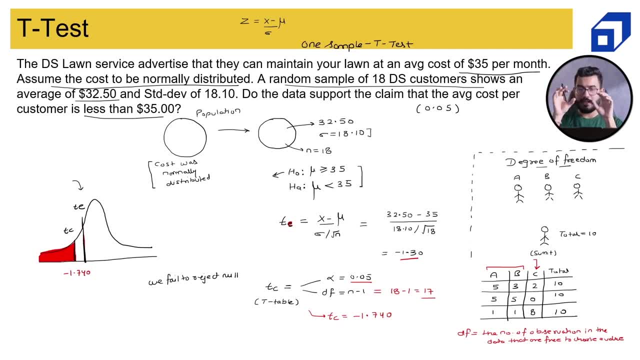 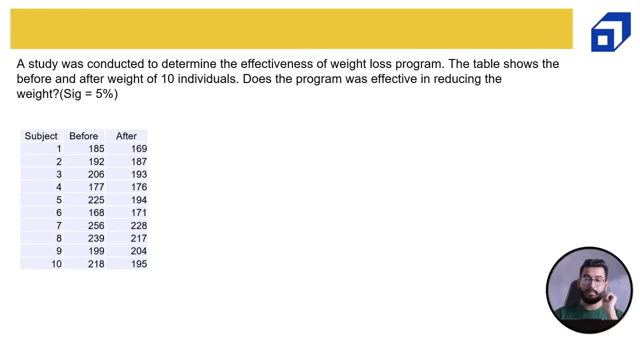 we have a known mean which is 35, and we are comparing the sample mean with the known mean. So this is one sample t test. Now in the paired sample t test, this is the example of paired sample t test. Okay, 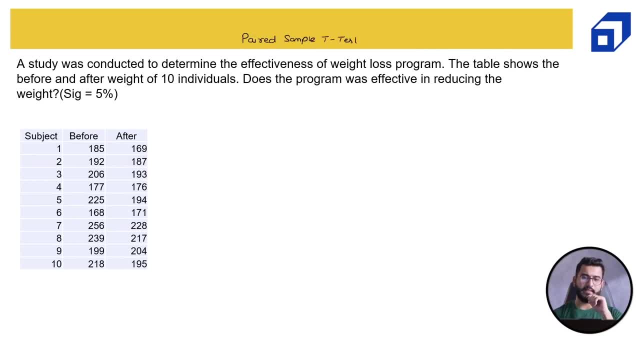 Okay, So here we compare the average of one group at two different times. So here you can see that we have before result and after result. Let's try to solve this problem to better understand this. So here in this question we are given with the problem statement states that a study 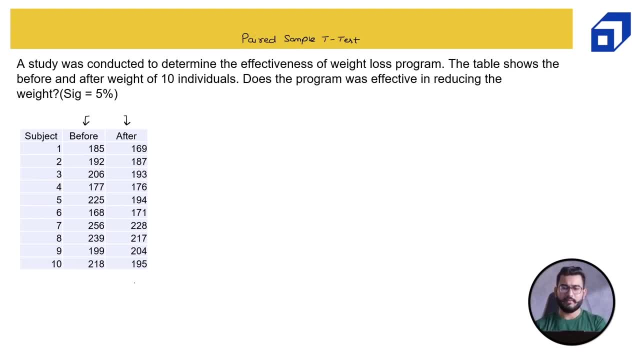 was conducted to determine the effectiveness of a weight loss program. The table shows before and after weight of 10.. Does the program was effecting in reducing the weight? We have to test at a significance of 5%. Now, if we logically think about this question, the program will be called effective when 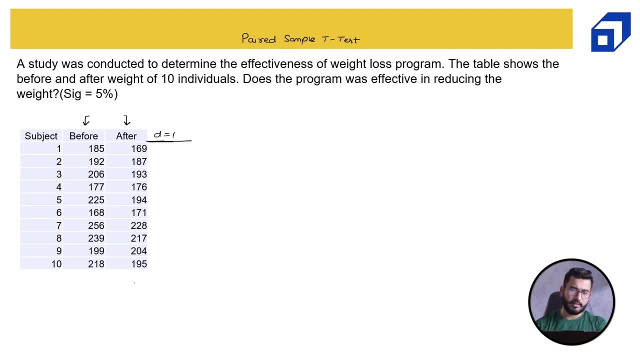 the difference. what is the difference after minus before, when the difference is negative? So let's calculate the difference. I have already calculated it, So I'll calculate it. Okay, So I'll just fill the table. So 169 minus 185 minus 16 minus 5 minus 13 minus 1 minus. 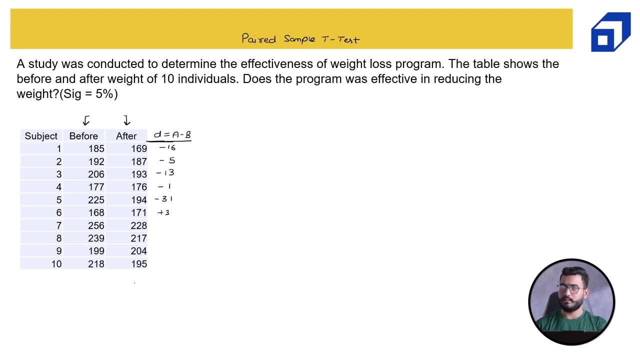 31 plus 3, minus 28, minus 22 plus 5 and minus 23.. Now these are the differences. If this difference is negative, that basically means the person obtained or the person achieved the weight loss. If it is positive, that means the person achieved the weight gain. So if 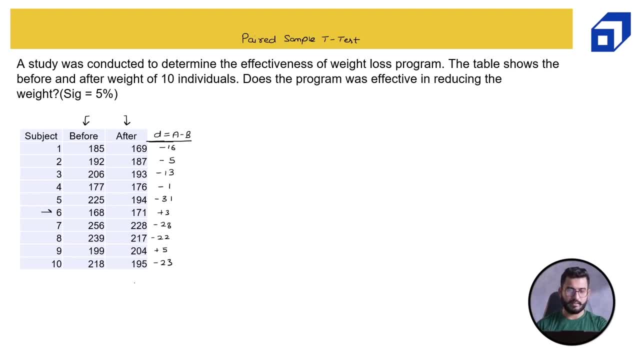 I look at this observation of individual number six. the person was having a weight of 168. It increased to 171. So the person gained one, three, three units of weight. Now the person was having a weight of 168. It increased to 171. So the person gained one, three, three. 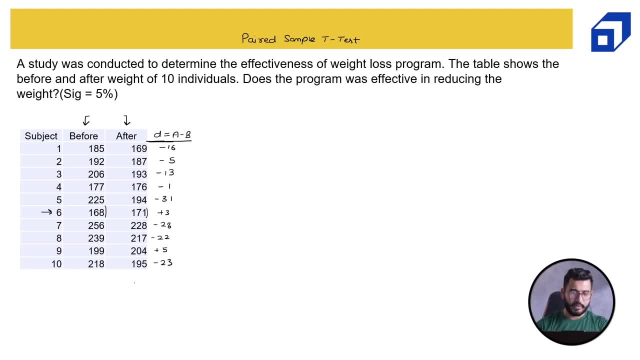 units of weight. Okay, While this person, whose weight was 218, now it came to 195.. So this individual achieved a loss in the weight of 23 units. Now I will call this program effective if the average difference is below zero. right Below zero means negative. So my alternate, my null alternate. 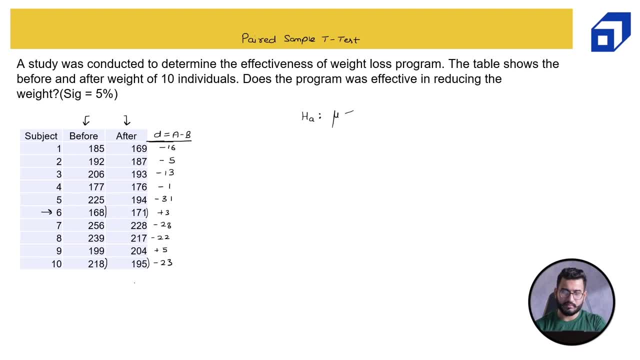 hypothesis will be Okay If the average is less than zero, because initially I will consider that the program is not effective. Initially I will consider that the program is not effective, So initial statement will be: the average is either greater than or equal to zero. So assume that this. 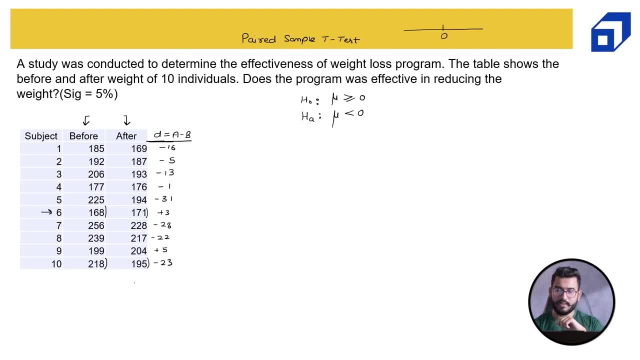 is a number line of differences D there. Uh, if my average average difference is zero or above- this is zero or positive, then my program is not effective. If it is negative, then my program is effective. So these are my null and alternate hypothesis. Now what we have. 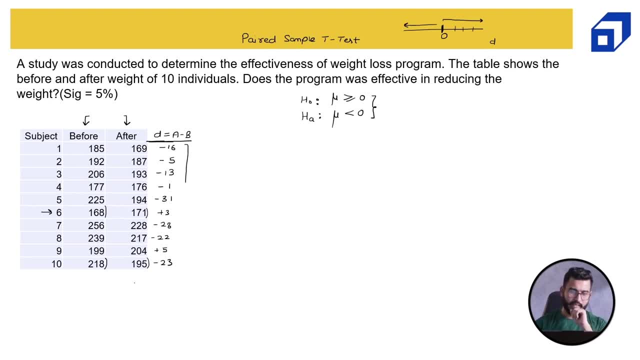 to do this is my sample. So I need the sample mean for mu X, my average of differences. So I will just write mu D, the average of differences. I have already calculated it. You guys can use Excel for this, for this quick calculation. So the average difference is minus 13.1 and the standard 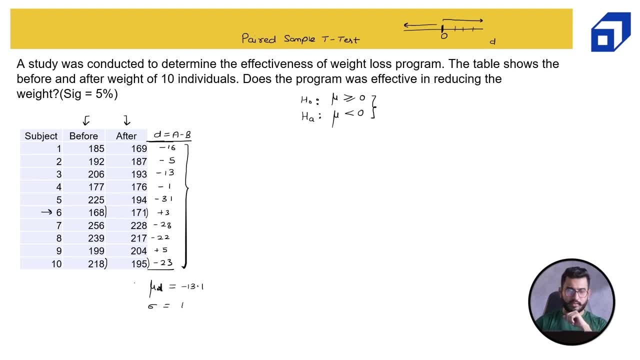 deviation of the sample is 13.02.. This is my sample statistic. Now I will calculate the T-estimate. T-estimate is X minus mean divided by sigma. divided by root of n, My X is minus 13.1.. My M is 13.1.. Population mean is zero. Population mean is zero which. 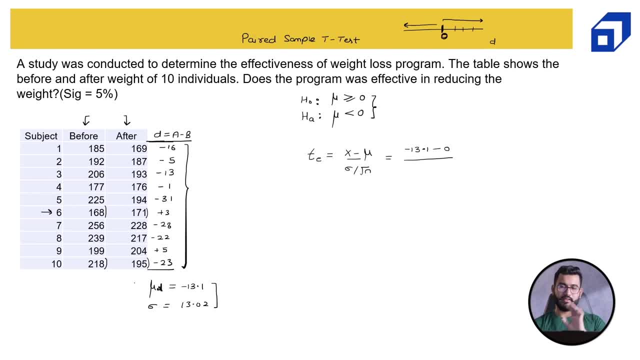 we have assumed that there is no change, There is no gain, There is no loss. Zero Sigma is 13.02. divided by root of n, n is 10.. Now this will come out to be minus 3.18.. Now, using 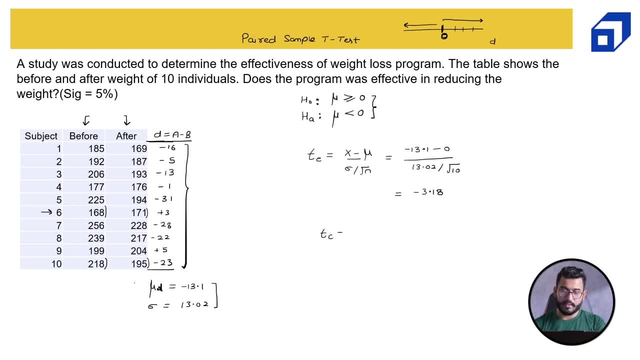 the alpha, which is 5%, so 0.05, and degree of freedom, which is n minus 1,, which is 10 minus 1,, which is 9,. I will find out the T-critical using the T-table. So let's quickly do this. 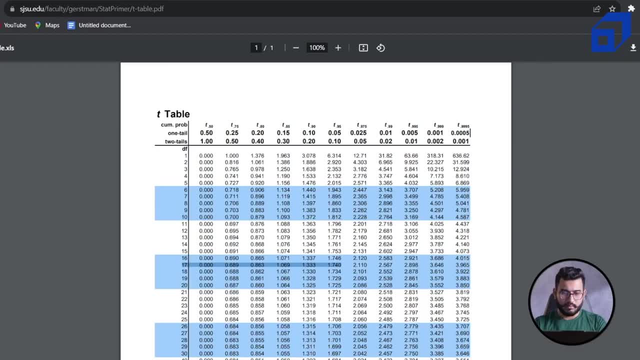 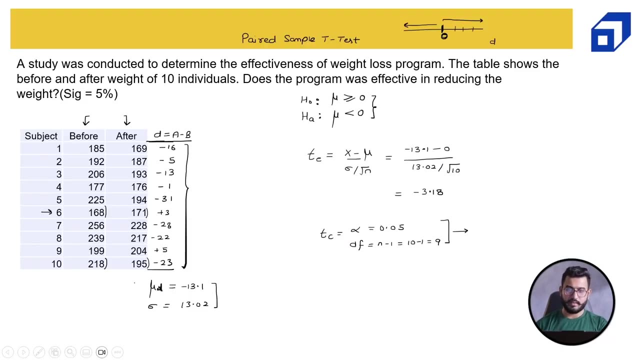 So degree of freedom. so this is a one-tail test. Significance level: 0.05.. Degree of freedom to be 9.. So here we have the value 1.833.. 1.833.. Now, since it is a lower-tail test, because 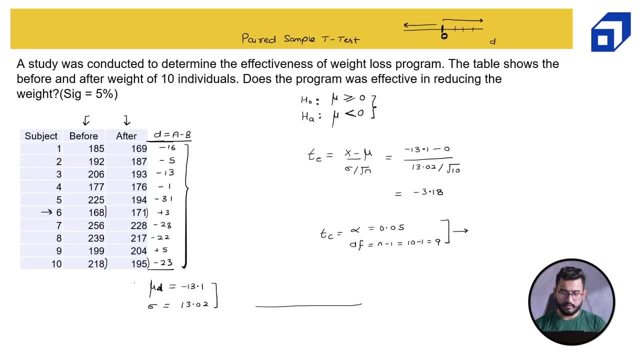 I am having lower sign or less than sign, the value T-critical will be. let's say this: T-critical is minus 1.833.. Now, where this minus 3.18 will lie, Minus 3.18 will lie over here. T-estimate Now, since: 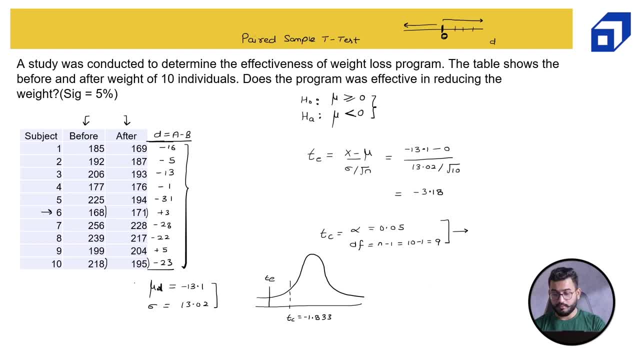 it is lying on the rejection region. we can do that. We reject null, which basically means yes, based on this sample, the program was actually found effective. So, yes, it was found effective, maybe based on this sample. However, we are also going to do this test to determine. 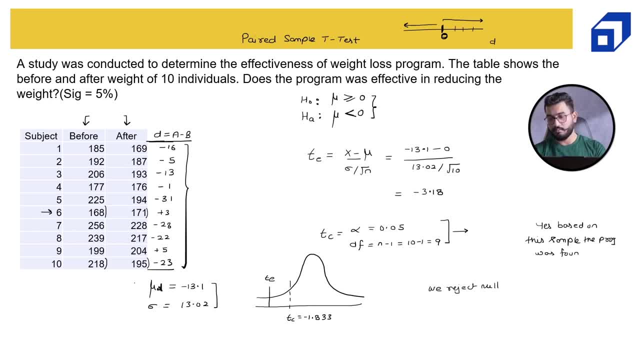 based on this sample, The program was found to be effective. Now here you can see that the reason we call this as a paired sample T-test is because we were having the same group, but at two different time, before and after same set of people. 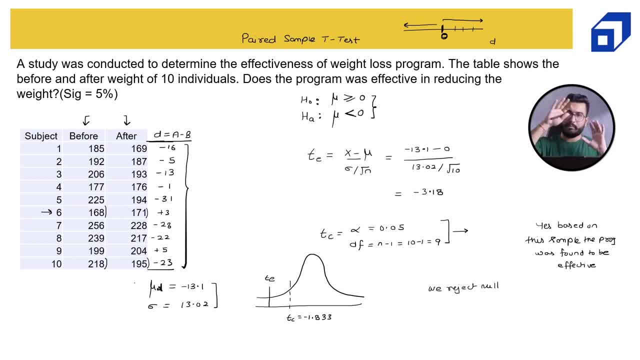 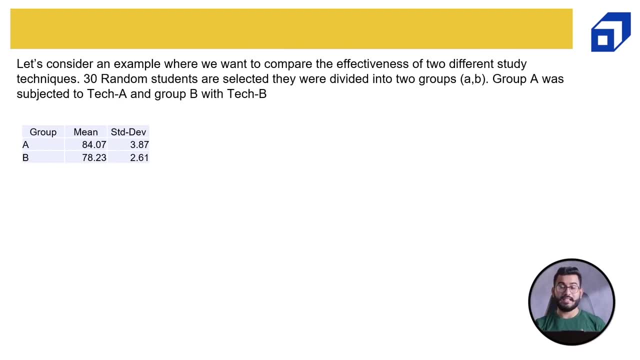 before and after. So Therefore paired samples are the same group and same set of people before and after. So paired sample t-test: We are comparing their average or the average difference. Now we have independent sample t-test, which basically means now we have two different group: group A, group B. 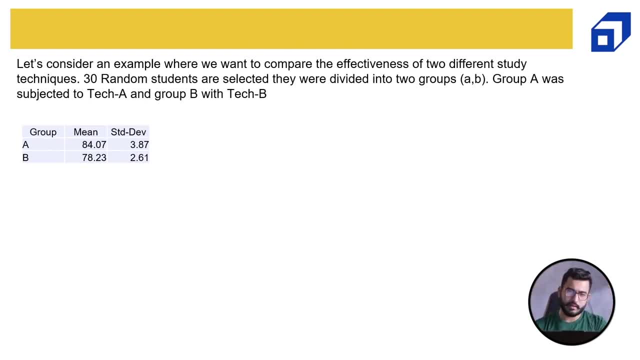 and we have to compare them. So let's see this example. So this is the example of independent sample t-test And in this particular test we are having two different groups. Now if you read the question, it says: let's consider an example where we want to compare the effectiveness. 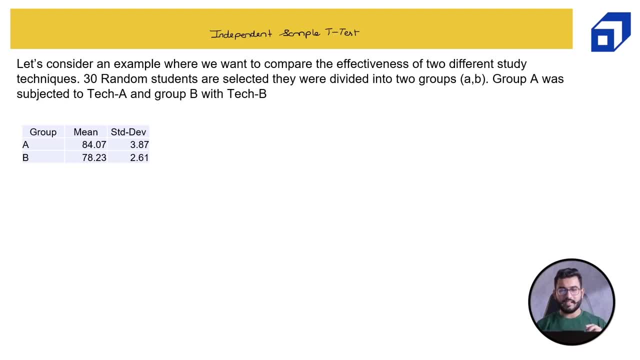 of two different study techniques, 30 random students are selected. they were divided into two groups. Group A was subjected to technique A. Group B was subjected to technique B. Now, please remember, I'm having total number of students to be 30, where we have divided them. 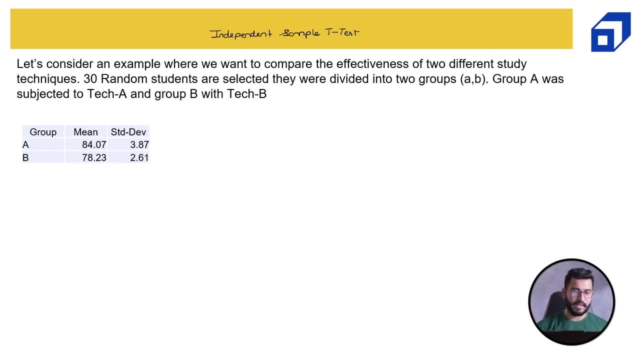 into two equal groups. So that basically means Group A consists of 15 students, Group B consists of 15 students. Group A consists of 15 different students, Group B consists of different students. So these two groups are not having any association between them. They are two different groups. Now I want to compare whether technique A and 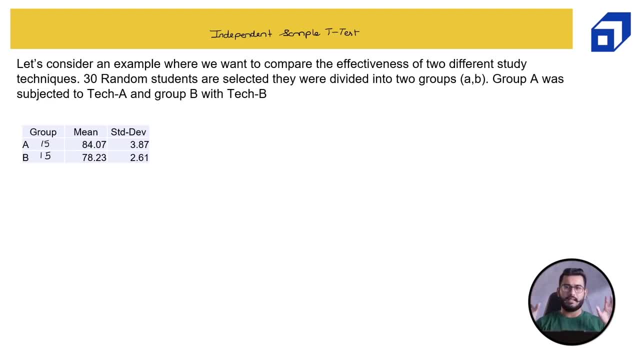 technique B: whether they are same or different. That's what my test is: Whether they are same or whether they are different. So my alternate hypothesis will be: average of A is not equal to average of B. My null hypothesis will be: average of A is equal to average of B. So 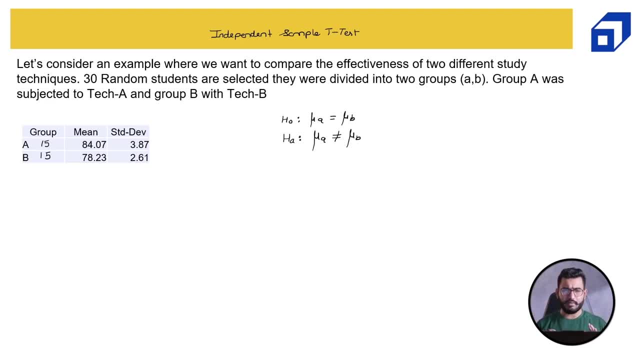 my null hypothesis is that I'm initially assuming that these two techniques are same, where what I want to prove: that these two techniques are different. So that's my null and alternate argument. Now we will follow the same procedure, but there will be a minute difference in the t. 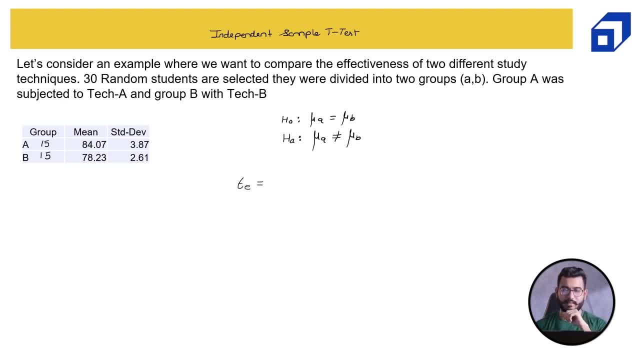 estimate. The formula for t estimate is: x1 average minus x2. average minus mu1 minus mu2, divided by square root of sigma1 square divided by n1 plus mu2.. sigma2: square divided by n2.. So here in my table I'm already given with mu1 and mu2.. So let's. 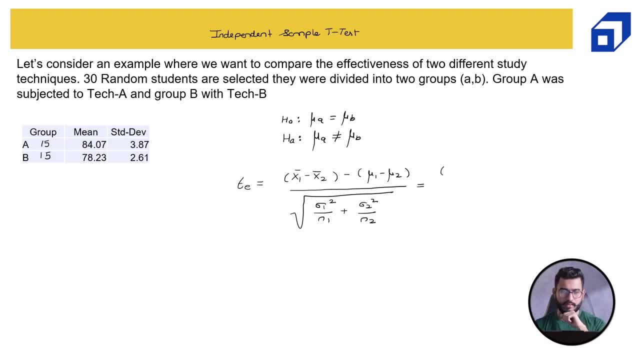 fill that table. fill this formula: Mu1 is 84.07 minus 78.23, minus mu1 and mu2.. So we are assuming that mu1 is equal to mu2.. So this will come out to be zero, Since we are assuming that mu1 is equal to mu2,. 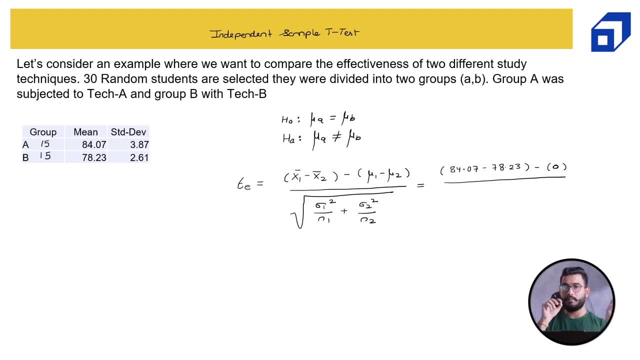 my null hypothesis is that these two average, the population average, are same, So mu1 minus mu2 will always be zero. Then square root of sigma1 square, So 3.87 to the whole square divided by n1, which is 15, plus 2.61 to the whole square divided by 15.. If I solve this, 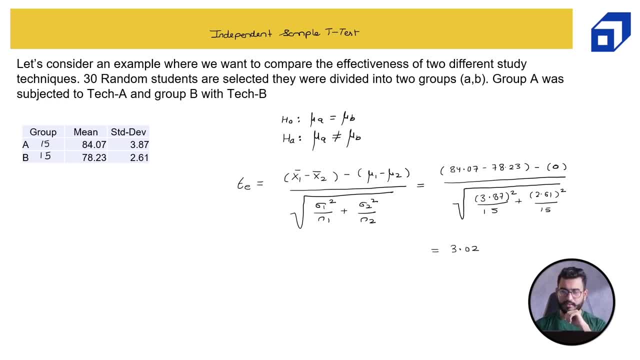 we will get 3.02.. This is my t estimate. Now, this is a two tailed test, right? This is a two tailed test because I'm having not equal to sign my alternate hypothesis. Two tailed test. We have not given with alpha. let's assume alpha to be 0.05.. So this portion will be: 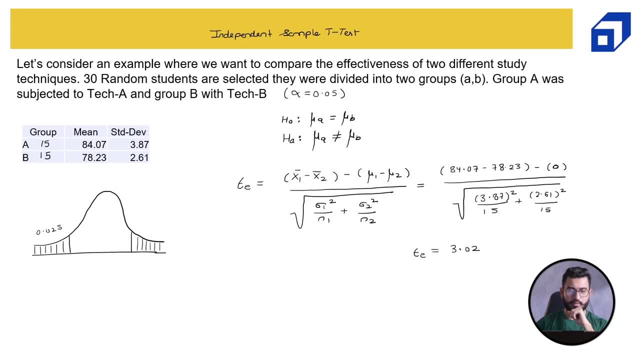 0.025.. This portion will be 0.05.. 0.025 and both are my rejection region. Now I want to find out T critical, which is this point? T critical? Again, we have to use alpha, which is 0.025, and we need degree of freedom. 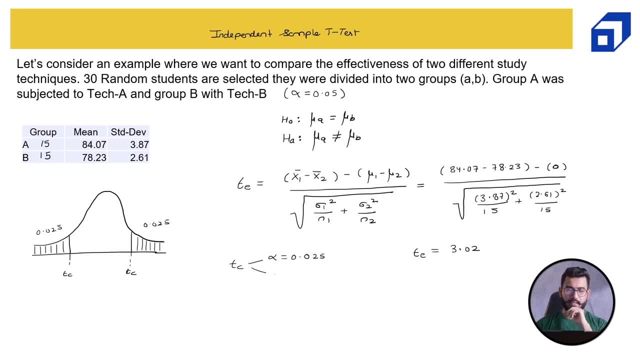 Now, in the case of independent sample T test, the degree of freedom is given as N minus, so degree of freedom is given as N1 plus N2 minus 2.. So my N1 is 15 plus 15 minus 2, which? 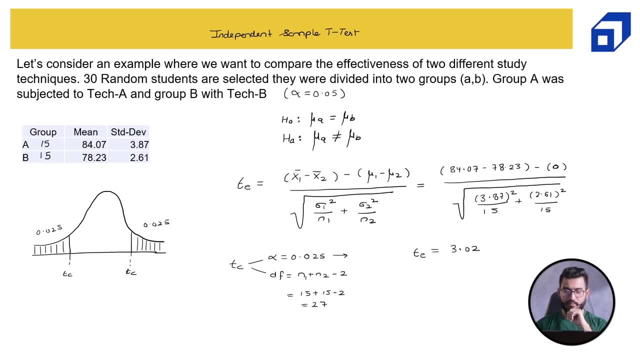 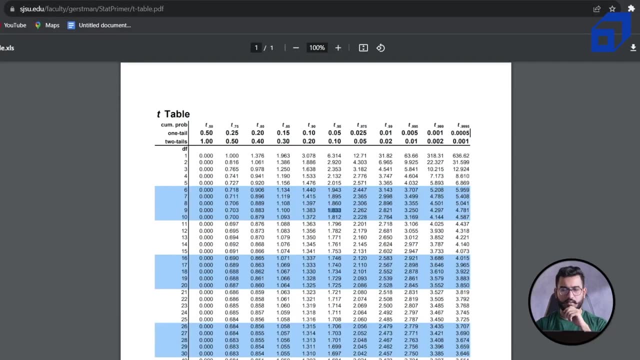 is 27.. So I'll be using alpha 0.05,- sorry, alpha 0.025, T critical as 27.. So I'll be using alpha 0.07 to obtain the T critical value using the T table. Let's do that So. 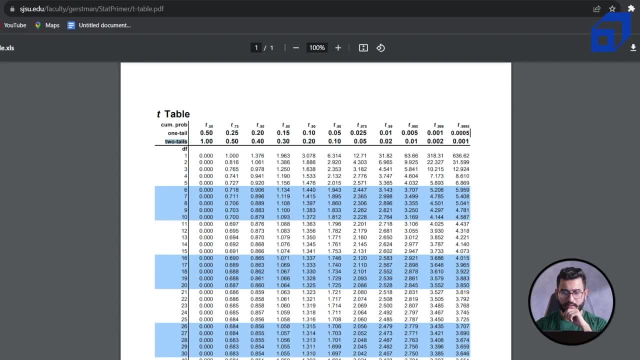 I'm now in the two tail test and we have to look at 0.025.. So two tail test: alpha is given as 0.05, right Alpha is given as 0.05.. We can use. So what is my T critical? 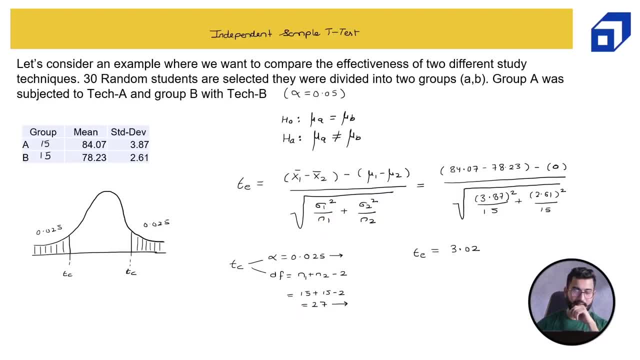 This is what I have done, Since I have divided it by two in my T table. it gives from the left. it gives the T critical value from the left. So if I go with 0.025 from the left, I will get this value. And if I go from this value to this, if I have to find out this, 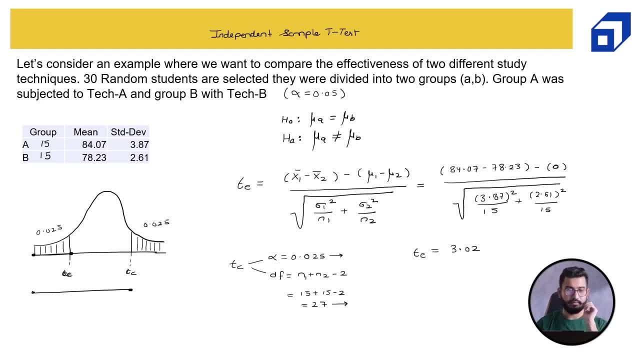 value. it will be 0.05, 0.95.. So let's use one tail test. Or, if you want to use, you can use two tail tests at the alpha of 0.05.. We can use any one of them. For avoiding any confusion, let's use two tail tests at the alpha of 0.05.. So 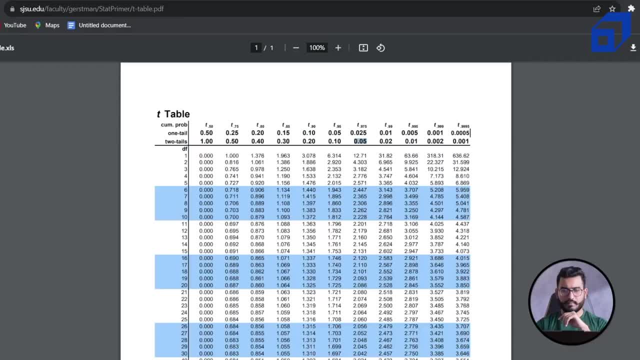 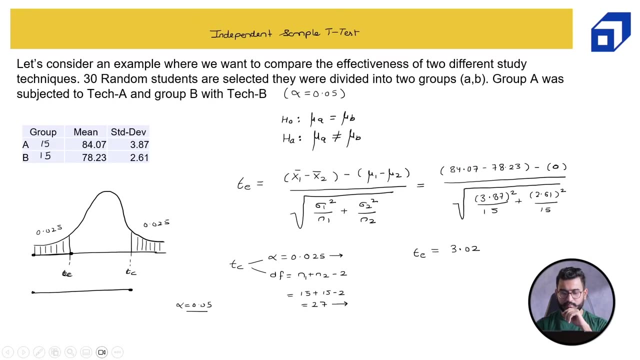 let's look into that. So two tail test alpha is 0.05, and we are given degree of freedom as 27.. This is 2.0, right, So I can use 2.0.. So my decrypt L is minus 2.052 and this will be plus 2.052, right, because always they. 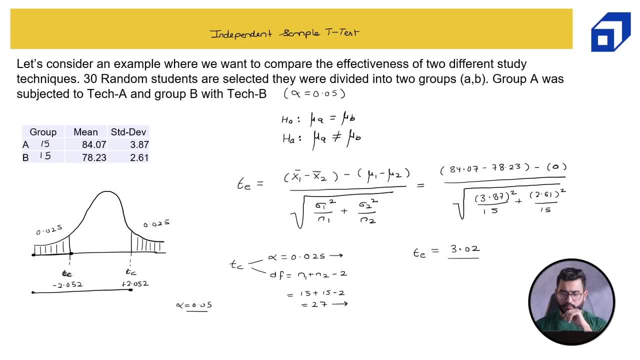 are complementary to each other: 3.02, where this will lie? 3.02 will lie somewhere over here on this rejection region. this is T estimate, since it is lying on the rejection region. we say that we reject null, And when we reject null basically mean they are not same. they. 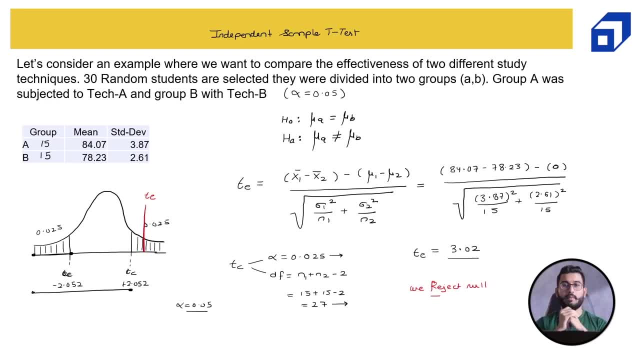 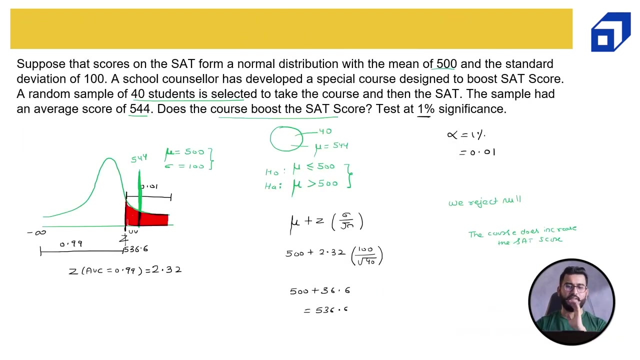 are different. So, based on this particular sample, we conclude that these two techniques are different from each other. So, based on this sample, we reject null. So what to conclude? with the unparalleled, un prevктне C? This is what independent sample ttest is. Now we have completed our discussion on hypothesis. 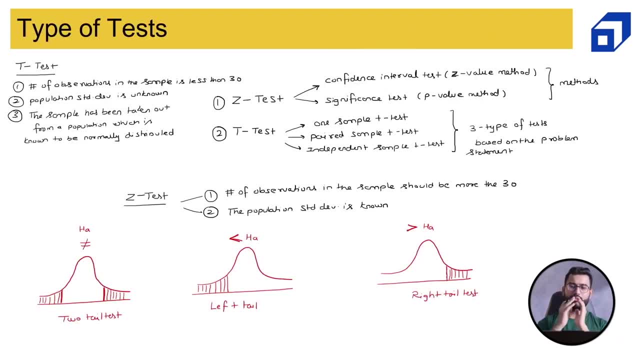 testing. So we are done with the hypothesis test. we now know about quantiting And pink and have talked about how we can perform. So we started our discussion with how to formulate the hypothesis. Then we talked about the two kinds of tests- Z test and T test- Within 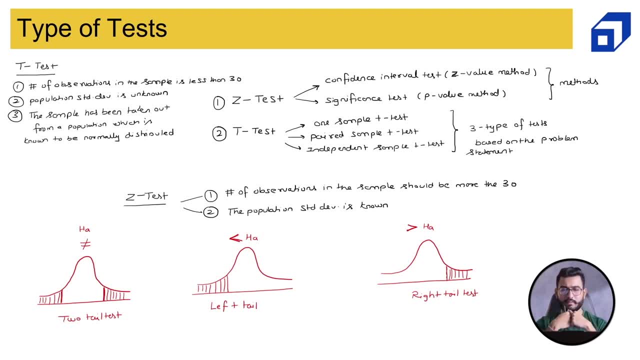 Z test, we looked at two methods: Z value method, P value method. Within T test, we looked at the various types of tests, which are based on various types of problem statements- One sample T test, paired sample T test, independent sample T test- and we solved a variety of. 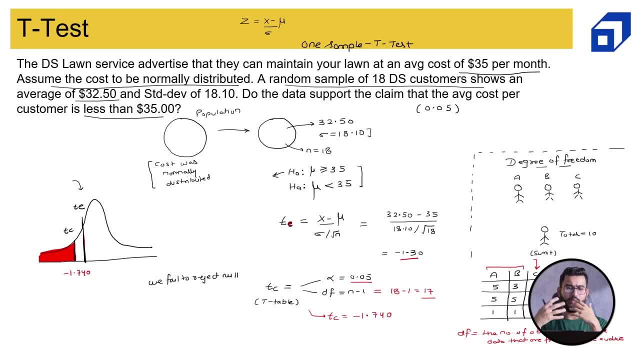 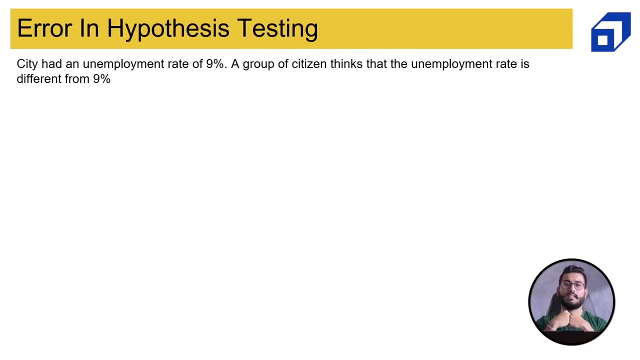 problems, also to make our understanding more concrete. Right Now, we are going to talk about a topic which is known as error in hypothesis testing. As I talked initially that there might be some uncertainty that my test goes wrong, right, Since this is a test which we 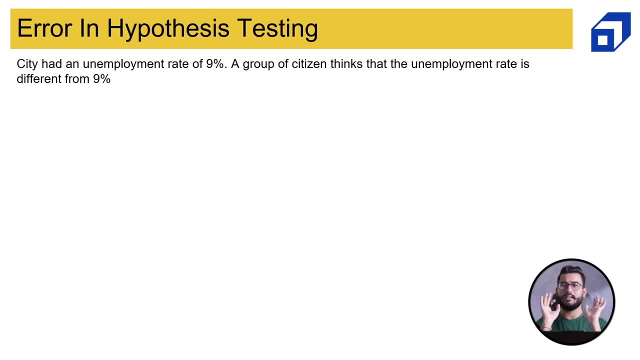 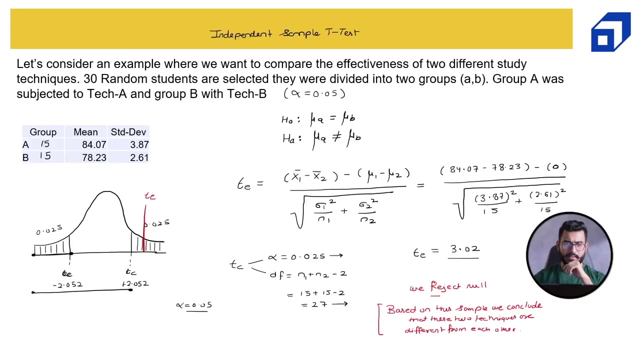 are performing on the sample. we can never be 100% sure that what result my test is providing us or the conclusion that we made from the test is always going to be 100% true. Let's say my test concluded that we reject null. or let's take one example In this particular. 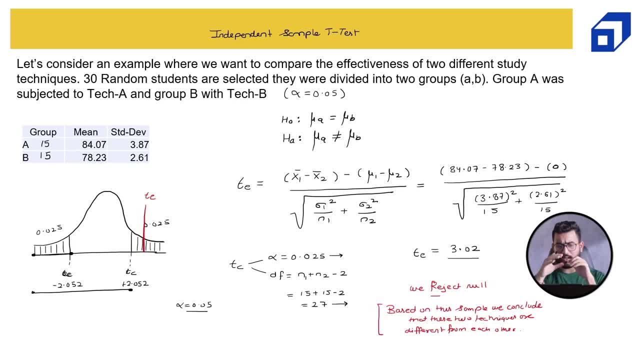 example, we have rejected null right. What if this was actually not true? So, based on these two samples, we concluded that we reject null. But what if, in reality, overall? so, as of now, we have taken a sample of 15-15 students and 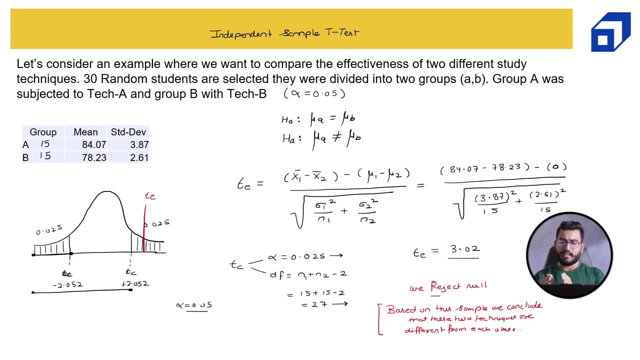 just because of the sample of 15-15 students, we concluded that we reject null. But what if? in reality, if I take a much bigger sample, in reality, this is not true. This is not true. Both techniques happen to be same. 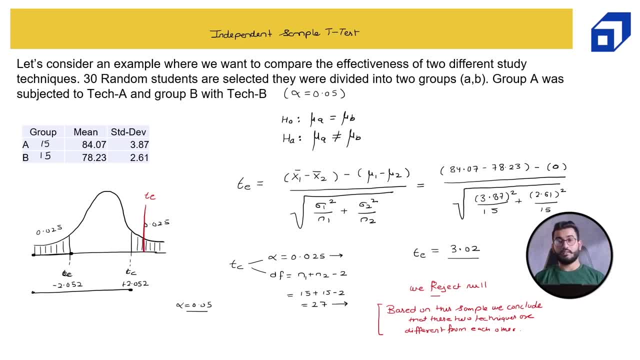 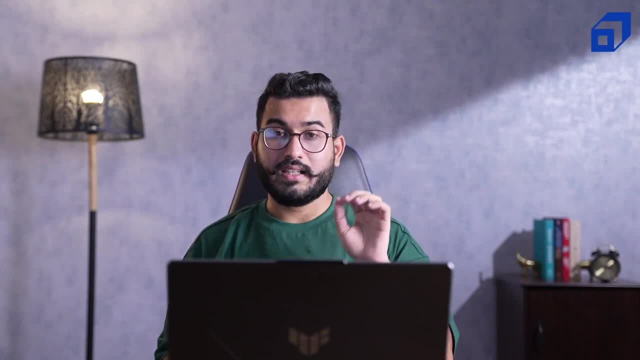 Then that is known as the error in hypothesis testing. So how we can avoid this error? Before we can avoid this error, we have to be very much clear with what kind of error hypothesis testing can lead us, or what kind of errors we can encounter. 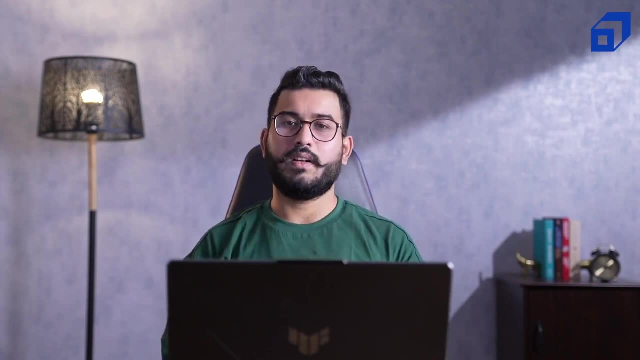 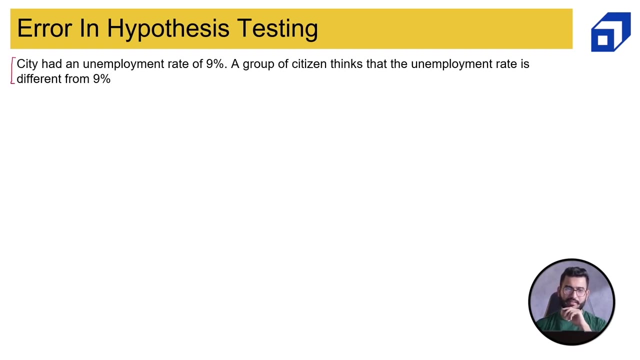 Okay, While performing hypothesis testing. Let's try to understand that now Before we talk about this particular problem. so I have written one condition or I have written one problem statement. Let's try to summarize what are the various errors we can encounter while performing hypothesis. 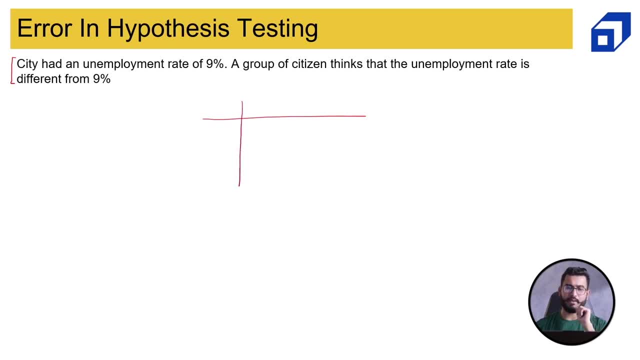 testing So we can summarize the type of error in a two cross, two matrix. This is the reality And this one is the test result, or hypothesis test result. hypothesis test result. Now, there can be four types of scenarios. So, in reality, the null hypothesis was true. 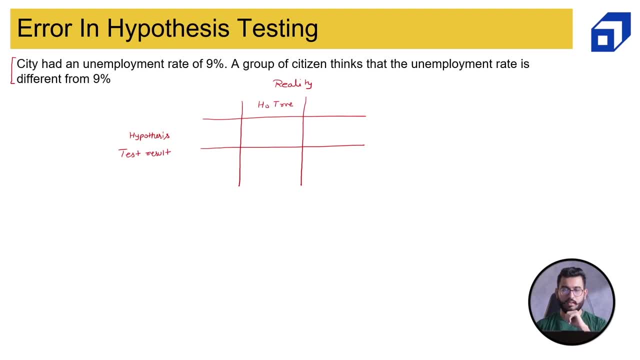 So H naught was true and H naught was false. Here we rejected H naught and we failed to reject H naught. Now, when H naught was false and we rejected H naught, this is a good thing, Right? So this is my correct conclusion. 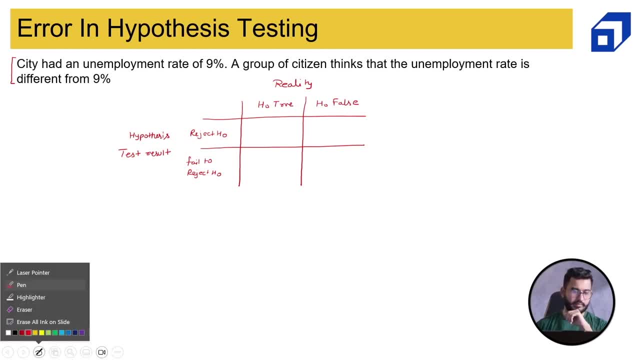 So I'll write correct Correct Over here. This is correct When my H naught was true and we failed to reject H naught. This is also correct Now. where is the error? error is in these two cases, when my H naught was true in reality. 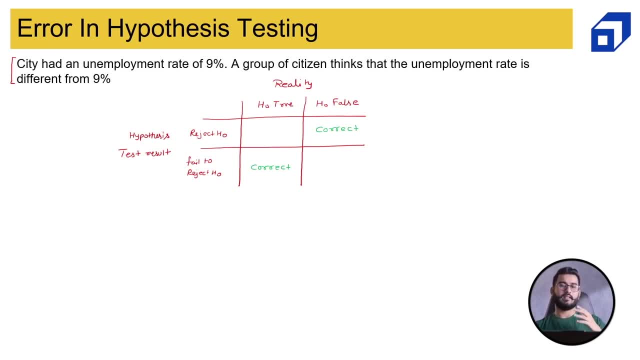 So in reality, let's say in reality, uh, I know that the program is not effective, So in reality, program is not effective, But based on the uh, based on the sample, we concluded that program is effective. So this is a wrong estimation or wrong result. 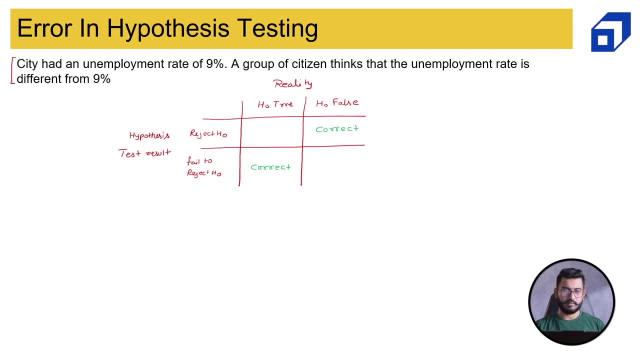 So this is known as the type one error, Type one error, And this is represented by alpha. So alpha, which is area of rejection in all the questions that we have solved, is basically the, So the probability of type one error. What is the probability that I will commit? the type one error is basically given by alpha. 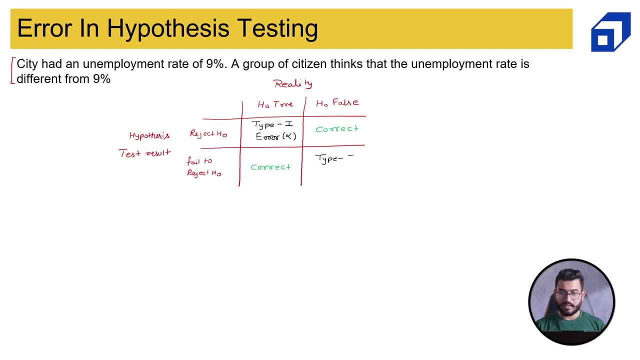 And this is known as the type two error: When your H naught was false. So in reality, my null hypothesis was wrong. So in reality let's say, uh, in reality let's say the program is not effective. So in reality, let's say the program is not effective. 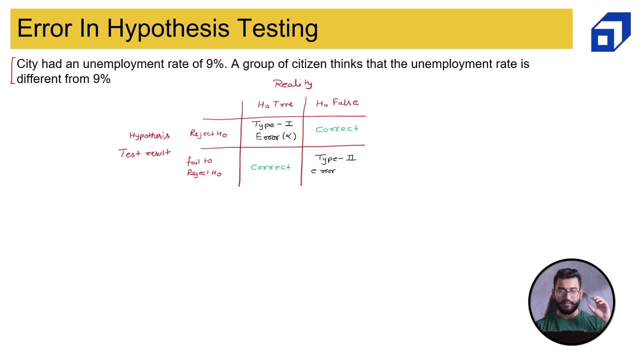 So in reality, let's say the uh. in reality, let's say the program is not effective. reality, let's say: program is effective and we fail to reject H naught, so we concluded that program is not effective. that's a type 2 error if this is. 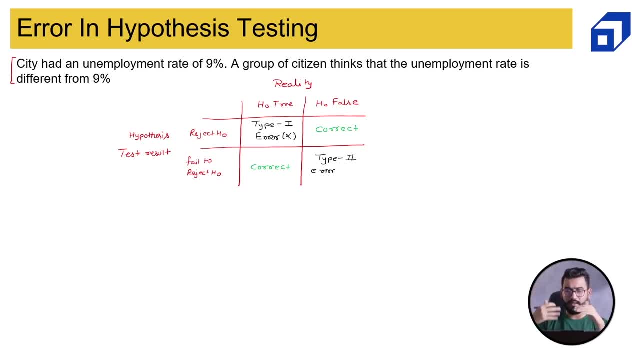 confusing you a lot, don't worry. now let's look into examples. let's look into this example. city had an unemployment rate of 9%. so what is my null hypothesis? my null hypothesis is that the city had an unemployment rate of 9%. group of 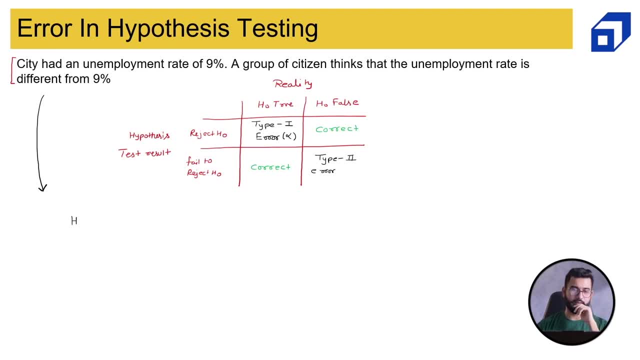 citizen things, that the unemployment rate is different from 9%. so alternate is averages not equal to 9%, null is averages equal to 9%. this is my null and alternate hypothesis. now if I commit type 1 error, then what happens? what will be the case? so type 1 error means H naught is true in reality, but we 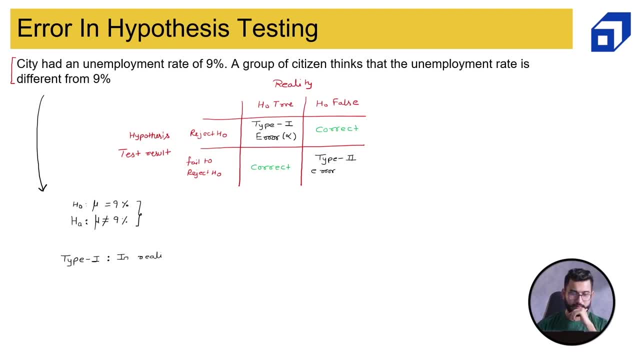 reject H naught. so what is the meaning of this? so, in reality, unemployment rate was 9%, but we concluded that it's not 9%. we rejected H naught, right? what is type 2 error in this case? type 2 error will be that, in reality, 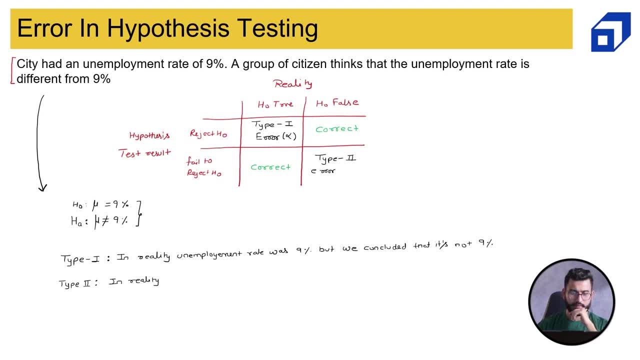 unemployment rate is not 9%. so what is the meaning of this? our solution: we are going to reject H naught, but we concluded that it was not 9%, so we fail to reject null. we fail to reject null means we concluded that the unemployment rate is 9%, but in reality, 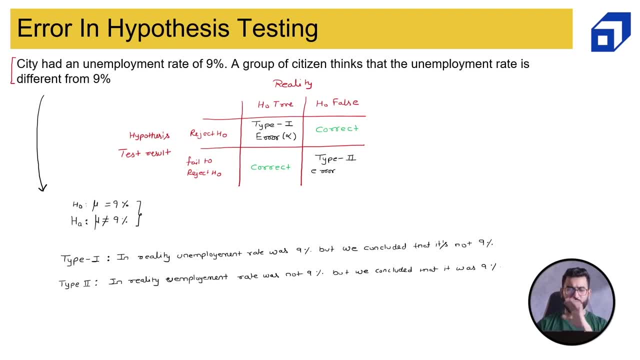 it was not 9% now, as of now. I am NOT talking about a which one is good, which one is bad. I'm just talking about how to identify the type 1 and type 2 error. Just remember that you have to just keep this particular table, or this: 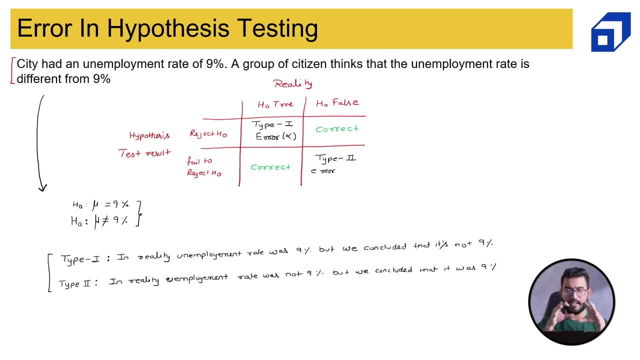 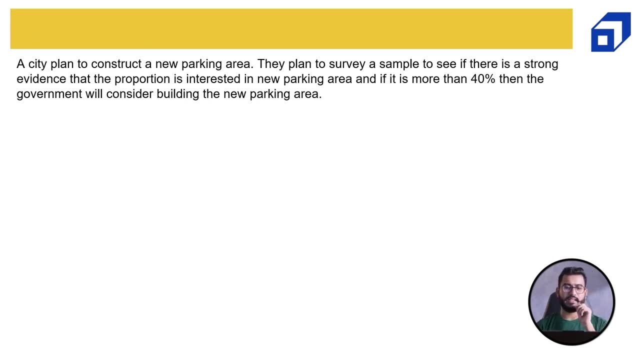 matrix in your head so that you can formulate type 1 error and type 2 error. Let's take one more example. A city had a city plan to construct a new parking area. They plan to survey a sample to see if there is a strong evidence that the proportion is interested. 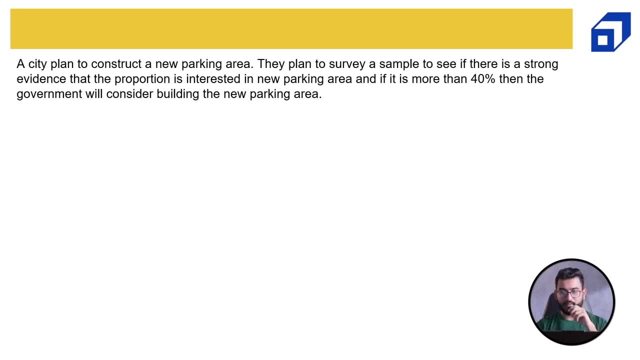 in new parking area. If it is more than 40%, then the government will consider building a new parking area. So the if, the if the proportion. so let's say, government has taken a sample of different, different individuals from the population And if this sample results, 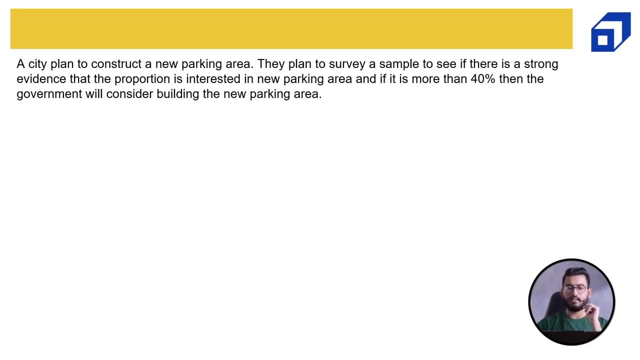 in 40% of the parking area, then the government will consider building a new parking area. So let's say 40% of the people in the sample are interested in the new parking area in the city. Then the government will propose a new parking area in the city. So what is? 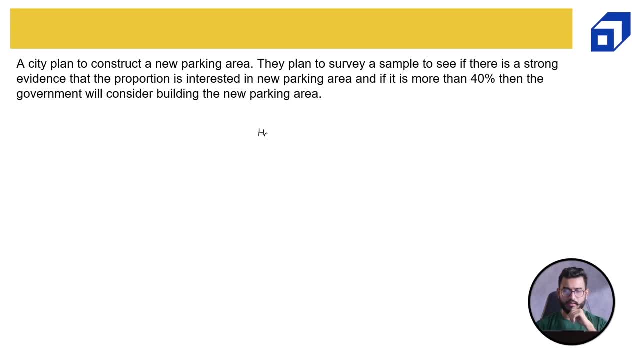 the null and alternate hypothesis. So my alternate hypothesis is that the average is greater than 40%, because this is what we were trying to prove. Null is the average is less than or equal to 40%. Okay, So initially, my assumption is that no one is interested. My initial assumption is no. 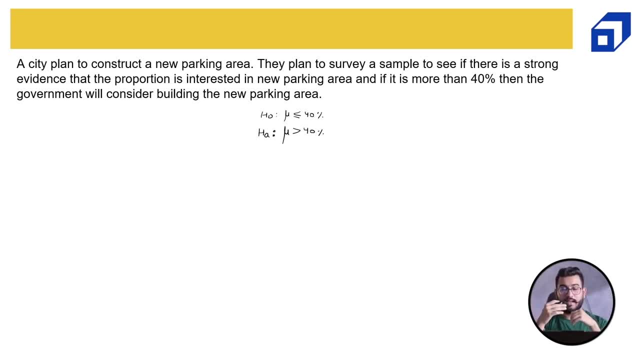 one is interested. I'm trying to prove that. uh, more than 40% people are interested in the sample. Now what is my type one error? Type one error is basically reject H naught, actually true, actually true. So type one error will be: uh, reject H naught, We will. 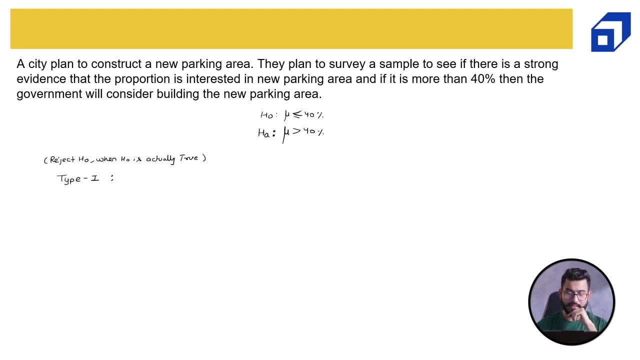 reject. H naught basically mean uh. we concluded that. we concluded that more than 40% people in the sample are interested in the new parking area. So that's the null and alternate hypothesis. But I think if the number of people in the sample or in the population are interested, 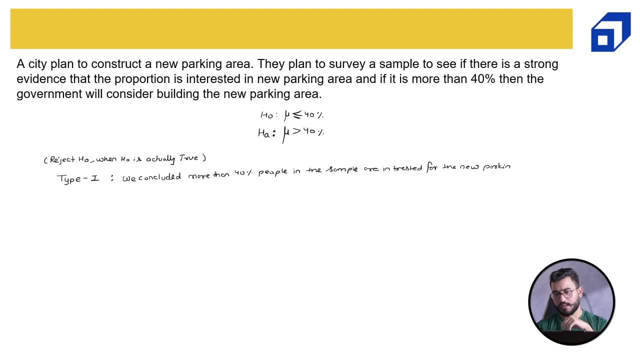 for the new parking area, while in reality, I'm going to convert it to null, and then we'll get an answer to some of these problems. A new parking area, A new parking area in the city? Yes, I'm going to convert this to null. 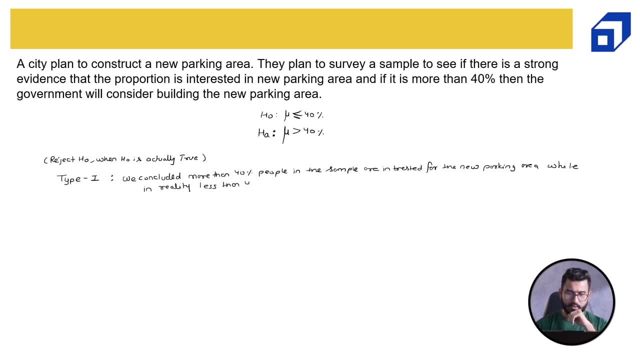 Okay, 40% people were interested. So this is my type 1 error. What is type 2 error? Type 2 error is basically we fail to reject H0. fail to reject H0 when H0 was actually false. So what is our? 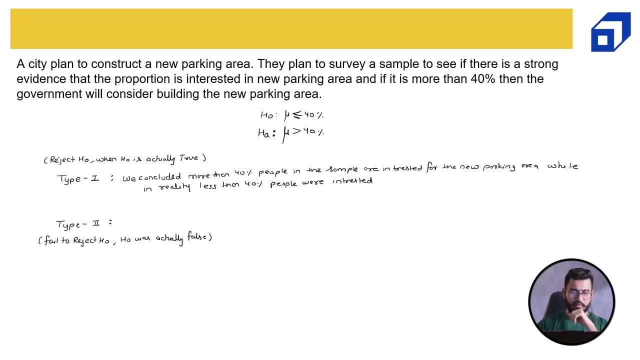 conclusion: for this, We fail to reject H0.. So we concluded: we concluded that less than 40% people are interested for the new parking area, for the new parking area, while in reality, in reality, H0 was actually false. So, in reality, more than 40% people were interested. 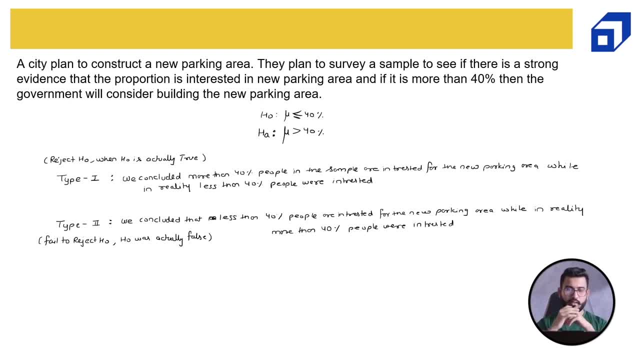 Now, if I ask you, if let's say you are a government body and you are performing this test, which particular error is more problematic for you as a government body? Now, if I ask you, if let's say you are a government body and you are performing this test, which particular error is more problematic for you as a government body? 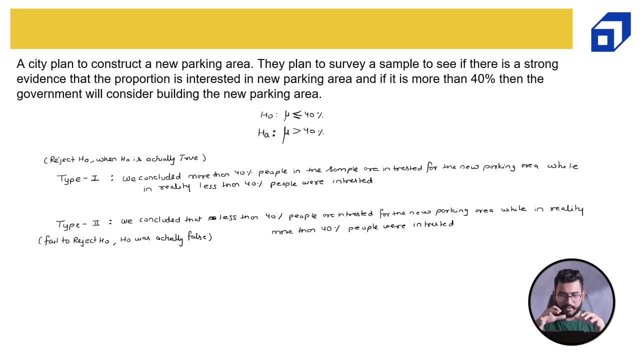 Now if I ask you, if let's say you are a government body and you are performing this test, which particular error is more problematic for you as a government body? As a government body- type 2 error- you can see that it is problematic for us because we have concluded that less than 40% people are interested in the new parking area, which basically mean we will not build the new parking area. 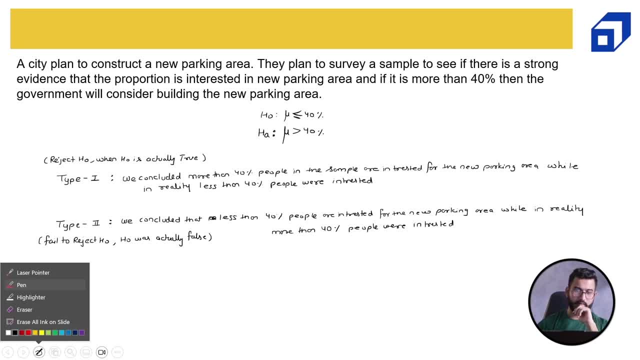 So the consequence of the type 1 error would be: government will choose not to build the new parking area. So the consequence of the type 1 error would be: government will choose not to build the new parking area, to build the new parking area when it was actually required. So what is the end problem for this? or? 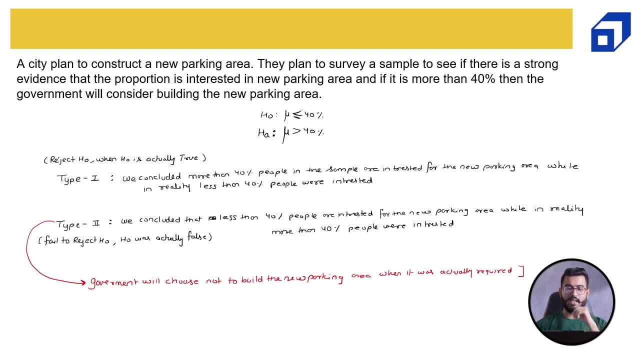 major consequence that will happen to the government. Well, people will not be happy with the government right. So people will not be happy with the government right. What is the consequence of type one error? Now, the consequence of type one error is that the government will build a new parking area. 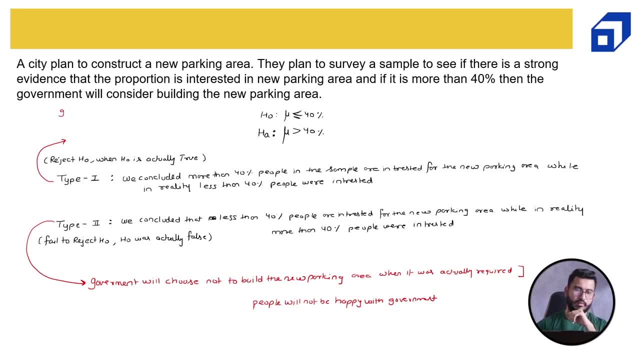 when it is not required. So government will end up building the new parking area when it is not required, And what is the consequence that government will be facing? Government will be investing some unnecessary amount from their budget in building up this new parking area, which will impact their budget. 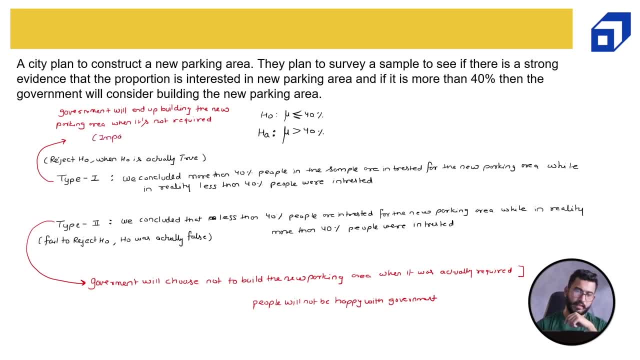 So impact in their budget. Now, as a government body, you need to decide which particular error you want to reduce Because, see, since we are doing hypothesis testing, since we are doing estimations, we can not be free from error. There will be some kind of error, but you have to decide which error you are ready to. 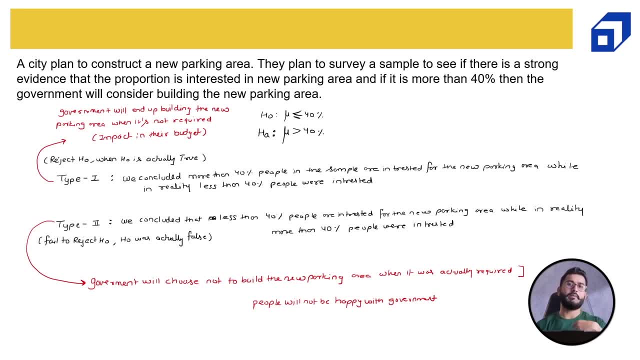 bear or which error is less problematic for you. So if you are a government body, you have to decide whether you are ready to face the impact in your budget or whether you are ready to face that people will not be happy with you. Well, if I would be a government, 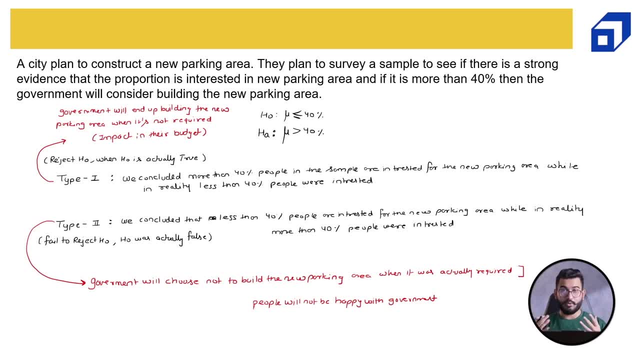 I would not be taking up the type two error on me, because I want my people to be happy, So I would do something with the budget. I would try to maybe cancel some ongoing projects or maybe cancel some new projects, but I don't want my people to be unhappy with the government. 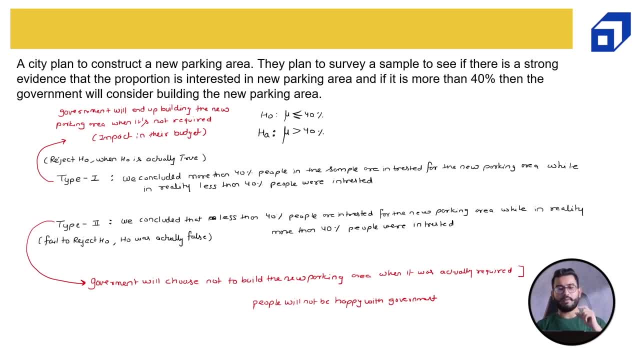 Right. Let's take one more example to understand how we can adjust the alpha. because we know the alpha value right, We can do the alpha value. We can increase or decrease the alpha value to increase the chances of type one error and reduce the chance of type two error. 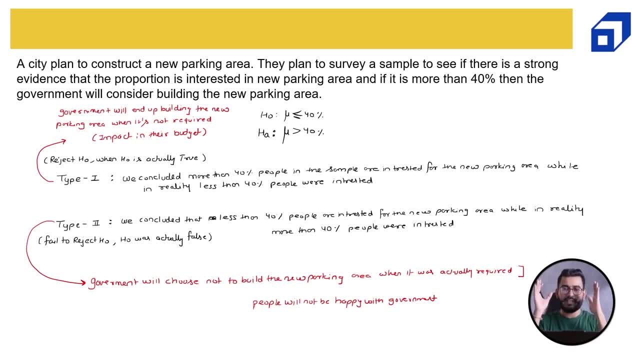 You can, you can assume that, uh, if we are, if I'm having a number line, then if I want type one error to be high, I can increase the value of alpha and it will eventually reduce the type two error, the chances of type two error. It is like a number and you. 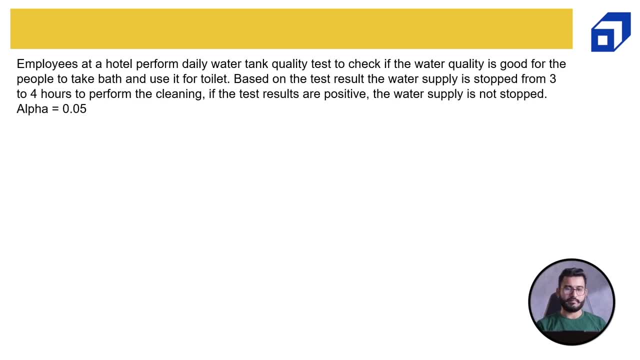 can shift it. Let's see one last example. So employee at a hotel performed daily water tank quality test. Okay, Okay To check if the water quality is good for the people to take bath and use it for toilet. Based on the test result, water supply is stopped for three or four hours for the to. 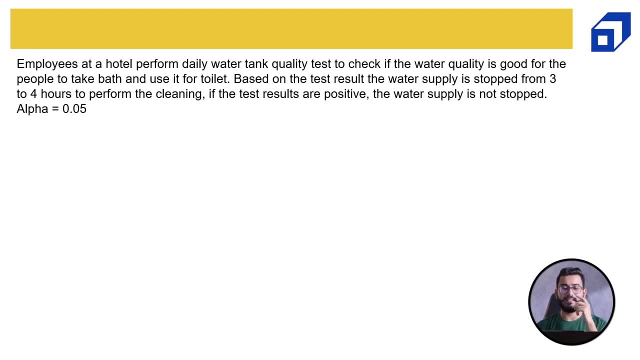 perform the cleaning process or for the cleaning process, If the test results are positive, the water supply is not stopped. Test at alpha of 0.05 and this question: we are provided with the alpha of 0.05.. What is the alternate hypothesis? 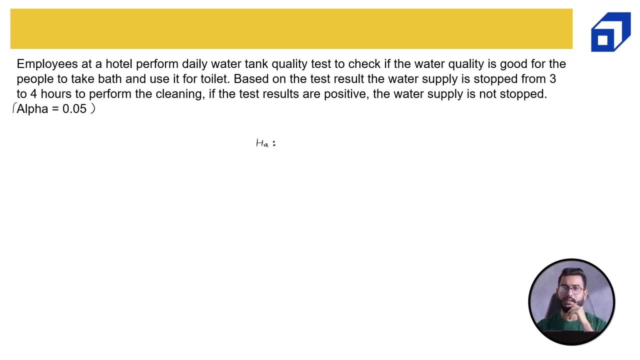 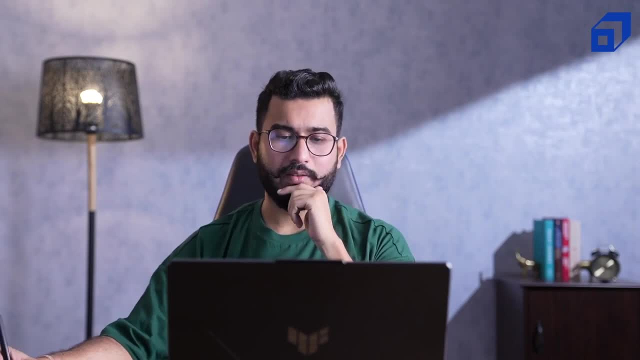 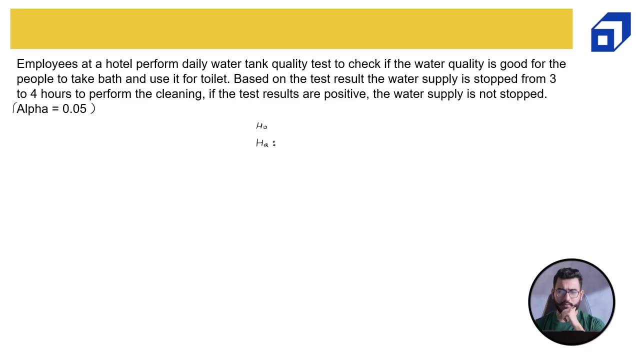 Let's- uh, you guys can pause the video, think about it and then you can maybe comment on the chat section. So now let's try to understand this question, And I hope you guys would have already guessed what is going to be the alternate and the null, null hypothesis, My null hypothesis. 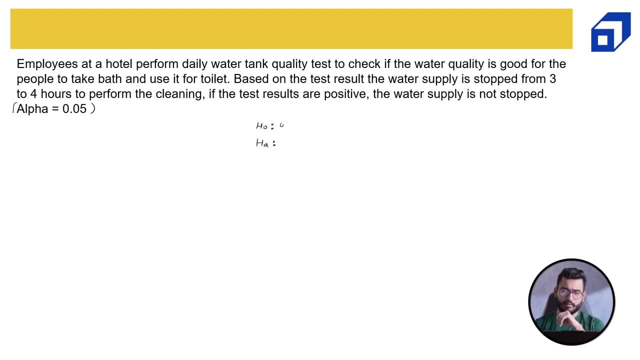 would be that the water quality is fine, So water quality is fine. It's good, Fine or good. So my null would be sorry. My alternate would be: Water quality is not good Right Now. what is the type 1 error? The type 1 error is basically: 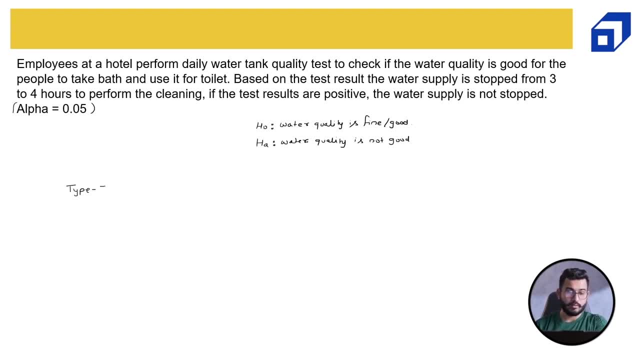 that we reject H naught when it divorce. So let's write it down: We reject H naught when it divorce. Okay, when H0 was actually true. in reality, right? So what is the meaning of this? We reject H0.. So we rejected that water quality is fine when H0 was actually true. So what will happen? 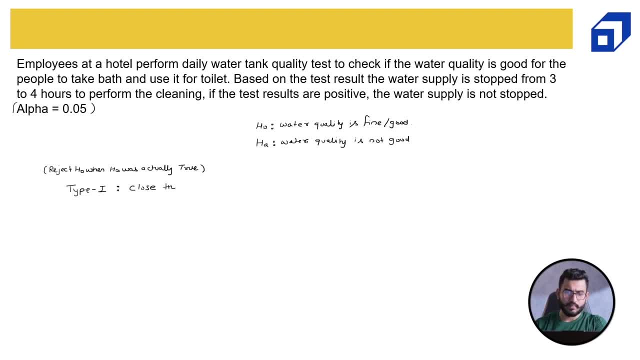 So we will close the close the water supply. We will close the water supply when it was not required, right? What is type II error? Type II error is we fail to reject H0, we will close the pool when H0 was actually false. So what will be the consequence for this? 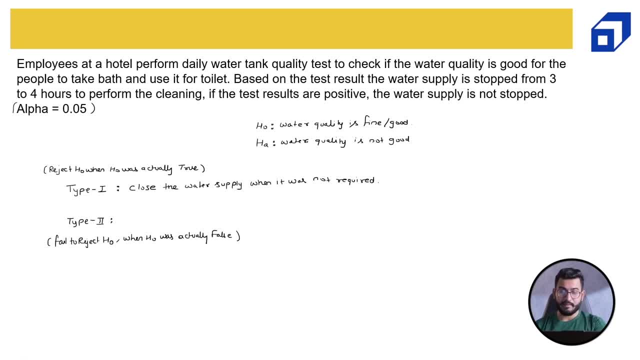 So we failed to reject H0.. So which basically means we concluded that the water quality is good when H0 was actually false. So that basically means we will not close the pool, or we will close the pool, We will not close the water supply, or maybe we let's not write. we let's write the water. 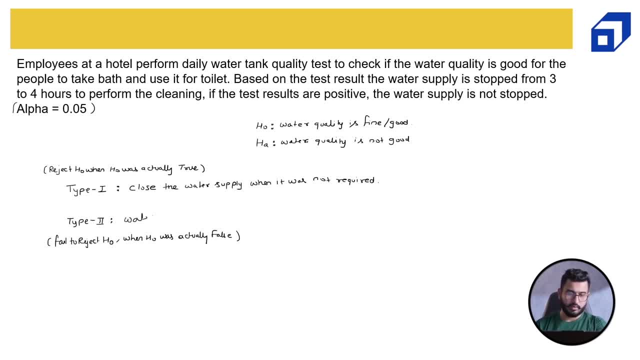 supply was not stopped. Water supply was not stopped when the water quality was bad. Water supply was bad or not good. Now which one is more problematic? So if you are a hotel owner, then which one is more problematic for you? So if I go with the type, I error. 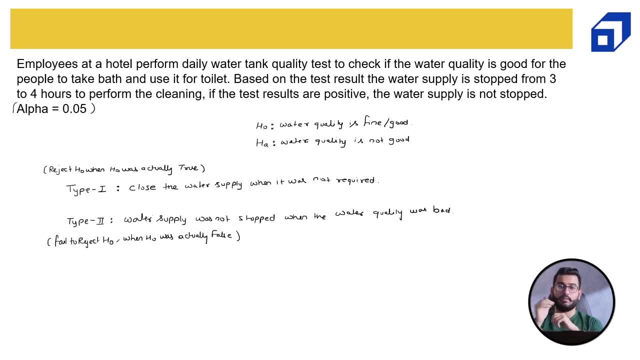 we have to close the water supply when it was not required, which basically means we will clean- or your, your employee, or the, maybe your, the, the, the people who clean the tank. they will perform the cleaning process, but there will be a stoppage of water. 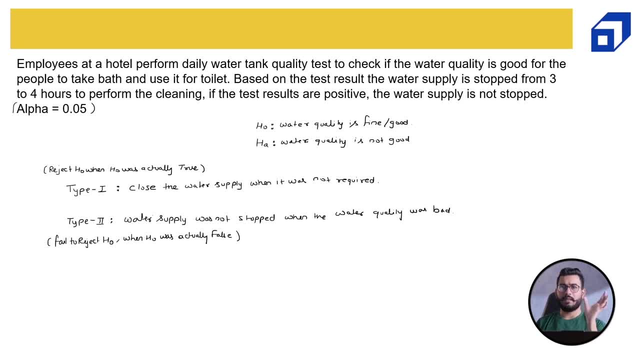 supply for three to four hours. Maybe this is not a big problem because maybe you can decide the window of afternoon and then the water supply can be stopped for three to four hours and it will not impact the service Right. So when you have to stop the water, 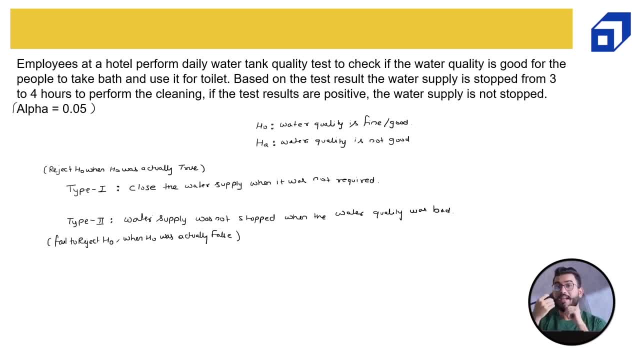 supply, you have to also think that it may impact the service, Right, So when you have to stop the water supply, you have to also think that it may impact the service, but it will eventually not going to harm you in a very large scale because you can choose. 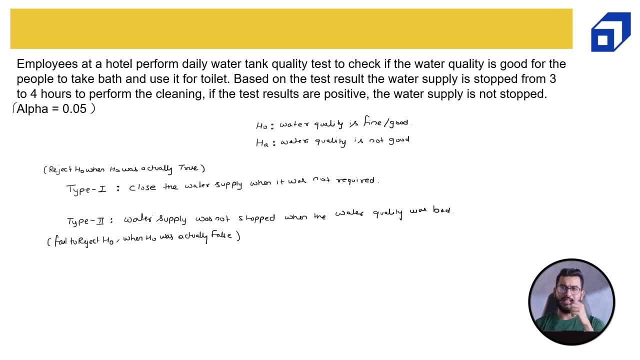 the window in the afternoon, when most of the people are either out of the hotel or maybe involved in some other activities, they would not be using the the bathroom right. What is the consequence of type two error? Water supply was not stopped when the water quality 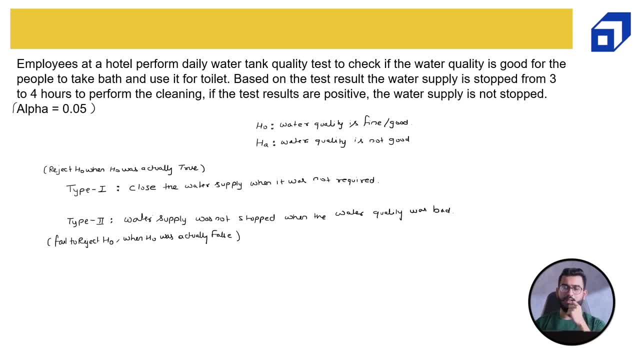 was bad. Now this is a mode problem. Let's say somebody is having a sensitive skin and that person is staying in your hotel And if you do not clean the water- and let's say that person has taken bath in the contaminated water- the person can attract some kind of disease which can eventually land your hotel. 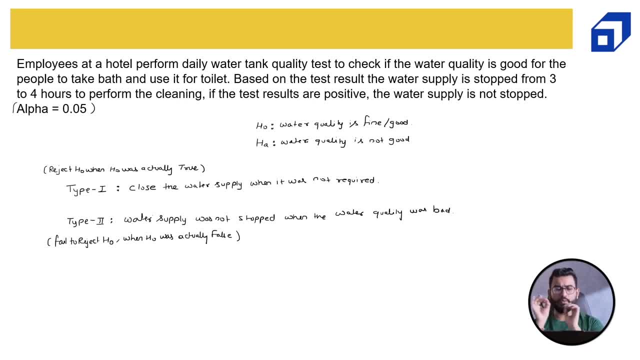 into a big problem, right? So type two error is definitely very problematic for you. Now we have already learned that water supply is not going to affect the service, Right? So we have learned that alpha is the probability of type one error. So alpha is the probability. 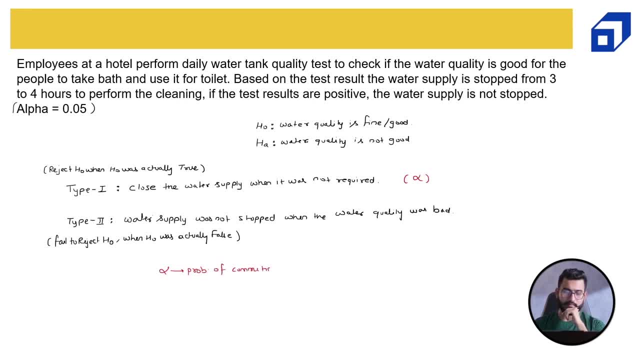 of committing type one error. So now, if I increase the value of alpha, there are more chances that I will commit type one error, but it will reduce the chances of type two error. So right now my alpha value is going to be less than or equal to type two error. So 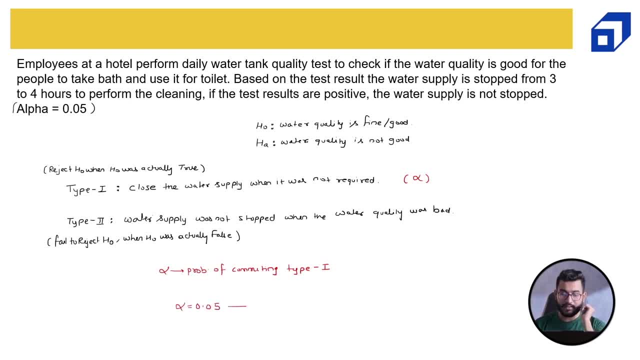 my alpha value is 0.05.. If I increase this to 0.10, then what happened? I increased the probability of type one error, So let's say this is type one error. I increased the probability of type one error, So it will reduce the probability of type two error, And this is what you should.